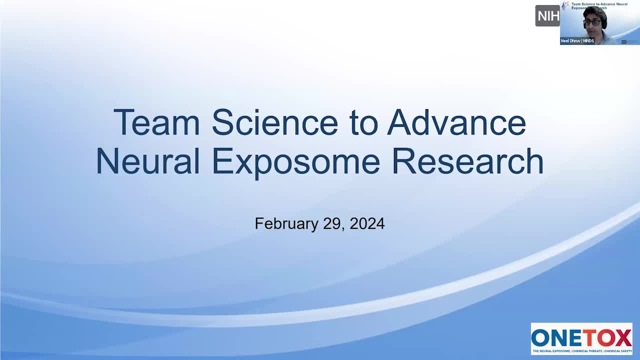 Her research focuses on mechanisms by which environmental stressors, including persistent organic pollutants, organophosphorus cholinesterase inhibitors and air pollutants, influence neurodevelopmental seizure and neurodegenerative disorders. She serves as Director of the UC Davis Counteract Center of Excellence and Co-Editor-in-Chief of the Elsevier Journal Neurotoxicology. 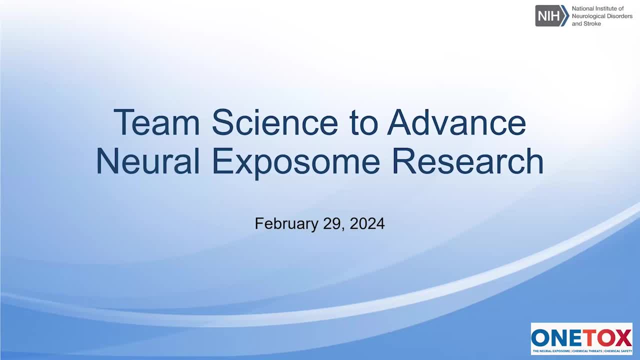 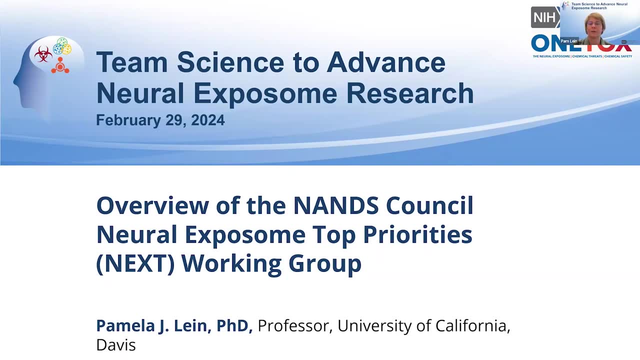 Pamela Line. Thank you very much, Neal. I think there should be another slide coming up here. Great thank you. So it's my extreme pleasure to be here. I'd like to kick off today's mini-workshop, which is part of a larger initiative launched by the NINDS to really determine how to move forward with integrating neuroexposome research into the NINDS mission space. 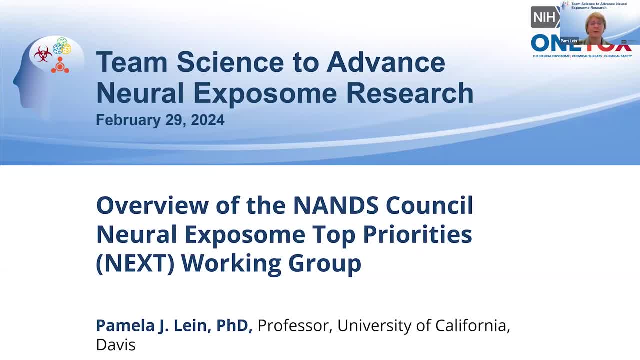 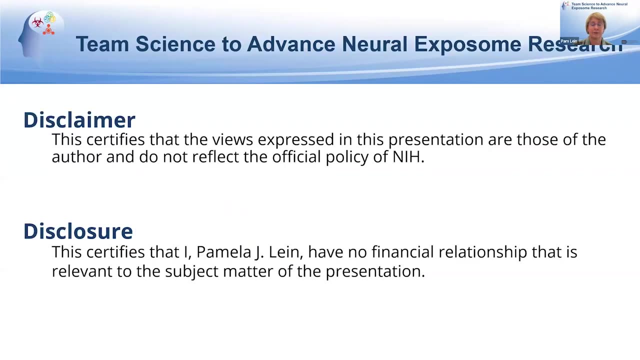 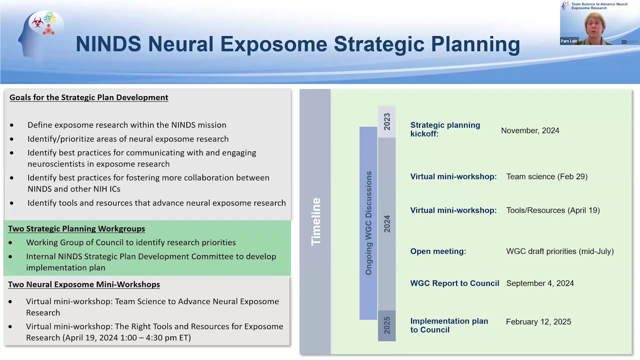 And so I will give a quick review of the NANDS Council, which is basically meeting over a year to do some fact-finding on. what do we know about the neuroexposome? what are significant research gaps in this field in the context of the NINDS mission space? and at the end of this we're hoping to put together a report to the NINDS with recommendations on research priorities- research gaps in the space of the neuroexposome as it pertains to the NINDS mission state. 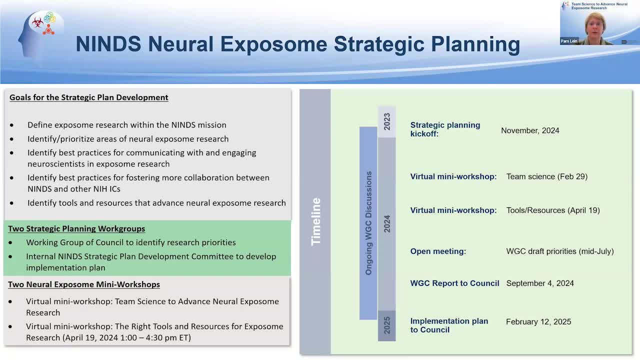 So what you see in this slide here is the strategic planning schedule, if you will. And so we have a number of goals for the NINDS strategic plan development. The first is that we really want to define exposome research within the NINDS mission, as I previously alluded to, And the goal of the working committee is to identify 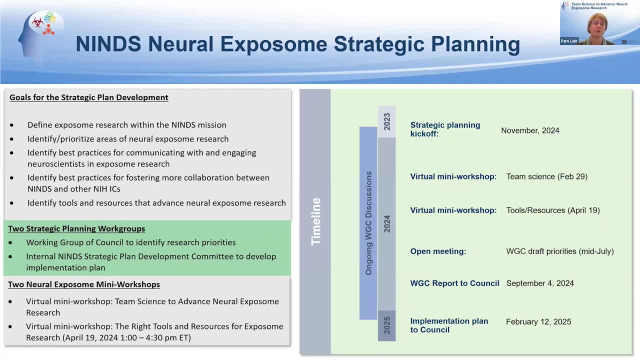 and prioritize areas of neural exposome research. We're also hoping to identify best practices for communicating with and engaging neuroscientists in exposome research, which is a new area for many people in neuroscience, And so one of the goals is to determine how do we encourage people. 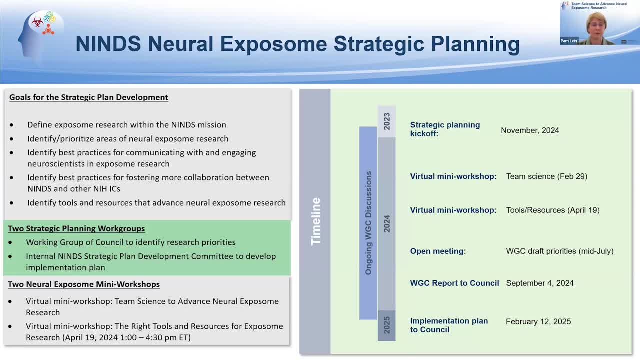 who don't have expertise in the exposome to start engaging in this type of research. And then also, we would like to identify best practices for fostering more collaboration between NINDS and other NIH ICs and, I would say, perhaps other funding agencies that have 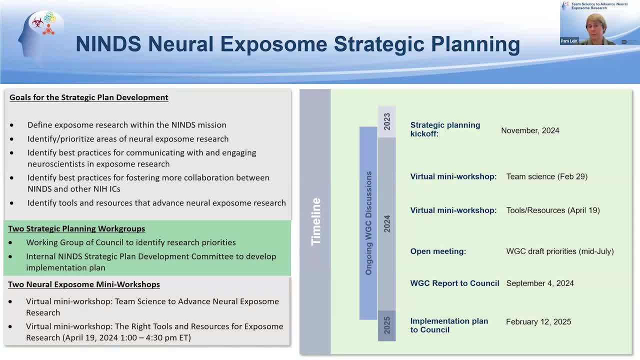 expertise that pertains to exposome research, for example NSF. We also are hoping to identify tools and resources that advance neural exposome research. I suppose one thing I should have said at the beginning, but I think Dave is going to say it. I think Dave is going to say it. 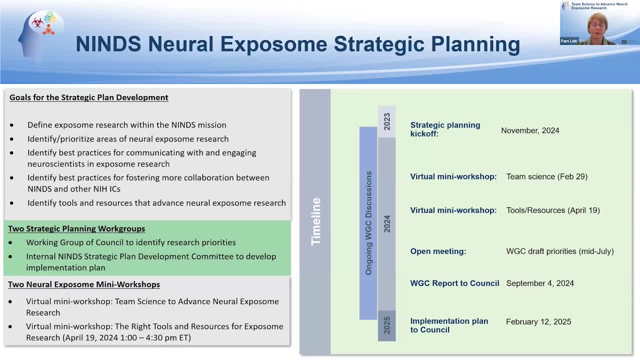 Dave is going to talk about this more. David Jett is. there is a great deal of interest in really moving NINDS into the area of exposome research because of the fact that I think we're all aware now that we really in order to make a lot of progress in a number of neurological disorders. 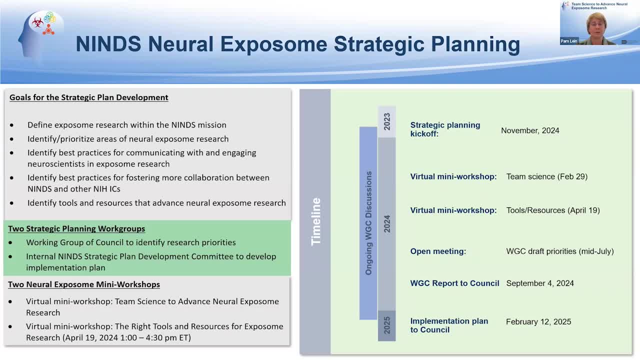 need to understand the entire environment and how it's interacting with disease processes and with resiliency to determine outcome at the level of the individual, And so that is the goal of looking at this field of exposome research in the context of neurological diseases. 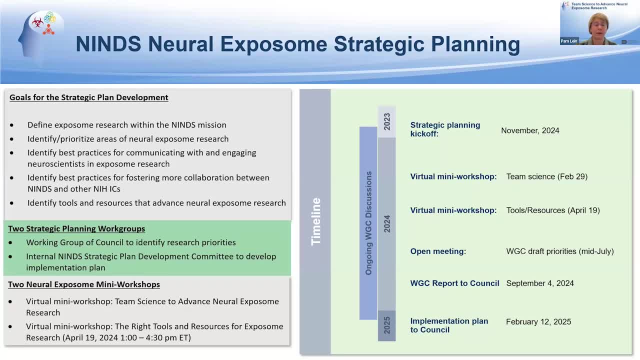 So there are two strategic planning workshops. I am chairing the working group of council to identify research priorities and there's a number of experts across different sectors in NINDS mission space that have been brought together to address this issue And then, following our 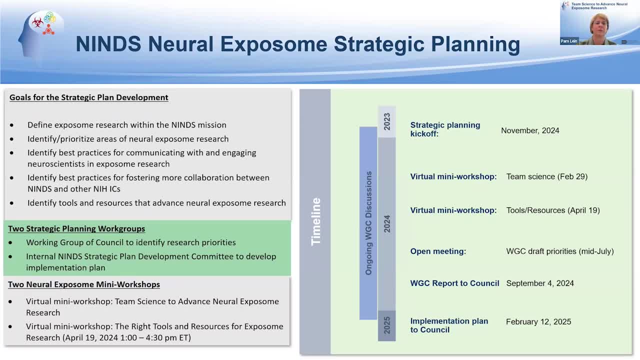 report to the NINDS. there will be an internal NINDS strategic plan development committee that will develop the implementation plan, And so, as part of our fact-finding mission, we have worked with the NINDS staff to organize two neural exposome mini-workshops. This is the 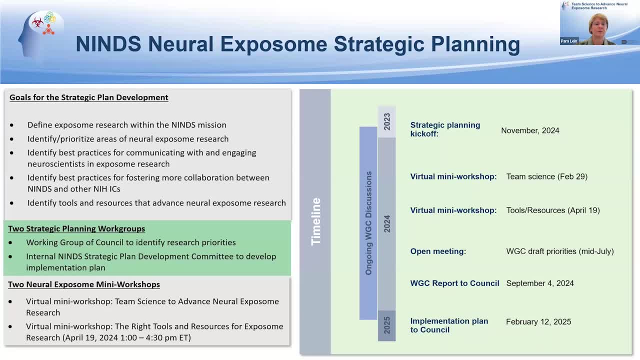 first of those two, which is to really focus on team science to advance neural exposome research. The exposome, by definition, involves many diverse sorts of data streams being integrated to inform effects at the level of the whole organism, And so by its own it's a very, very, very very. 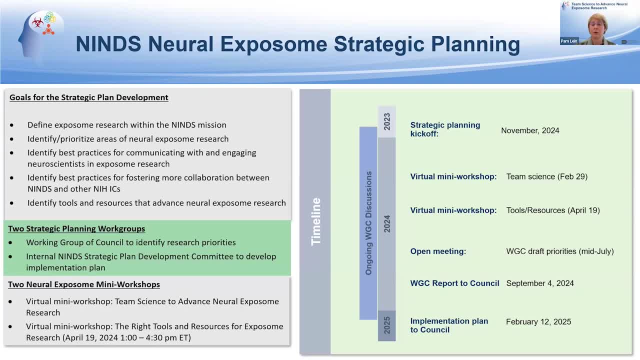 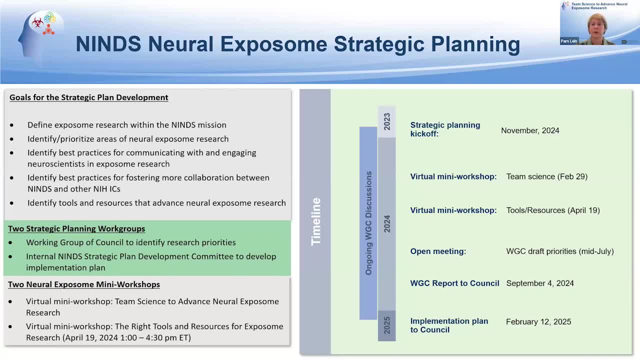 really integrate the exposome research field into classic neuroscience research, And so that is really the goal of today's workshop is to determine what are best practices in team science. Are there any unique aspects of the exposome research involving team science that the working? 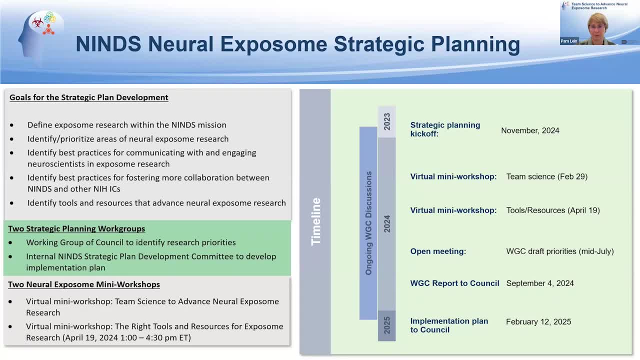 group of council should be aware of as we start to form our recommendations to the NINDS. There will be a second mini-workshop, which will be focused on tools and resources that are available for exposome research and, importantly, identifying gaps in the tools and resources that would be. 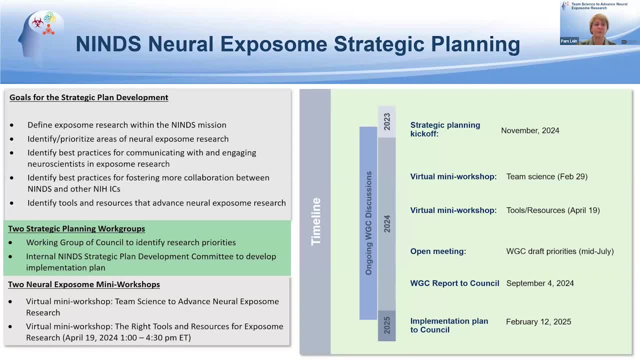 needed to really advance research in the neural exposome. So you can see that is scheduled for April 19th and we hope many of you will be able to join us for that as well. But again, the goal of these mini-workshops is to really provide information to the working group of 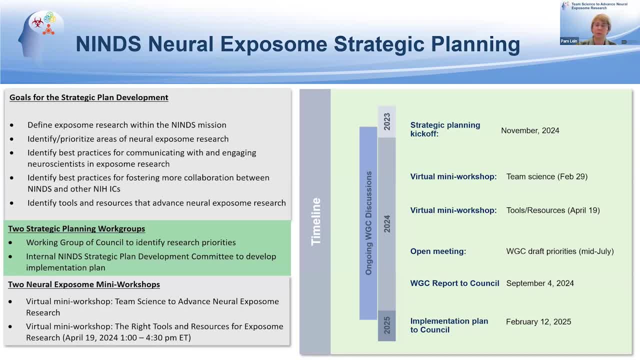 council to help us form our research priorities. in the report that we'll be providing to the NINDS, The timeline for these activities are shown on the right of the slide. So we had our strategic planning kickoff in 2023, and then, through 2024, we've had a number of meetings of the Working Group. 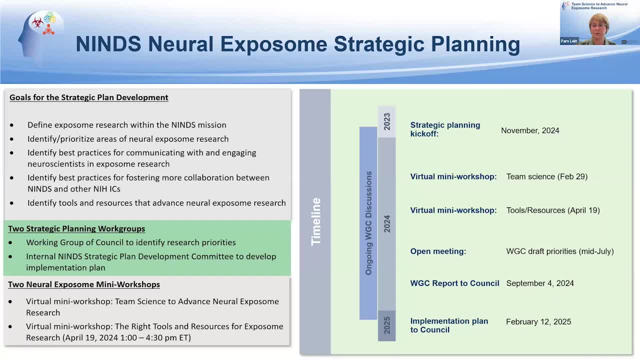 which has been divided into three subcommittees, and then we all meet back together to share the outcomes of the subcommittee research and we have the two virtual mini-workshops. So we're hoping to basically have an open meeting to discuss where we are in both the material and the doji project. 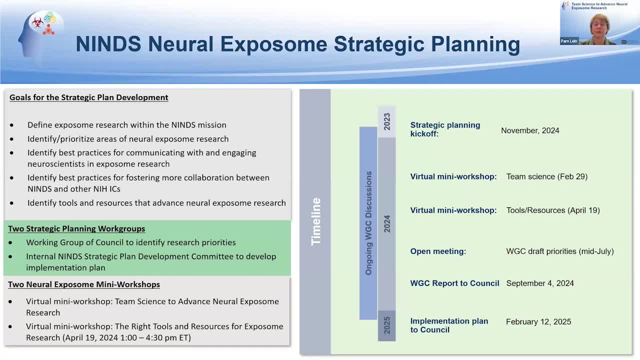 the research priority draft that the working group puts together sometime in mid-July so we can invite public feedback on that and then to finalize our report to Council in September of 2024.. And then the goal of NANDS is to have an implementation plan to the Council by February. 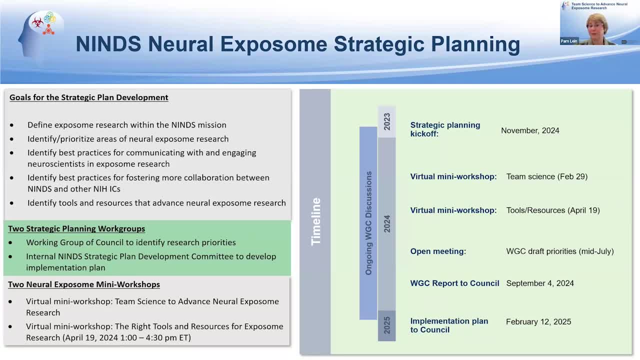 of 2025.. So hopefully we'll have lots of great input today to inform our decision-making and encourage all of you that are engaged in today's workshop to reach out to any of the members of the working committee and that's published on the NANDS workshop with any recommendations you. 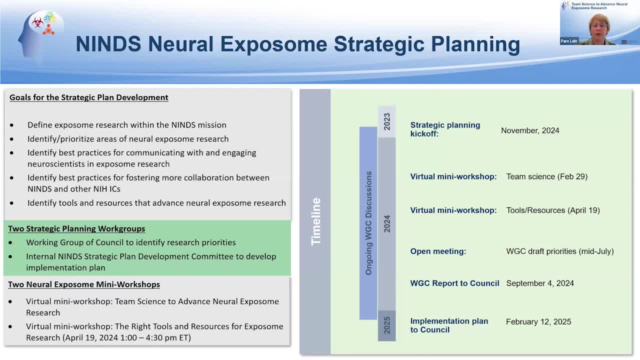 might have following today's mini-workshop, And with that I will turn it back over to Neil, Thank you. Thank you very much, Dr Line. I don't see any questions, so I'd now like to introduce Dr David A Jett. 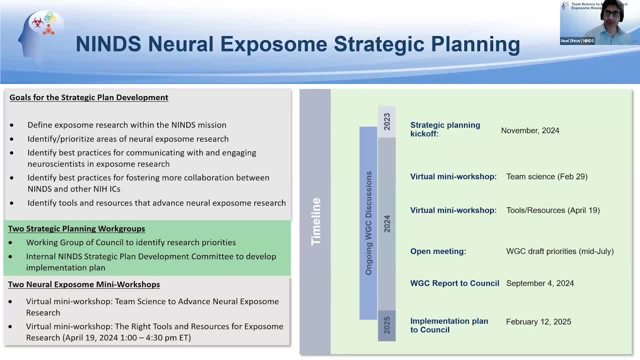 David Jett, Director of the Office of Neural Exposome and Toxicology at NANDS. Dr Jett's scientific interest is in the impact of chemical agents on nervous system function, including the molecular and cellular mechanisms of cognitive and neural development. Dr Jett has served on 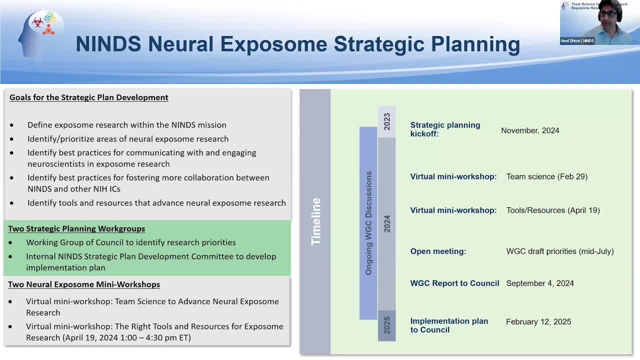 White House and intergovernmental committees that set the nation's research priorities, as well as science advisory panels for the Environmental Protection Agency and the Department of Defense. Dr Jett, Thank you, Can you hear me okay? I just wanted to say there's a typo up there: November 24th should. 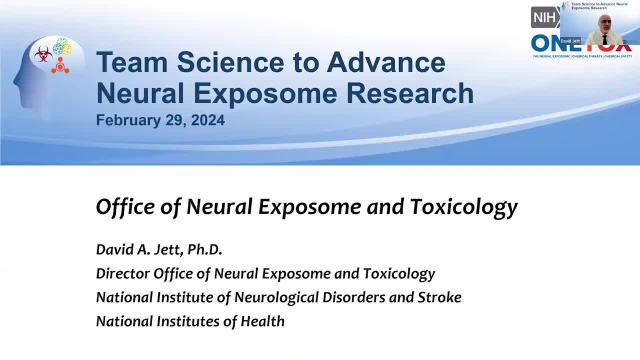 be 23rd, obviously, So, yeah. So, first of all, hello everyone, And I am the director of this office. I've been here for a while. For that I was faculty at Johns Hopkins and the neurotoxicologist. 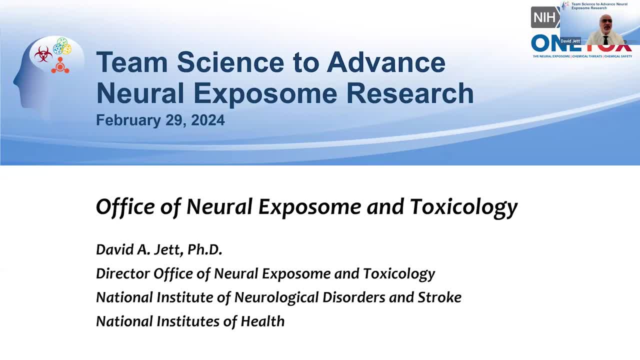 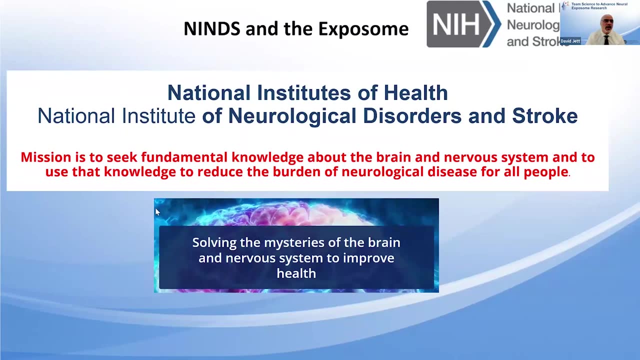 Dr Jett- And this will be a short presentation, Dr Jett, On what we're doing in exposome research at NANDS and why team science is so, so important. That's just a disclaimer thing. So, as you know, our focus is on the brain and the nervous system. 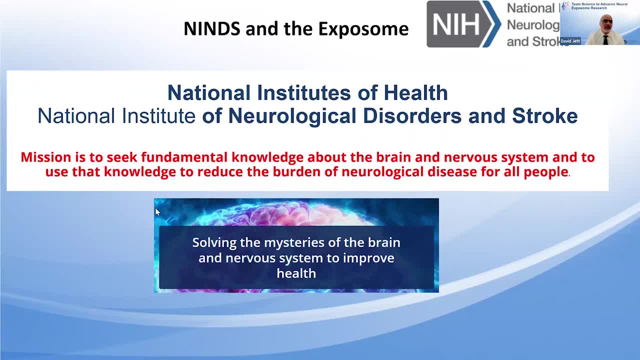 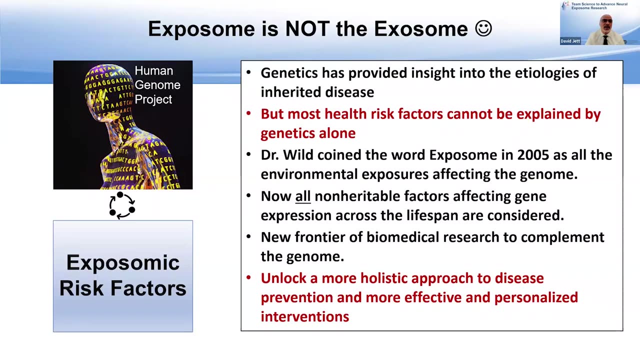 and we're more, I guess, of a disease-driven institute maybe, But we also have a very strong basic research component to figure out the causes of these diseases. So first is, what is the exposome? And I always tell people it's not the exosome, that's. 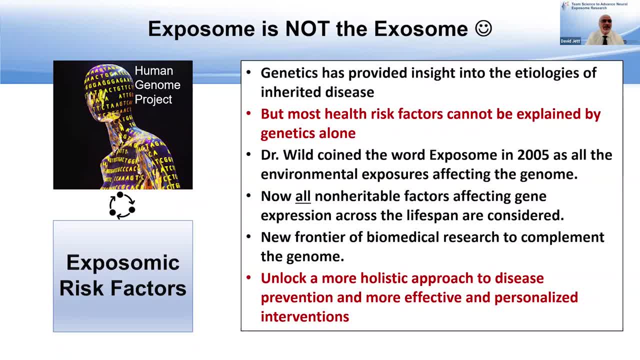 different. I'd like to say that this is really the next step after the human genome project, And what we'll get out of this work will be the integration of genetics and exposomics. So we know that genetics are well, we know that it provides insight. 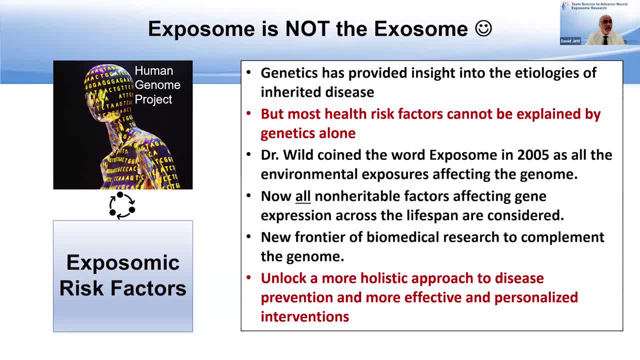 to the etiologies of inherited diseases, but actually most health risks cannot be explained by genetics alone, And some people say maybe six to 16% can be explained by genetics alone. So there's 80 more things that we haven't looked into. 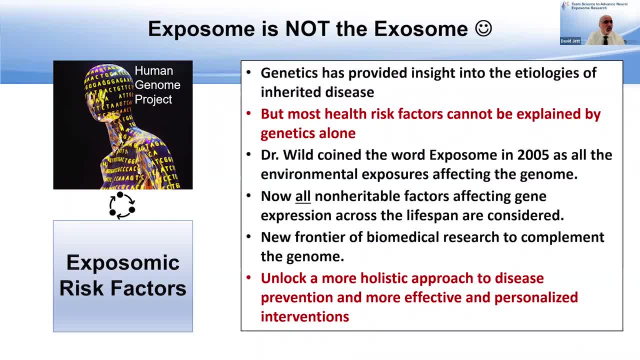 So back. so Dr Weil coined the word exosome back in 2005, and it was really just on environmental exposures. Now it's really on all inheritable factors that affect gene expression and it's across the lifespan. So I think this is a new frontier of really. 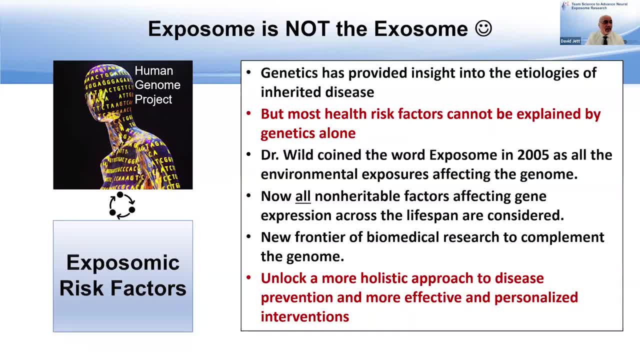 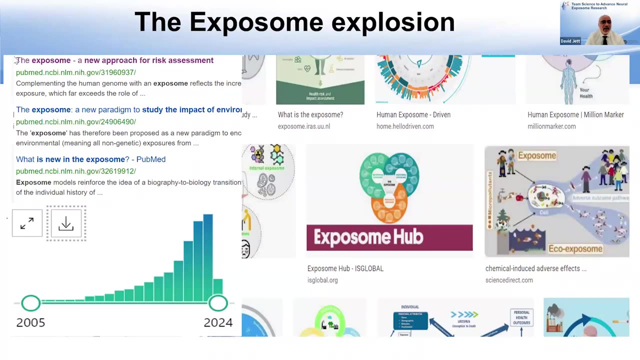 of all biomedical research. that will, I think, compliment what we've learned with the genome And I think at the end we're gonna see that it's gonna unlock more holistic approaches to disease prevention as well as better interventions. So there has, I think, been an explosion of papers. 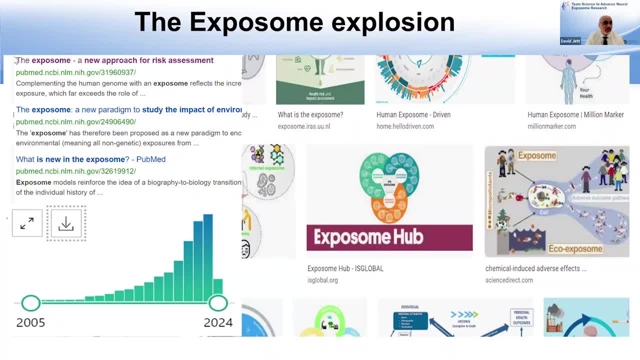 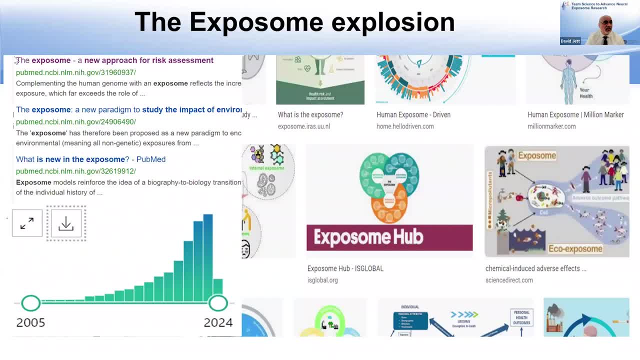 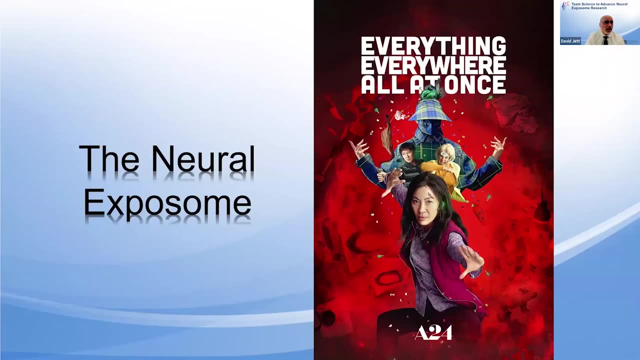 are about the same thing really. But yeah, I mean, if you go in and look and you'll see just many, many, many, many, many of these figures on the exosome. So yeah, I always put this and actually a lot of the exosome talks. 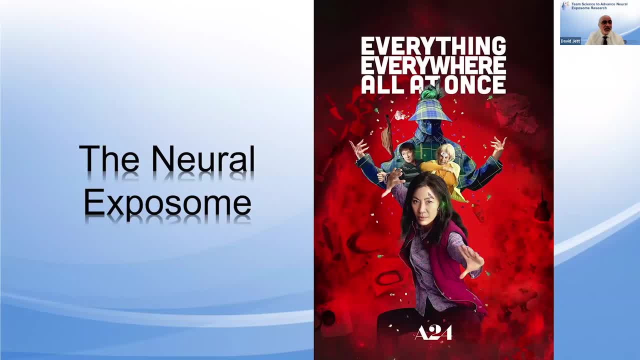 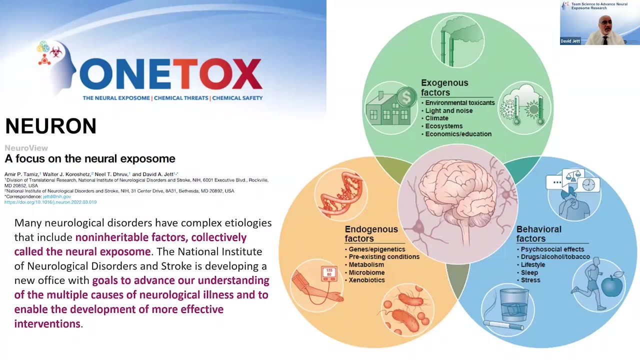 are now using this movie advertisement and in its broadest sense you can make the argument, and in its broadest sense you can make the argument that the exosome is really everything everywhere all at once. Now, when we think of the neurological disorders. 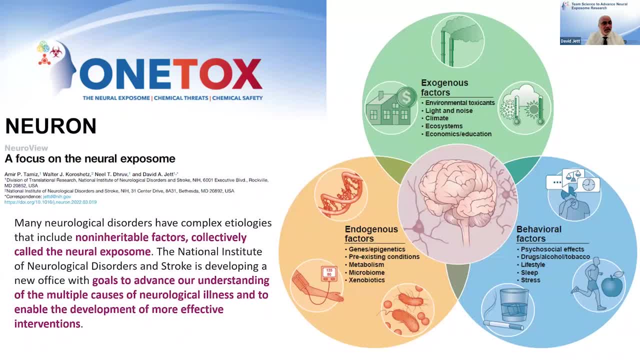 we know most have complex ideologies that include these non-inheritable factors. that include these non-inheritable factors and we're calling them the neural exosome. So, as this effort was growing, we put together, of course, we put together- a paper of one of our major journals. 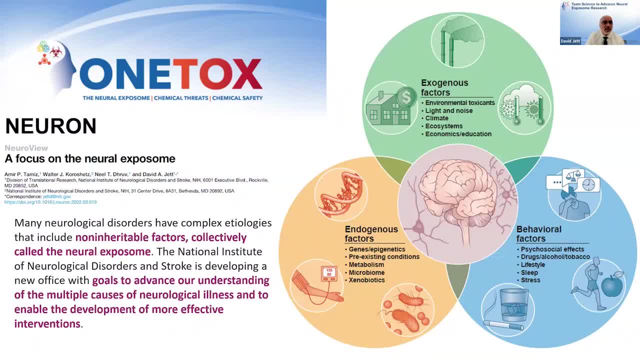 to describe our initial thinking for the office. It includes our own view of what the neural exosome looks like And I'm happy to say others are now using this picture in other papers coming out. And what you see here are three of these little areas. 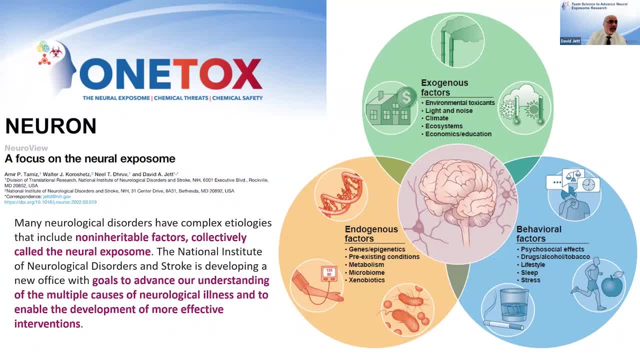 that we are calling the exosome One is exogenous factors such as, of course, environmental toxicants, but also things like noise and climate change, and then endogenous factors, which you put genes and epigenetics in there, but also things like the microbiome and xenobiotics. 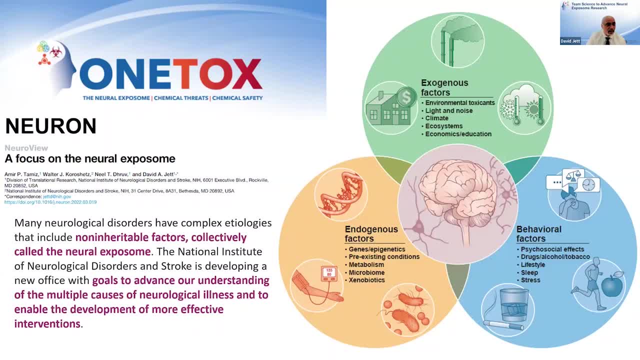 And then taking it just to its own ball, I guess, are the behavioral factors, which, yes, includes the psychosocial effects, but again also things like lifestyle, sleep and stress. So now, a true exosomic research project would include: 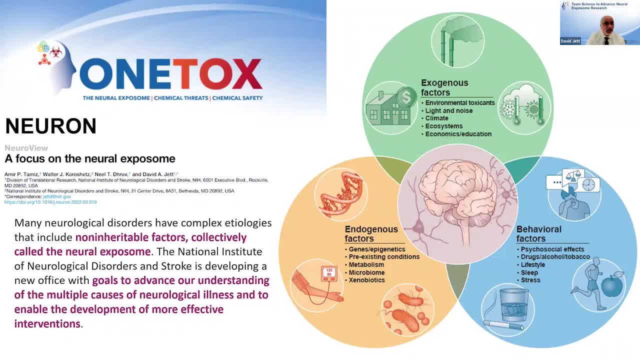 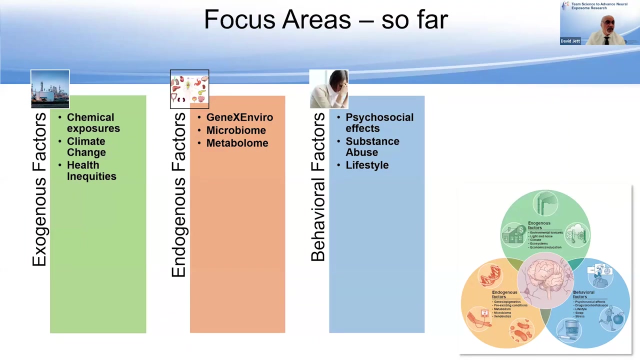 for example, sleep and air pollution and microbiome. So you can see that this kind of work demands team science and the need for these three areas to be. you know, have the scientific expertise So here, so we have an early focused area. 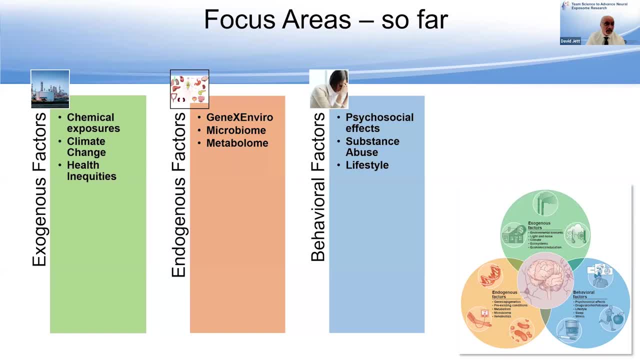 that will require team science. I say early because, as you know, we have a group of experts working on a strategic plan that will help us decide what our priorities will look like- But sort of- as we've already seen- exogenous factors. 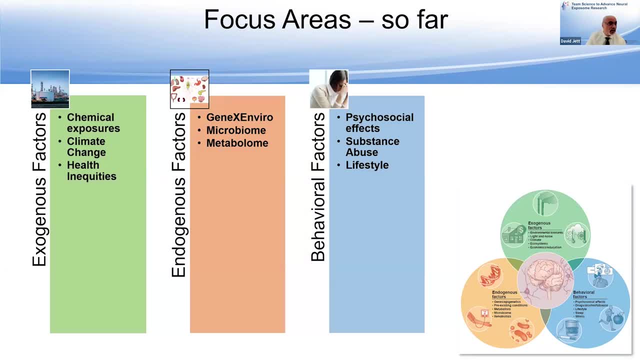 chemical exposures, climate change, and we're doing a lot in working with our other office in health disparities, And then gene, environment and actions, microbiome, metabolome and then behavioral factors. We've already done some work in the psychosocial field. 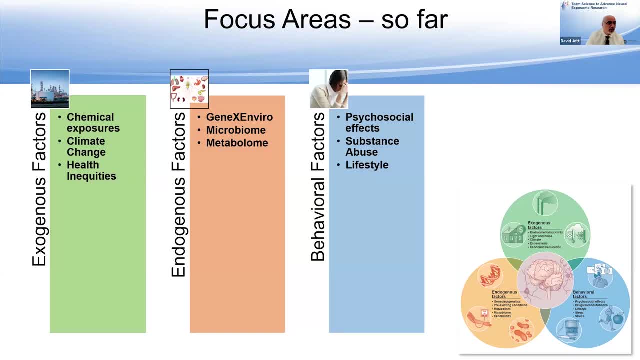 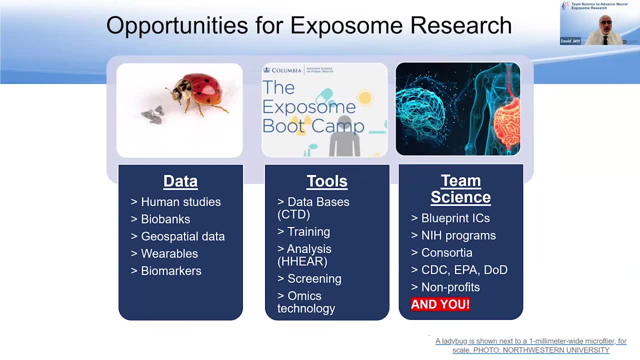 So that's basically so far what we're doing Now. so these are just, I think, some of the reasons the exposome is timely. There are opportunities that now have become more available, things like the data, human studies, biobanks. 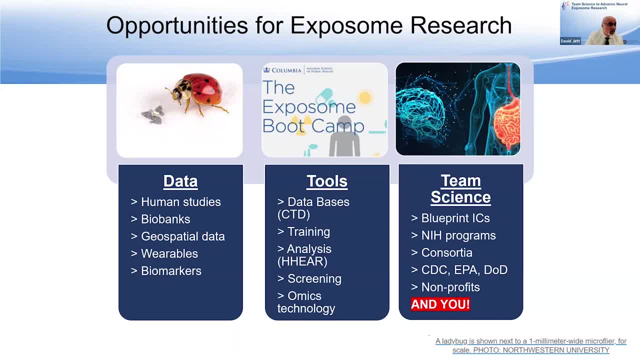 wearables, biomarkers, tools And, by the way, this picture that you see of the- I guess it's a ladybug with those little things in front of it- are these things that you can let free in the air and they will fall down to the ground? 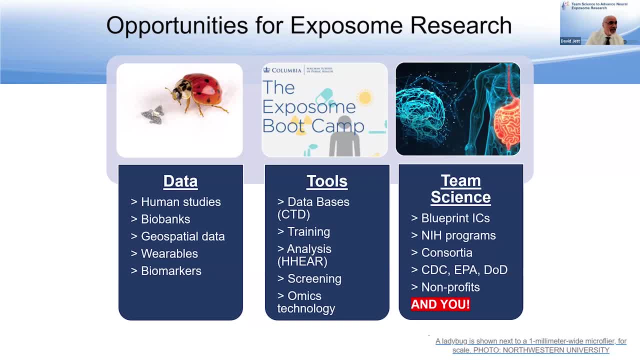 and you can actually look at air pollution with those. So I mean there's a lot of stuff going on In the middle. the top is the exposome bootcamp at Columbia And those other tools like databases, like CTD, the HEAR program here at NIEHS and other things. 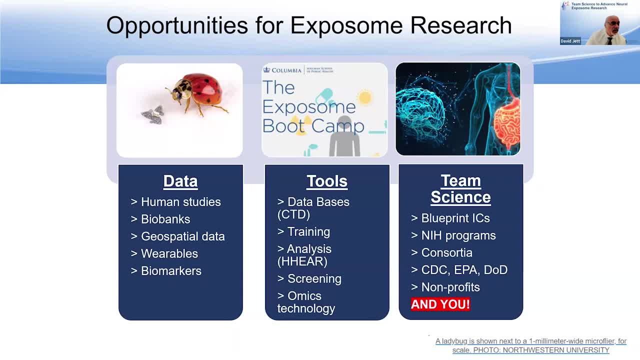 And then team science, which is absolutely critical, And a lot of it's going to depend on all of us and you to really think about how to do more true team science, Because without it, the exposome, in my opinion, isn't going to work. 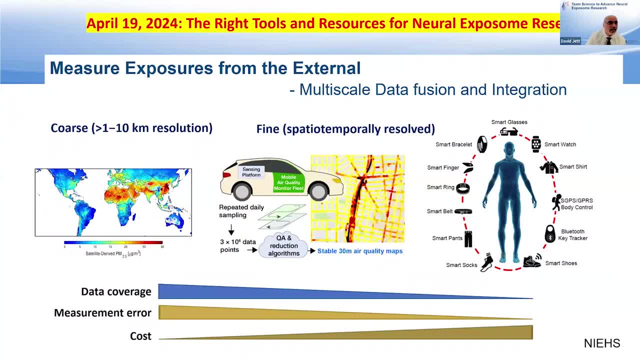 OK, this is my sneaky reminder of part two of this. It will be in April and it's on the tools and resources that science needs for work on the neuro-exposome, such as the wearables that you see here. It's just mind-boggling how many different kinds. 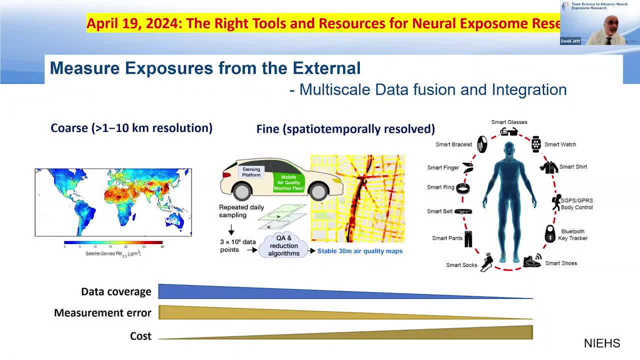 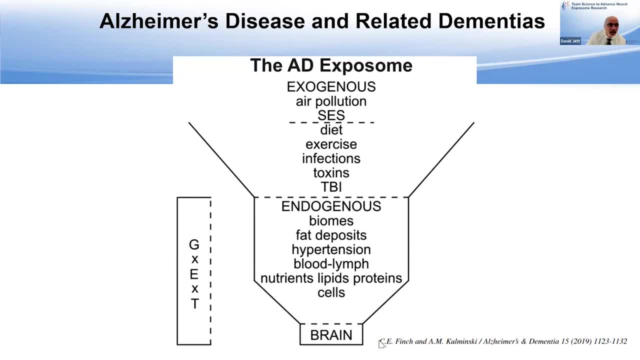 of wearables there are now OK, so let's skip to a few examples. Many of the diseases you think about in our NINDS mission space are already being studied within the exposome Here with Alzheimer's disease-related dementias. 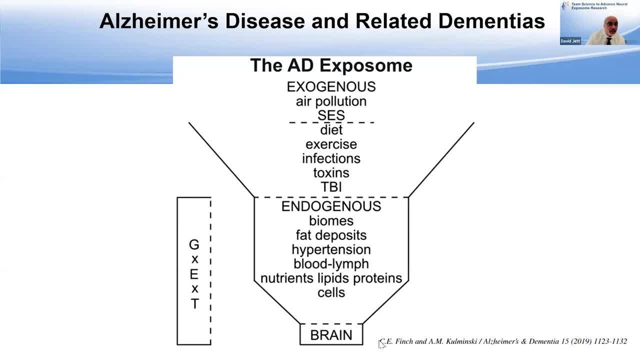 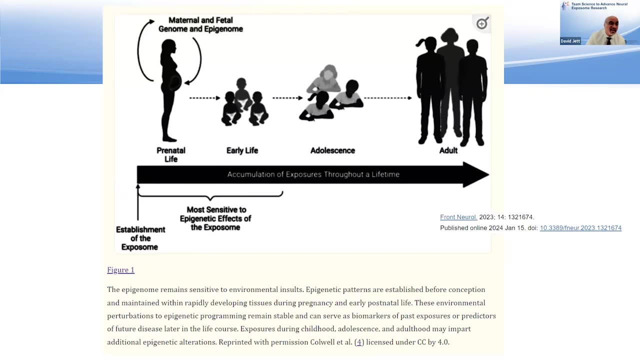 you see exogenous and endogenous factors and its interaction with genetics. but also you see the importance of time, For example. here the exposome really starts in prenatal life and follows through early adolescence and adult life And the epigenetics effects actually happen very early on. 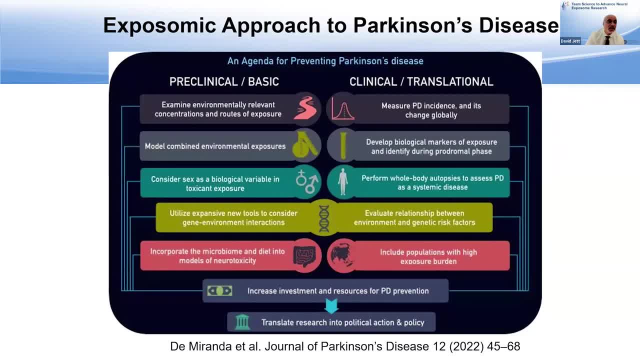 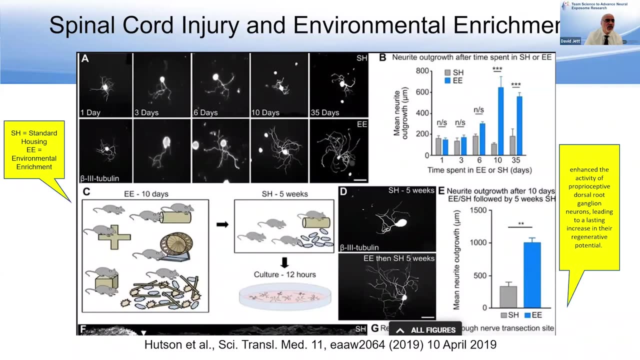 Here's just a slide for Parkinson's disease, with an agenda that includes the environmental factors in both preclinical and clinical aspects, where they are both important. So even things like spinal cord injury. in this case, a simple environmental enrichment gauge in rats: increased regeneration. 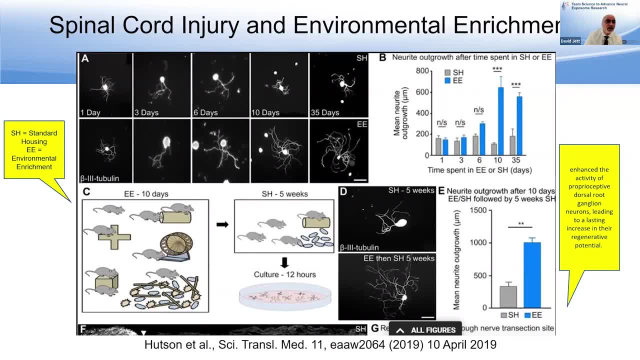 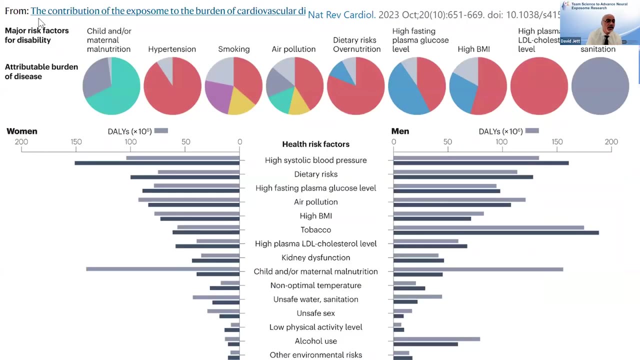 of the dorsal root ganglion and neurite outgrowth after transaction, nerve transaction. So with this I mean think about what that could do in human studies and in human treatment. So here it's just a, it's a review, where they show 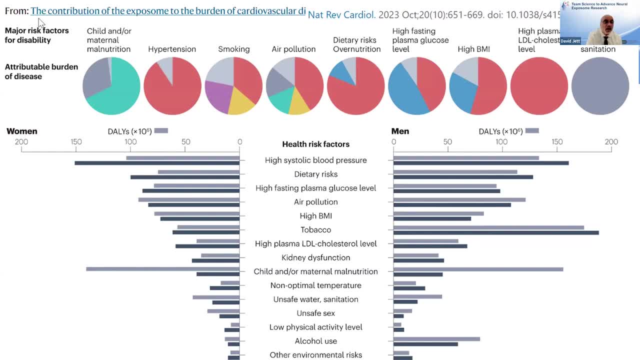 many exposome factors of cardiovascular disease and things like air pollution, child malnutrition and climate. The important part is think of what this data can do for future health research as well, as you know, as preventative medicine And you can see all of the different. 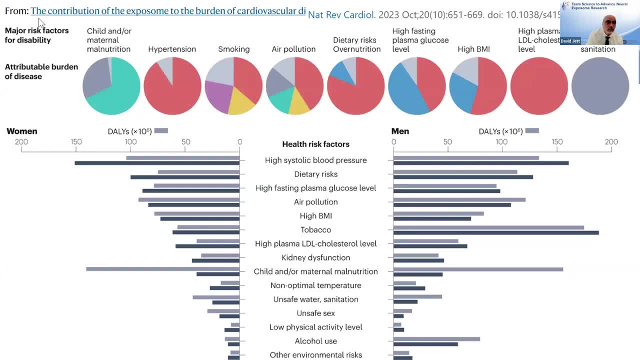 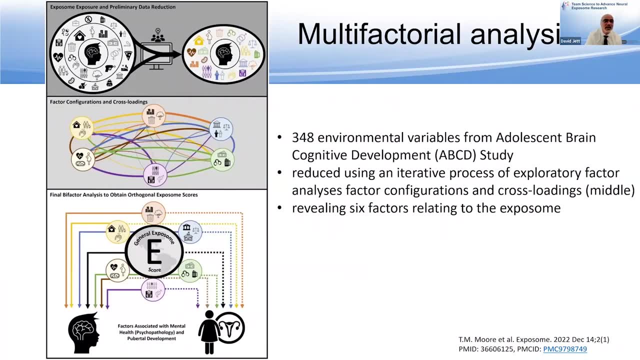 different things that they looked at. Okay, I don't want to just a couple more of these. This is one on multifactorial analysis and basically 348 environmental variables from this was from the ABC study- were chosen for representing the multiple dimensions. 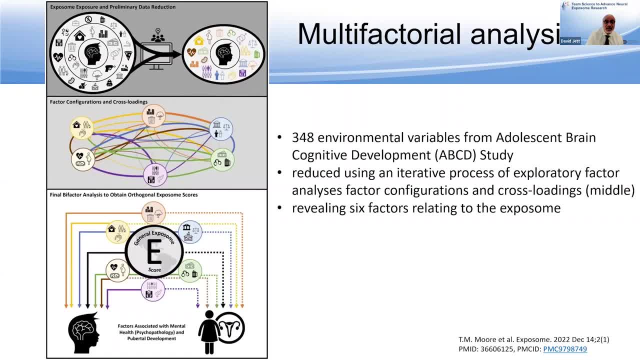 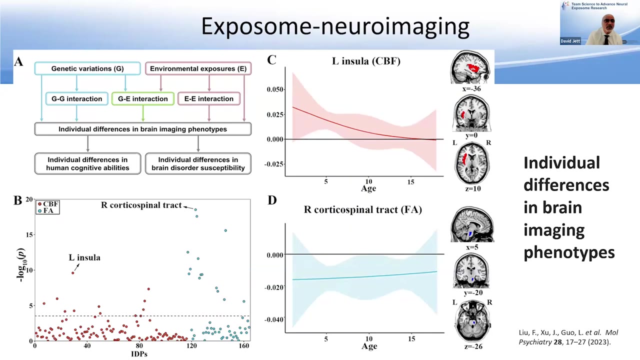 of the exposome And basically they were reduced using this iterative process of exploratory factor analysis and ended up with only six. six of these factors, And this is one on imaging, neuroimaging. The bottom line was they showed that brain imaging phenotypes. 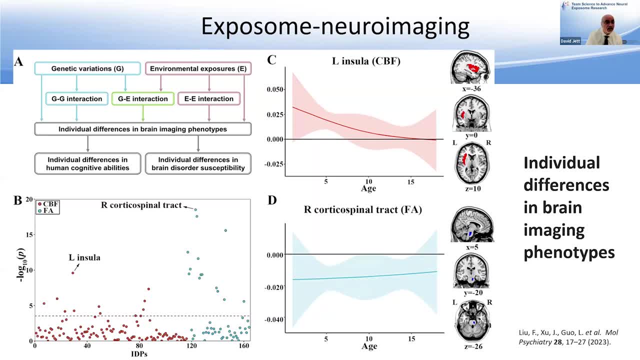 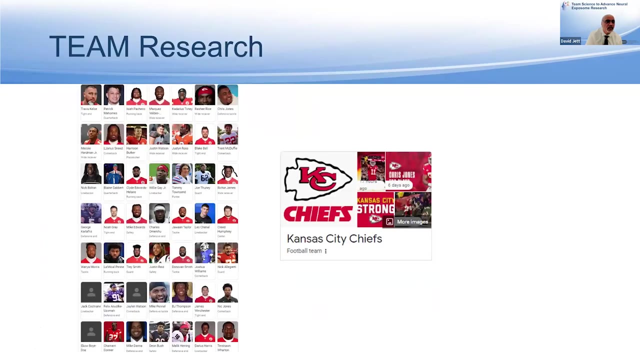 are determined by genetic variations, but also environmental exposures, gene gene interactions, environmental environmental interactions and gene environmental interactions And the brain imaging phenotypes will result in individual differences in cognitive ability and other things. Okay, so for team, so first, so I put this random football. 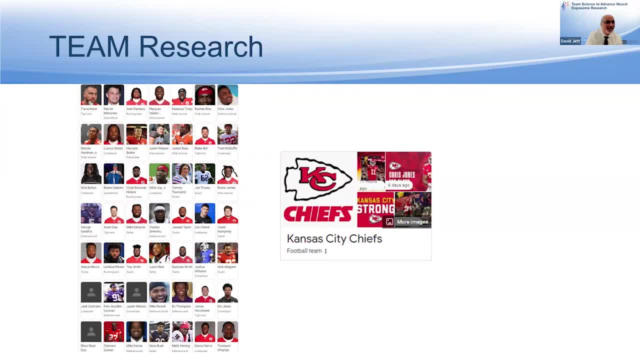 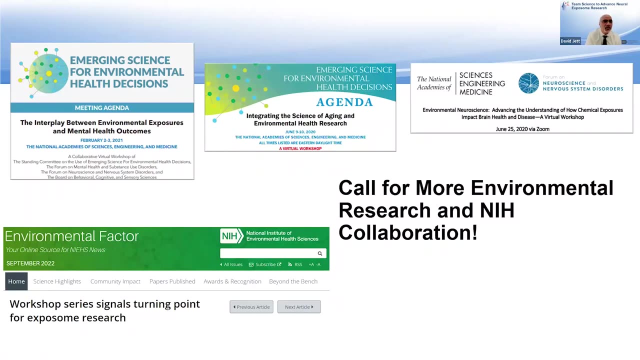 football group together just to show how important teams are. I mean, you need a quarterback and runner and kicker and a defender and et cetera, And I think that really one of the major parts of why my office is timely, I believe. 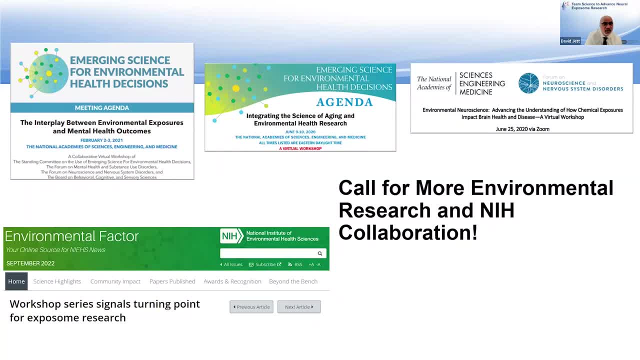 are the different workshops in the past five or so years that focused on environmental research as it relates to disease, and workshops included mental health, aging, one we did on brain health and disease, And the thing that they all had in common was the need for more research and, more importantly, 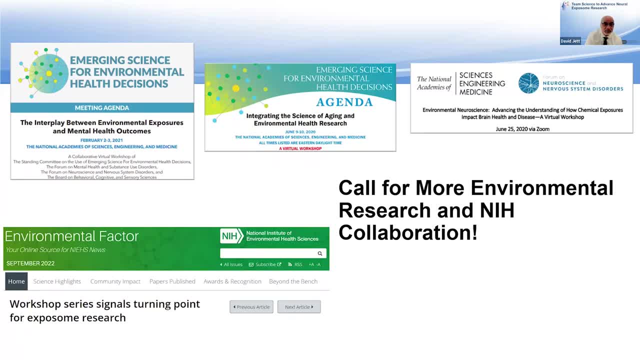 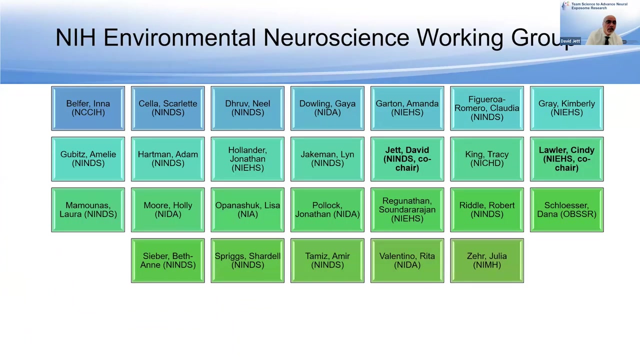 more team science, collaboration and team science, And so also the NIEHS led a comprehensive series of workshops that helped- at least help me and others- understand what we're up against in fully understanding the exposome. Another thing we did very early on in this office was 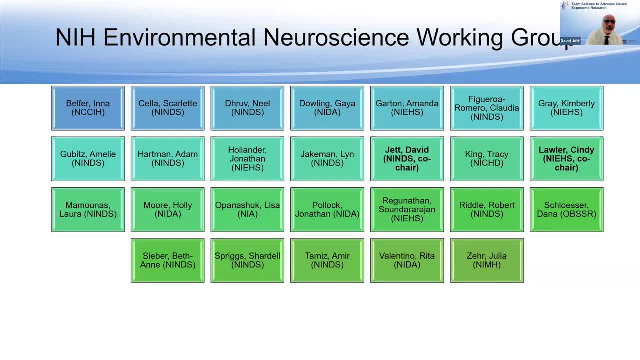 we fostered a more collaborative across the more collaboration across the NIH ICs institutes and centers And we put together an NIH wide environmental working group to talk about everything from ideas from you know, collaboration and new programs to request for information. 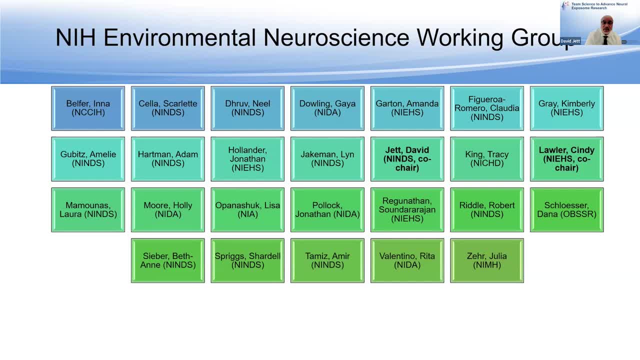 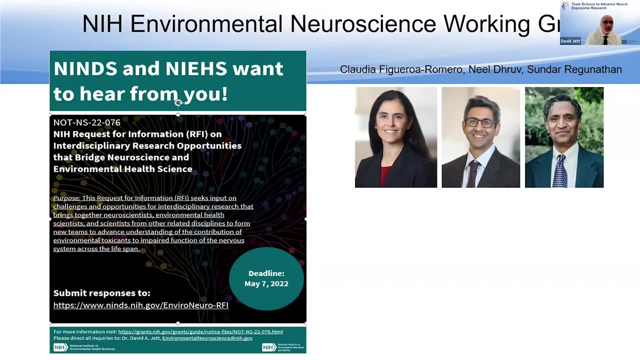 from the public ideas for SOT and SFN symposiums and bringing in speakers on the exposome for our group to look at, And this is the our request for information. that we did a couple a while back actually, And thanks to Claudia and Neil Sondar for that. 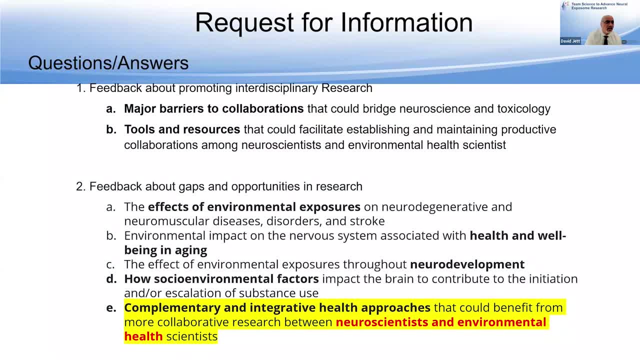 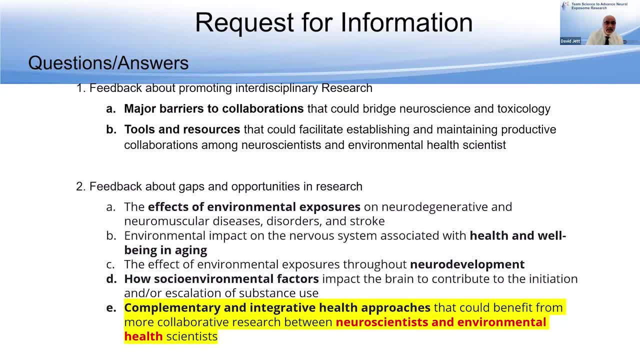 And this is the workshop on team science And, as I said before, we'll have the other one in April, And we received a lot on specific topics, but what I want you to see is what has been on my mind, at least for the most. 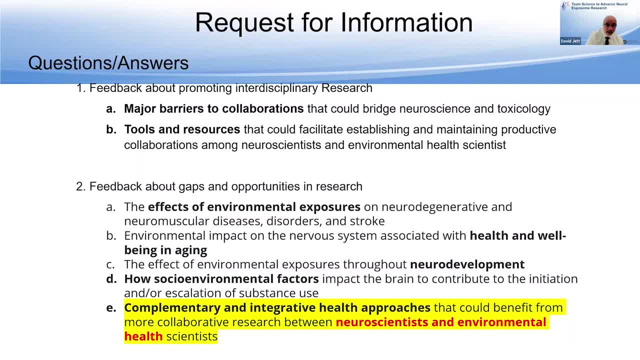 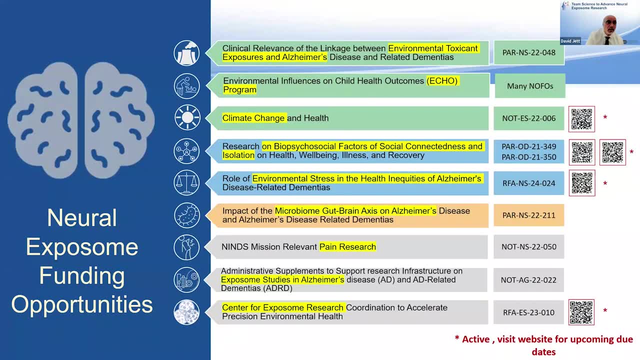 and that is engaging more neuroscientists. you know, with thousands of them, only a few are engaged in exposome research. So, last but least, we started early. I didn't want to wait too long, So we started the science with several funding opportunities. 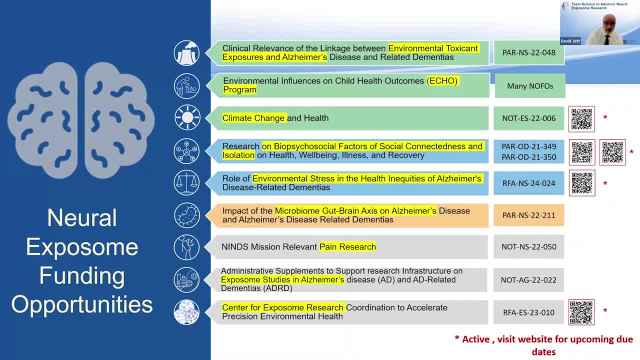 both on our own and some with other institutes. These included so far things like environmental toxicants, worked with the ECHO program. We did some work with climate change. we did biopsychosocial factors, in this case with the social isolation and connectedness. 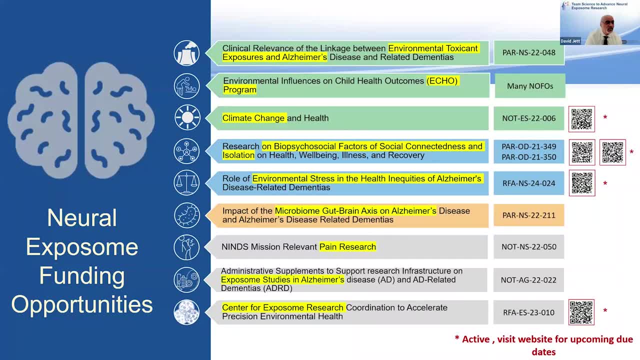 Let's see environmental stress and environmental stress in the health inequities of Alzheimer's disease. to really look at what we're looking at for health inequities, Other things like the microbiome pain research, some other kinds of exposome studies, 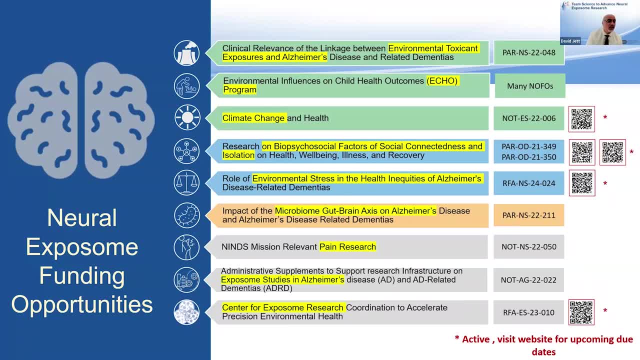 And we also have a center for exposome research, And I'll say now that there's two more that will be out soon, One on the exposome and Lewy body disease and one on nervous system exposures, And they'll be out soon. 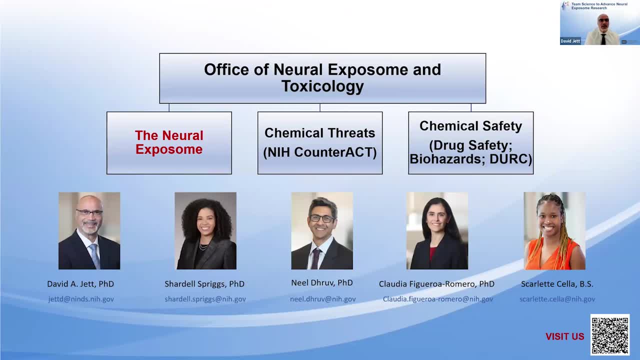 Okay, so that's it, And thanks to our office, we have three branches And we focused on the exposome branch. I have a fantastic small group that runs the office, but you can imagine- and it's not surprising- that for exposome we work with all of the people at NINDS. 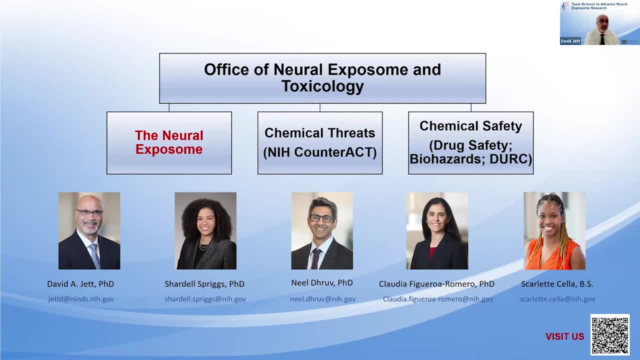 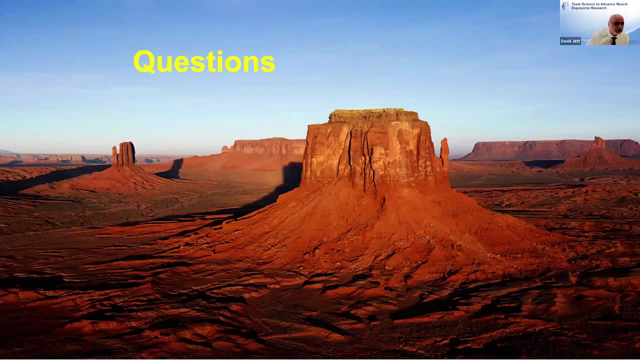 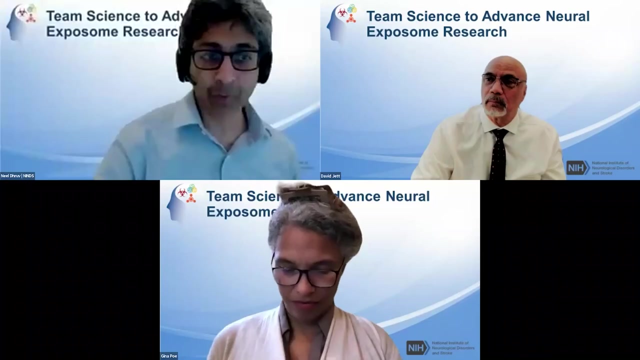 and many other ICs as well, and other agencies as well. So that's it for me And thank you for listening. And I don't know if there's questions time, but thank you. Okay, I don't see any questions. 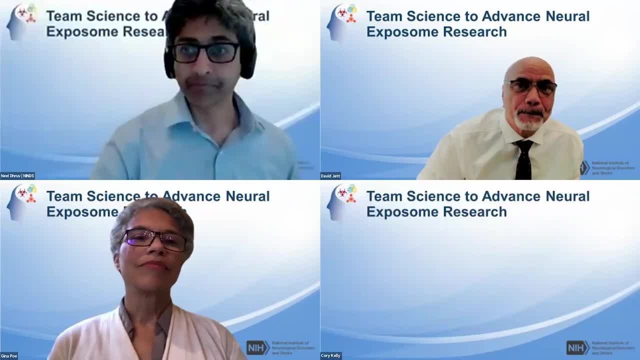 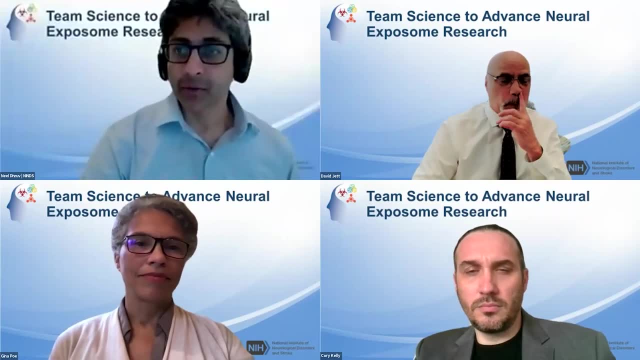 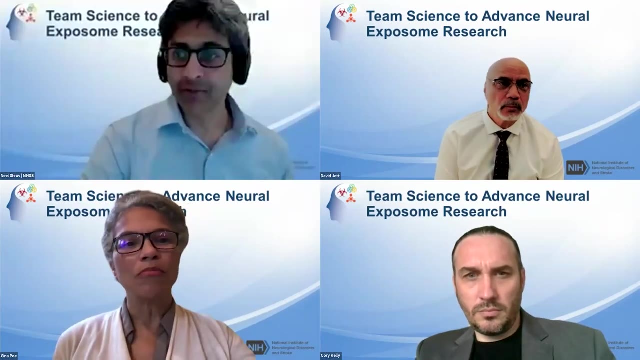 So we'll move ahead with the agenda. Thank you, Dr Jett. We next have a team presentation for today's mini workshop on team science. This one is from Dr Karen David and Mr Corey Kelly, both from NINDS. 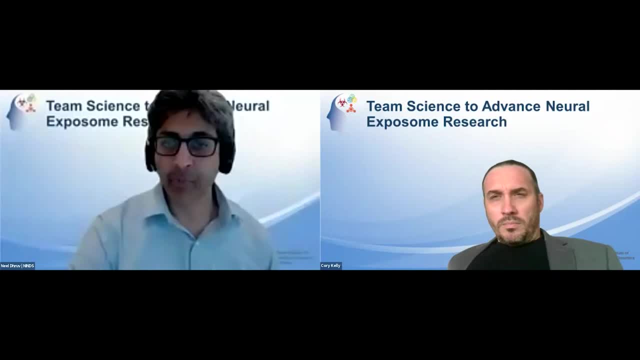 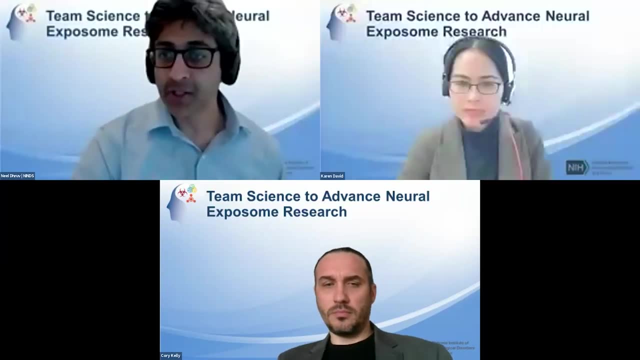 Dr Karen David is a program director with the goal of promoting team science, enhancing species diversity and neuroscience, fundamental neuroscience and the integration of multi-scale approaches to solve complex systems neuroscience questions. She led the creation of the new team science funding opportunity, the NINDS. 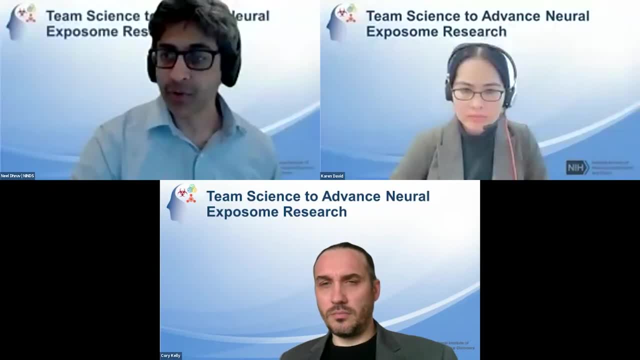 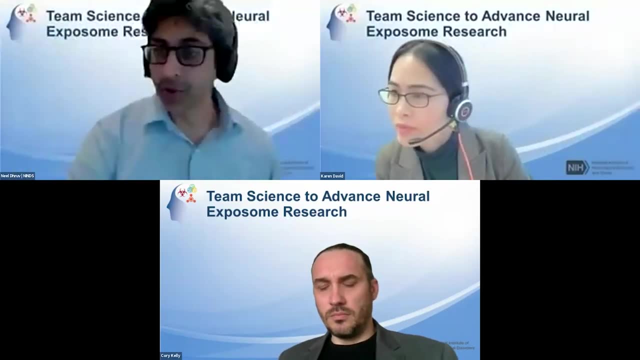 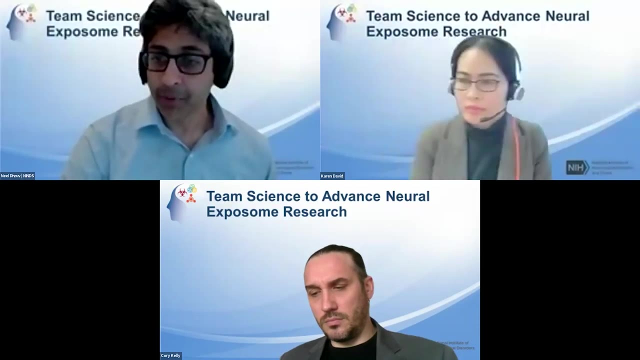 collaborative opportunities for multidisciplinary, bold and innovative neuroscience program- the COMBINE program- which she currently co-leads with Corey Kelly. This COMBINE program, as part of the NINDS strategic plan for research, is designed to support interdisciplinary research teams. 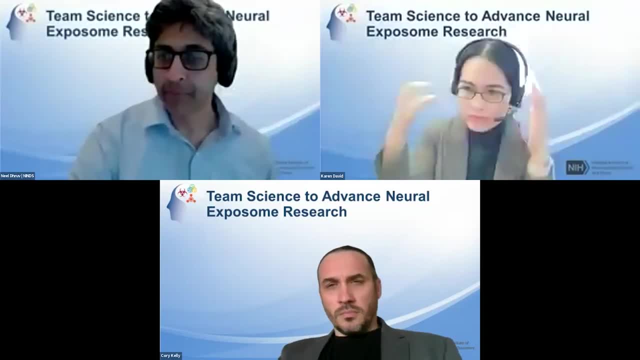 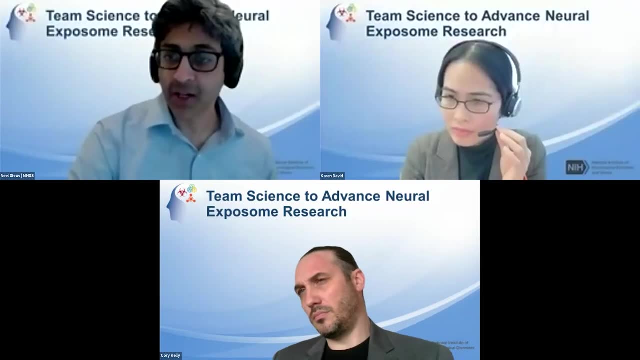 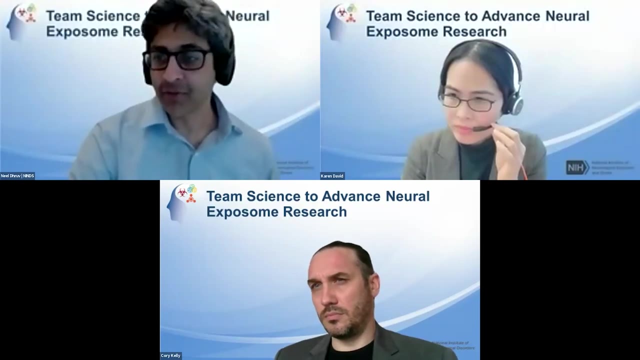 to achieve transformative goals that could not be met by individual or parallel efforts. In addition to co-leading the COMBINE program, Mr Corey Kelly serves as the advisor for research operations and program implementation in the research operations branch within the NINDS Division of Extramural Activities. 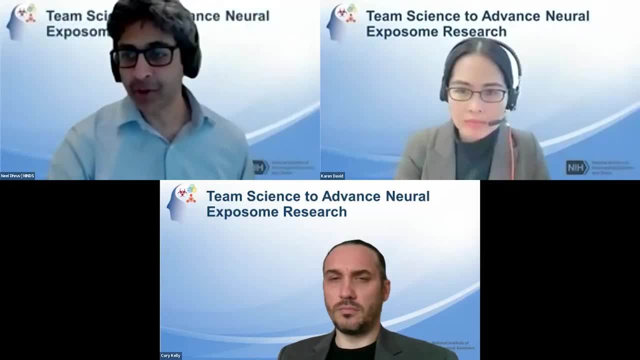 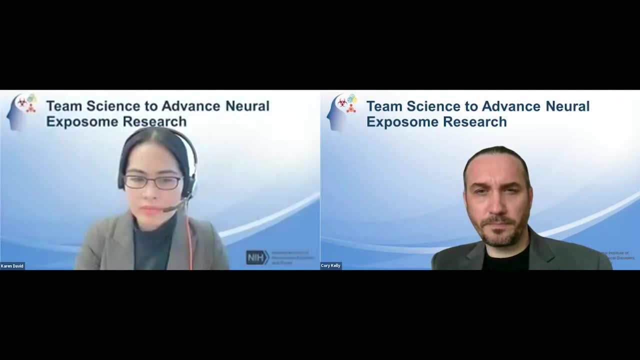 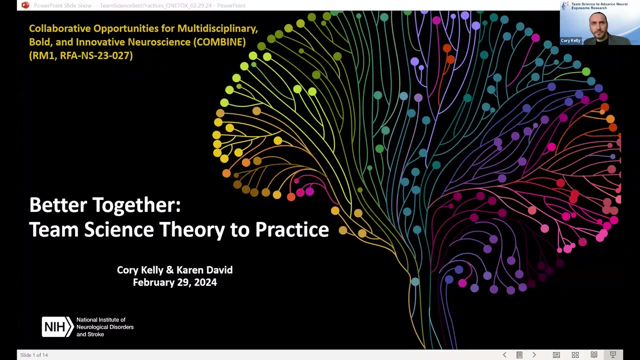 Their talk is titled: Collaborative Opportunities for Multidisciplinary, Bold and Innovative Neuroscience. Thank you, Neil. All right, Good afternoon everyone. My name is Corey Kelly. As Neil said, I'm a program officer here at NINDS. 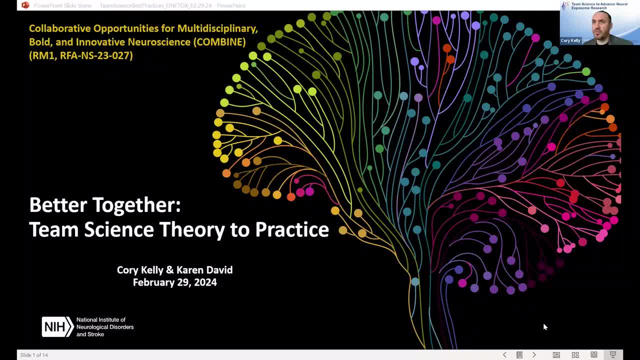 where my work focuses on team science, research operations and program implementation. First, I'd like to thank the NINDS OneTalks team for holding this critical workshop, as well as my fellow speakers and, most importantly, the NeuroExposome community. 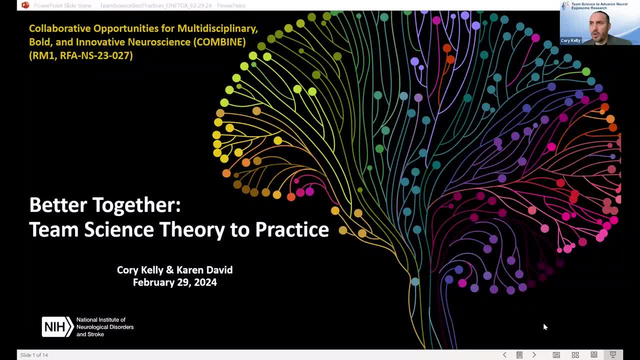 for your interest and time. Today, along with my excellent program co-lead, Karen David, we're going to be discussing the NINDS flagship team science program, the COMBINE program. First, I'll provide some background on the landscape. 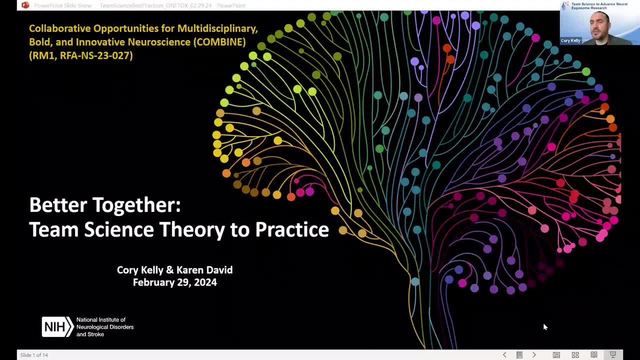 and best practices of team science, and then Karen will discuss how we've integrated this knowledge into our COMBINE program theory and implementation. I must also thank our exceptional COMBINE NINDS scientific review officers Bo-Hsuan Chen and Li Xia. 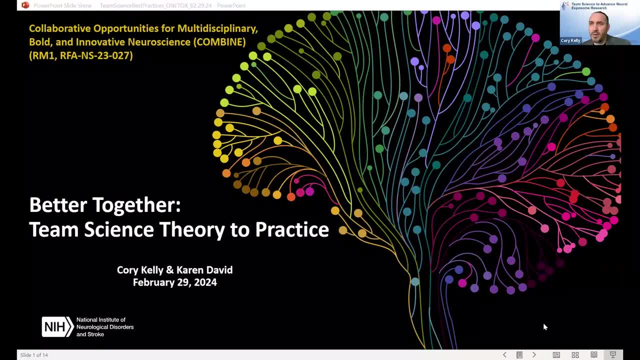 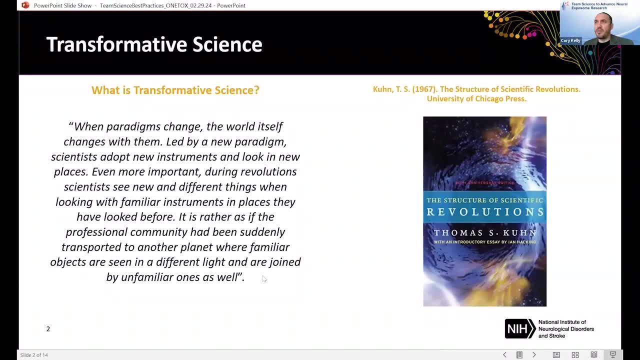 as well as the study section members and all of our amazing NINDS staff that helped make this very complex program happen. My talk today will primarily be about team science, but the COMBINE program specifically was created, you know, by a group of NINDS members. and we're going to be talking about team science, but the COMBINE program specifically was created, you know, by a group of NINDS members and we're going to be talking about team science, but the COMBINE program specifically was created. 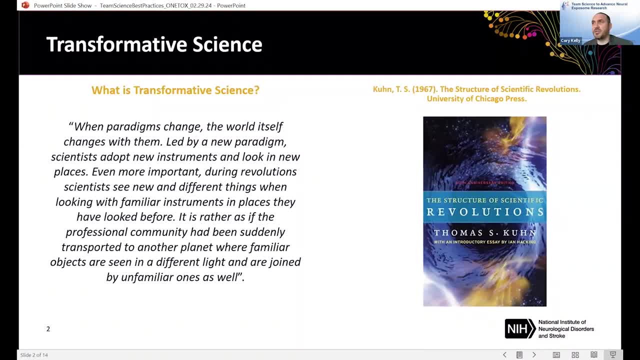 to utilize the power of team science to achieve the most ambitious goals in neuroscience, to achieve transformative science, a paradigm shift, a revolution in our understanding of the brain. I often find myself going back to Thomas Kuhn's structure of scientific revolutions, commonly known as structure. 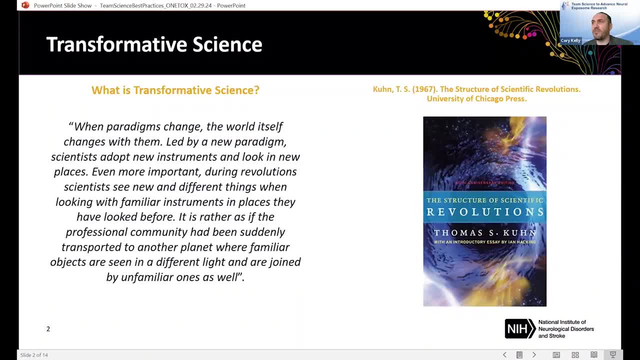 Kuhn wrote: during revolutions, scientists see new and different things when looking with familiar instruments in places they've looked before. It is rather as if the professional community has been suddenly transported to another planet, where familiar objects are seen in a different light and are joined by unfamiliar ones as well. 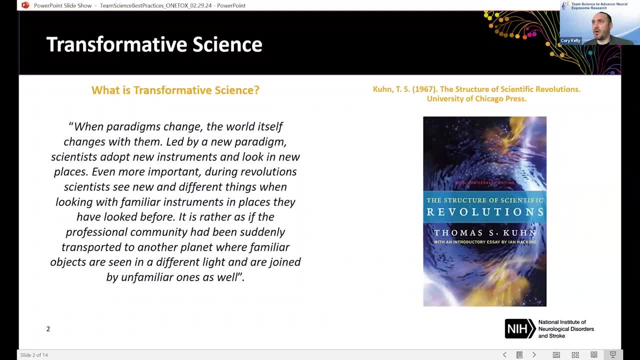 So the COMBINE program specifically was created, you know, to utilize the power of team science to achieve transformative science, a paradigm shift, a revolution in our understanding of the brain. There's been a great many paradigm shifts in neuroscience throughout the course of history. 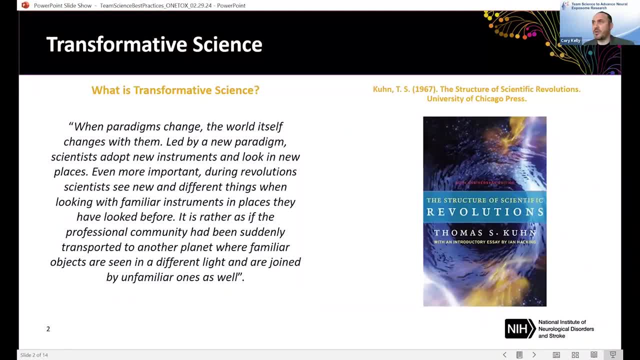 where our concept of normal science completely changes. I myself was first drawn to neuroscience through the classical discourse on the duality of the brain and the mind: Aristotle, Plato, Descartes, Aquinas, Locke and my. how far normal science has come. 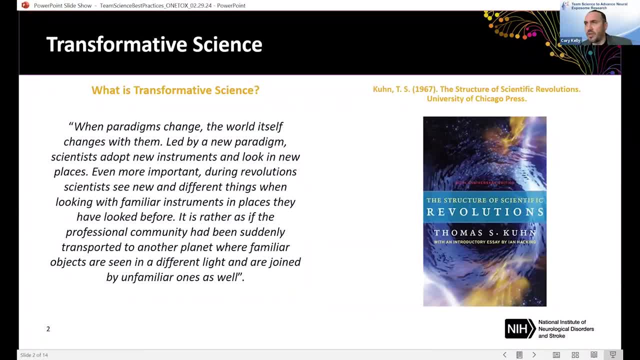 since the era of antiquity: Luigi Galvani's discovery of electrical excitability of neurons, Camille Golgi's staining methodology, Paul Broca's theory of the brain and structure, Bernard Katz's modeling of the synapse and Marion Diamond's work on neuroplasticity. 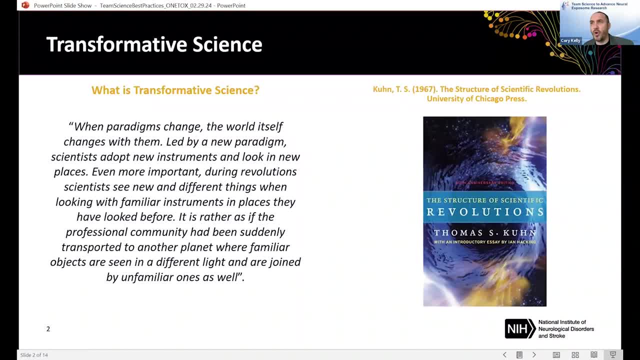 that serves as the foundation of modern neuroscience, and many more. Yet despite all of these great works of which we stand on the shoulders, neuroscience and the brain still remains the great final frontier of biomedical science, And the COMBINE program was established. 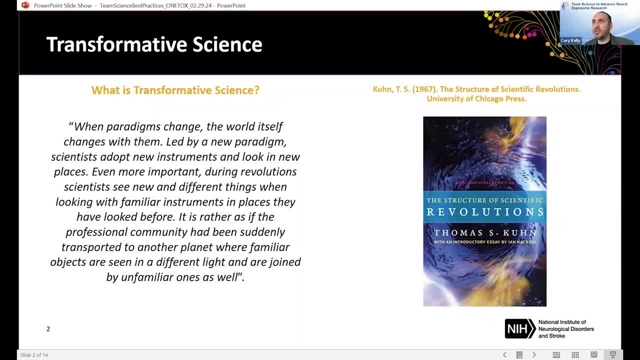 for those investigators willing to take the risk of eschewing neuroscience, pushing the boundaries of our understanding, and achieving this transformation, this paradigm shift, this revolution, this fundamental change in how we understand the brain. However, the most ambitious goals and challenges of modern neuroscience research: 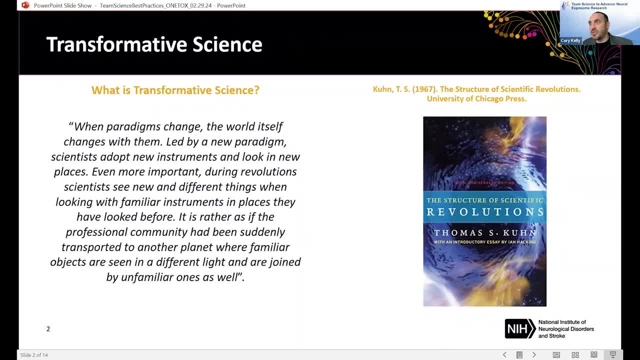 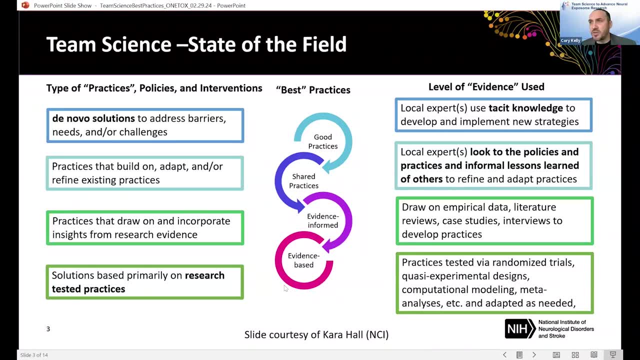 are increasingly dependent on collaborative approaches that leverage not only diverse disciplines, expertise and perspectives, but effective interaction between team members. Team science is still a burgeoning field. The roots of team science began in the 1990s here at NIH, and as NCI began to seek transdisciplinary approaches. 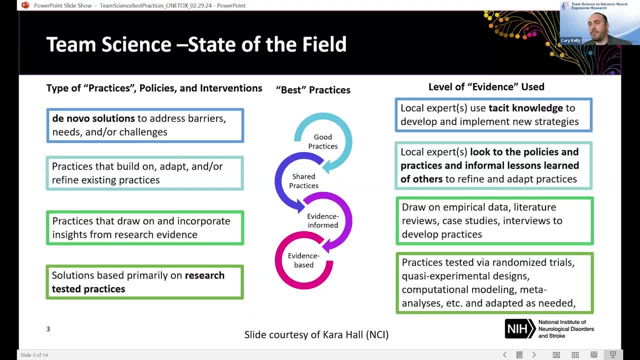 to understanding the myriad of factors that contribute to cancer pathology treatment and care. We're quite honored today to have one of those NC pioneers of team science, Michelle Bennett, as a speaker. Dr Bennett's collaboration and team science field guide was first published in 2010.. 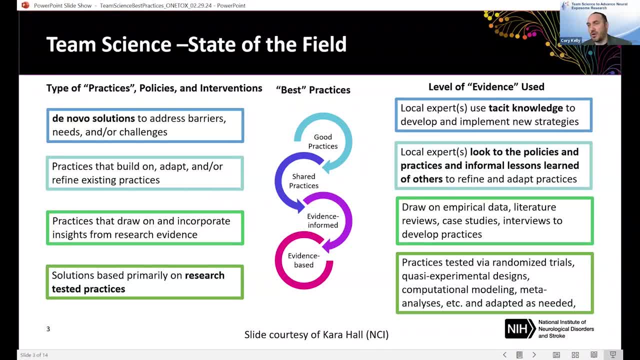 It's considered by myself and by many others- by myself and many in the team science field- to be the foundational work that established our field. Over the course of the last decade, there have been a proliferation of work in team science, but the field is still just beginning to transition. 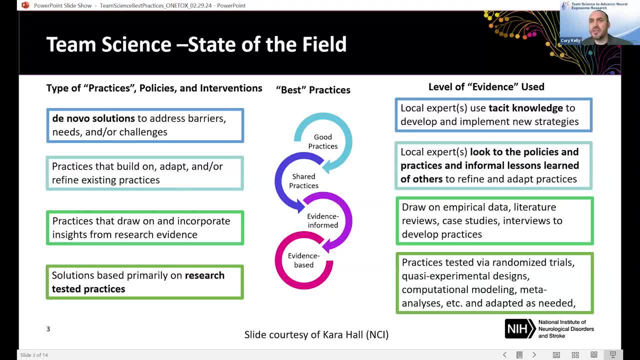 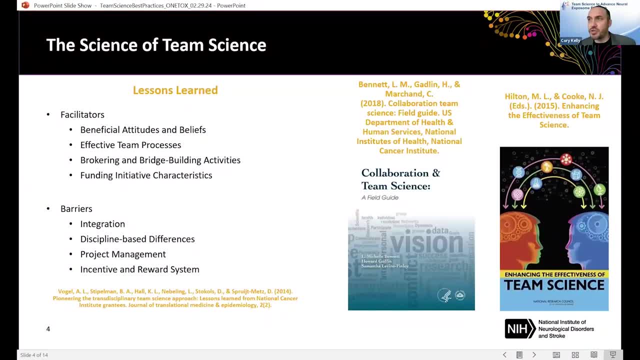 from shared practices to evidence-informed and evidence-based practices. the science of team science: As we build team science programs and team science research projects, we can look towards this pioneering work for lessons learned. We found that facilitators of team science include beneficial attitudes and beliefs. 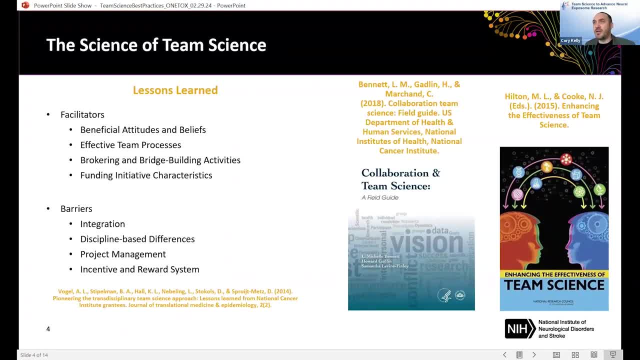 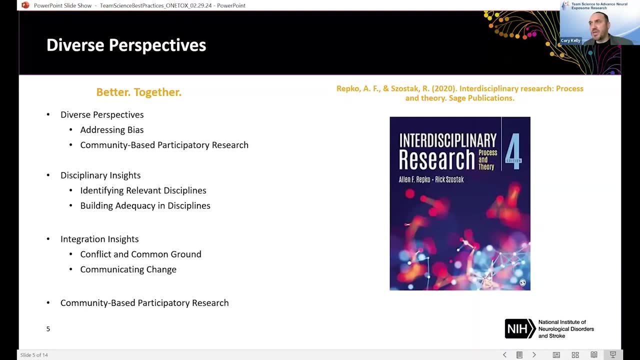 effective team processes, brokering and bridge-building activities and funding initiative characteristics, while barriers include integration, discipline-based differences in project management and the incentive and reward system. Moreover, a critical component of team science is the inclusion of diverse perspectives, A fundamental tenet of team science. 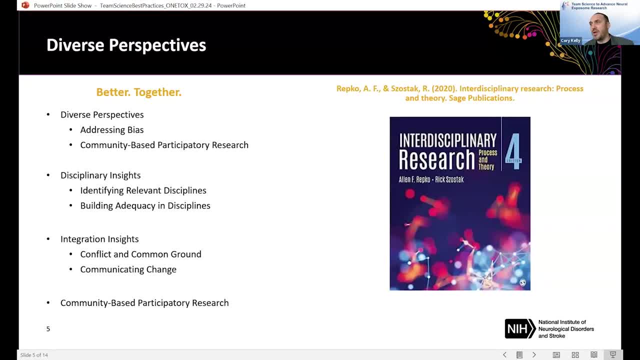 is the concept that, despite our best intentions, everyone will always have residual bias. but by bringing together diverse perspectives, the impact of our residual biases can be mitigated and ultimately our findings can be more generalizable. But bringing together diverse perspectives requires not only which perspectives are required. 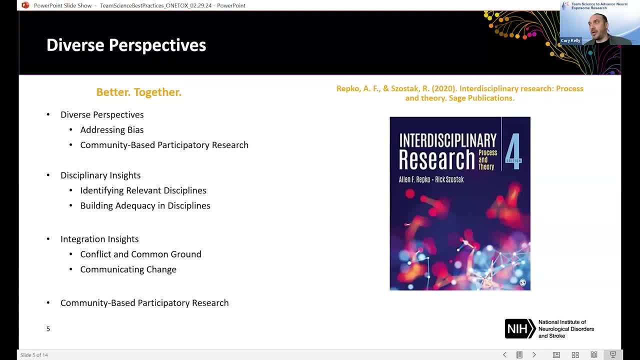 but also how to manage conflict and create common ground, which I'll talk about in a later slide. Last, I would like to highlight community-based participatory research, a powerful team, science-based methodology for building sustainable interventions. CBPR goes beyond patient advocacy or patient outcomes. 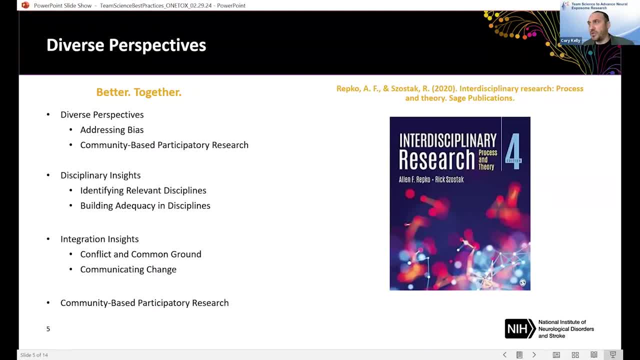 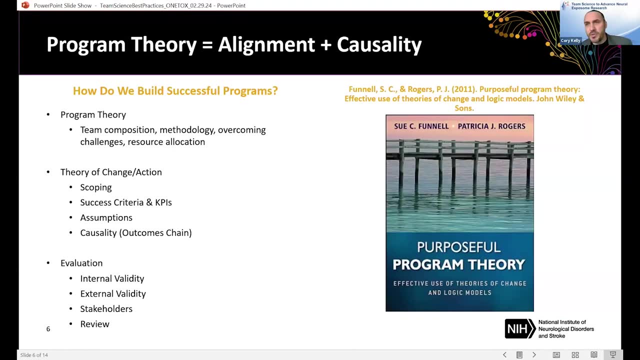 but integrates the community members as a collaborator from the very start of the research. The researchers work alongside the community to identify the problems, develop the interventions and sustain change. So how do we build effective team science programs? First we start with purposeful program theory. 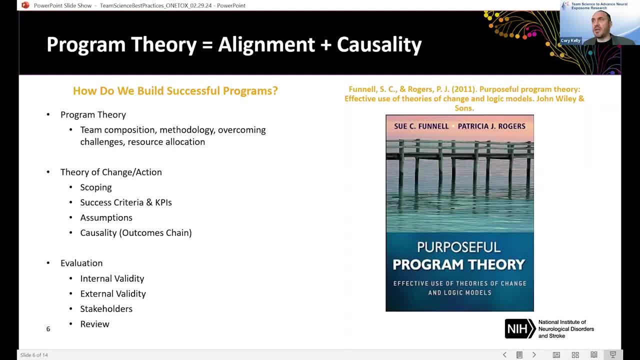 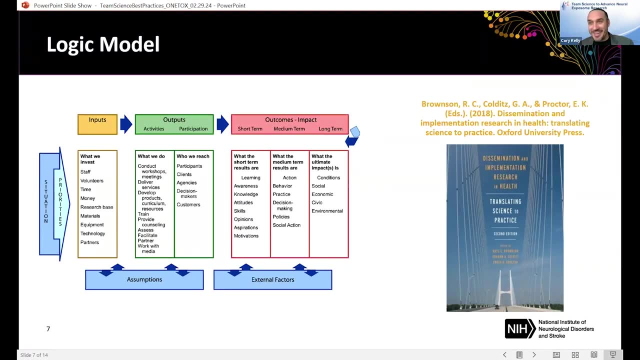 This means the alignment between the problem statement, the research questions, the conceptual framework, the methodologies and the outcomes. Simply, alignment allows for a stronger argument of program causality, that the program is indeed the driving factor of change. I'll give a caveat. This is my favorite slide. 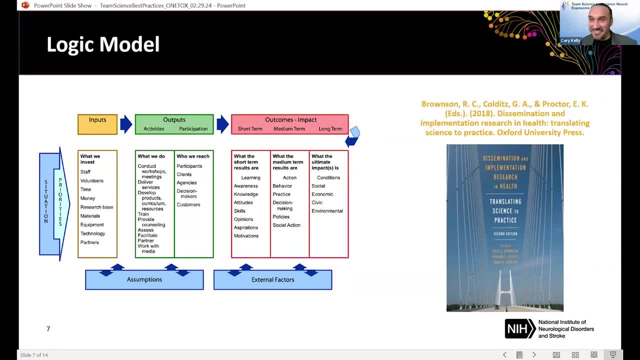 and anybody that knows me knows I could spend an hour on this slide alone, but I won't do that to you. today. I want to present a program theory tool that's very powerful. It's called a logic model. I encourage everyone to take a look at these. 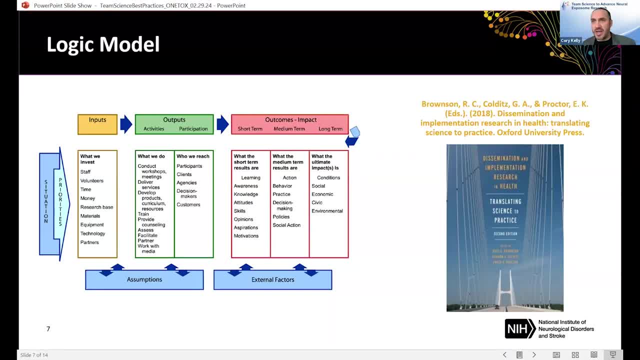 when you're developing programs or research projects. This is how you can establish causality. This is how you can demonstrate progress. Working backwards from the ultimate long-term goals, we can create a chain of logic from the long-term to the short-term. 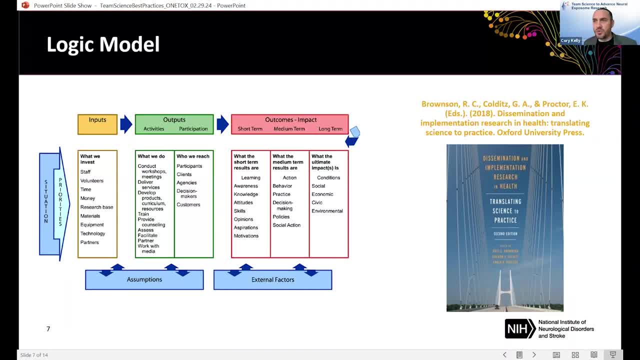 We can then determine the specific activities and participants requisite to achieve these outcomes and the requisite resources to perform these activities. Each of these elements- it also considers the assumptions and external factors that are necessary for success. Last, and perhaps most importantly, a logic model has key performance indicators for each factor. 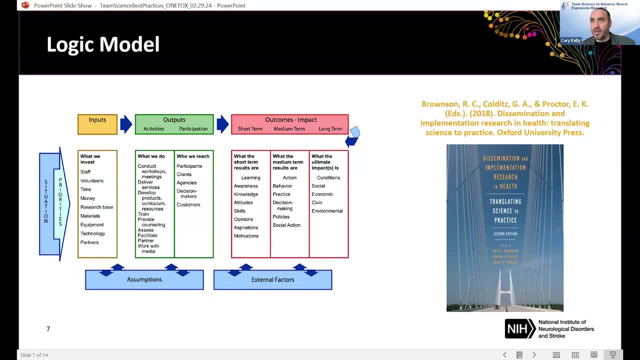 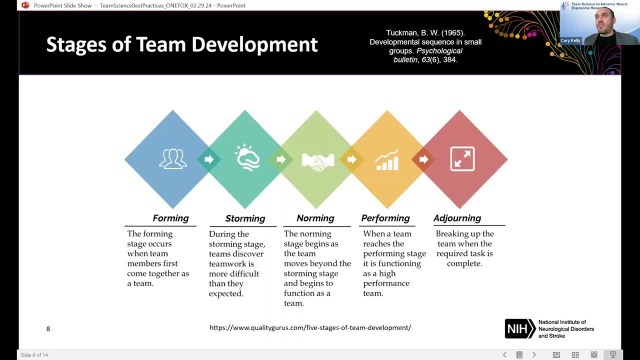 which allows for a very granular assessment of what's working and not working towards achieving the outcomes. One of the fundamental concepts of team science implementation is Bruce Tuckman's stages of team science development. First is forming, when the team comes together. then is storming. 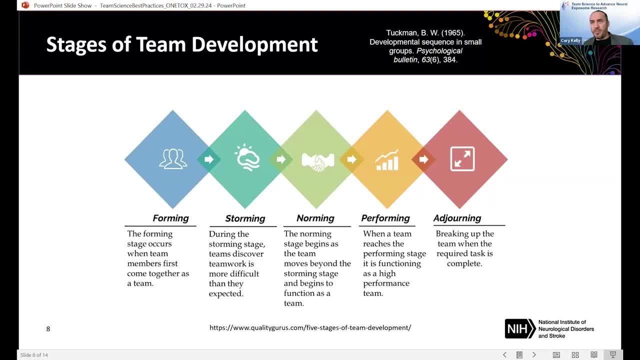 which is where you're really trying to figure out how your team dynamic is then is norming, which is, once you've kind of established the norms and the boundaries and the parameters of your collaboration, and then performing, which is where you're in the groove. 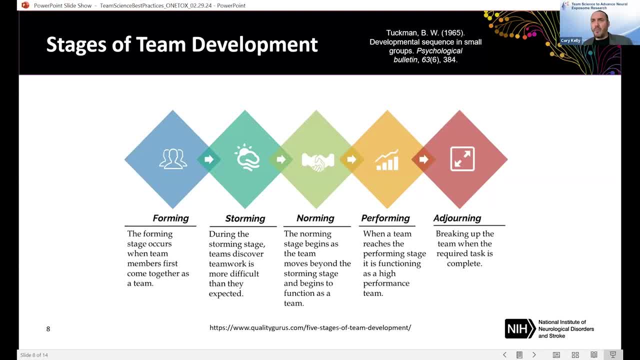 and you're starting to produce research products. and, lastly, adjourning, And this is that every team should be intentional: come together with a purpose and adjourn when the task is complete. So, now that we've talked about the team, 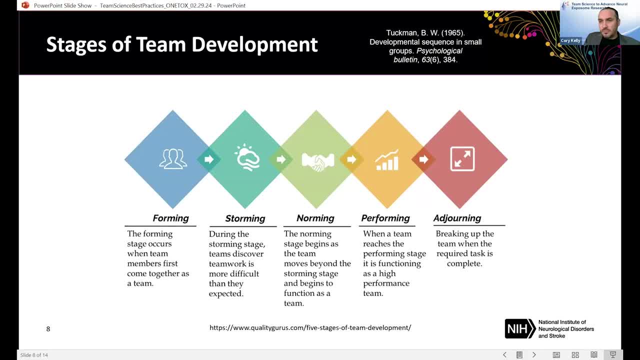 we're going to move on to the next slide. So the first thing that we're going to do is we're going to talk about the team And we're going to talk about the team. So we're going to talk about the team. 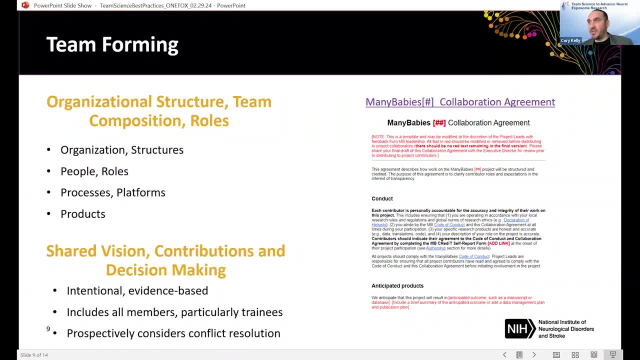 So we're going to talk about the team. So now we've discussed the foundational concepts and structure of team science programs. What are the best practices for team science implementation? The first practice is clear, organized organizational structure, team composition and roles. 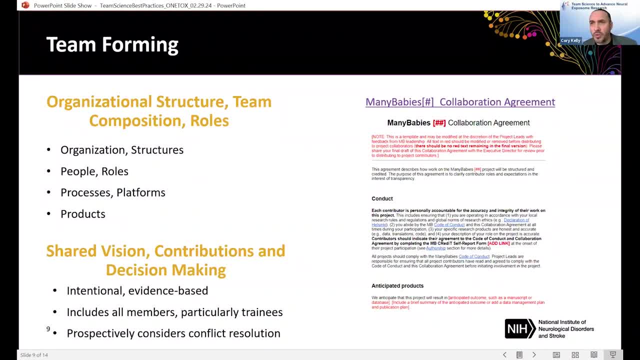 We say that the organization and the structure enables the people and the roles to utilize the platforms and processes to produce meaningful products. In the same light is shared vision, shared contributions and shared decision-making. Teams should come together for a specific purpose and requisite composition of the team. 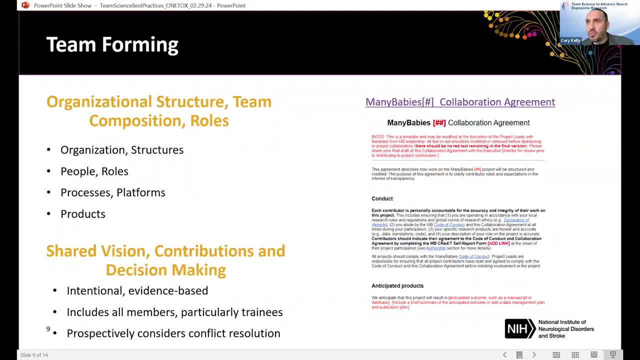 should be evidence-based. It should be intentional. Particularly for the Combine program, we very much want trainees to be involved not only in the conduct of the neuroscience but the team science, so that the future workforce is better enabled as multidisciplinary leaders. 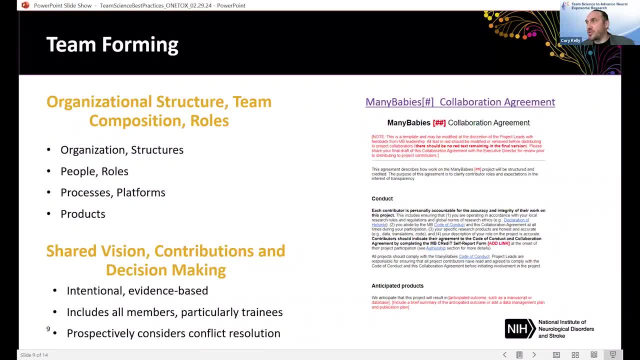 Last conflict is normal and often inevitable. Having conflict resolution plans in place prospectively is far more effective than trying to figure out what to do in the heat of the moment. An excellent way to support all these practices is to generate a collaboration agreement upon team formation. 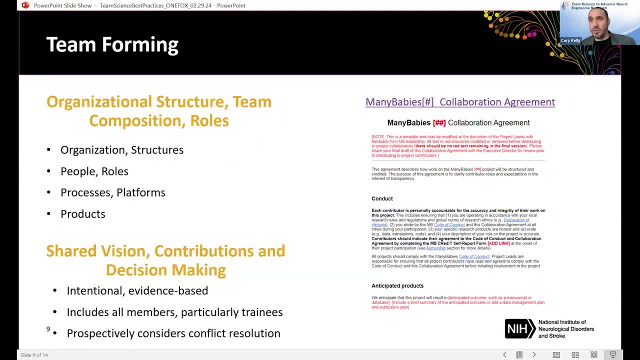 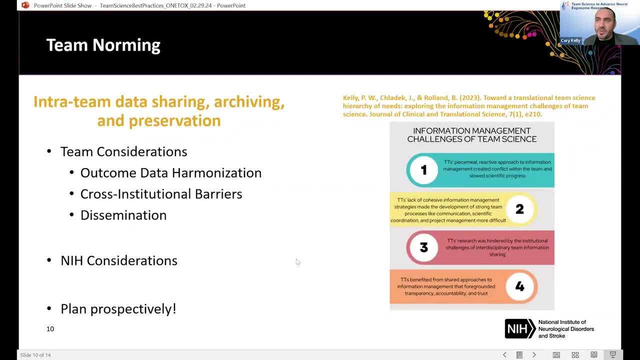 I've provided an example from the Many Babies project, which is a large team science or a big team science project. Data management and sharing is already a complex and sometimes a laborious task. that's further complicated in large collaborations. First and foremost, consider how you may need. 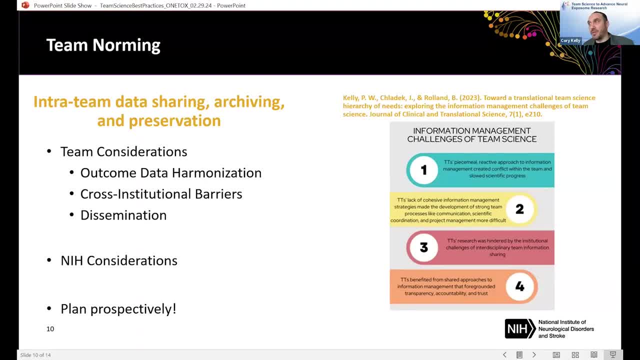 to harmonize outcome data from the various disciplines contributing to the project. Second, work early to identify cross-institutional barriers and have the requisite agreements in place. Third, consider how you may best disseminate these data to facilitate uptake and translation, Of course, as of 2020, we're still in the process of doing so. 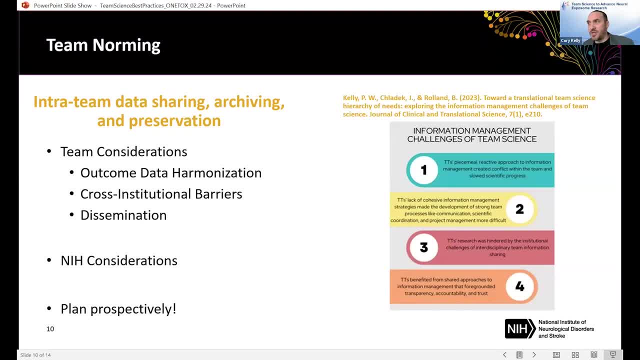 as of 2023,, the NIH has additional requirements for data management and sharing. We have an excellent NIN staff group in this space, and I encourage everyone to visit our NIN's website, where you can gain more information and potential repositories specific to neuroscience. 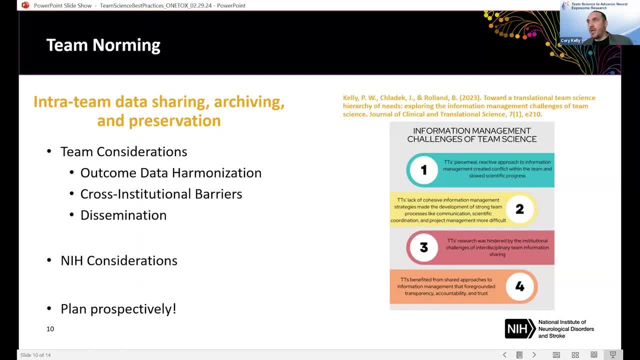 You can just Google NIN's data sharing and it should come up as a result. Last and most importantly, plan prospectively. The worst thing that can happen is you reach the end of a five-year award and you realize that you can't harmonize your data in a meaningful way. 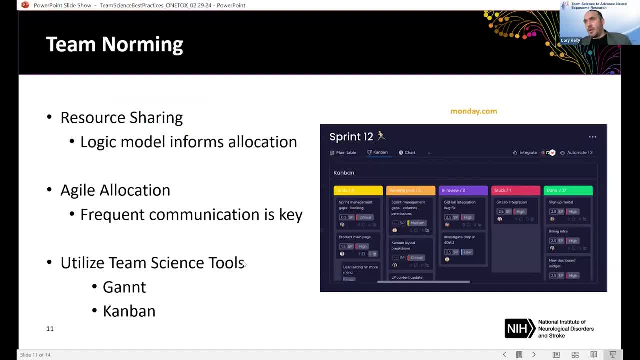 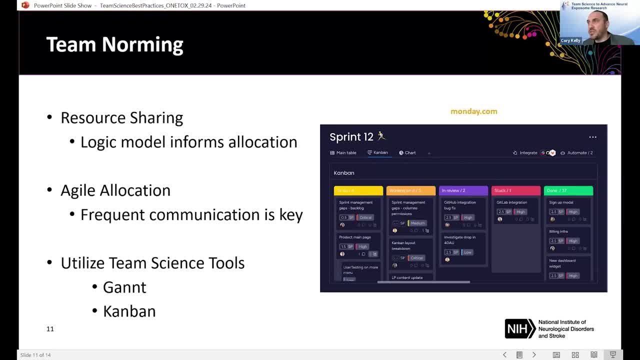 particularly for complex projects. The journey to the goal, the approaches, the expertise: it changes. Again, I encourage the use of logic model and the key performance indicators to inform where resources can best be utilized. Moreover, to achieve this level of agility, 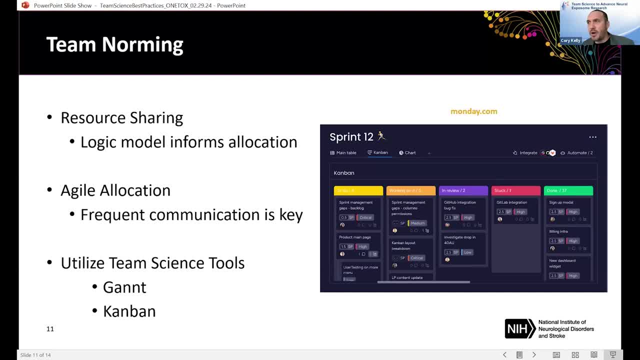 it's critical to have frequent communications with all members of the team to understand progress, barriers and next steps. There are many platforms to support effective team interactions, such as the Gantt chart that visualizes long-term activities and their dependencies, which is something 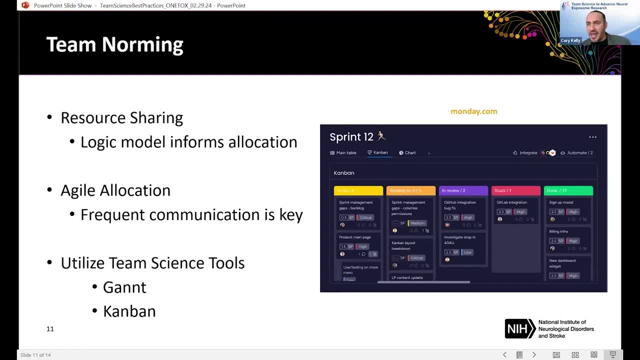 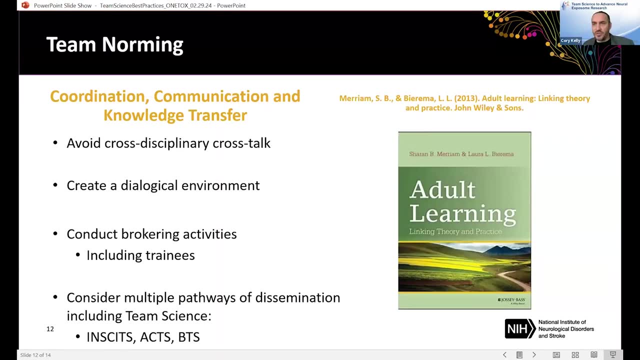 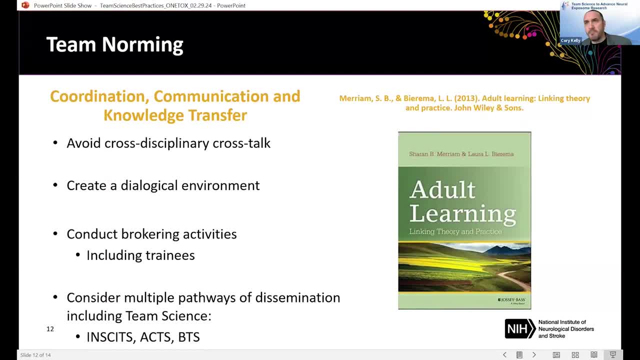 make the right adjustments more broadly, and what will determine their capabilities in the sense that the data remains aserel in its Кор такая relevant team science and even more relevant in this era of big data and multi-omics? First, it's critical to avoid cross-disciplinary crosstalk. 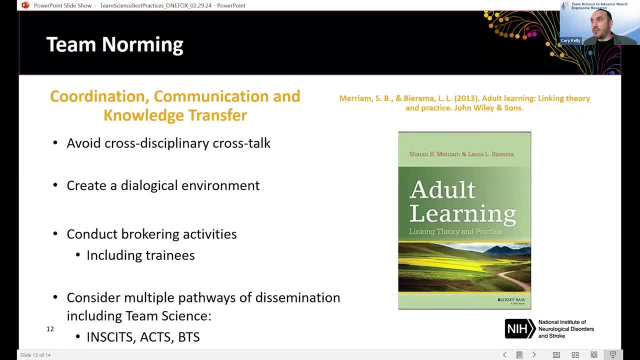 This occurs when there's a false assumption of a shared understanding between team members with different disciplines. Next, create a dialogical environment, a culture of interaction that's founded on conversations between team members rather than the traditional dictation between a team leader and a team member. 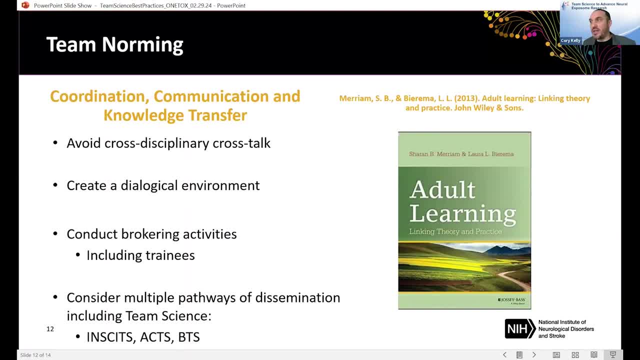 In this sense, thisリキ, you can make probing In this same vein, conduct brokering activities, activities that are specifically meant to facilitate conversations and transfer of knowledge, as opposed to activities that are simply for the implementation of the project. Last, cross-disciplinary research provides additional avenues for dissemination, including the field of team science, which very much seeks to learn from the lived experience of all fields. 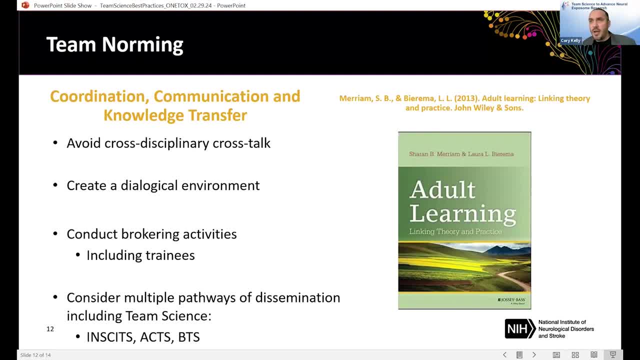 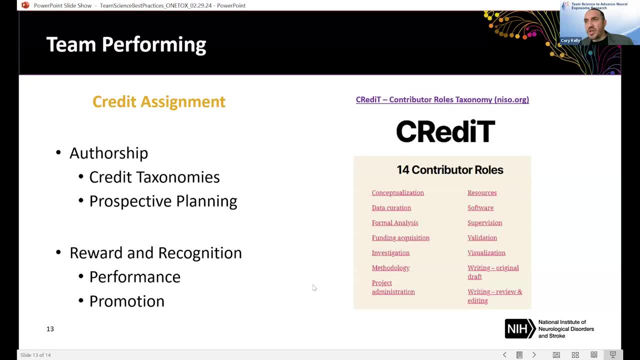 Some of these outlets include the International Network for the Science of Team Science, the Association of Clinical and Translational Research and the Big Team Science Organization. As teams begin to generate scientific products, credit assignment is often a source of acute conflict in scientific teams, especially in the era of collaboration. 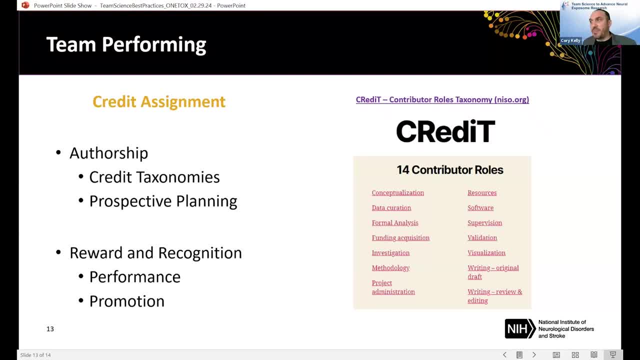 It is essential to adapt and utilize a credit assignment taxonomy that prospectively defines the roles and the effort to warrant credit on scientific products. Another of the pressing topics in team science right now is the recognition of team science and performance and promotion. RO1s and first author papers aren't necessarily the primary measure of success in team science. 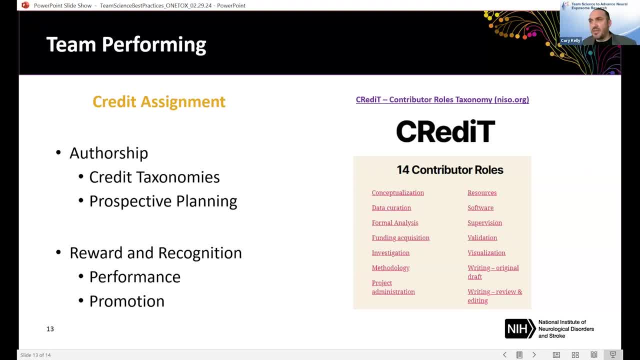 And we need to begin to work. We need to take away the merit of team science alongside these traditional measures. This is really a call to action to all scientists and all administrators, whether leading a lab, a department or an institution, to think about how we can recognize and celebrate these collaborative successes just as much as individual performance. 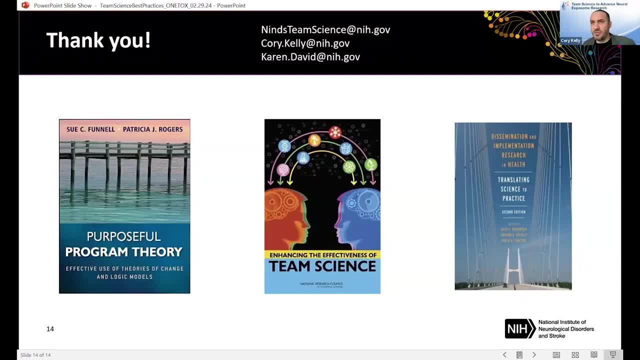 In summary, how do we develop and conduct team science to achieve meaningful change? We start with purposeful program theory to establish probable causality. We then rely on implementation and dissemination to ensure fidelity of the program and uptake of the findings. We then use team science to work together to achieve the goal and that this team can work together effectively. 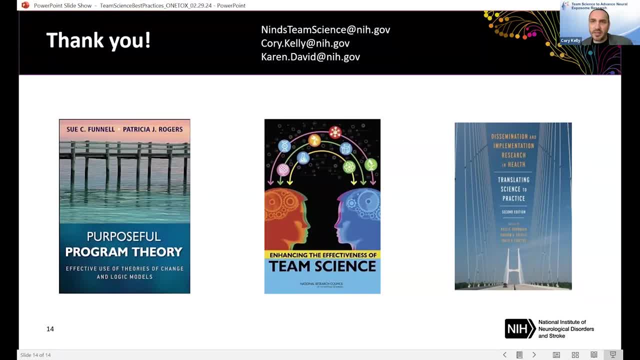 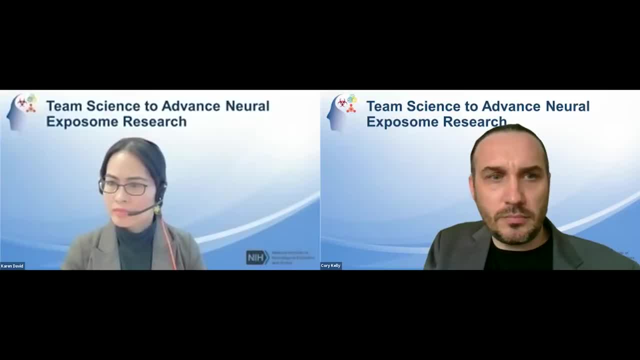 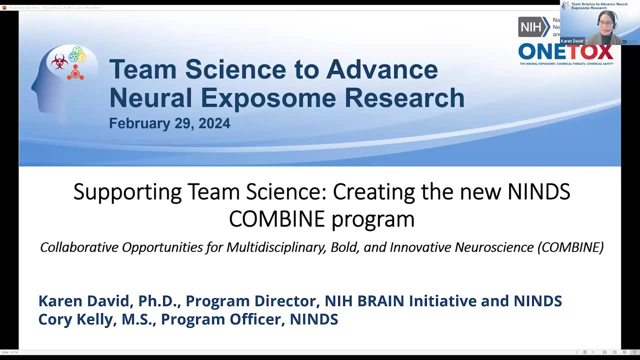 Thank you, and you can reach both Karen and I at NINSTEAMScience at NIHgov. Great Thank you, Corey. Share my screen. Good afternoon everyone. I'm Karen DeVede. I'm a program director at NINDS and the NIH Brain Initiative. 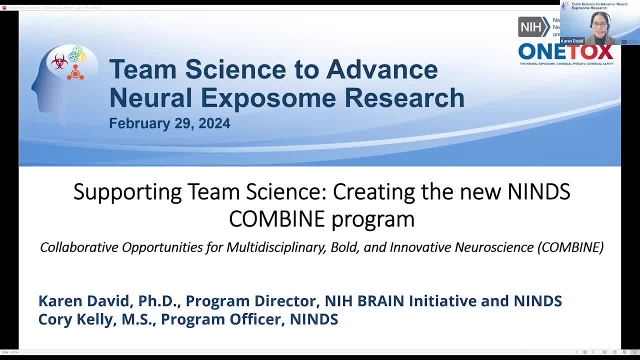 I'm a program director at NINDS and the NIH Brain Initiative And, following Corey's talk on considerations regarding team science, it's my pleasure to describe to you our new team science program at NINDS and how this program came about. So my colleague Jim Knott and I led our NINDS team to create this program, and the resulting team science program, called the combined program, is currently led and managed by myself together with Corey Kelly. 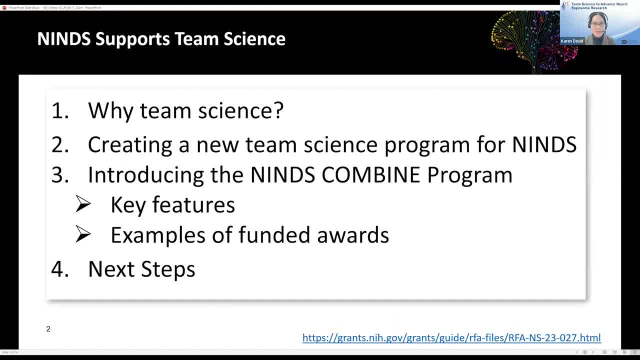 So first I'll talk about why are we supportive of team science, Then I'll walk you through the thought process behind designing our new team science program for NINDS and I'll be highlighting its features. In this way I can note to you the elements that we consider to be important for collaborations, to increase the likelihood of success. 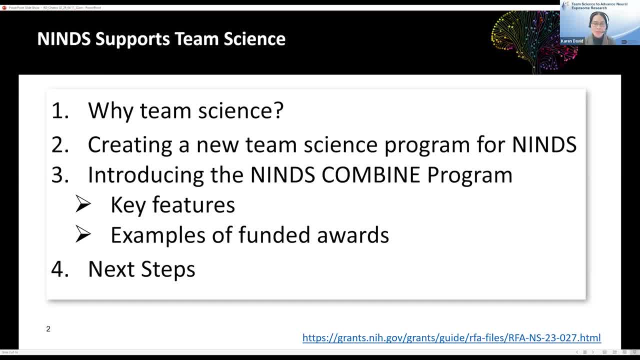 And this can also inform us how we can go about in combining or integrating disciplines to advance neural exposome research. So we're also excited to have with us today our panel of speakers whom we draw inspiration from regarding our team science practice, And I'll point out in my talk which aspect of our thinking is related and informed by findings from our speakers today. 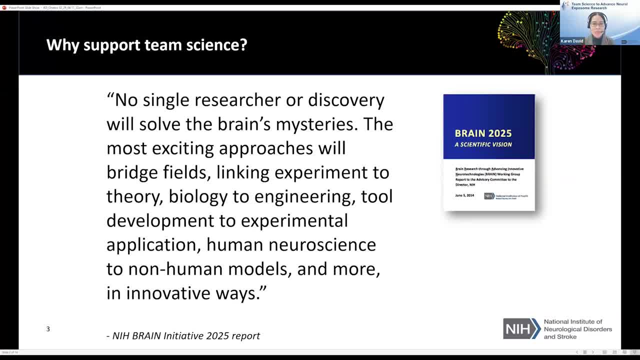 So, first, why team science? We very much identify with this quote from the NIH Brain Initiative 2025 report highlighting the importance of collaborations. No single researcher or discovery will solve the brain's complex mysteries, and the most exciting approaches will be interdisciplinary, bridging and combining distinct expertise and disciplines. 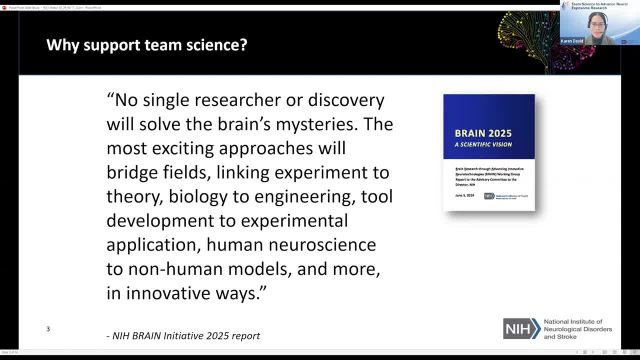 So a team science approach affords us the opportunity to extend beyond the limitations of a single lab effort, and it enables us to tackle neuroscience problems in a more comprehensive, rigorous and mechanistic manner. And so, given the importance of team science, we set out to create a new team science program for NINDS. 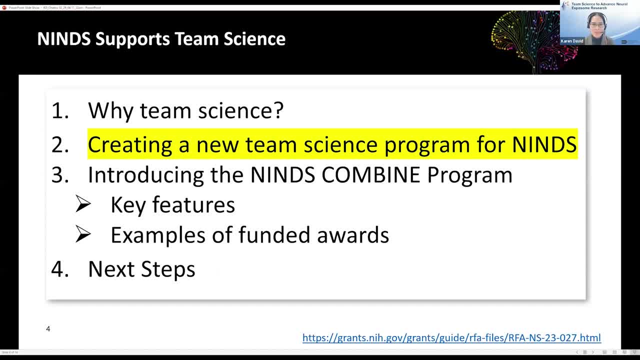 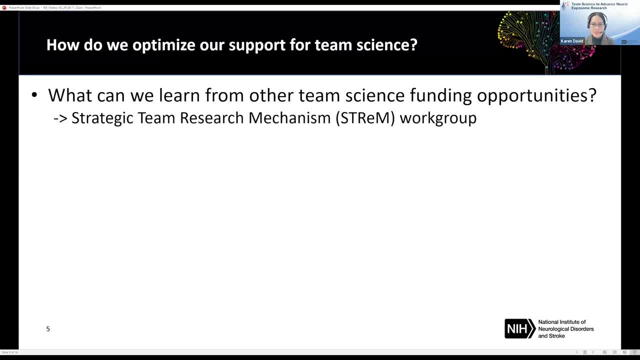 So first we started by asking how do we optimize how NINDS supports team science? And to answer this, our Strategic Team Research Mechanism Working Group compared and contrasted how other institutes, programs and funding agencies support team science, so that we can learn about the best practices and challenges associated with team-based approaches. 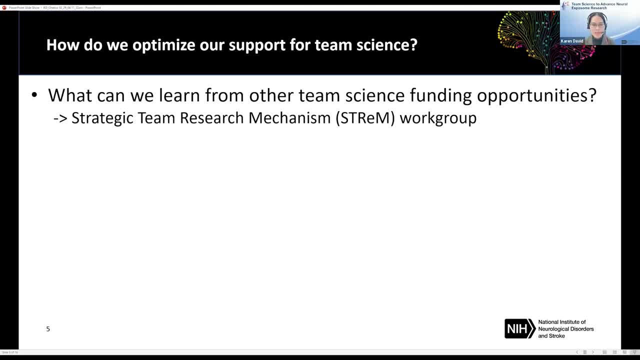 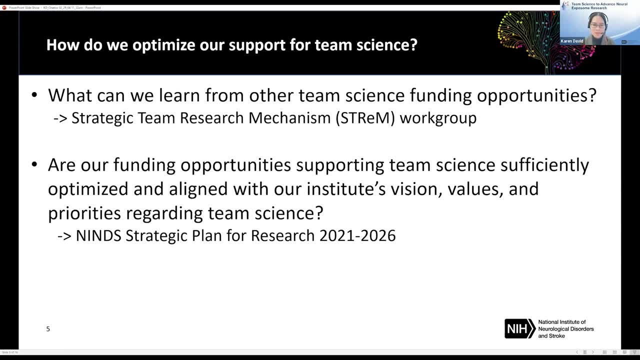 We were also driven by the goals outlined in the NINDS Strategic Plan for Research, which recognizes the importance of supporting team science of broad scope and complexity, And we would also like to further mobilize the scientific community to collaborate to leverage their diverse expertise. 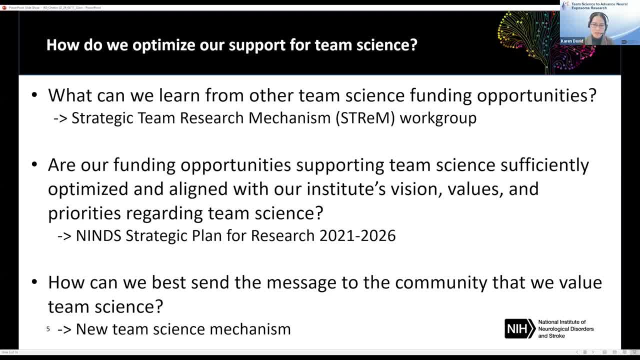 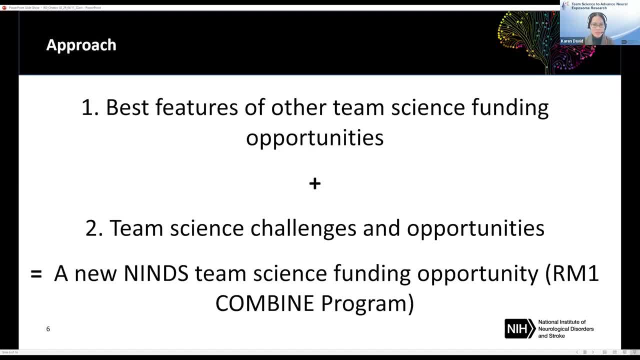 and to take advantage of the increasing knowledge base and technological capabilities in various fields, And so we set out to design a new team science funding opportunity for NINDS, And our approach was to take the best features of other team science funding opportunities and discard what we don't want. 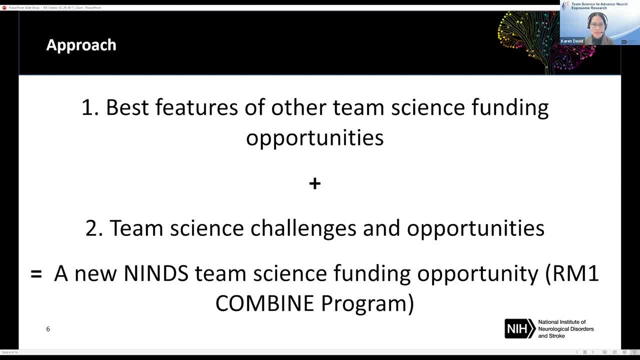 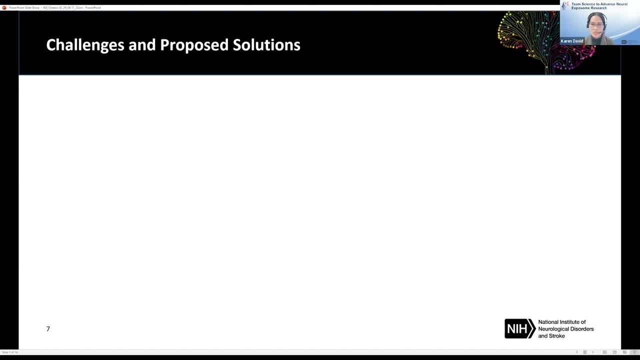 and also to learn from our collective experience with various team science programs regarding the challenges and opportunities associated with team-based approaches, And so we built this new combined program using our lessons learned from other funding mechanisms. For example, some of the projects we've supported did not achieve the extent of integration that we envisioned. 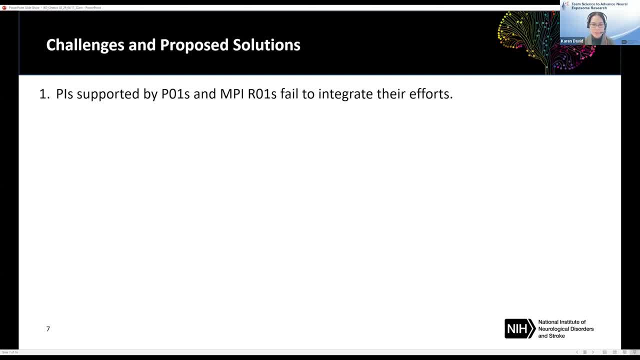 Some are a collection of projects or parallel efforts rather than an integrated effort across the PIs, And some seem to be large R01s driven by a single PI with sidekicks. So towards this, inspired by the NIGMS RM1,. 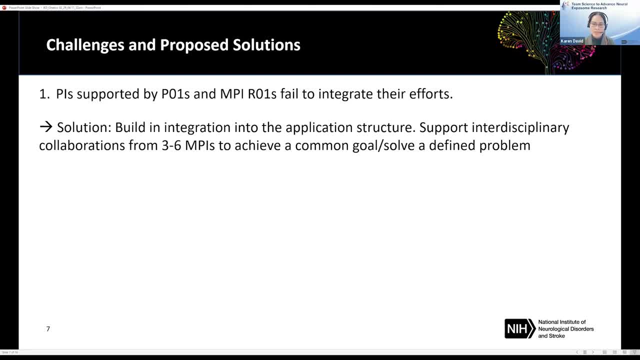 our combined program emphasizes interdisciplinary collaborations: from three to six PIs who will work together, converge their expertise to solve a defined problem. And also we've noticed that some team-based efforts suffer from poor team management, which negatively affects the science. So we consider having a well thought out team management plan to be very important. 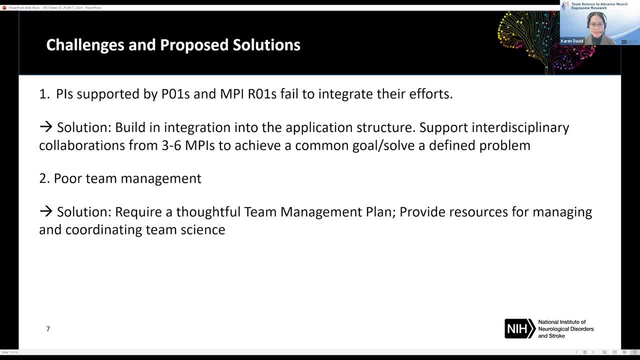 And I'll talk more about this in the next slides. We also would like to set these teams up for success by providing the resources and infrastructure needed for managing and coordinating these efforts. And, lastly, team science efforts are a great opportunity for us to promote diverse perspectives in the team. 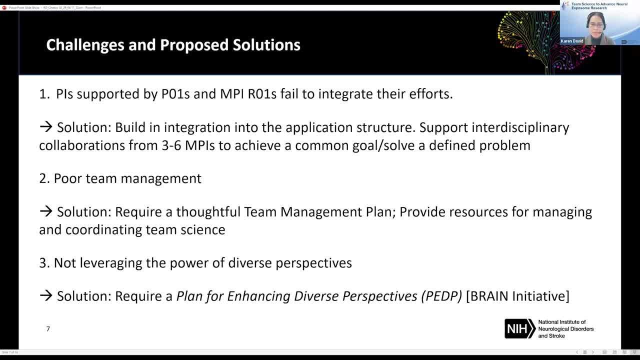 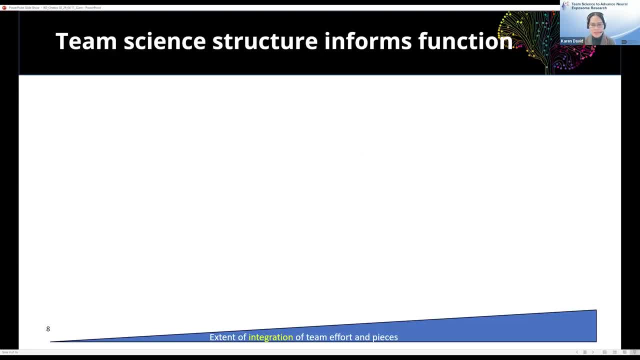 And so we are borrowing from the NIH BRAIN Initiative. this required attachment of a plan for enhancing diverse perspectives, And another observation about team science that stood out to be particularly important for us is that the team science structure informs function as well as the extent of integration across the efforts of the PIs. 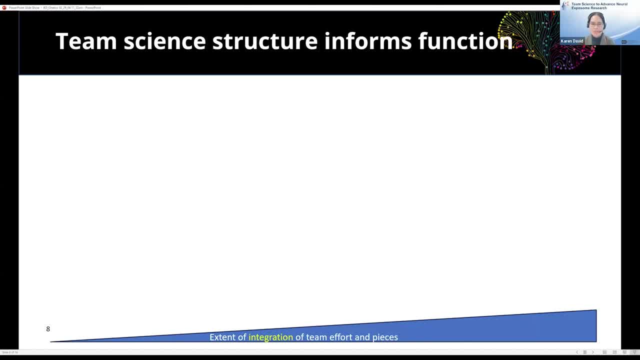 So what do I mean by this? To illustrate, I'll be going through an overview of the differences across the current ways. that NINDS supports team science, So the blue circle here is meant to symbolize a single project or component, And so for the P01 program project, we depict its multi-component structure, where you have some number of projects plus course. 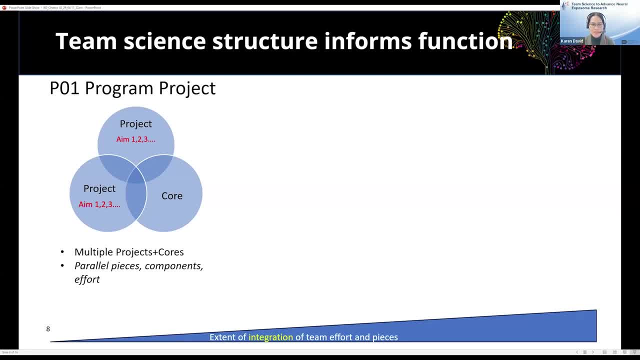 and these components will have interrelated and parallel goals, And the consequence of this structure is that it promotes parallel, distributed and interrelated efforts across the PIs rather than a fully combined team effort. And there's another way to get collaborations funded at NINDS, and that's through a mechanism that most of us are familiar with, and this is the parent R01.. 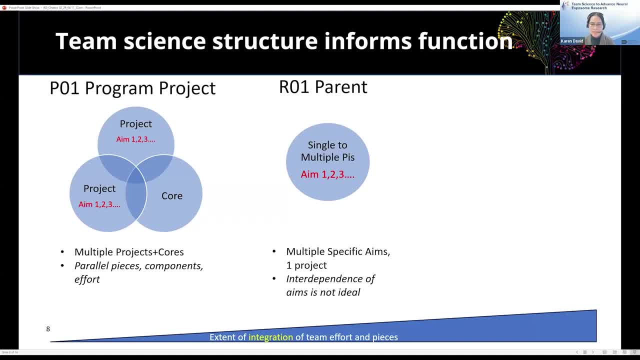 And, in contrast to the P01, this will be a single project with multiple specific aims. So this R01 can come from a single lab or a collaboration from a multiple set of PIs. And what we've noticed? that although the R01 is a single project, we still could not get the extent of integration that we wanted. 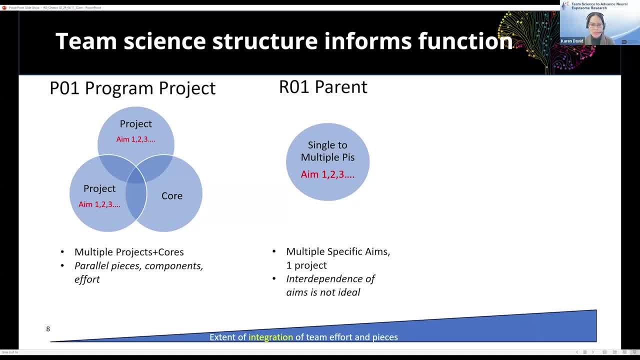 because the PIs have to structure their project into multiple specific aims, And this is because the usual assumption is that specific aims need to be independent rather than interdependent. And so, for the R01 combined program, our goal is to achieve a degree of integration currently not possible with these other mechanisms, such as the P01 and R01.. 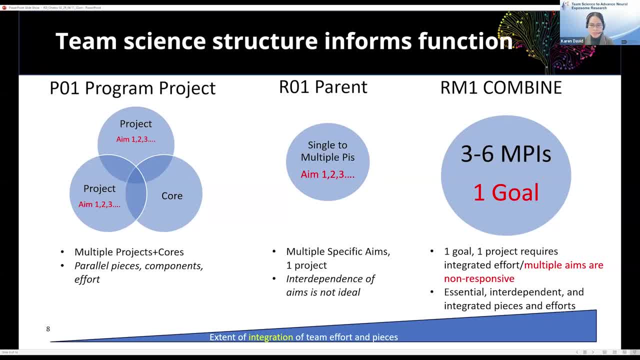 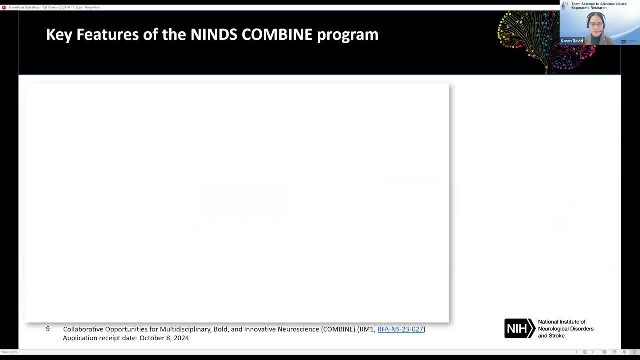 And the way we were able to achieve this is: we asked for a single focus goal that, by design, would require the merging or combining of disciplines to be achieved, And also we freed up the PIs from the constraints of a specific aim, And this is the resulting product. So here we summarize the features of our new combined program. 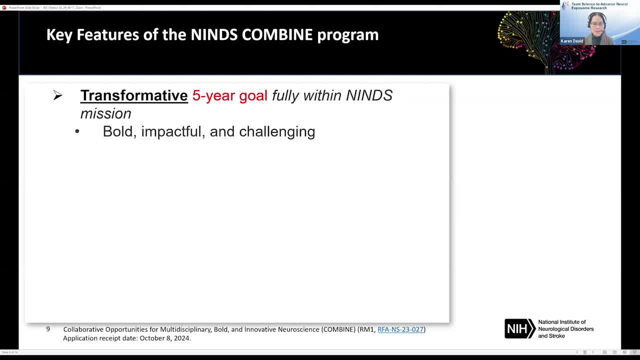 So we consider team science to be powerful, And so we expect that the goal proposed is bold, impactful and challenging, and achievable within the funding duration of five years. We also emphasize that teams work towards a single focus goal and not propose a collection of independent pieces or aims. 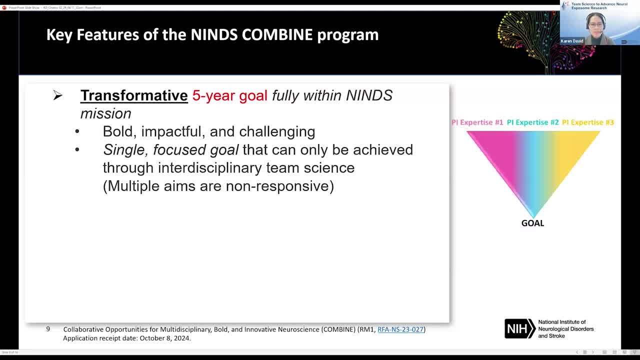 So we want a goal that can only be achieved by the combined efforts of three to six multiple principal investigators, each with a distinct and essential expertise, as well as adequate bandwidth and equivalent efforts. We also expect that projects are of a larger scope and of more complexity than what you would typically see in a parent R01.. 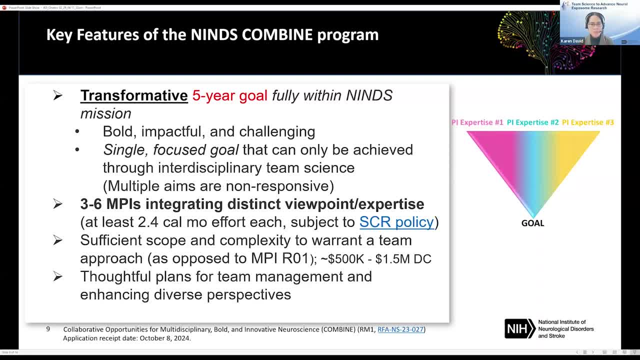 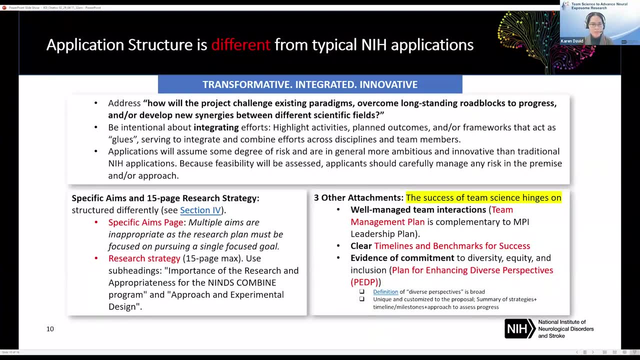 And because team science is a social activity, we're also looking for thoughtful plans for team management, leadership and coordination and for plans for enhancing diverse perspectives. And also the structure of the application reflects our priorities. So first and foremost is the science, And we recommend to applicants to make sure to describe how their work is transformative, integrated and innovative. 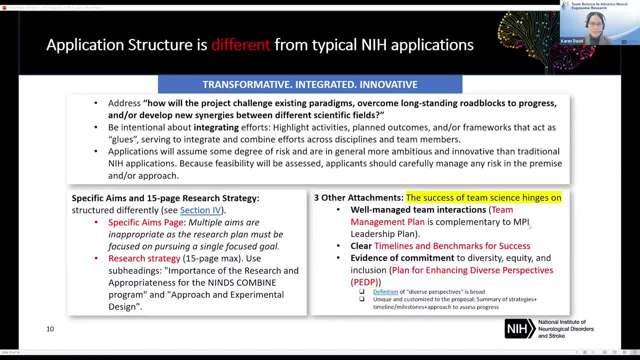 And the application also requires three other attachments based on the considerations that we find are important in increasing the likelihood of success. The first: we ask for a thoughtful plan on how the team will be managed and led. And second, we ask for a timeline and benchmarks for success, And this will be the team's roadmap to success. 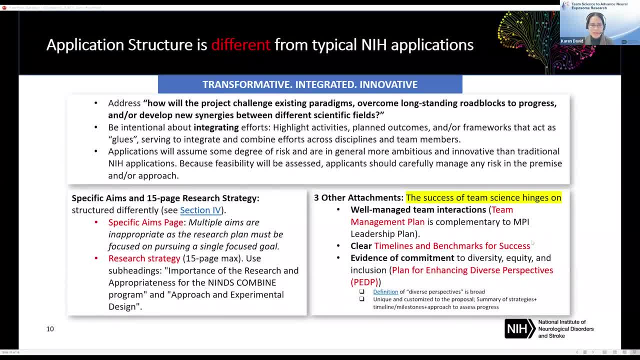 And third, we ask for plans on how to capitalize on and enhance diverse perspectives through this project. So I'll be going through what these attachments entail, because these are important team science considerations regardless of the funding mechanism. So team science needs effective leadership, management and coordination to be successful. 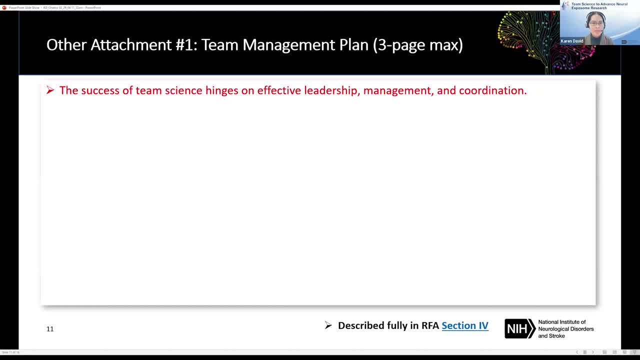 And, although team science promotes cross fertilization across disciplines, the actual practice of bringing people from different backgrounds together to converge their expertise. This brings several challenges, especially in disciplines with our own specialized language, So we recommend to applicants that they consult this document that NCI put together with practical suggestions such as, for example, having a collaborative agreement template that you can find in the appendix. 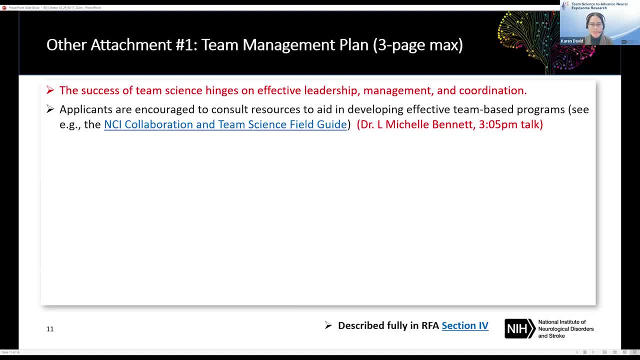 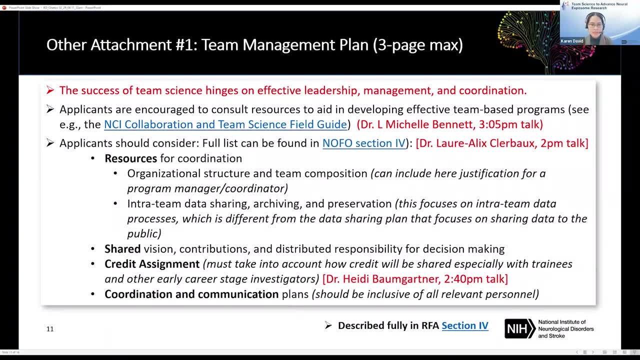 And we're very pleased to have with us today Dr Bennett, who co-authored this field guide, And I'll just point out here other important considerations when building a team. So we have the funding opportunity, and Corey talked about some of these points. 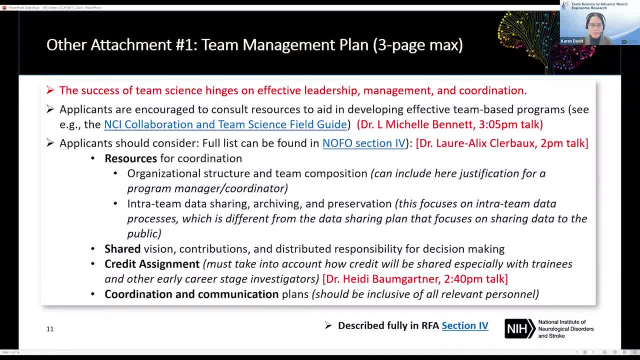 And this list is informed by the NIGMS, RM1, the NCI field guide and from our experience with our funded teams, And we look forward to hearing from Dr Clairvaux about some of these team coordination elements and resources that facilitated her large team collaboration. 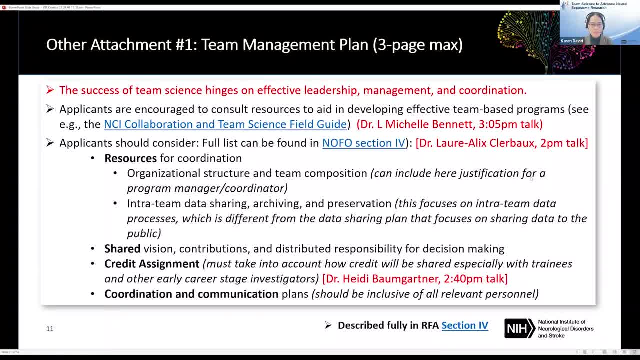 So in this document, here is where the applicants can ask for the support that they need in running the team. So, for example, this is where they can include justification for a program coordinator or manager, as well as other needs that may arise. 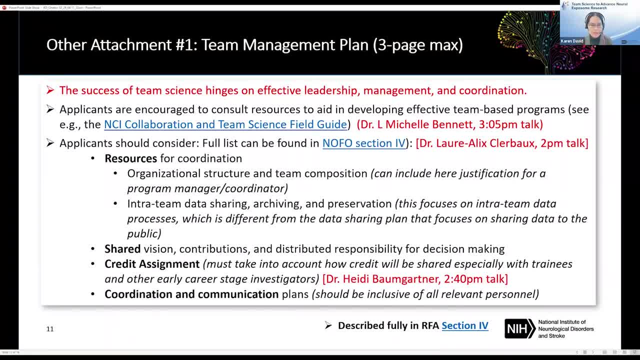 For example, Corey Kelly talked about data management, And so this is where you can ask for resources for data management across labs. You can ask for professional staff, if needed, to help make that multimodal or multi-scale data talk to each other or have it be accessible across labs and by the greater community. 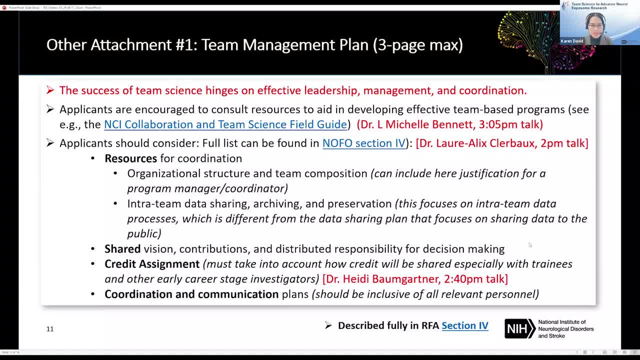 And there's also the challenge here of credit assignment and authorship policies, especially with team effort, And so we look forward to hearing from Dr Baumgartner about her experience and useful tools to navigate this challenging issue, especially that our trainees and early career stage personnel have to navigate the individual focus nature of incentives in science. 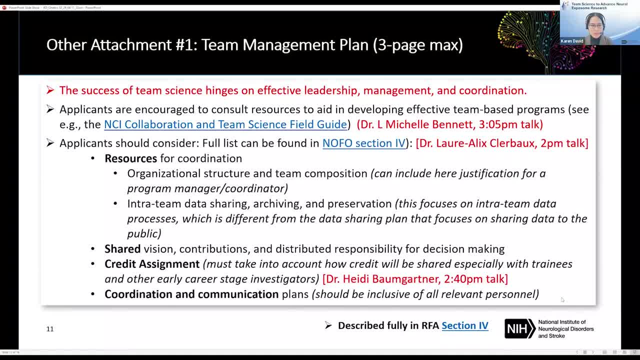 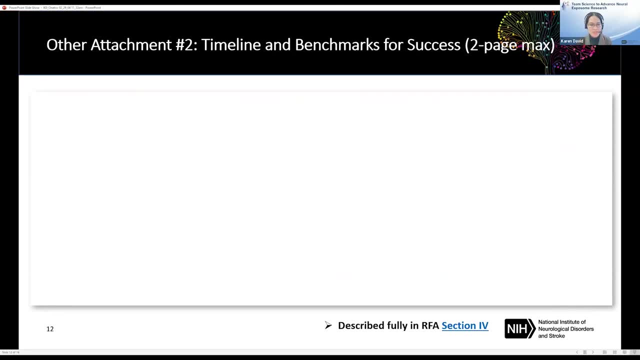 And also we've asked applicants to consider the practicalities and logistics in coordinating and communicating across the different team members. So, overall, these are important points to be thinking about when planning a collaboration, regardless of the funding opportunity. Okay, so the next other attachment we asked for is the timeline and benchmarks for success. 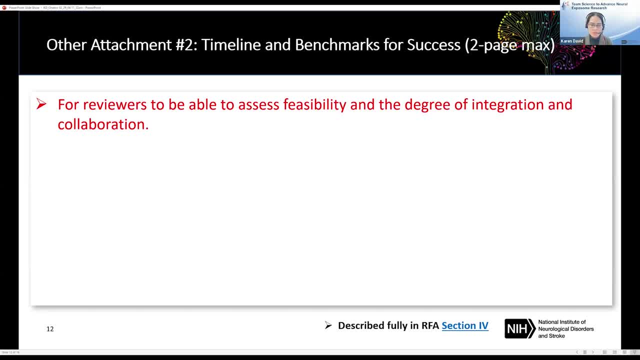 And this is for reviewers- to assess the feasibility as well as the degree of integration and collaboration. So this serves as the roadmap to success for the team And it includes a timeline and chart noting the tasks and benchmarks, as well as points of integration. 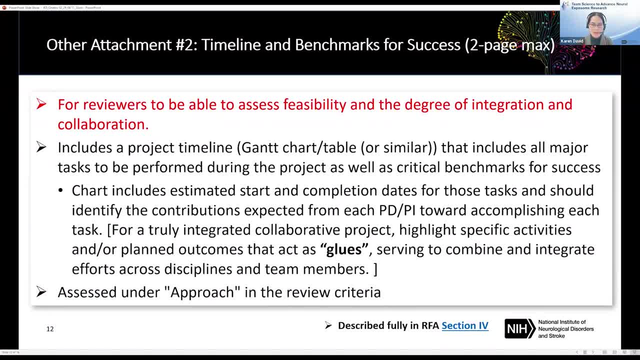 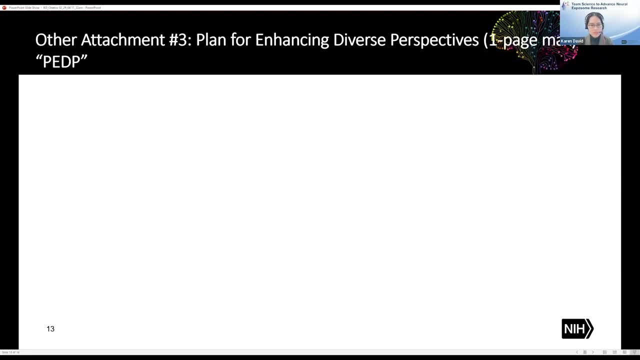 So for collaborations, it's really clear that the team members are very much aligned with what they consider to be benchmarks for success collectively as well as for their individual contributions. And the third attachment that we asked for is the plan for enhancing diverse perspectives, and this was pioneered by the BRAIN Initiative. 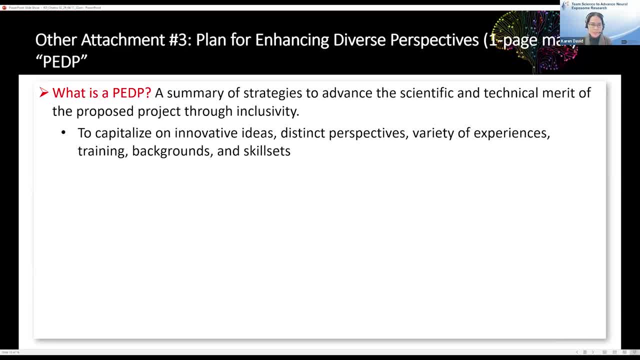 And the motivation for this is to capitalize on what diverse perspectives have to offer. So PEDP is a summary of strategies and activities by the team to advance the merit of the science through enhancing inclusivity. And our definition of diverse perspectives is broad, and this includes diverse perspectives from those doing the research. 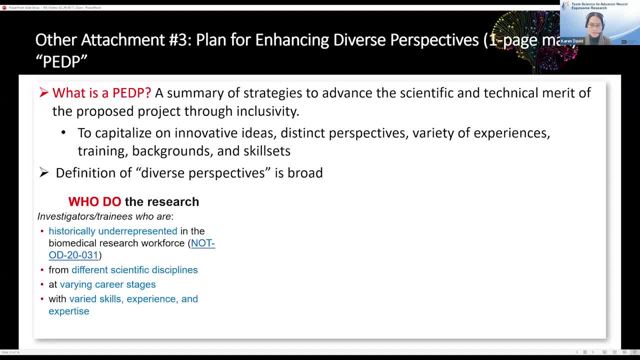 For example, those who are underrepresented from different scientific disciplines, career stage, backgrounds and so on, could also come from those participating in the research. For example, who's being recruited in your human neuroscience studies, or where are the specimens coming from, how is it obtained, and so on. 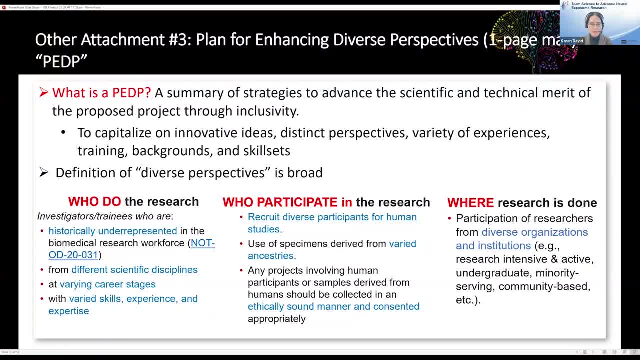 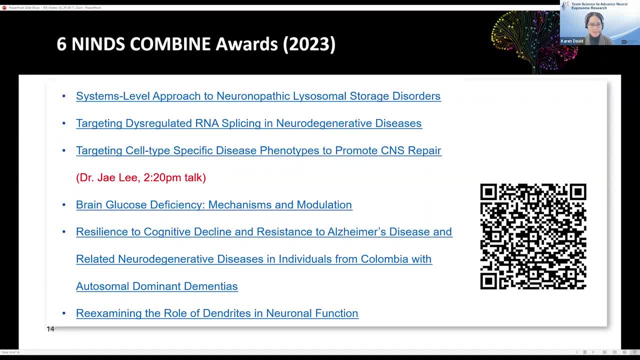 And also where the research is being done, and this could be reflected in the different types of institutions. So we're very excited to share that we've awarded our first set of combined projects, and the diverse topics covered include basic research, translational research and various disease topics. 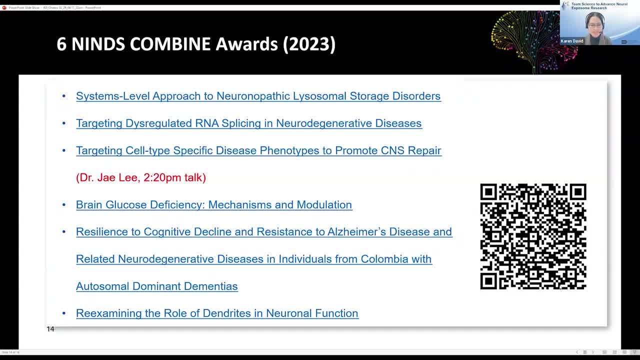 All of these integrate different disciplines and I recommend checking out this list using this QR code. And we're grateful to have one of our RM1 combined teams join us today to talk about their combined project. So thank you, Dr J Lee. 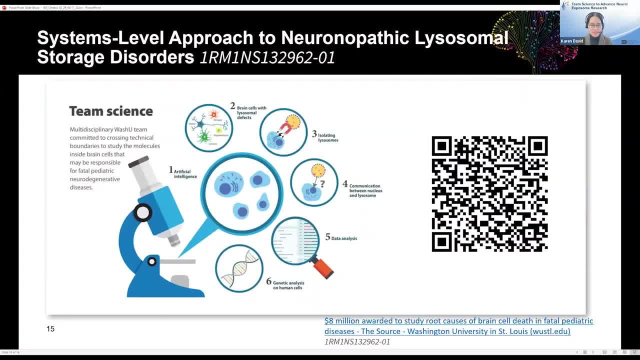 And one other project I'd like to highlight is this one that released a nice summary of what it's about, and here's the link to the article. So here we have six teams bringing together scientists in pediatrics, genetics, bioinformatics and psychiatry to understand how and why cells die in two lysosomal storage disorders that affect the brain. 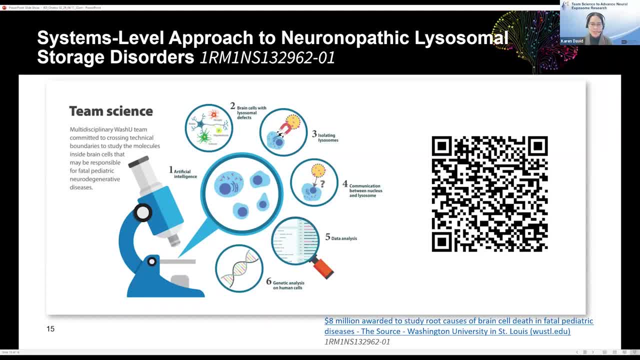 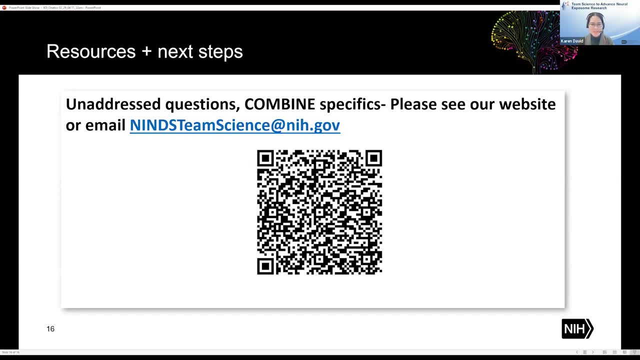 So the central hypothesis that's gluing them together is that they hypothesize that it's the changes in the communication between the lysosome and the rest of the cell, rather than the storage-related issues itself, that is driving the disease pathogenesis. So thanks again for having us, and hopefully we're able to tell you about what we consider to be important in collaborations, as well as describe to you the potential challenges to anticipate regarding team science. 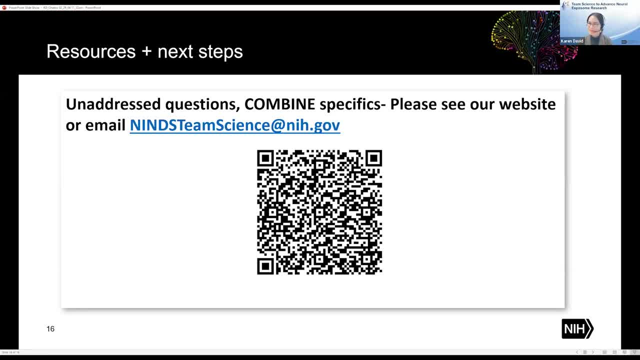 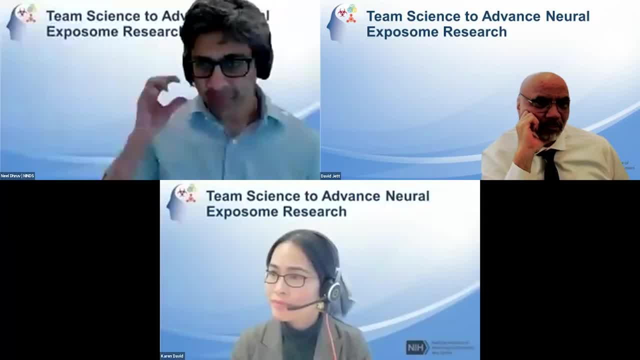 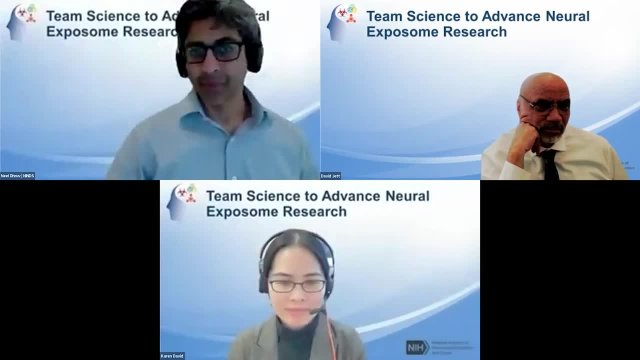 So that's it from us. Thanks again. Okay, thank you very much, Karen and Corey. We have time for a question. I don't know if there's anyone any of the panelists have a question? While we wait, I'll ask one that came in through the chat and that is: 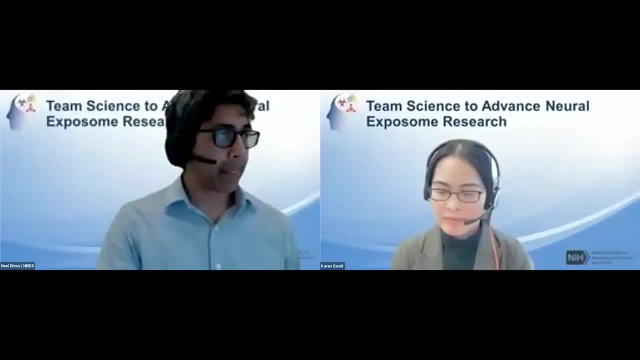 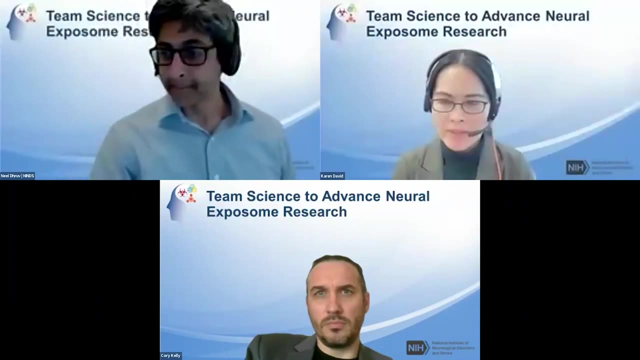 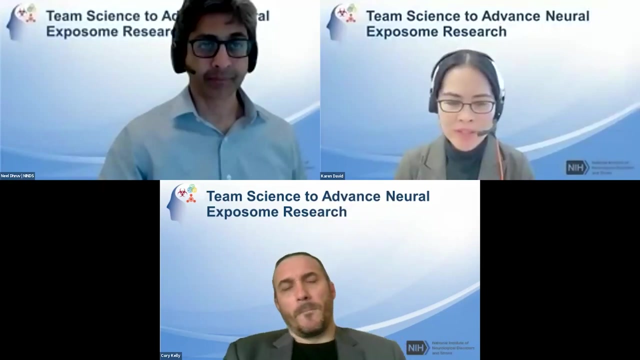 Karen, can you elaborate or expand a little bit on what you mean by data management? Okay, thank you, and Corey Kelly will chime in too. So the data management that we talked about- that was also drawing from our experience from our Brain Initiative teams- is where you have, for example, very diverse data set that needs to be combined together or shared across labs. 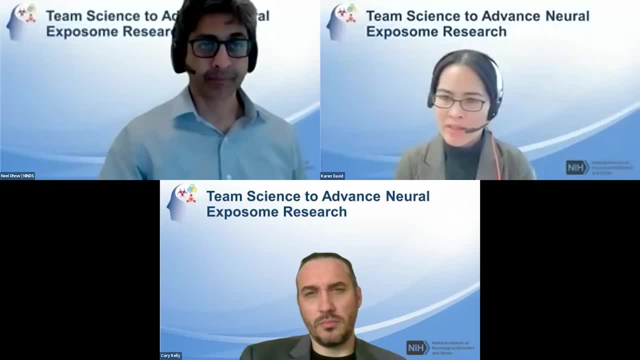 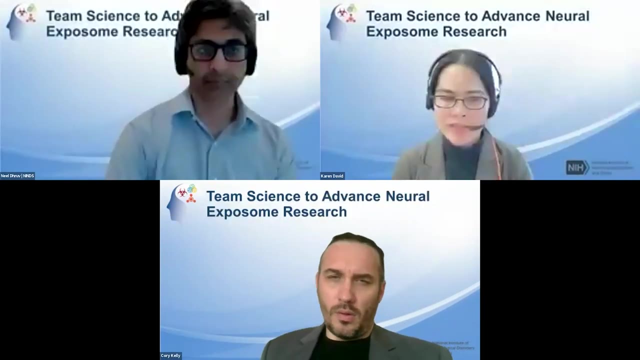 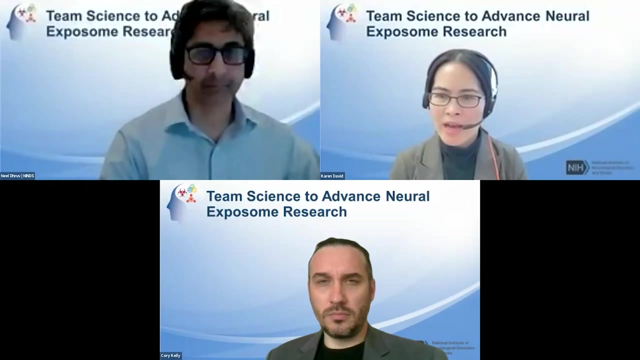 And that kind of infrastructure needs to be built and it's not available anywhere else, because it's also peculiar to the type of data set that you're trying to integrate. So we allow for those kind of resources to be asked for in the combined funding opportunity, because these are something that needs to be worked out from the ground up and hopefully, how these data sets are integrated could be informative to other types of science that will need to integrate these diverse data sets. 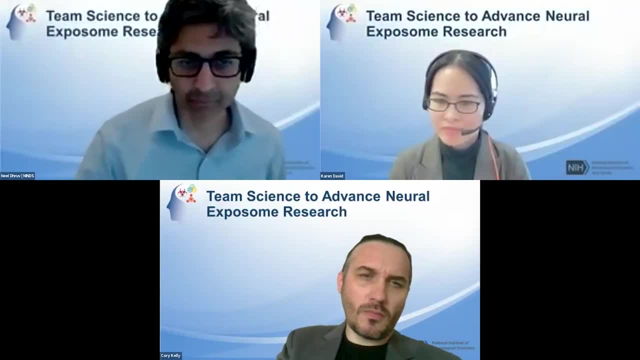 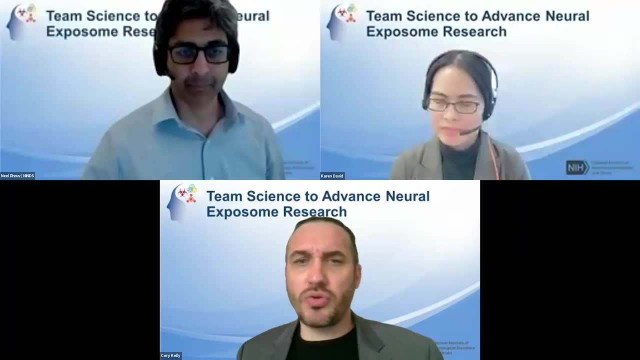 Corey. Yeah, thank you, Karen, And thank you for the question. Perhaps I can give an example from my extramural career. I worked in neurological surgery research. What we did was we used intravascular ultrasound measurements of blood flow and combined those with computational models and genetic models. 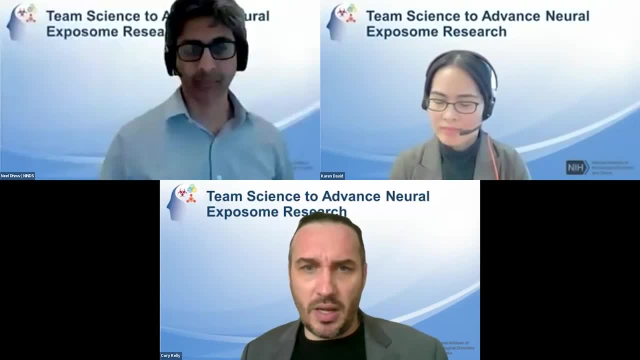 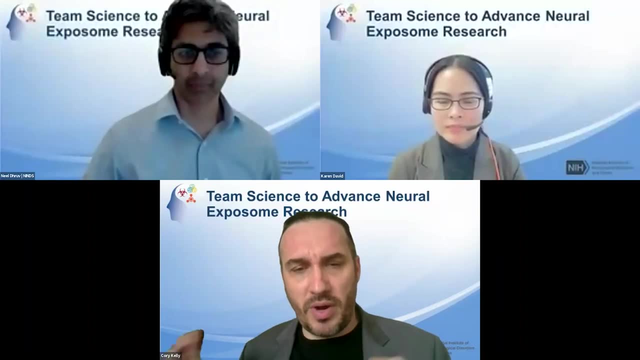 And so what we had to figure out was how do we harmonize these data so that the engineers are utilizing our images correctly, so that their models are set up with the correct parameters, And how can the geneticists and the biologists match their in vitro experiments with 3D modeling of blood vessels to align all that together? 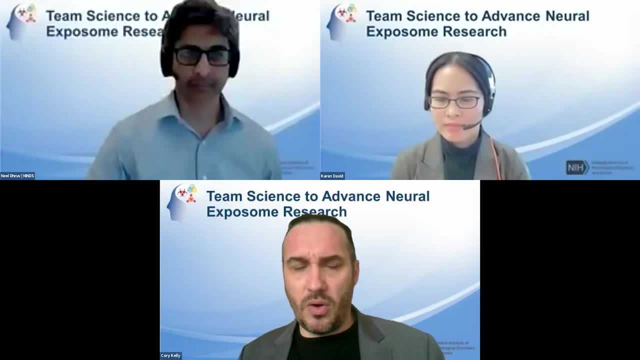 And so we first had to think about how are we going to bring this data together and integrate it and harmonize it, And then the other aspect of that is we had to figure out simply just how are we going to share this data among labs that are in different locations, in different fields. 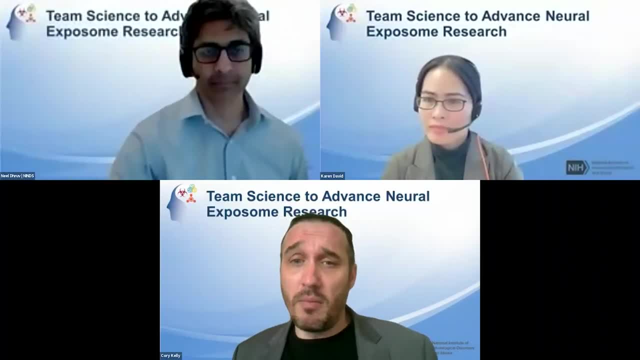 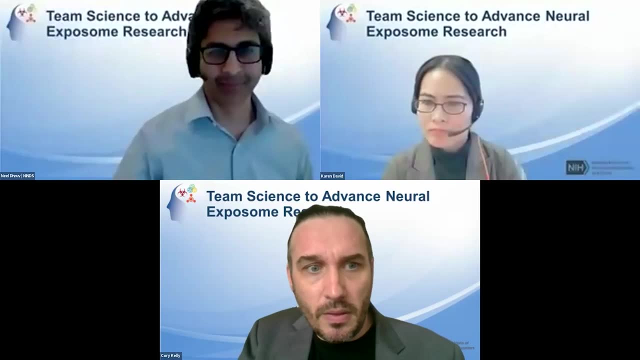 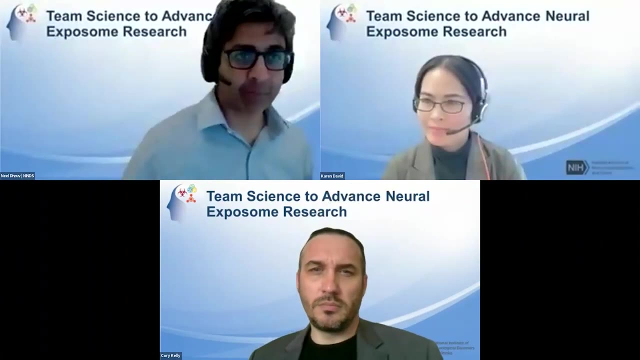 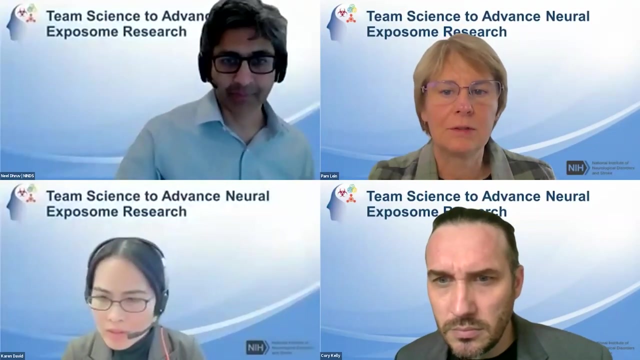 And ultimately we decided our solution was to purchase our own network-attached server where we had complete control and fluidity of the data between the labs. That's great, Amazing, Amazing solution. Pam, you have a question If you address this and I missed this, but did you set up special emphasis panels to review these combined grants? 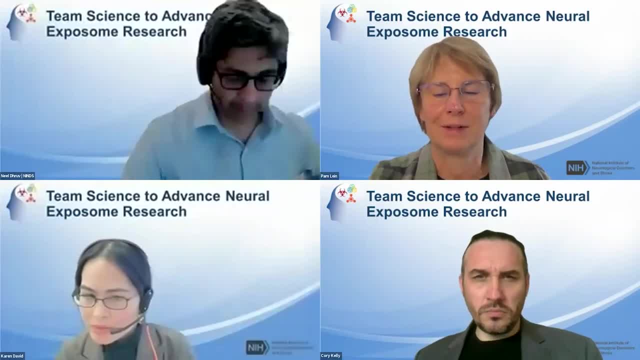 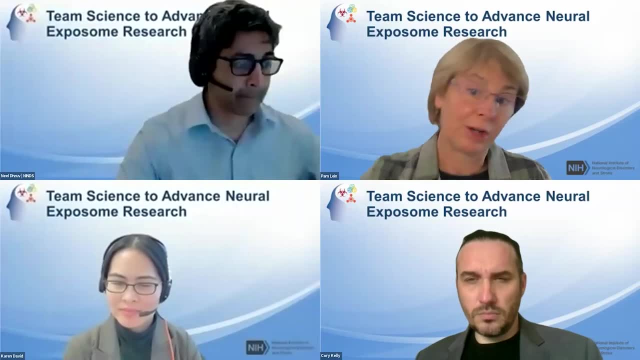 Because I think one of the questions or issues that the working group is kind of grappling with is obviously going to team science. The traditional study sections aren't necessarily trained in how to evaluate that kind of science, So any comments you have on that would be much appreciated. 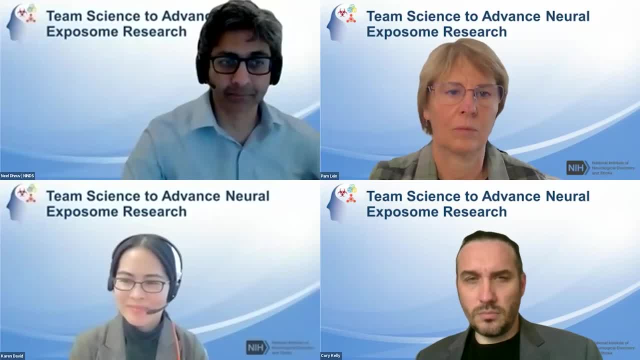 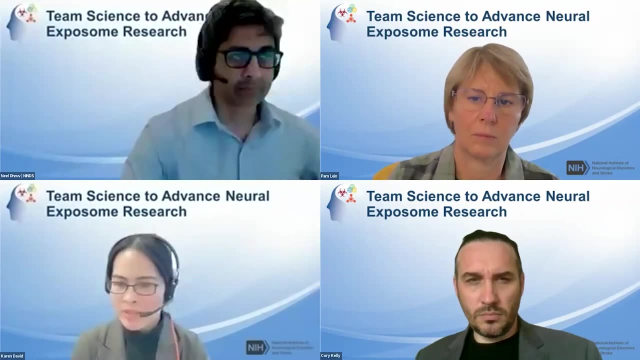 Right- And I can't emphasize it enough- that the need for a special emphasis panel, because this is a unique program with different set of priorities And we're also trying to go against, for example, what's typically accepted or how do you regard an apparent R01,, for example? 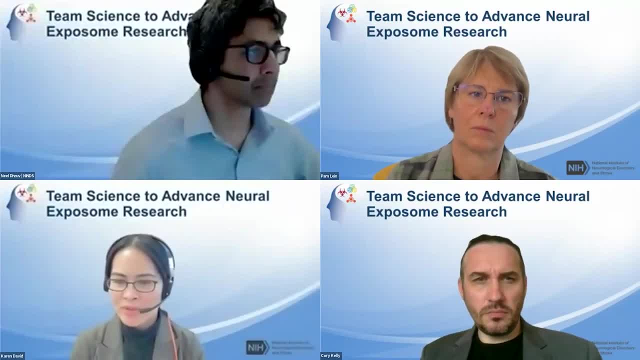 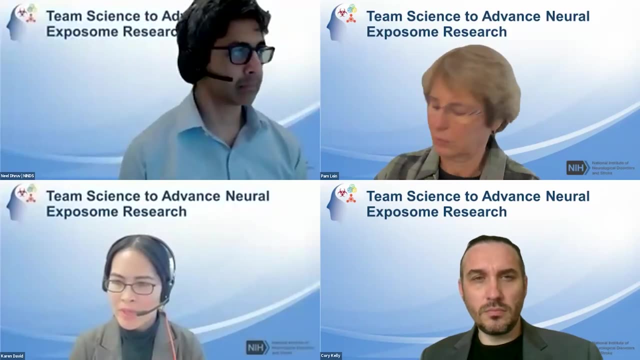 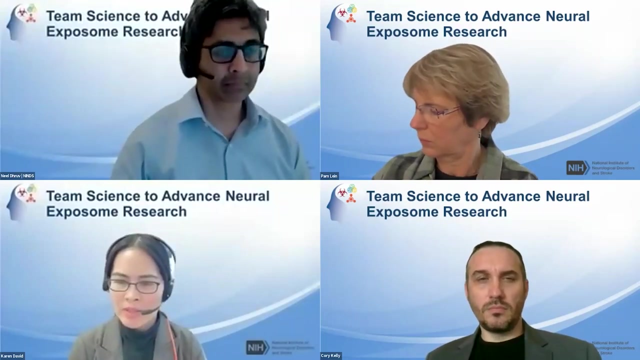 So we want reviewers to stop thinking about that, because this is not business as usual. So we do have a special emphasis panel and we do reviewer orientations before the review as well as a reminder of what priorities are on the actual review. And this also what works for us is our strong partnership between program as well as our wonderful SRO, because these are very 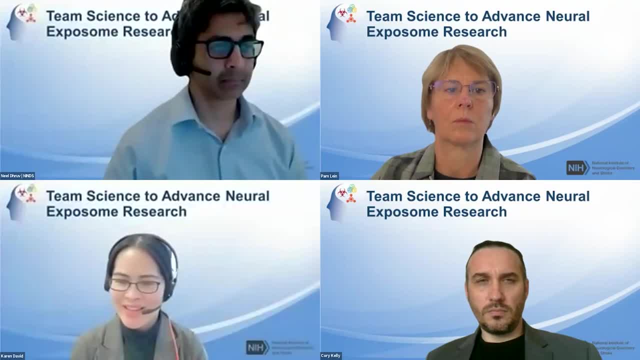 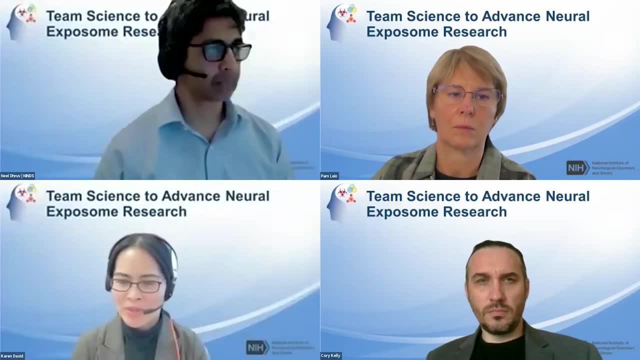 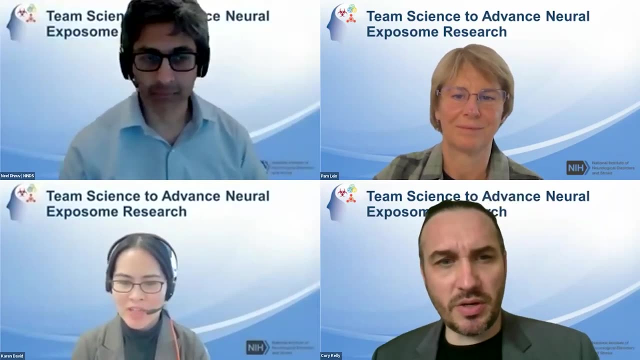 Basically, the review is a key, essential piece That determine the success of the program. So this very collaborative relationship that we have has been really beneficial for us, Corey. Thank you, Karen. Of course, I echo our thanks to our SROs and our study section. 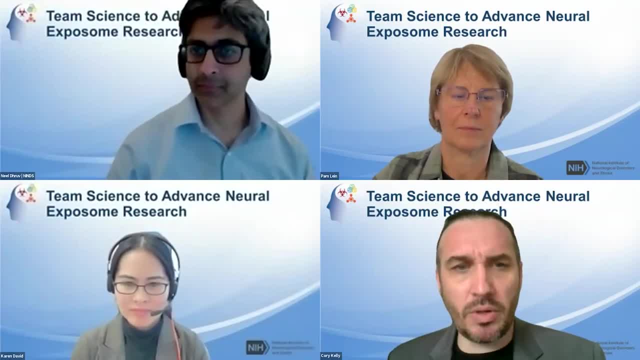 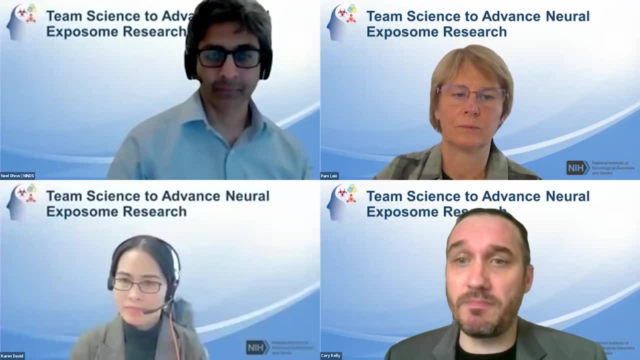 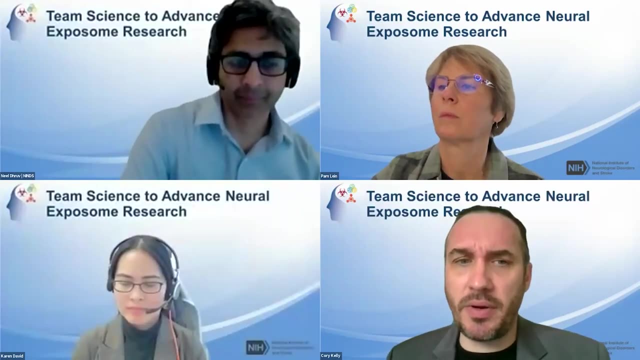 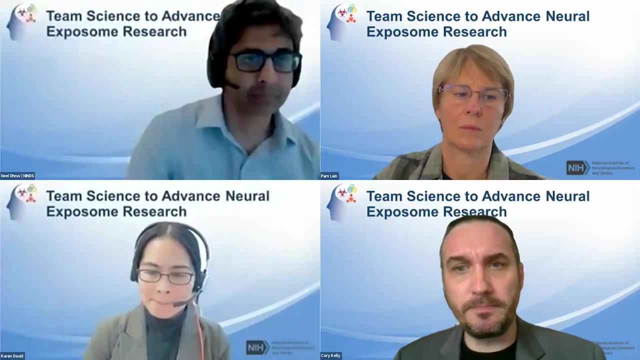 I think the only other thing I would add is we were very particular in the composition of the study section to make sure that we balanced what was quite a burden: the diverse scientific disciplines on every single application, As well as scientists who had experience in large transformative collaborations and could provide more of that team science perspective as well. 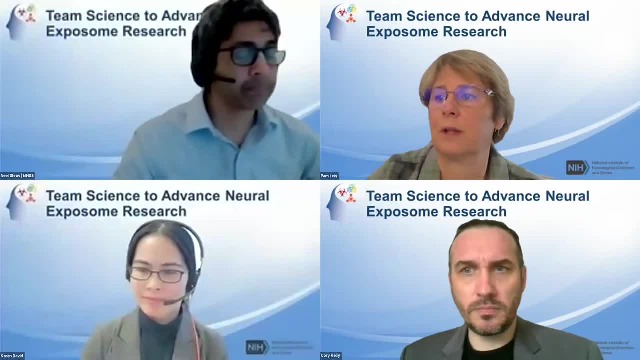 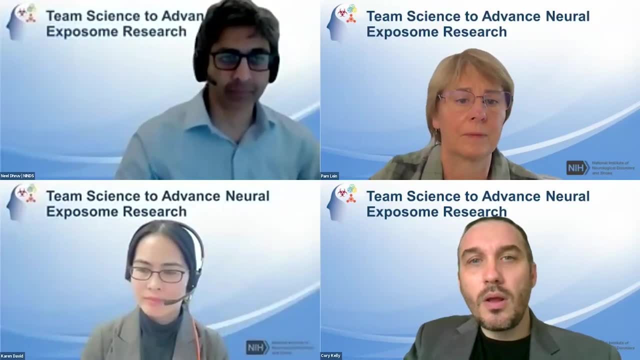 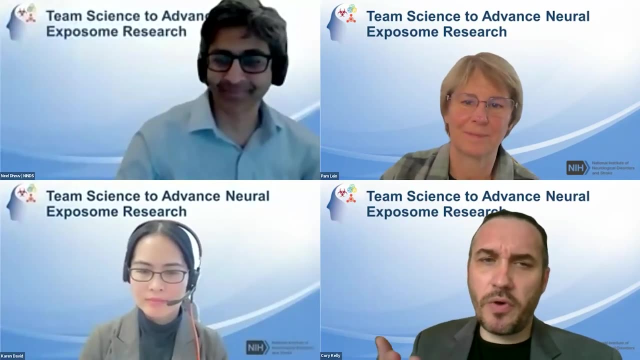 Thank you. This is very helpful And I do see that has a follow-up question to mine, which is: are these across institutions with subcontracts etc? I can answer it, Karen. Go ahead, Sure. Thank you. So for our program. there's a couple questions in there. 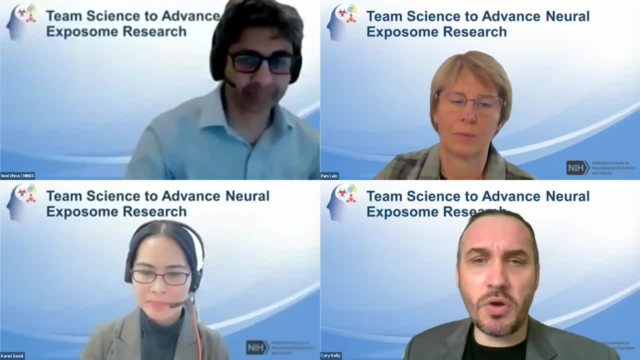 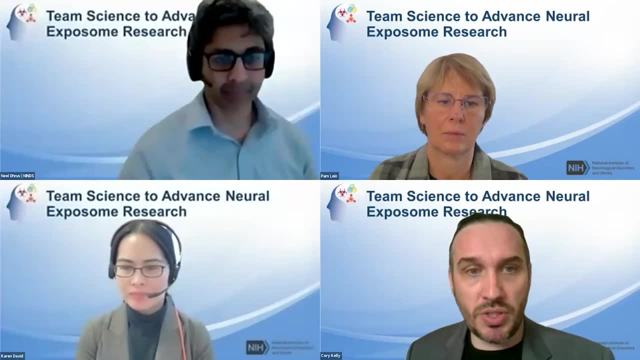 Different institutions yes or no, and subawards yes or no. So for our program we have no preference for if teams are in the same institution, same department, different institutions, different fields, We ultimately want the scientific goal to drive the team composition. 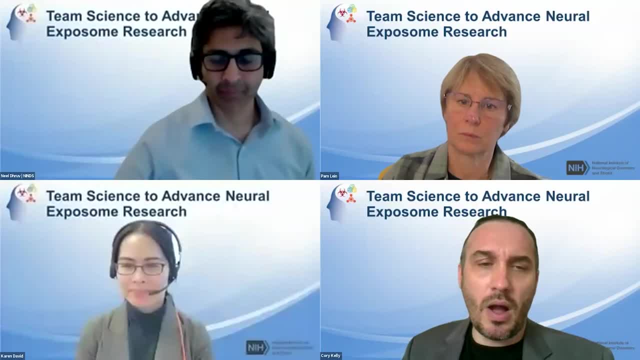 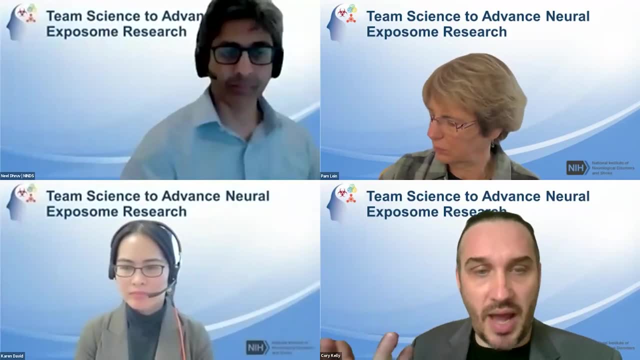 And so we want the best people to achieve that goal, no matter where they are. And so the second part: we require three, a minimum three to six PIs. So we do have a contact PI for the team, We have a contact PI for the administrative purposes. 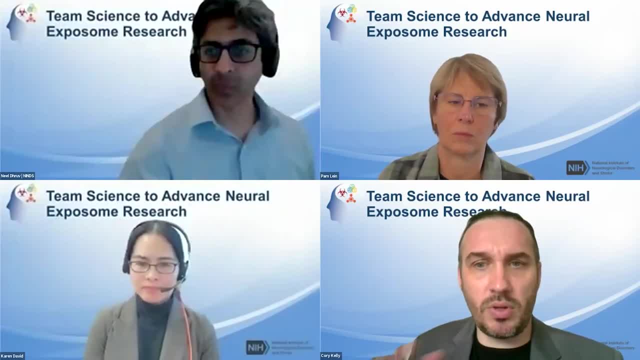 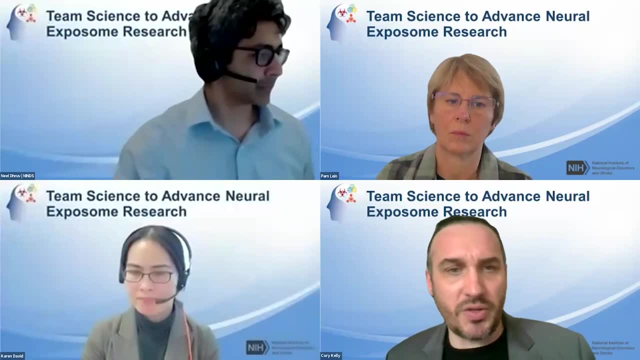 But the PIs, as Karen mentioned, are supposed to have an equitable and equal distribution of decision making. So one would be the contact PI and the others would be subawards to the other PIs or co-Is or whatnot. 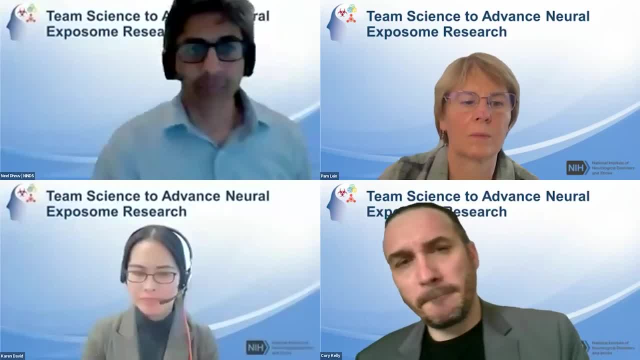 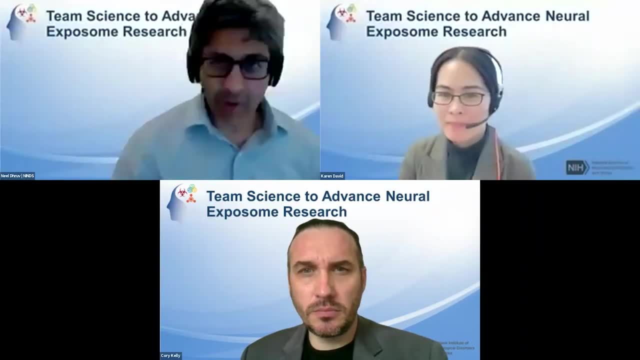 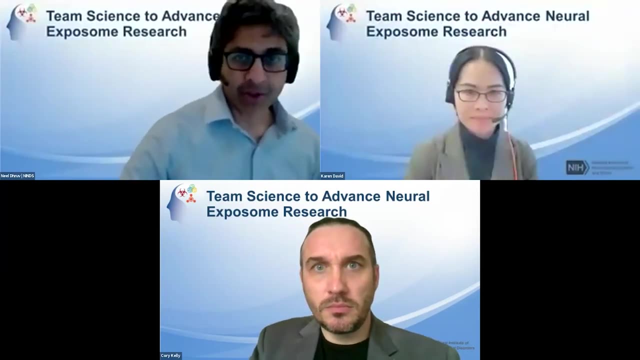 Yeah, Okay, That's wonderful. There may be more questions that come into the chat, but we'll answer them kind of asynchronously. At this point we're going to take a short break and give us all a chance to stretch our legs. 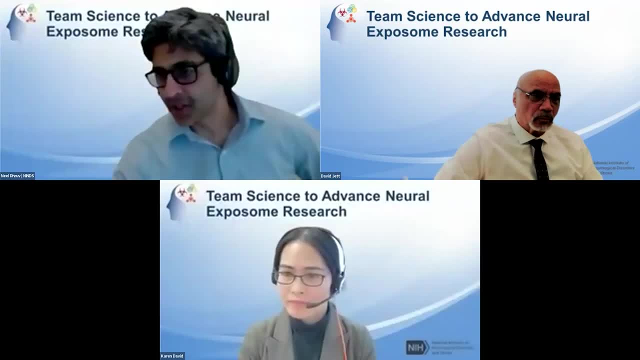 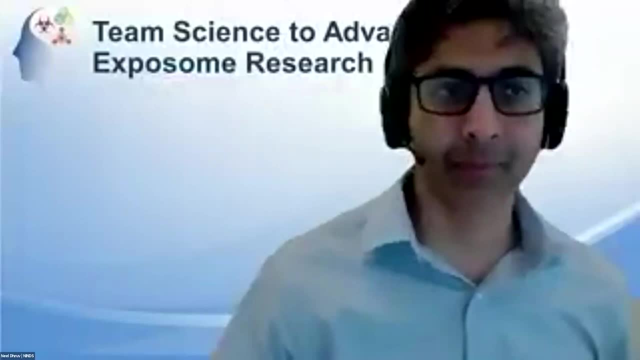 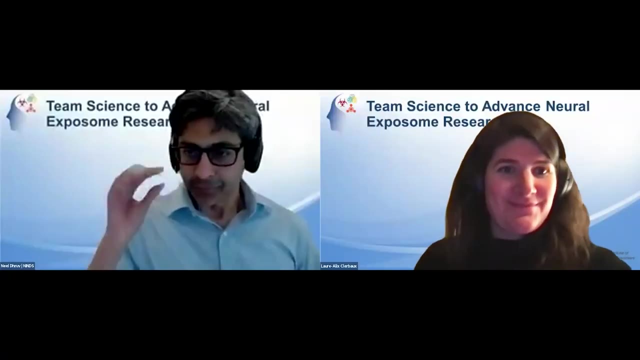 We'll meet back here in five minutes, which I have as 205 Eastern. Okay, We're ready to get started. Welcome back. Our next speaker is Dr Lor Alex Clairbeau. She is a professor at the University of Michigan. 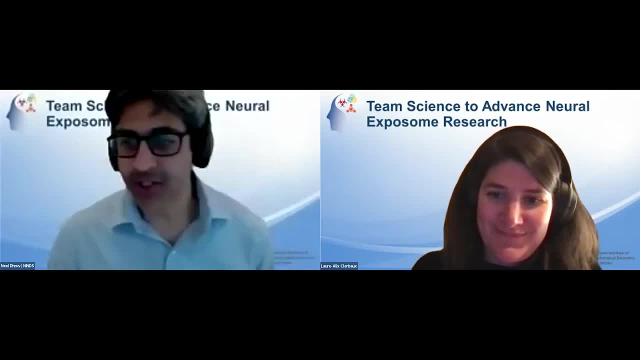 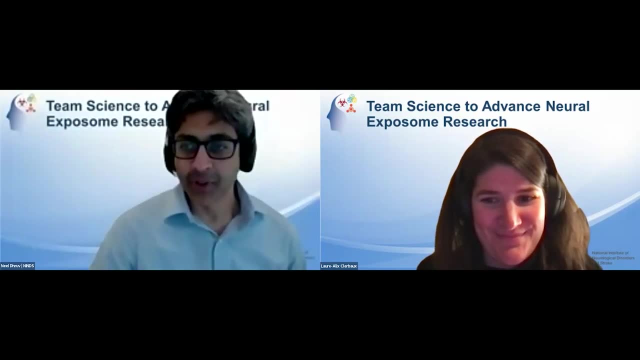 She is a senior researcher in the Institute of Experimental and Clinical Research at the Catholic University of Louvain in Belgium. Dr Clairbeau's work is driven by an interdisciplinary approach based on synergistic collaborations and translational research. During the pandemic, Dr Clairbeau worked at the Joint Research Center of the European Commission as the main coordinator of an interdisciplinary project involving more than 70 scientists worldwide. 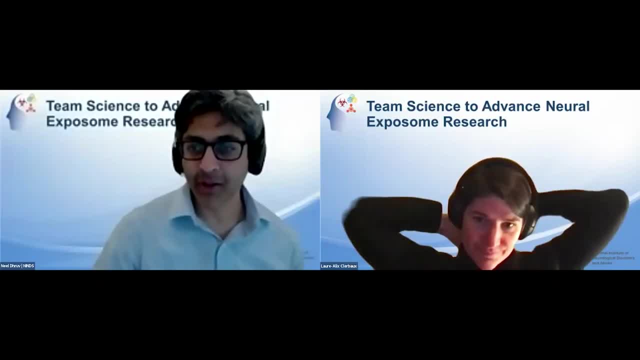 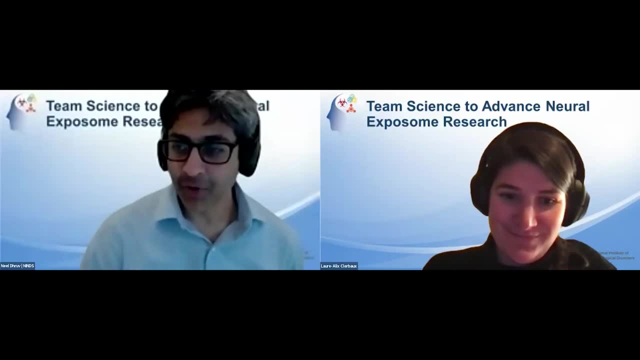 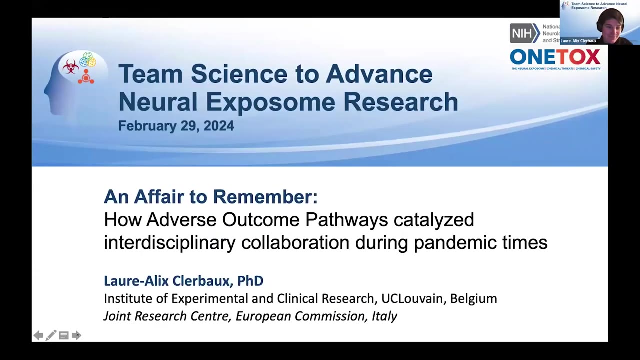 Aiming at organizing the plethora of experimental and clinical data on COVID 19.. Her talk today is titled An Affair To Remember How Adverse Outcome Pathways: Catalyzing Interdisciplinary Collaboration. Thank you for the kind introduction. Thank you for giving me the opportunity to present an affair. 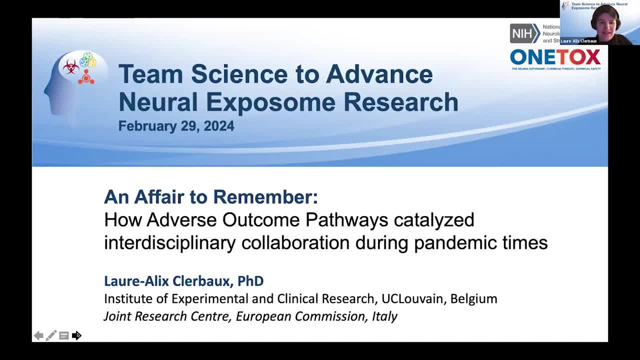 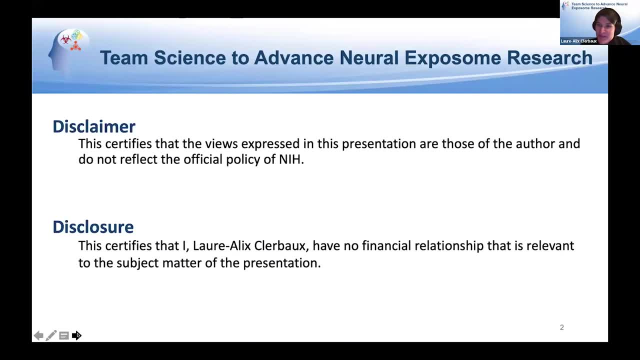 that you believe it. June 10th 2012. Outcome Pathways: catalyze interdisciplinary collaboration. Yes, I was. I considered that interdisciplinary collaboration during pandemic style, So my only disclaimer is that the work I will present is really the work of a team that. 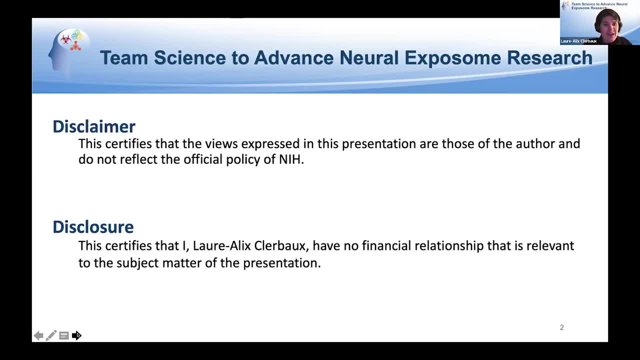 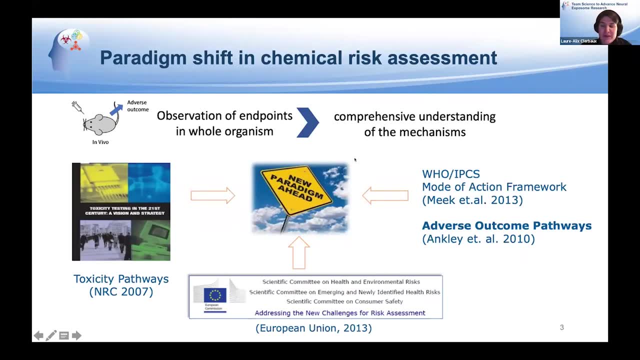 I have just the pleasure to be the one presenting today. So let's start, maybe, with what is an adverse outcome pathway and with this paradigm shift in the chemical risk assessment, which aims to move from observation of adverse endpoint in a whole organism towards really a comprehensive understanding of the mechanism. 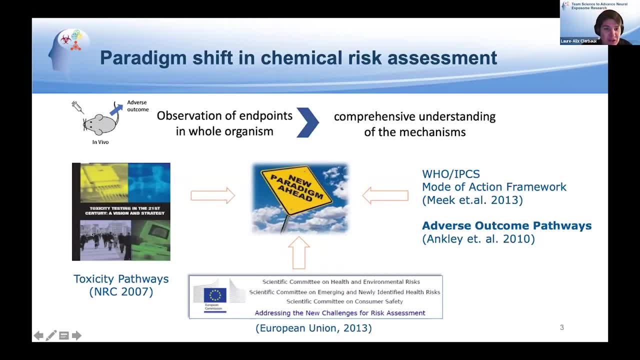 And this was already proposed in the toxicity testing in the 21st century vision and strategy back in 2007,- but also at the European level, how to address the new challenges for risk assessments, And that's why there have been different peer review, publication or reflection group that 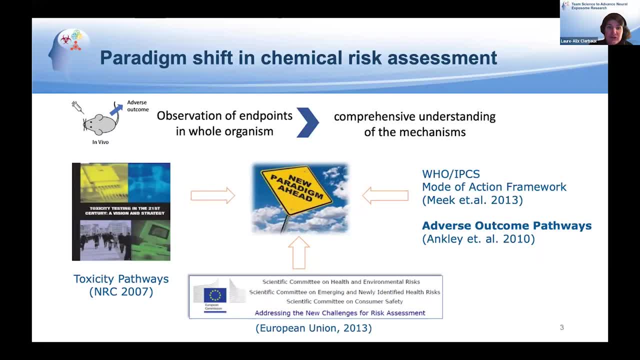 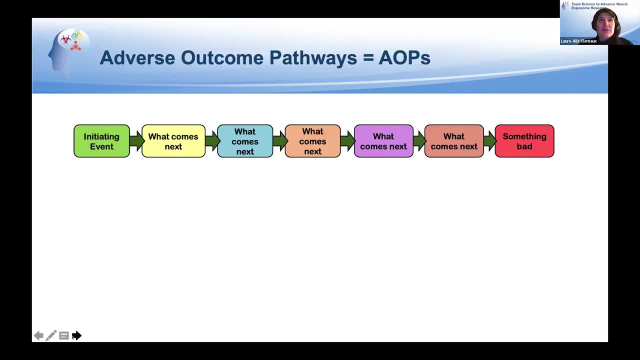 propose first the mode of action framework, but also the adverse outcome pathway. So adverse outcome pathway or AOP, that's the acronym. It's really a way of framework to represent Somehow the domino effect. So we have an initiating event that leads to something, next something, next something. 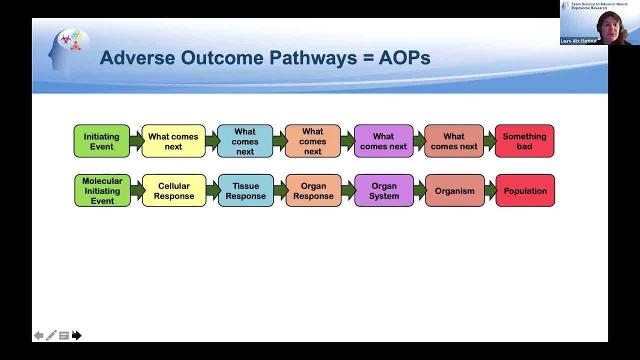 next up to something bad. And if we look into what happened into a body, when a body is exposed to a chemical, it will start with an initiating event: the connection between the stressor, the chemical, with the body at the molecular level. that leads to a cellular response, tissue response. that will 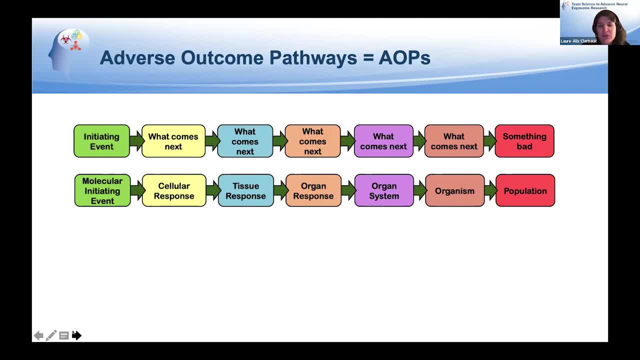 induce an organ response, up to an organ system response, tissue response, An organism and up to adverse outcome at the population level. A metaphor that we use to propose to really understand what is an AOP doesn't really aim to depict all the pathway and all the possible way of pathological pathway leading to an adverse 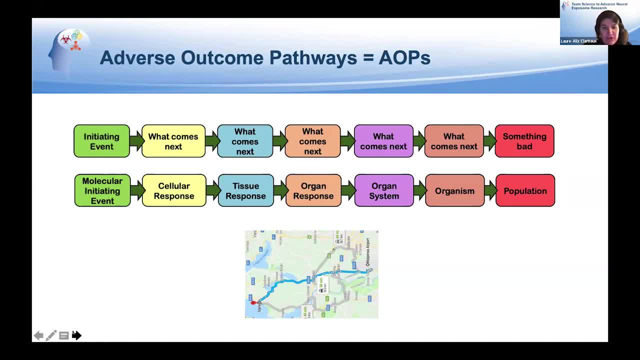 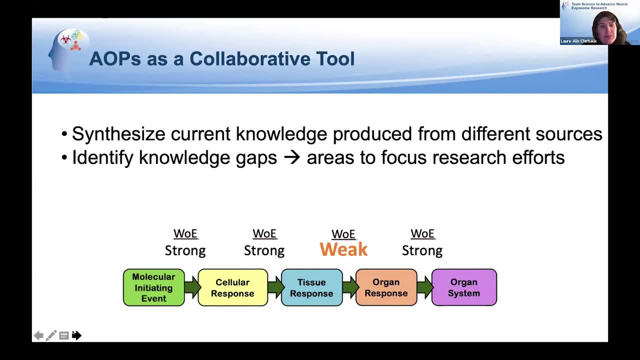 outcome, But it's one way to go from A to B, like for this Google map example. So AOPs are really collaborative tool because they help to synthesize the current knowledge that are produced from different, Different sources, because it's cross along all the biological levels. but it also helps to 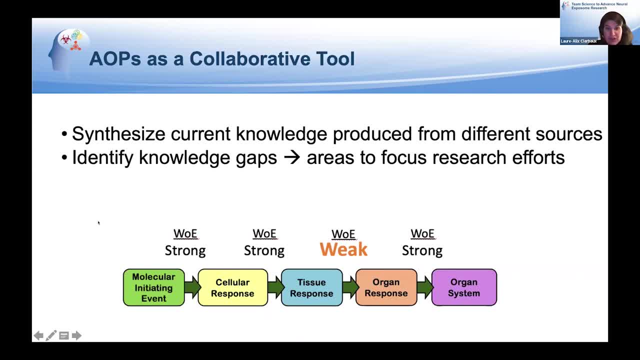 identify the knowledge gaps because you can look into the literature. It's based on what's in the literature, what is known, what has been already produced. If we have evidence that this causal relationship is strong or weak, and that when the evidence are weak, that give us areas to focus the research effort. 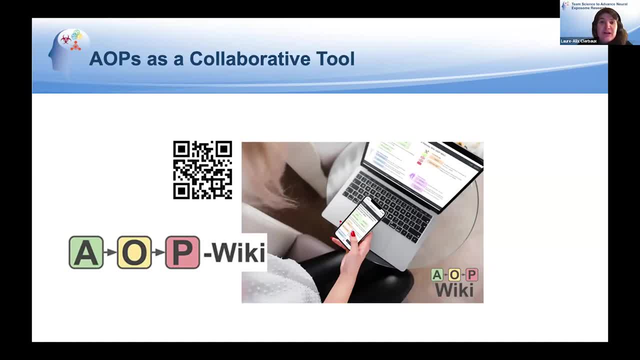 And actually the different AOP that are currently developed or are in development can be found on a open access platform that is called AOP Wiki, and you have the QR code here. So this platform, but itself as well, works as a collaborative platform where everyone can. 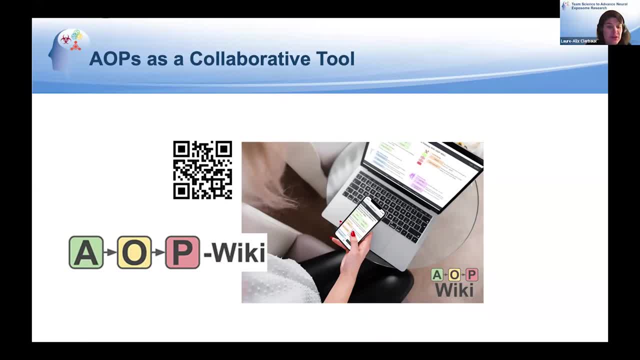 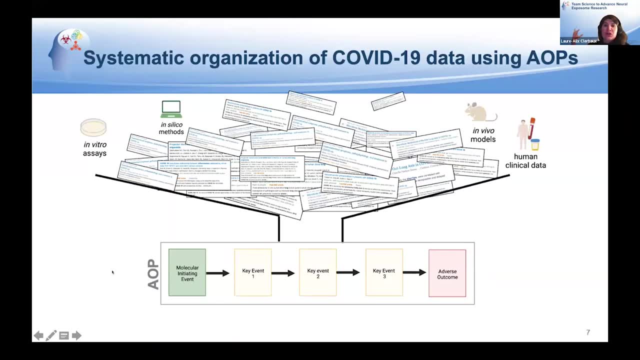 access, check the AOP, but also propose some improvement for the AOP when new information become available. This is why, back in the early times of the pandemic, some people working nanotoxicologist at Karolinska Institute, Péline Almarsch, said 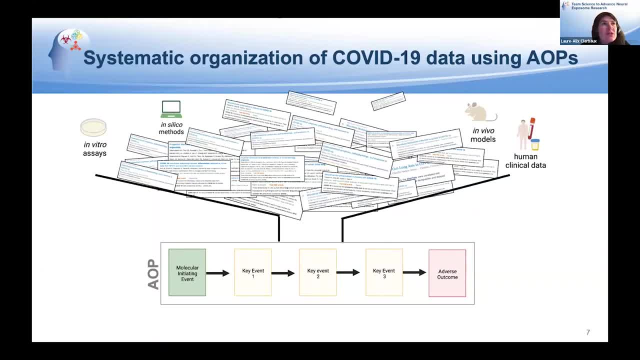 But what is happening with this virus of COVID-19 really looks like the mechanism, looks like what I do observe in the lungs with my nanoparticles. That's why we saw it. But AOP could really be a framework to organize all this information, all this prediction of. 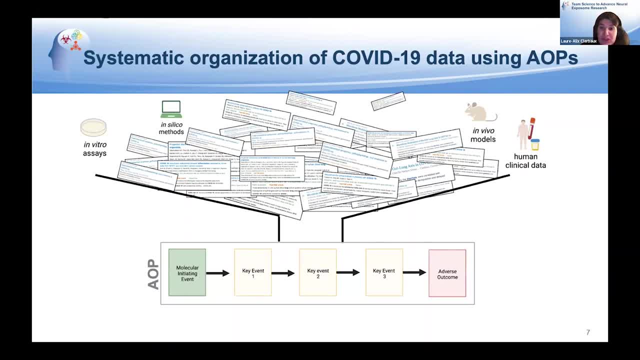 knowledge, this tsunami of data about the COVID-19 pathogenesis that were coming from different sources, because, by essence, as I said, AOP do integrate, does integrate data from different research area and method, And this is what we called the Chao project. 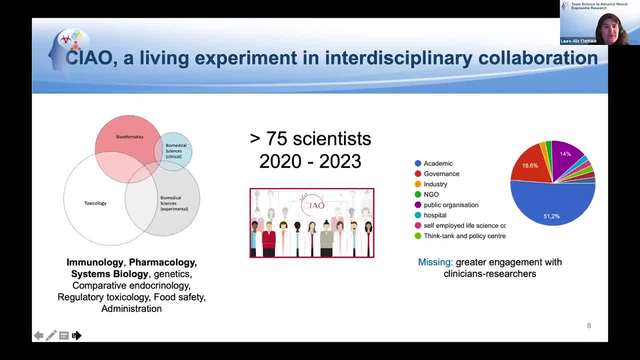 So that started in April 2020.. And so it was really a living experiment in interdisciplinary collaboration, because more than 75 scientists were collaborating together during around three years on a voluntary basis on top of a daily job. They come from different disciplines, but also different type of institution. 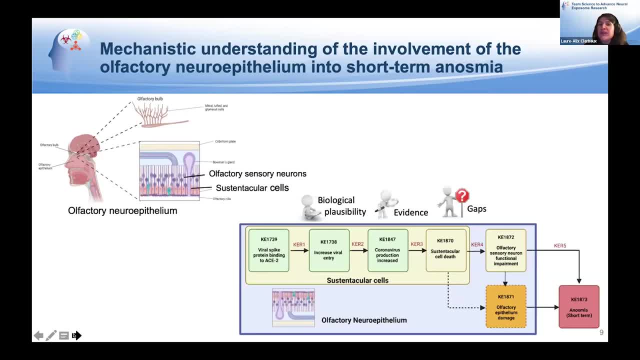 And this is only one example of one of the AOP we developed within the project, Because I have not the time to go through all of them, So I picked one that is more related to somehow the neural aspect. So you will dig into the literature, see proposed some biological possibility of a pathway. look at the 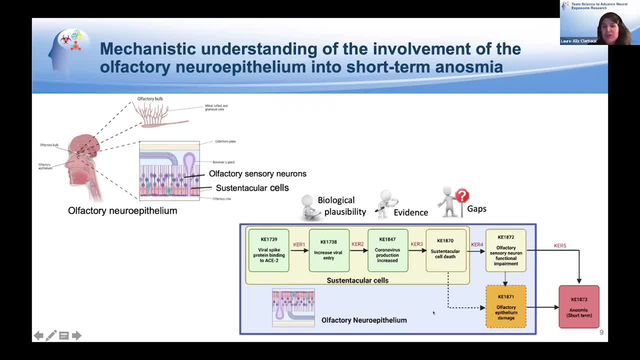 evidence and then identify the knowledge gaps, And this one was focused on the adverse outcome, that is, short term anosmia. So maybe some of you experience this loss of smell when they had COVID that then disappear after a while. And let's have a look. 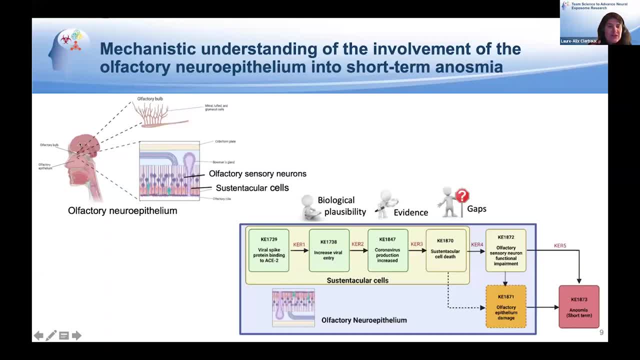 So a look here at this olfactory neuroepithelium that is really located at the rooftop of the nasal cavity. It's quite a complex epithelium, But here there are two cells of stress for us here, the systentacular cells, which is really the cell that. 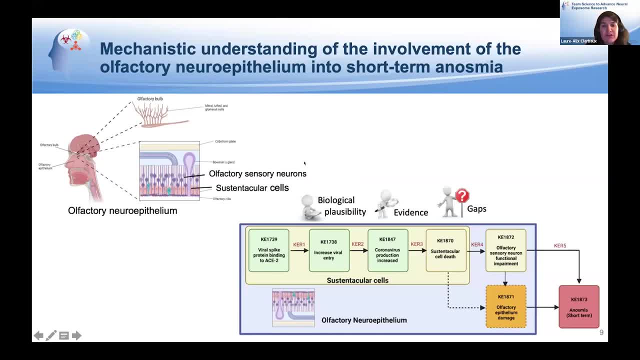 will structure the epithelium and the olfactory sensory neurons that will bring the message to the brain, And actually the systentacular cells. they do express the receptor for the virus, the ACE2 receptor. So there were some evidence in the literature that showed that then the virus can really enter into those. 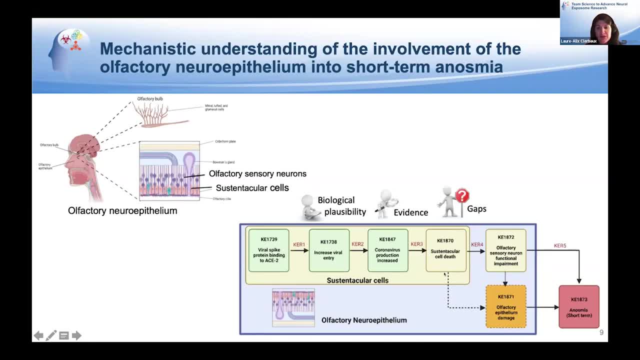 cell replicates and that leads to the death of those cells that disorganize the whole epithelium. that leads to a functional impairment of the olfactory sensory neuron. But these cells could regenerate And this is why this anosmia is only short term. 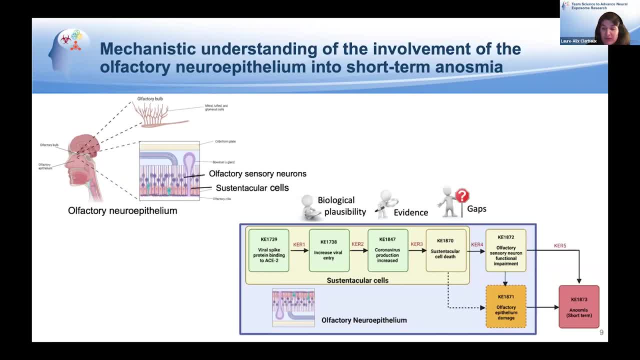 And the mechanism behind the long term anosmia is really different And this type of AOP were built and evidence were collected Thanks to the working groups here that to give you some example of the different disciplines we had around the table, we have Ali and Katia that were biomedical researcher from Finland that really take the cells from this. 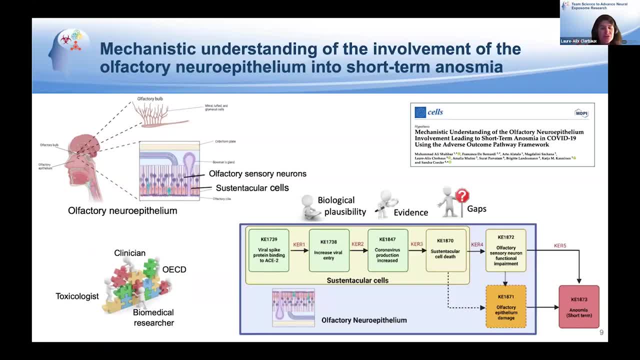 neuroepithelium and look how permissive they are to SARS-CoV-2,, how they do react to air pollution. But then Francesca de Bernardi: she is a medical doctor in a hospital in Italy where she really treat patients with anosmia. 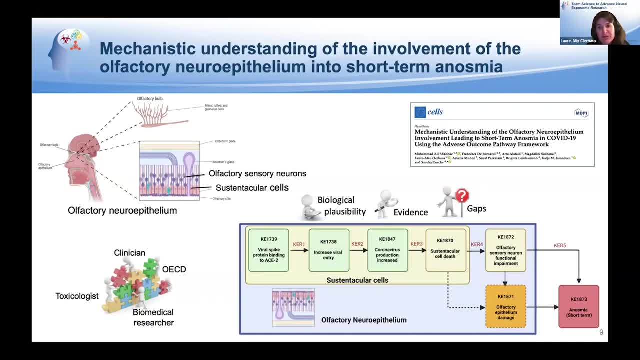 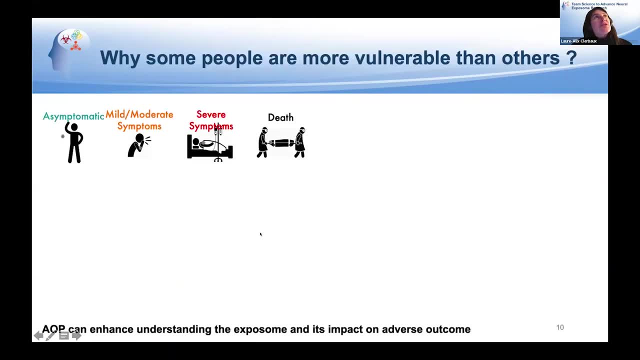 And Magdalena, for example, is really an expert in this AOP concept. This is just to cite some of them, But we had also a great interest in understanding why some people are more vulnerable than others, because it was obvious for COVID-19 that 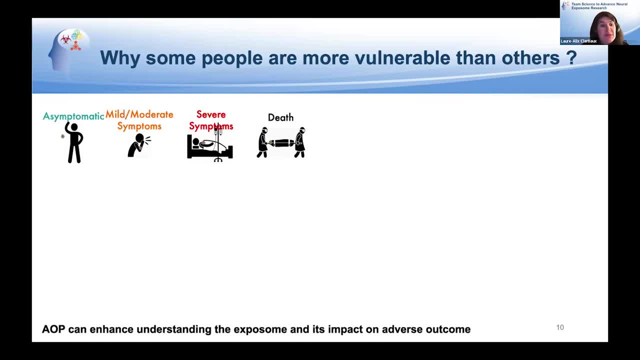 the outcome very ranges, from asymptomatic to death. So we look into the modulating factor. So there are some that could be intrinsic, like age, sex or genetics, as we say, but even pre-existing comorbidities, And one of the things that we looked into is the modulating factor. So there are some that could be intrinsic, like age, sex or genetics, as we say, but even pre-existing comorbidities, And one of the things that we looked into is the modulating factor, And the last one that I can cite here, it's really the gut dysbiosis. 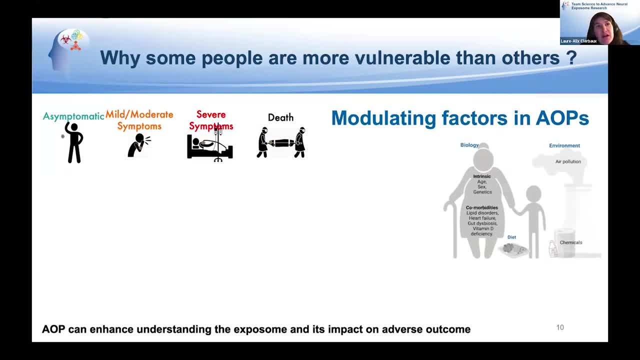 So before that you were infected with the virus, you had already an alteration of your gut microbiota that could really modulate the way you will react to the infection. But there are also some external factors that can modulate the way the body will react to the virus. 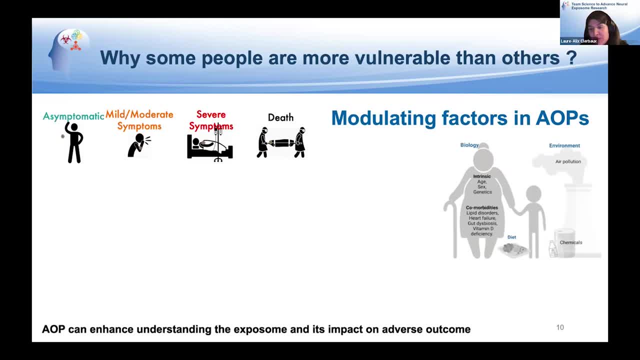 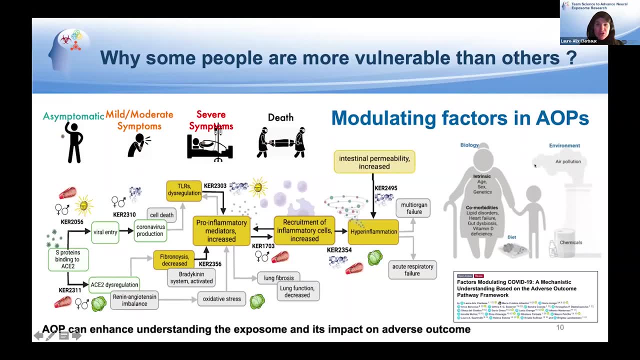 It's, for example, exposure to air pollution or exposure to some chemicals, And here we looked at the exposure to pfas, And so we had data showing that there is indeed older men are more vulnerable than other to fatal severe disease. But then we were interested in using the different AOPs, the different pathological pathway described by the other working group in the project. 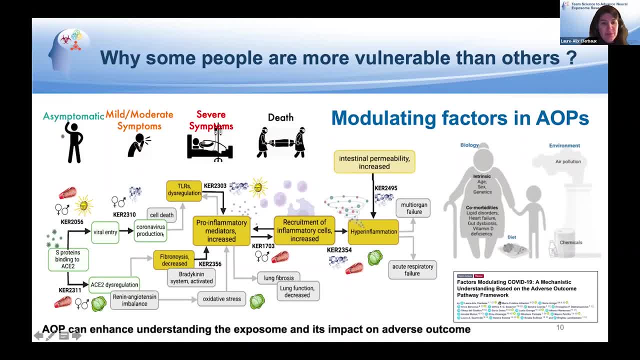 to really look into the literature where, in this different step, those different factors do modulate the different step of the pathway So that at the end it does have a different impact on the adverse outcome which was here, this cytokine storm or the hyperinflammation. 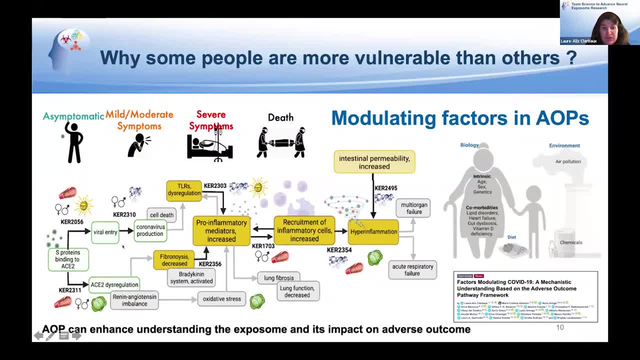 So an excessive inflammation response, human response of the body. So the AOP can enhance the understanding of the estrosome and its impact on adverse outcome. But this was really the first time in the CHOW project we really paved the way on how to use those, how to integrate those modulating factors. 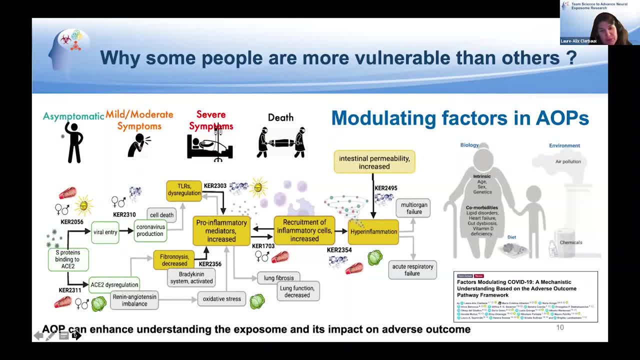 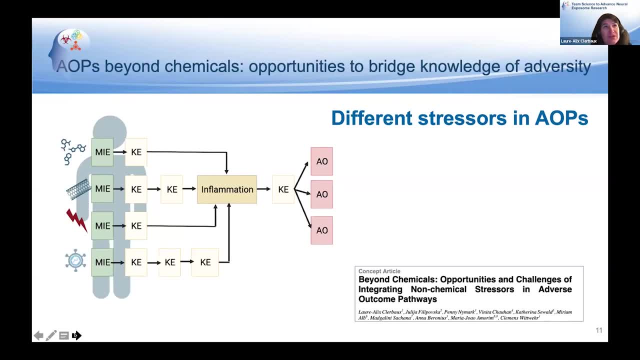 But there are still somehow some challenges to that And I also mentioned initially that AOPs were really developed to support this budding shift towards an understanding on the mechanism leading to adverse outcome that are triggers by chemical. But here, when we explored it, when we use the AOP, behind the chemicals that give us opportunity to bridge the knowledge of adversity, 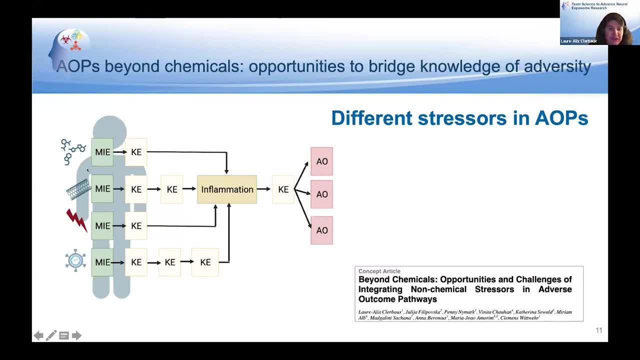 Because, whether we're exposed To chemicals and the low material radiation or a virus that will trigger a response into the body that sometimes could be leading to the same perturbation with the perturbation of the same biological event, like here is schematize or the exemplify with inflammation. 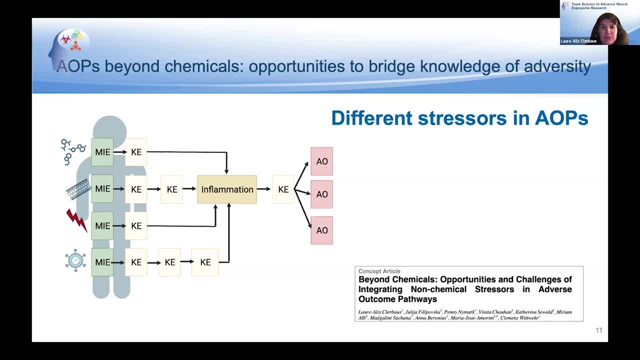 So by considering different type of stressor in the AOP, that could also help us to understand what happened inside the body. That is more reflective, The real multi type of stressor, the real scenario, the exposure that we are really facing as human. 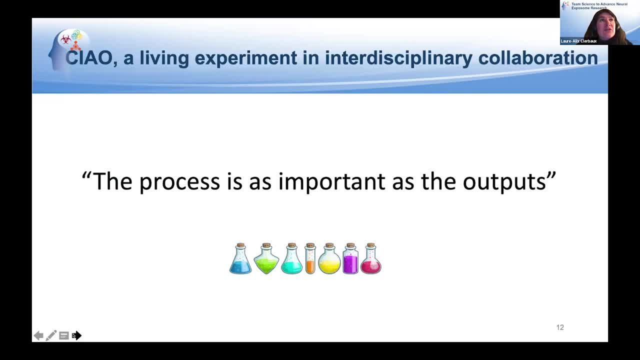 But also regarding the team science. we said from the beginning of the project, we said that the process of how we work together was as interesting as the output that I just presented you. So we we were lucky to have beyond us in our group and Anna-Maria Carroussi, who is a philosopher and social scientist. 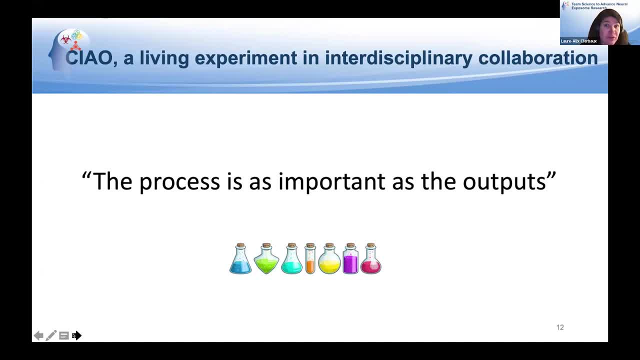 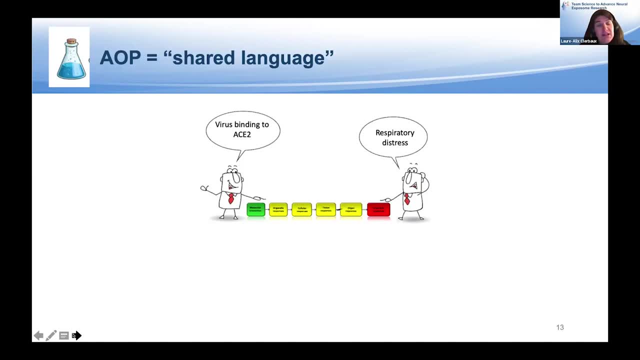 Really interested To understand how scientists work together or even how efficiently scientists work together. So we really dig into the different ingredients And honestly, the AOP first was really working as a share language or conceptual mediator to put people from discipline different disciplines around the table, but also different disciplines that use sometimes to look at one side of the biology. 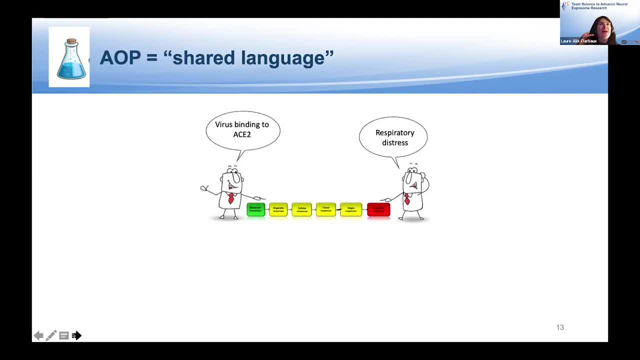 the molecular, the cellular level or more the clinical symptoms, And so we had to sit. Sometimes it takes time and discussion to really agree on what one word means or what we means when we want to look at this aspect. So it was really a bridge between disciplines. 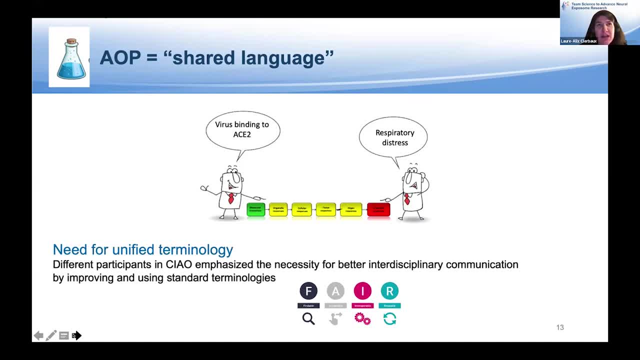 However, still there is a need really for unified terminology. So different participant in CHAR really emphasize the necessity for better interdisciplinary communication to by improving and by using standard terminology that makes all the knowledge in the data more fair, So findable, accessible, interoperable and, at the end, reusable between the discipline as well. 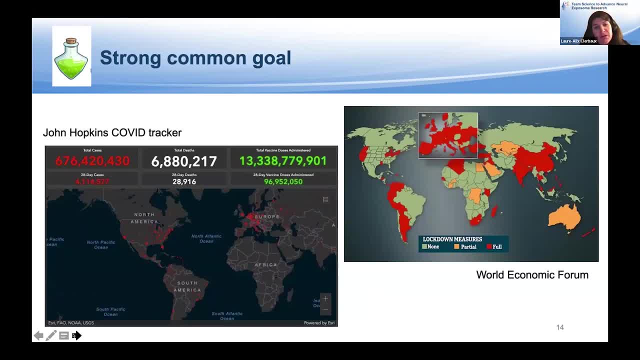 In our case, of course, another ingredient was a strong common goal, So it was to fight disease. that was a pandemic situation that leads to too many deaths, but it was also during lockdown time, So people were somehow stuck at home, And so there they were really strong. 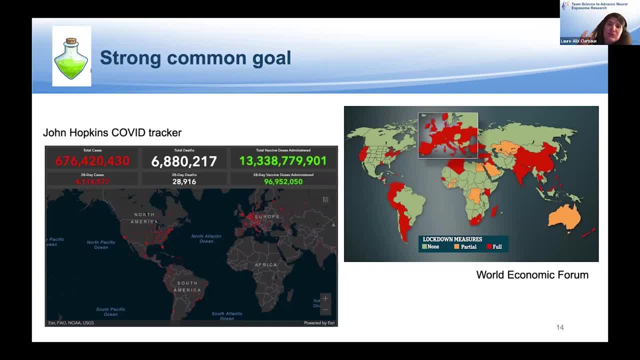 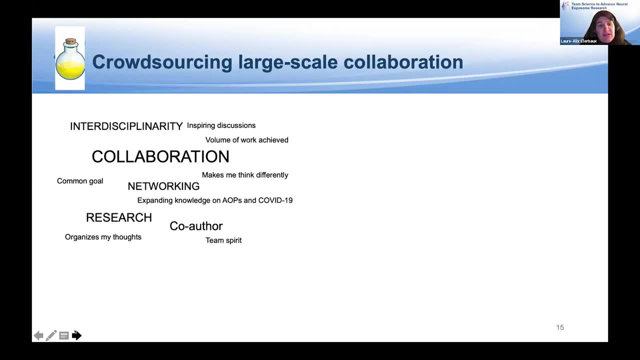 Motivation to do something, to fight, to contribute, to participate, to fight this disease. The model is so. our model was interesting. It was, as I said, offer for most of the people on top of the daily job. So it was a crowdsourcing, large-scale collaboration models. 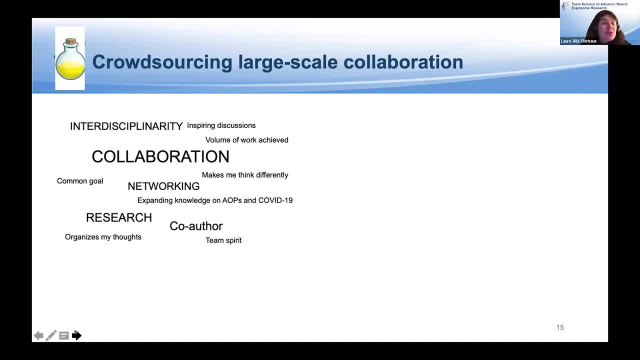 And when we ask the participant what is the most rewarding for you to participate in CHAR, You can see this workload. It was really collaboration, networking, interdisciplinary, but also, as we will Discuss, about credit, It's also the quarter ship and the fact that also we, they all feel and then often mentioned that we had a logo. 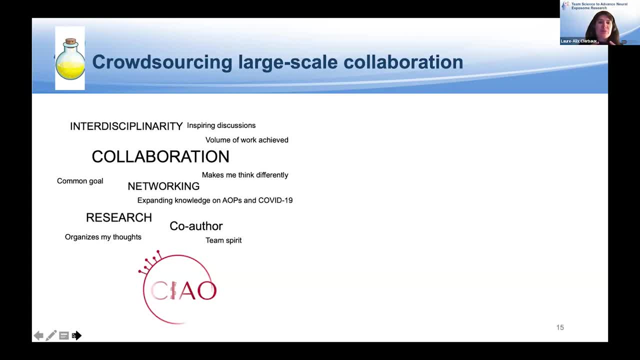 We had a team. We feel like being part of the community. So the people did participate to chow are really happy and proud of that. But this has to go with terms of collaboration. They should be set at the beginning and they should not be considered as implicit, even if it's a crowdsourcing or based on a voluntary basis. 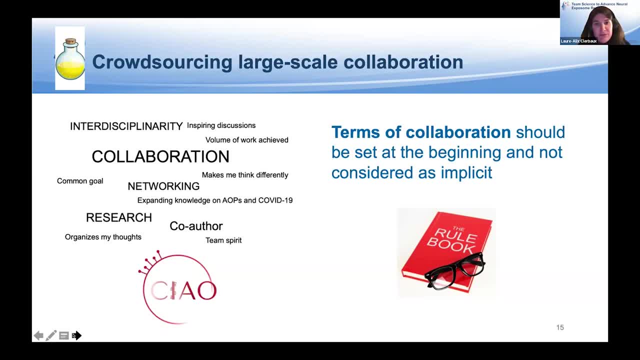 That's maybe the storming step that Corey Kelly mentioned before, that we had to come with these terms of collaboration and also process, also to deal with conflict when they appear, because we were more than 75 scientists coming from different disciplines with different opinions. That's what makes the project successful. 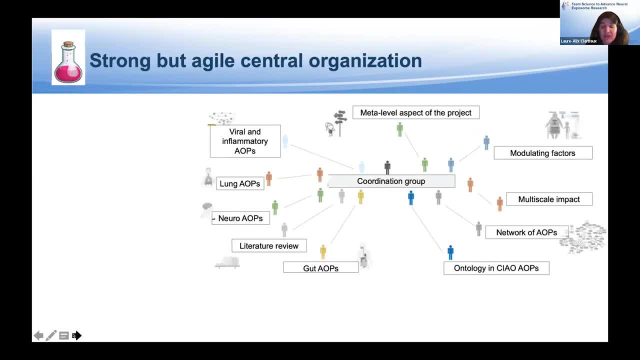 But then we need also to have terms of collaboration And then, importantly, as the current David mentioned, we believe that One important ingredient why 75 scientists stay and collaborate during these three years, It's because we had a strong but agile central organization. 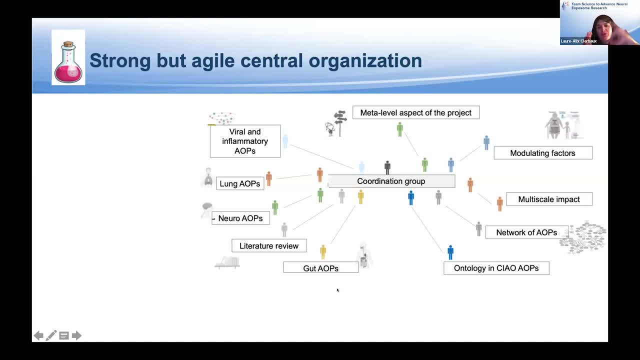 So the different scientists were working in different, smaller working group, either depending on the organ of interest, like the neural group I presented the shorter monosmia- or so depending on some aspect of the project, like the modulating factor I just mentioned, and for each of these working group, 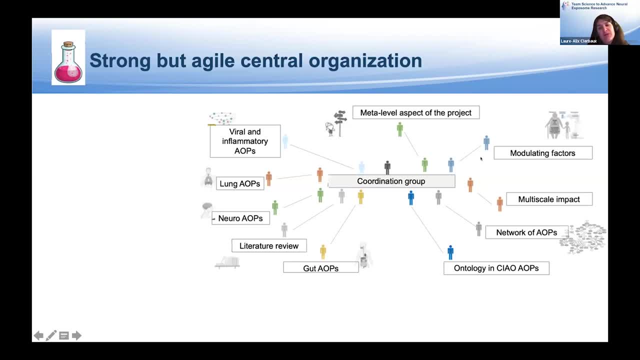 We had one coordinator that was also participating to the coordination group that met twice a month and I was really making all this concept Agile but centralized and harmonized, because we had a coordinator that was a scientific coordinator for each of the working group working individually, but then also a coordinator that was more administrative coordinator that make sure that we did organize, for example, twice a year. 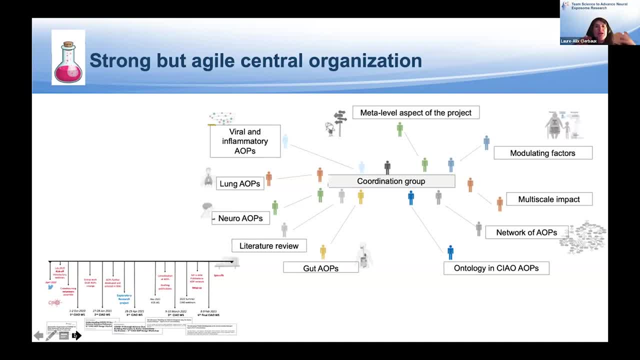 A virtual workshop of two days, but we all get out together to present what we're doing, to harmonize the way we're working, to present the different challenge. We also had every week a child internal newsletter to be able to communicate the different aspect between the different working groups. 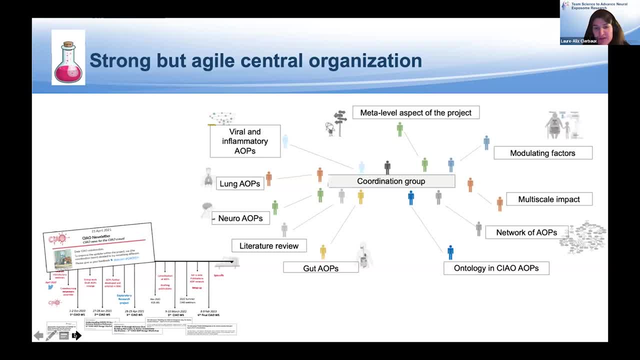 Again, if we were some challenge or the progress of the paper And most of the people, as I said, where they're not paid, I was the only one I paid full time to really coordinate everything And what I used to say, being a coordinator or coordinating such a project, is really acting like an enzyme. 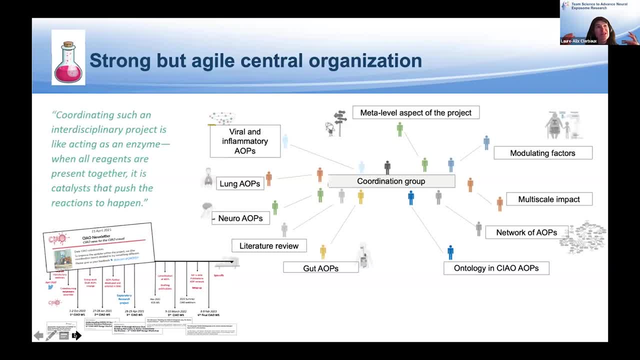 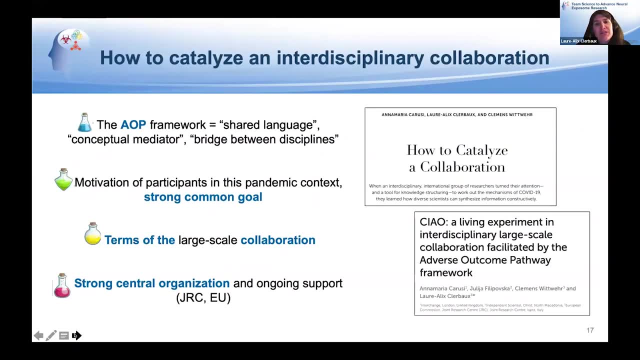 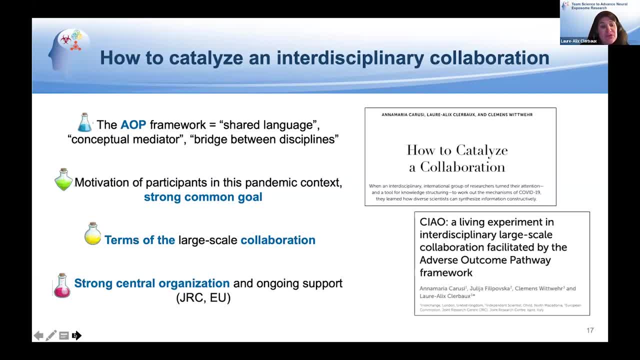 It's really that the AOP framework is really useful, instrumental, as a shared language, as a conceptual mediator or bridge between disciplines. It's really that the AOP framework is really useful, instrumental, as a shared language, as a conceptual mediator or bridge between disciplines. but there was so motivation of the participant in this pandemic content that was a strong common goal. 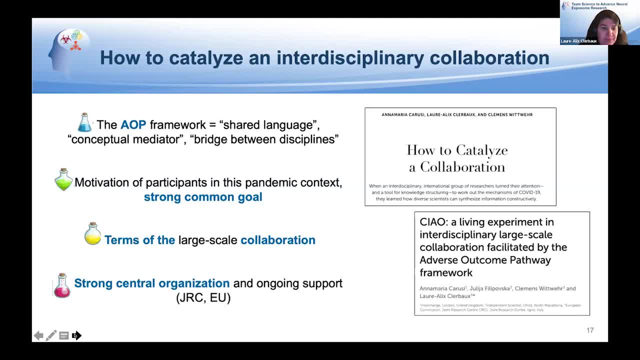 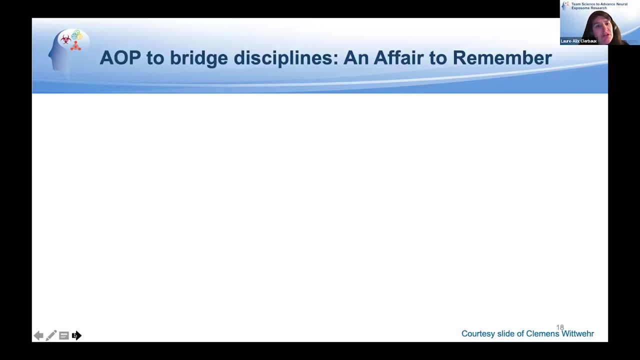 Also the terms of the large scale collaboration needs to be said and to be clear, and then the strong and central organization and ongoing support that, in that case, was really possible thanks to the Zhong research center of the European Commission. So maybe to conclude, I would like to finish with these two points. 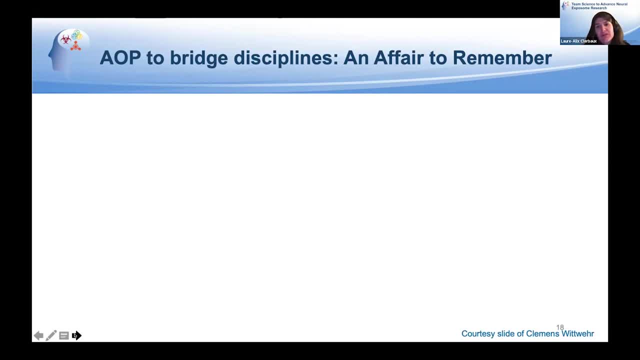 So maybe to conclude- I would like to finish with these two points- that AOP to bridge disciplines. it's an offer that is worth to remember, and the model can be applied to anything where one thing leads to another, or even when one thing is followed by the other. 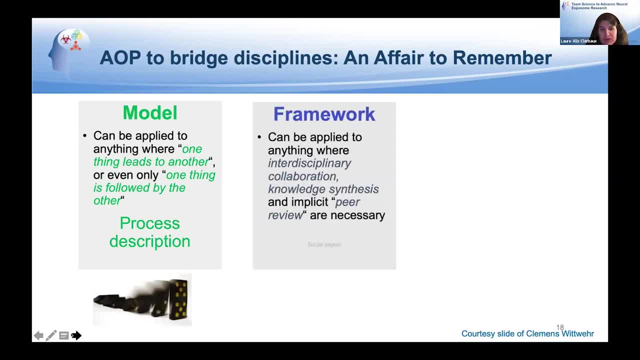 So this is the process description, but the framework can be applied to anything where interdisciplinary collaboration, knowledge synthesis or implicit peer review are necessary- And this is more the social aspect of the AOP- And then the content can be applied far beyond bioscience. 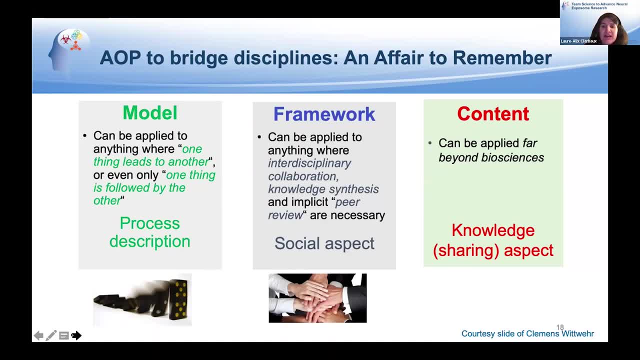 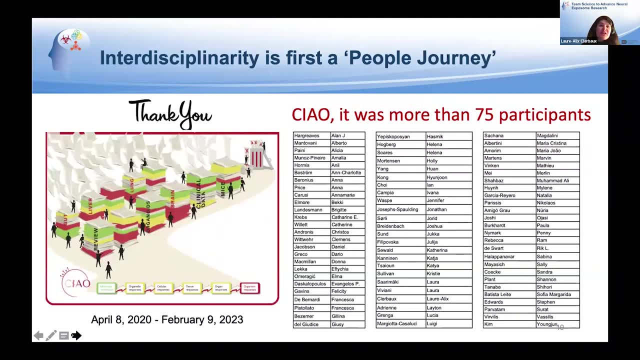 far beyond chemicals first, but also far beyond bioscience, And this is the knowledge sharing aspect. And so I will finish by saying that interdisciplinarity is first, for me, a people journey, So it's possible only thanks to all the participants. 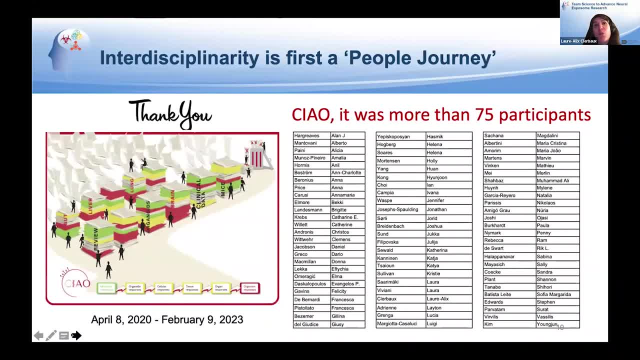 the 75 participants that I named here that really I wanted to share, to learn from each other and to be part of this journey. So I have to finish my presentation by taking the opportunity to find all of them again And I'm happy to take any question. 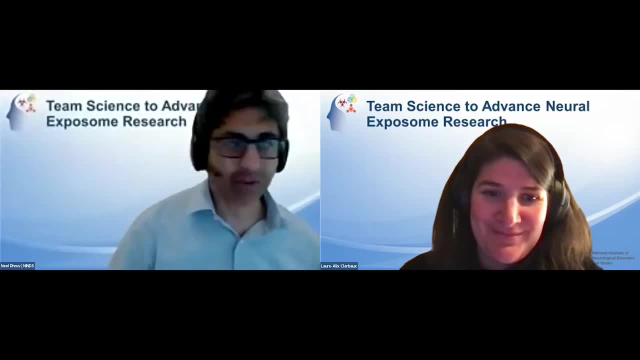 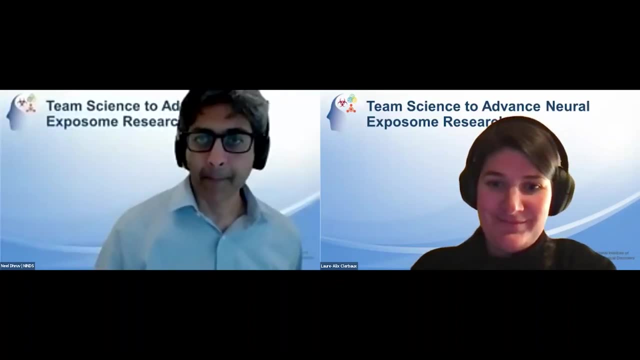 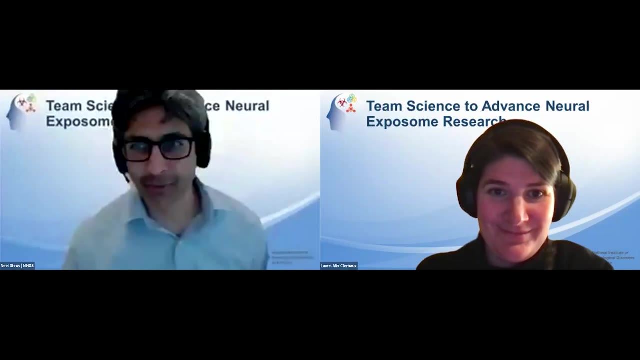 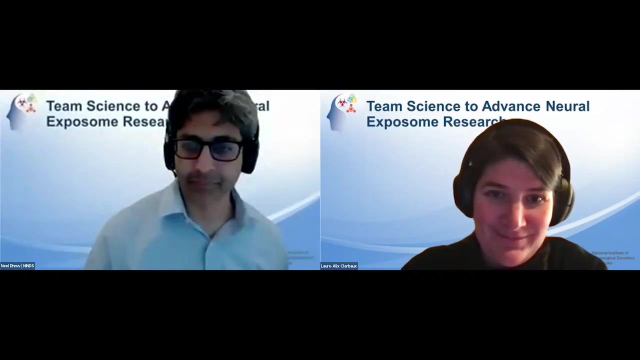 Okay, Thank you very much. I don't know if there are any questions from the panelists, So I had a question. Please go ahead. Yeah, My question would be about: I mean, this is really just really remarkable And how did you mention that? a lot of the people 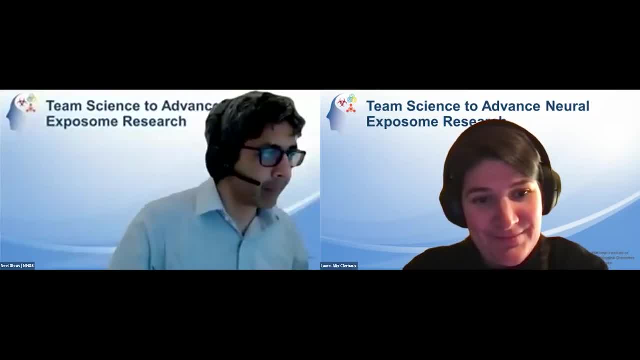 that were participating were not getting paid, And I'm just thinking. I didn't hear any of this. Well, it was on the voluntary basis. Yeah, I think it was on the voluntary basis, Yeah, Yeah. So I'm just trying to figure out how. 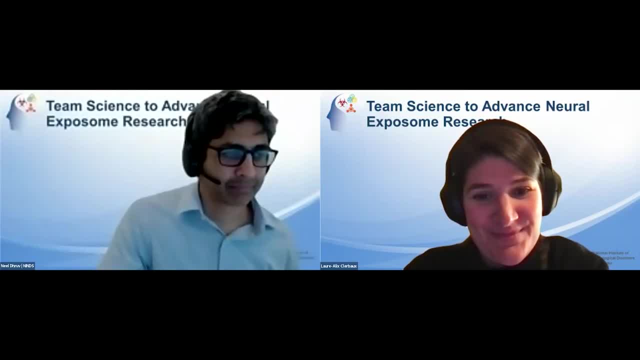 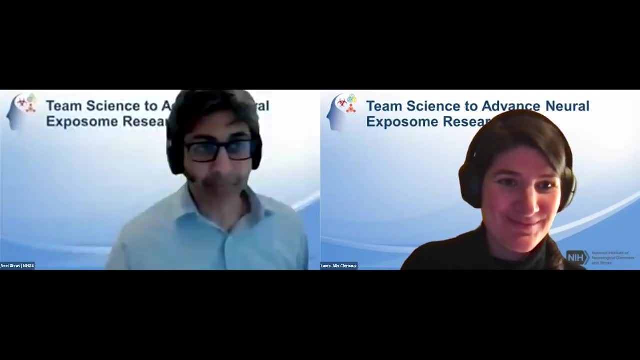 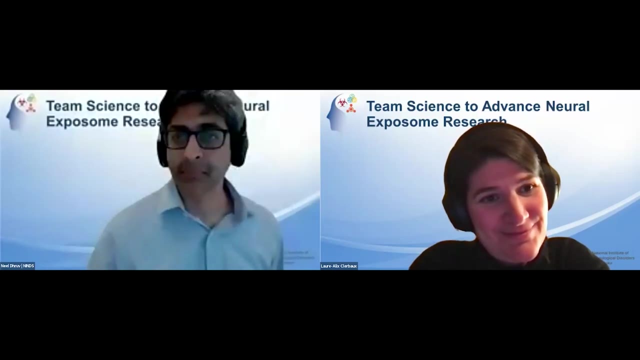 that would work here, but it's something to think about and something to try to make happen. So, yeah, really, really awesome. This is good stuff here. Thank you, Dr Rai. Yeah, Thank you for that excellent talk. there was just a silver lining to the pandemic. it allowed us to peek behind the curtain and really 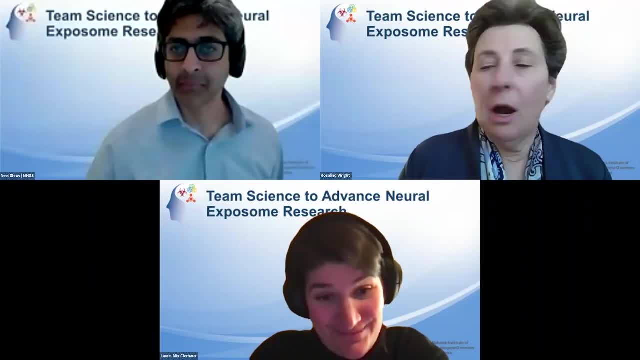 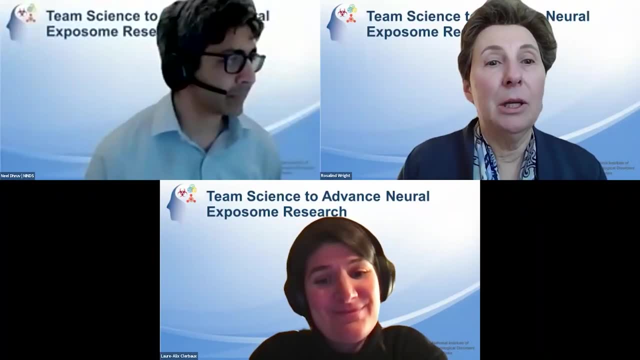 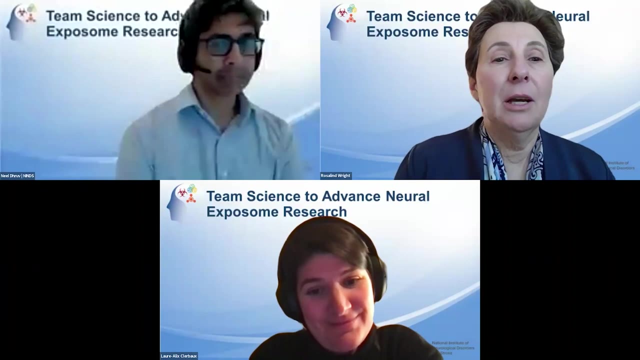 see what team science can do when we are truly focused. you on a, on a one purpose, and it had to happen and everybody sort of was on it, and you exemplify that in in what you accomplished and how you pulled this team together and organized. that was kind of going on lots of places. um what? 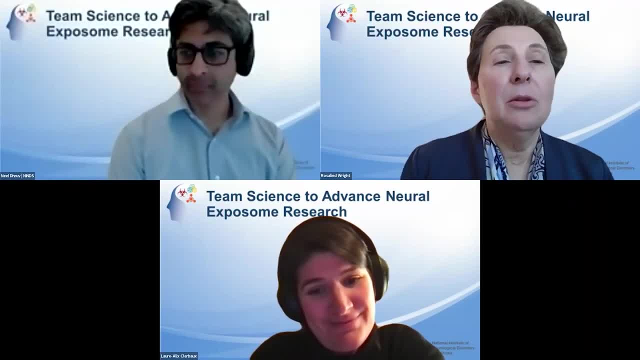 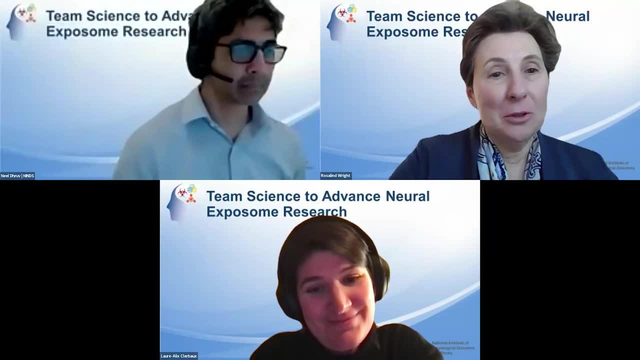 you know, I think we should all be taking those lessons learned and not losing that potential. we talk about this all the time at our own institution, in our bigger groups, and that I thank you for that, and it's something we should come back to, I think, when we do do the panel. 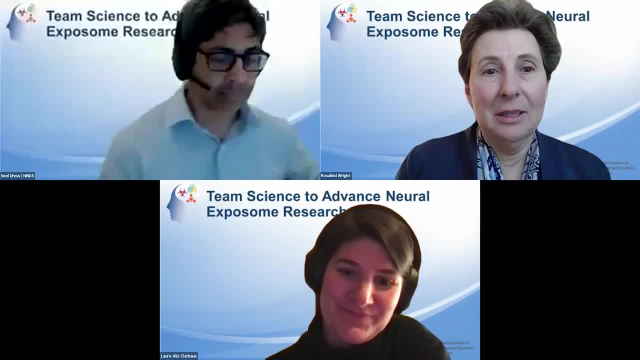 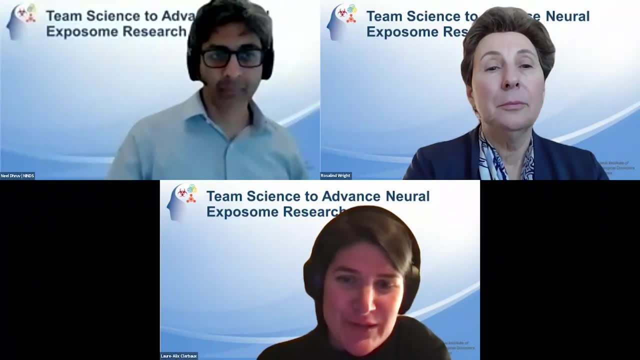 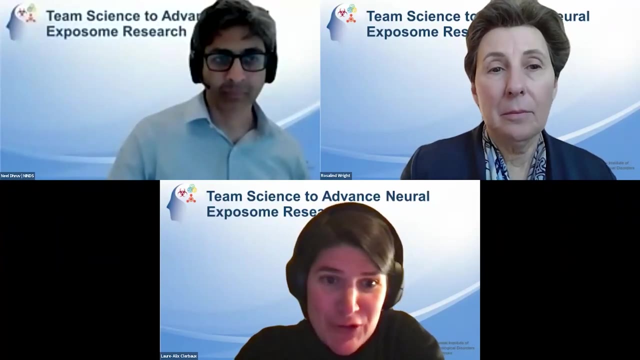 discussion, because there were definitely lessons learned there. thank you for your comment and actually, as I said, we were really trusting in the outputs- that I could not present all of them, of course, but also by the process and we really want to continue to share um the lesson learns and that's why we really try to. 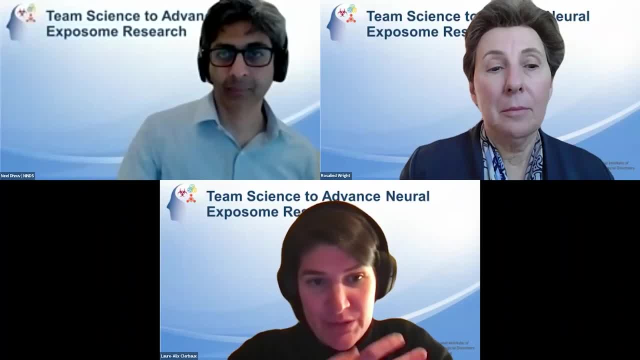 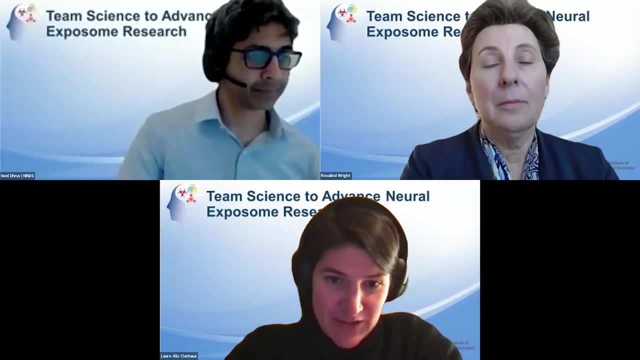 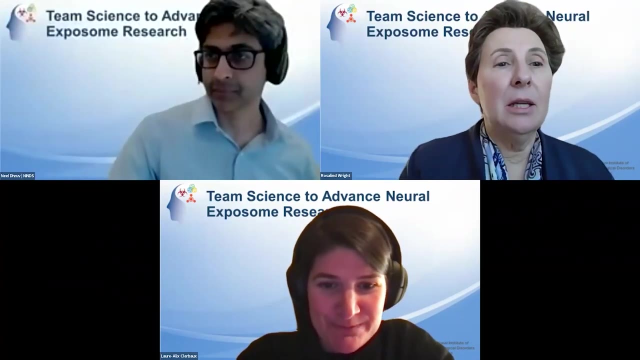 understand the ingredients. we have publication that you, we invite people to to read, but, as I said, also one of the ingredients was this specific pandemic time, so that was also something to to take into consideration. it was a specific moment but to be excited about the potential of team. 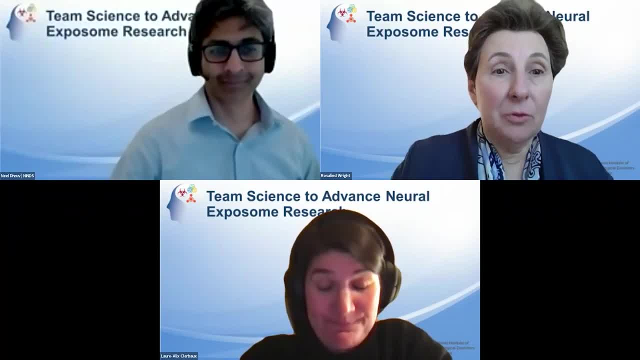 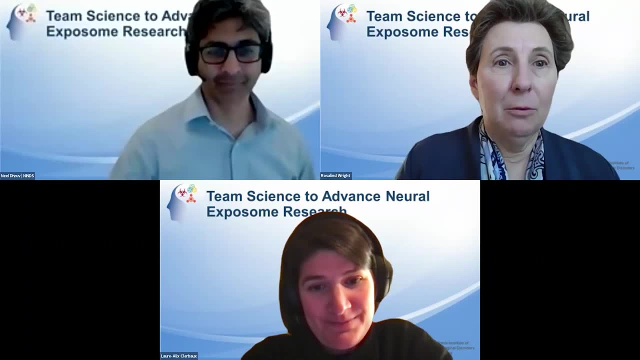 and lots of us did things that were unfunded mandates. right, because we we wanted to roll up our sleeves, be involved. what you're talking about here in NINDS, to put funding behind that now, right, because you can't do that outside of the pandemic. we do have to, you know. you know, pay the bills, or? 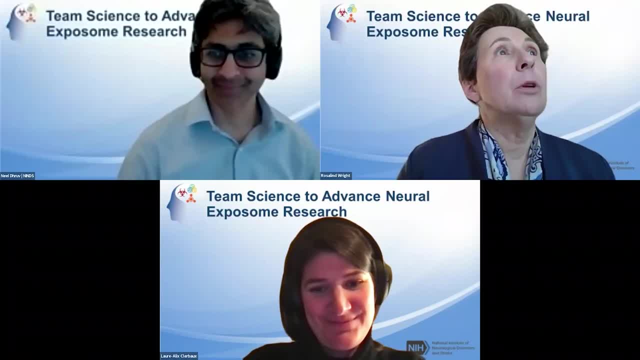 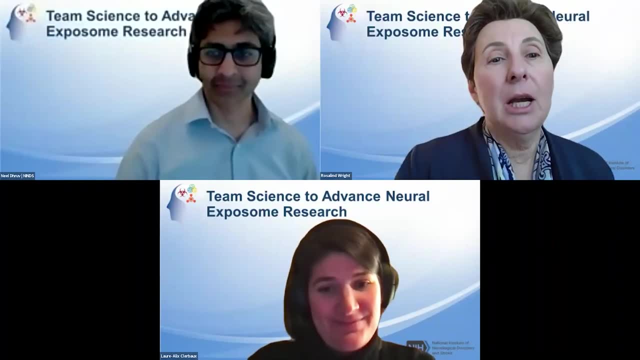 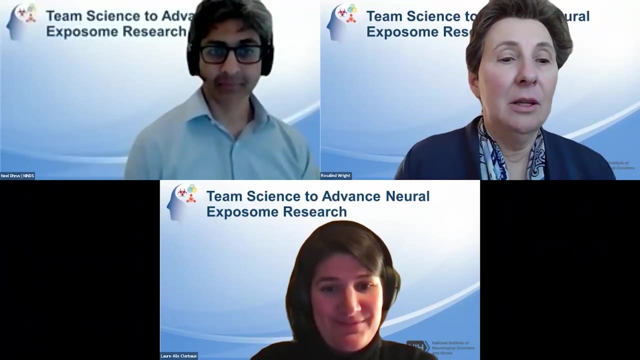 get things done. so but but I think we the takeaway is: is that one purpose the team is focused and how much can be accomplished in a very short period of time relatively. and that's what we're trying to do here: to make real impacts for exposomics in in. 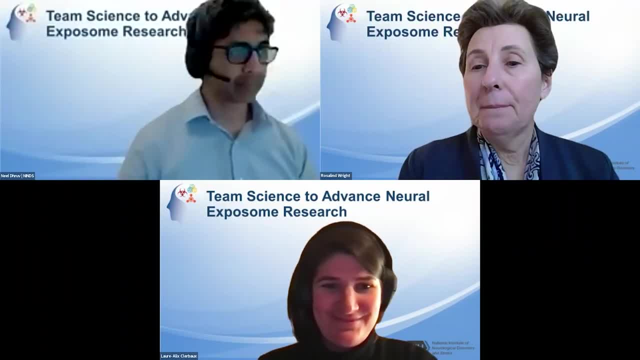 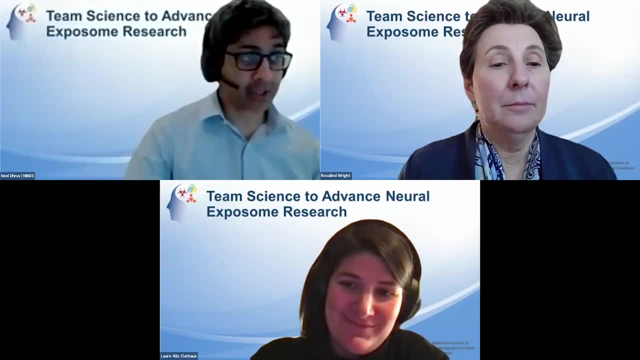 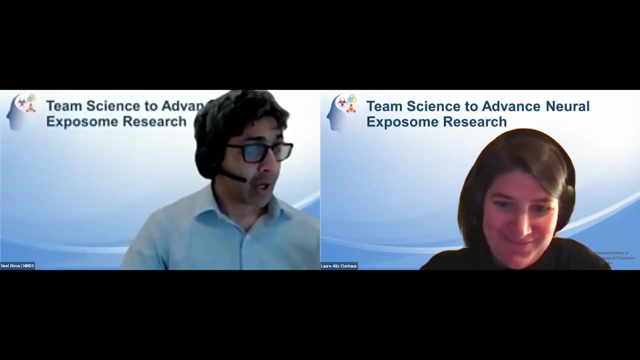 neurological diseases. yeah, great, and let's definitely follow up more on this during the discussion. um, for people that are entering questions or that, can you know, have questions, um, we're going to move on for now. you know we can come back to these during the discussion or we can. 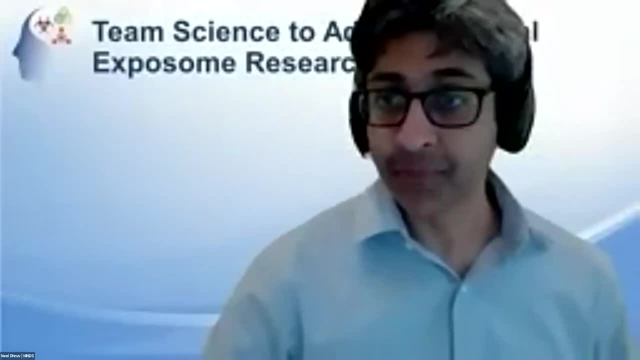 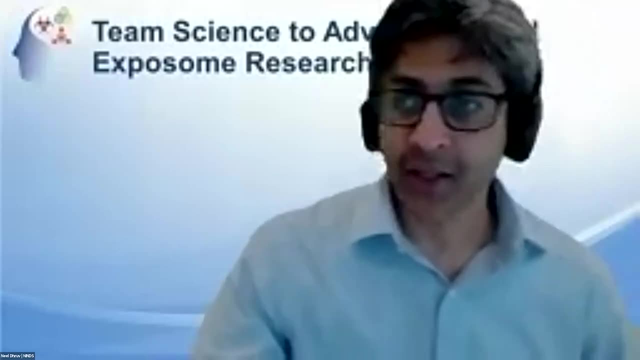 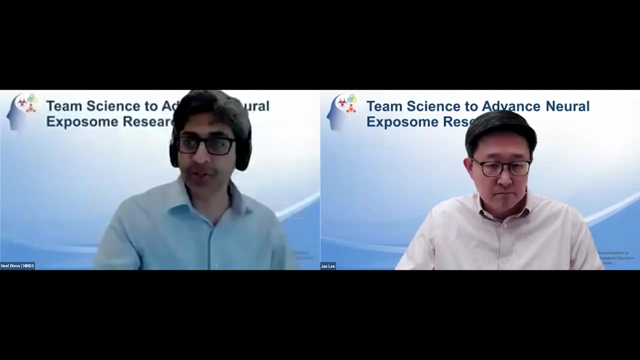 answer them in the Q&A box. uh, asynchronously. thank you very much, Dr Clerbeau. uh, our next speaker is Dr JK Lee, the Christine E Lin Distinguished Professor in Neuroscience at the University of Miami School of Medicine. he has spent his entire research career on the pathobiology of 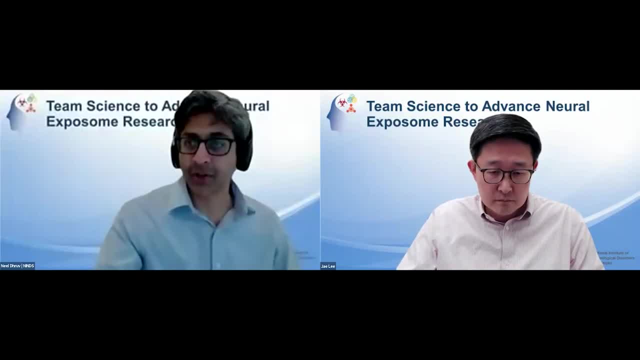 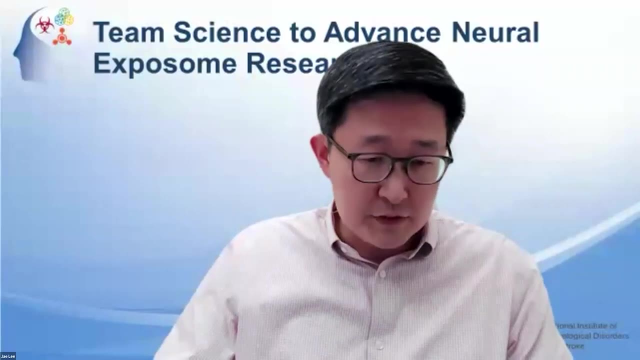 spinal cord injury, and his current research focuses on how the glial and immune response after spinal cord injury can be therapeutically targeted. Dr Lee's talk is titled fails and some successes in team neuroscience. Dr Lee- hey, thank you, Neil, for the kind introduction. let me share my slide. 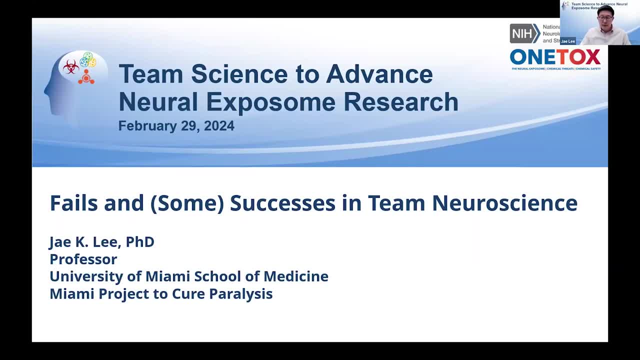 okay, so I think it's being shared. yeah, thanks again for the invitation. when um Aaron and call Corey emailed me, uh, about this talk, I I really don't didn't know know, kind of uh, what to expect in terms of the content. it was a truly a unique. 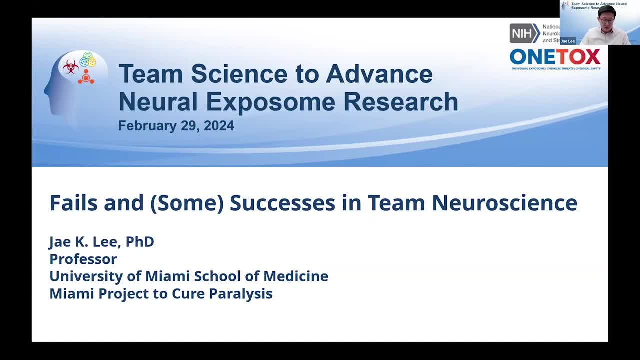 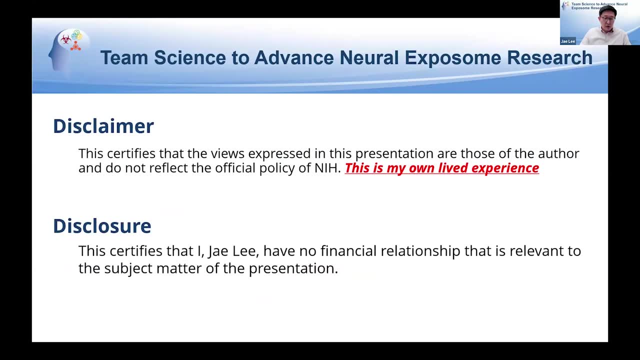 um opportunity. so I I hope that I get to meet all your expectations today. I'll start with my disclaimer slide: uh, so, uh, this is really my uh own lived experience. it doesn't represent, um, the views expressed by anyone else but me. um, so I just I'm. my hope is just that there might be. 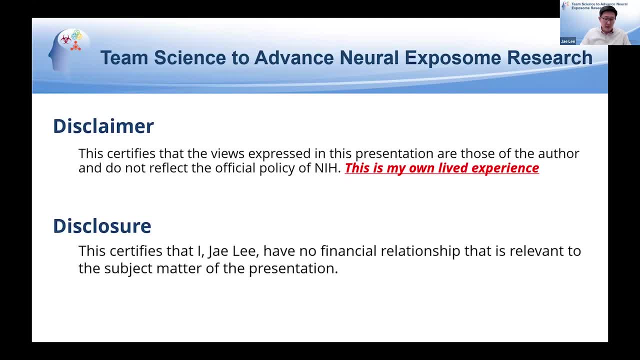 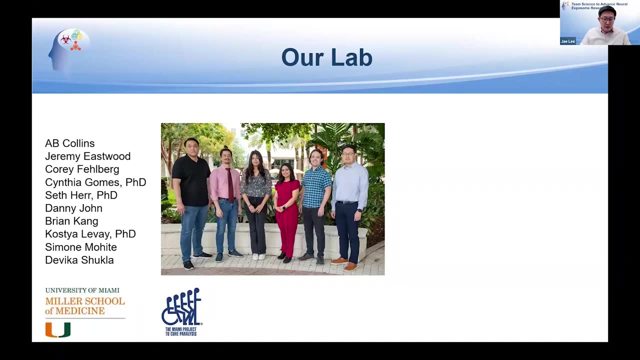 of you who can learn from my mistake, and my subtitle reflects some successes. The disclosure is that I had no financial gain from any of the slides that I'm about to present today, So I guess this is a little bit different in that I'm supposed to kind of present the 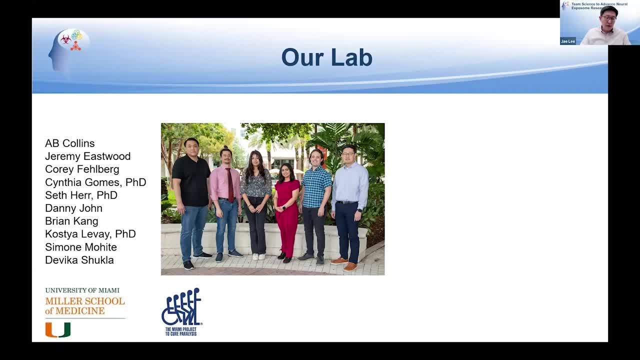 aspect from my view as an awardee of this award. So I'll start with kind of my lab and kind of what we do. This is a bit of an outdated picture. There have been some recent members that have joined, but this is my team of trainees, graduate students, postdocs and scientists. 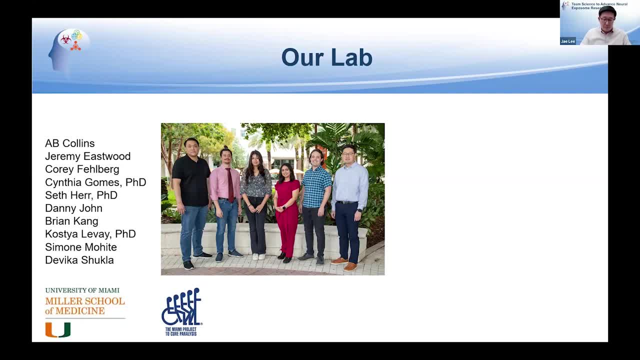 in my lab that tries to tackle a big problem in the field of neuroscience, which is that there is no cure for spinal cord injury, And so this is a little bit of a picture of what we do. This is a little bit of an example. This has been true for forever. There is no treatment, There are no therapeutics. 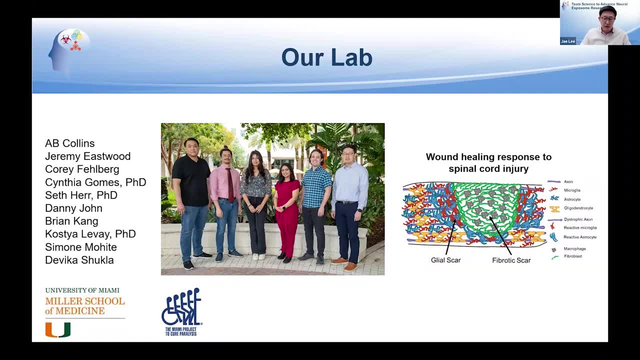 So this particular biology of spinal cord injury that I study is that of the injury site. So what is happening during the wound healing process after spinal cord injury? After the initial injury, there's inflammation, cell proliferation and tissue remodeling that leads to- Let me turn my laser pointer. 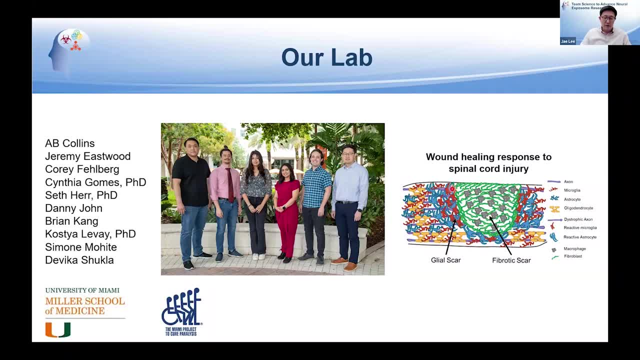 That leads to what we typically call a scar in the field- that's comprised of both neural cells- glial cells like astrocytes and microglia, and oligodendrocyte progenitor cells that surround a central core of non-neural cells comprised mainly of macrophages and. 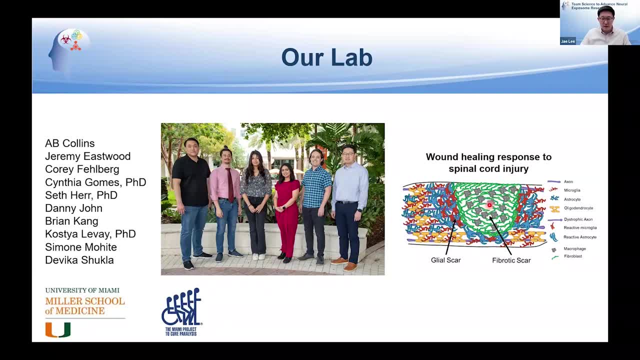 fibroblasts, And so that's kind of the biology that I study, And I think most, if not all, of us in the field realize That in order for us to make any gains in this field in terms of discovering a therapeutic 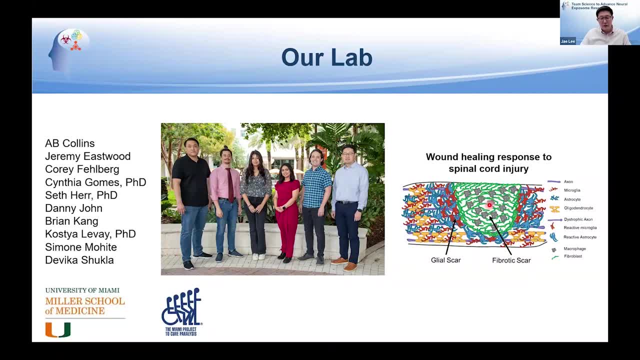 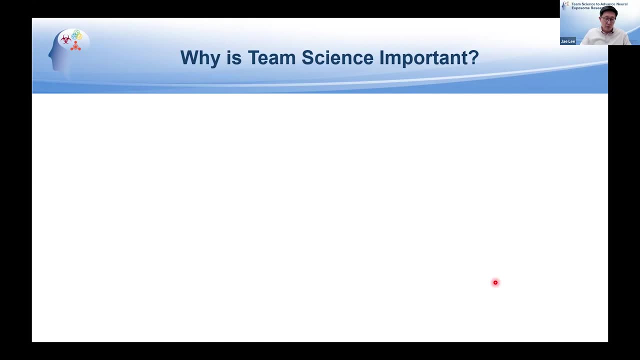 that we really need to work with others, especially those that are outside our field, to give us new insights into how we might find the treatment, And so you've heard a lot about why team science is important. I think different people will give you different answers, And 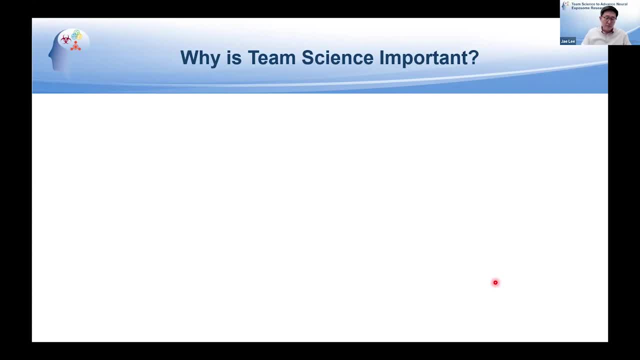 I think all of them- many of them- are correct. My view on team science has been that it really promotes creativity and innovation, things that we wouldn't have thought of ourselves. if we interact with other people, There's a light bulb that goes off in our head and 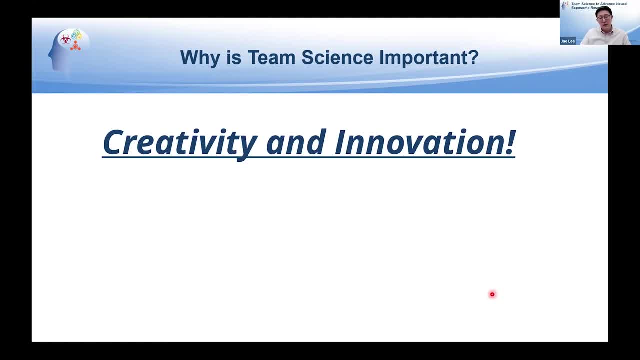 we come up with new and innovative ideas to tackle an old problem, And Steve Jobs once said that Creativity is just connecting things, And in the context of neuroscience, which I believe a large portion of the audience is from today, that has a special meaning. So connecting. 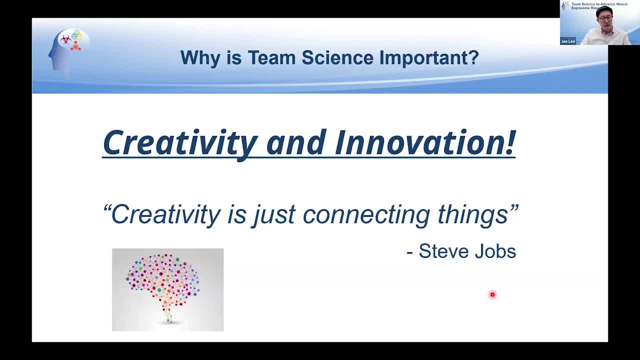 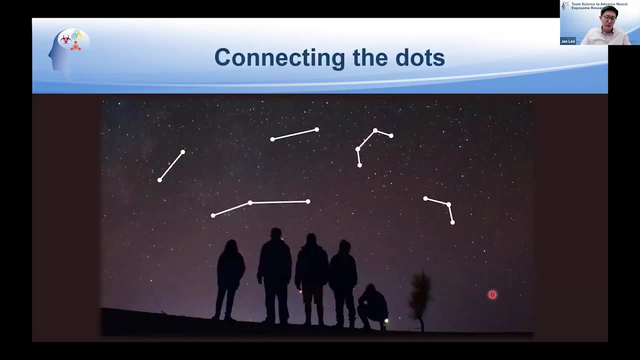 things in the brain, the connectome and that. So we kind of have that understanding of what connection means in terms of neurons and how those are certainly important for the circuitry of the nervous system. But we as scientists connect things all the time. So if you have 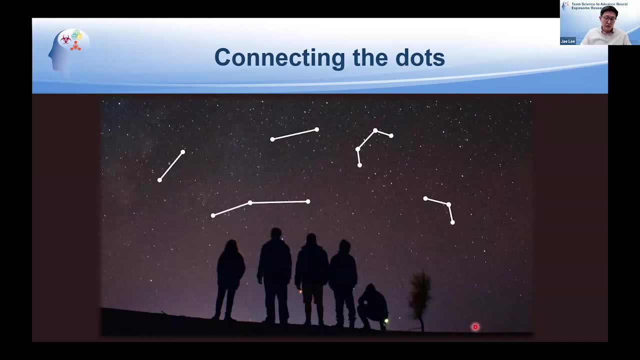 a group of people And you just think about your own scientific careers. we've all connected dots, whether it's within our field or across our fields, And we come up with new ideas when we try to do that. So I study the immune response after nervous system injury. spinal cord injury. 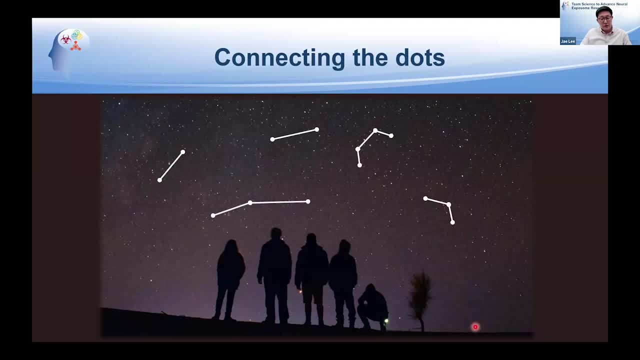 But as I received some of my PhDs in neuroscience, and when I was doing my PhD courses, you know I learned barely any immunology right. But I find myself right in the middle of studying the immune response after central nervous system injury, And so you know I've been 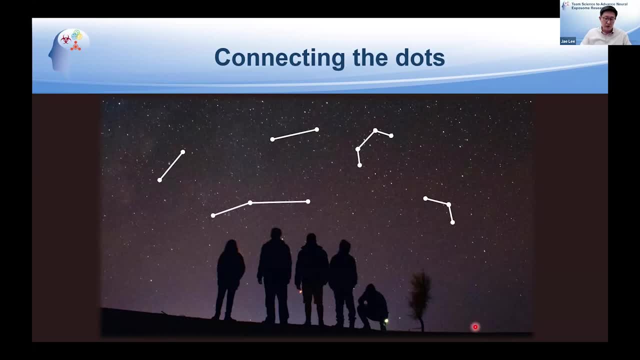 forced to connect those dots between neuroscience and immunology And I've had to learn also a lot about cell biology. So, as you know, neuroscientists, the emphasis really on neurons. Well, your neurons don't move and they don't divide right, Whereas a lot of glial cells 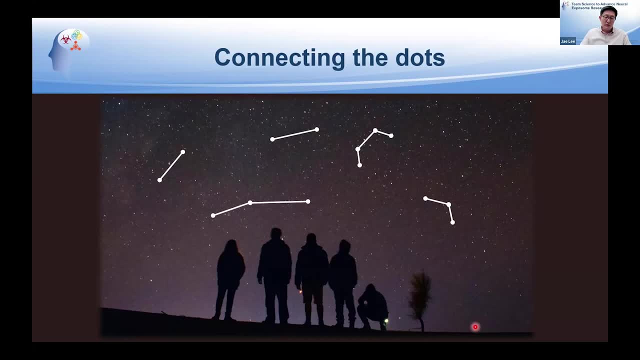 do, And so I've had to, you know, teach myself and interact with a lot of cell biologists to really learn about basic cell biology that drives the glial and the immune response after CNS injury, And so we all make these, you know, connections between dots. 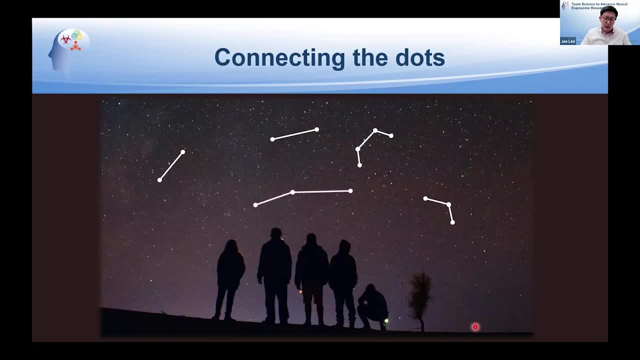 But when we work as a group, right, the hope is that all of these dots that we see and connect individually will come together into a much clearer picture that provides a much bigger impact to the field that we're in. And this is kind of the significance. you know, that's all usually we have to address. 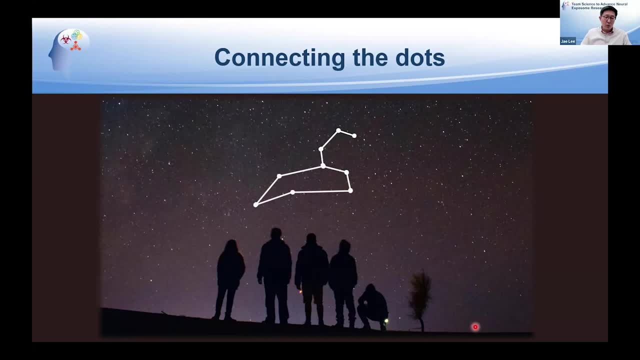 in our NIH applications right, And so we're able to address very significant problems, just like Dr Klebro just described, during the COVID times, When we come together to bring all of our resources and our past experiences to connect the dots in order to make this big. 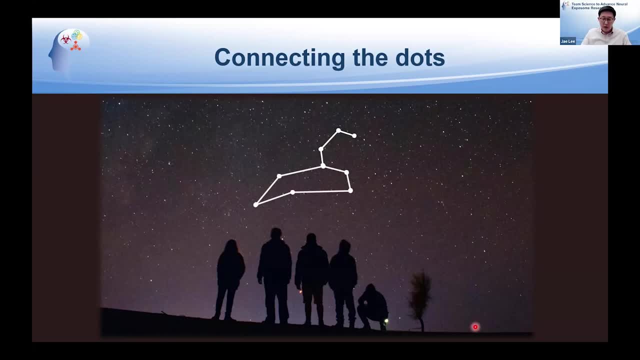 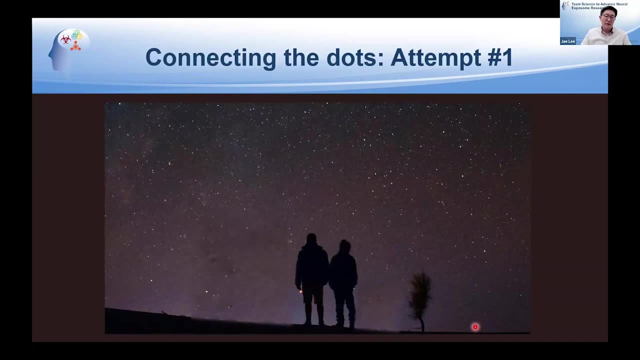 we can all tackle these big picture problems. So this is kind of quote unquote, hypothetical attempt right at tackling into connecting these dots as a team. So one day scientist one or A says, hey, I have an idea right, And so this is just during. 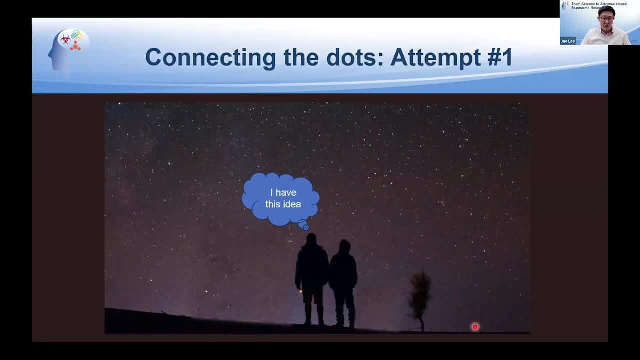 a conversation that we might have with our colleagues during a meeting, conferences, you know, or when you have an invited speaker, you have an idea, you present the idea and your collaborator or friend or colleague says, hey, I know somebody you should collaborate with that can help. 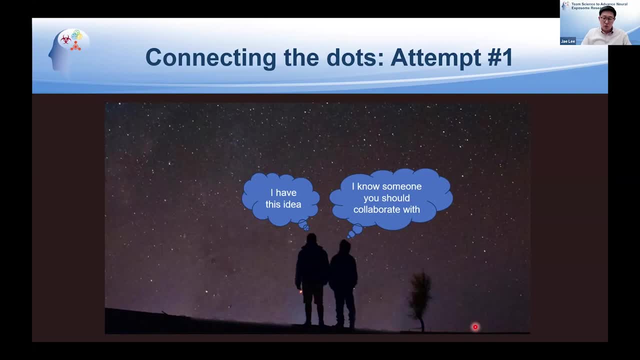 you with that idea right, And so you recruit a team, okay, and you have this vision of what this problem you're going to solve and how you're going to do it, and you write your project NIH application and then you get it funded. everyone's excited and you start. 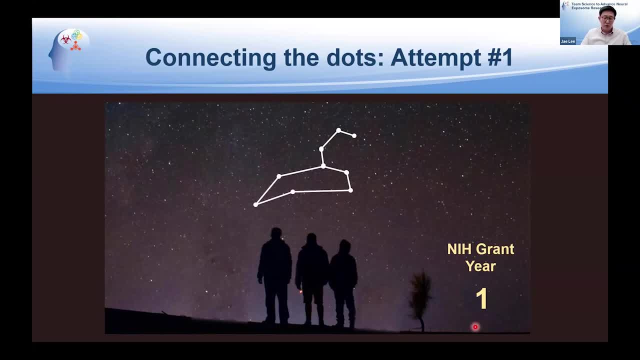 to do your project and kind of progress, you know, with the experiments that you proposed And when you initially start. obviously you know, hopefully everyone starts with a clear vision, clear goal, clear picture of what it is that we're trying to tackle, And then 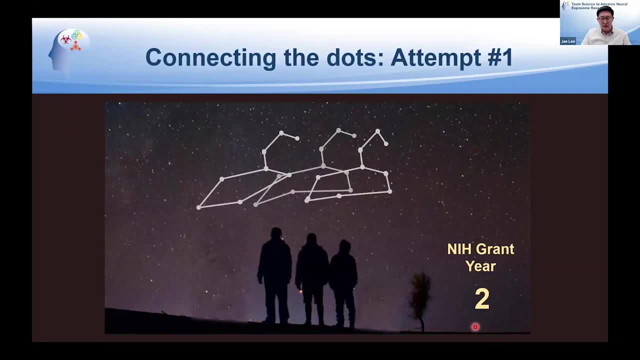 you know, we get to the year two of the project, Okay, Okay. So you know, the NIH gives its awardees a lot of freedom to pursue new directions. It's not like a contract, right? So we have this freedom, but you know, I think that 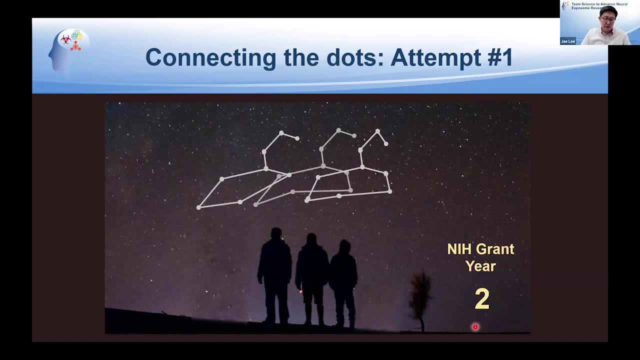 freedom kind of is both a blessing and a curse. So you know, and I think a lot of us probably have experienced this, And because of this freedom, the each of the team members start to kind of have their own vision about what this project is and how it fits into their own professional 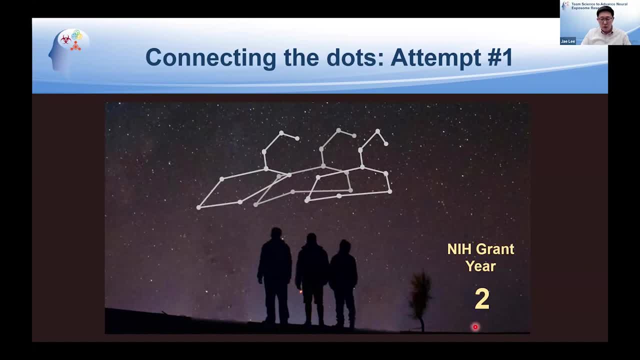 careers. And then, over time, right, the original vision kind of starts to disappear. right, The original goal, the original problem and that vision we've had together kind of starts to disappear. But not only that, members of the team start to kind of fade away as well. 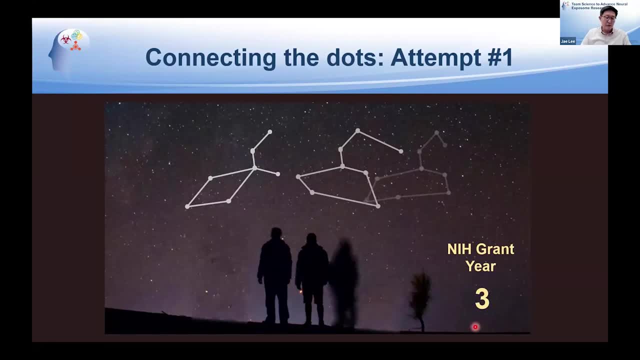 right, And that member's contribution and that vision you know is kind of going to disappear, Right, And so the vision you know, that member's vision, also starts to fade away And you're left with, now, a much different picture than you initially started with And by the end, 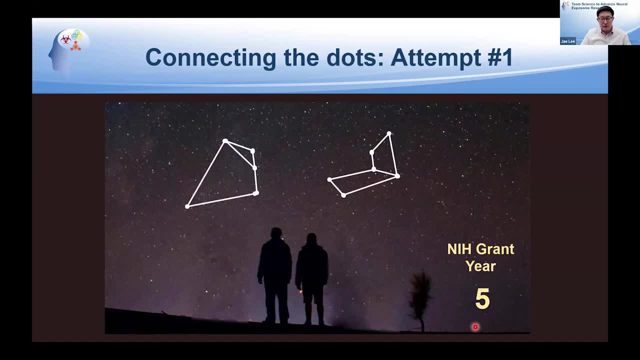 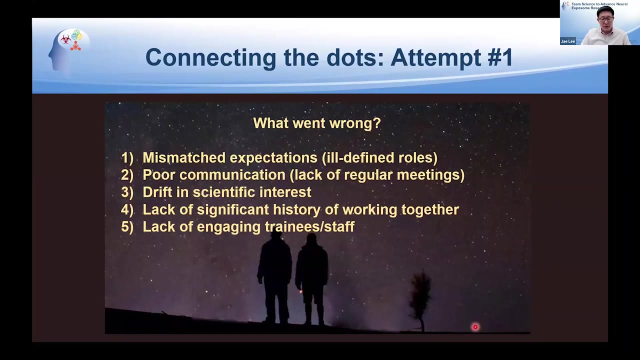 right It's, it can be completely two different visions and completely two different directions that each team member is going into, And so you know, in retrospect try to figure out what went wrong. there were many things, and I think some of the things that went wrong is that one there were 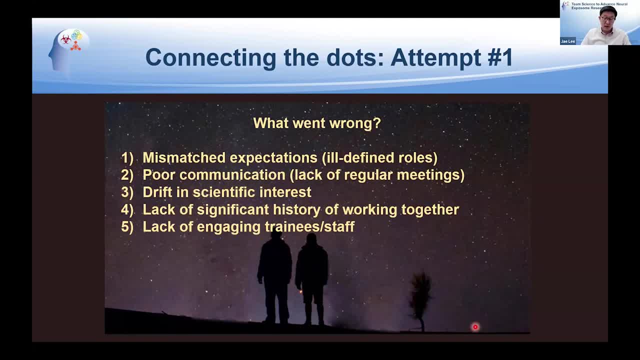 mismatched expectations. a lot of these are some of the things that you know the previous speakers already spoke about, and so mismatched expectations, and they kind of arise from the fact that there were ill-defined roles to begin with. we think we kind of know what each person or scientist. 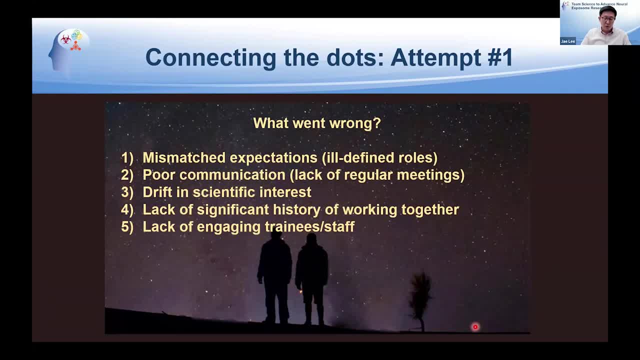 or PI should be doing. but you know, when you really try to put it on paper, it's, it's, it's really. it wasn't clear to begin with there was poor communication. there's usually good communication when you meet. I think the problem is that we tend to we're, you know, with our busy. 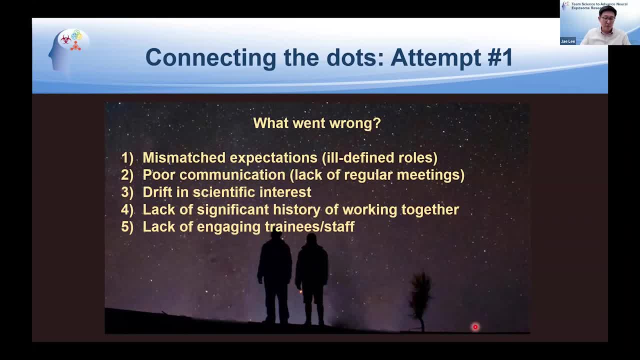 schedules. I don't think that we meet regularly enough to make sure that everybody's on the same page about the progress of the project. um, these two things tend to be the same thing, right, you know, and that tends to lead to drift in scientific interest, right? so we're doing our. 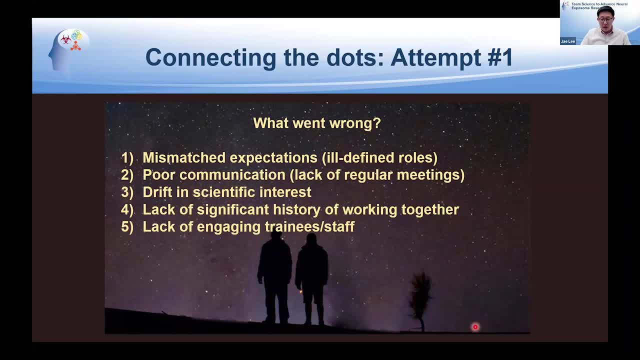 experiments. we, we think we're contributing to the goal. but you know, we all have our personal biases, whether we're conscious of it or not, and we have our personal goals and interests right. so if you take three different, three scientists from three different fields, they're going to want to. 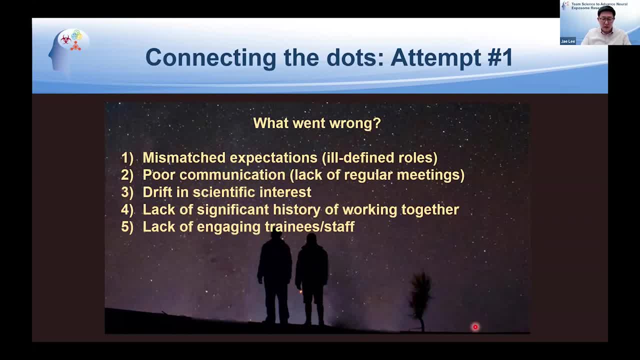 view things, to view data and view experiments and propose new experiments, context that they're most comfortable with and that tends to cause drifts um a history of working together, I think is extremely important, and and the fact that the trainees and staff that were involved in the project were not engaged enough. so when we had meetings it was just with the PIs. 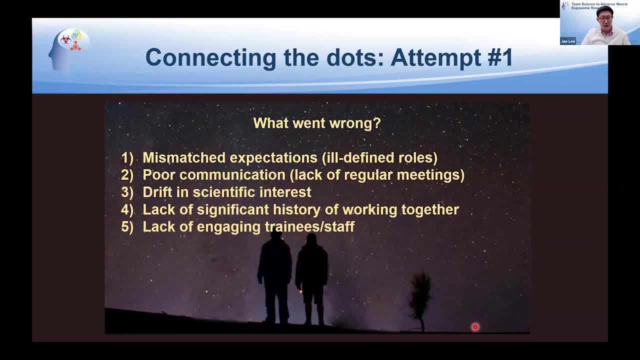 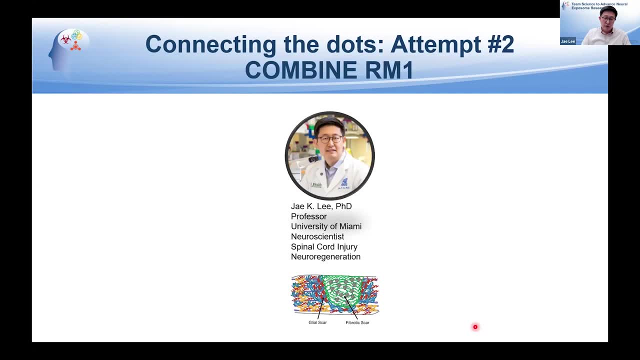 and, and I think in retrospect, that was a a mistake and so okay. so then, this is now attempt number two through the combined program. so when, the when I first received this award, I think this was the first iteration of the program. it was originally called the interdisciplinary team science program. 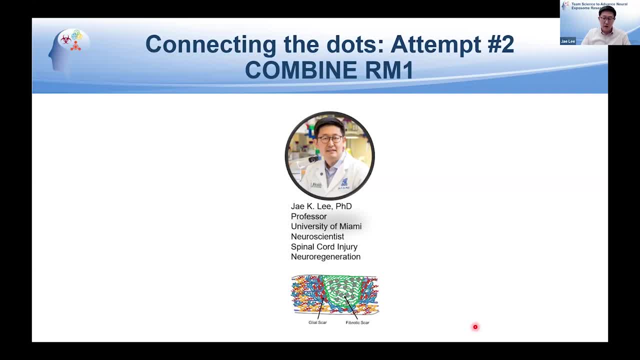 rm1 that has now been uh branded into the combined program and, as Corey and Kelly described before, um. so this is me trying to solve this uh problem of finding a therapeutic for a for spinal cord injury and you know, one of the main issues that we described in our applications- kind of the problem, right- is that. 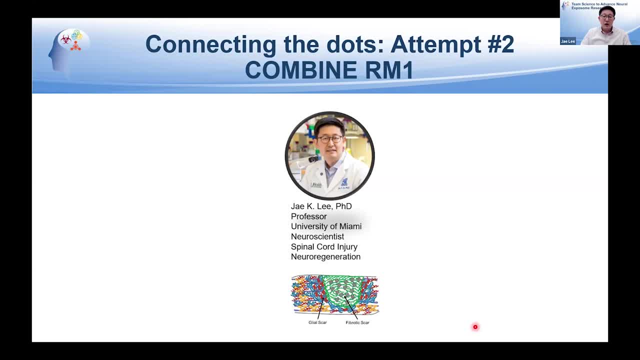 the problem, obviously, is that we don't have a therapeutic for spinal cord injury, but a major contributor to this problem- not just spinal cord injury, but I believe this is true for a lot of other neurological disorders- is that, you know, as basic scientists we study a biological 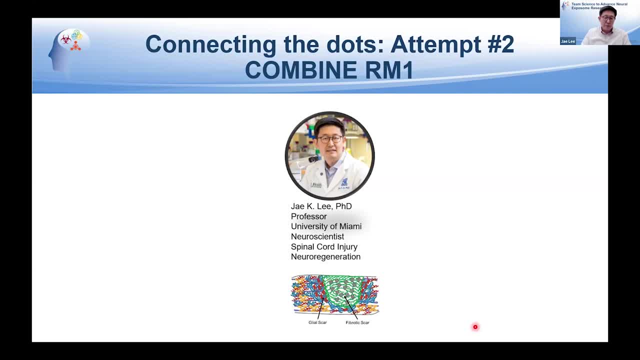 process that has relevance to some disease and that biological process tends to be in a certain cell type. so you might study microglia, you might study neurons, you might study astrocytes and then you think that oh, here is a protein that contributes this to this biological process in this particular 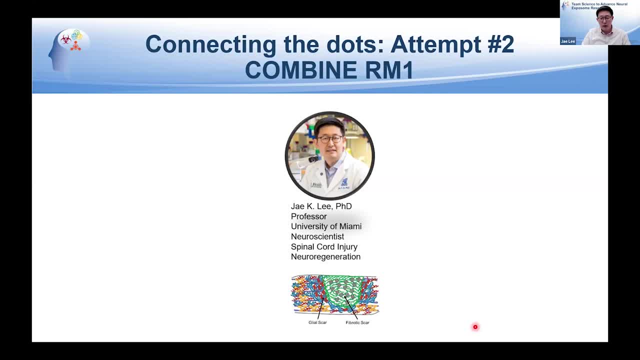 cell, and if we block this protein with a compound, it improves that biological process and and reduces the disease burden. so great. so then we now um give this drug to the entire central nervous system, completely disregarding what that drug might have, what effect that drug might have on other. 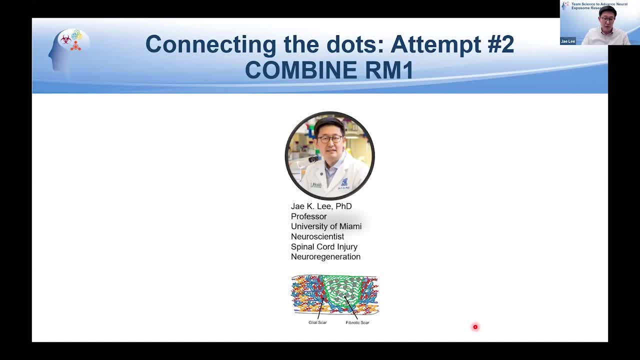 cells and other biological processes- well, similar biological processes, but in other cells, and I'm sure you can think of many examples where a same biological process in two different cell types leads to two different end results. and but this is the kind of approach that you know, that that 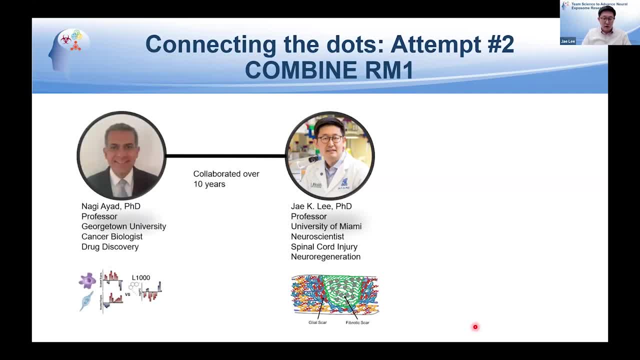 that we take um. so I had a good friend and collaborator, Nagi, who was a colleague of mine at University of Miami and recently moved to Georgetown. He's a cancer biologist And so I described, I kind of told you briefly about 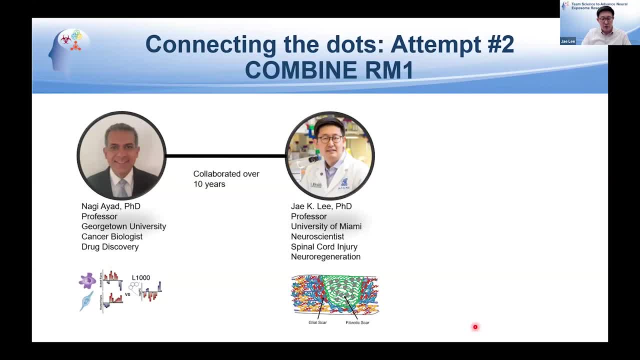 the fact that neuroscientists usually have a poor understanding of how cells proliferate and move, but cancer biologists have a very good idea of how that happens, And Nagi happens to also be involved in drug discovery. So Nagi came out with this bioinformatic platform where it takes. 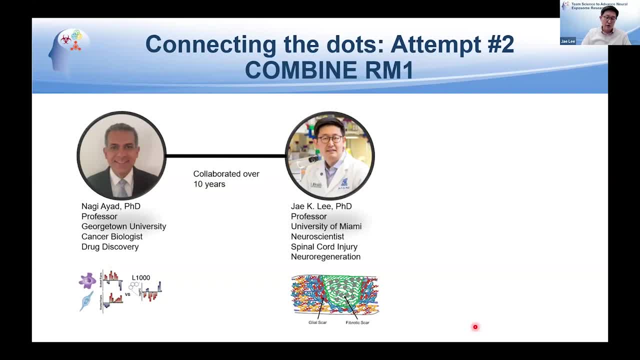 advantage of the LINCS L1000 data set to obtain, use single cell data, sets in a so from a single cell type and to calculate a disease signature for each cell type, and then uses the L1000 database to predict compounds that might. 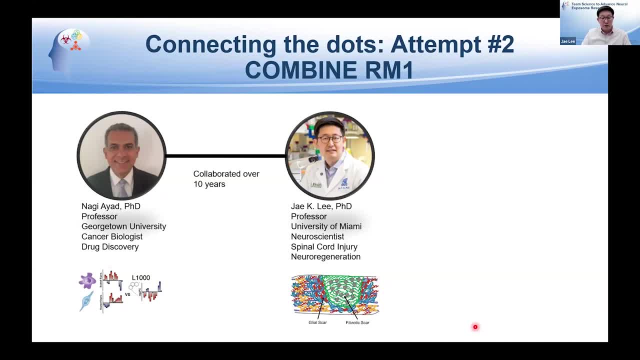 reverse that disease signature. Okay. So that was great because it was tackling a problem that I thought we had in the field. but we had another problem that, okay, so we find the drug but we still have to give it to the whole body. right, So we can find the compound that's specific for a. 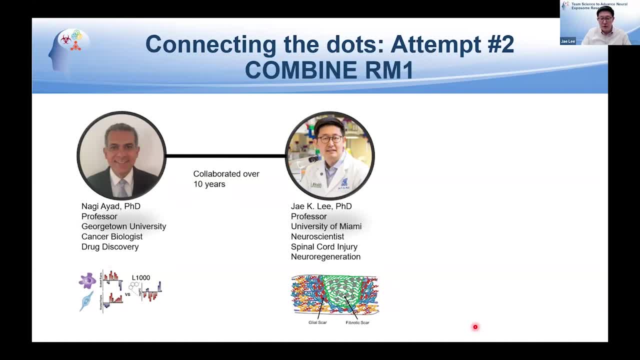 cell, specific cell type, but how are we going to give it to that particular cell? And so then enters Kibam Lee. He's a professor at Rutgers University. He's a chemical biologist by training and his specialty is in drug delivery systems, especially pertaining to nanoparticles. So I had collaborated with Kibam. 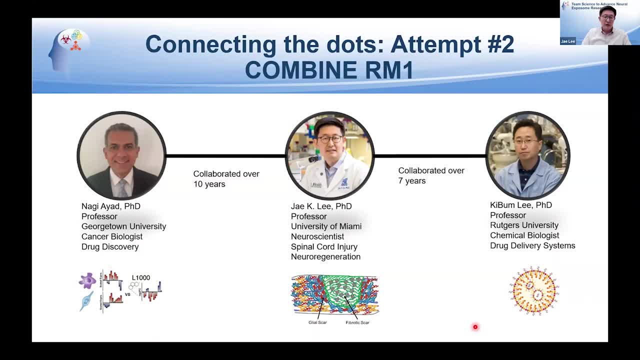 for a while We've had papers and grants together, And so because, as I served as the middle person between this team, Nagi and Kibam had never had met but never really collaborated, And so I pulled this team together to tackle these common problems. One simple problem of let's try to find a drug. 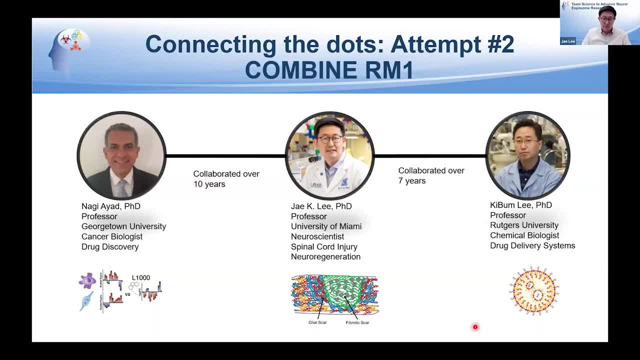 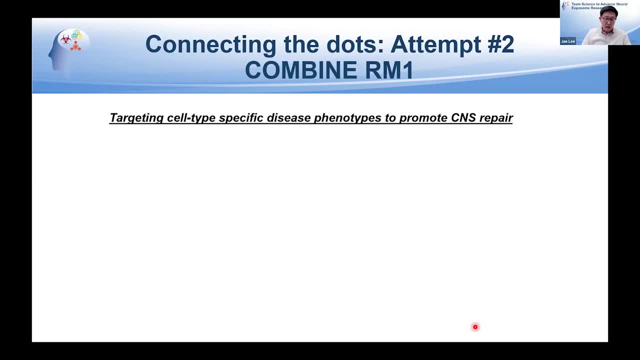 to treat spinal cord injury in a cell type specific manner, And so that has the kind of you know kind of the title of the, the application, And so I kind of described this process to you already We've. so we're taking single cell and spatial transcriptomics data set so that we can get cell. 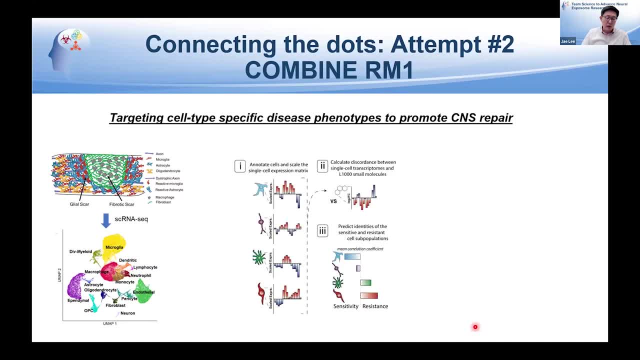 type, cell type, specific information. We put it through a novel bioinformatics platform. We'll take that disease signature to predict compounds and not reverse it. And then we make novel drug discovery platforms and nanoparticles that will be tested in animal models of spinal cord injury. 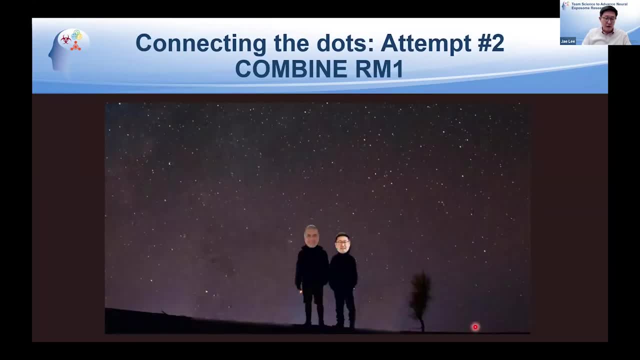 And so this conversation obviously not well, not obviously, but started just like the other one. you know, Nagi said: Nagi, we had this discussion. Nagi said: hey, I have this idea right, And so 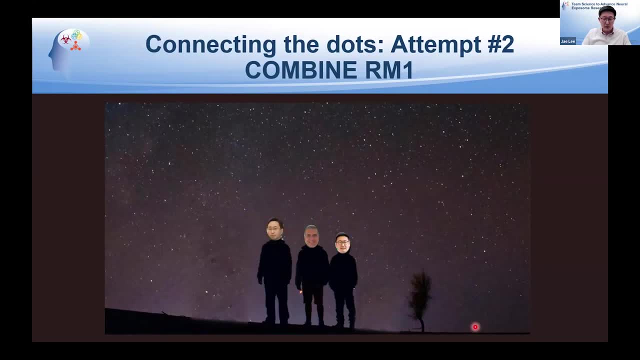 and then I said, hey, I know somebody we should collaborate with, And that's when Kibam joined the team. And so the three of us now, you know, share a common vision. okay, And in order for for us, the three of us, to really make make sure that we maintain this vision, 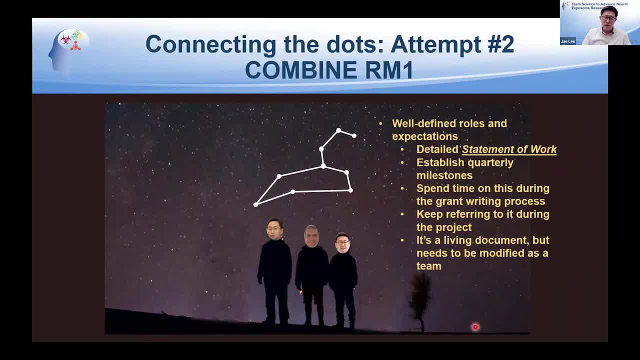 right. We knew that we had to make well-defined roles and expectations for our project, And so when we wrote the application, you know we paid, we spent a lot of time writing and detailing the statement of work And and so kind of. you know where I learned what a statement of work was when I was writing. 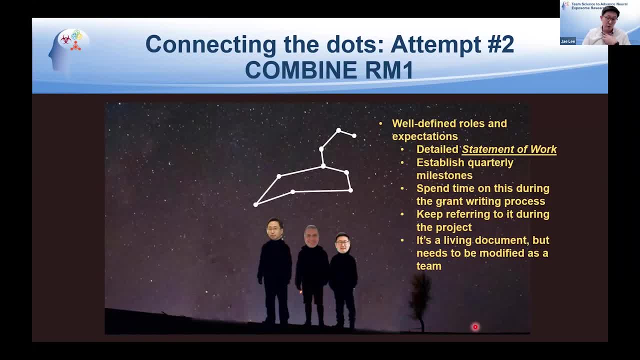 applications for Department of Defense required for for DOD applications, And, and and so kind of. I took my experience writing statement of work for DOD applications and try to apply in this. with this collaboration we established quarterly milestones And, and you know we. 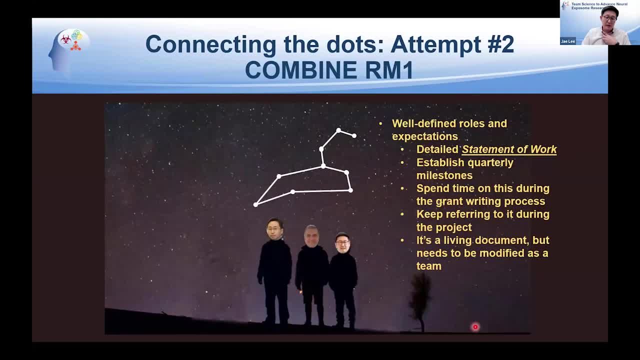 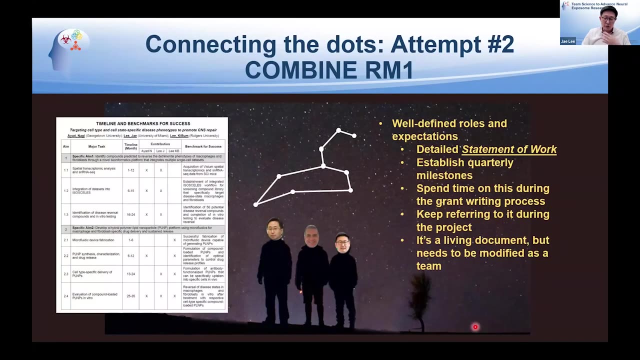 we told ourselves that it's on paper now, but this is a living document, But you know it and it can be modified as a living document, but it needs to be modified as a team and not as individuals. And so this is kind of you know, if you, if you're familiar with DOD applications. 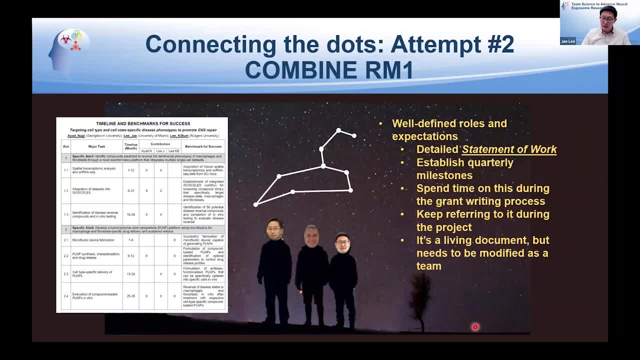 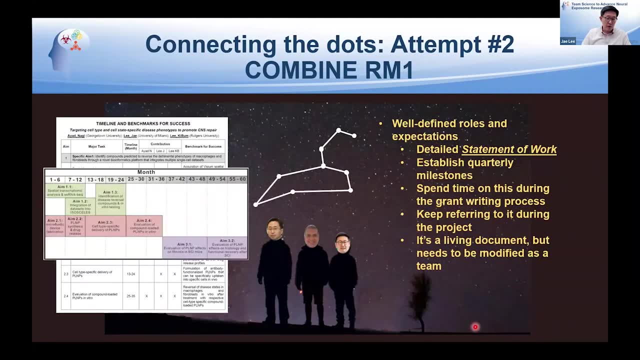 you may have seen this kind of the, the, the style, And so you know we spent a lot of time drafting this and I, and as well as the GAN chart that Corey and Karen mentioned before, And and so 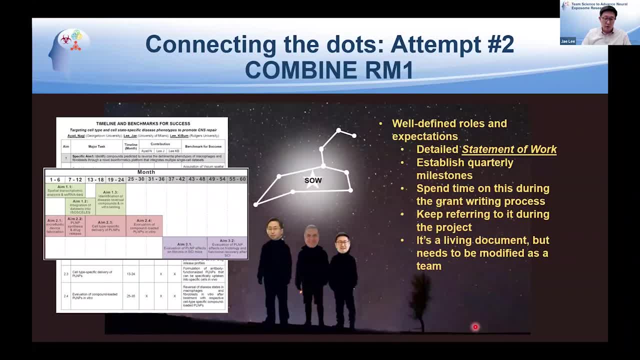 you know, we told ourselves that this is now going to serve as our North Star, so that whenever you know we are are kind of facing issues with progress or directions, we're going to refer back to this. In fact, we refer back to this regularly. 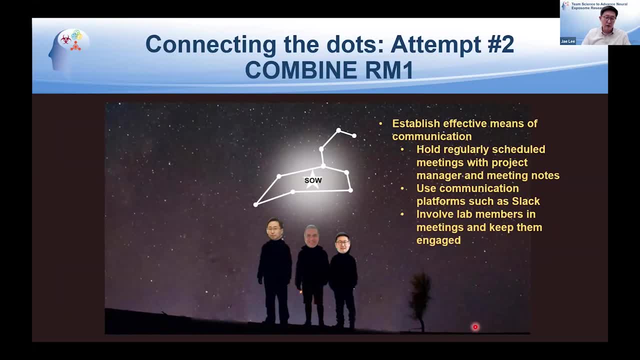 and that gets to kind of my next learning: learn experience, which is established and effective means of communication. So I think this is also really really essential to a successful collaboration And we, we're going to communicate, um, but we don't don't think we give up enough ourselves enough. 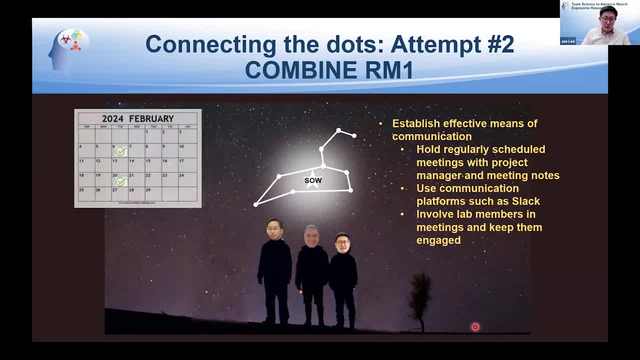 infrastructure for this to occur. so i think one thing that you know that we as a team- uh kind of told ourselves is that we're going to have a week regularly scheduled meeting every two weeks. obviously, when we launched the project it was weekly, but then it moved to bi-weekly. 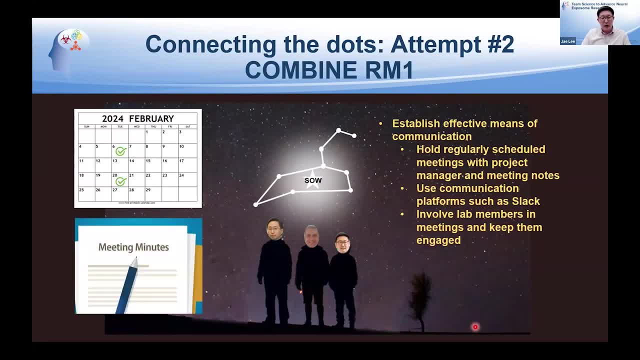 um, and then we designated our project manager, which is uh required for this rm1 mechanism, to take careful meeting notes, and there are lots of resources on how to take meeting notes appropriately. and then, uh, but you know, we don't want to just communicate every two weeks, we want 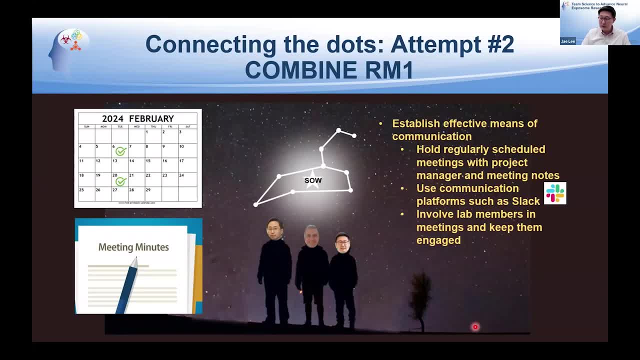 to make sure that there is a mechanism for ongoing communication, um, and so we are. we utilize slack for that. so when we have new data that we're excited about, or just something that we're овые to send out to the group, we use slack to do that. um, and you know it's. i think it's really. 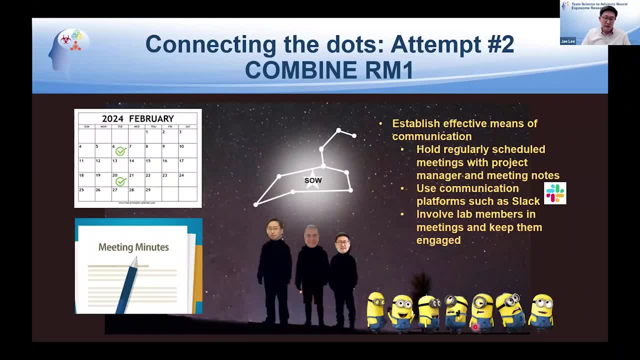 really important that we keep our the team, the trainees and other staff members engaged in our in in the project. uh, they actually seem to enjoy it very well. um, i think the impression that i've had so far is that they really like learning about other fields. they like being part of this novel. experience, where they're really interested in the local approach of houses, where they're really good for dealing with making communications available to the group, which is one of the most important. it seems like it's much more important to be able to get more information about the project and 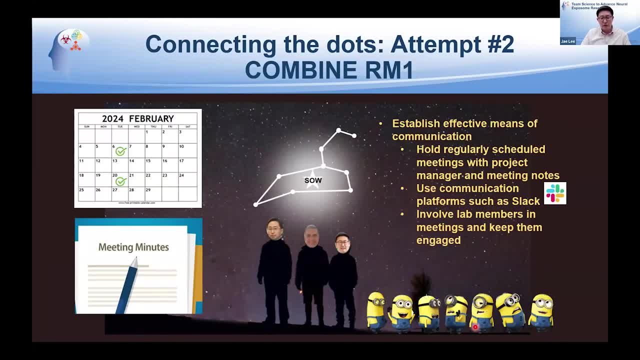 they're probably going to be willing to stay for a few years to get that time, um, but one of the things is that they're really excited about really being able to see the impact of that project, which is where it's truly interdisciplinary and truly a team work. 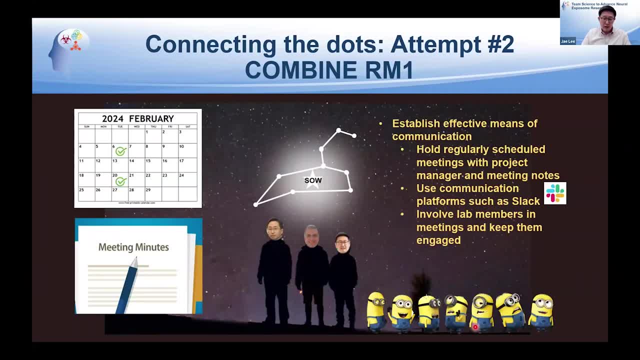 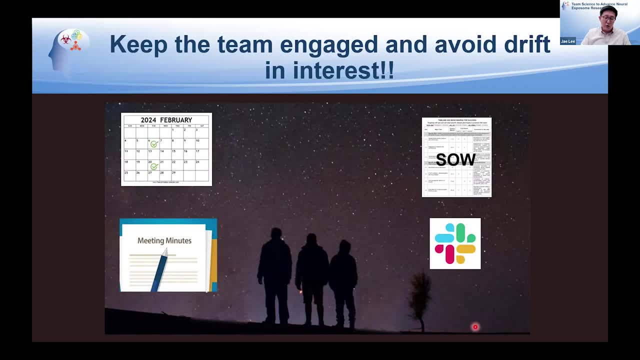 I think they like participating and learning about how to do this, But this takes a lot of resources, And so I think, if you estimate that in a percent effort you're gonna be spending 25%, you should probably put about 20% more than that. 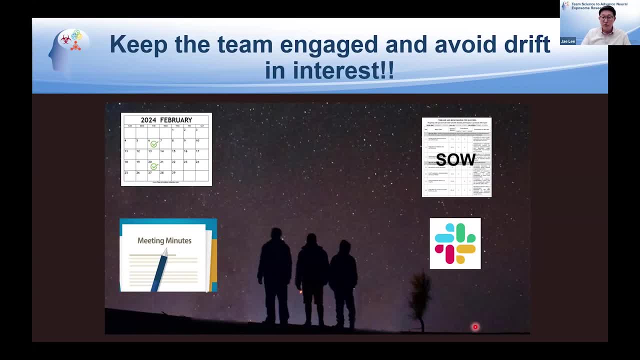 because working as a team takes a lot more effort than working alone, And you really need to set that firm aside to allow yourself to do that, And so these are the things that I think has been helping us so far, And I will stop there. 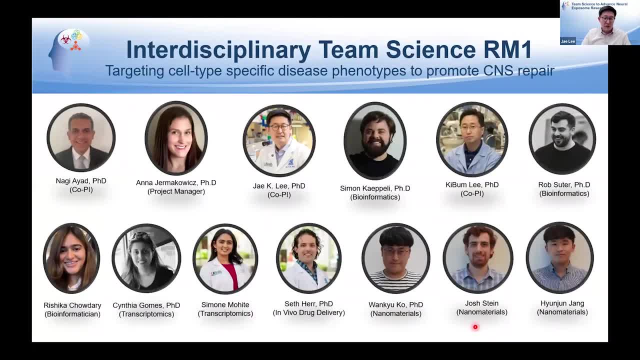 because of time, except one more slide, sorry. So this is the actual team. The PIs I've introduced before, but there are many other. which I should emphasize is a diverse team across race and field and professional status, And so these are the people. 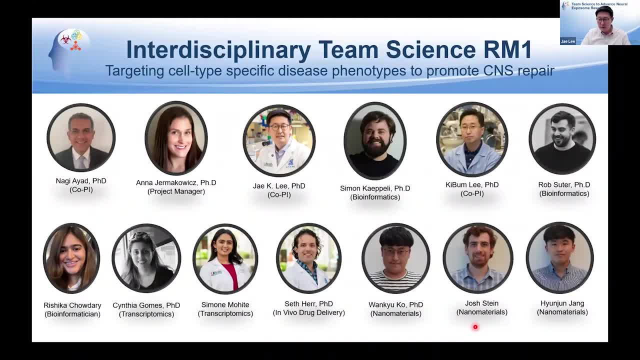 that have been contributing to this project so far, And I'll stop there, Okay, Thank you. Thank you so much, Dr Lee. We have time for maybe one short question- I don't know if there are any, or we can just reserve them for the general discussion. 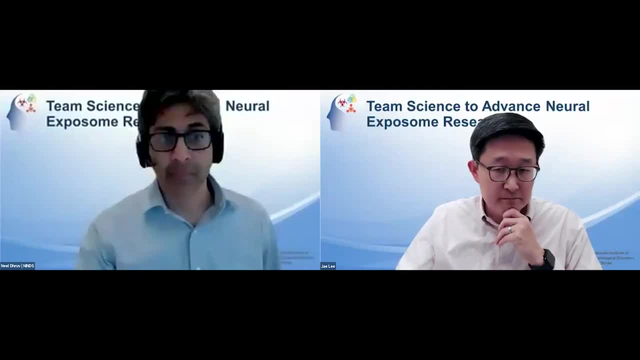 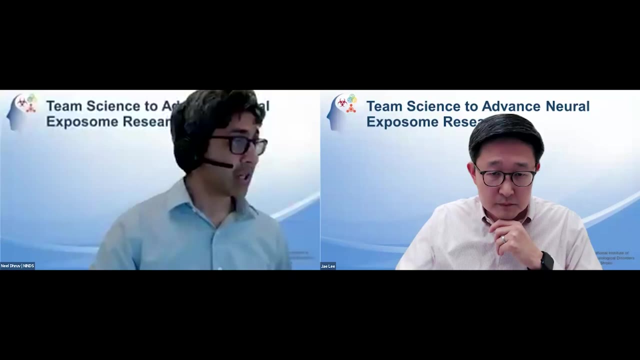 We've got time 꺠 for questions you'd like to ask better. Any other questions? Okay, There's one question in the chat for Dr Lee. Yeah, So, Dr Lee. the question in the chat says: did you have meetings that combined in-person? 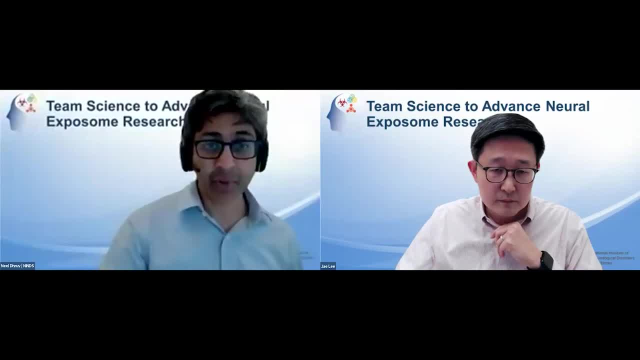 and remote participants, And are there any lessons that you have to share from that Right? So, Tom, you met up. Yes, So our bi-weekly meetings are through Zoom because of geographic reasons, but our kickoff meeting was in person. 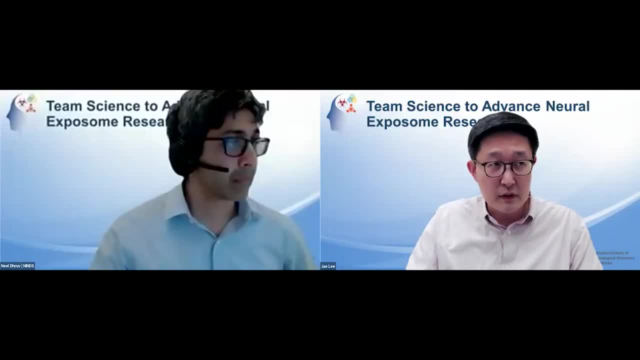 And that was fortuitous because it all happened – last year's SFN happened to be in DC and because one of the PIs is in Georgetown, we kind of had a chance to meet there. So and then from that, based on that experience, we told ourselves that we're going to have annual in-person meetings, because it was such a fruitful event, especially for the trainees, and so we're going to try to have our annual meetings in person. 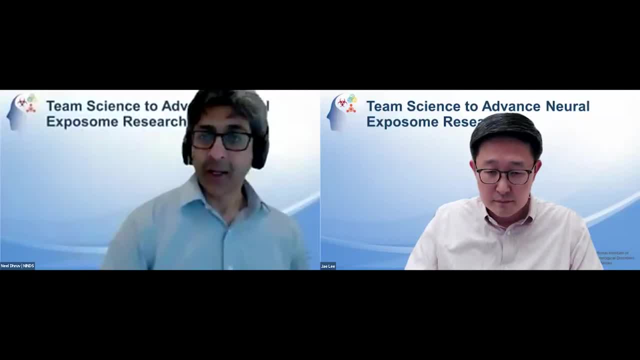 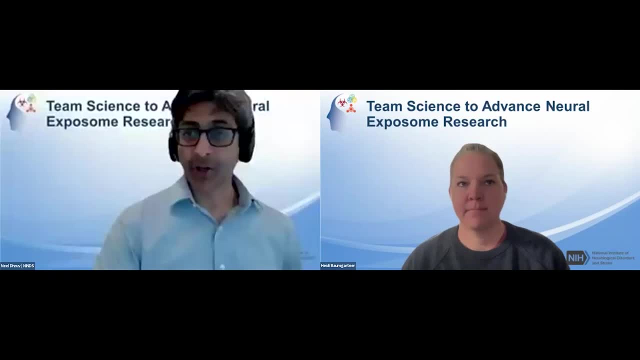 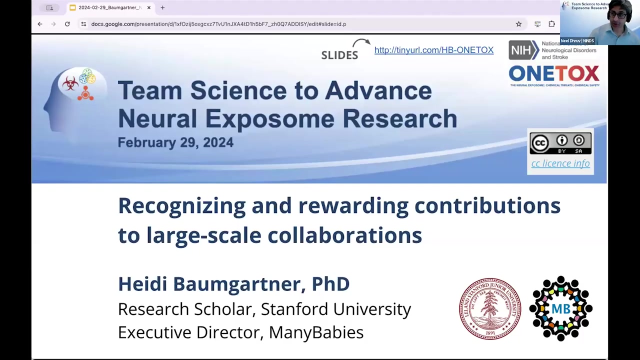 Okay, That's great. Thank you Okay, So moving to the next talk. Next we have Dr Hyde. Dr Hyde Baumgartner, a research scholar at Stanford University. She is the co-director of the Stanford Big Team Science Lab and executive director of the Many Babies Program, an international collaborative network in developmental psychology research. 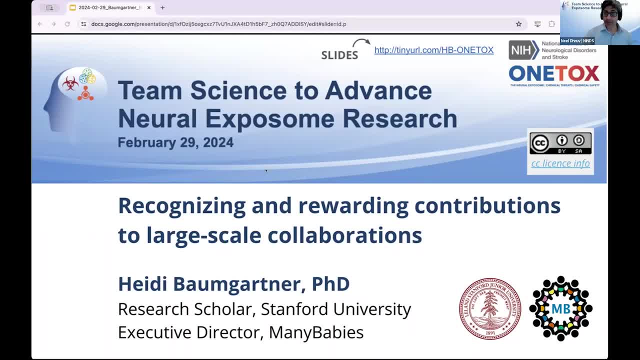 Dr Baumgartner will give a talk titled Recognizing and Rewarding Contributions to Large-Scale Collaborations- Hi, Thanks so much. Can you see my slides? okay, Yeah, they're great, Okay, great. So let me start out by thanking the organizers for inviting me to talk to you guys today. 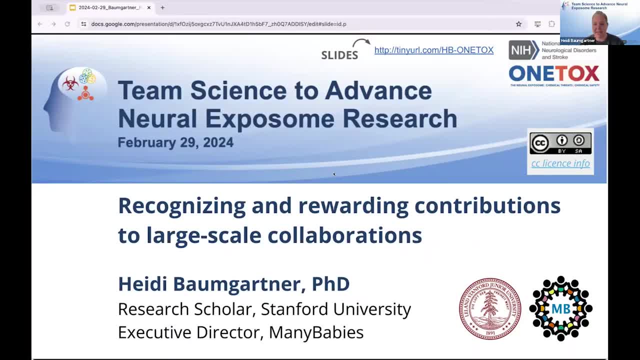 I'm Heidi Baumgartner. I'm a research scholar working at Stanford and I'm an experimental developmental psychologist by training, and my main job is as the executive director of a large collaborative network of developmental psychologists called Many Babies. So I'll talk today about some work that colleagues and I have done recently regarding recognizing and rewarding contributions in these large-scale collaborations. 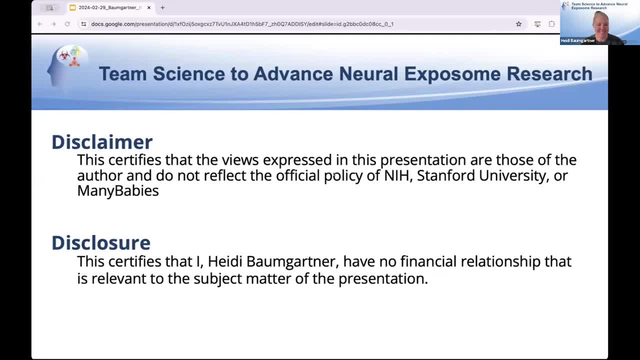 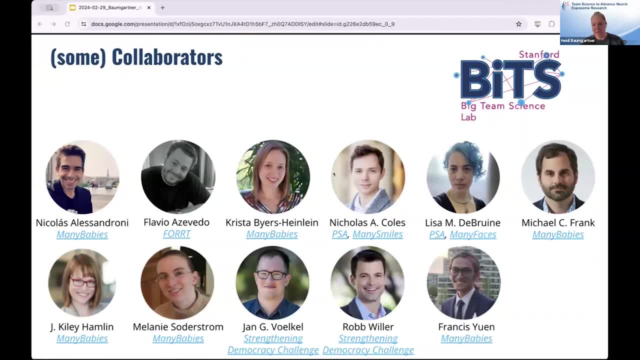 This is just my disclaimer. I have no conflicts to disclose. I want to just start by acknowledging the folks whose work I'll be talking about today. So a few of us who are based at Stanford started a group a couple years ago called the Big Team Science Lab. 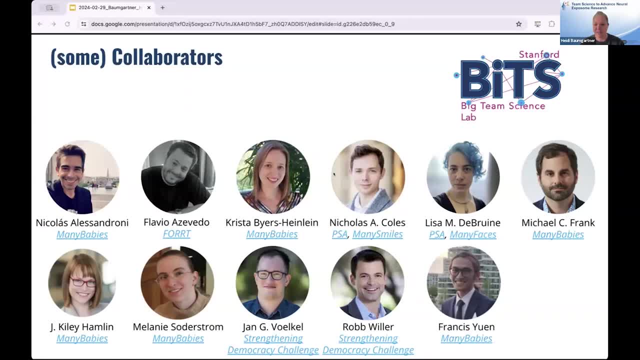 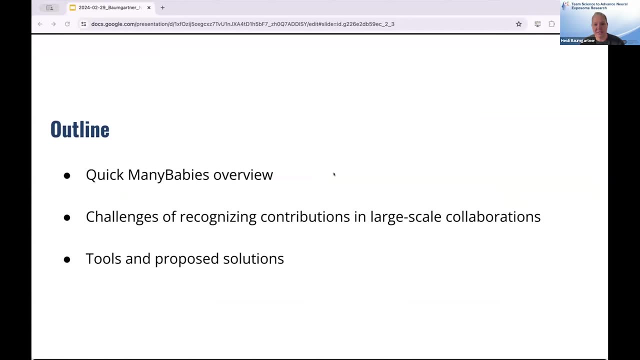 And we invited people who are working in various big team science efforts to join us, and so some of the work that I'll be talking about stems from work that this group has done amongst our larger collaborative teams as well. Just a quick outline. I'll start with a very brief overview of my group- Many Babies- and then I'll talk about some challenges of recognizing contributions and large-scale collaborations and then move on to some tools that we use and sort of proposed solutions that could be implemented in the future. 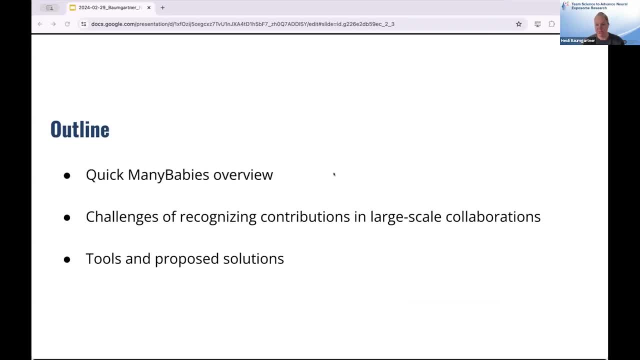 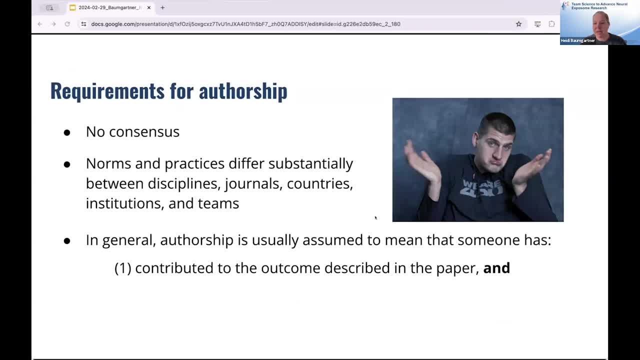 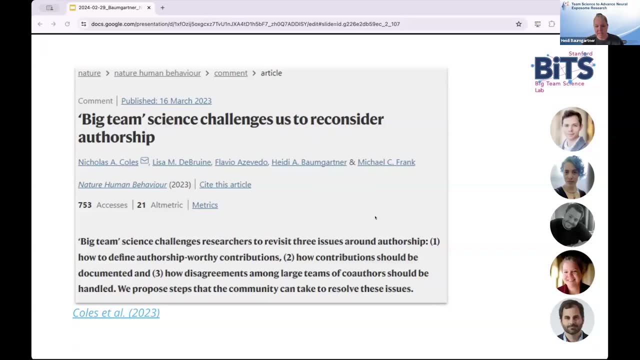 both contributed to the outcome described in the paper and agrees with the content of the paper and assumes some form of responsibility. But are these the right assumptions, especially in the case of large collaborations? So our group has recently been thinking about this question. We have this commentary that came out last year and we talk about how big team science can. 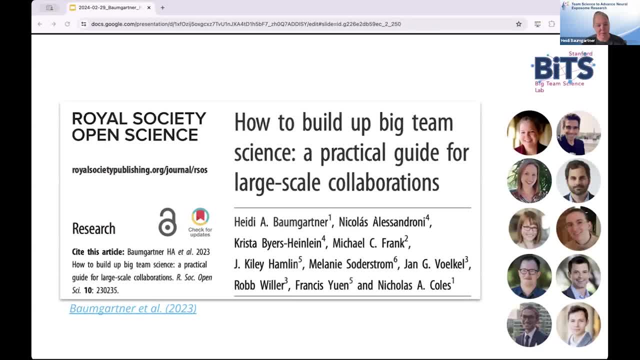 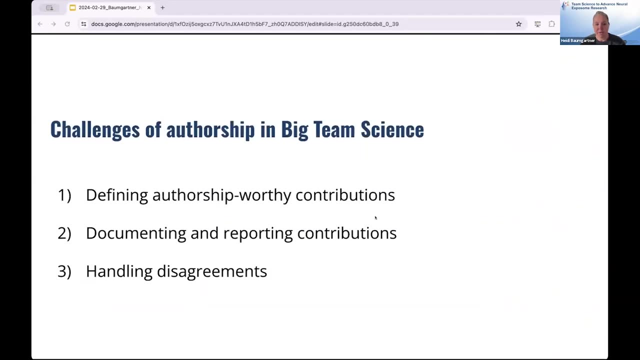 challenge traditional assumptions about authorship And we have another paper that also came out last year where we sort of compiled some of our experiences into practical advice into starting and managing large-scale collaborations. So, with regards to authorship, we identify three ways that big team science challenges authorship. So I'll go through each of these. 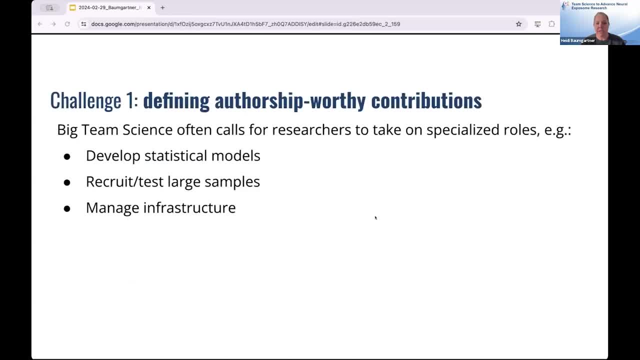 pretty quickly. The first challenge is how to define authorship, And so we have a lot of questions about how to define authorship, And so we have a lot of questions about how to define authorship, And so we have a lot of questions about how to. 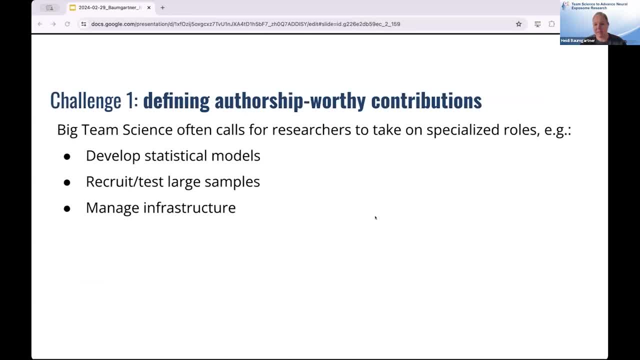 define authorship-worthy contribution. So big team science often calls on contributing researchers to take on specialized roles such as developing statistical models, collecting data or managing infrastructure. While you might fill all of these roles for a typical project within your own lab, 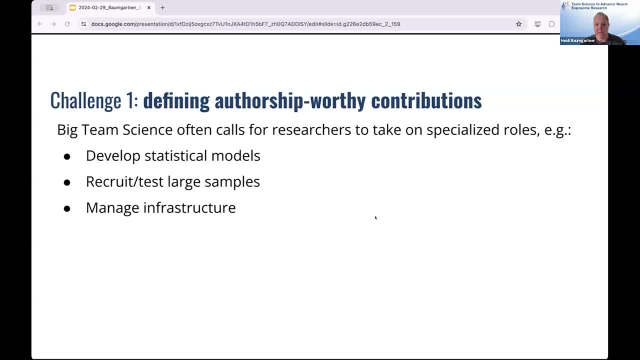 you might only take on one or a subset of those roles in a big team science project. So, even more so than in single lab projects, there can be ambiguity around which contributions are authorship-worthy. So, for example, do contributing to things like translations or project management. 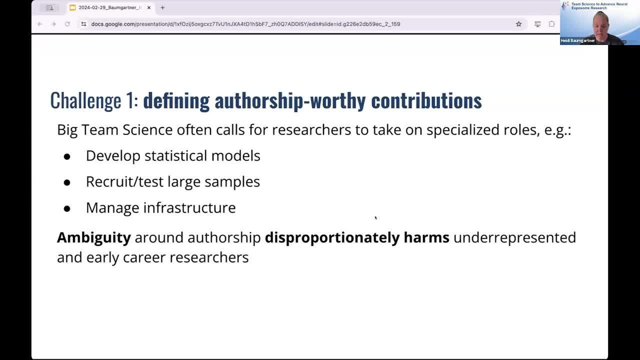 or infrastructure development count as an authorship-worthy contribution to a project. Moreover, this ambiguity tends to be it tends to disproportionately harm less powerful researchers, including those from underrepresented groups, and early career researchers who might not have the sort of knowledge of the. 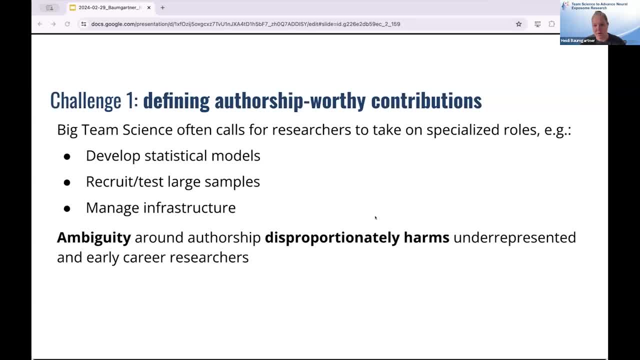 the unwritten rules behind authorship, or don't have you know experience, or you know powerful mentors to advocate for them. So, in general, ambiguity tends to serve those who are already in positions of power and disproportionately harms those who are not. 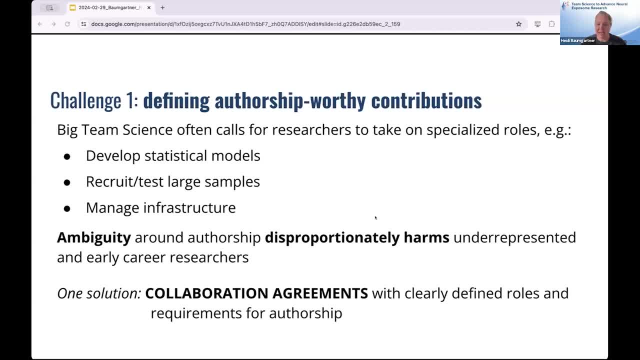 So one solution that's come up in a number of the talks already today and that I really advocate for are collaboration agreements which documents it's clearly defined- roles and responsibility as well as requirements for authorship, And this should- these things should be clearly defined and shared with all, both current and prospective- members of a research team as early as possible and throughout the project. 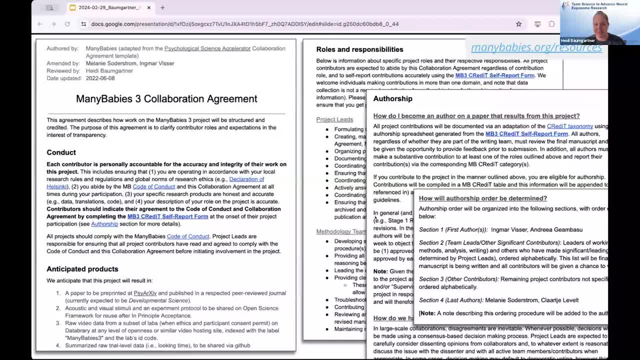 Okay, so actually I think Corey shared sort of a screenshot of our collaboration in his talk earlier. This is a lot of text to be on a slide. Don't worry about reading this. There's a link at the top of the slide. 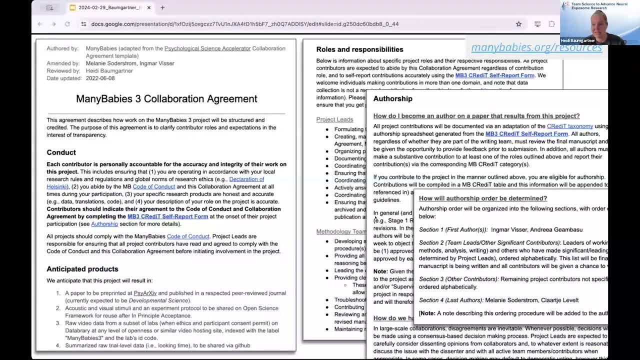 where you can view this on your own time if you'd like. But I just wanted to show you know we have sections on expected conduct of participants, the anticipated products of the collaboration, various roles and responsibilities, how authorship is defined and the planned authorship order, things like that. And again, as Jay just mentioned, we consider these to be living documents. 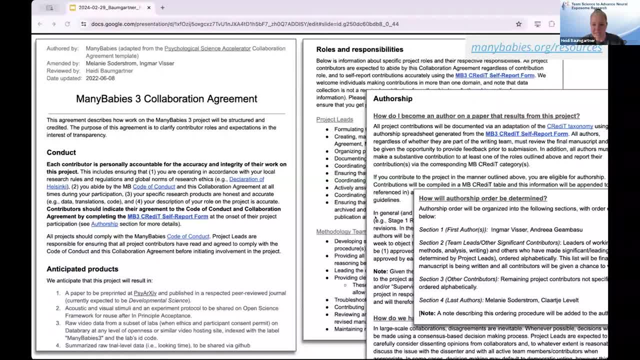 So this, from our perspective, is not to be like a formal legal contract. It's rather meant to be a transparent outline of project expectations as a way of reducing ambiguity and ensuring that all collaborators on the same page as authorship. I sometimes think about this as sort of like project insurance, So it gives you a chance early on to think about you know what your plans are, what could potentially go wrong, and gives you a way to think about. 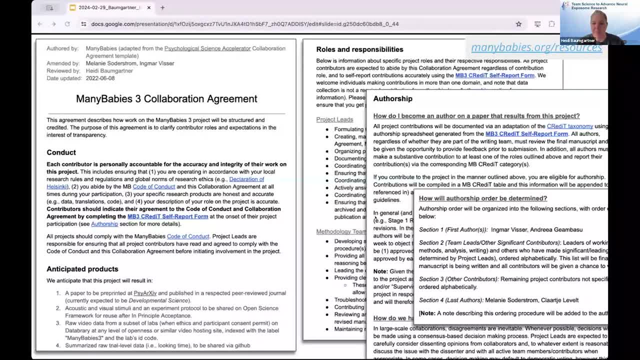 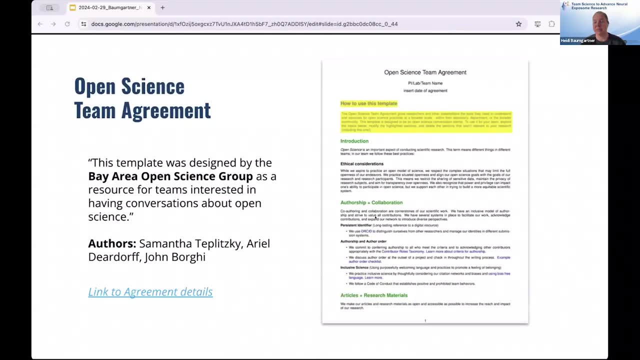 how you'll handle disagreements as they come up, rather than waiting until something has gone wrong, by which time it's kind of too late to plan for Okay and here. so that was our collaboration agreement. I'm actually we've been thinking about trying to reformat and simplify ours. 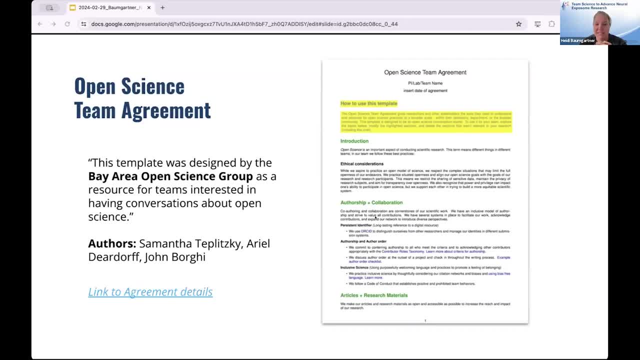 And I recently became aware of this document called the Open Science Team Agreement, which is drafted by the Bay Area Open Science Group. I highly recommend checking it out, This great resource at the link I've provided there. It covers similar things as our collaboration agreement and is just a really great tool for any type of large team. 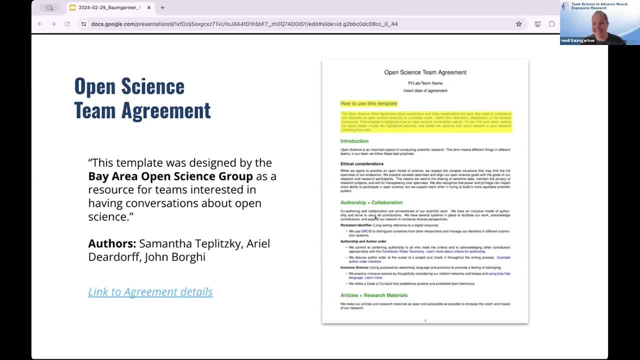 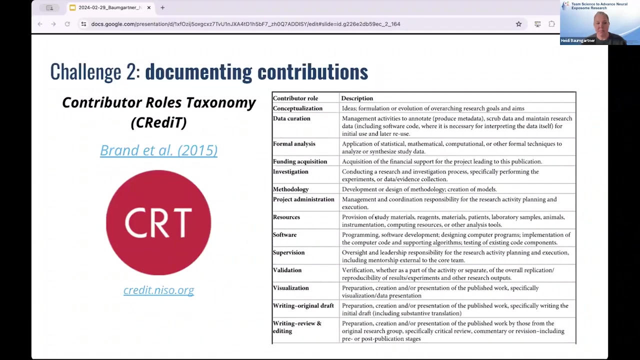 And I will say not just large teams. I advocate for these types of agreements even in single lab settings. Again, any way that you can reduce ambiguity and anticipate issues. It might seem like overkill if you're working with a small team, but it's really a great resource to have. Okay. so moving on to the 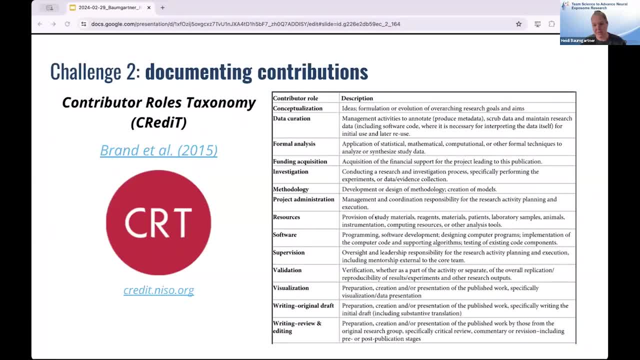 next challenge, which is okay, once you've decided what an authorship-worthy contribution is, how do you document it? So our group, as well as many of our peer groups, have adopted the contributor roles taxonomy, known as credit. This has also come up in a number of the talks. 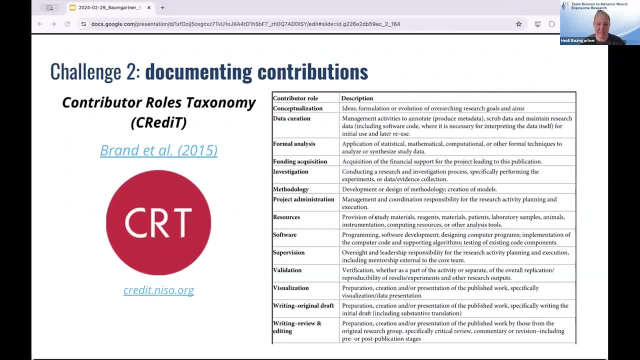 This has become the standard across a number of fields in science, So there's 14 categories. If you're not familiar with it, there's a link there to the NISO website that has a better description of the taxonomy, but there are different categories and they've provided a short. 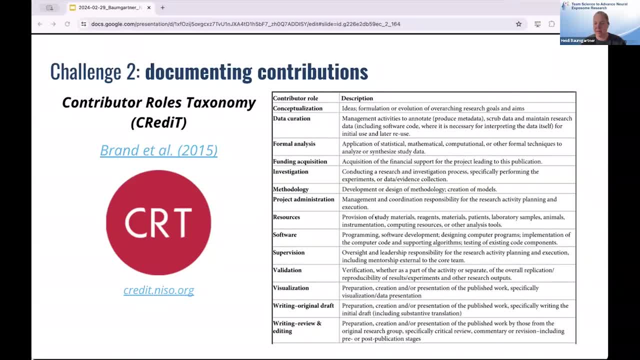 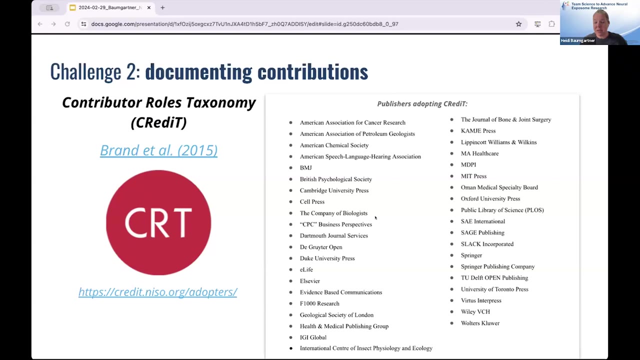 description of what those categories mean, and so the idea is that if everybody is working from the same taxonomy, then it's easier to interpret what an individual's contribution to a project means in this sort of shared language. When we decided to adopt credit with our group as our default tracking system just a few years ago, 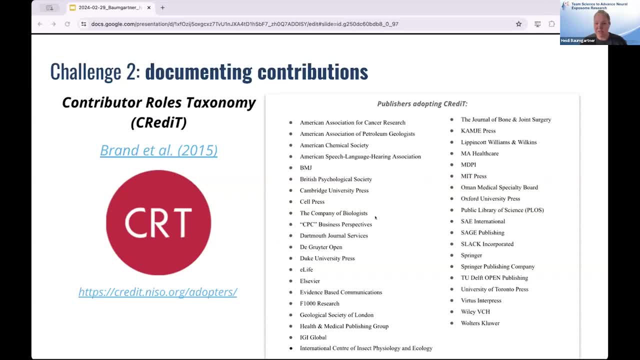 it was a relatively unfamiliar tool to most of our contributors, but it's quickly become the standard tool that we're seeing that many journals are requiring at the time of submission. So I've just put up on the screen here a list of publishers who have adopted. 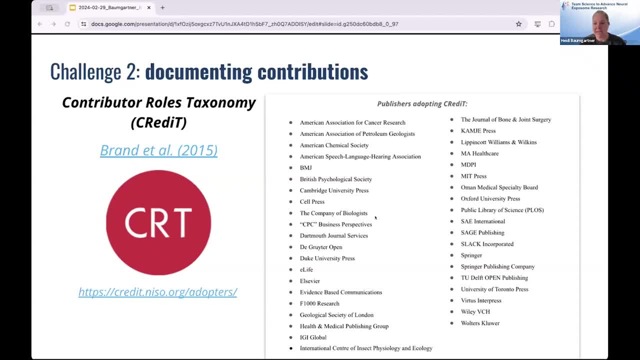 this tool, And actually this screenshot is from close to a year ago, so it's probably a longer list of journals here, but you can see some very familiar names. So if you yourself haven't already been asked to provide credit info with a submission, you likely soon will be. 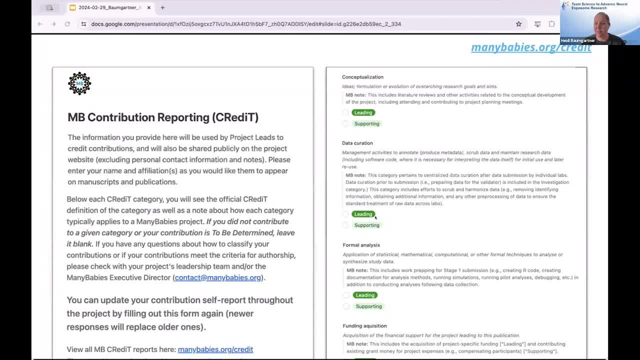 So, as you can imagine, the larger number of contributors you have working on a project, the harder it is to keep track of these contributions. So what our group is doing is we're creating an online form where we ask all contributors to any of our projects. 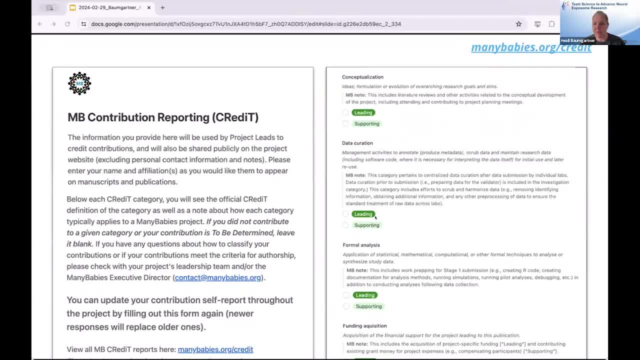 to fill out the form where they provide some information, including their affiliations, their ORCID, and they report their level of contribution to each of the 14 credit categories. So what we've done is we've also gone ahead, in addition to the credit description, 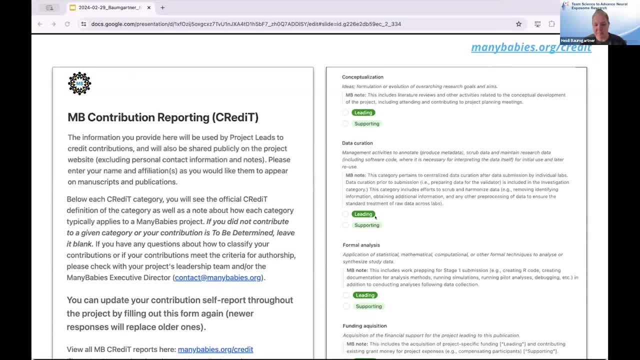 we've added a little blurb that is listed here as the MB note- MB for many babies- where we've gone ahead and added how the that category typically applies to one of our projects, because sometimes it's not always incredibly straightforward because the taxonomy was written to apply to lots of 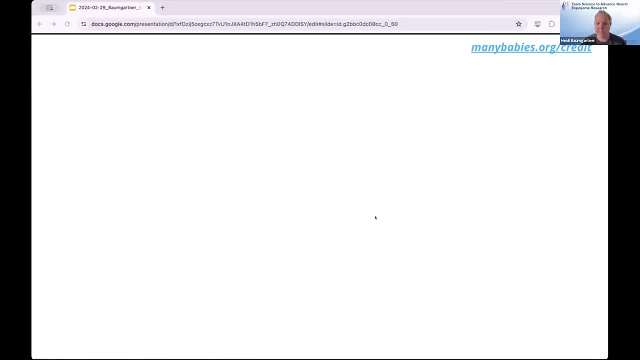 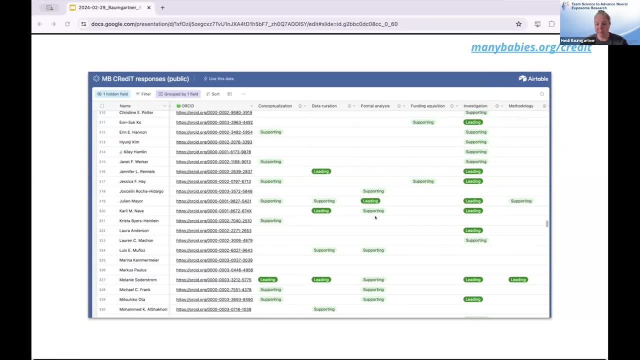 different domains. so once people have filled out that form, their tape, their entries populate a table which is publicly accessible on our website. so all of these reports are totally transparent. anybody who's participating in the project can view their own contribution as well as everybody else else's reports from the project. and again, this is just part of our, our commitment to being 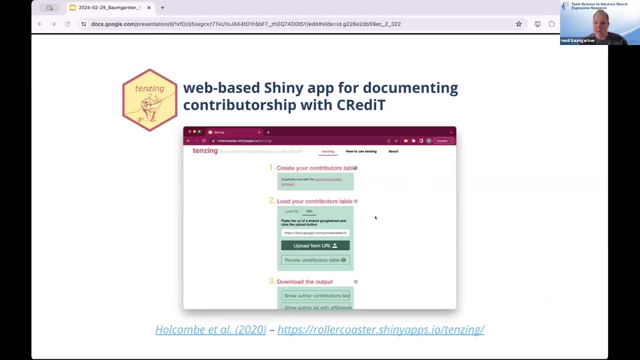 as open and transparent as possible. once you've got sort of a spreadsheet with all of this info, there's a really great handy web tool that's called Tenzing that you can use to easily compile this information into a post publication friendly format. so here's what their provided template. they provide a google sheet. 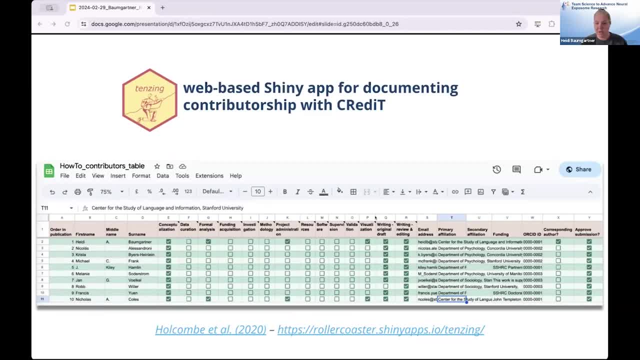 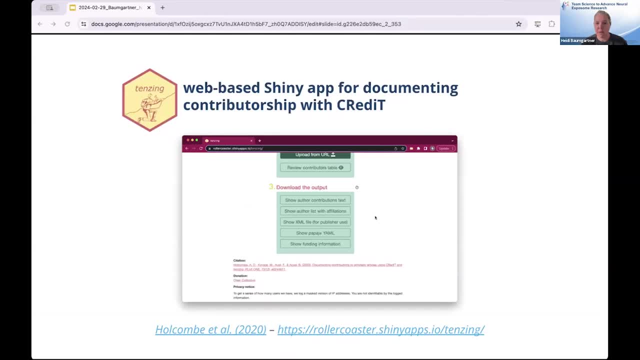 template, or i believe they have a csv file that you can download so you can just transfer your information in into this type of spreadsheet, upload it to their web app and then you can download the output that you want in a number of nice formats so you can get author contributions. 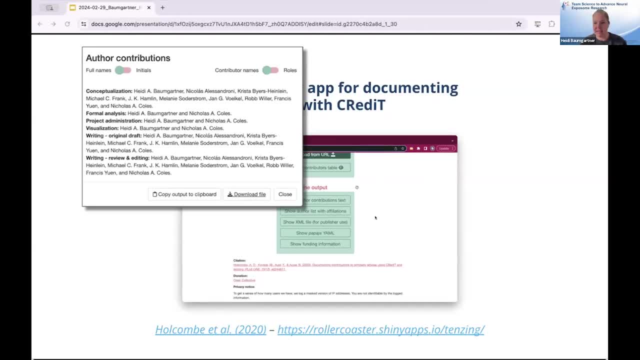 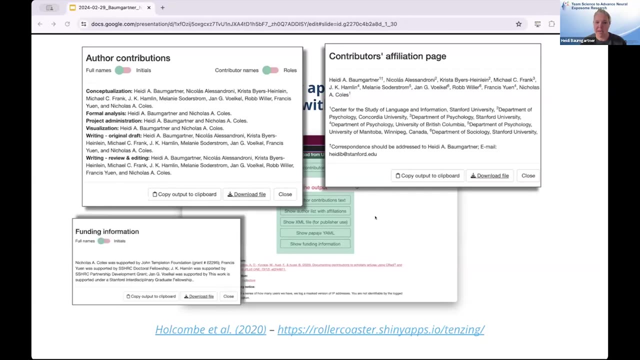 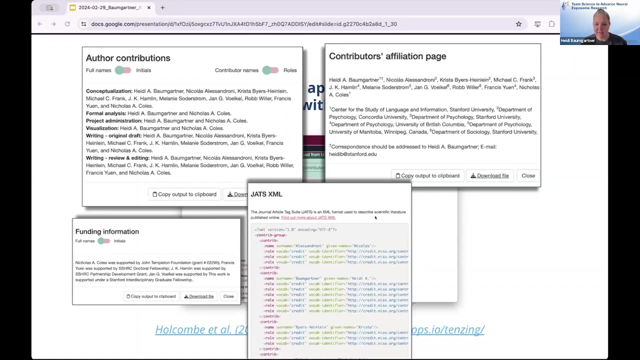 by credit category. so you might have seen tables like this in publications. you can get a table, a list of the contributors, affiliations. it does all of the formatting with the superscripts and numbering for you, so you don't have to worry about that. you can export all of the funding information that people report. you can export an xml file. 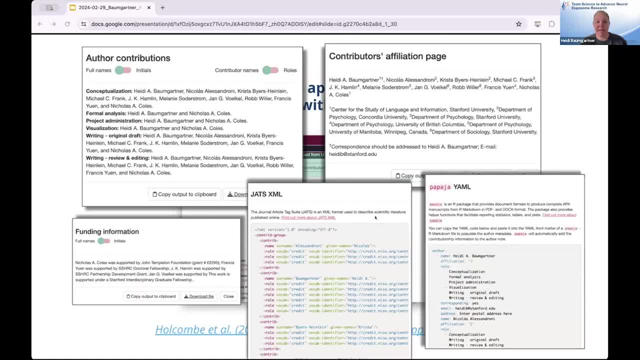 that can be provided directly to publishers, and a yaml file that generates code like if you're writing your manuscript using latex or our markdown. so, as you can imagine, like you know, you know how hard it is to put this information into a cover page for a publication with not 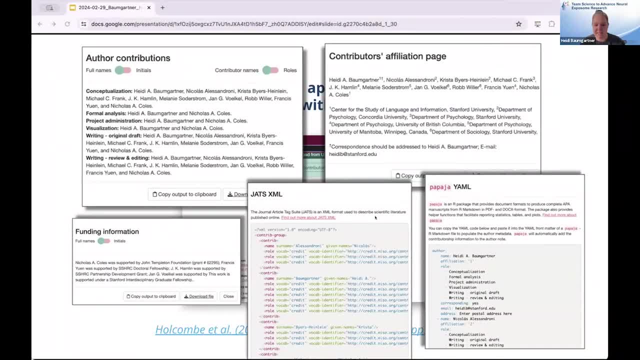 that many collaborators. once you start scaling up this tool, this tool can save you a lot of time and then if something changes, it's easy to just update that spreadsheet and re-export all of these tables and then just very quickly we have sort of this idea, that's. 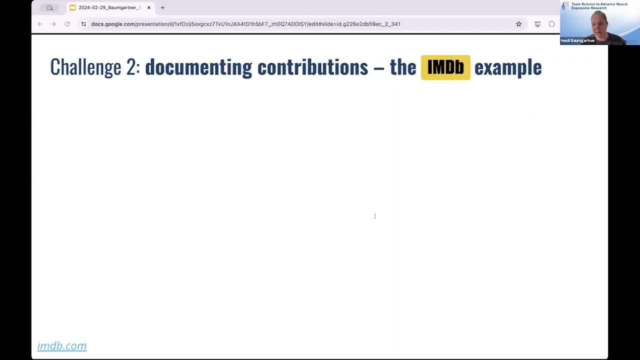 floated around. our group of you know using the credit reports to create something that's more akin to something like the internet movie database. so if you go to imdbcom, you can see all of the people who participated in a given project- actors, crew members- organized by their role. you can click. 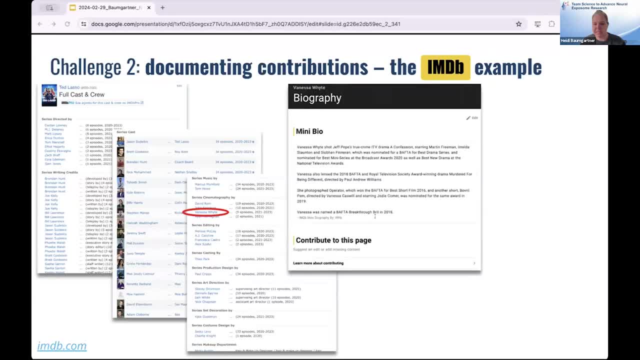 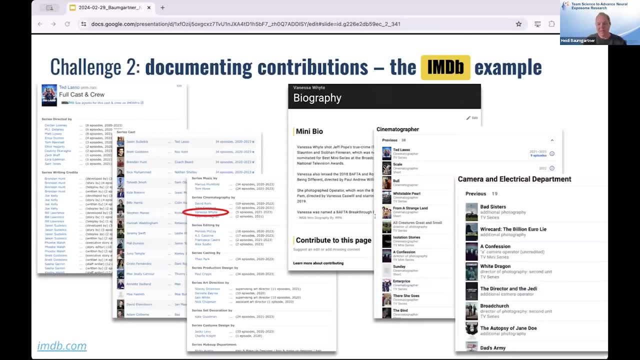 on someone's name to see what else that person has done: a bio, other projects they worked on in that same role or in other roles. so it it's. it's nice to imagine a not too distant future where we can use credit information in this way to add to our databases where people's contributions to projects 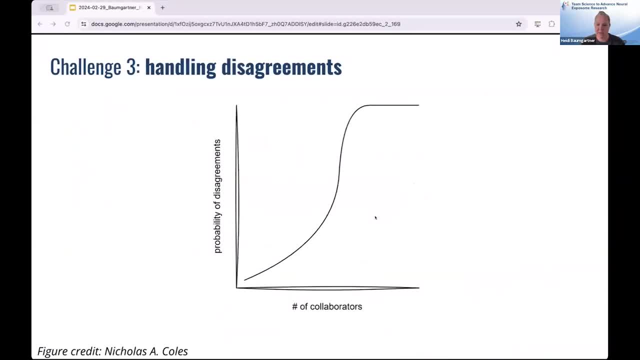 are very transparent and um searchable in this way. okay, and then just the last question that i want to bring up is how to handle disagreements. so, again, this has been touched on earlier, but um a lot of times when we think about how to handle disagreements, it seems like a pretty obvious. 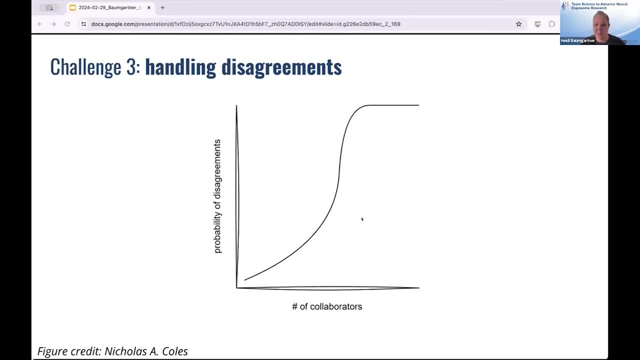 statement is as as teams get larger, the number of collaborators increases and the probability of disagreements occurring gets higher as well. so collaborators might disagree with. you know the the logic of a proposition phrasing in the manuscript, all of this stuff. so there, there are a number of ways we've identified to think about handling these things. so 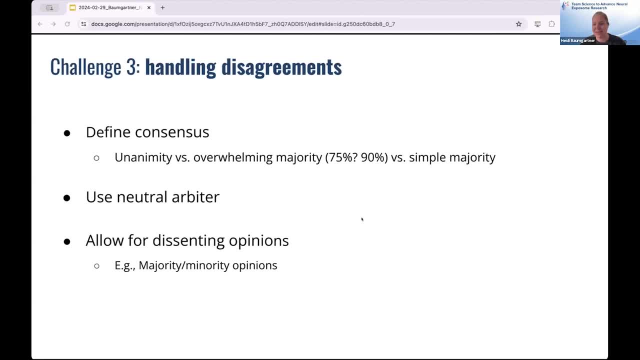 one of the ways we've identified to think about handling these things is by using a consensus based model, where you can define how your group is going to make decisions. so you can say: you're going to use a consensus-based model, but does that mean decisions have to be unanimous, overwhelming? 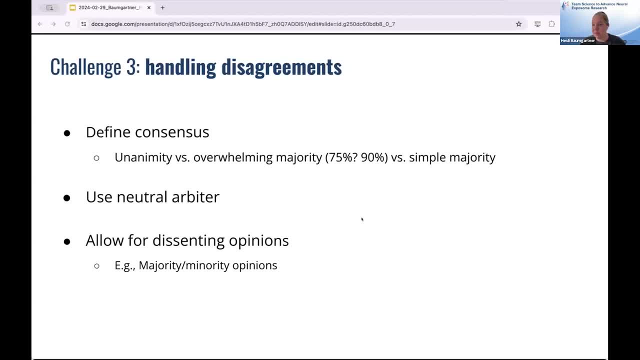 majority, simple majority. it's important to make that decision and lay it out in your collaboration agreement. another option is to try and resolve disputes using a neutral arbiter, where both parties can sort of make their argument and agree to rule by a stand, by the arbiter's ruling. so a lot of 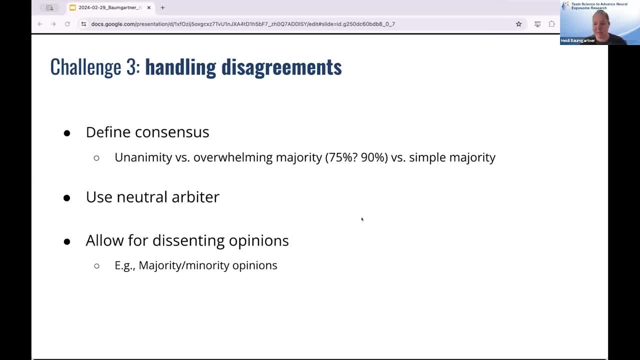 people just want to feel like their argument has been heard and considered um, rather than ignored or dismissed, and this can help head off disagreements as well. and then another idea is to allow for like dissenting opinions again, to allow for people to participate in these projects without, without feeling like they have to rubber stamp everything that the main group decides on. 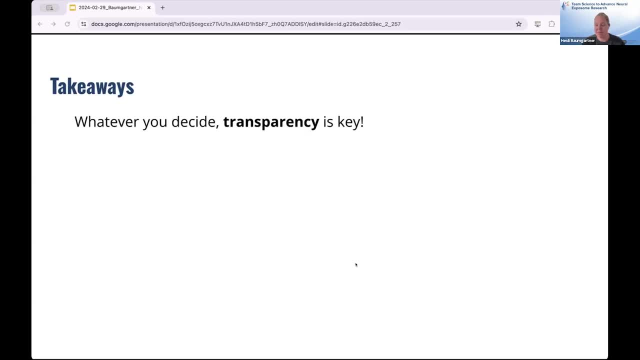 so, just very quickly, the last takeaways: whatever you decide, transparency is really key. make decisions on how you're going to define authorship, define contributions and handle disagreements as early as possible, and document all of these decisions in a collaboration agreement that's shared openly. and, again, these don't have to be specific to large team science. 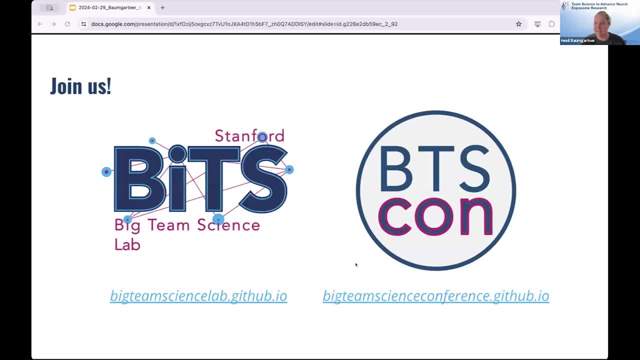 these are great tools to use in your own labs as well. um, and lastly, i'll just say, if you're interested in learning more about the big team science lab- or we put on an annual conference that we call the big team science conference- please visit those links and i'd be happy to talk with anyone who's interested. 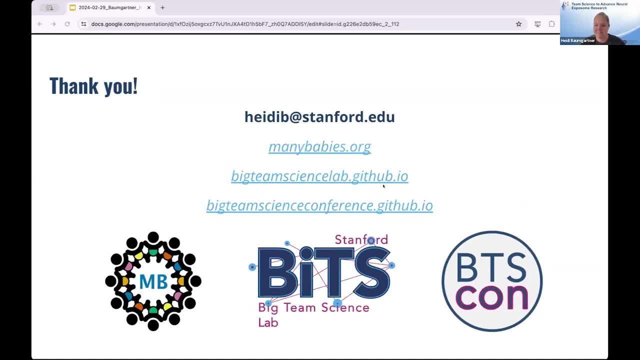 thanks so much for having me. thank you very much. we have time for one quick question. i don't know if there's. oh, uh, pam, you have your hand up. yeah, thanks, so great presentation, heidi. really cool stuff you guys are doing. um, i just wondered: have you? how do you decide authorship? 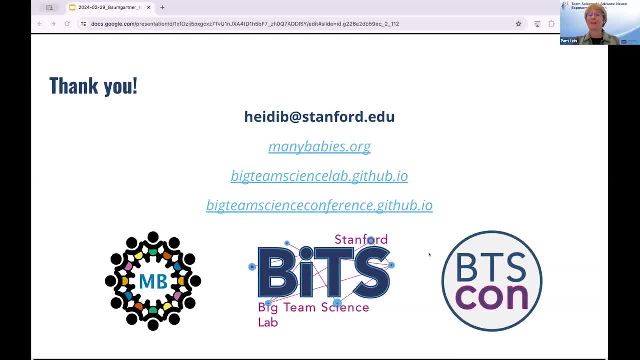 is there a unit of authorship that is like a general order if you have a large paper with a gizli of people on it and is it possible to use the credit um whatever excel spreadsheet or whatever it is you're putting together, to try and figure out uh order of authorship on a paper? 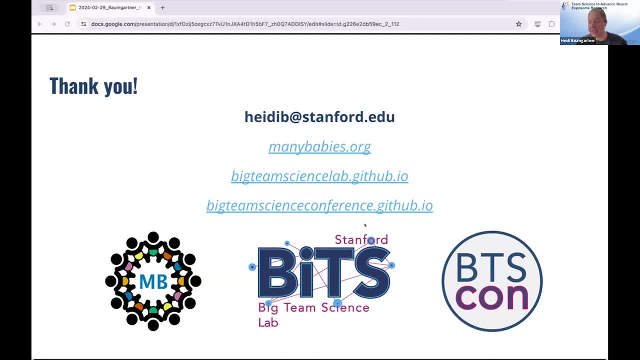 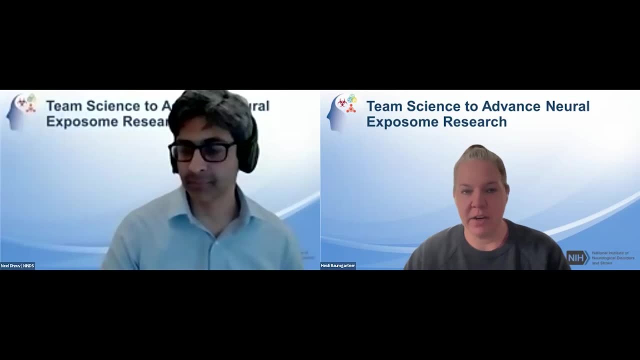 yeah, that's a great question. so generally, the way our projects work is: each project has a leadership, a core leadership team that consists of three to six people, i would say, and so generally, um existing publications, those people serve as, like, the first and final author positions, depending. 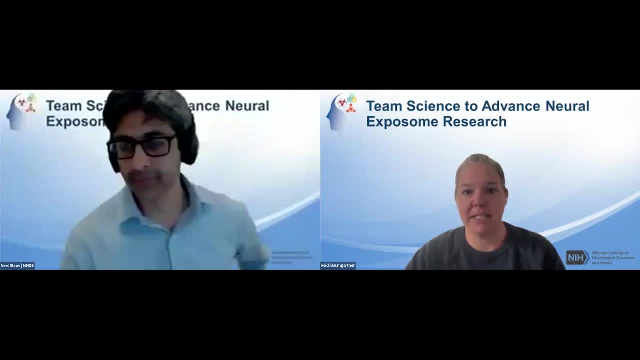 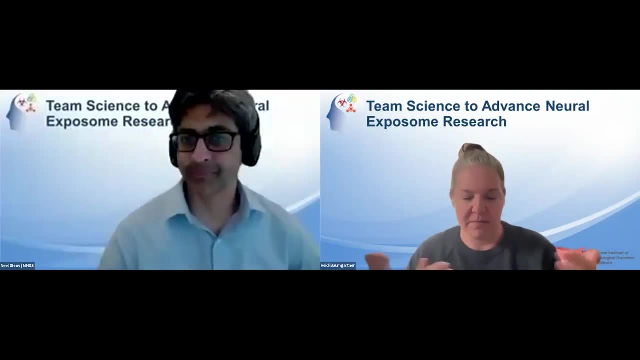 you know, sort of those groups decide on their own. the best way to do that we have a couple papers with shared first authors, because there are leads who have really served in that role, and then we might have another group of authors that appear right after the first authors of. 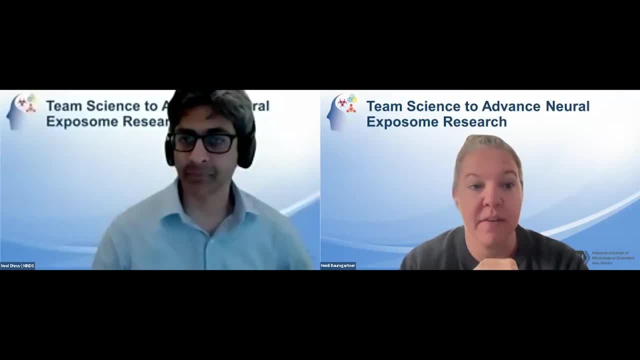 people who led working groups or made significant contributions in another way, and then we'll have the bulk of the contributors that appear in alphabetical or reverse alphabetical or some other sort of random method that's predetermined, but you can certainly think about using the credit reports to do that. so far it's worked for us to just have those groups be defined. 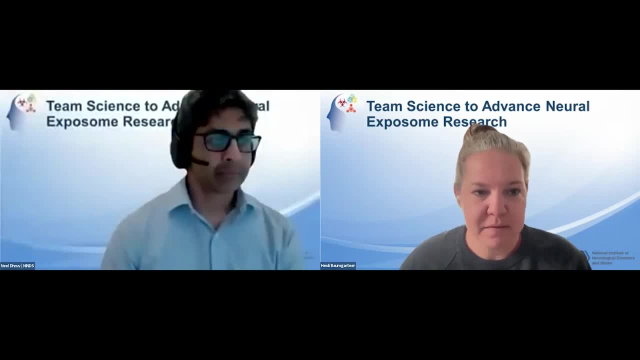 by the leadership group and by the teams themselves, um, but regardless of the authorship ordering um, we'd have that, that credit report that shows on a granular, granular level which categories each person contributed to. great thank you. yeah, let me just real quick state um. great thanks, heidi, and i was just curious about um and i put 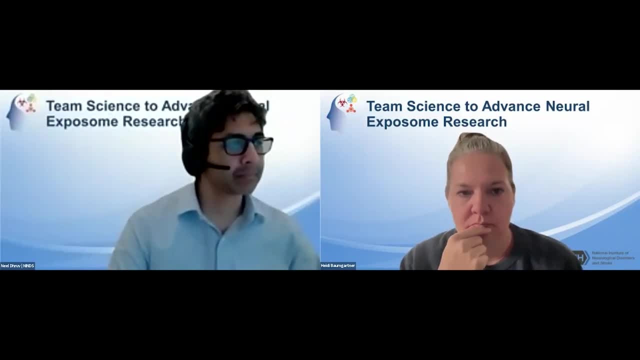 this in the chat about: would the contributors know where they're going to be on a paper before they agreed to join the team? and i know that's kind of a weird question, but it could. that could come about there, yeah, so again, we um, we try to have that collaboration agreement drafted as early. 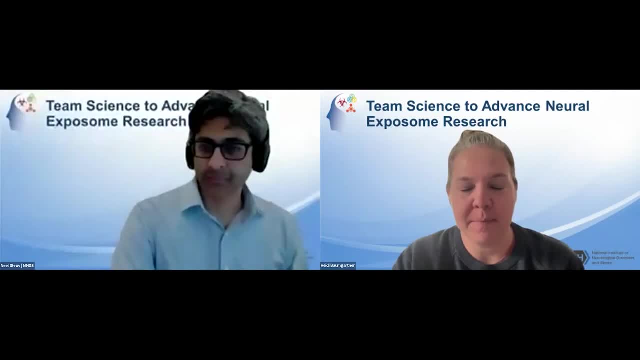 in the process as possible. so, um, yeah, the transparency is key there. we- we don't necessarily have it ironed out- the exact list and the- the people, who people join our projects on the project- have the authority to be used to determine who's involved and who isn't. but 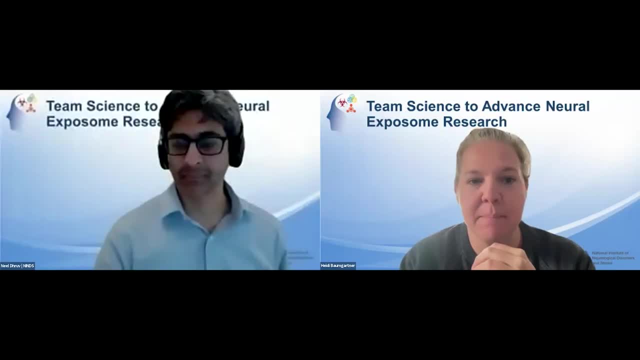 i would add that, uh, if the author is not involved in the process, then the author is not involved in the process, then the authorship order. so it's very general practice, um, that you're going to have to sort of figure out your ways out of the process of. okay, well, i was going to 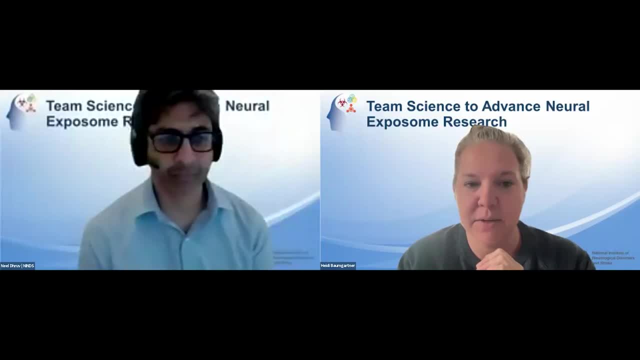 do this and i'm going to do that all the time, and that's great. and then, for the last thing i just wanted to point out is that, uh, we, we're going to, we're working on a case study for the local library department, so that's the one i'm currently working on and that's our future item. we're going. 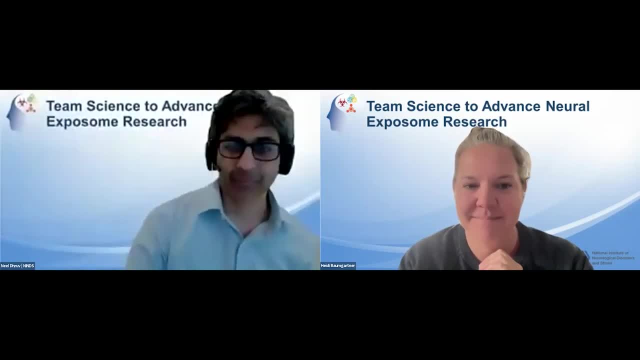 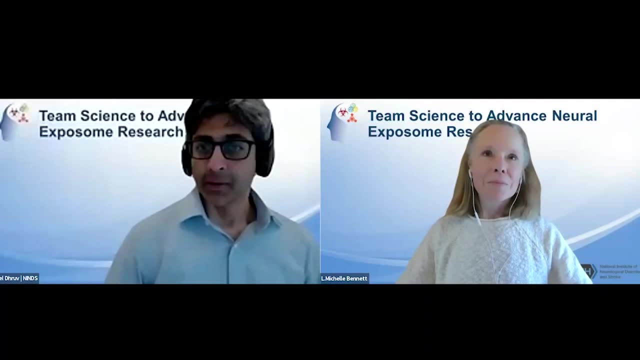 to be doing that, so i'm going to be working on a case study on the site as we go through that. um, i'd like to it when we discuss it. fantastic, thank you very much. uh, dr baumgartner, welcome back. the last presentation is from dr l michelle bennett. dr bennett is currently principal. 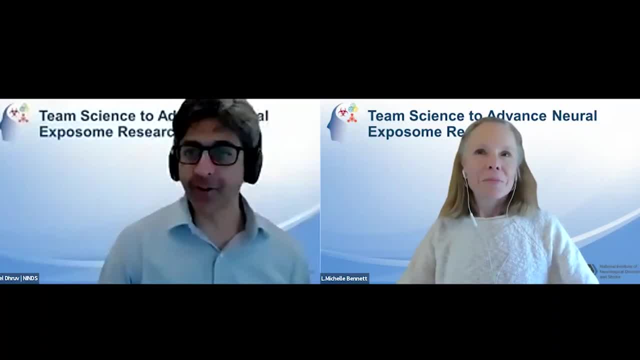 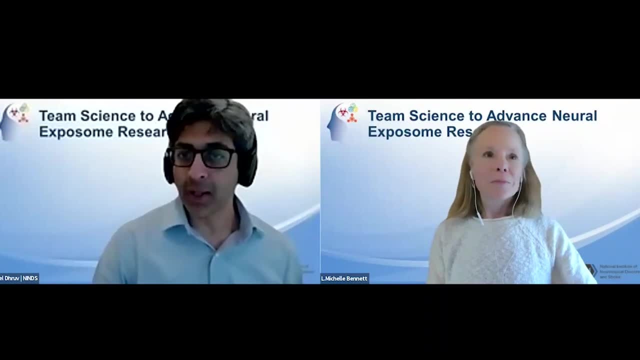 and owner of lm bennett consulting, having departed her position as director of the center for research strategy at the national cancer institute in 2021. while at nih, dr bennett's passions pulled her to focus on effective research, collaboration, science, administration and executive coaching. this combination provided her with opportunities to grow into leadership. 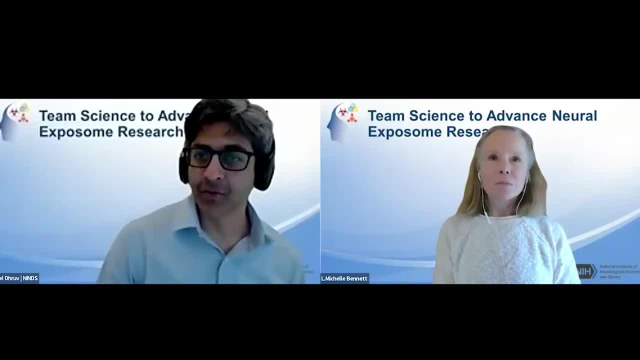 roles that focused on strategic scientific planning, creating conditions for successful interdisciplinary collaboration, workforce diversity and health disparities, as well as organizational change management and development in research institutions. she has extensive practical experience in promoting collaboration and team-based approaches by bringing together research scientists with diverse backgrounds and expertise across many dimensions of difference. 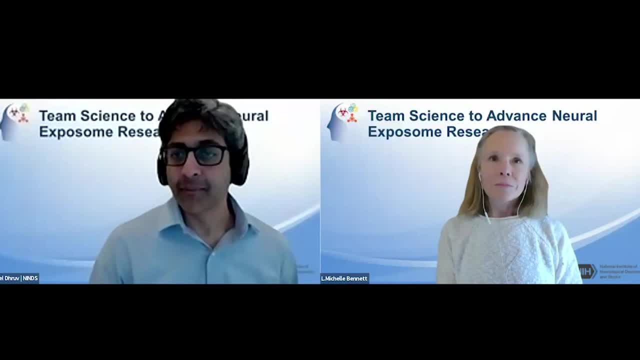 she co-authored collaboration and team science, a field guide that serves as a primer for investigators who are building or participating on research teams. today, she'll be talking about how research can be developed, and how research can be developed, and how research can be developed and collaboration thrives on productive conflict. 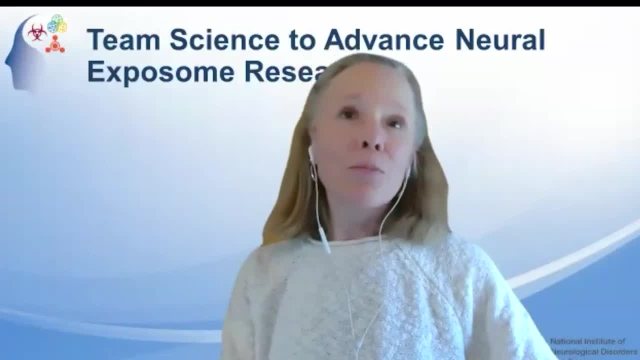 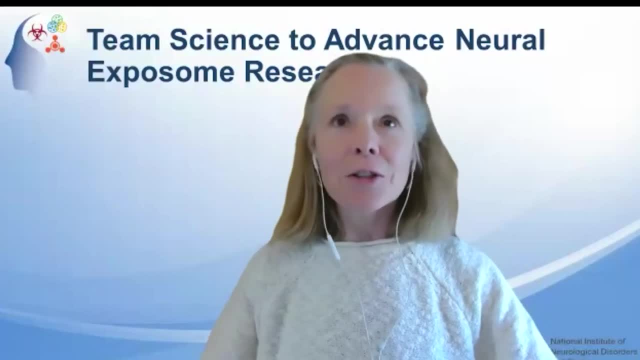 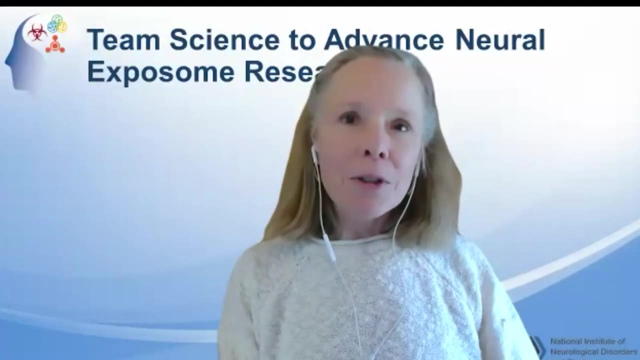 thank you very much, neil. um and i- and i am sorry, i guess i want to say that i actually changed my title after i had a chance to see the speakers and to learn a little bit more about, um, what you were hoping to hear from me. so i'm gonna get my slides up and while i'm doing that, 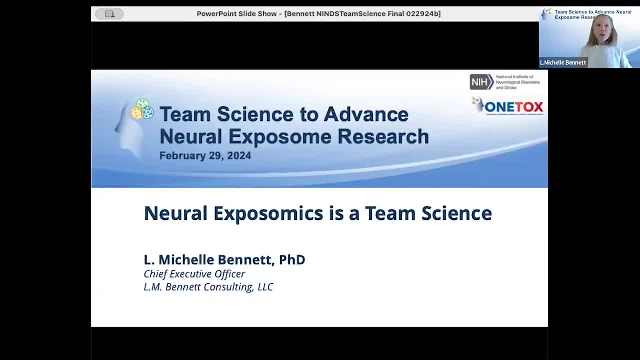 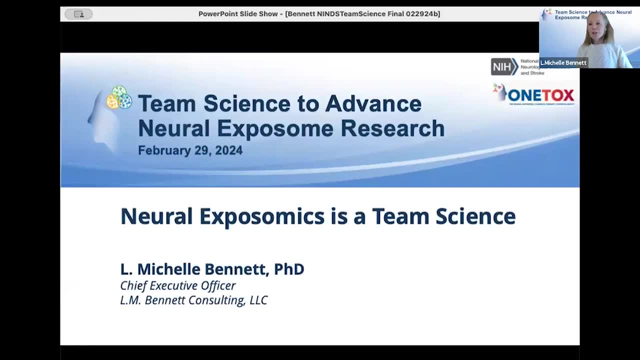 i just want to thank you all so much for inviting me to participate. this has been a really amazing um series so far. i've really enjoyed listening to all of the talks and hearing the exchange of ideas. um, so i think i'm gonna start this off by saying that, uh, and maybe even 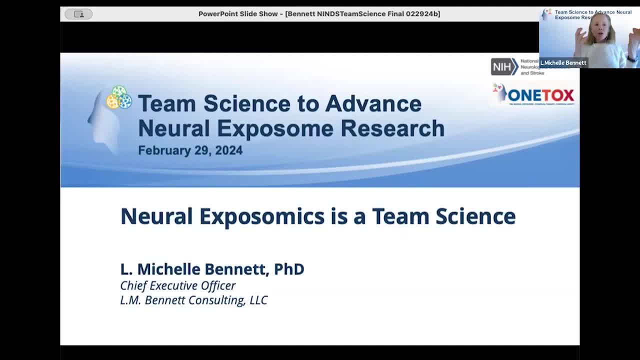 reiterating some of the things that folks have said, in that the three examples that we heard of these, of the teams that are being led um, are just phenomenal. I've enjoyed each of the presentations so much and I'm so impressed by what each of 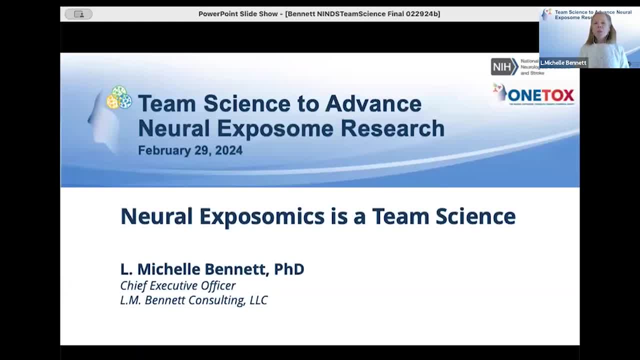 you have done. It's hard to even put into words, And so I think the main message that I want to convey in saying that is that these aren't the kinds of teams that you need to worry about. It's really the teams that are struggling to figure out how are we going to work together. 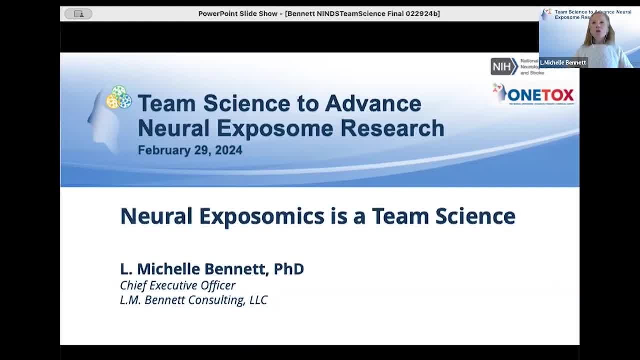 as a team, And people who don't have these natural abilities or recognize the necessity of combining both the science with being attentive to the people and their needs, and learning how to work with each other, as they're starting to work with each other. So I think my talk is going to focus a little bit on that, because there are a lot of people. 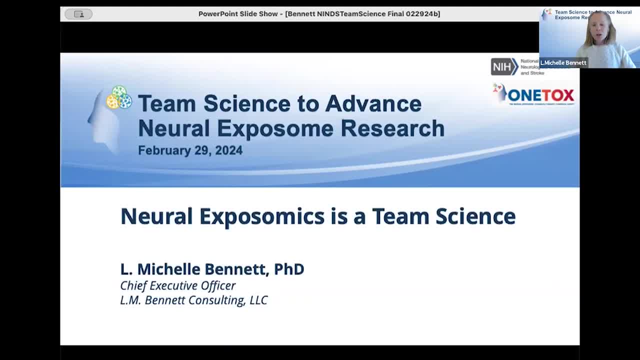 out there who start teams and are not successful in really getting To a successful conclusion with them or even able to sustain them. So I titled my talk Neural Exposomics as a Team Science, or retitled it Neil. Sorry about that, Because as I was preparing for this talk, it became really clear to me, I think, that 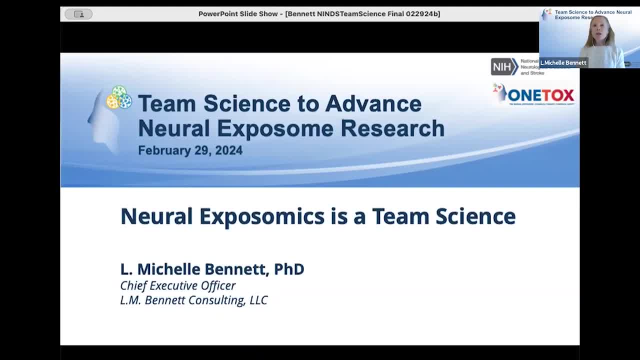 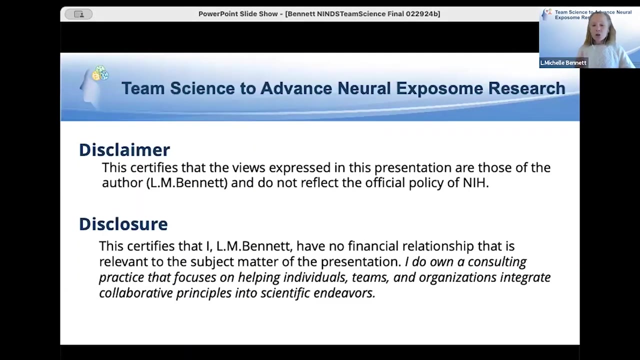 NINDS was really interested in trying to understand. you know how are we going to put team science into practice through the neural exposomics, And so I wanted to address that a little bit more directly. So disclaimer views are my own and I have no financial relationship to anything. I'm 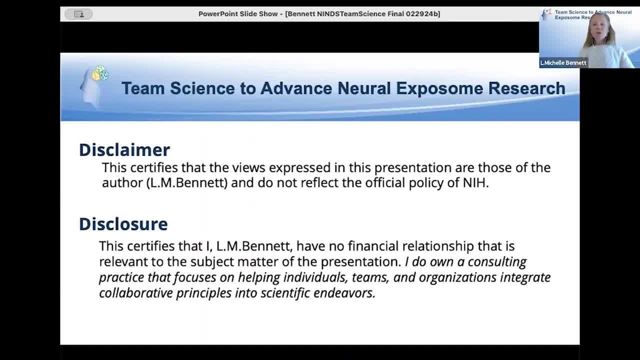 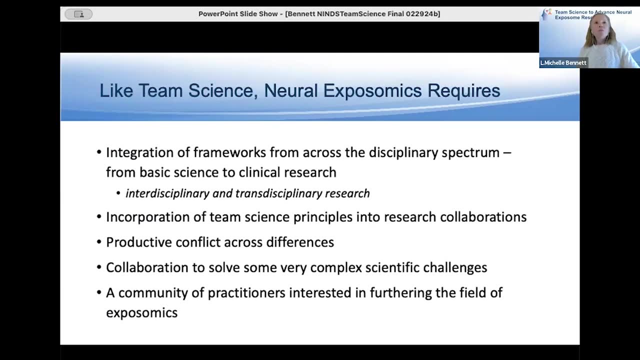 going to present per se, but I do want to own up that I'm starting my own consulting practice that does focus on helping individuals, teams and organizations integrate collaborative principles into scientific endeavors. So, like team science, neural exposomics requires a number of things, which has led me to title. 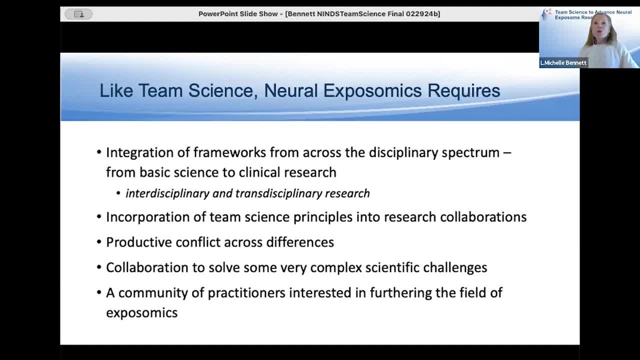 my talk the way I did. Neural exposomics requires the integration of frameworks from across the disciplinary spectrum, from basic science to clinical research, And I think we've seen a number of examples of that through the different talks that we've heard. I have focused mostly on interdisciplinary and transdisciplinary. 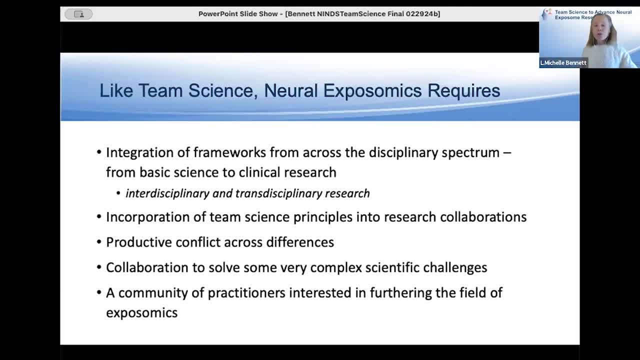 I'm going to talk about interdisciplinary research and how those teams function and how they are successful. And for those of you not familiar with the vocabulary of interdisciplinary and transdisciplinary research, I'll explain that to you in a moment. Neural exposomics really requires the incorporation of team science principles into research. 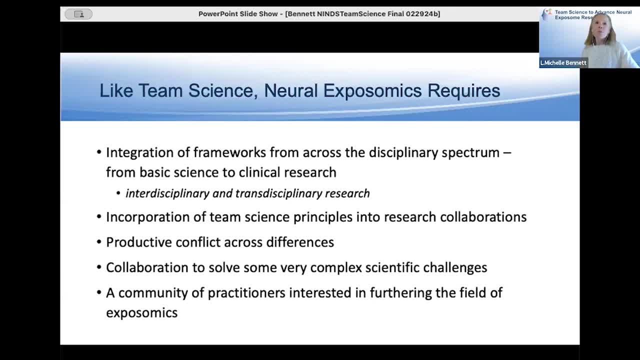 collaborations, And I think we've heard that mentioned along the way- It is essential that there be productive conflict across differences. I think one thing that I hear a lot of people talk about and mention is the issue of conflict. You know what do we do when there's conflict. 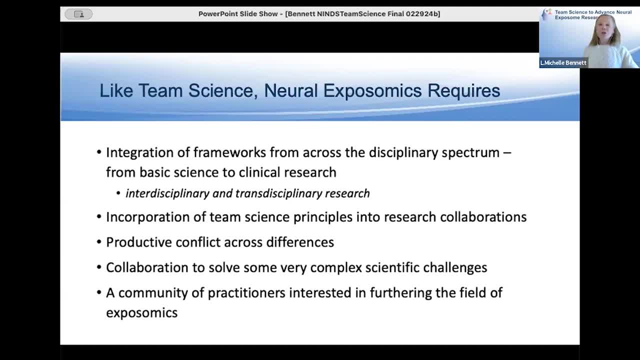 I will say to you that you want conflict in your teams. You want to bring together people who are thinking differently, And the reason that you want to do that is precisely what Jay was talking about. It's when you have people with different perspectives that you're able to make those two connections. 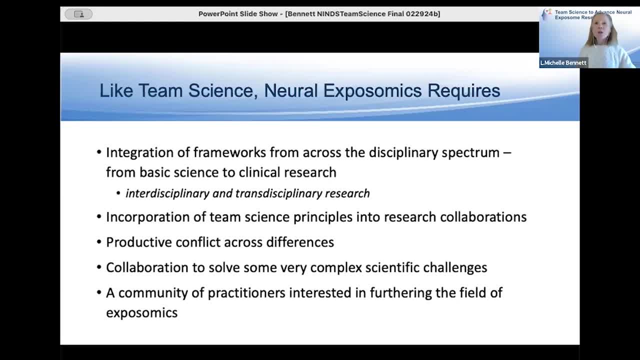 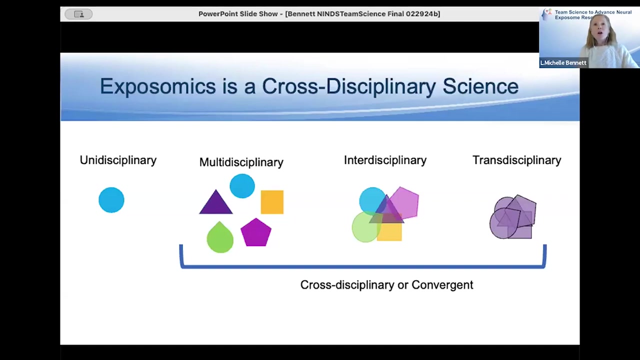 We know that the community of practitioners interested in furthering the field of exposomics- And I heard- I think one of the things I've heard too- is: how do you recruit more people in neurobiology, the neurofields, together and to participate? So when I talk about exposomics being a cross-disciplinary science, this is what I mean. 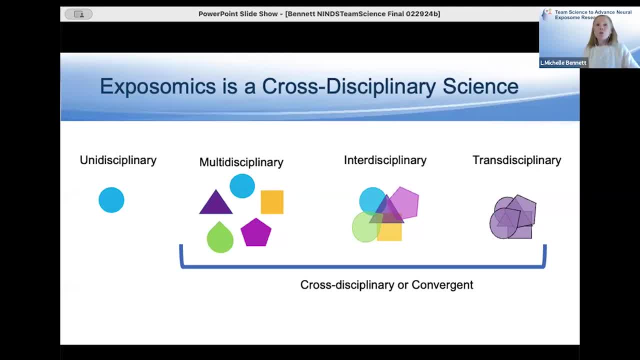 is that there really is a disciplinary continuum, from unidisciplinary to multidisciplinary, to interdisciplinary to transdisciplinary. You could call the multi to trans as sort of the cross-disciplinary arena or convergent. So really what this means is that as you are increasing the 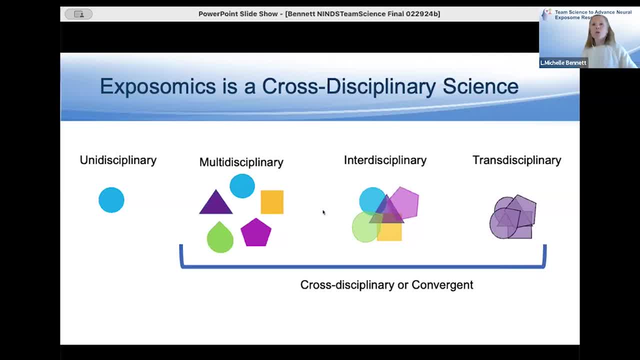 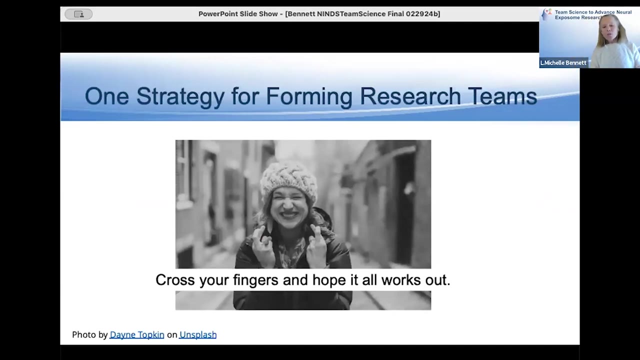 levels of interaction and integration across this continuum. you're really moving from a number of different separate frameworks that sort of exist on their own to beginning to be merged a little bit to a whole new framework that is unique and distinct to that particular collaboration. So I spend a lot of time with teams, with organizations, with individuals who are 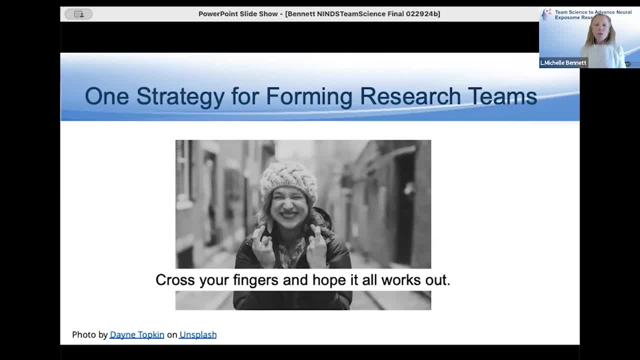 interested in forming teams or have formed teams and have had not so great experiences, And I would say that this is one strategy that a lot of people take: when they put together a team, They cross their fingers and they hope it's all going to work out. I don't think like a lot of. 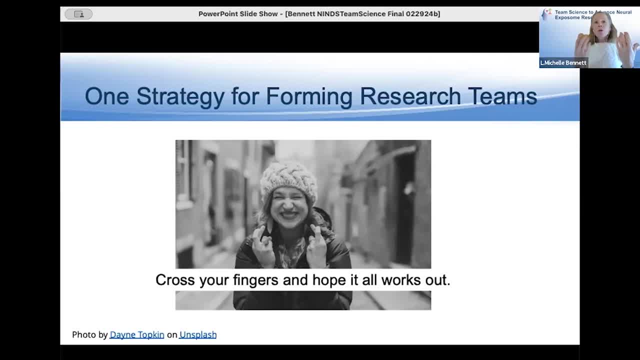 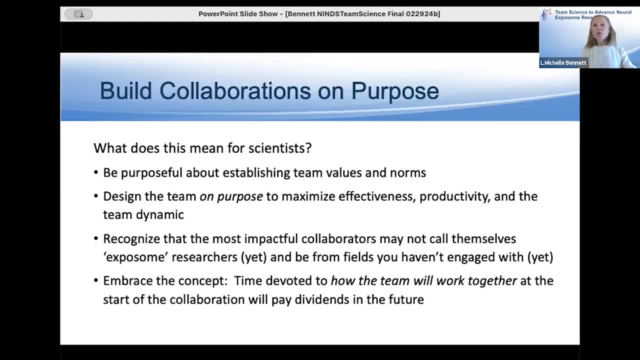 the investigators that you just heard present, that everybody realizes that you can design your team on purpose. You can be very, very purposeful for how you design your team and it can make a huge difference. So I am a huge proponent of building your collaborations on. 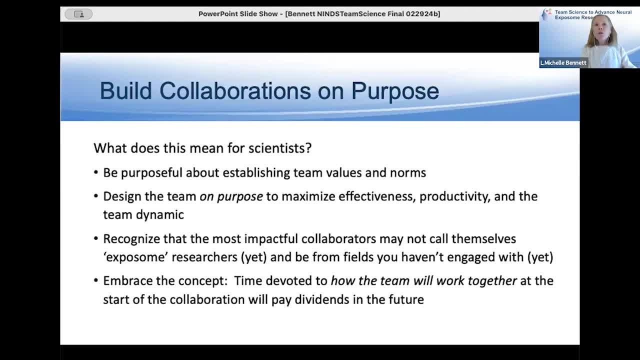 purpose. So what does this mean for scientists? That means that they really need to be purposeful about establishing their team values and their team norms. We've heard a lot about norming and the norming phase, which is putting those processes into place. 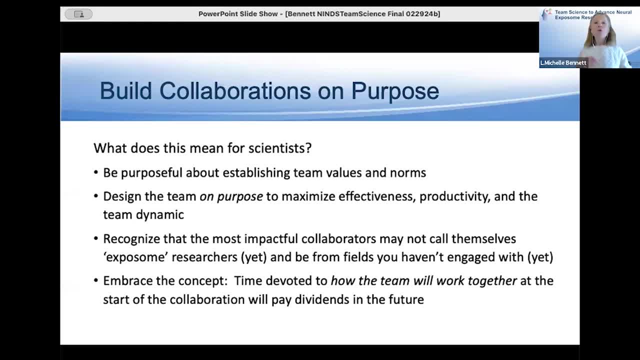 putting those processes into place and then putting those processes into place, Putting the structures into place, that is really going to help inform the team and around which the team can agree to implement in order to achieve their goals. What we really haven't heard anybody talk about is what are the values? And when I talk about values, I mean the values. 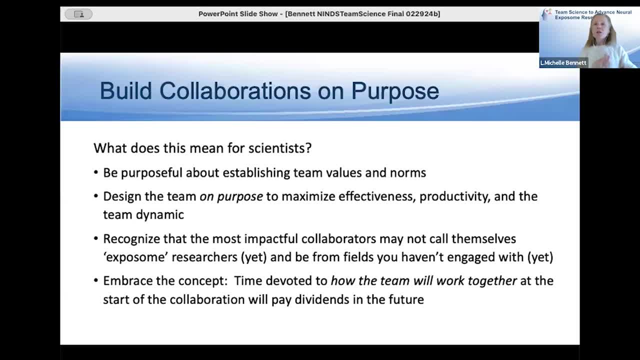 and beliefs of that team. So, as a collective, what are your values, What are your beliefs? And the reason this is so important is that your behavior or what you do as norms, how you get to your norms, is all dependent on your mindset in being. 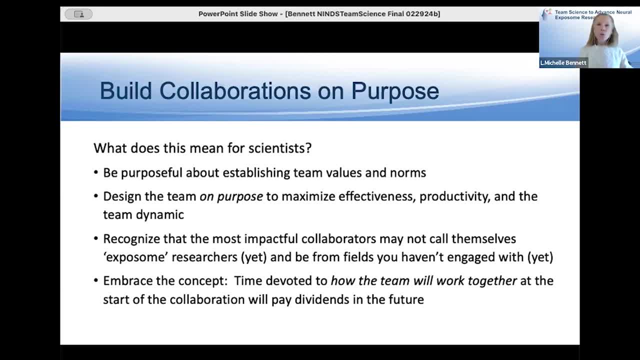 collaborative in nature. If collaboration is really important to you, then those values like transparency that Heidi was talking about, curiosity, like Jay was talking about, are all things that cascade from there, that enable the team to be really successful. So those values are really the culture of the team. What kind of team culture is it? What kind of team culture is it? 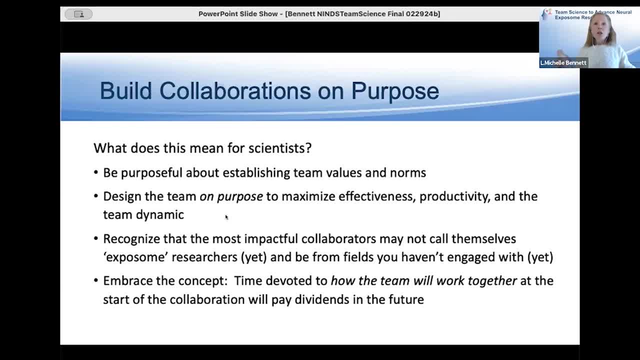 What kind of team culture do you want? So designing the team on purpose can maximize your effectiveness, your productivity as well as the team dynamic. The other thing that I wanted to say is: I think for a lot of scientists, they don't always necessarily understand that they're going. 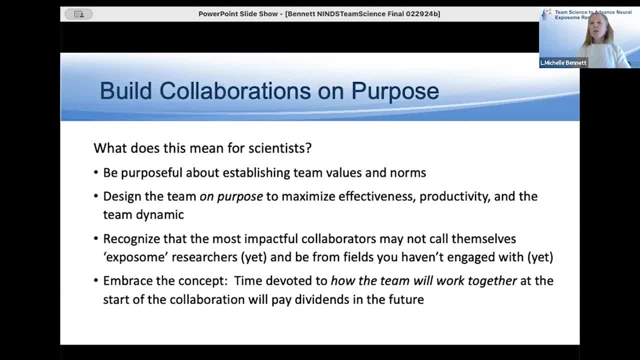 to probably end up meeting new people who might not even consider themselves exposome researchers yet, And they probably will be interacting with people from other countries, And so I think they're going to be interacting with people from fields that they've never interacted with before. 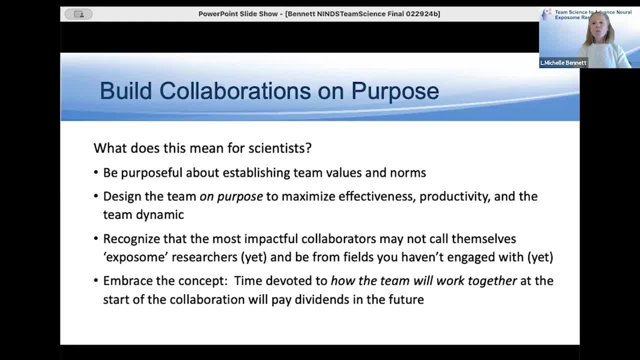 And this is part of the excitement I think that you've heard in the voices of those who have come before me about the opportunities around team science and the value, And then I really like- a lot of no surprise to people who might know me- that if the team spends time in addressing how 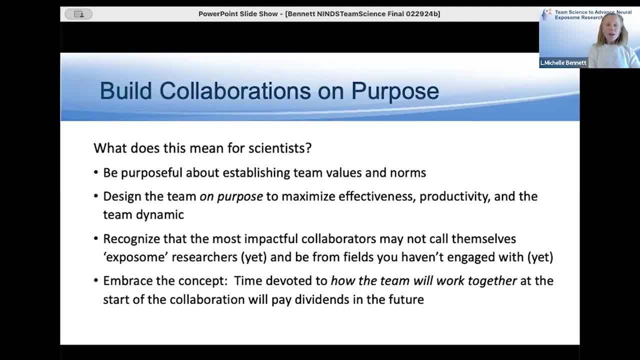 they're going to be working together at the start of the collaboration, integrating that into how they move forward. it will pay huge dividends in the future And I think each of these groups that we've heard talk about had some sort of collaboration agreement. 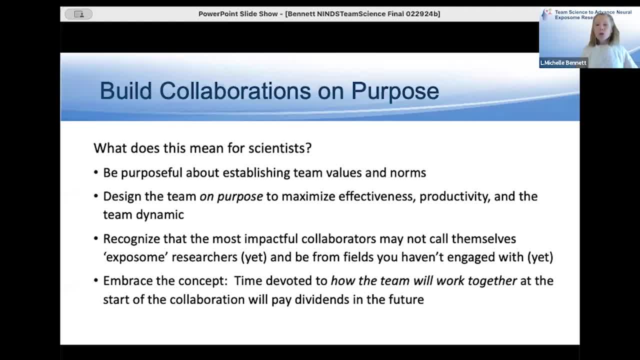 which does take time, as we've heard, to put into place. It takes everybody's time, But I can. I'll give you a bit of an example in a second of where that really has. we've got some really nice evidence about how beneficial it is. 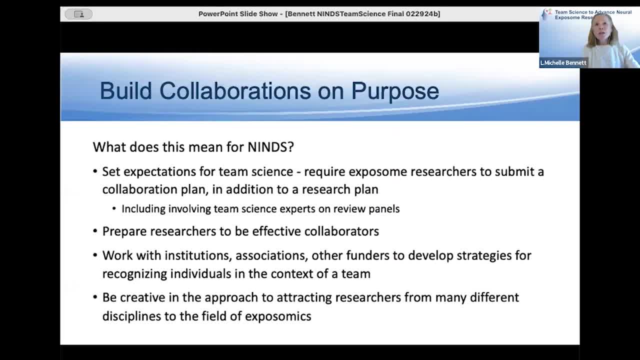 So what does this mean for NINDS? And I tried to think about, like, from a funder's perspective, what do you need to think about as you are implementing programs that are incorporating team science or that, or science that is team science in and of itself. So I think, setting 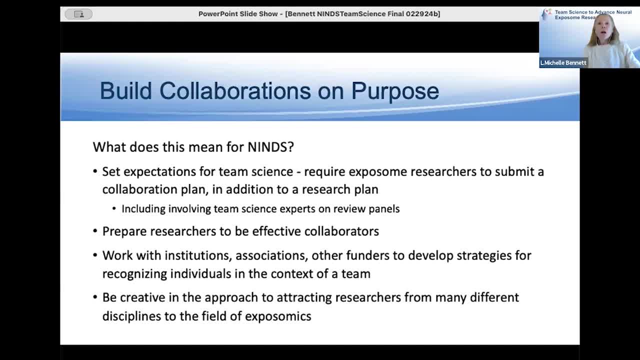 expectations for team science is really important. You're already starting to do this- is requiring researchers to submit a collaboration plan in addition to their research plan. I think the only thing I would add on to that is making sure that there are team science experts. 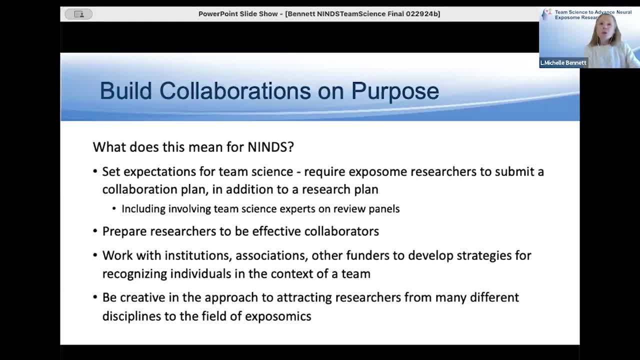 on review panels. This is something NSF does and it's really interesting. I've been a team science expert on a number of panels. now I know very little or anything about the science, but I know about collaboration And so I can contribute very substantively in predicting how effective. 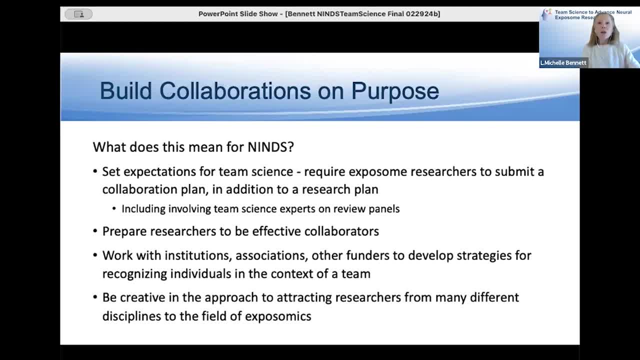 the team is going to be in actually getting the work done that they say they want to get done. I would say: prepare researchers to be effective collaborators. I have a great opportunity on many occasions to run workshops for people who are early in their career And I hear over and over. 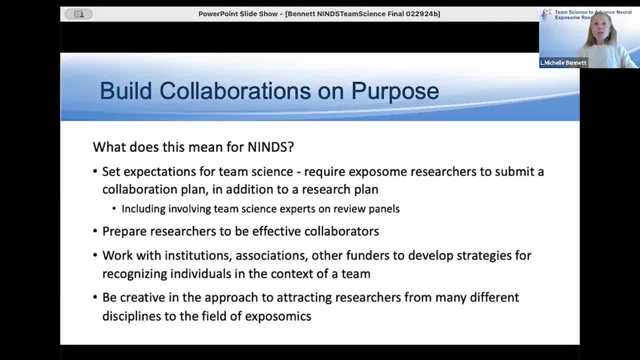 and over again. you know, we don't learn this kind of stuff anywhere. We don't learn about how to collaborate, We don't learn how to be effective, And so being able to work with folks who have that need to learn how to collaborate, I think is really important, And so I think it's really 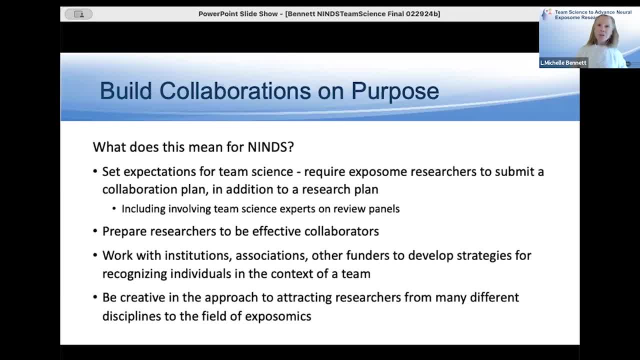 important to learn how to work better together so that when they actually do put teams together, they can be effective right off the bat. on attempt number one is really powerful. The other thing I would say is work with institutions, associations, other funders to develop strategies for recognizing individuals in the context of the team. 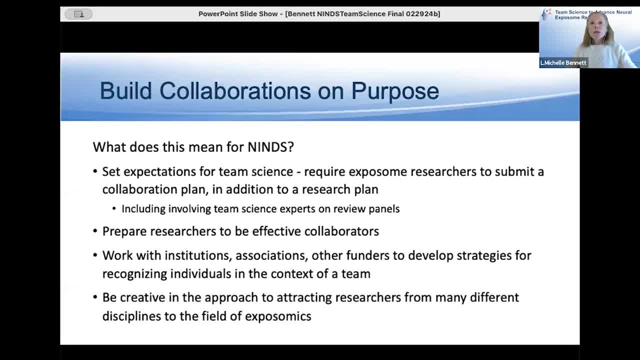 I think if I were to make a plea, this would be it. You know, I think I heard earlier this morning- maybe it was David and I apologize, David, if I got that wrong. It might have been Karen, But you know, on these multi-PI grants, you know you have three to six PIs. That's really. 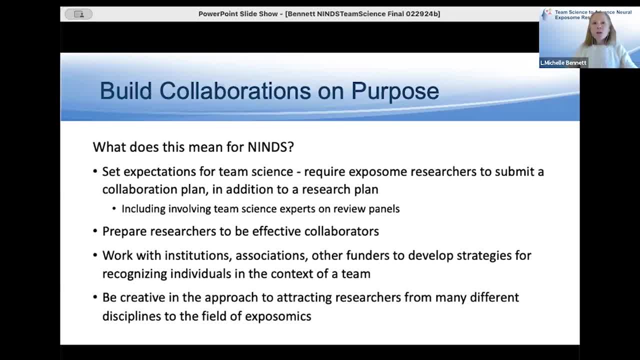 great. And of course we have the contact PI as well. I don't know how many investigators you've talked with on the outside, but many investigators view the quote-unquote contact PI as the person recognized by the NIH as like the main person which can really impact the team, And I think 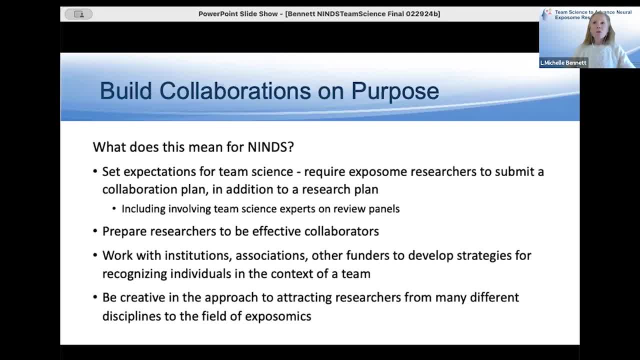 it's really important to think about how you can actually impact them in their recognition and review processes at their institutions. So if there's any way to be super clear about it's just an administrative function or working with people to help them understand what it really means when 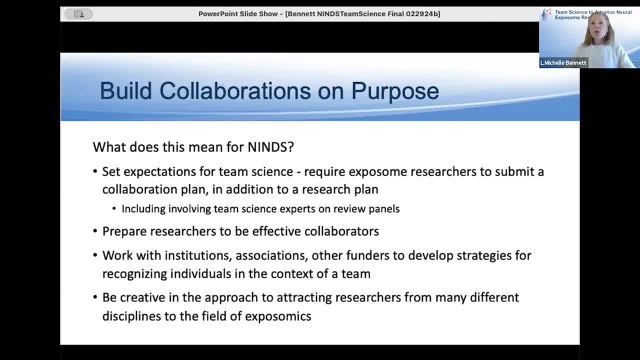 these scientists are going up for recognition and reward And be creative in the approach to attracting researchers from many different disciplines to the field of exposomics. This might be the of thing where one of the granting opportunities or FOA, might say: you know, we're looking for a. 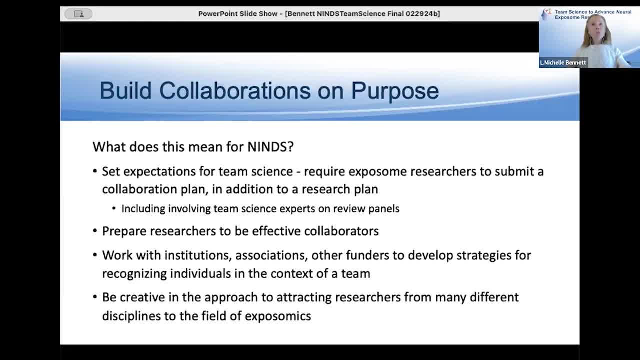 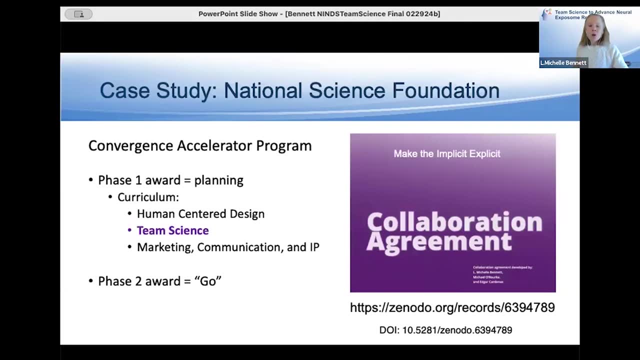 neuro researcher and we're looking for them to partner with somebody who's never been involved before or somebody from a completely different discipline. So I wanted to share just a really brief case study with you. So I've been a faculty member for the National Science Foundation's Convergence Accelerator. 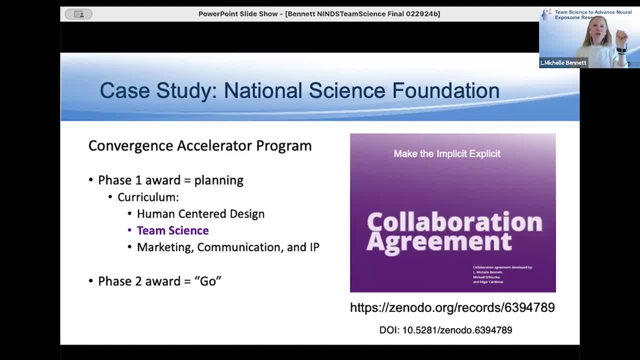 Program for the last. I'm really sorry I'm going to pause myself and cough. Sorry, All right, hopefully that worked. So I've been. just to repeat that I've been a faculty member for the Convergence Accelerator Program for the NSF. 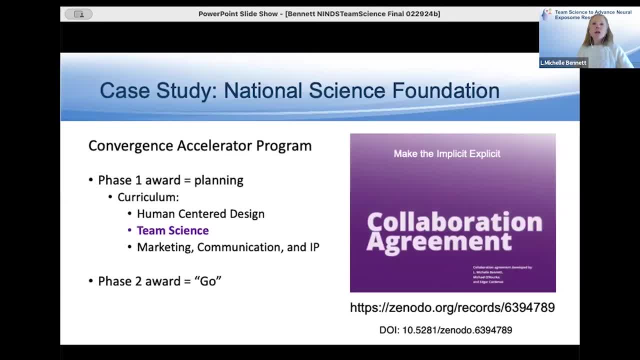 for the last I think about five years, And over the last five years we've sort of grown and evolved this team science component of their funding award and really matured. it had an opportunity to mature it. So how the Convergence Accelerator Program works is that there's a phase. 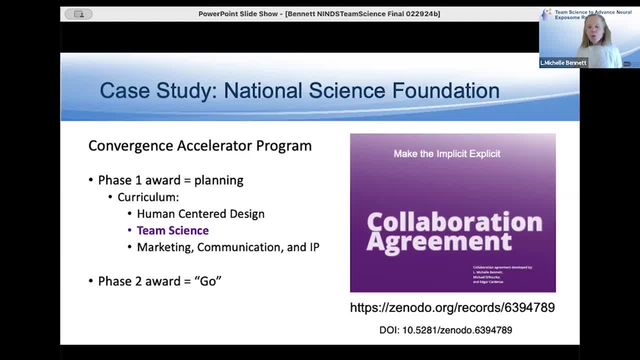 one award which is really a planning award, And during that award phase the teams get, I think, about nine months and they're run through a pretty rigorous curriculum run by the NSF. So I'm a member of the team science faculty. They also have a segment on human centered design. 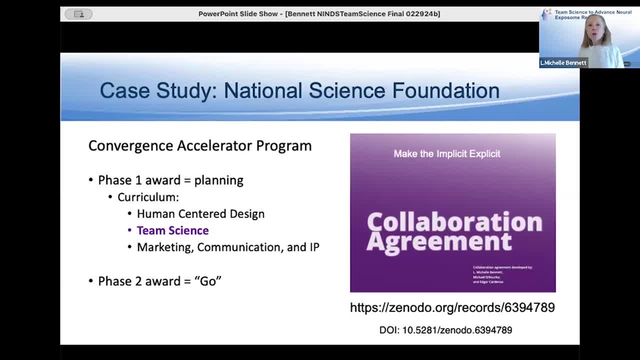 They also do marketing, communication and intellectual property. So as part of our the curriculum I've developed with my two collaborators, we created this collaboration agreement and you've already got a bazillion references now to collaboration. You can also see some of the collaboration agreements that you could take a look at. 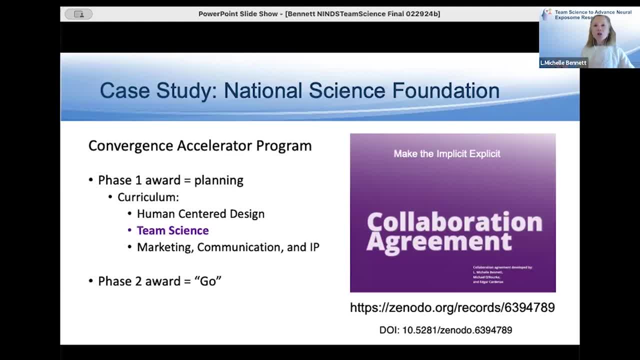 We developed this one for, again, the NSF. They let us genericize it And you can find it at this link if you're interested in taking a look at it, But it just gives you a sense of some of the things that are. 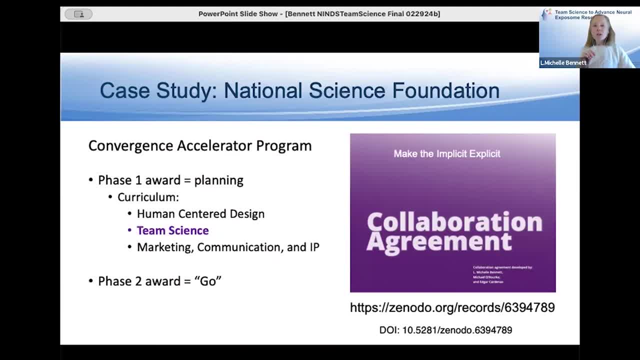 are, I guess, front and center for us, as we, as we see people work together and where the challenges really occur. So you've heard a number of great reasons to put in a, to put together a collaboration agreement, collaboration agreement. and I'll just mention a couple more. One is when you bring a new member. 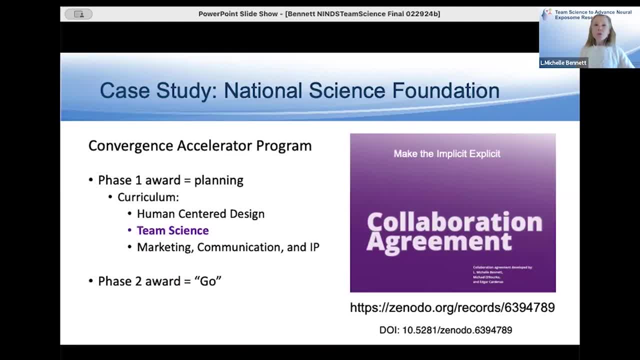 onto the team. it's a fabulous document to share with the new member to say this is how we work as a team. Read it over and then let's all sit down and talk about it. They might see things that you don't- new things and that's worth talking about. How are you going to handle? 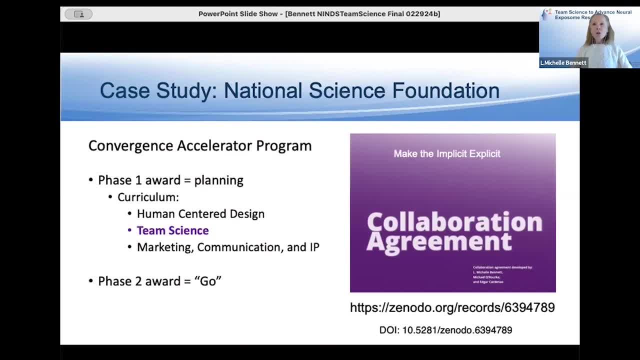 intellectual property. This can be a huge issue. If you think authorship is a big issue, IP issues can be really big too, and so those are really worth talking about up front. If I get one question over and over and over again, it's: how do we hold somebody else accountable, especially when you're 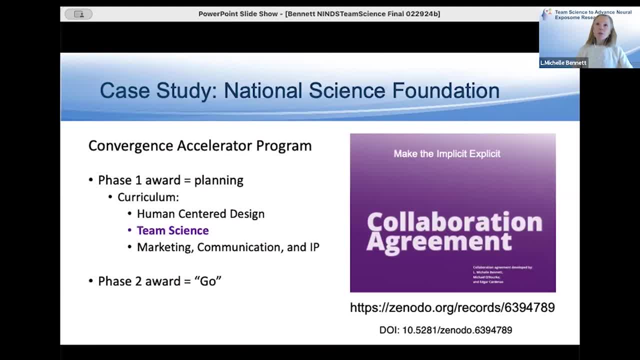 bringing together PIs, peers from different disciplines, and that's another area that you can cover in the collaboration agreement. But the point I really wanted to make with this slide is that all of the teams who, during phase Phase one, took the team science curriculum seriously and put a collaboration in place. 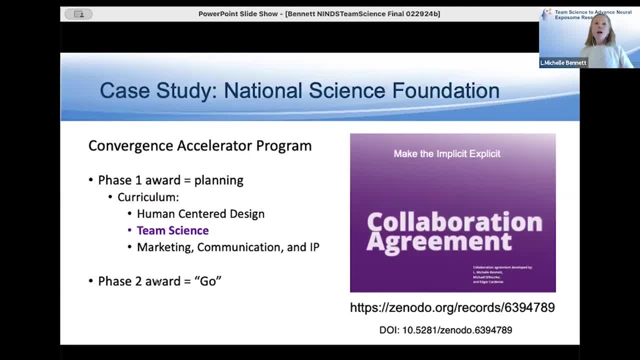 a collaboration agreement in place and really worked together as a team, have been successful in the phase two award process, And I think that just kind of speaks loads to the impact that being clear about how you're going to work together can have in a funding application. 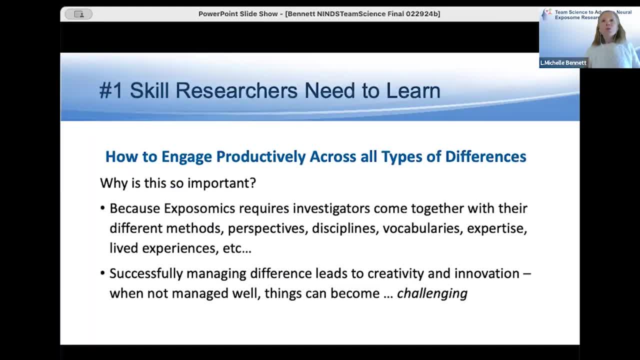 So what do I think the number one skill researchers need to learn is really how to engage productively across all types of differences, And when I say differences, I mean all of the differences that you've heard each of the investigators talk about up until now. And why is this so important? Because 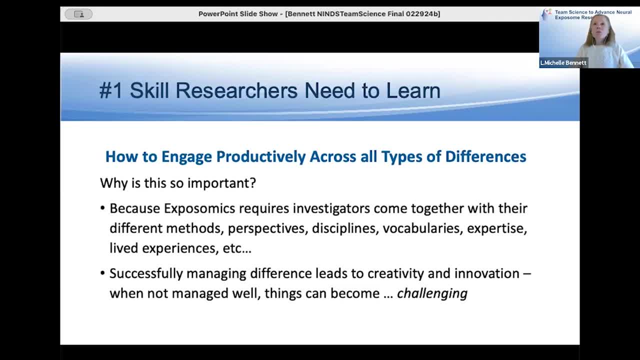 exposomics requires that investigators come together with so many different things- different methods, different perspectives, different disciplines, vocabularies, expertise, lived experience, etc. in order to do more than any one of them can alone- And I think you've already heard about some of the challenges- and just even harmonizing data. 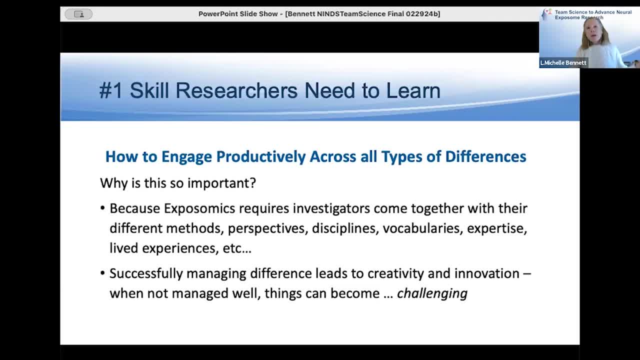 for example. So successfully managing difference leads to creativity and innovation, And when it's not well managed, things can become really challenging. And so, when I We talked a little bit earlier as well about productive conflict- for scientists to learn how to engage in conflict in a way that, where it's not seen as something negative happens, but it sees it's seen as something positive that happens, that can be easily overcome. 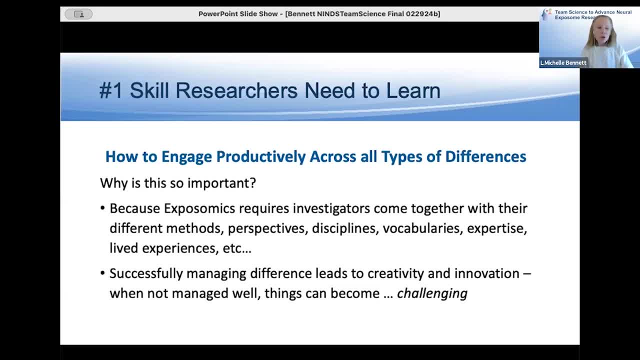 And that's whether you're having those types of issues in the context of the science. I think for scientists it's easy to engage in productive conflict over the science, at least more so than relationships. But if you can treat those relationship challenges in a very similar way, they can be incredibly productive as well. 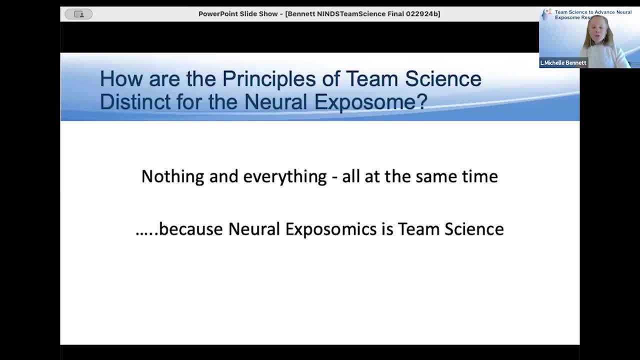 So when I had a pre-meeting with David and Karen and Corey and And a few other people, one of the questions they asked me is: how are the principles of team science distinct for the neural exposome? So here's my answer: Nothing and everything all at the same time. And the reason I say that is because I think neural exposomics is a team science. 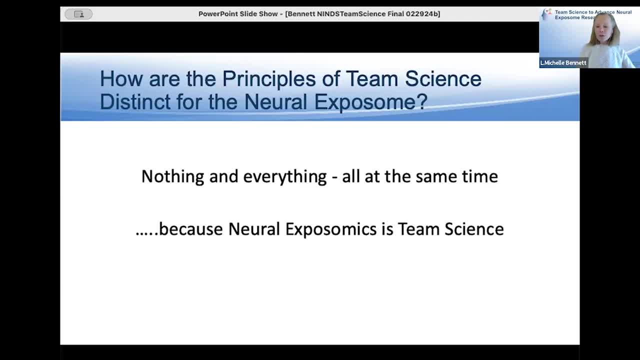 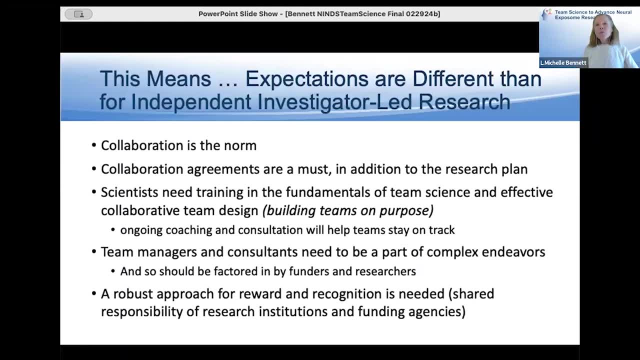 They're one and the same, And I think that's a huge opportunity, and it's probably also a huge challenge at the same time. So what does it mean? It means that expectations are different than for independent investors, And so the goal of the team science is to have partnerships and to have people who are involved in the team science. 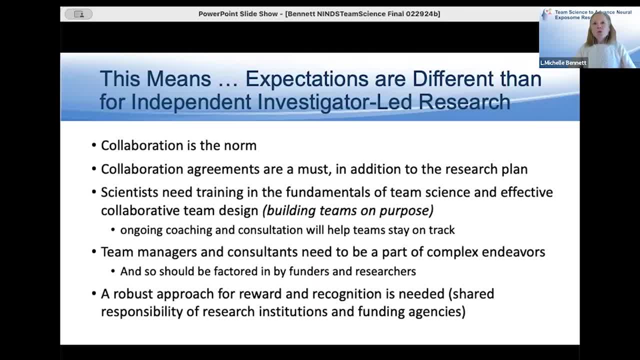 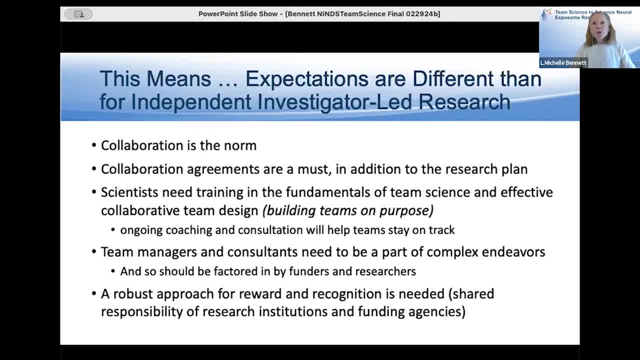 So this is a very important point, And what I think is really important is that collaboration is the norm. It's not the exception. The collaboration agreement is a must. in addition to the research plan, Scientists need training in the fundamentals of team science and effective collaborative team design. 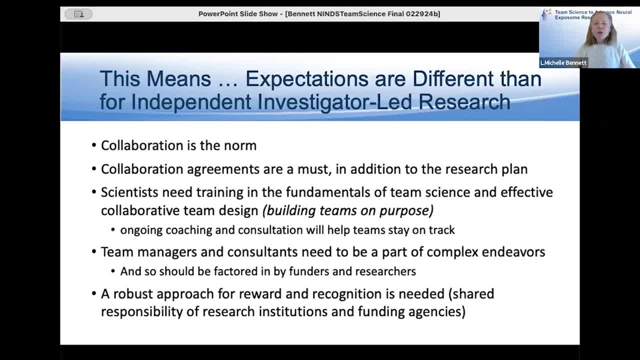 So this is back to my building teams on purpose And providing opportunities for them to have ongoing coaching and consultation can really help them stay on track. I think the three previous speakers made this look so easy, Like oh yeah, anybody can do it, And I really applaud them, because not everybody can do this And especially those people just starting out can really use a lot of assistance and understanding how they can go about doing it. 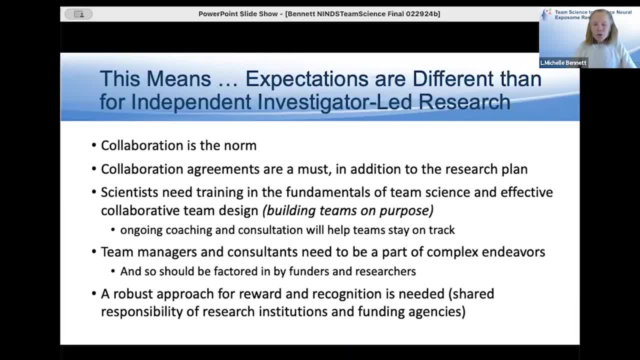 I heard some discussion about how team or project managers or team managers have been integrated into some of the funding announcements And I think that that's absolutely essential. I think asking people to form very complex collaborations and not funding them to have a team manager or consultant or people to help them along the way would be really problematic. 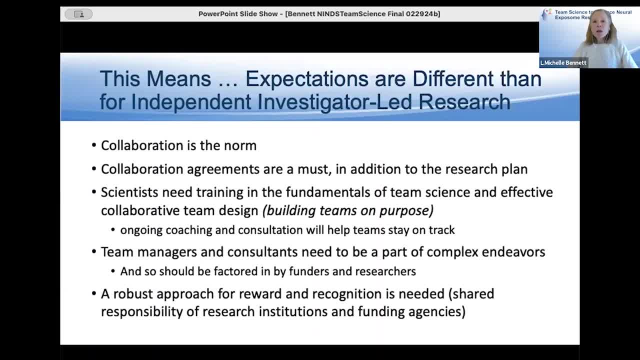 And then I just will build on what Heidi said: Having a robust approach for recognition and reward is needed, And I think this is a shared responsibility between research institutions and funding agencies, so that there's some back and forth. When I was at NIH, I was told by a number of very prominent NIH leaders that well it's. you know, it's really the research institutions. 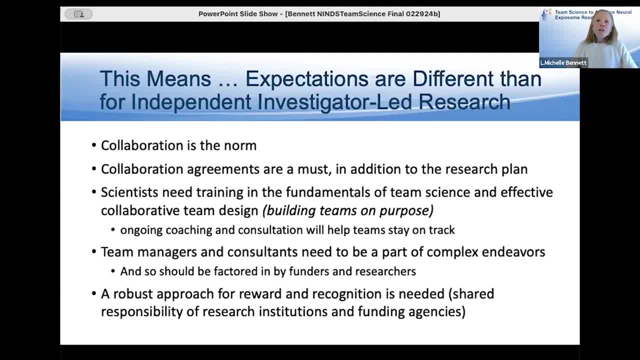 It's the research institutions problem to figure it out, And I actually think this is a place where collaboration could work really well, because I think research institutions are trying to do their best to recognize and reward their faculty, And I think if there's any way for funding agencies to work collaboratively with research institutions to make sure everybody's on the same page, especially as funding agencies are funding more and more team science, I think that'll just be much more powerful. 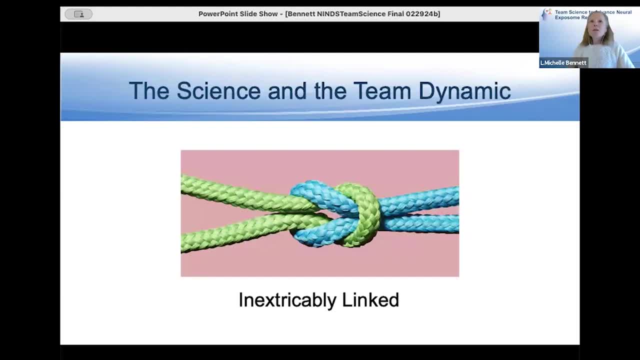 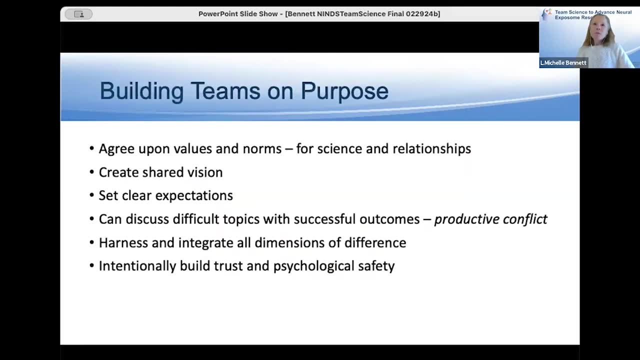 So team science and the team dynamic are inextricably linked. You can't have one without the other. And in order to build teams on purpose, these are the things that you can think about: Agreeing on values and norms, creating shared vision, setting clear expectations. 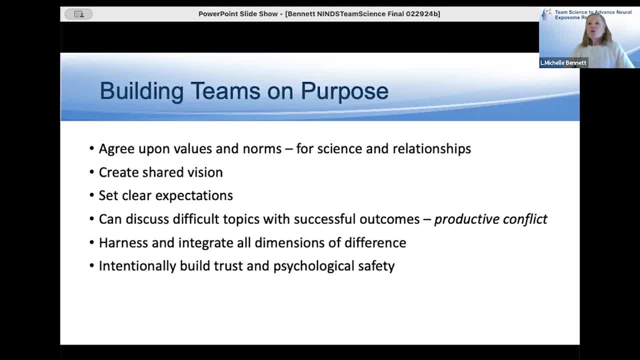 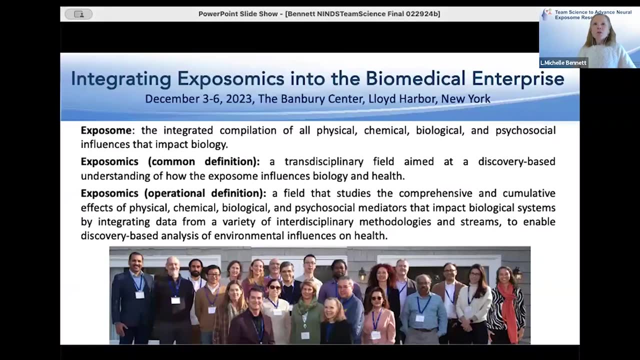 And I won't say the rest of them because I think you've heard them all already from everybody else. I will mention the building, trust and psychological safety, because they are absolutely essential and maybe haven't been spoken to as much. So the last thing I wanted to just mention is that Gary Miller- I think he's still on the call- 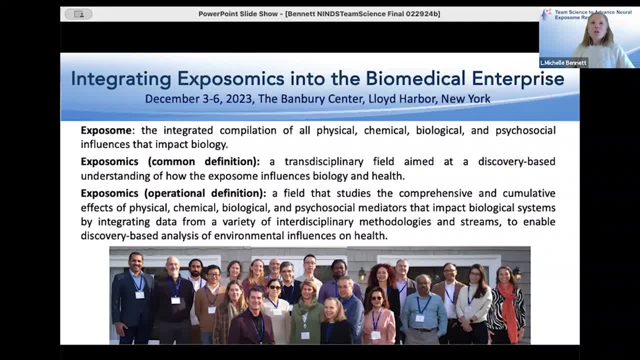 Yep, he's still there- Reached out to me late last year and told me that he really wanted to bring together a number of scientific experts, A number of scientific experts, A number of scientific experts- And we're really focused on exposome- and bring people together from all the different disciplines that they represent to put in place a definition for exposome and exposomics. 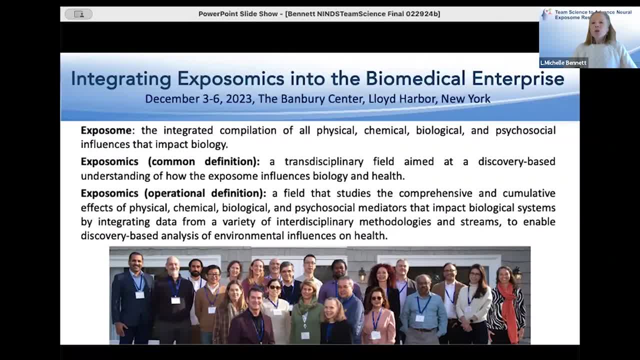 And so that the research community could be much clearer about what this is, what its foundation is, and how different disciplines- disciplinary areas like the neuro space- could build upon that and create a definition. And so that the research community could be much clearer about what this is, what its foundation is, and how different disciplines- disciplinary areas like the neuro space- could build upon that and create a definition of their own. 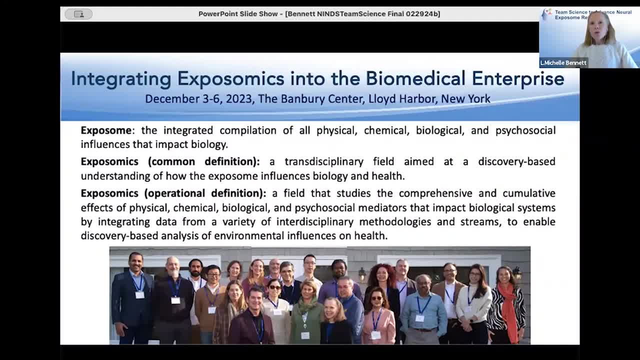 And so we worked together last year to design this conference and bring a very, very diverse group of people together to take on this task. It was so it was viewed as such a challenge that a number of people told us that it wasn't even going to be possible. 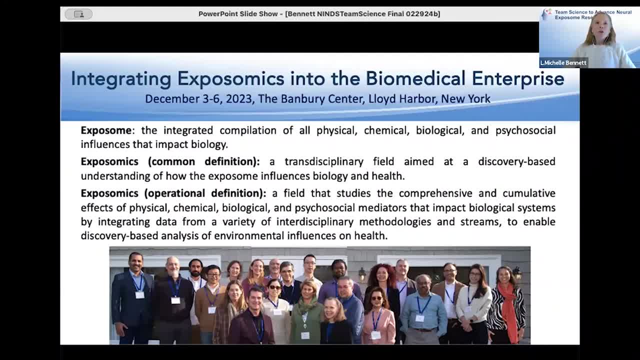 But we met in early December and I think we ended up being very successful and being able to walk away from that conference. Pam was there, David was there, Sophie was there And we were, I think, really heartened that you know, it is very possible to bring people with very different backgrounds together to do something really, really important. 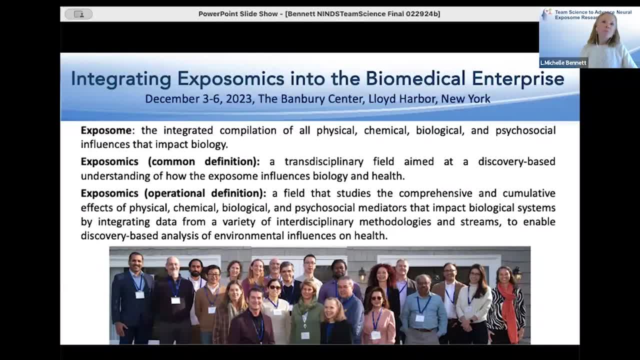 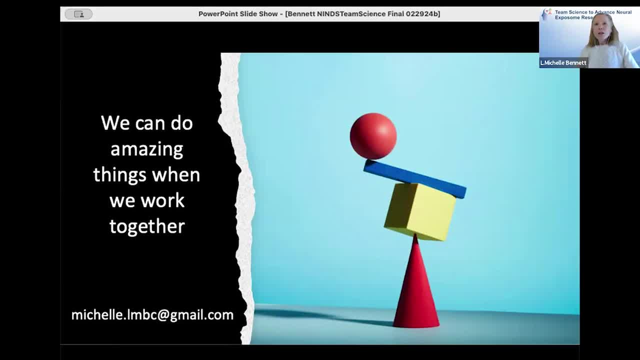 And so I just didn't want to fail to mention that as I closed up. So my last note: we can do amazing things when we work together, And I want to thank you very much for the opportunity to talk to you. Thank you. 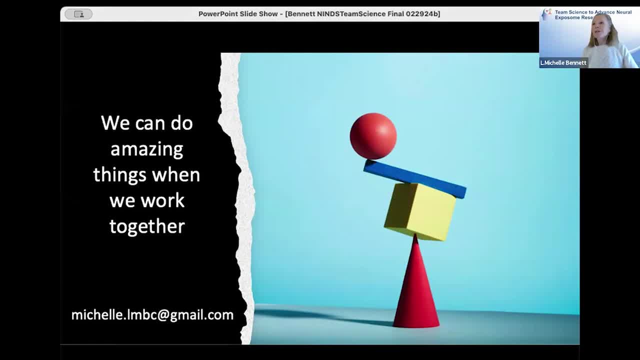 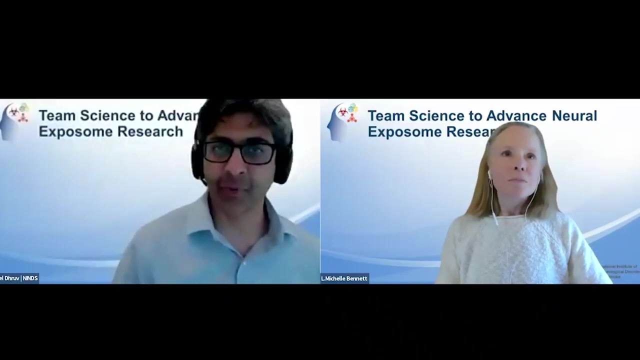 And I think you probably figured out that I enjoy this area a lot. I'm very passionate about it. Okay, Thank you. Thank you very much, Michelle. I'm going to take the. you know, let's hold questions. Well, I think that you know. the next thing that we have is the discussion. 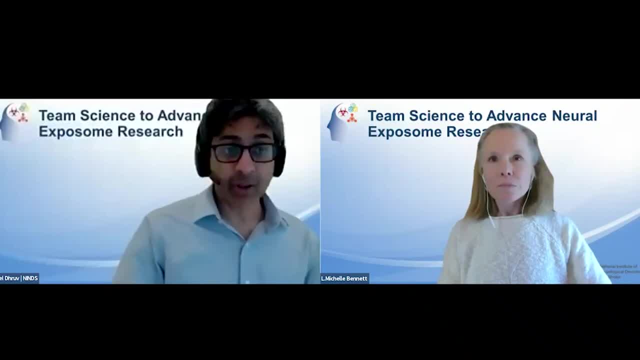 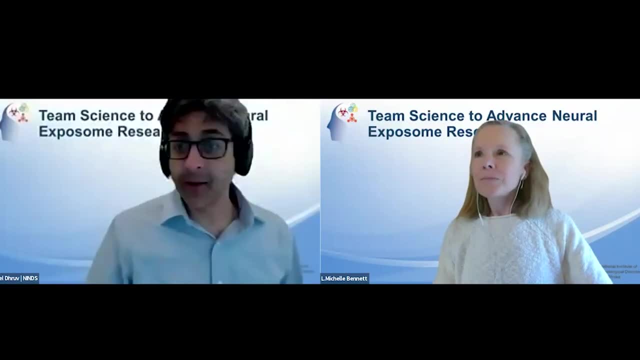 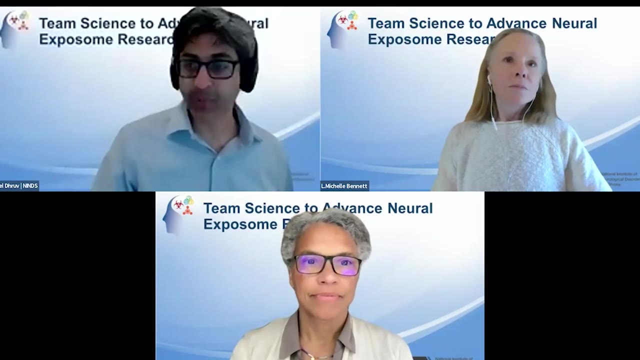 So Maybe the questions for Dr Bennett can just come in as part of that discussion And I also see from that. there was a question in the Q&A asking if the workshop recording will be made available. The answer is yes. I will email all registrants when that is posted. 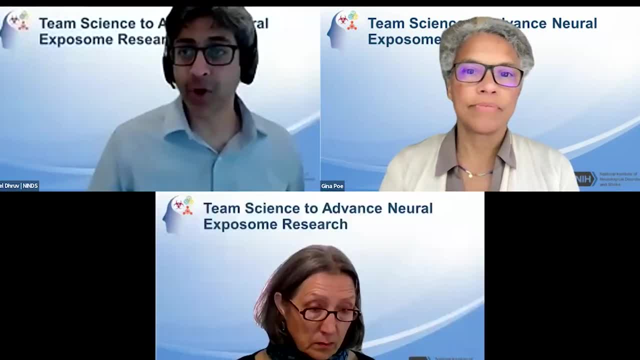 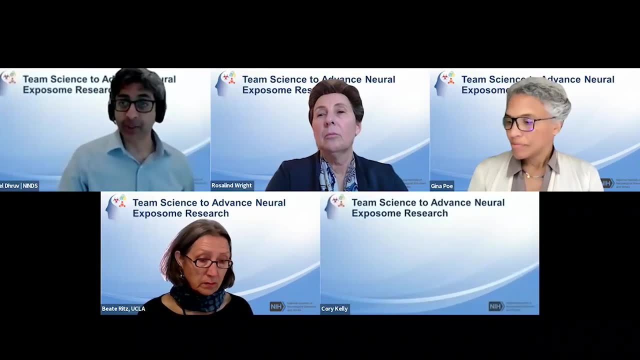 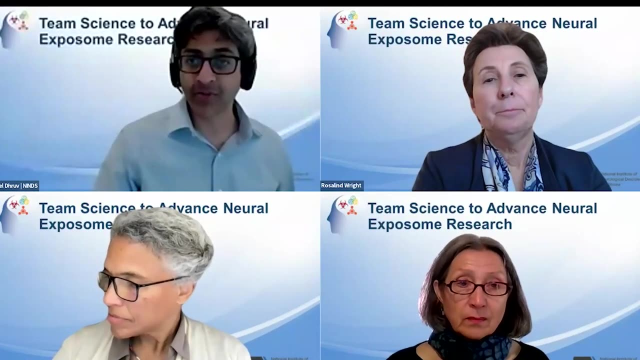 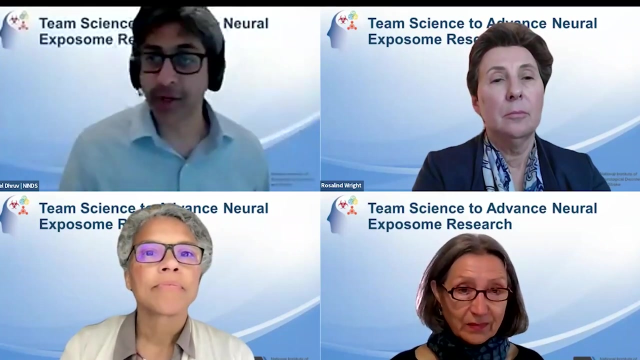 Okay, So now we will move on to the panel discussion. in addition to the speakers that we've had, We have two panelists joining us: Dr Beata Ritz and Dr Rosalyn Wright. Dr Beata Ritz is a professor of epidemiology at the UCLA Fielding School of Public Health, with co-appointments in environmental health sciences and neurology at the UCLA School of Medicine, and a member of the Center for Occupational and Environmental Health. 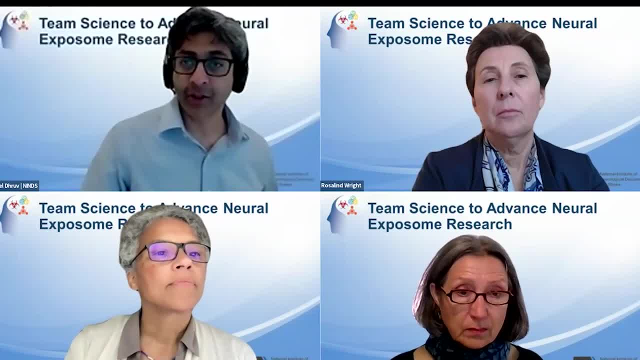 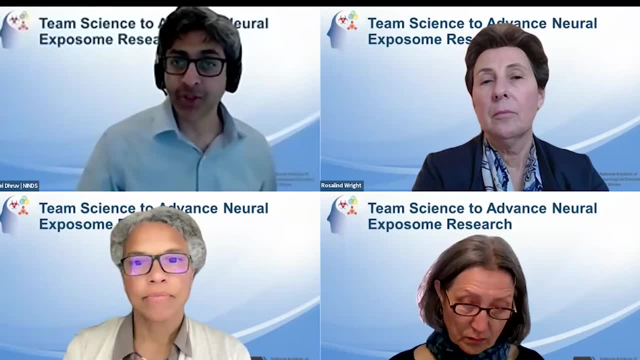 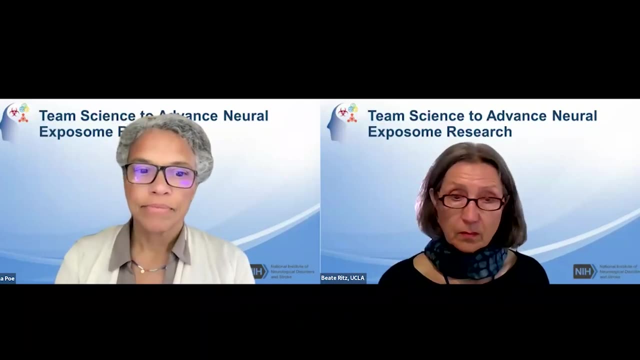 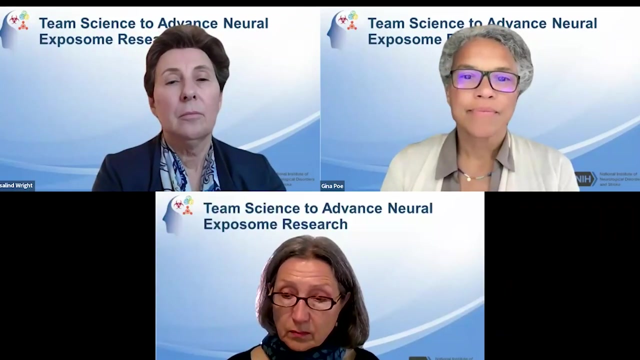 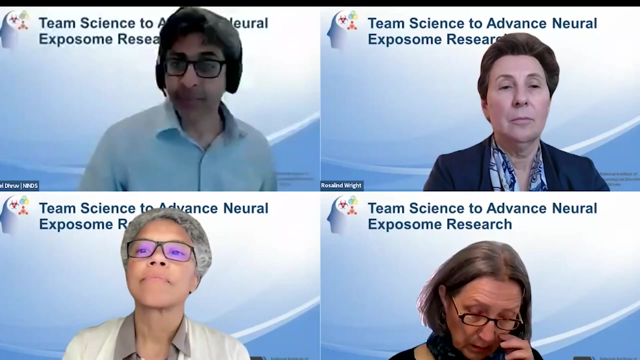 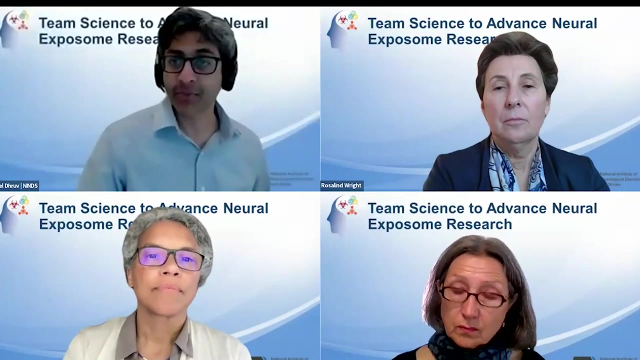 She co-directed the NIEHS-funded Center for Gene Environment in Parkinson's Disease at UCLA that included neuroscientists, human geneticists and clinicians. She initiated She initiated the field of air pollution and pregnancy outcome research in the mid-1990s and her lab has studied the effects of occupational and environmental toxins, focusing on air pollution and pesticides, developing geographic information, system-based exposure assessment tools and, more recently, omic tools to discover biomarkers for environmental factors impacting pregnancy and reproductive outcomes and neurodevelopment. 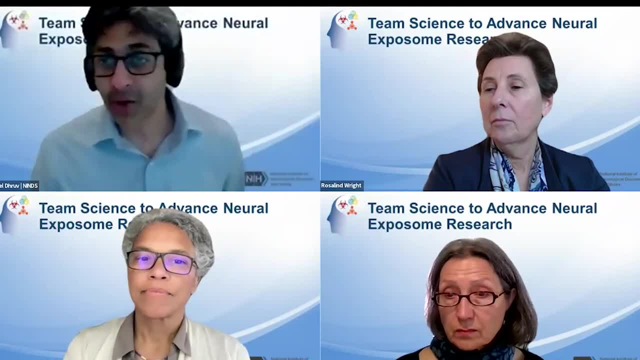 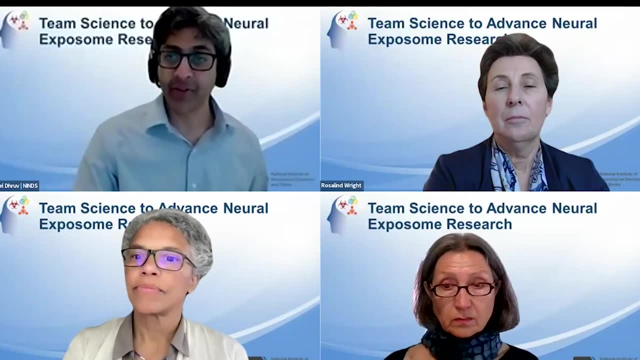 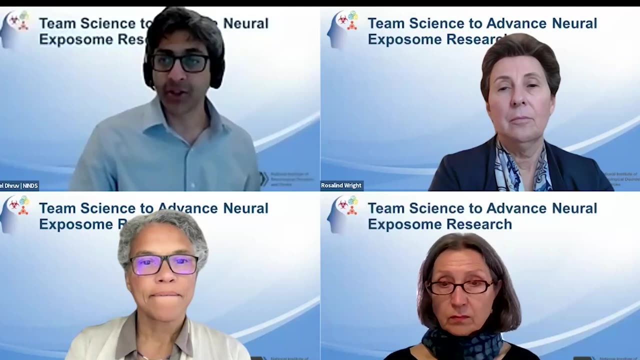 Dr Rosalyn Wright is the Horace W Goldsmith Professor of Life Course. Dr Dr Wright is a professor of environmental health research in the Department of Pediatrics and Environmental Medicine and Public Health at the Icahn School of Medicine at Mount Sinai. a physician and an internationally recognized life course epidemiologist with transdisciplinary training in perinatal environmental programming of chronic disease risk. 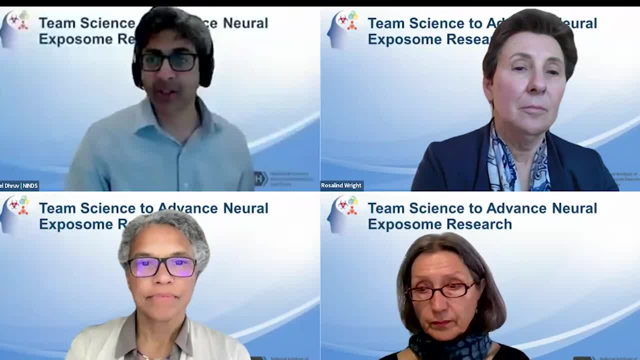 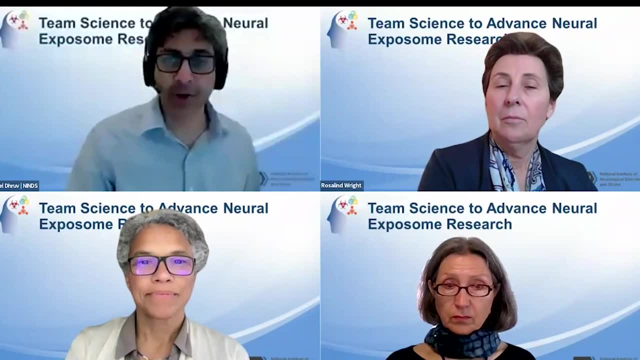 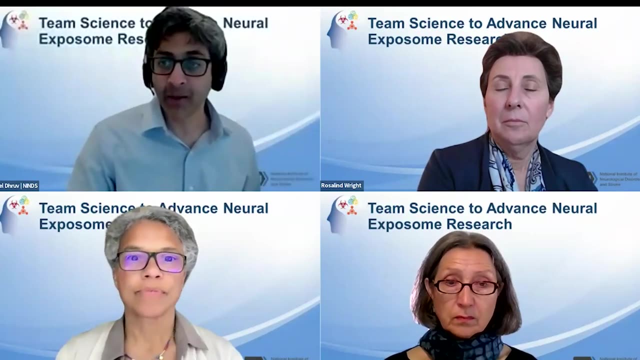 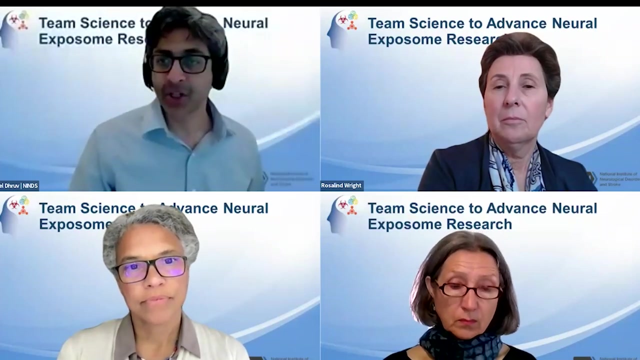 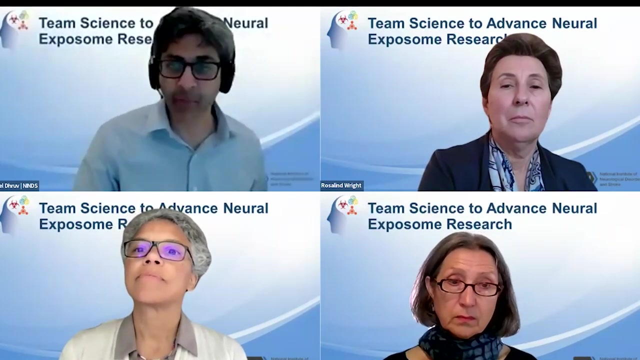 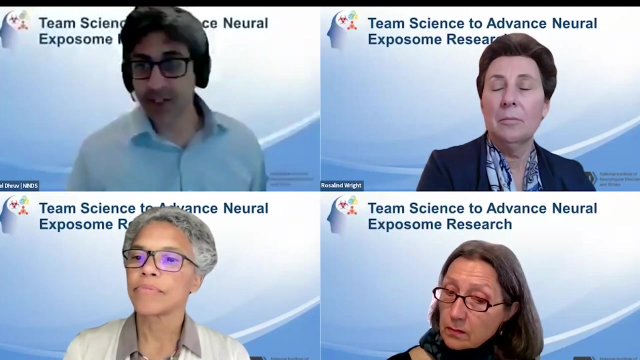 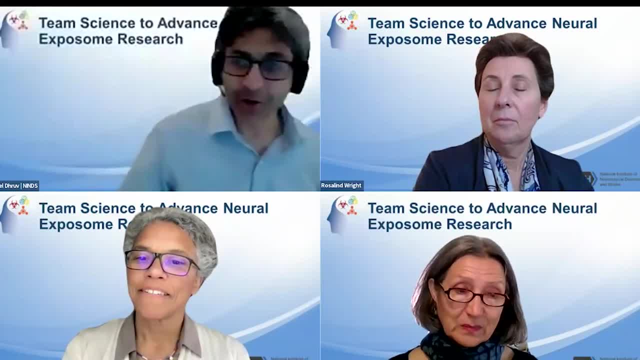 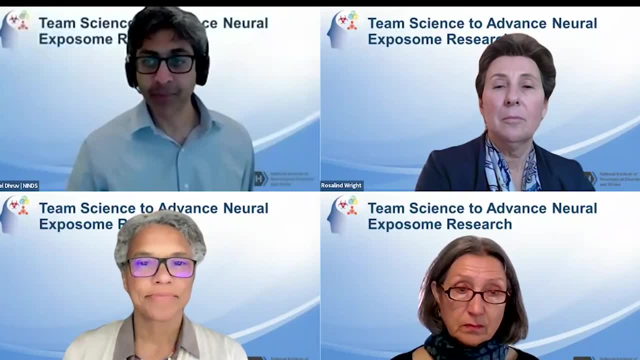 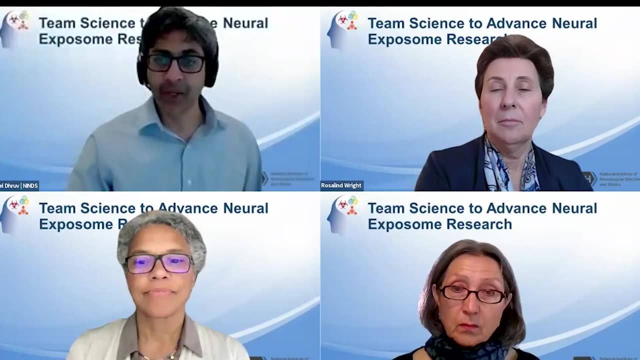 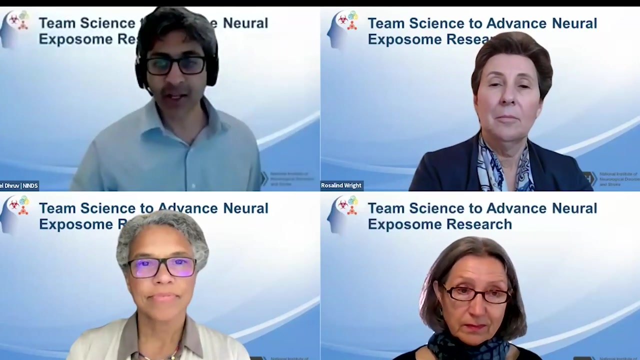 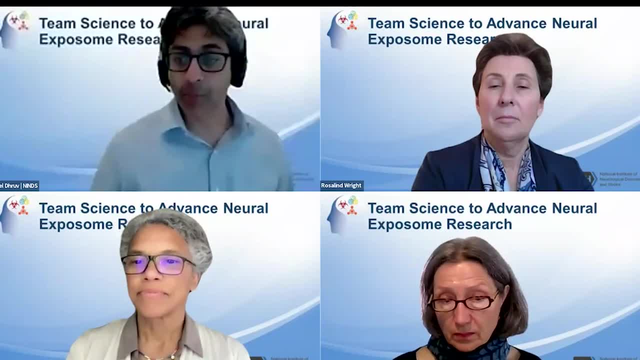 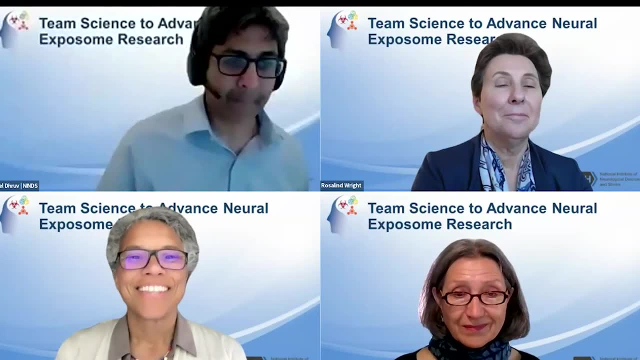 I'd just like to encourage you to keep entering your questions through the Q&A box. We'll be able to incorporate those into the general discussion. Gina, I'm happy to hand it over to you. Thank you so much, Neil. Thank you everyone. This has just been amazing. 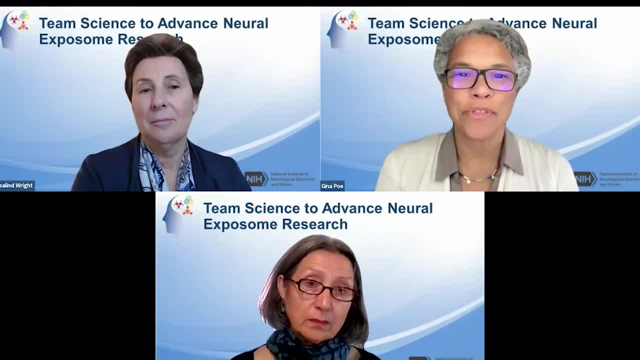 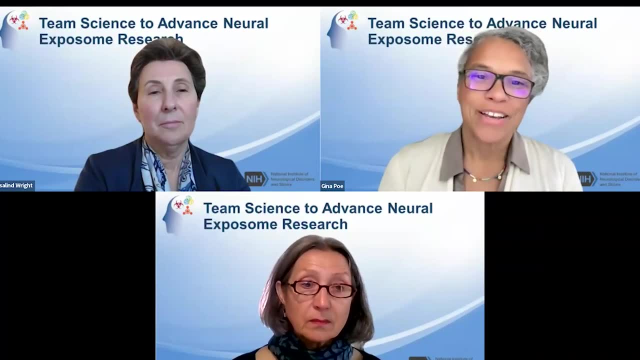 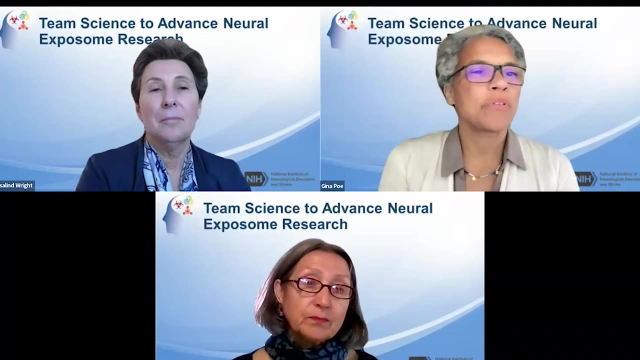 So the purpose of this panel discussion Q&A is to really sort of thump a lot of the points that were made and also to bring up new considerations given the breadth of experiences that our panelists have. So I'm going to open up with the first one for both of you, which is really why is team science important in neural exposome research? 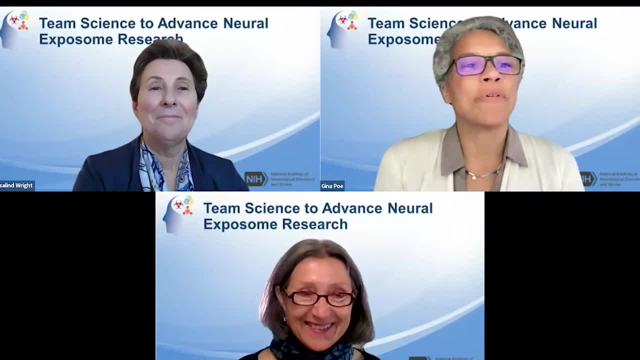 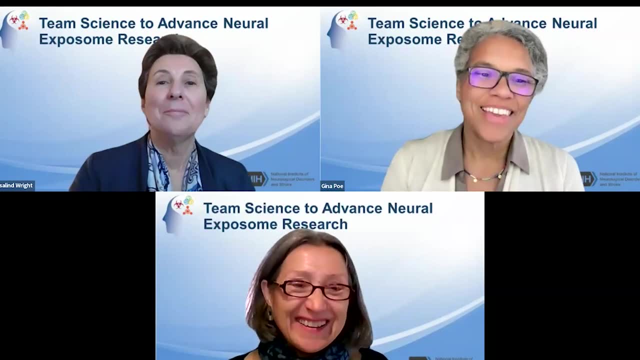 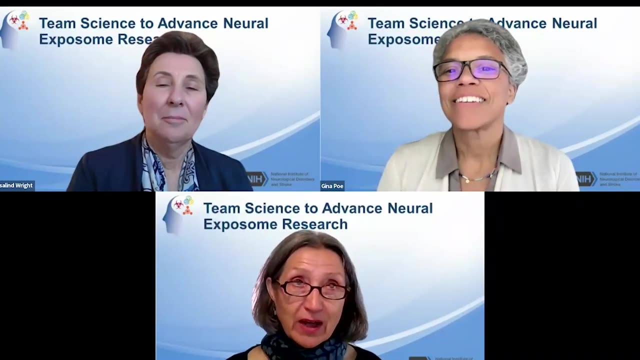 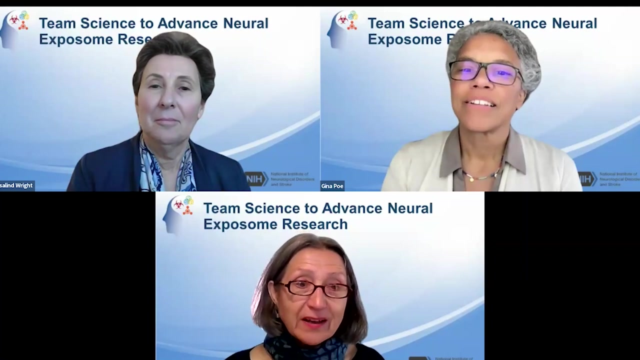 Why can't we do this the old way, like individual cowboys with our ones? So you want us to answer? Yeah, I think so. So I would say I would have never had so much fun doing research if it hadn't been interdisciplinary and, in the end, transdisciplinary. 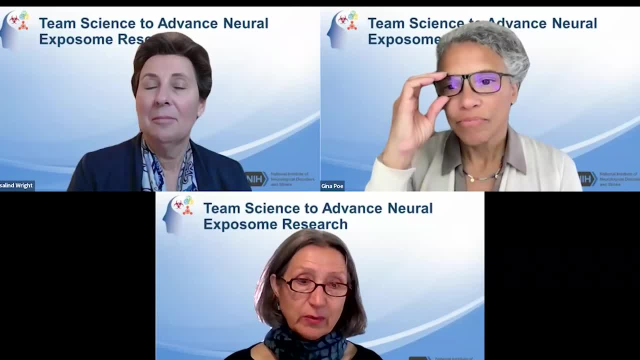 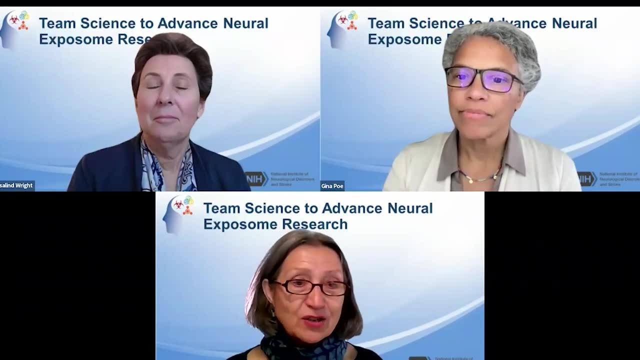 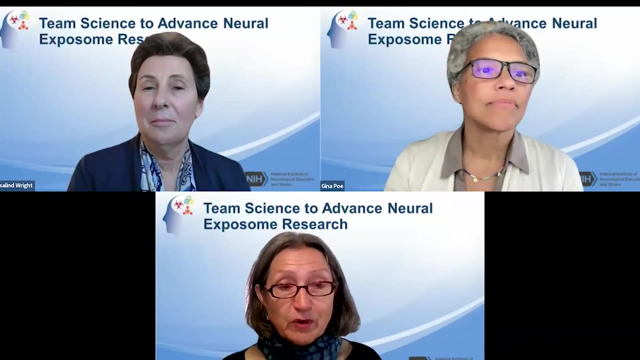 And I would like to say that it's not just bench to bedside, which we are all familiar with, but it's really cells to populations, And you know I'm at the end of the population spectrum here And these kind of scientists that I represent, we deal with humans and we deal with populations outside of hospitals. 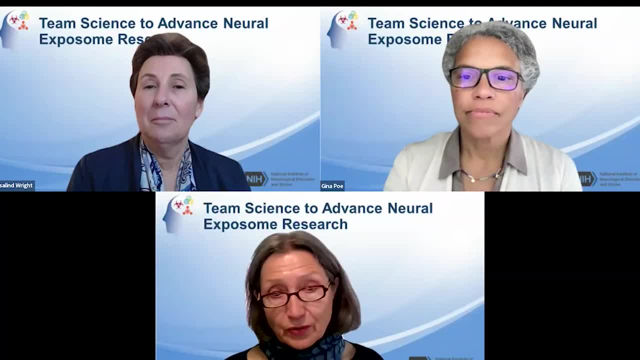 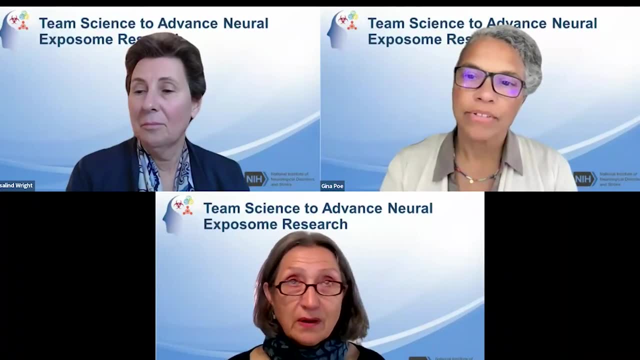 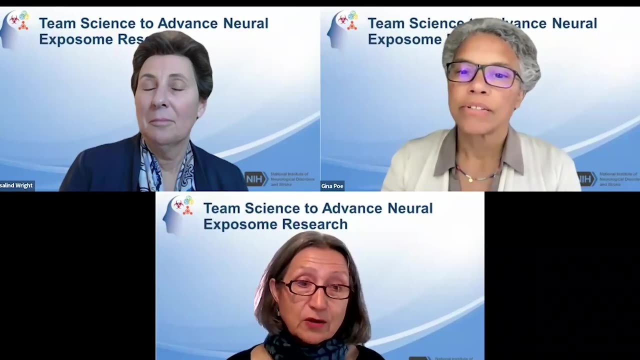 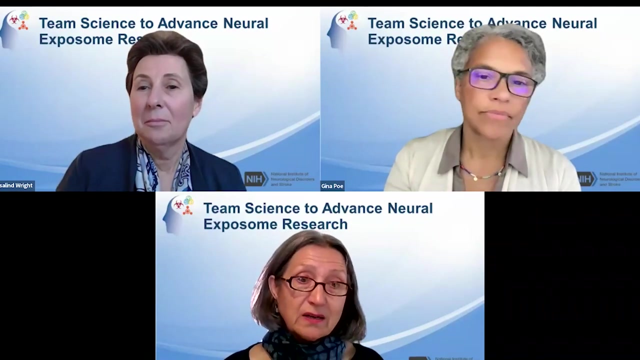 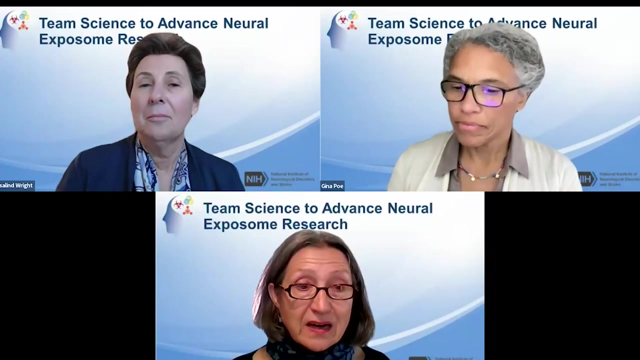 And that's sometimes extremely difficult Because you try to do population based research And within that environment you're trying to. you try to define the environment for populations and for special groups that may be disadvantaged because of certain types of exposures And to bring that back to basic scientists and toxicologists, who have very different questions to answer in with lab animals and cells. 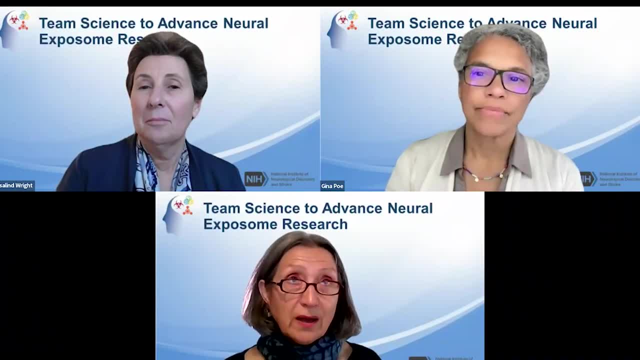 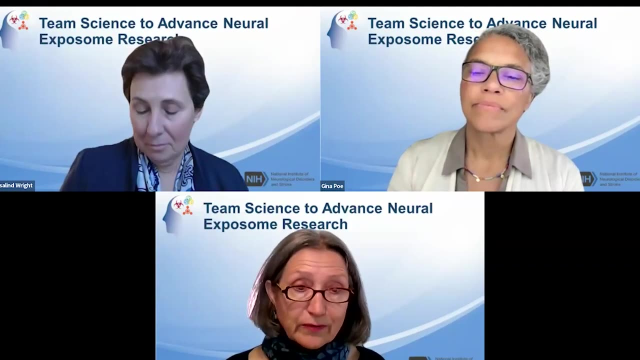 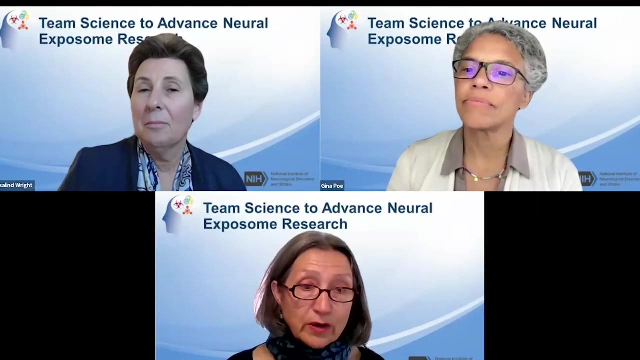 That takes a lot of energy and communication and translation And I think especially kind of going beyond our own value systems- And that is one thing I learned over the last 25 years of talking to many scientists from other areas- is we have very different value systems in the way we look at science and scientific validity. 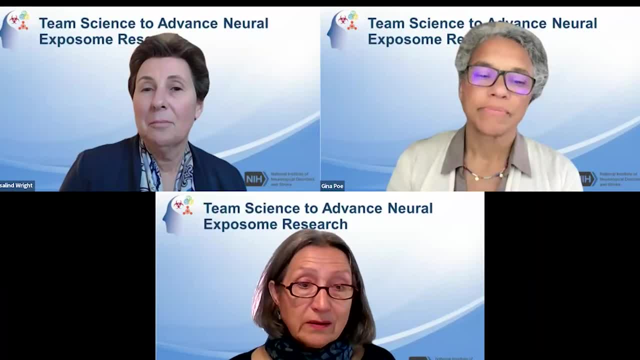 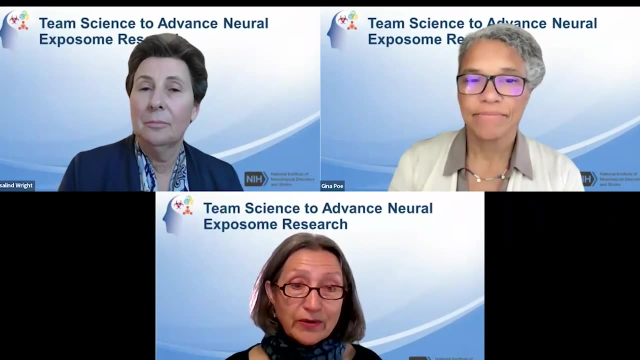 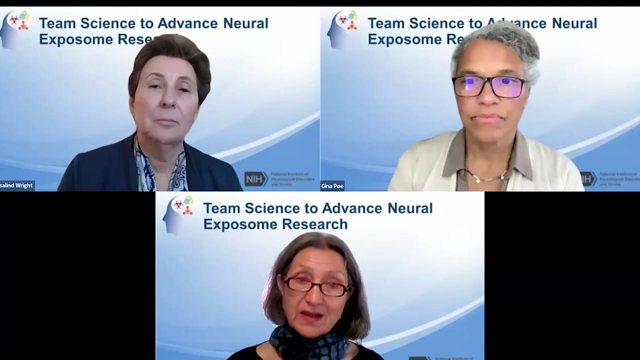 And we have to learn to respect each other And to kind of speak each other's language and find a way to not disparage each other, which is something that actually has happened many, many years when I was a junior scientist and felt, like you know, population sciences are really not valued by basic scientists because we don't have a lab. 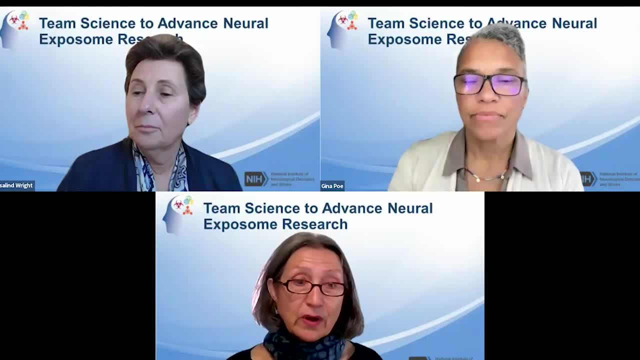 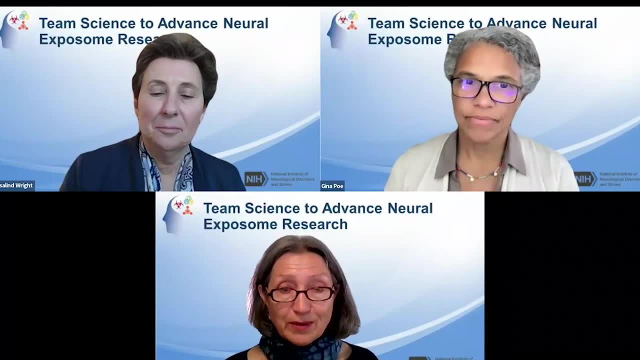 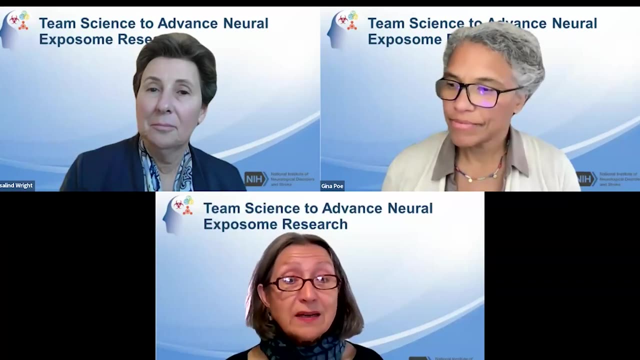 We don't do experiments, We just observe. So everything is an association And in the end we don't know anything. And to fight that was really a big struggle. But the big, the big challenge that that encompassed really made it much more interesting what I did. 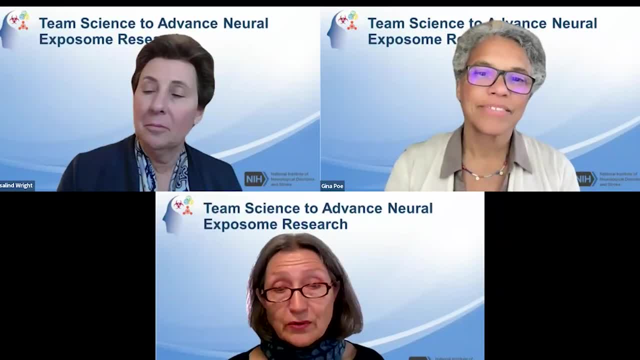 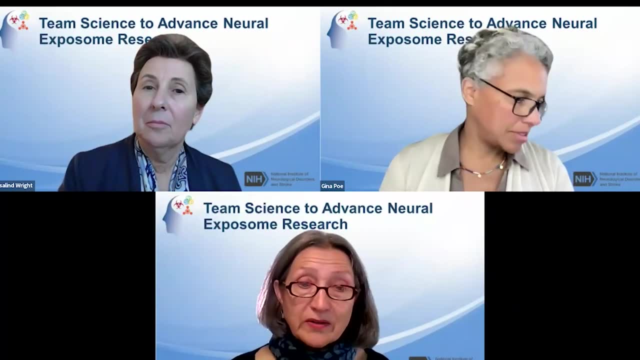 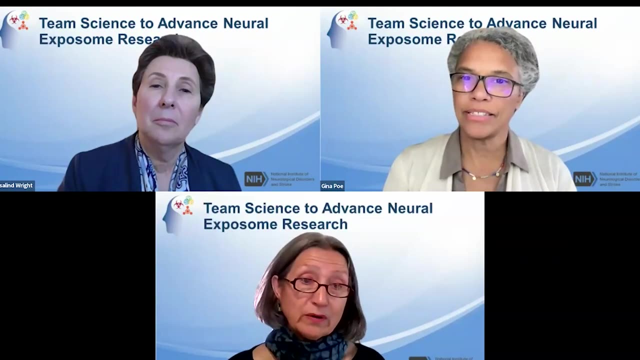 And I was able to probably introduce into population sciences a lot of tools and techniques as well as insights that, without being challenged, Those tools, Those supported that specific purpose. And you know I never stepped a toe to those tools because I was definitely getting challenged by my collaborators. 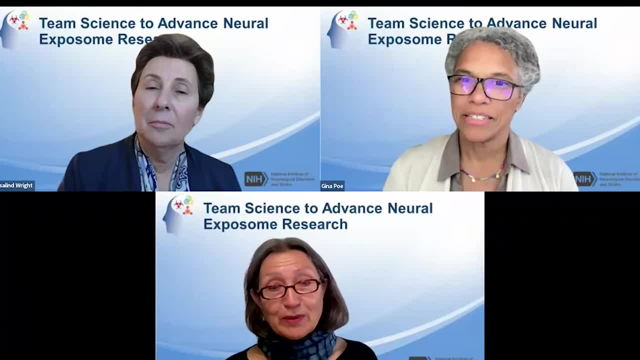 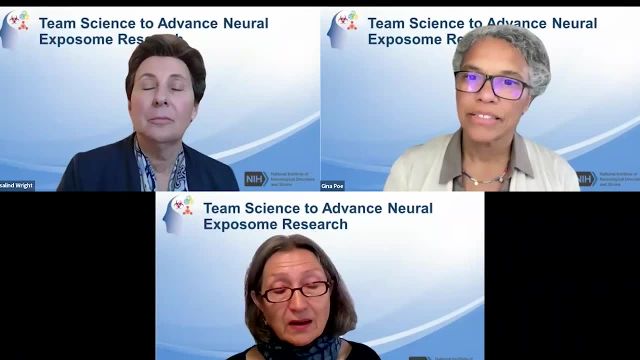 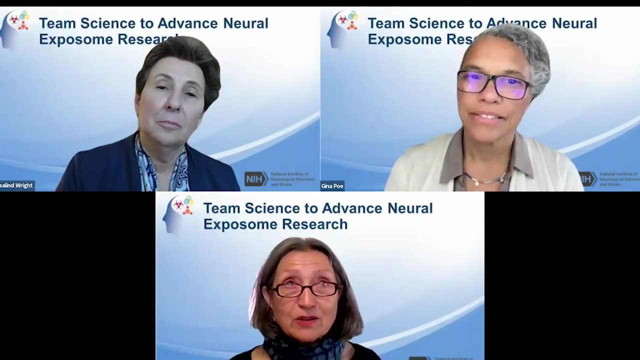 I never wouldn't step a toe in, And so I went from being a straight population science association type analysis person to understanding a lot more about cells and metabolomics and genetics and epigenetics, And I see how much my trainees actually enjoy being able to use all of these tools and to reach out and figure out where there's actually space and surface there. 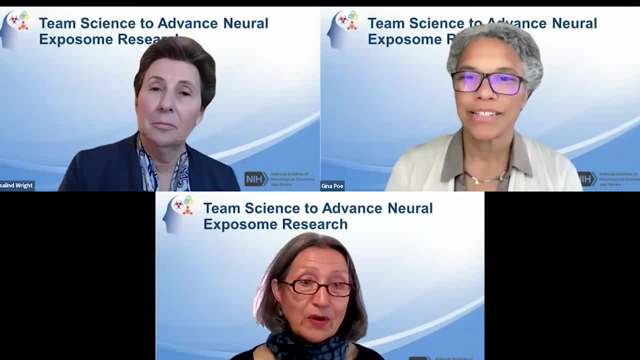 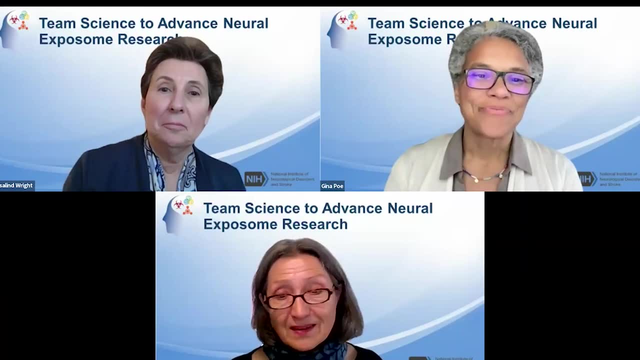 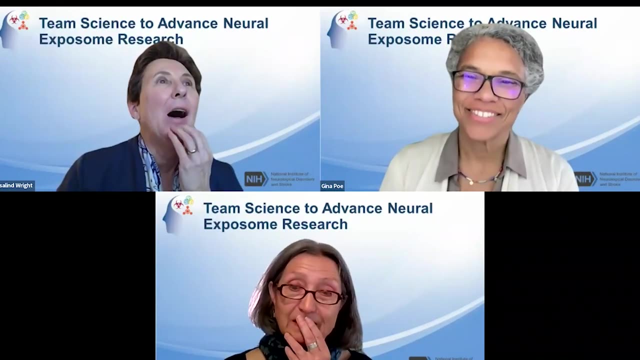 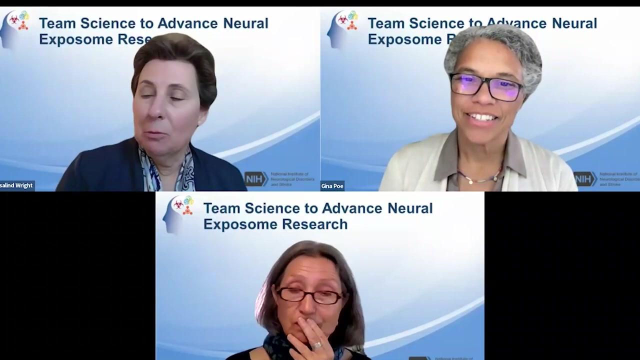 out, And they are much better at this than I am, So I want to really compliment everybody who says we have to bring the trainees in. Rosalind, do you have a perspective on this? Absolutely, I think I became a team scientist in a transdisciplinary research, much in the way. 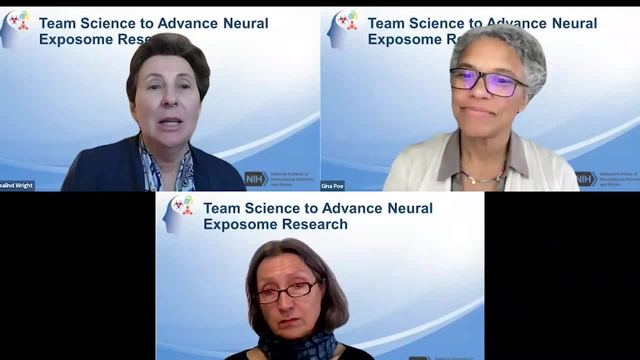 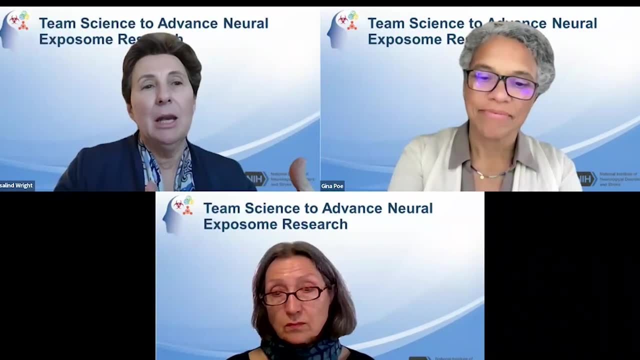 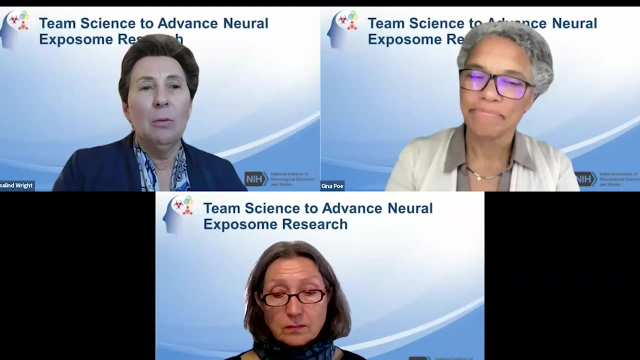 that I think Dr Jay Lee was talking about in his talk. He trained, he had great training in neuroscience, but he realized he, he, he was limited in being able to ask and answer the types of questions you know. he ultimately ran out of runway to say: well, wait, I, this isn't. 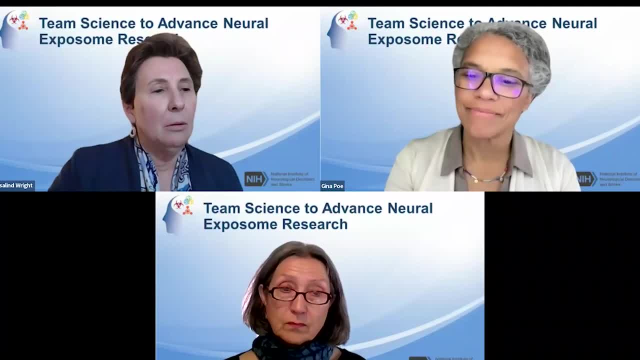 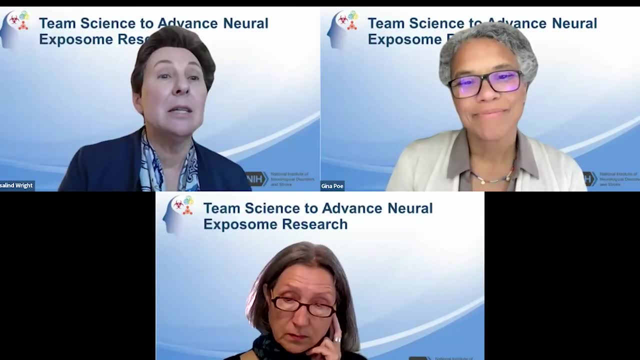 getting me further. And then he's he along the way. you learn, well, maybe I need to know something about immunology And maybe I need to know something about basics Cell biology. And we kind of did that, We felt our way because team science wasn't something that. 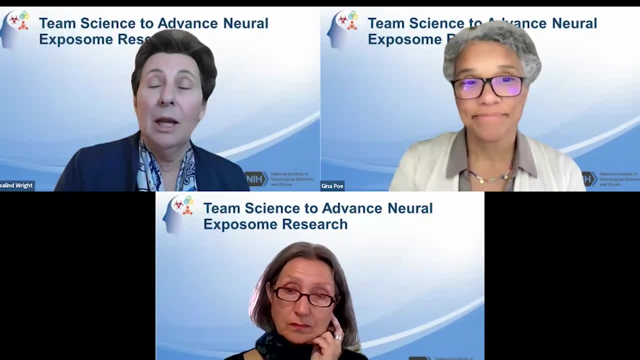 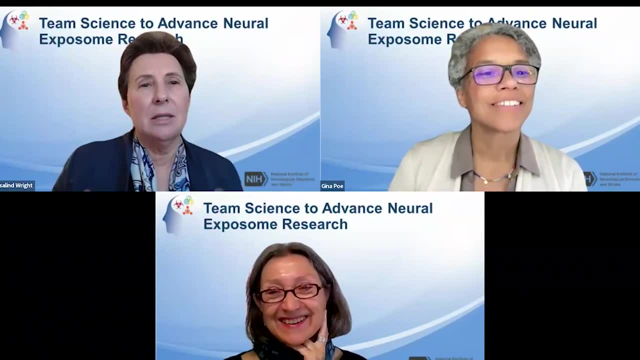 was being talked about when I was kind of coming through And actually people would tell me I was unfocused because I would say I need to talk to this And they would actually see it as a as a detrimental thing. Now, clinically I'm. the one thing that grabbed me in medicine was 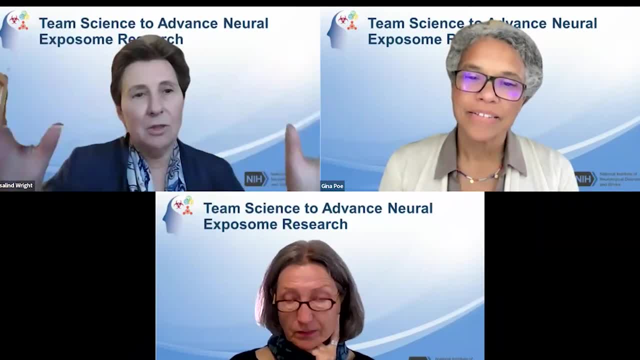 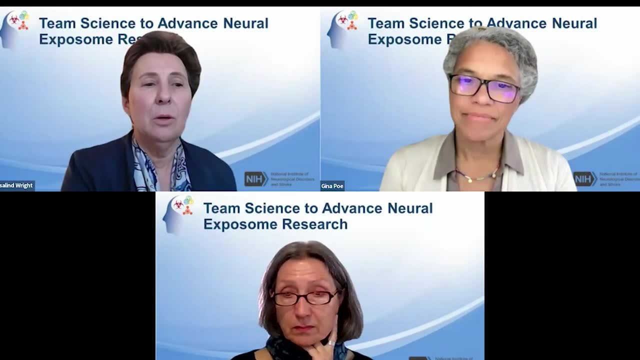 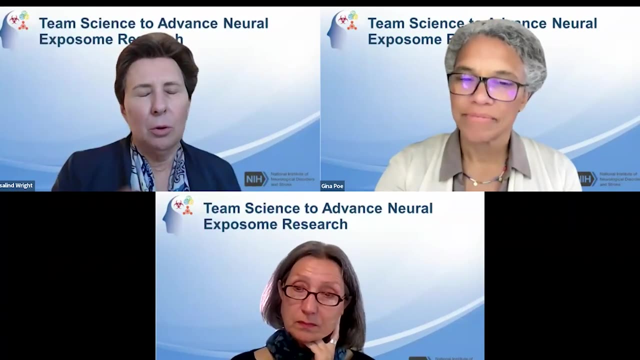 critical care medicine because I wanted to understand the whole and I'm an adult, trained critical care Intensivist. but my research all goes back to how far back do I need to go to prevent chronic comorbidities and early you know? you know shorter lives et cetera. And I go back all the 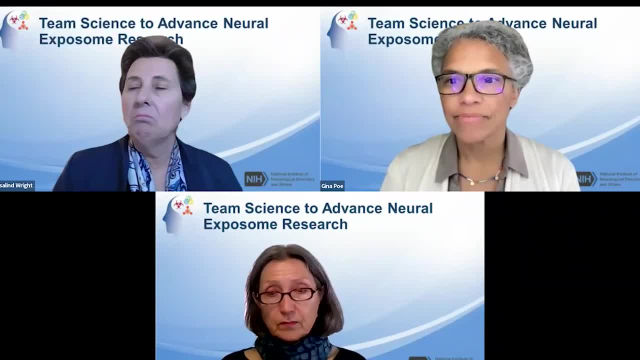 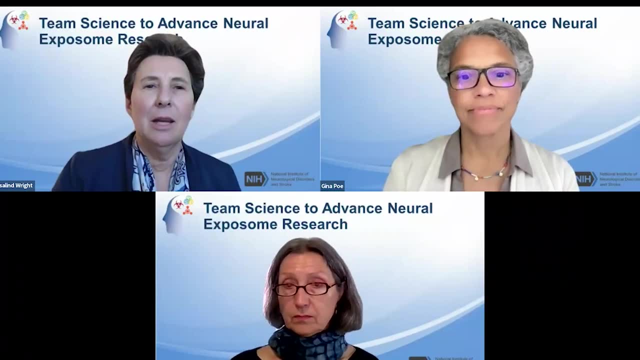 way to the prenatal period And then you start to want to understand: well, why is it different in different populations? And you know, I was trained originally in genetics and I realized it's not in the genes And we talked about that. Dr Jet talked about that right at the beginning. Can't be. 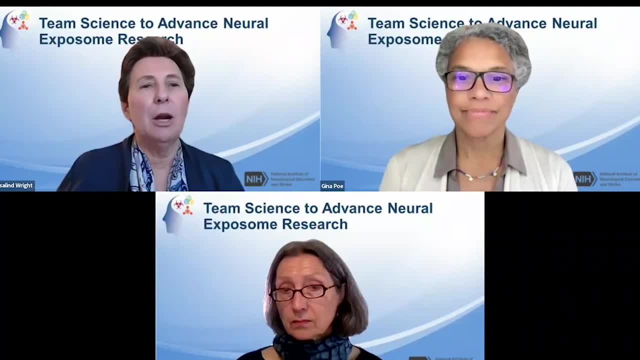 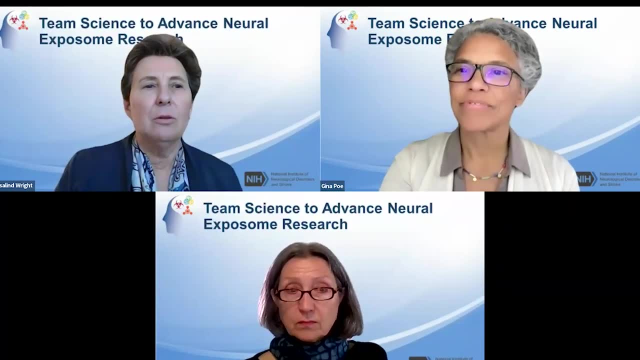 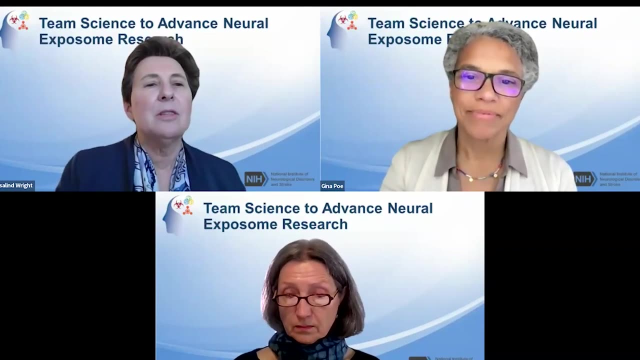 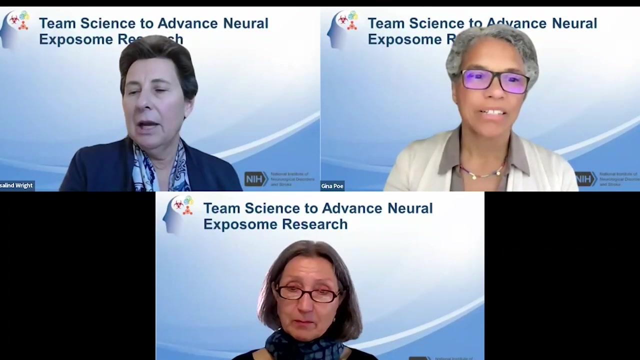 happened too fast. Well, now I need to go get some training in biochemistry. And I'm like: well, I need to go get some training in biochemistry And I'm like: well, now I need to go back and get trained in stress and health. So I was. I really liked the fact. 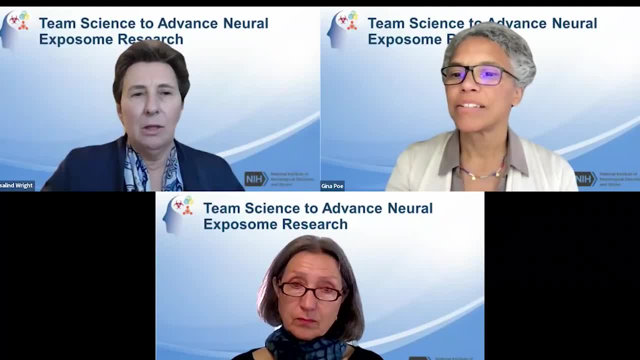 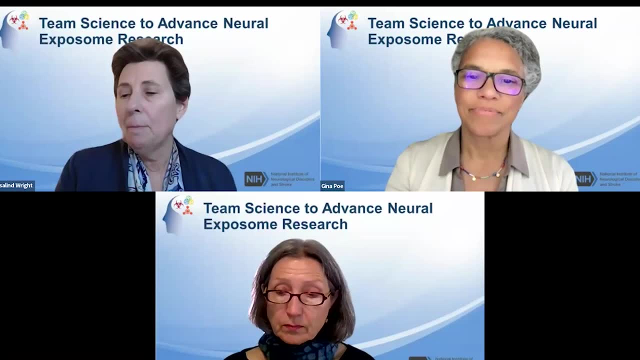 everybody touched a piece of it, Cause we see how big it is. It's been exemplified in the presentations today. Everybody gave us a piece of it And I'm like, well, now I need to go back and give some part of it, big parts of it, But I liked that Dr Bennett got to. we need to go from. 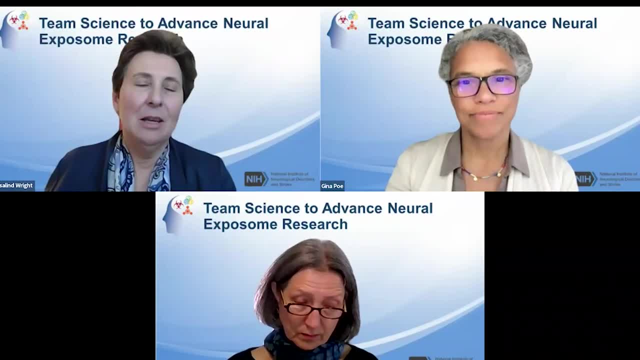 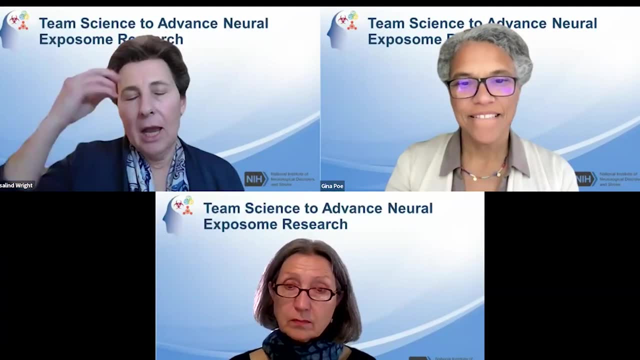 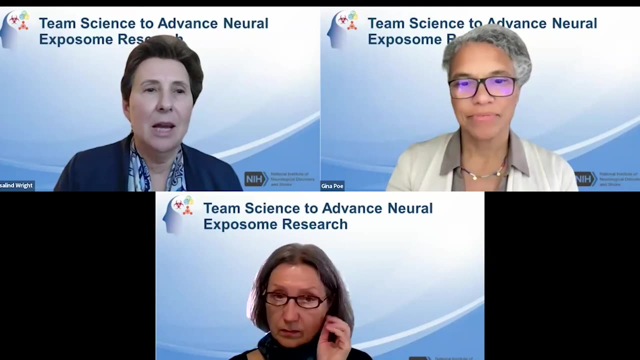 interdisciplinary to transdisciplinary teams. We need to be training our scientists to do that. And- and I want to make a shout out to the other hat I wear at Mount Sinai as I lead our CTSA, our clinical translational science award, which is supported through NCATS, the National Center- 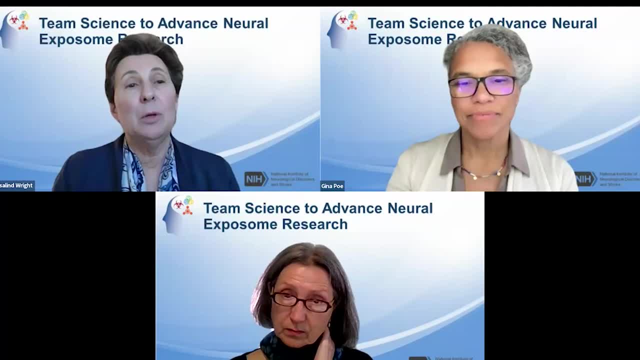 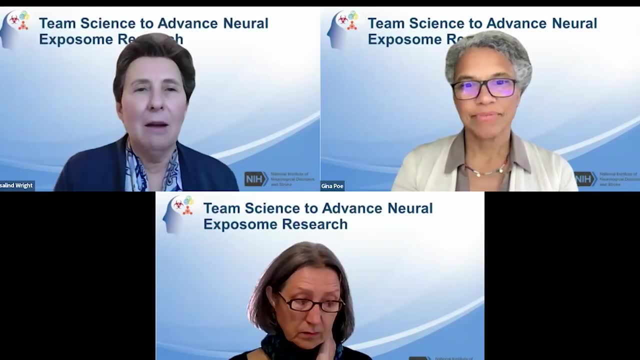 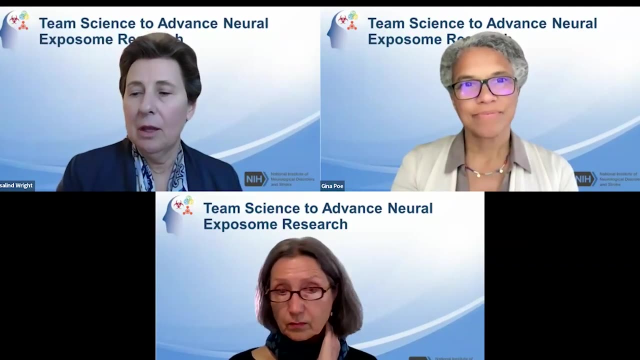 for Advancing Translational Science And it is the science of doing translational science and they're big on team science And that's we that they should be in this conversation, because we do need to train that next generation And- and that really struck me particularly with 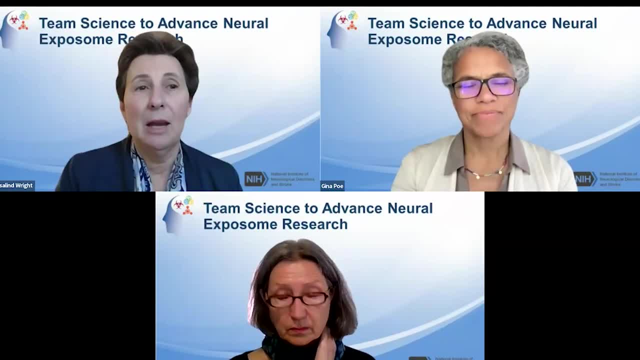 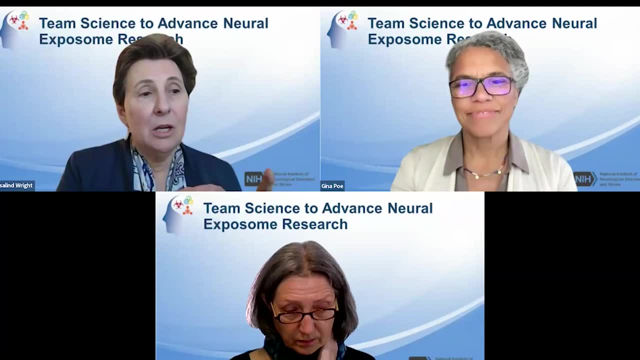 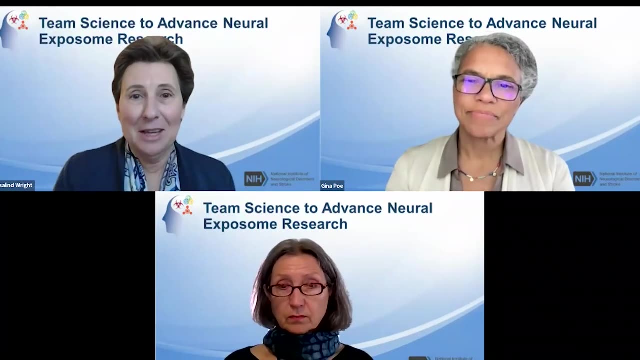 Dr Lee's talk and then Dr Bennett's talk who I think brought that right back to it. I do this because I know I, I, your reduction is you get only so far. That's important part of science. It absolutely is a part of even team science, right? And 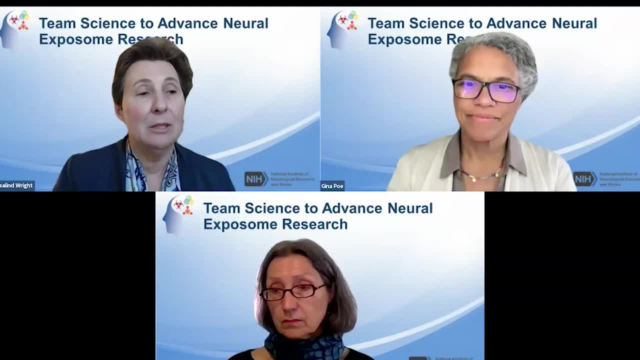 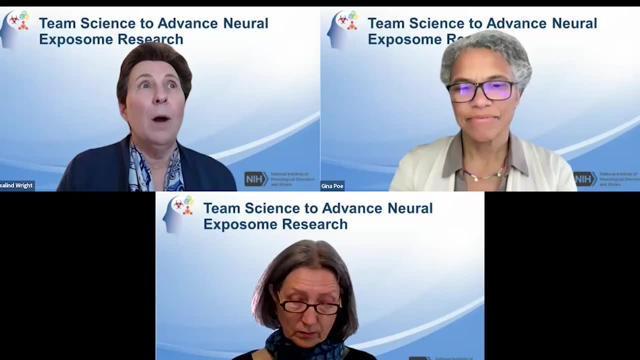 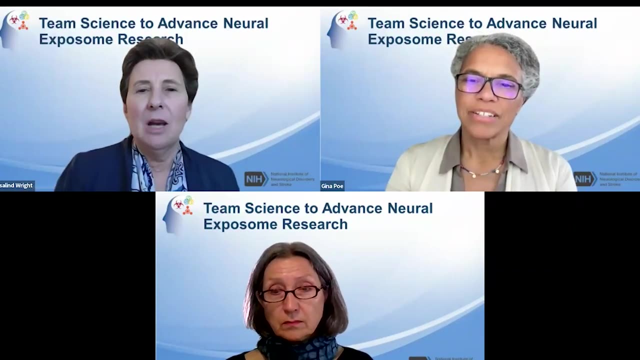 and the, the exposomics. we, we do need to drill down at different times, but I, I'm, I do team science And as I discovered that, wow, if I really opened myself up and talked to this person, that I never imagined we'd have anything, you know, maybe scientifically to do together And 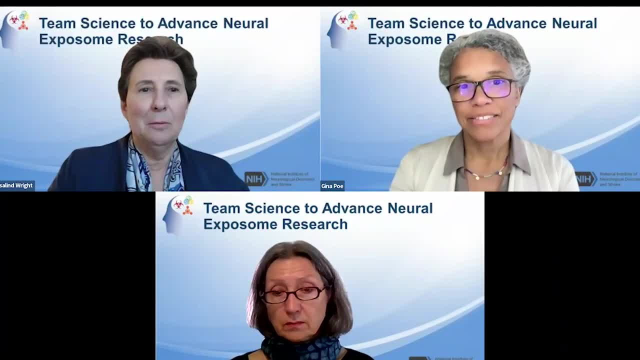 you, you like the spinal cord injury where he talked to the- you know those, the two different people- and brought them together to do drug discovery. I thought that was a great example of it, And so when you get bit by that, you're like, okay, this is, this, is the way to do it, This. 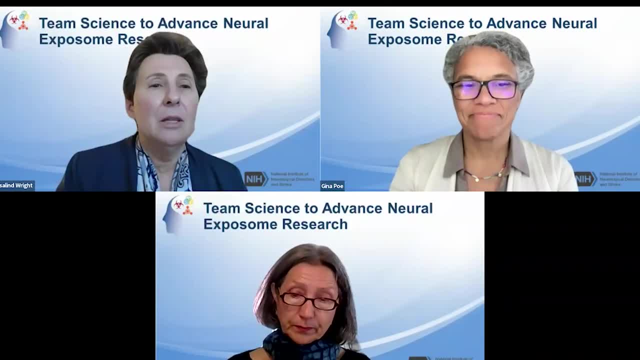 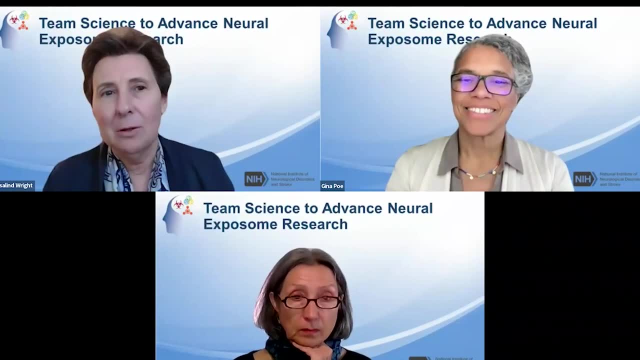 is the way to tackle these big hairy problems And and nothing's bigger than exposomics. And then you look at the complexity of the neuro, the. you know neurodevelopment, and then you got to have life course theory in there. You know you need to know when and, and you know 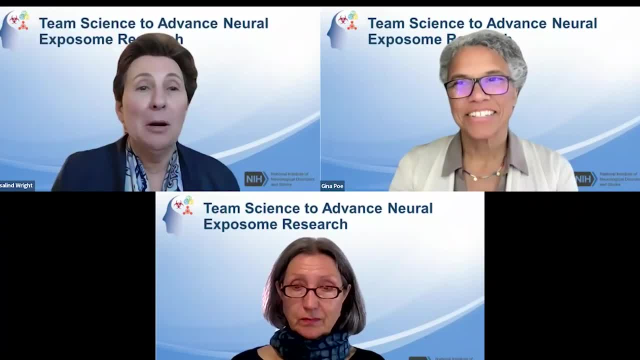 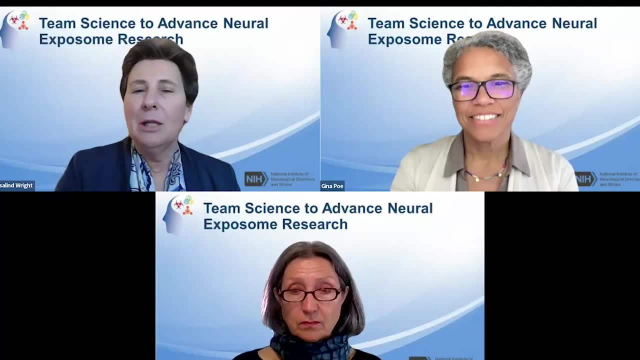 in the life stage to me, that's, I want to be a part of that, any part of that, And, and you, you can light up the, you know, junior people coming into this and everything else, once you know you're going to be able to do that. 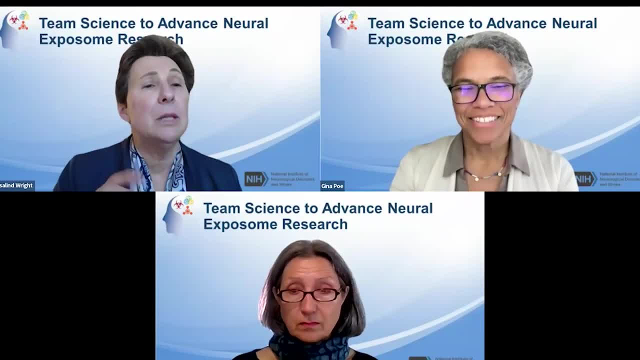 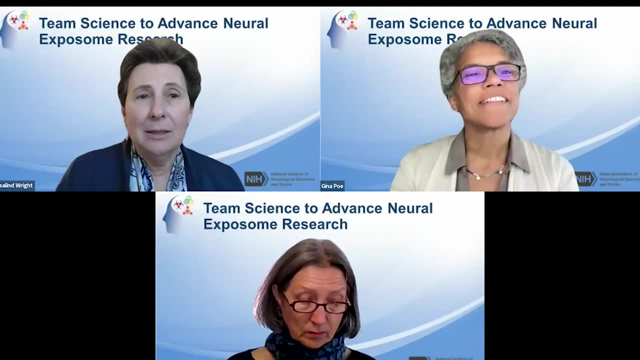 You see that you can do something bigger together and support each other. be transparent. Lots of the things that were said just practically you know. set these things up early on right. Come to some consensus of how you're going to run this thing. That's so important. I totally agree. 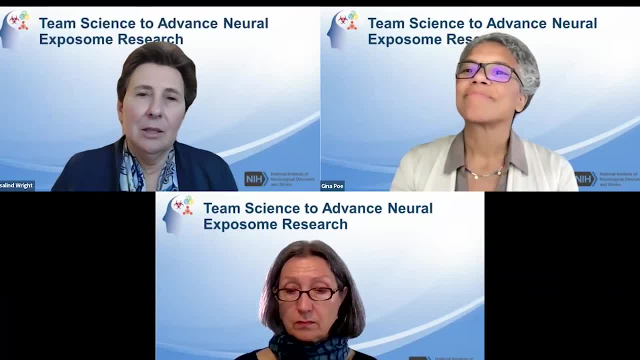 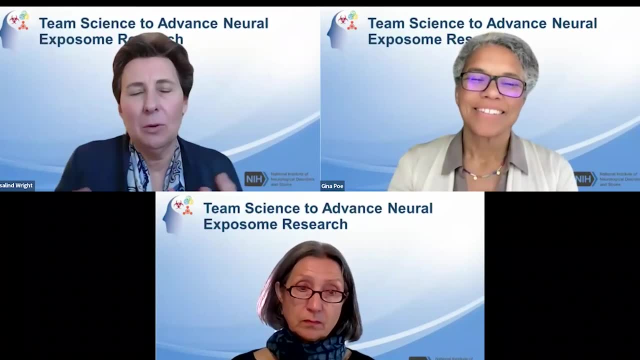 because we've all done it the other way And and then you have to expend your energy fixing it, and you don't want to. you want to keep moving. That's what I would say. That's what I've gotten out I've. I was looking forward to the talks, but it was even more important to me. 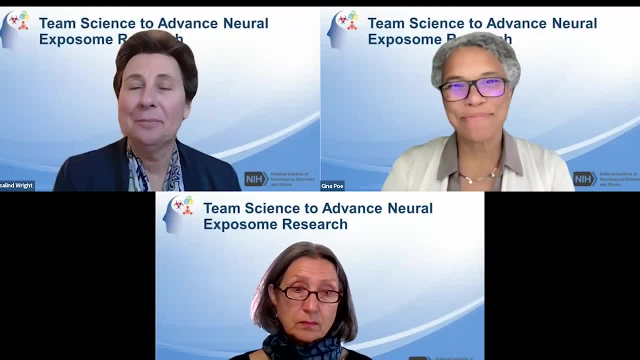 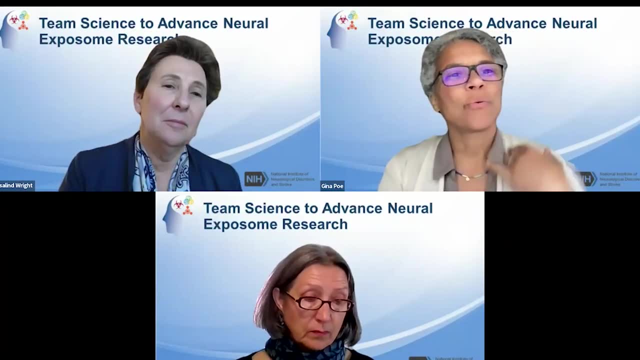 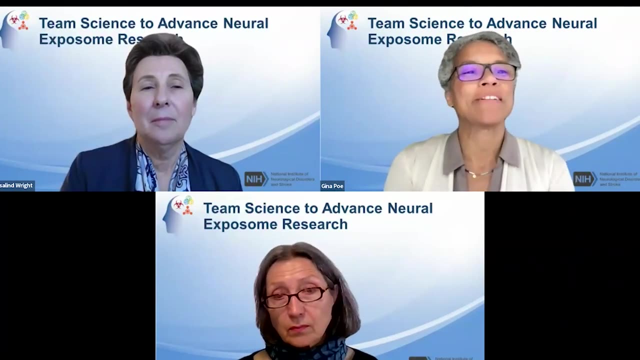 Better than I anticipated. I agree a hundred percent, Which you know. some of the things that you were saying leads us to my second big question, which is: you know what are the really biggest challenges for developing team science in this neuro exposome research environment, and how? 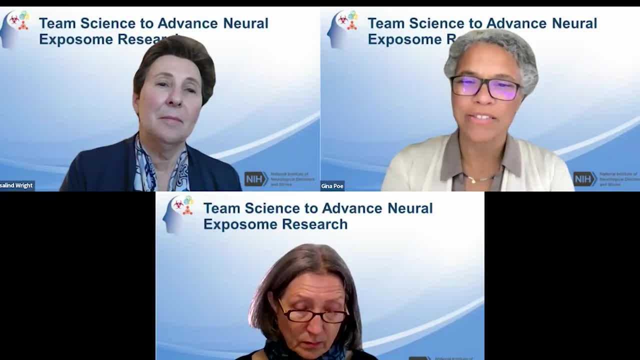 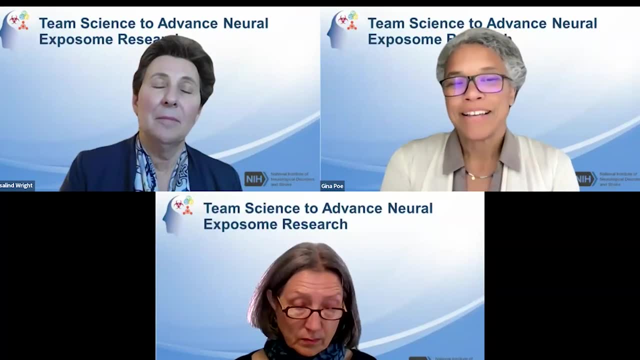 can they be addressed? And I think it was addressed in a lot of the different talks, various things, but there are still lots of other challenges, things that you might not expect to run into. For example, you know great to use Slack, but Slack has changed its funding platform and now it's really expensive. 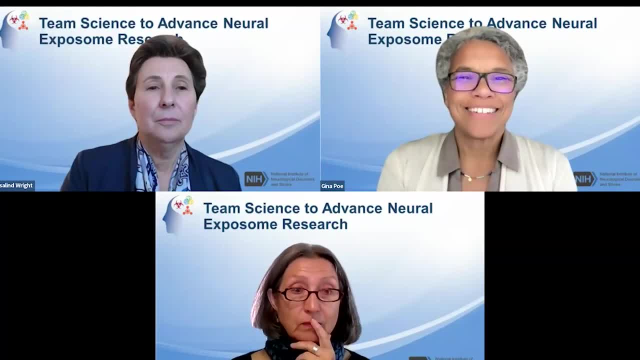 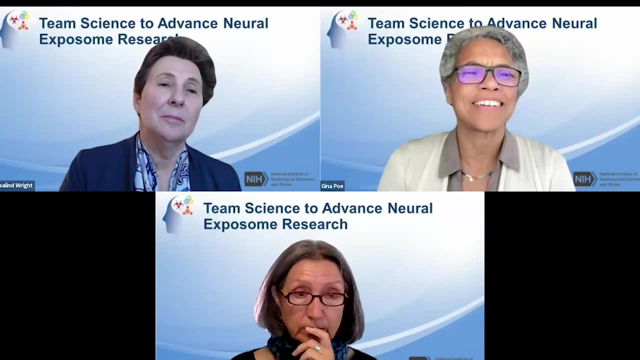 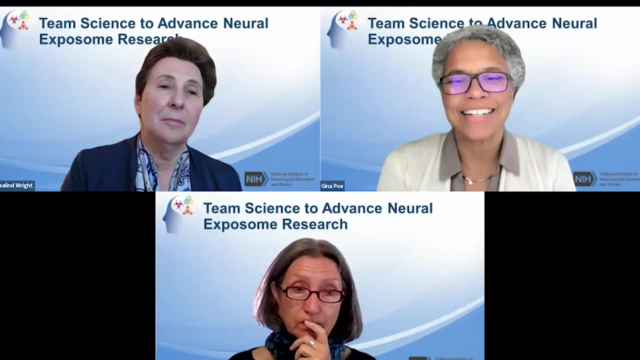 They charge a lot of money for each person And and if you try and make one institution responsible for the Slack, then you know it's just login issues, all kinds of things that could happen. So in your minds, both of you, Hannah, what are the biggest challenges and and how could? 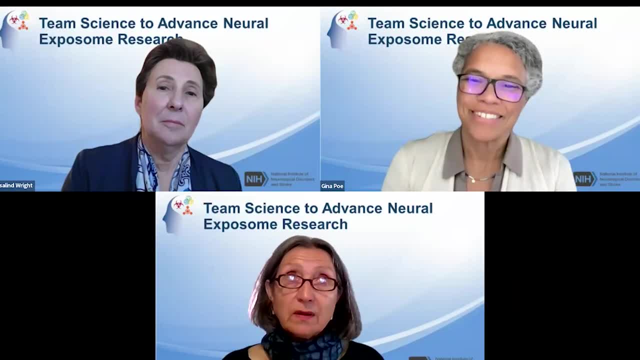 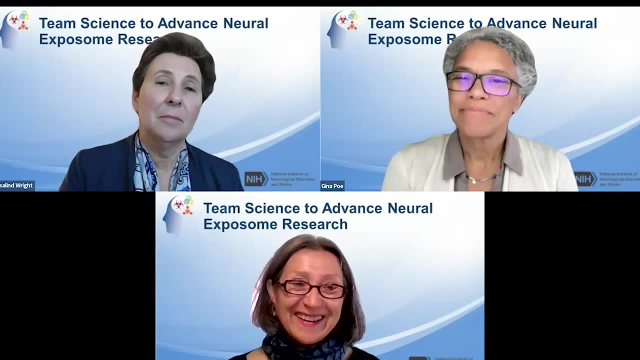 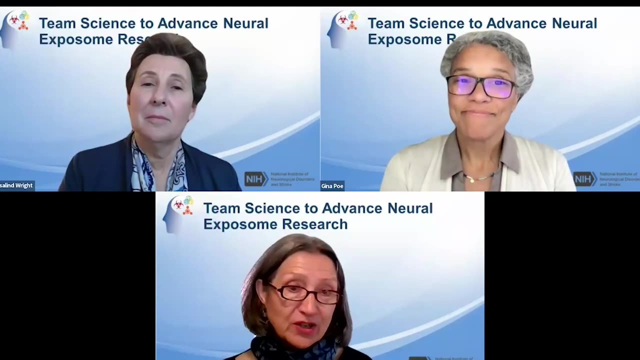 they be addressed and how can we do this together? Yeah, So I have a feeling the biggest challenge is to actually find the team members, And you know somebody said: bring a friend, but you know that might not be the right person for the project and 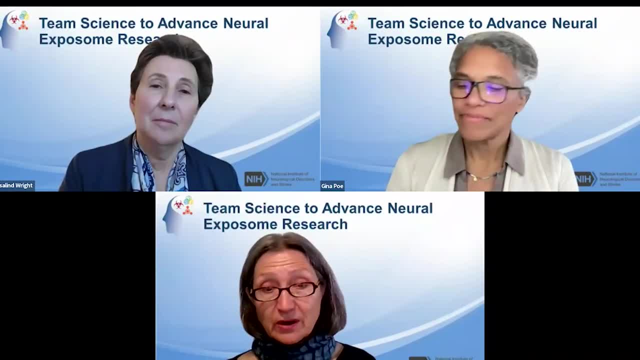 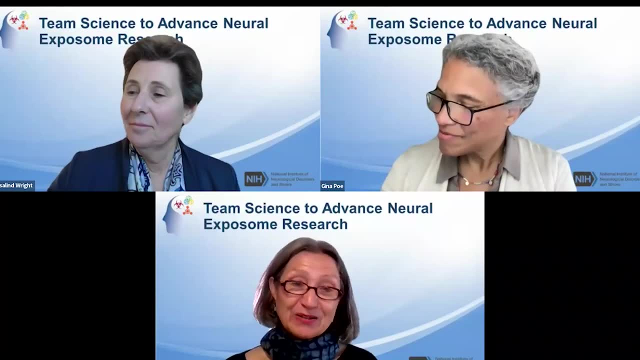 the question I'm asking. And then I'm asking a question and I know which expert I need, but I can't find that person, or that person doesn't want to work with me or, you know, just doesn't like population science and doesn't see a role for them in what we are doing, or is. 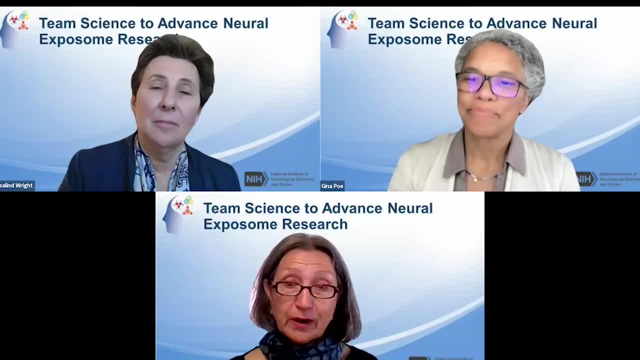 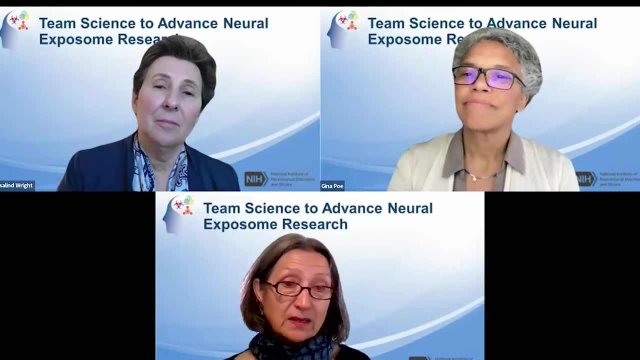 expecting something, And I think that's a big challenge. And I think that's a big challenge. That's really not something that from us that we cannot deliver, And if you, if you just look around the room at your institution or you know your friends at your other institutions, that you get to. 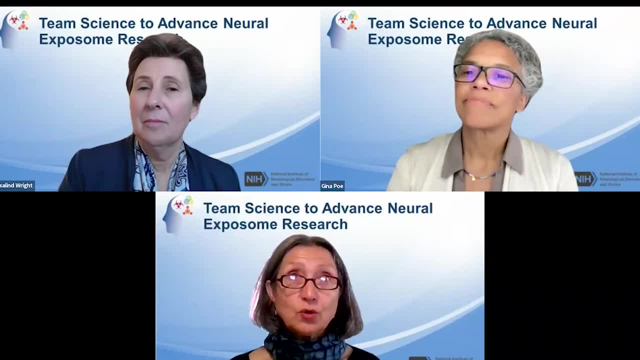 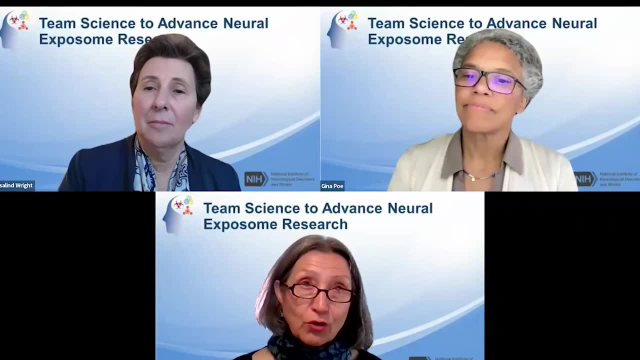 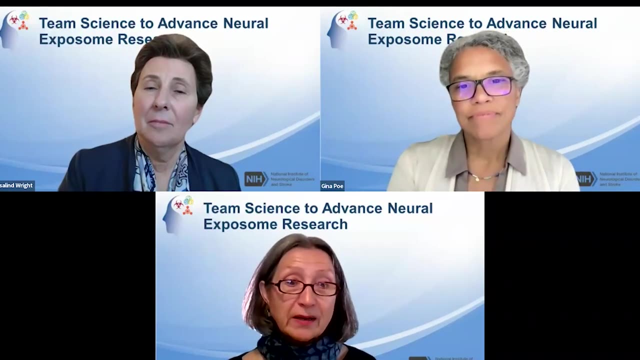 know it, maybe some conferences you kind of stay too close within your discipline many times, or too close to your discipline um to really reach across um departments and across disciplines. Yeah, hard And I've seen it work a few times, especially when you have a strong leadership. 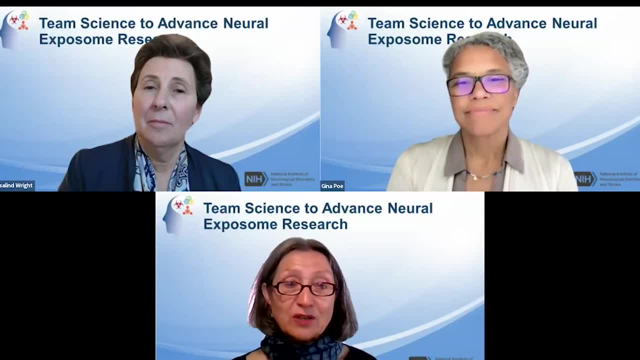 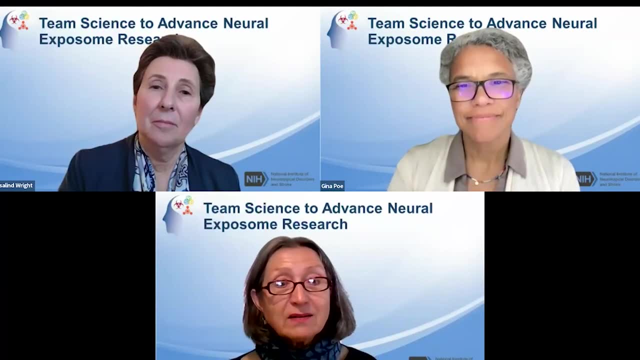 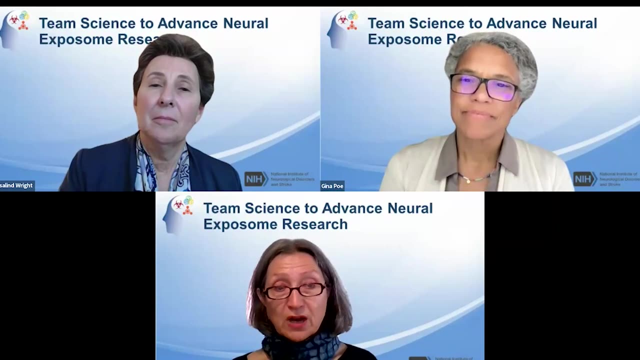 who believes in team science and reaches out to members of different departments- That's what happened to me at UCLA- And then you get a feeling for how you can integrate over the years. So the other real challenge is: how does that team then grow together? And it's through many, many meetings. 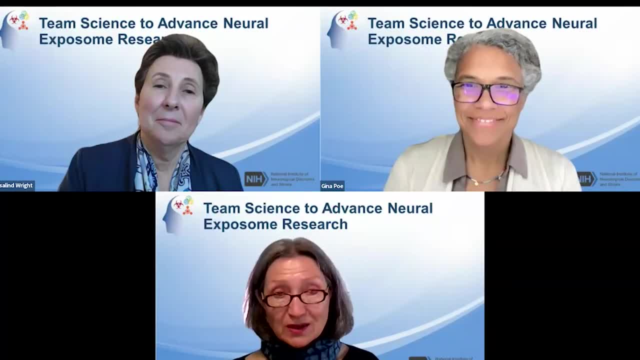 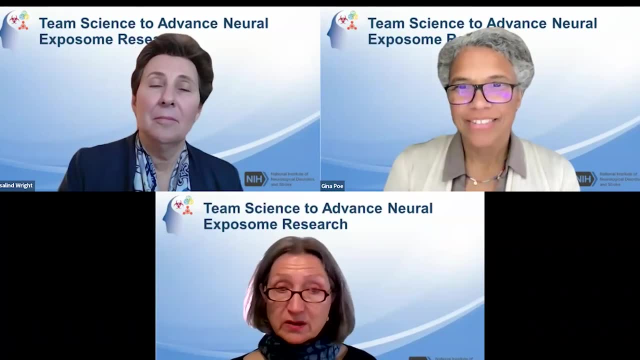 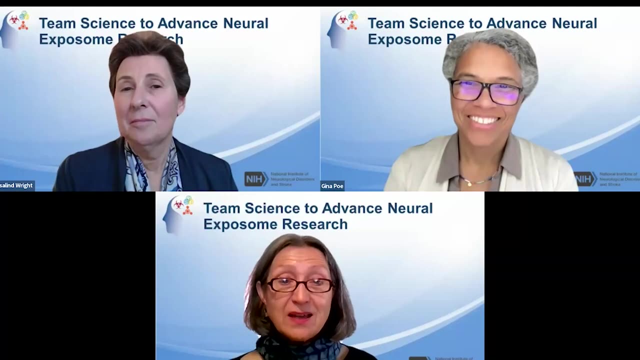 where you're forced to be there And you're forced to sit through two hours of some people talking about things where 80% of the time, you don't understand what they're saying- And I mean it, you know, And it's a real challenge- And in the end you find out well, that 20% is really. 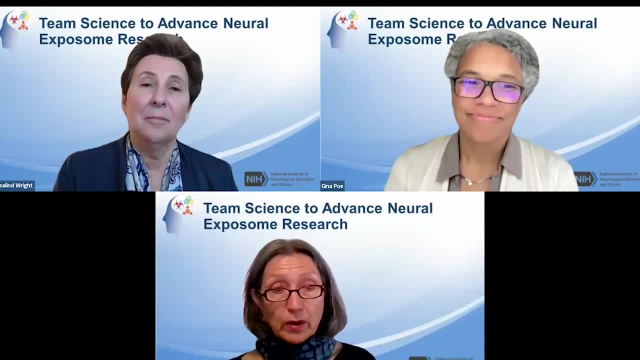 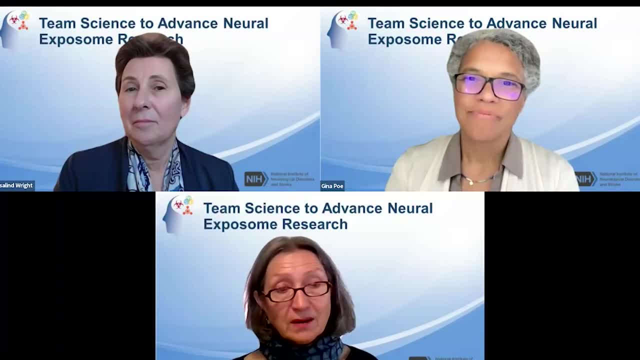 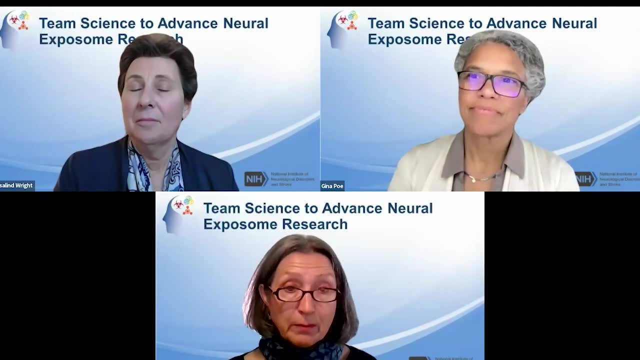 you know, keeps moving towards it. So it's: yeah, it's partially in the leadership, It's partially in the respect of the leadership for each team member And of finding also a place for each team member to express themselves and to feel valued and to bring the best to the team that they. 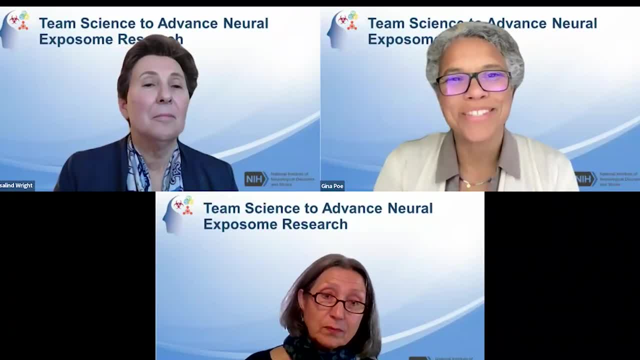 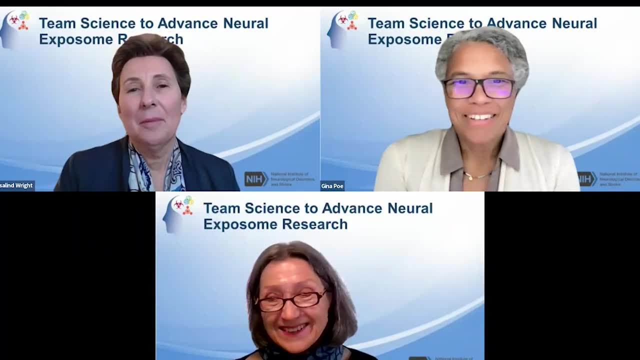 actually have, And I think that's a really important thing And I think that's a really awesome. Is there a way to reduce the 80% of the time you don't understand what someone's talking about? I mean, can you try and do a translation thing at the beginning when I say: 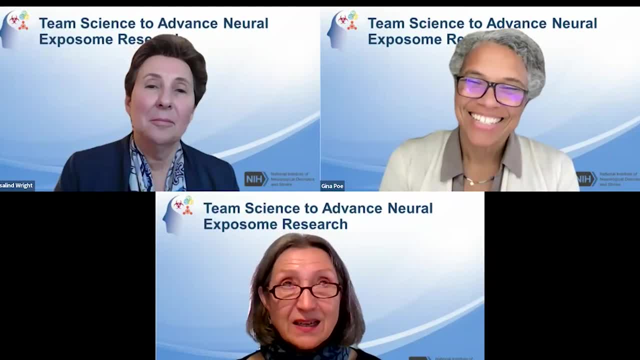 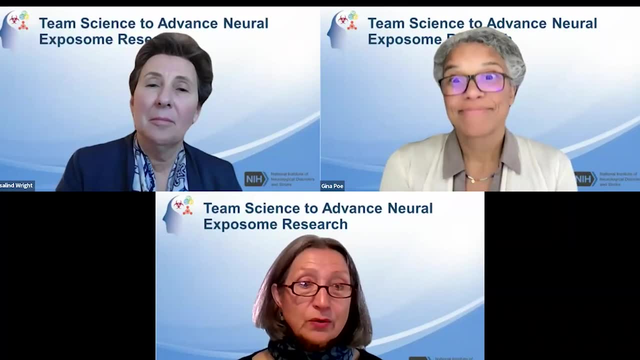 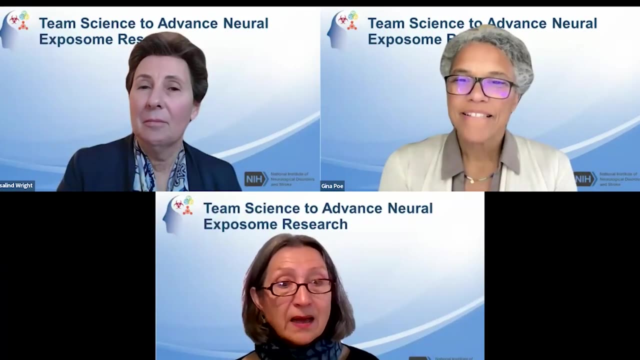 this. I mean that, Yes, it's, I think. I think it gets better when we remind ourselves not to use acronyms and to actually try to talk in a way that you know you talk to a lay, lay, educated audience And that's actually a great skill to develop because it also helps me. 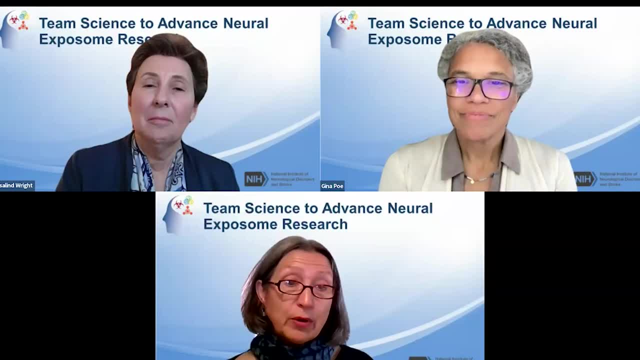 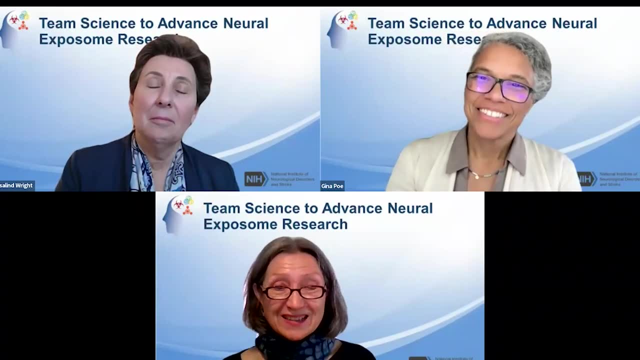 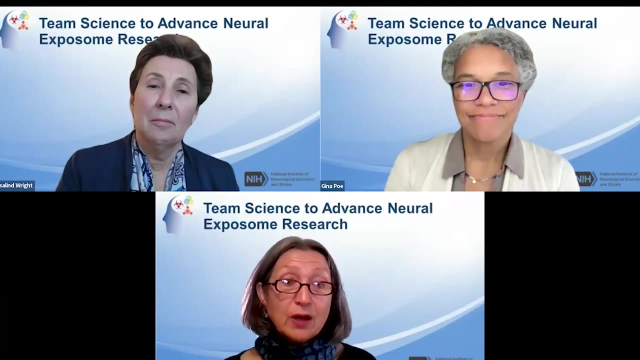 when I go outside of academia to actually tell politicians or journalists or anybody who wants to listen to me what I have to say about my science. So I think that's another real positive of this team science approach. You actually learn to talk to somebody who is educated enough, so you 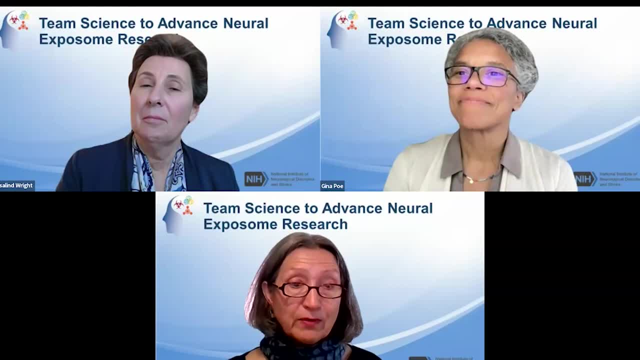 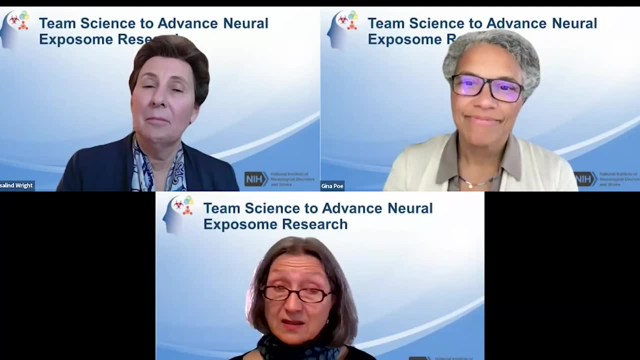 don't have to give all the principles, but you talk In a type of language that translates to what the other person already knows, And you know, and I think that's that's also a great value. Fantastic, Rosalyn. 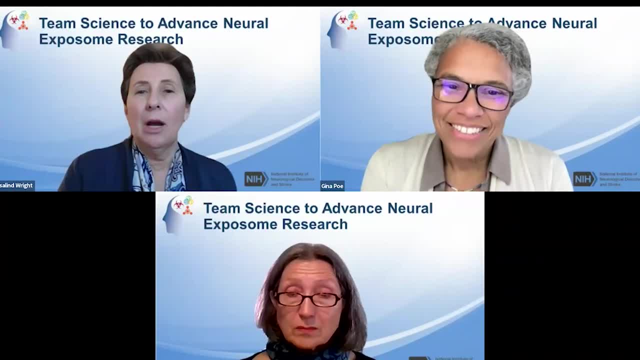 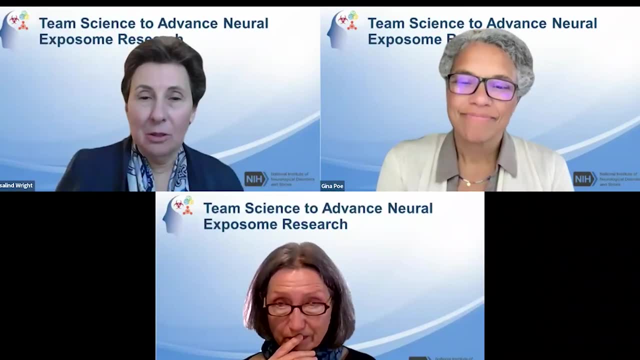 I think too- I'm just to you know what you described, um it or happening organically. like you're, you continue to reach out and broaden your exposure to these different things within your own institution, within across institutions. you know meetings like this. 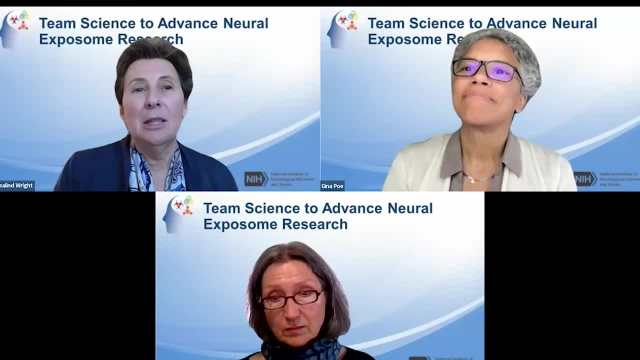 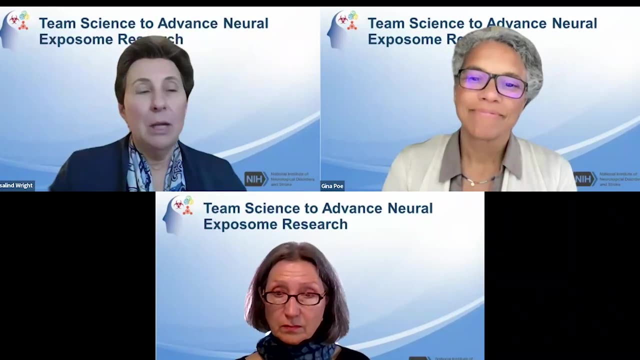 or or where we bring together disparate people to to sort of hear and start to think about how how do we implement this? you know, and, and people who've been successful. um, what are the big questions we're facing? And and and people start to meet, the more we can do this. 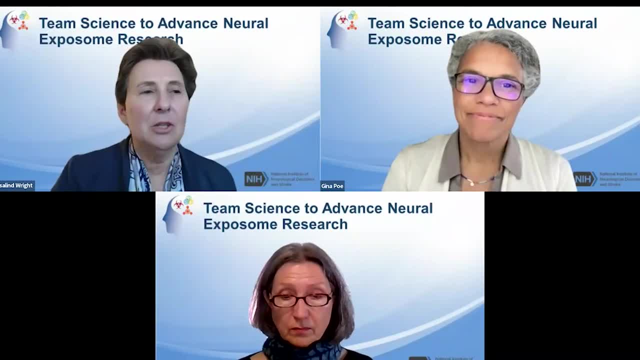 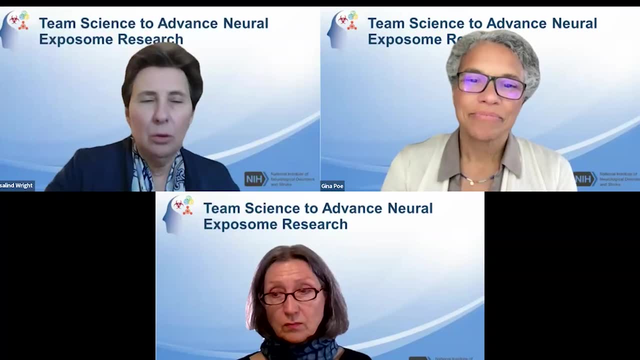 the more the funder- you know NIH, other organizations, NSF- brings us together to do this, have these kinds of conversations. It accelerates that Um beyond what you, you yourself, can do. That's always was very frustrating to me early on when I 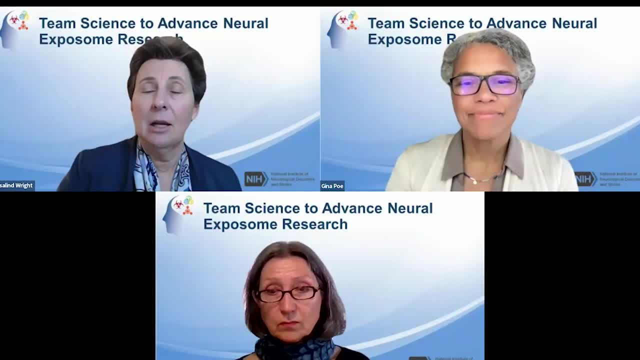 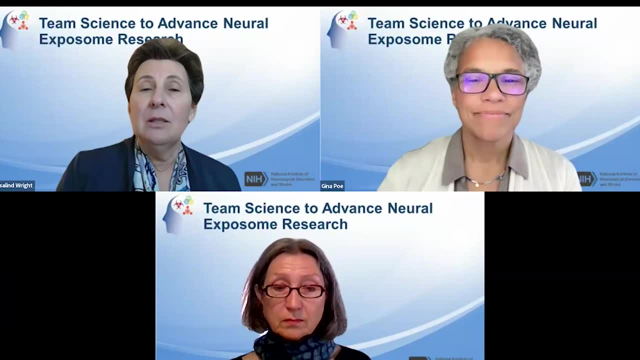 wasn't maybe a part of these. So I think somebody has said it a couple of times here: bring the junior people into these conversations as early as possible, because it is frustrating: until you've established yourself a little bit, you don't get in the room. So the sooner we get in the room, 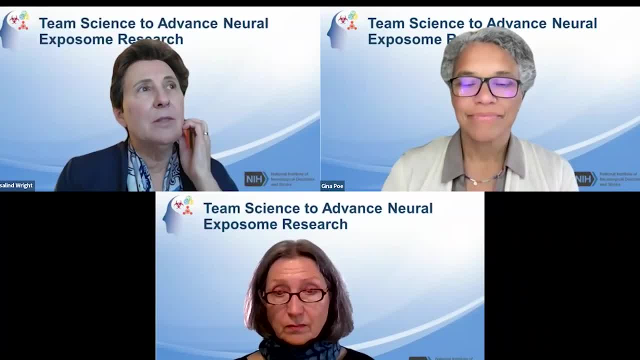 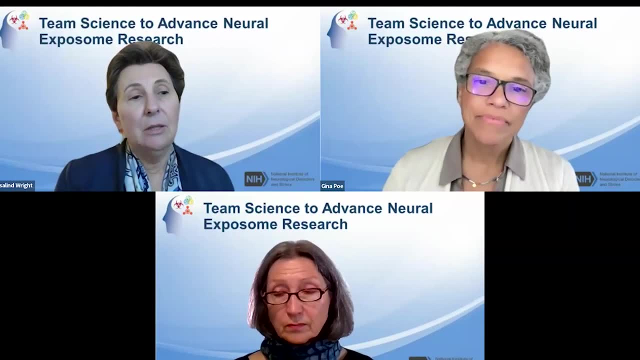 together, the faster this can go Um. the other thing I would say, and it's come up here a couple of times as well: I think it's absolutely essential That we have to bake this into the ecosystem of every academic um research Institute. 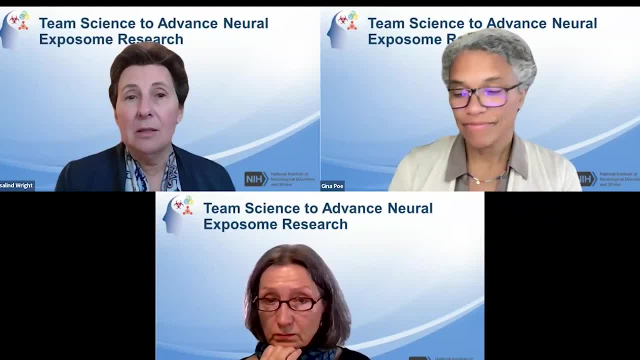 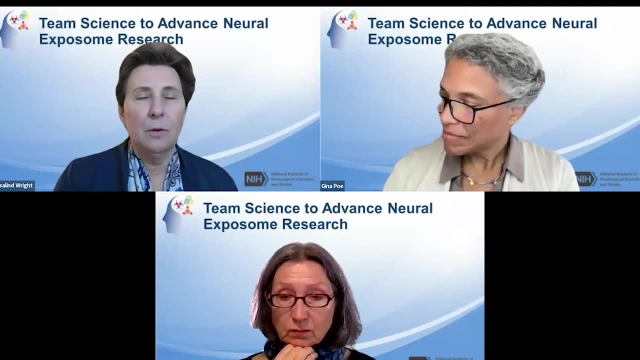 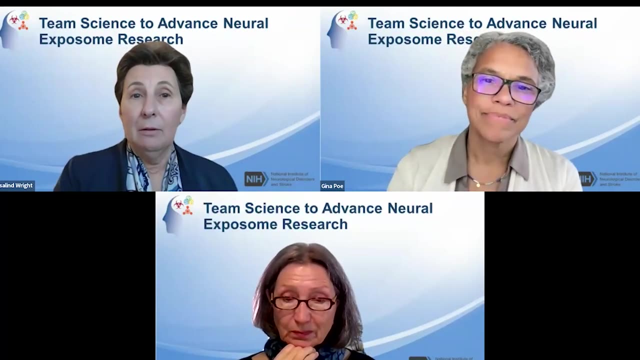 institution, medical center, whatever. that team science is where we're going for some of these issues and that people get credit for team science And it's not if you're just first or last author or, you know, communicating multi PI or not. Um, and we've come a long way. 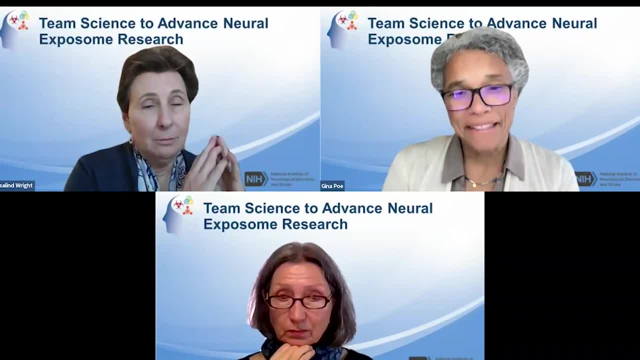 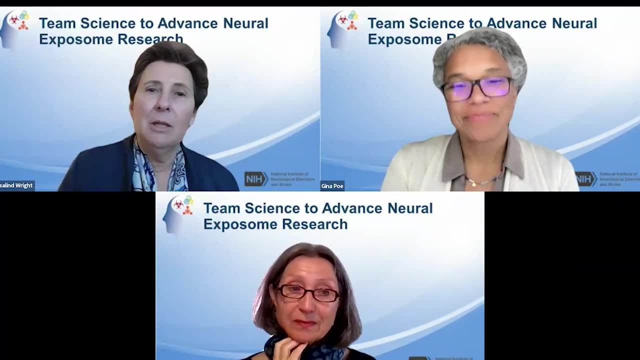 from what used to be that was said to me. you know, just outright: if you're not first or last, don't give a minute to you. know things like this I heard along the way. I mean crazy Cause. 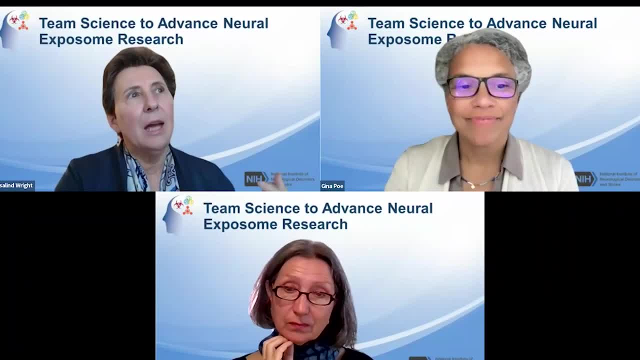 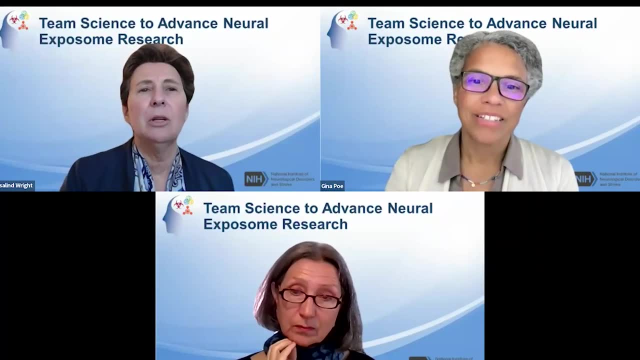 and then you start seeing the value of team science. Well, that has to change right, Um, culturally at across this, And I think we're we're moving in that direction. What we'll do, it is, when NIH and other funding organizations do these kinds of things, you're going. 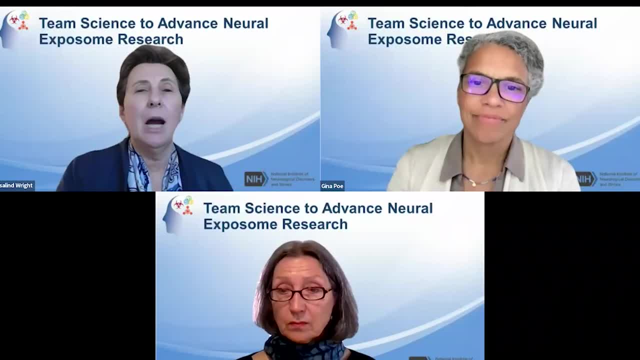 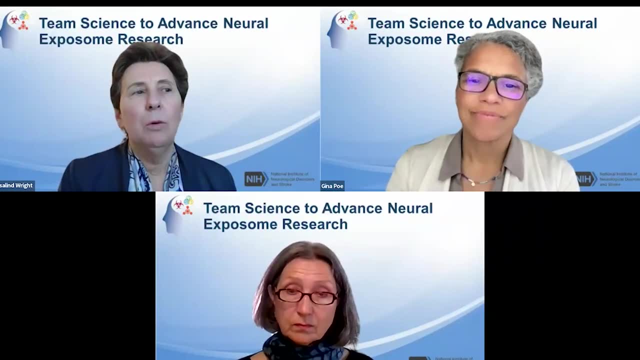 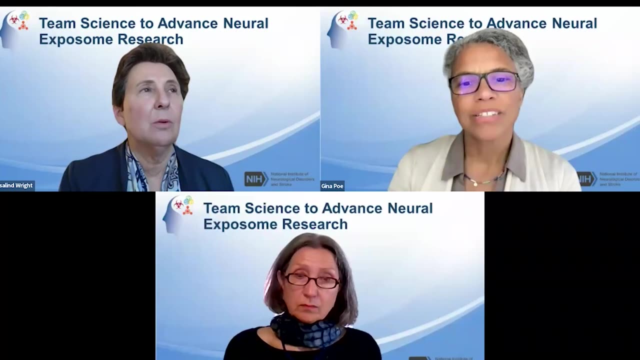 you're funded as this. you highlight it- Multi PIs adds value. The this has been. these are um critical things when we in our promotions committees, where I am at my institution- it's the first institution I've been at where it's just. 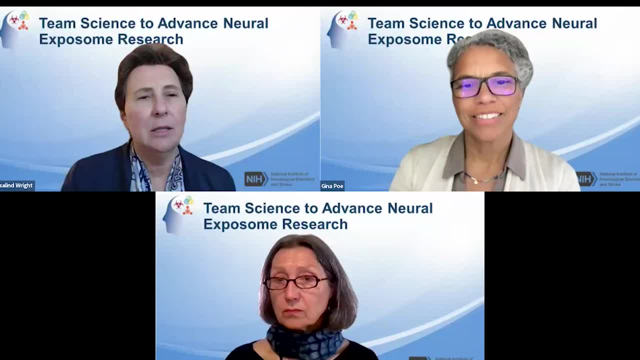 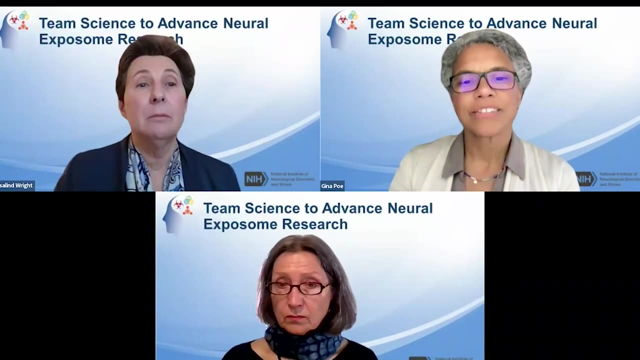 really written right in their team science. You can annotate your bibliography. maybe your your co-author, you know co-first, co-last, but also annotate: Why are you important? Someone brought up? should we be? does the someone who builds the data infrastructure warrant? 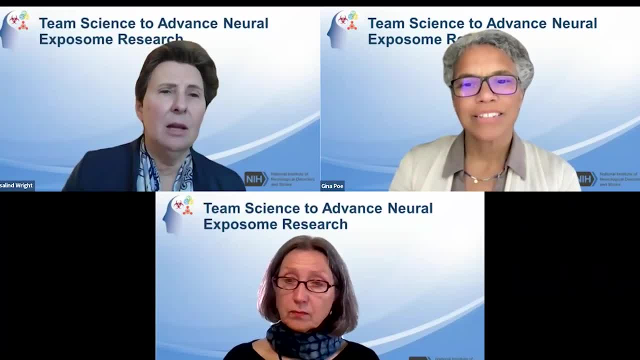 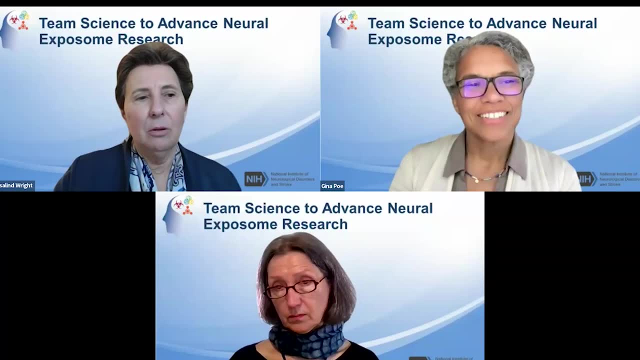 warrant um authorship. There was a time where you didn't think that that. you know that's their job. Boy, I feel very I couldn't do this work and pull all this data together and wrangle this data and harmonize this data, et cetera. Those people are are co-authors and 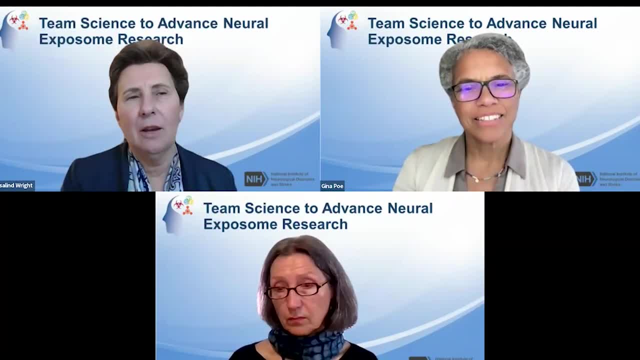 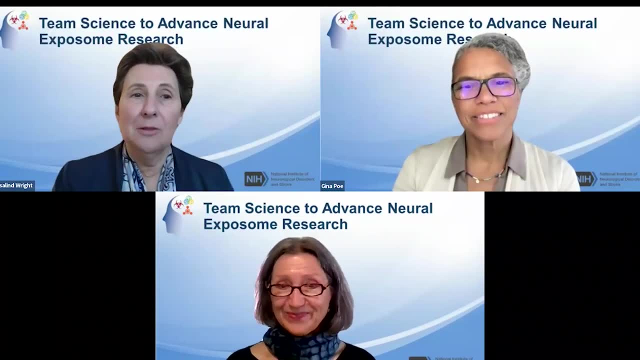 they're critical to having it And you know you do it in different ways. You have mastheads or what have you, you, but you, you write those things out and people have said that. right, This is our rules of engagement And that takes. 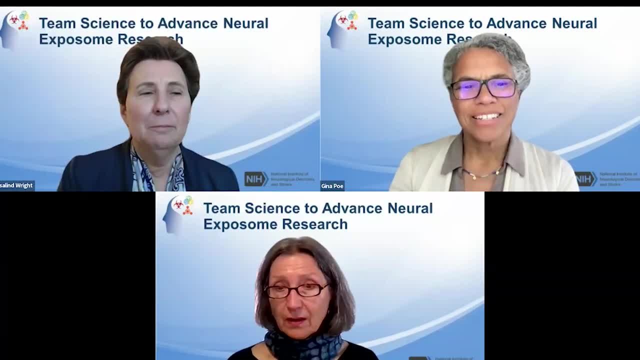 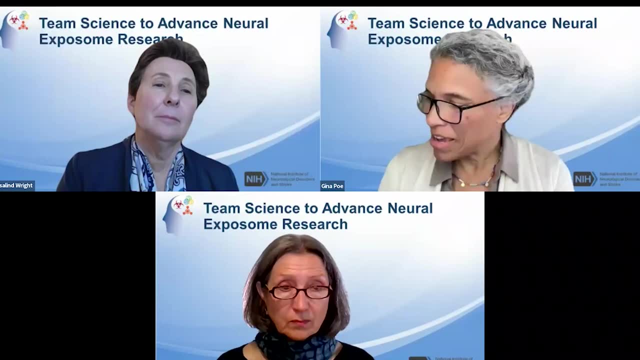 it takes extra time, but it's so valuable in the long run. Yeah, You guys have both mentioned something that it's really near and dear to my heart, which is, you know, letting junior people in the room and um and the problems and. 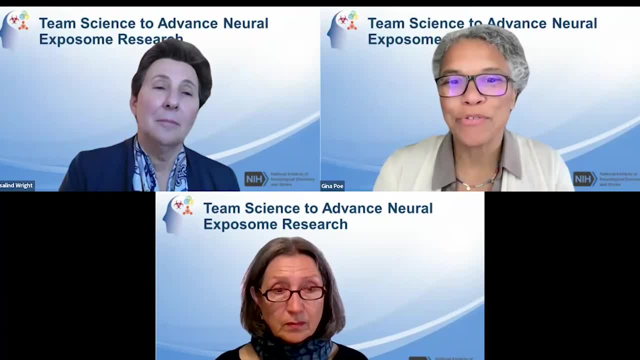 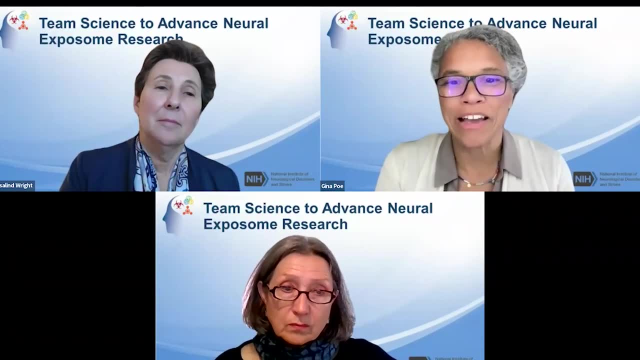 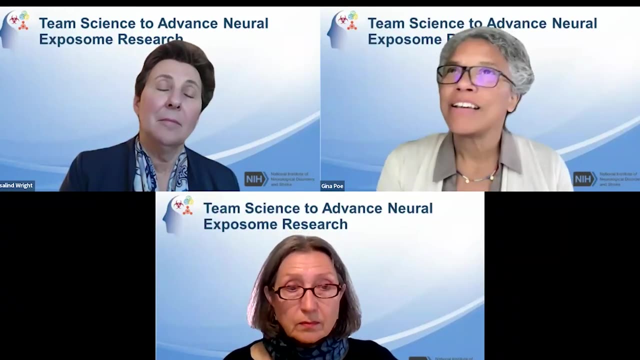 um, the good parts about the bring a friend kind of way of diversifying, and that is, diversifying the voices that are involved in solving these really difficult, really complex problems. Um, and so letting junior people into the room helps that, um, and then bring a friend- is is great in in terms of an easy way to 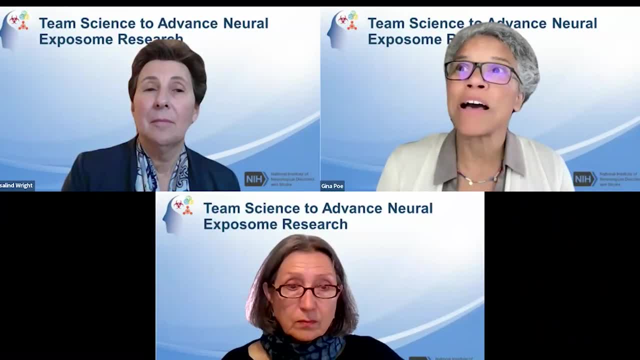 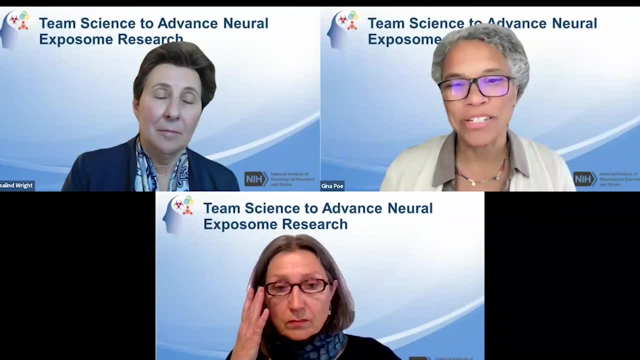 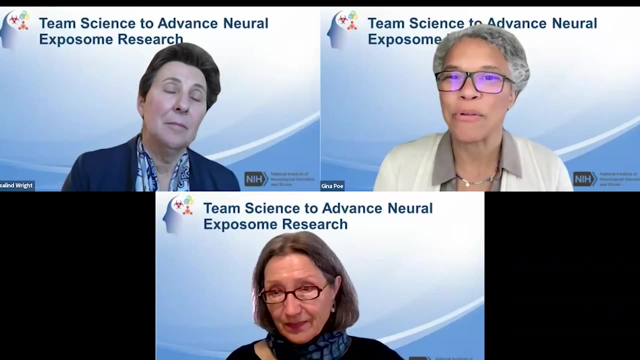 to broaden the team um with trusting people. however, that also can buy into the whole good old boys network and having the same people doing the same things all the time. So what might be another way to to increase diversity in the team, which we all know is healthy? 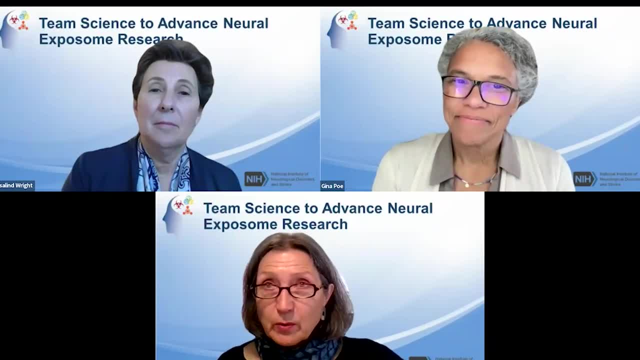 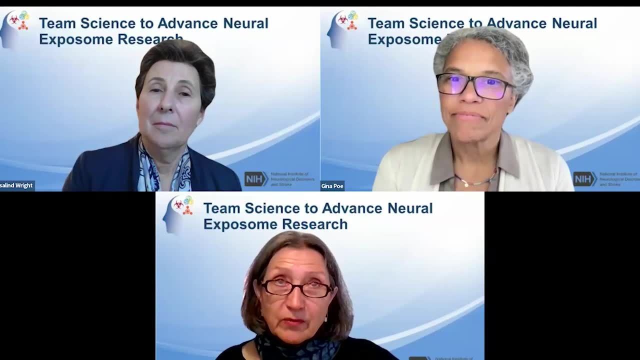 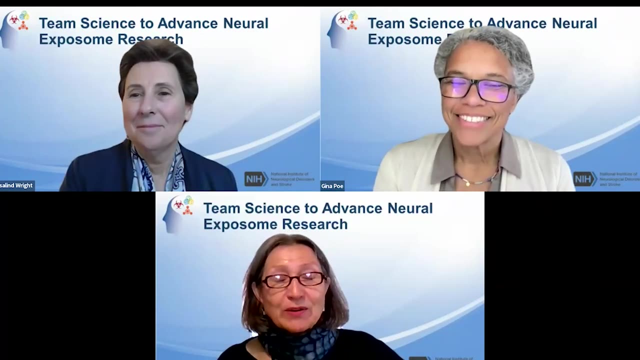 So so what I really found the most helpful when I was part of all these centers were actually the annual meetings where all the different um fundees were getting together- And uh, I see two of them, at least on this call- And what was? 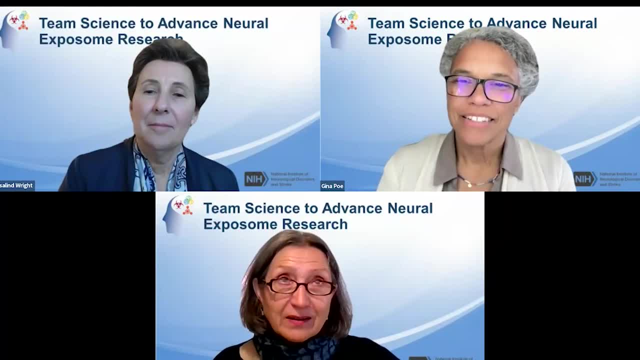 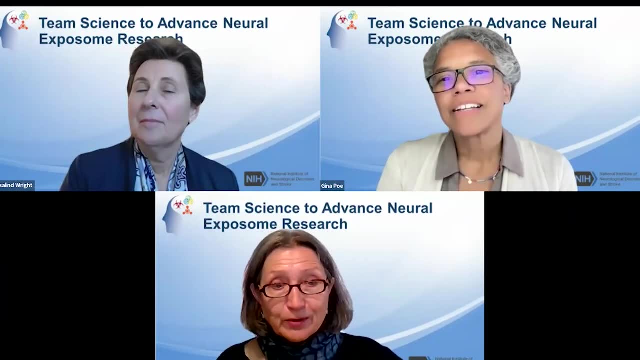 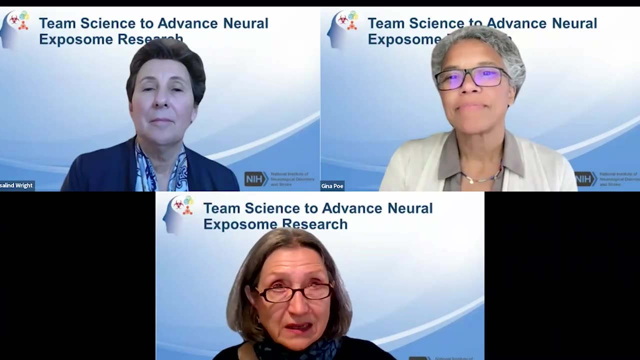 so fantastic was. it was the um, uh- senior people who helped organize it and structure it, but it was really a platform for the junior people to show their research and to socialize and to be to be able to talk to the senior members of other teams in a really comfortable and 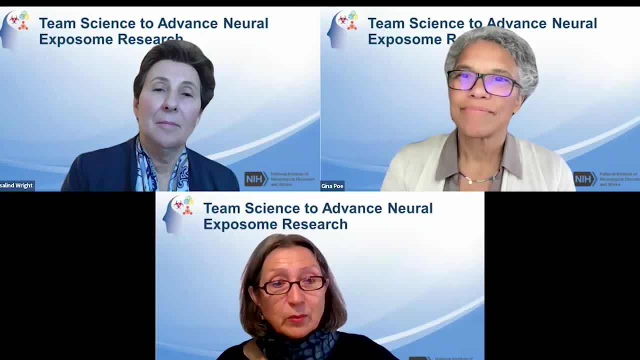 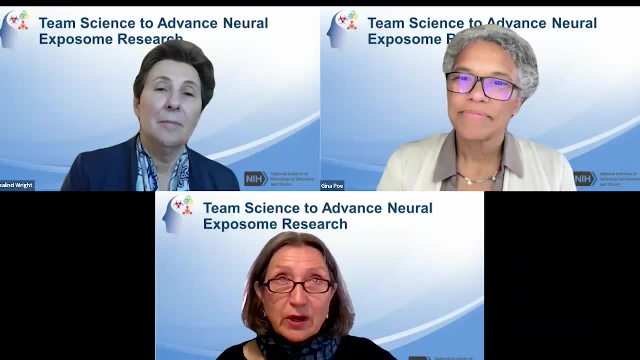 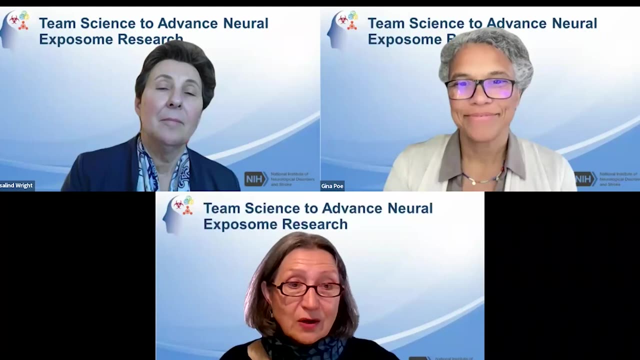 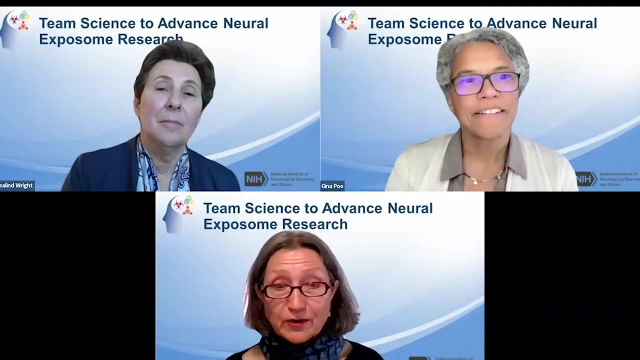 um, yeah, reassuring context, And we were able to build collaborations and um communications that I thought were extremely valuable and unique and really lasted over decades in the end. So, yes, I think these um, these, these environments that you know foster this. Gordon conferences have that a lot. 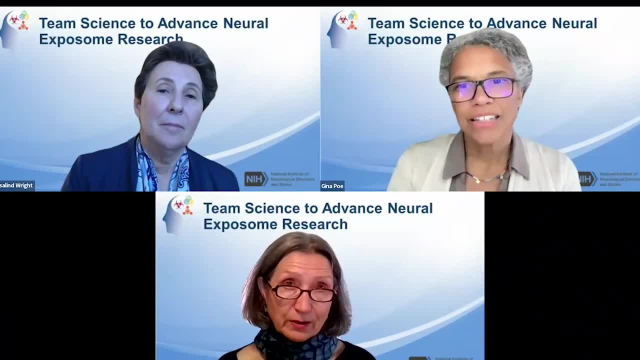 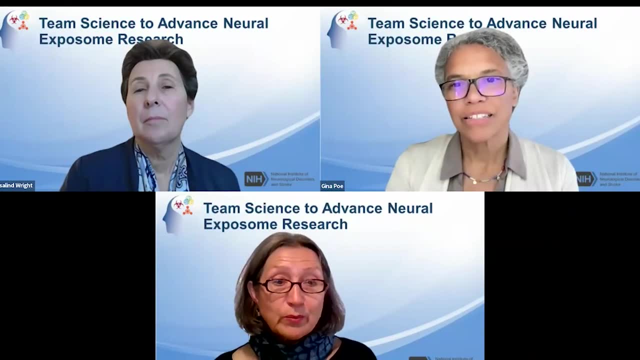 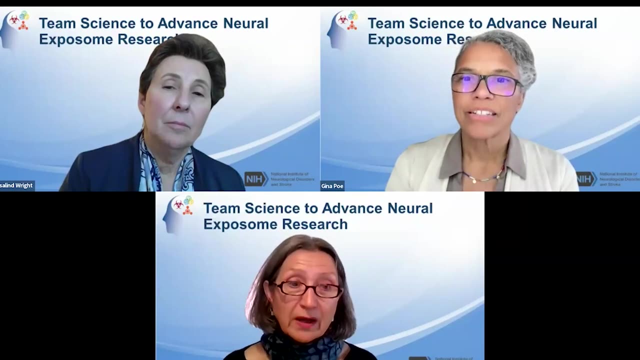 for example, or um, some, some other, um uh, private institutions have these workshops over a week where you know where they bring together seniors and juniors to talk to each other about a theme. I think they're extremely valuable. Yeah, I love that training. Yeah, Go ahead. 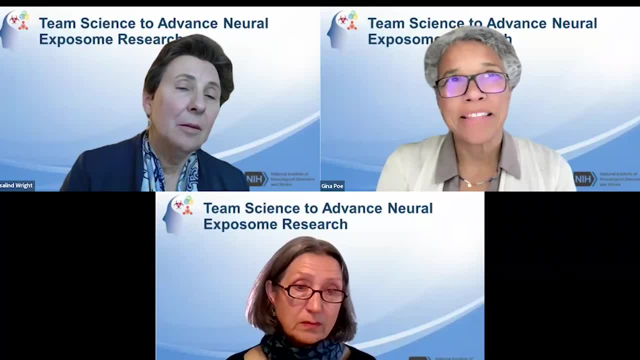 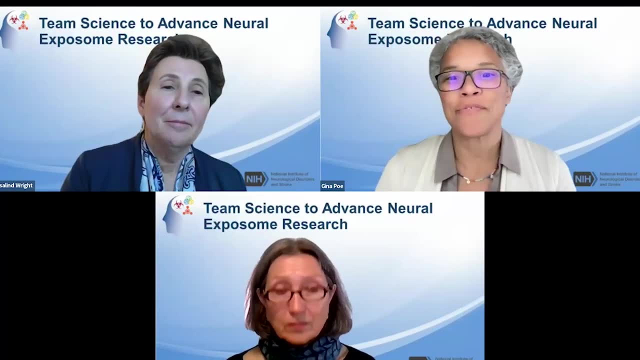 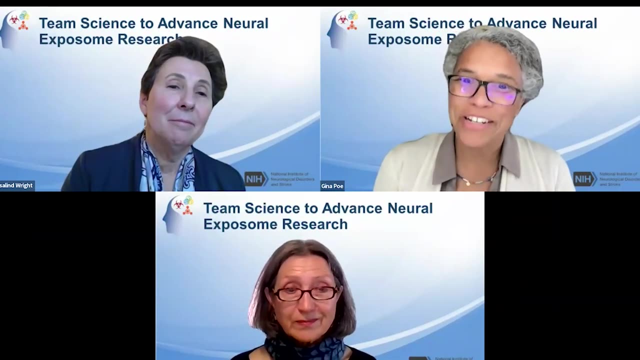 Well, I I also, Rosalind. you said something that was really also very interesting and important, which is the cultural change that needs to happen within institutions to value team science. And, as we all know, culture can change quite slowly, but it could also change quickly given the right impetus. 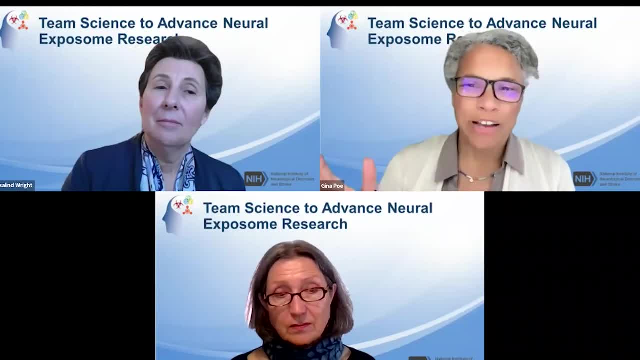 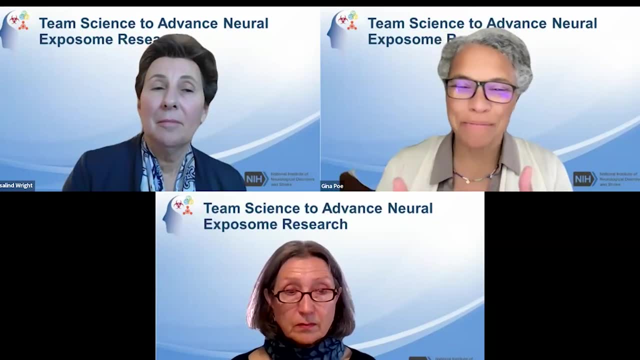 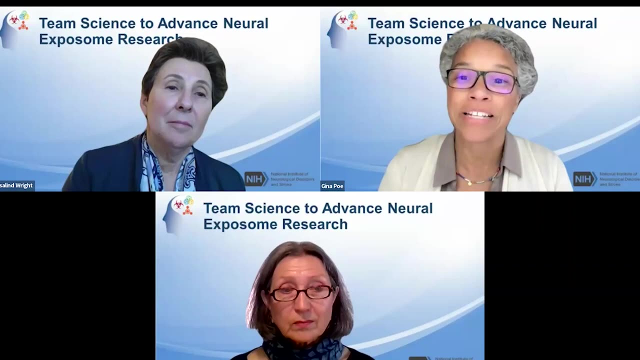 So, and all of these things that you guys are mentioning sort of brings me to the idea that there needs to be a high profile, short, pithy article on best practices and team science. and what's going to move the needle so that we can do this better is 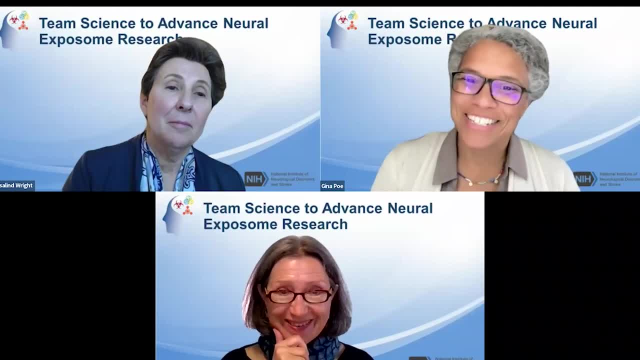 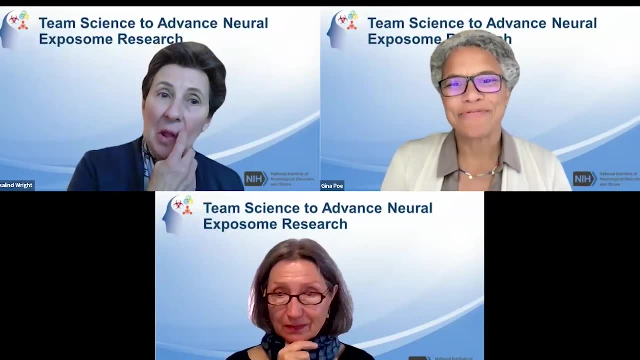 So if we were to write such an article, if someone were to write such an article, what kinds of things would be put in there? What are the best practices, do you think? I mean, we've already mentioned a few of them. 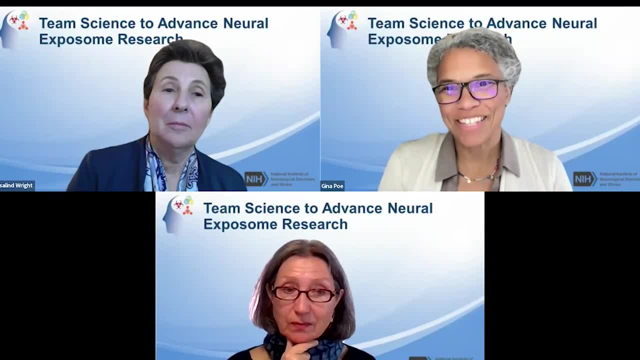 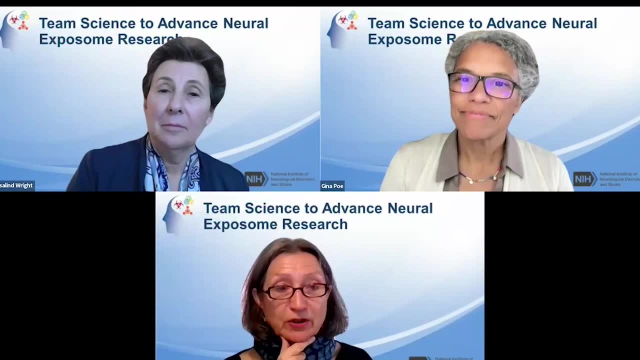 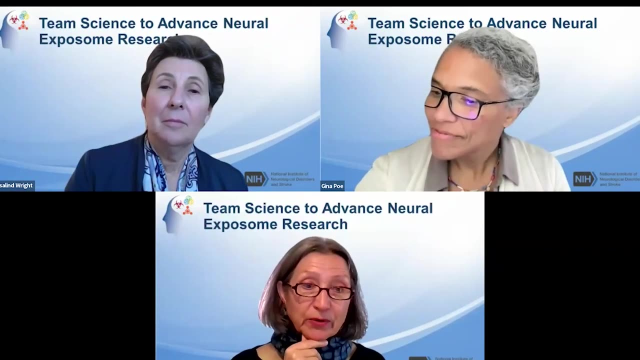 Maybe we can recapitulate them, and I mean say them again. I think we also need to reach out to professional societies to actually pitch this concept, because I now, as a more senior scientist, am asked to write letters and evaluate people six times a day. 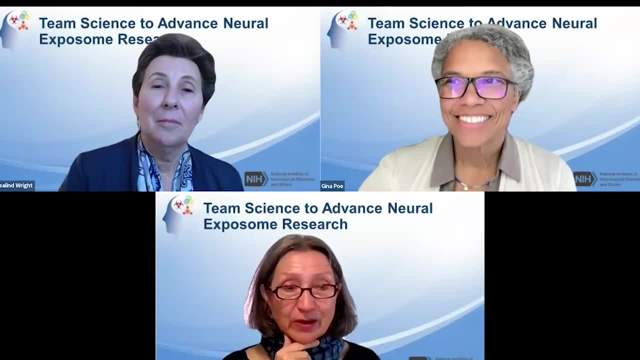 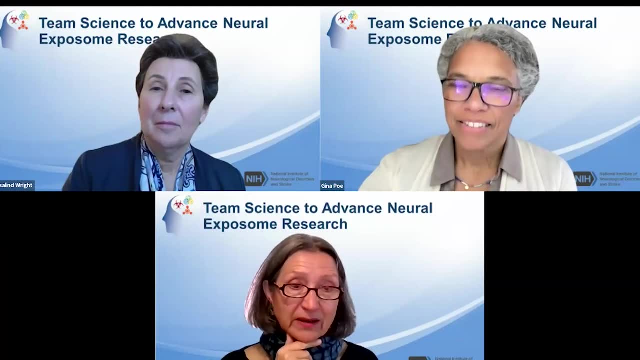 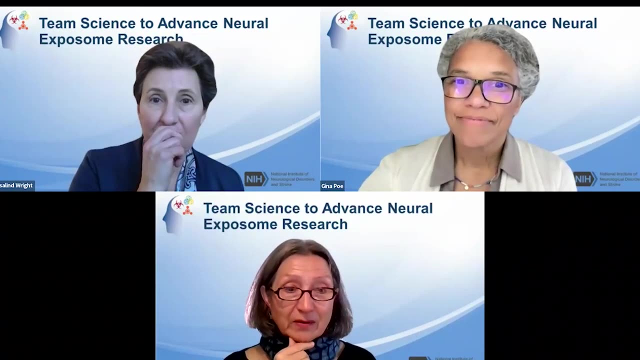 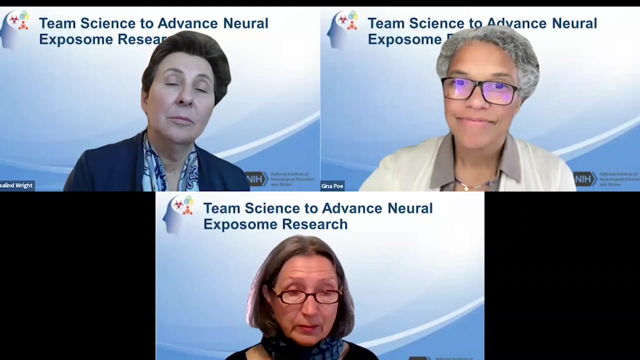 I don't know, but you know, and I have my criteria And I usually look for This team science aspect And I make a big deal that it's not just first and last authorship when we are looking at leaders or team members that we need to. actually, you know, I try to figure out what it is that this person contributes. that is a team science aspect. 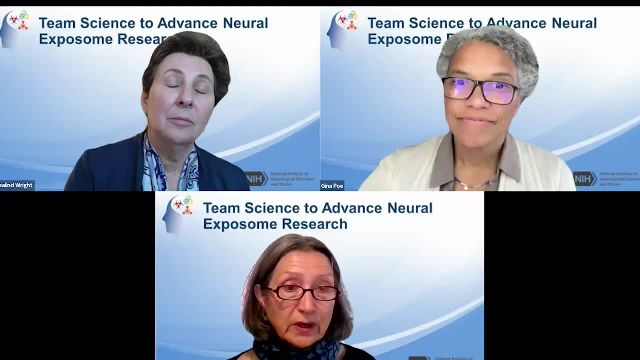 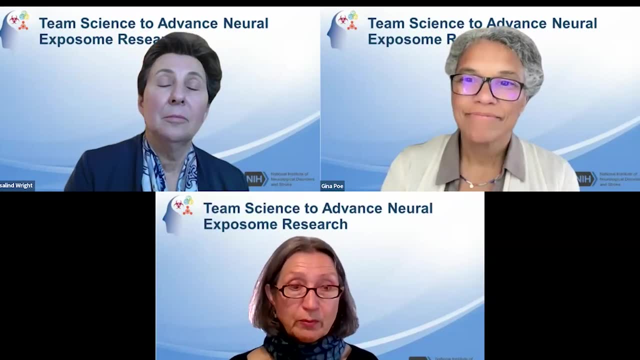 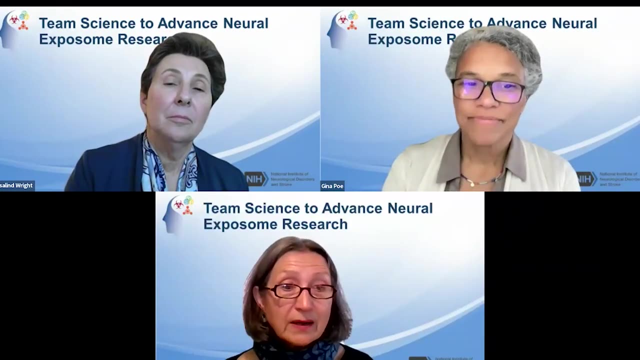 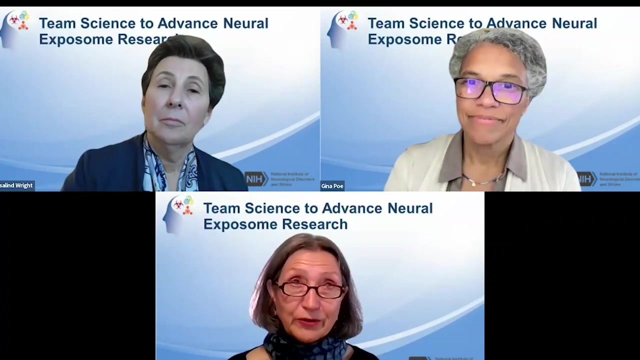 And I think that's something we can all learn how to do and we can promote across our professional societies and encourage people to be Positive and not negative. in terms of transdisciplinary sites of researchers, you know not, I've been when I was a student in medical school. 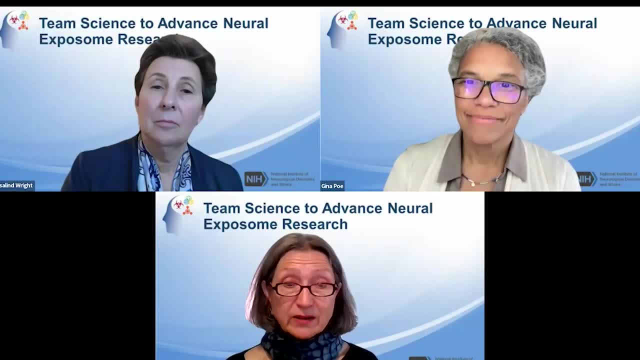 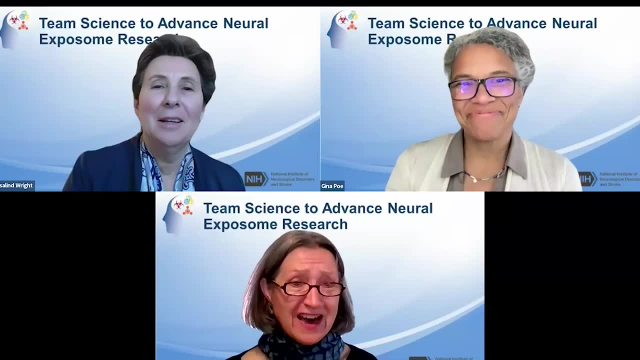 I asked my advisor what I'm good at, And he said: Beate, you're good at nothing, but good at a lot of different things. You're a generalist. Just go with that, You know so. So, and when I came to the US, 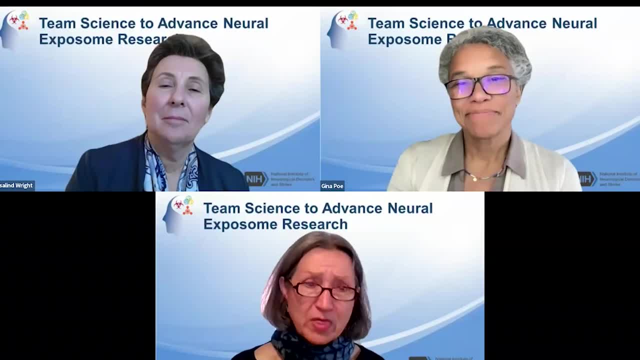 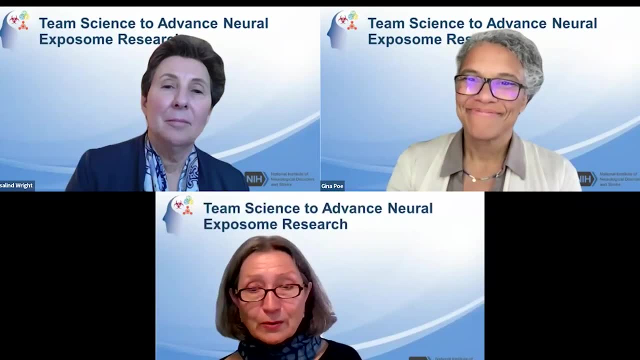 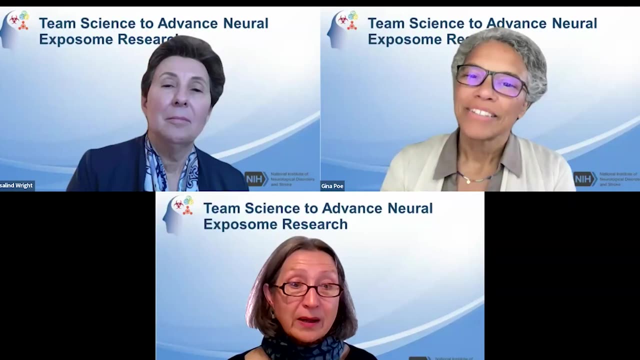 I was told: well, you have to really become the expert in this one thing, and then you're going to be making it. And you know, I was never that one expert. And so I keep telling my students: you know, we might become that one expert, but we might also just be a good team member And 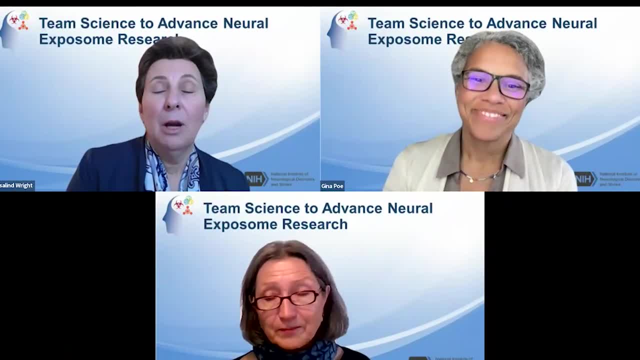 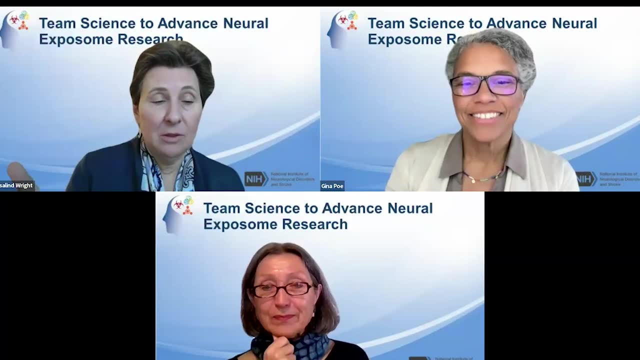 you know that should be as valuable Right. It depends on what question you're trying to ask and answer, whether you have to be- And that was that was the you know. that was told to all of us. You have to be known for one thing: What is it? And that was when I was told I was unfocused. 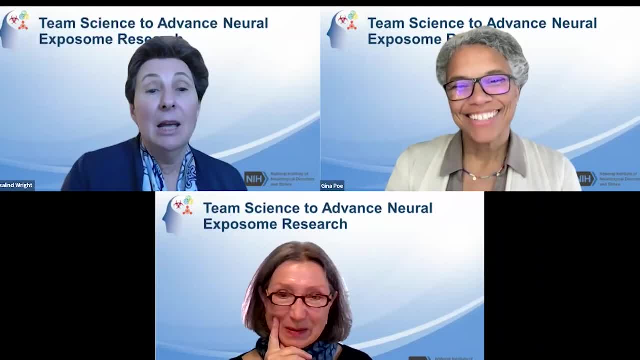 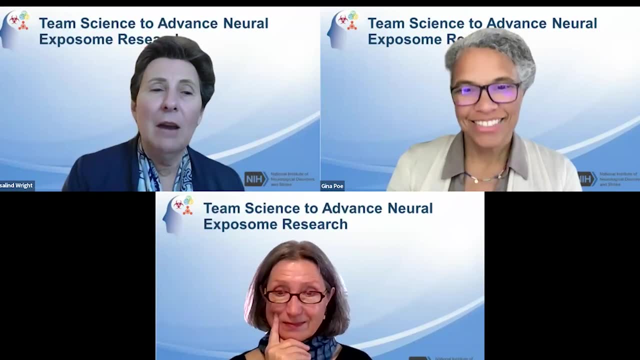 because I didn't think I needed to be known for one thing And I was comfortable there. Okay, fine, It doesn't work out, but at least I'm searching for the answers I'm looking for. You have to kind of believe in that and have that, do that, have that internal barometer. 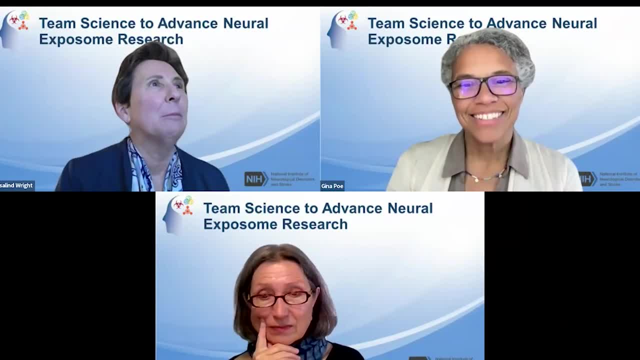 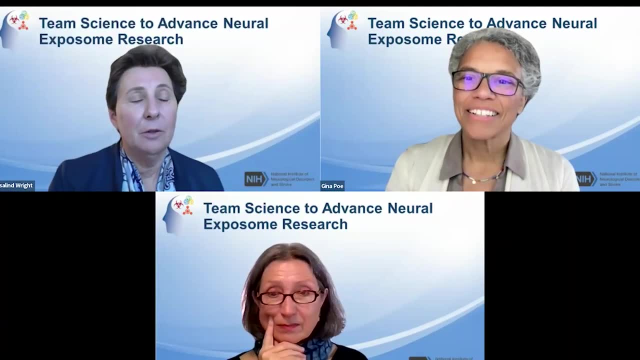 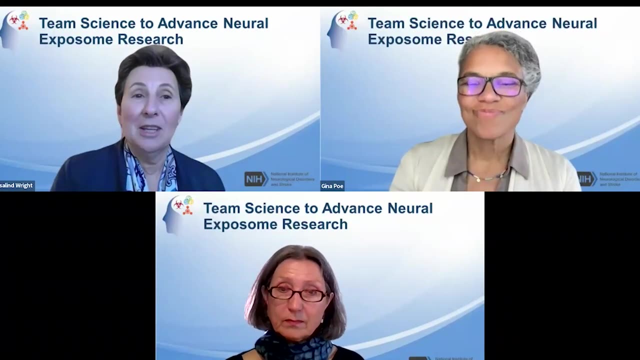 of where you're going and what you're trying to do, I think for a best practices paper in this context. I mean, we've said it here, It was exemplified in several of the talks- this is just a team science problem, Neuroscience exposomics- you put those together. It can't be. 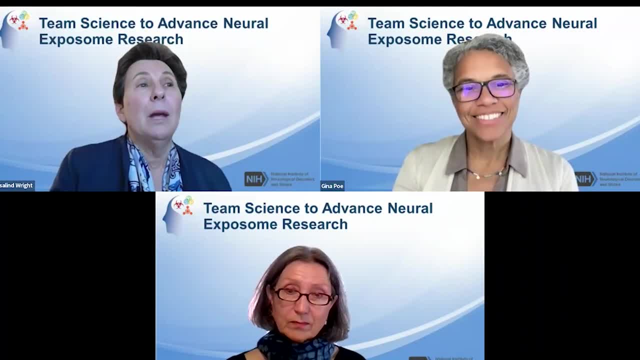 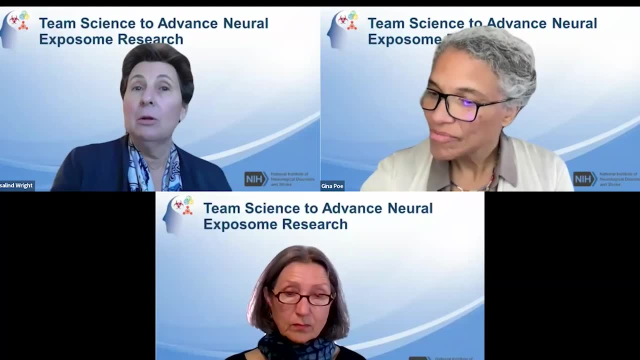 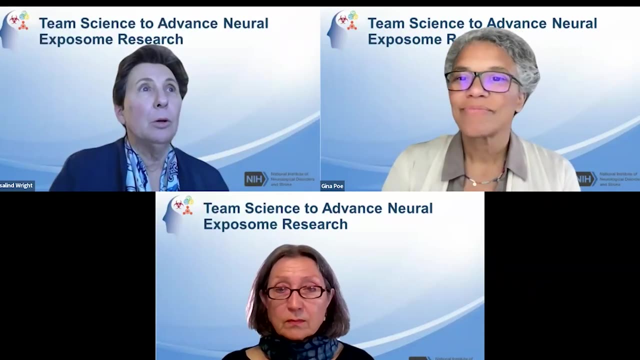 done any other way. What maybe lessons learned from the combine program be a part of, maybe leverage that, because we heard some talks that really showed that and you know lessons learned. some of it's going to be, you know, more universal team science, best practices, that kind of thing. 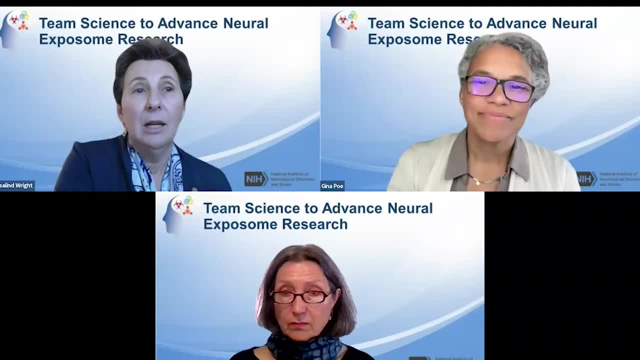 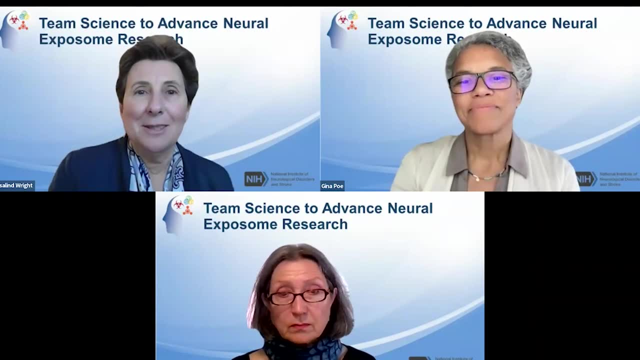 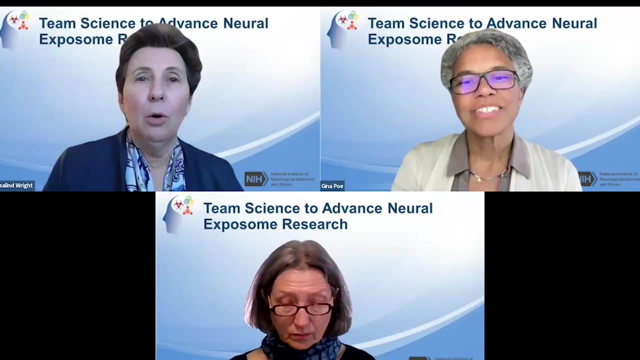 But how do you apply it here to move things forward and have people start to see the successes? I think, on the face of it, it just is obvious. This is a team science and we need to help. We need to start to solve it. You don't have to do it all to make big steps forward. Exposomics. 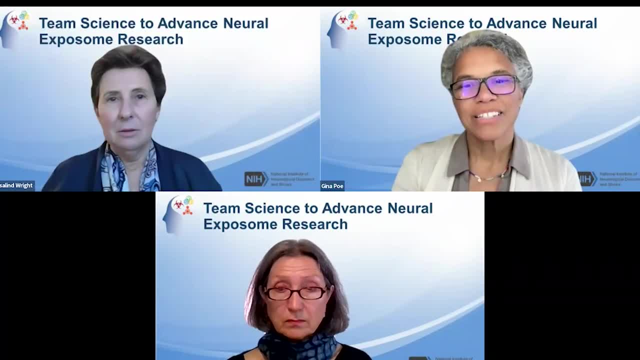 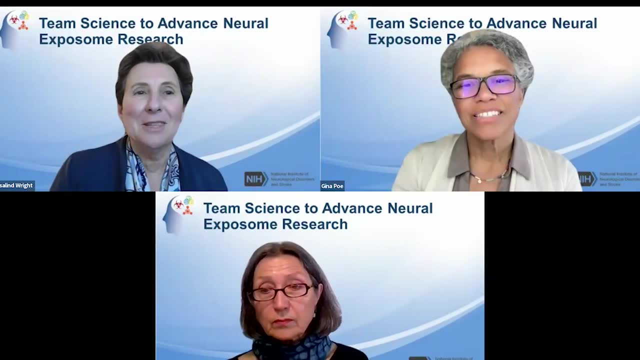 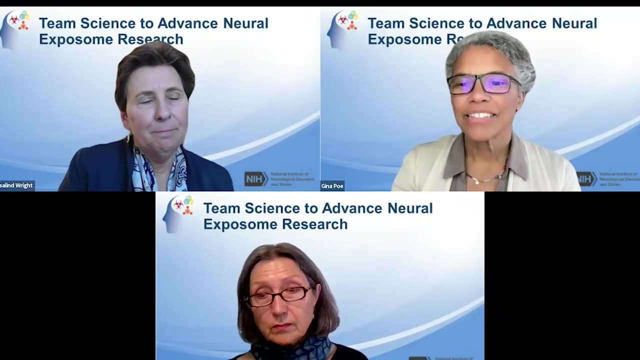 I always say: you don't have to measure it all. We the ideal. you know from cradle to grave, everything you've been exposed to over the course of your life, plus the internal response to those things You're done right there, because you think, well, that's impossible, Then you, if you unpack it some. 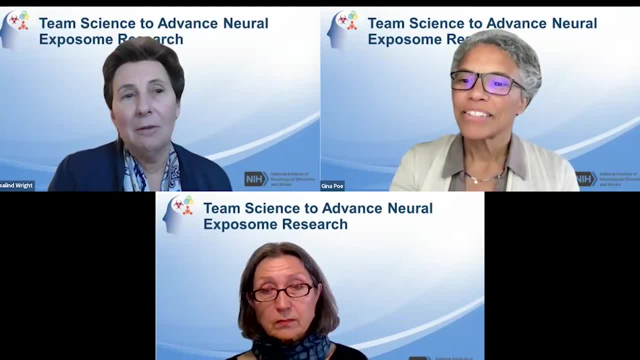 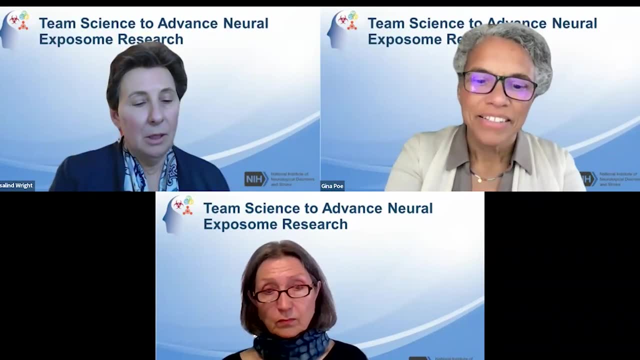 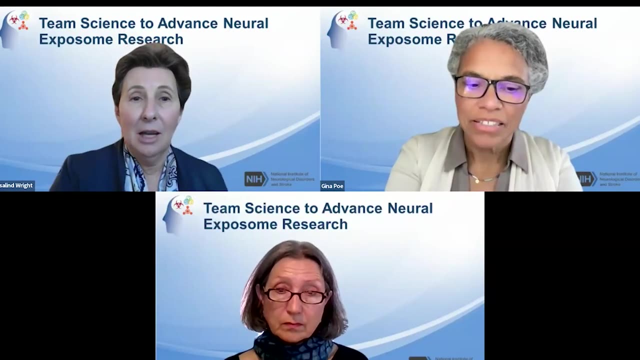 You really make huge advances by doing just pieces of it in as team, in a team science approach, in a bigger, bigger way. And we, it pushes us to develop the tools, the technologies, the computational science, et cetera. Right, Just like genomics, as we, you know, started to say: hey, we need to sequence the whole genome. 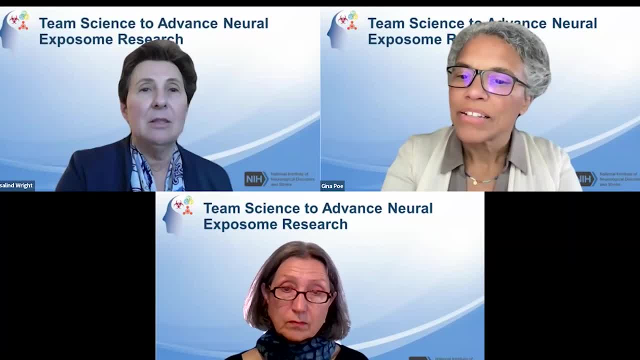 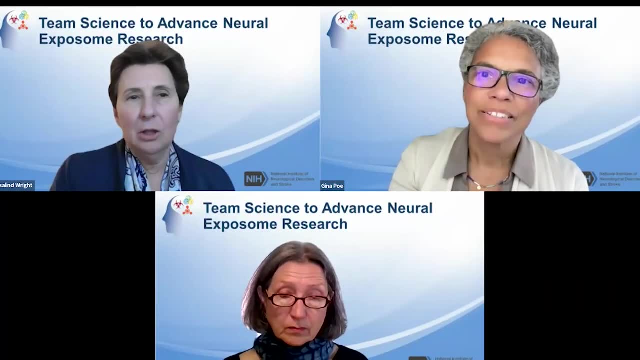 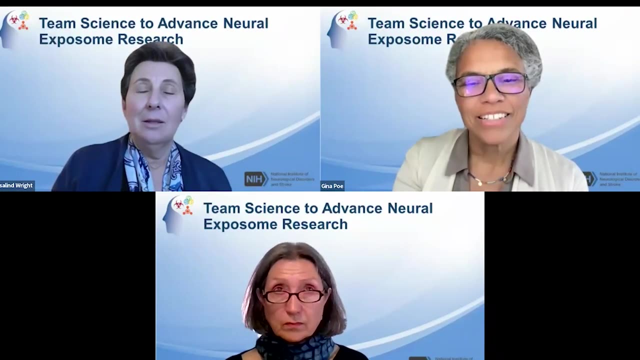 We have to do deep sequencing. People started investing, We got the tools, the technology, But you know, our statisticians help develop methods that we could actually look at all this data Now we have a eye in and we're at this inflection point, where that's, you know. 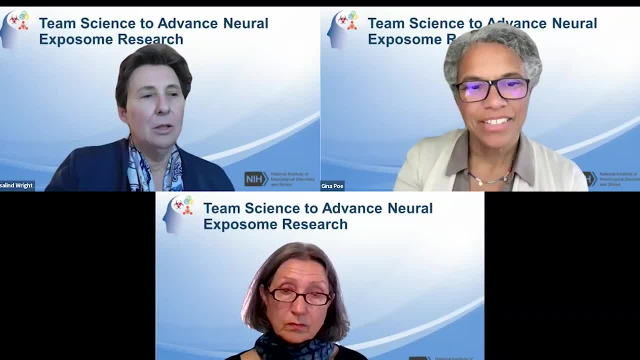 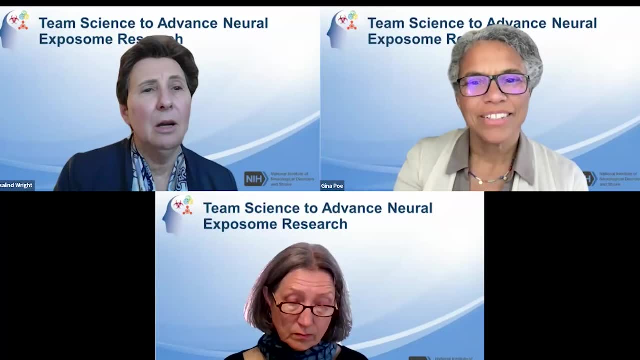 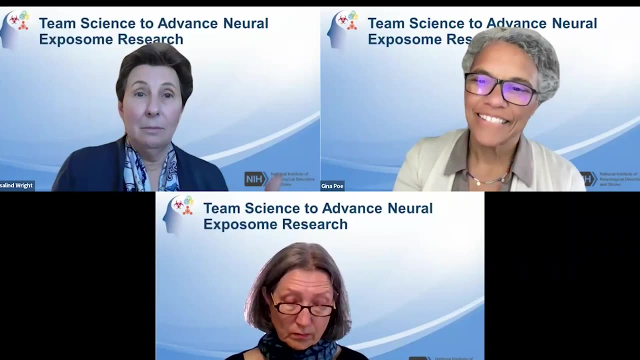 that's what we need to be able to look at. you know, four hundred and hundreds of thousands even of different things at one time. Right, Can't do it with the human brain, but we need our, our data science. We need to invest in the computer power that's going to house this data. 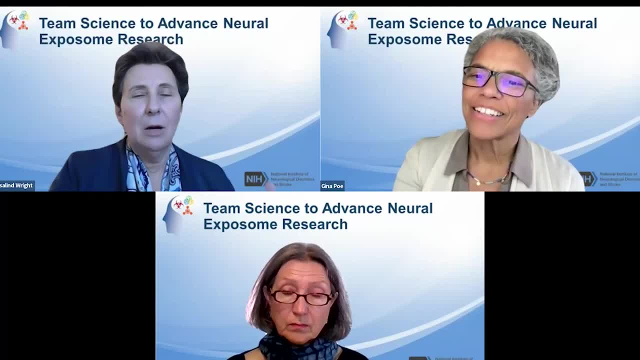 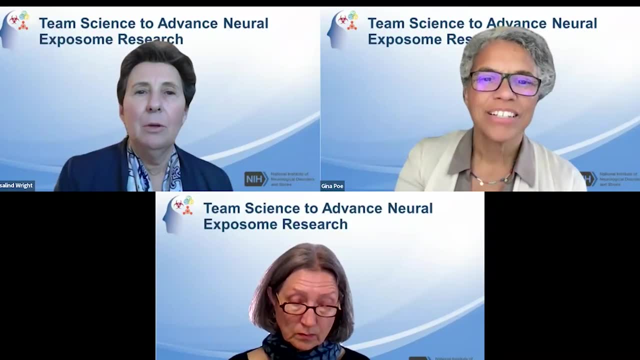 We had an example we heard of. Well, this is how we solved it in our situation, But- but you know, we need to think about that- How much do we need to invest with? If we're really going to move forward in this way, there's going to have to be a huge investment in that type of interest. 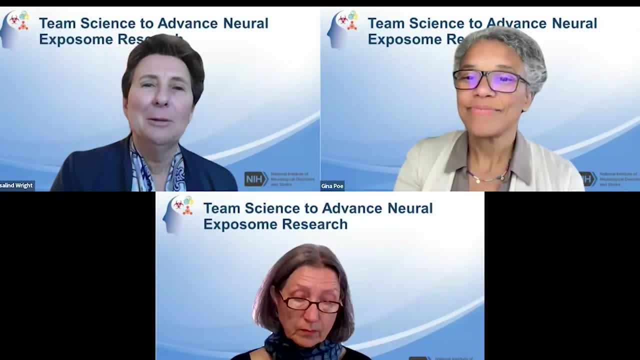 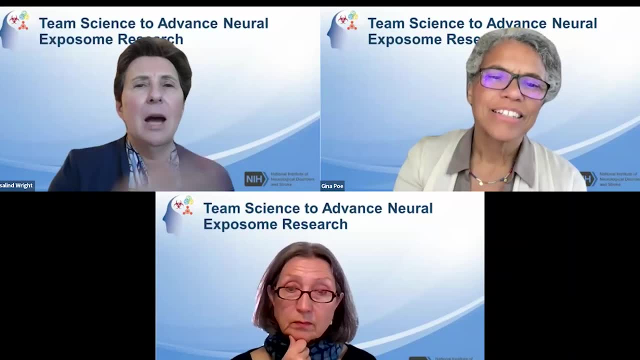 And this may be coming in the April workshop, you know, but? but you do need to start thinking about it, Right? You're thinking that way, But I think the best practice is: why not build from this combine program? you know, and just say it out, right? 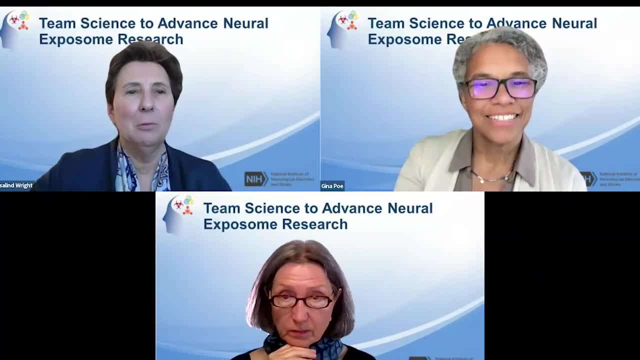 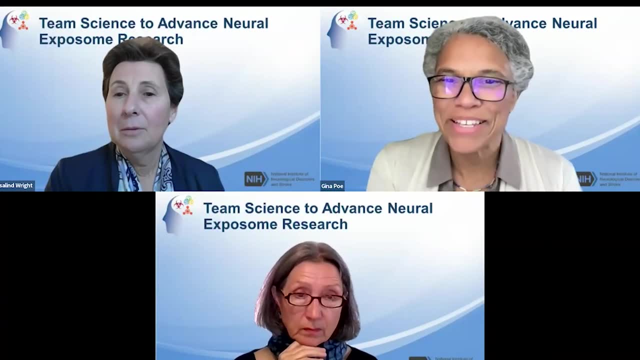 It's got to be team science. Here's how we started. Here's what we've learned. Where do we go from here? That kind of thing That would be interesting to me. That would be fantastic. So I want to do two things at this moment. 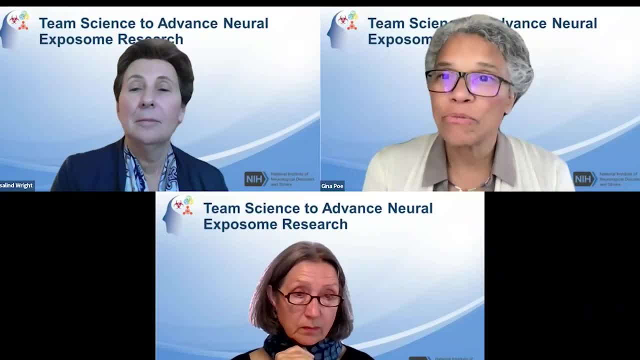 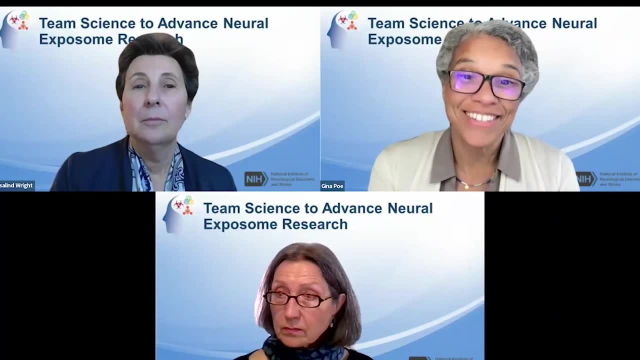 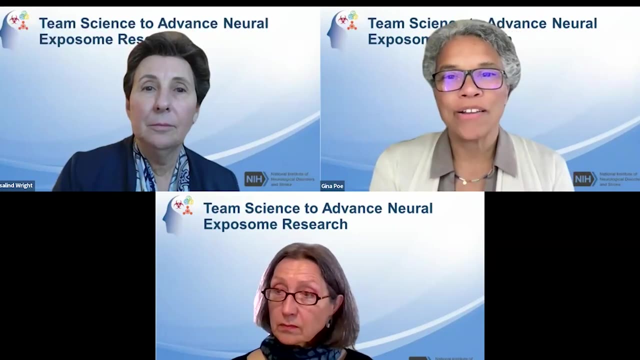 which is invite the audience members to make sure and they put their questions in the Q&A, because this is the time for us to discuss your questions Allowed and open, And also to invite the other panelists and speakers that are on this call right now to chime in. 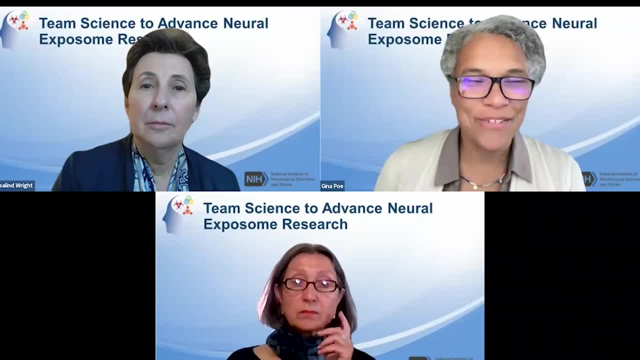 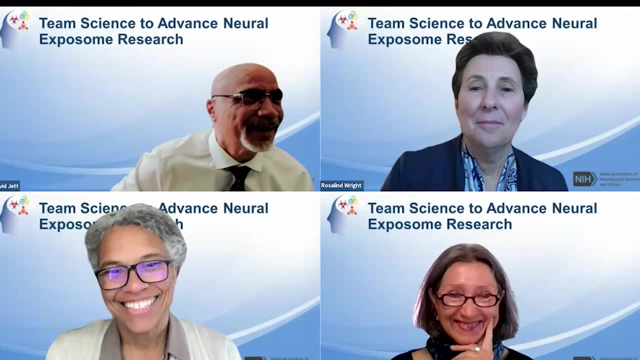 I would love to hear from some people. David, you've got a question or comment. Yes, please take it away. Feel bad. as the first one. I want to start with the hardest thing. This has been so great. I feel so much better. 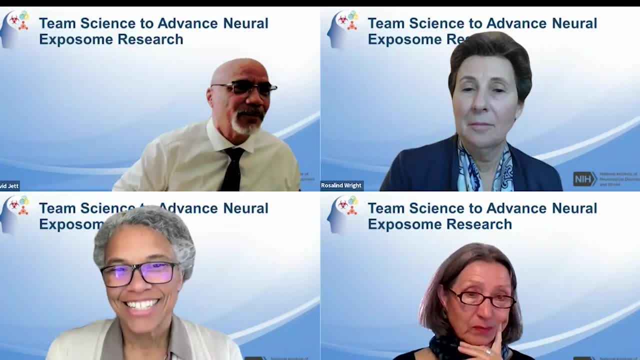 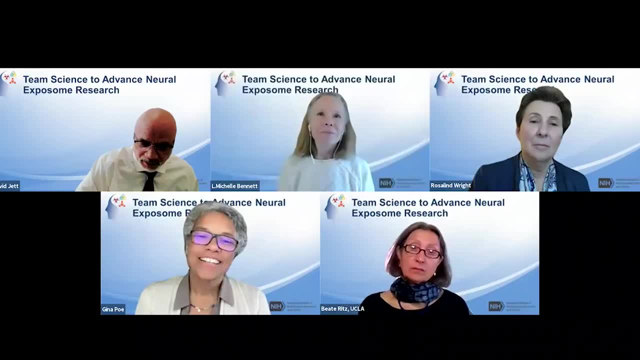 I mean, you know, I really think that we're going somewhere now. So I want to start with the hardest thing that I can think about, And that is: These are all great ideas. I'm thinking something like: so, if you're going to study, 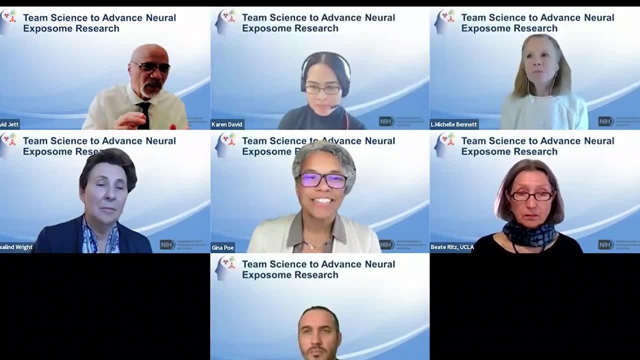 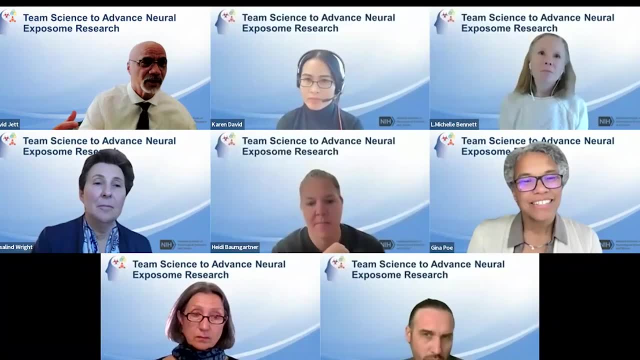 Lewy body disease and you're going to have different people. I do it this way and I do it this way, I use this, I use that And you bring them all together. That's good, You know you bring it up, But we're talking about somebody who does social stuff. 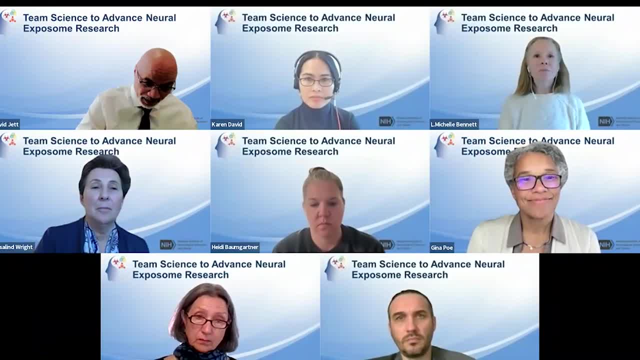 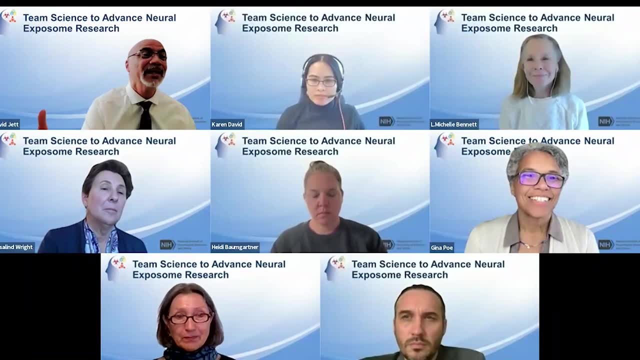 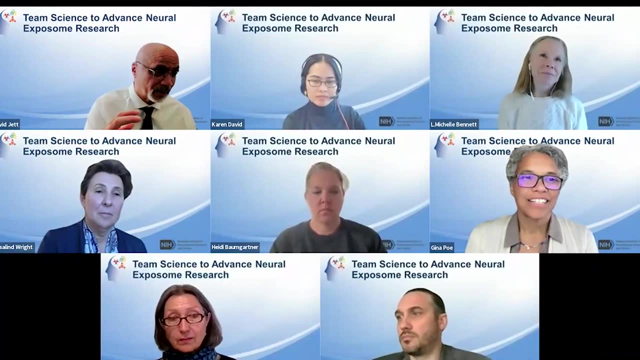 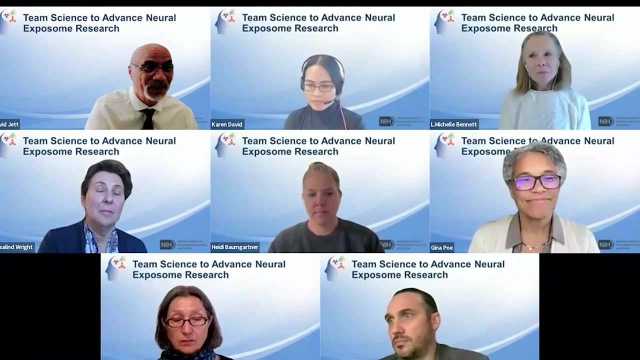 Other ones do. Do chemical chemicals Other than the sleep, other reduce climate? That's the part that scares me. You're bringing those get, bringing them together, making them work together And making the directors of the of the part that their work from say that this is good to do and it's going to help you. 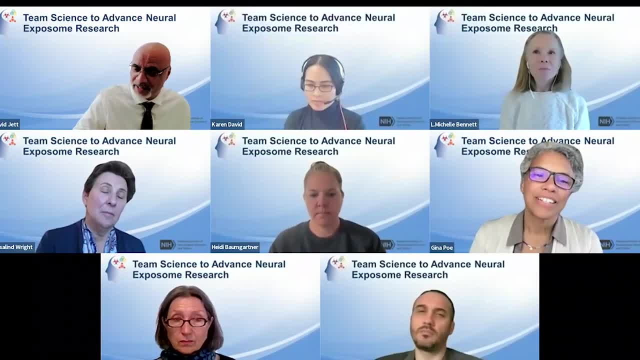 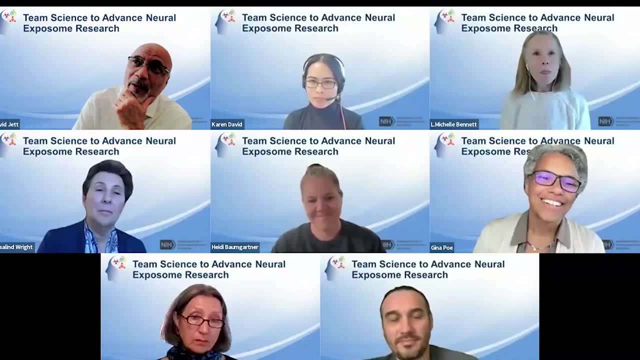 That's the thing that I, and it's just that. And then the other thing I already said about you know getting. We're going to have to do this one at a time, But let's just do one at a time. I'll just stop there, because that's, that's the hardest part. 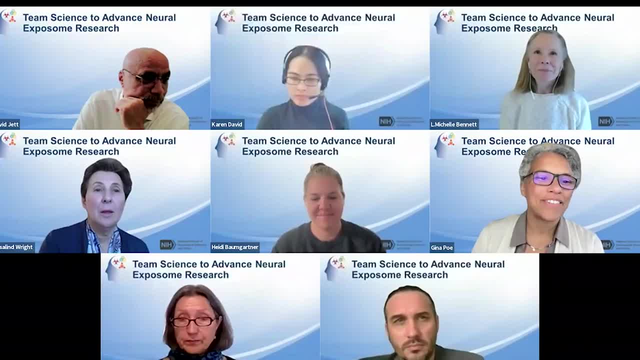 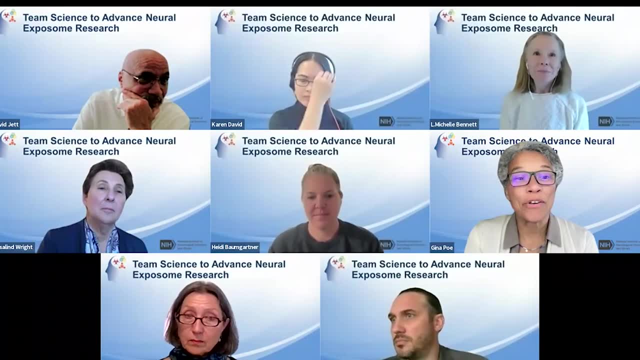 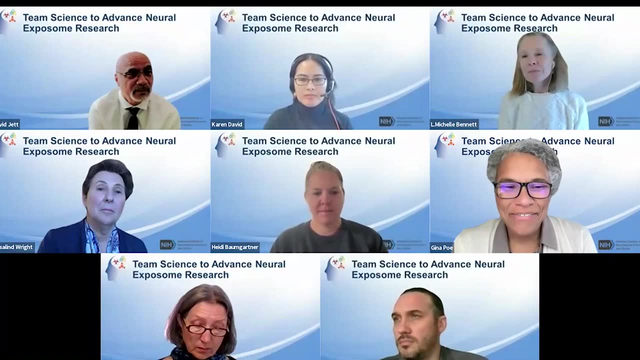 I don't know how much more time Stop there. Yeah, So you're saying, David, that the hardest thing is getting all these people to talk to each other and getting the community to value each member individually. So does anyone have a perspective on this? 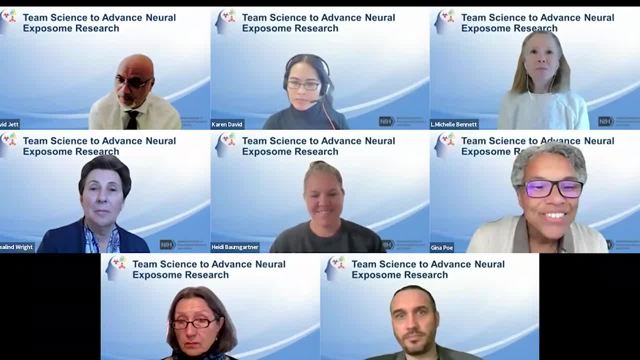 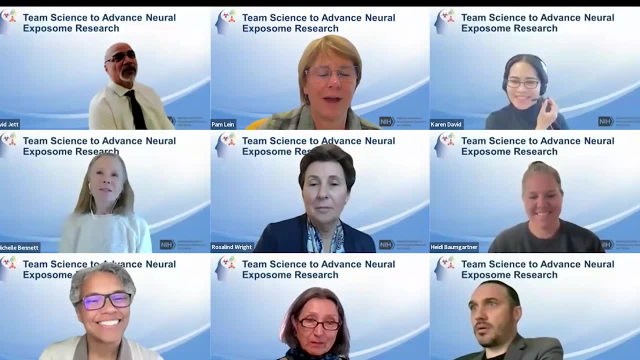 Heidi, Yeah, Go ahead, Go ahead, David, Go ahead. I raise my hand, So I'm like Dave, I just jump right in. But I think you know the the obvious and most difficult answer to that, and most challenging answer, is money. 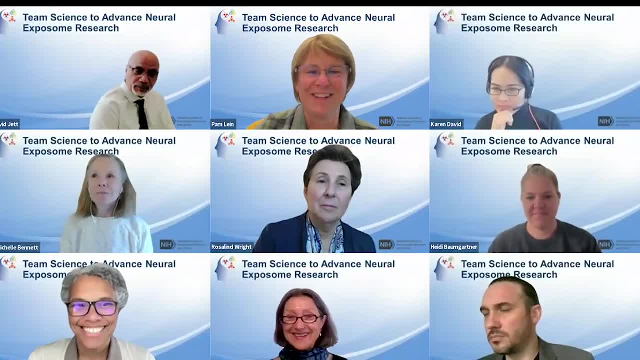 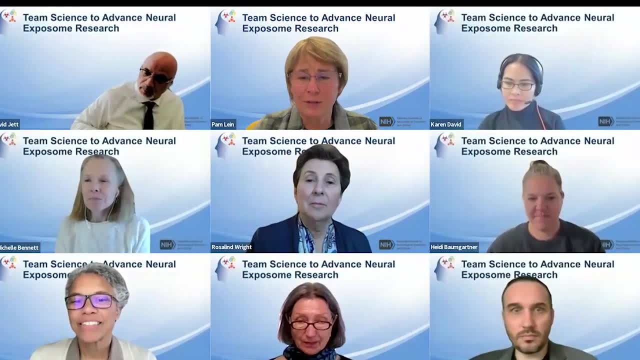 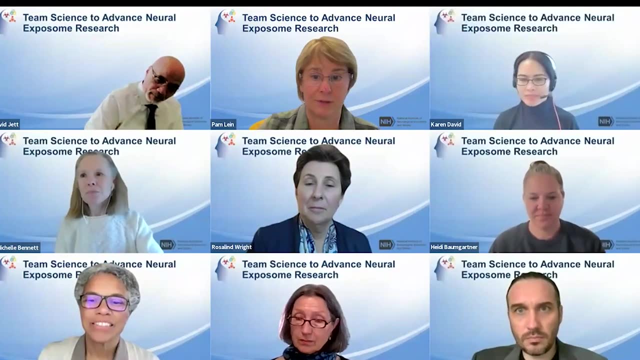 You know researchers are going to follow the money, David, You know that. So if you make it implicit in the funding opportunities that it has to be a was word, that Michelle is cross-disciplinary effort in order to be competitive for funding, That will force these people to talk to each other. 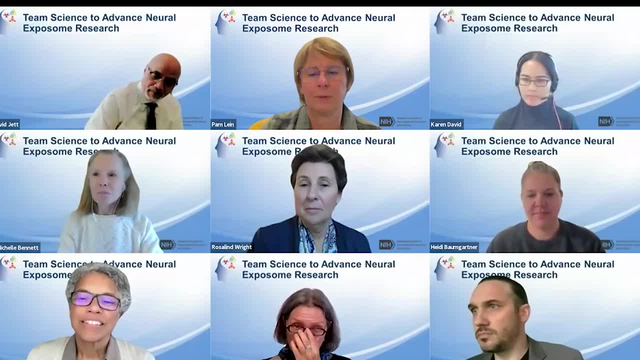 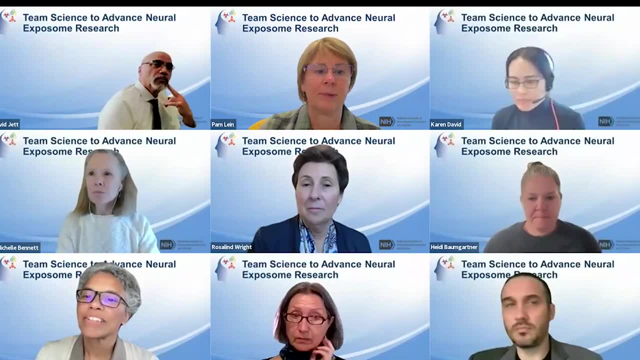 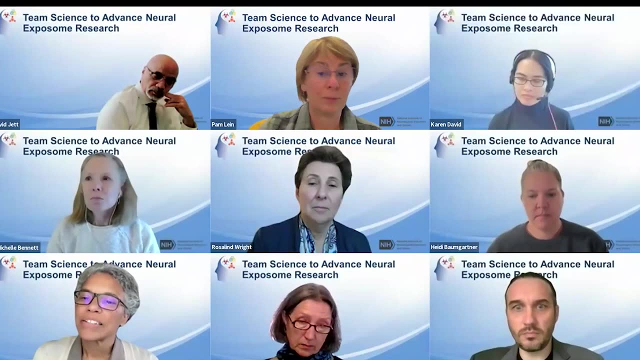 I also think that it will be important for the field to move forward that we find leaders who are really good at this- And we have some examples here on this panel who can lead by example. And then, third, I think institutions themselves- a lot of them have opened up- are embracing the concept that team science is going to be essential to solving grand challenges. 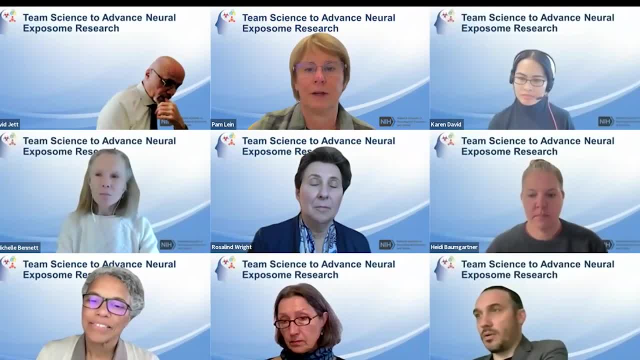 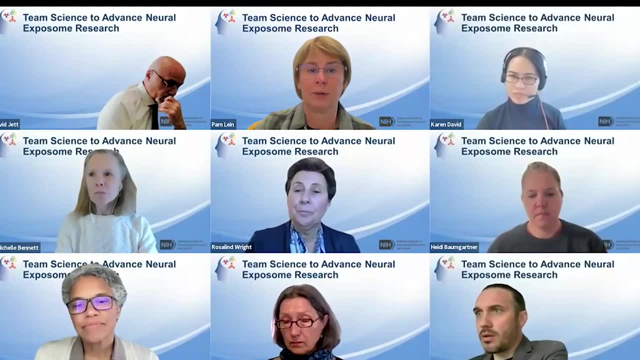 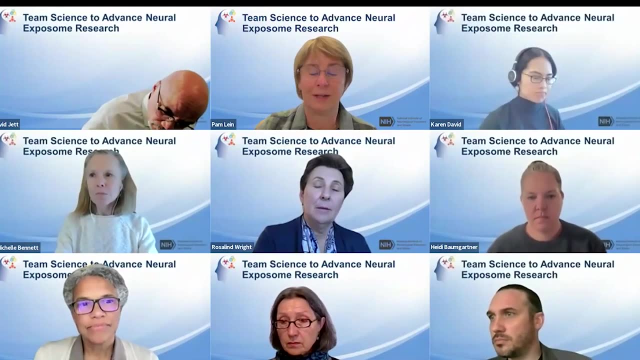 We call them wicked problems. that you see, Davis. But you know there's a lot of money within the State of California being put forth by you, cop. There's a lot of foundations that are putting money into bringing together these cross-disciplinary teams to really tackle these very, very challenging questions that are threatening society. 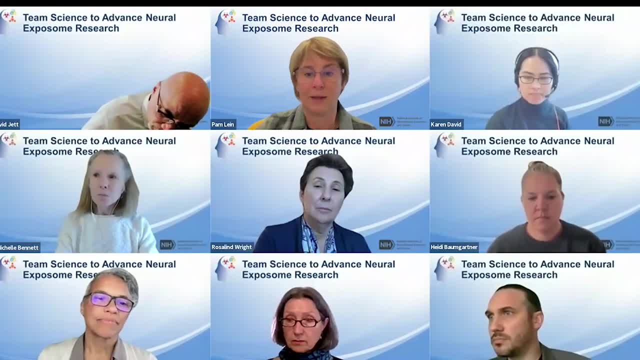 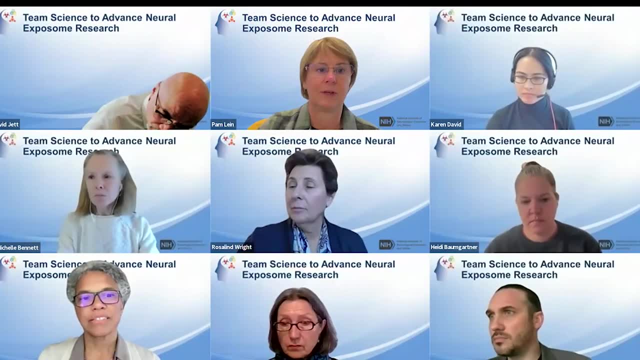 I mean, I think we're sort of on the cusp of understanding that our society is a risk as we know it and that we need to really begin to work together to address some of these. So I think we need to leverage that. 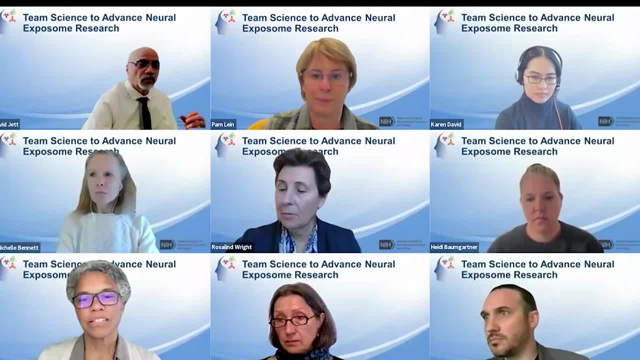 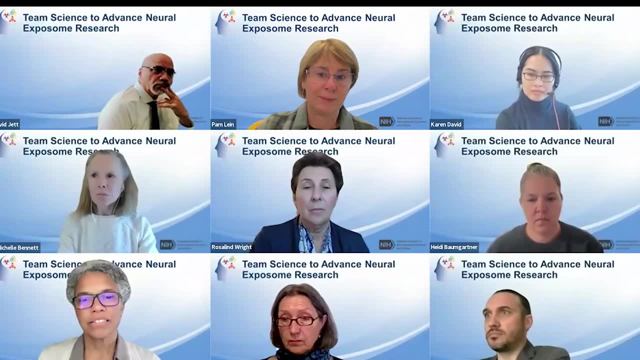 And I think we need to have a really strong, swelling recognition of you know, no one person is going to solve this on their own, And I know at least a lot of the people I talk to at the meetings I go to- and I may be preaching to the choir or talking to the choir- 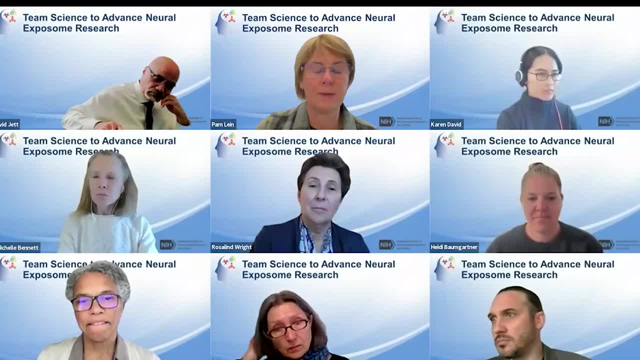 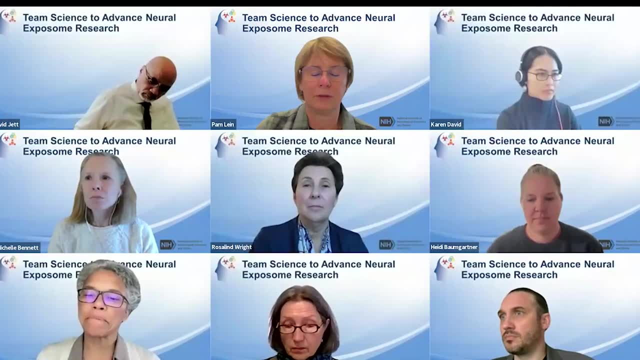 I'm not sure, But you know, they they all feel a personal commitment to wanting to do this is not just a scientific commitment, but it's a personal commitment to improving the world for our kids, for ensuring there is a world for our kids, And so I think we really need to. 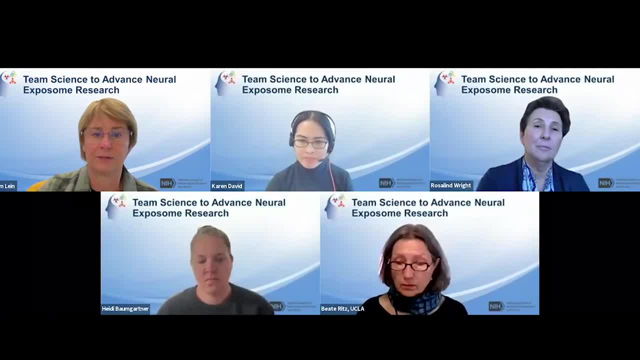 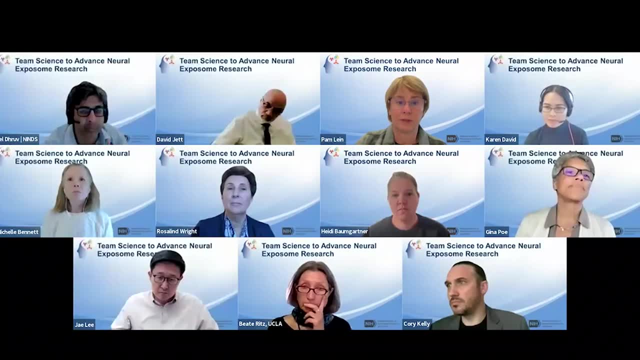 We really need to kind of leverage that and, you know, say and make it clear that that the kind of science that NINDS wants to fund is going to help us reach that, that goal, or achieve that goal. Karen, that's wonderful, Absolutely, Karen. 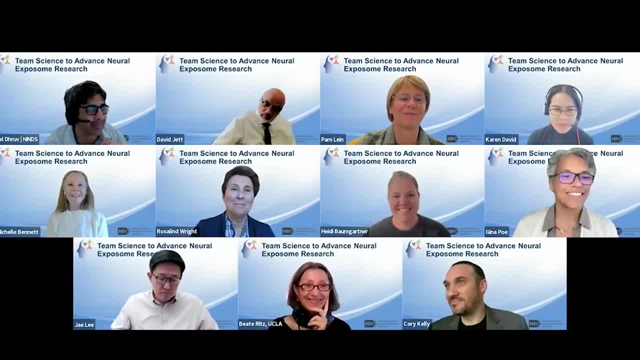 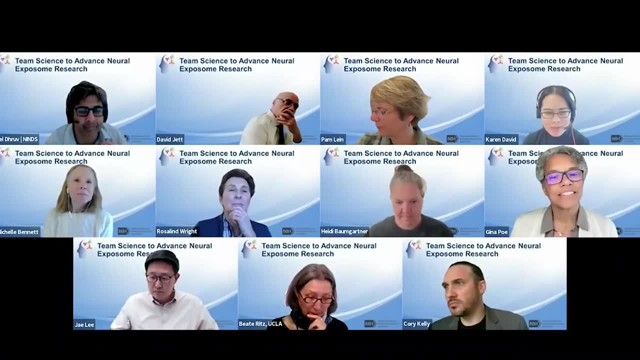 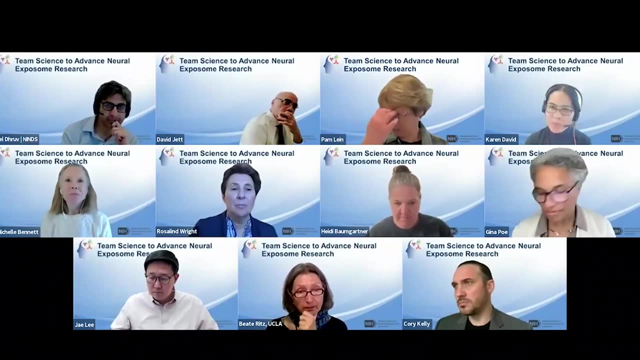 Right, I heard Pam mentioned money, so I'm going to chime in about funding opportunities. So we- I think we had this issue or kind of recognizing, for example, we did Brain Initiative, We did Brain Initiative, We did Brain Initiative- We were, we had in mind specific scientific disciplines that we wanted to bring together. 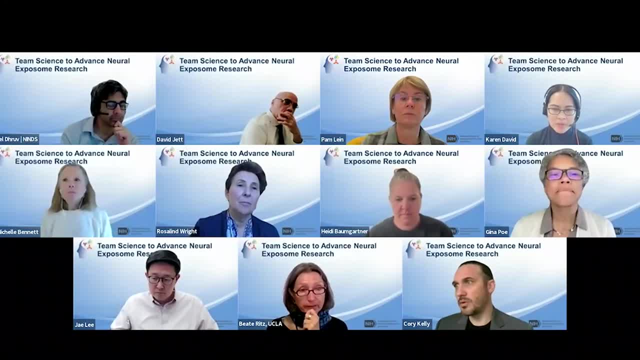 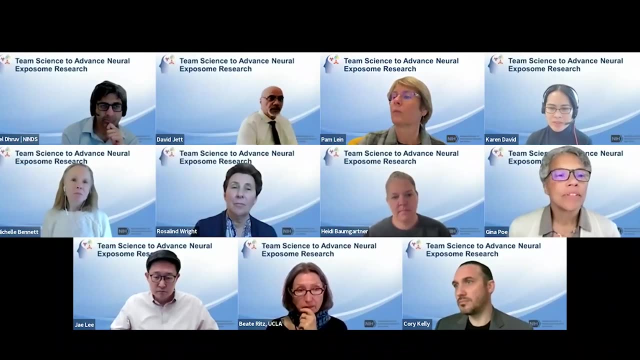 And so I think, in our perspective, there are two ways to go about this. one is you hope that the science proposed will bring in all these disciplines that you wanted to see there, or you could just encourage or be prescriptive in your funding opportunity that this is you want. we encourage discipline x to collaborate with discipline y. 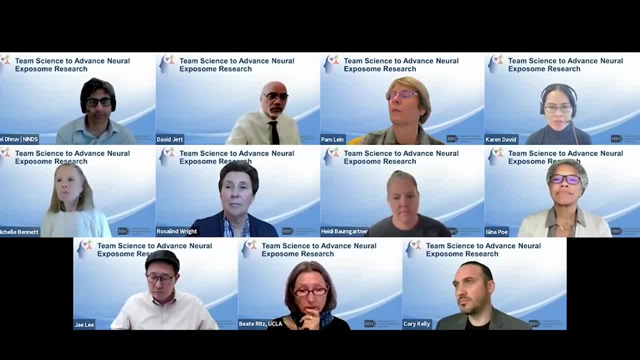 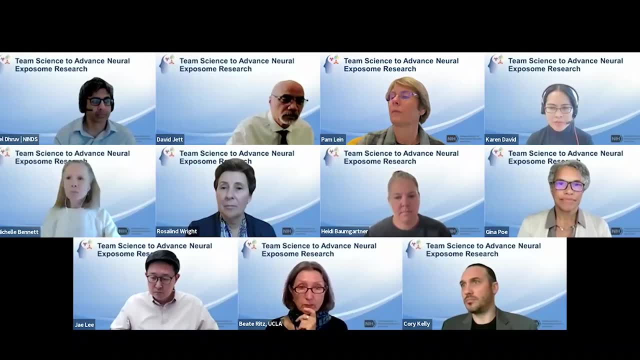 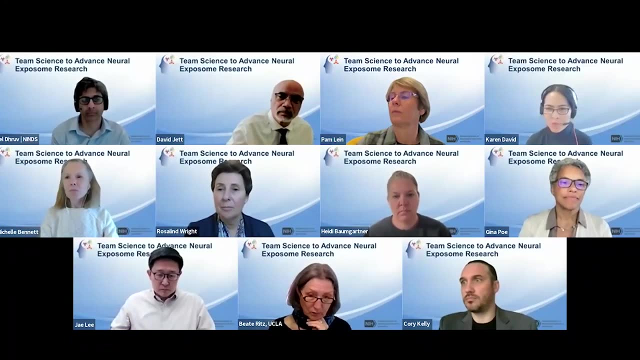 And that's what we did for the Brain Initiative, where we wanted to bring the theorists and experimentalists together, and so that's one of the things we encourage explicitly in our funding opportunities, So that and then we provide resources to promote that kind of 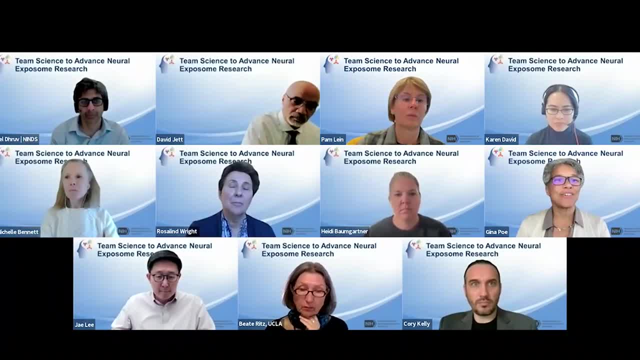 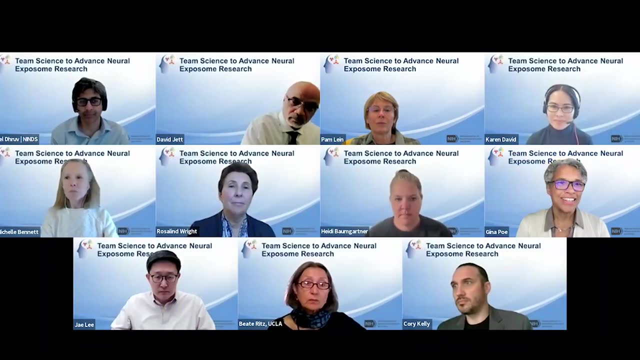 Yeah, but getting someone to review these things is also a huge challenge. Because if, if, if a grant application is wonderful, Yeah, but getting someone to review these things is also a huge challenge. Because if, if, if a grant application is wonderfully transdisciplinary but you can't get a reviewer that can see that or see the value of it, then it's not even discussed and program officers can't even pluck it out of the file. 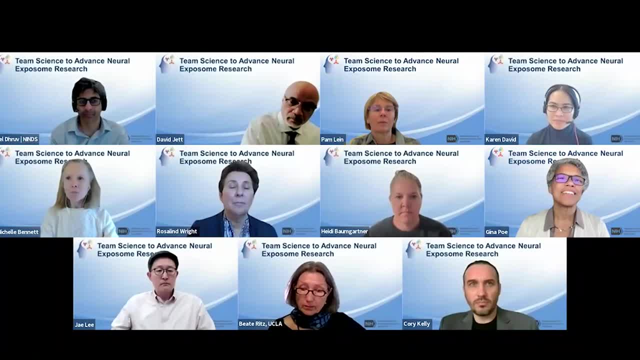 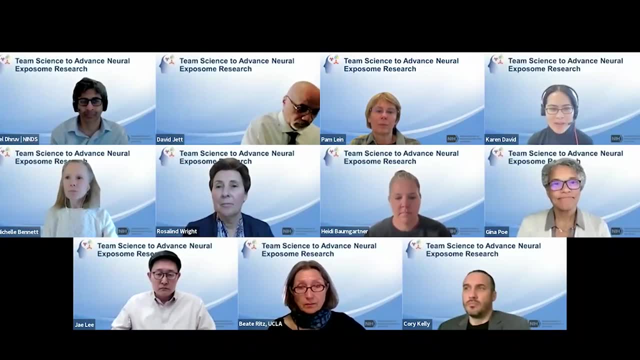 So that seems to be a huge challenge, Right, if I can chime in on that too- and that's where the value of having a special emphasis panel and that works so well for the Brain Initiative and also for the combined program- there is the challenge of making sure you have the appropriate 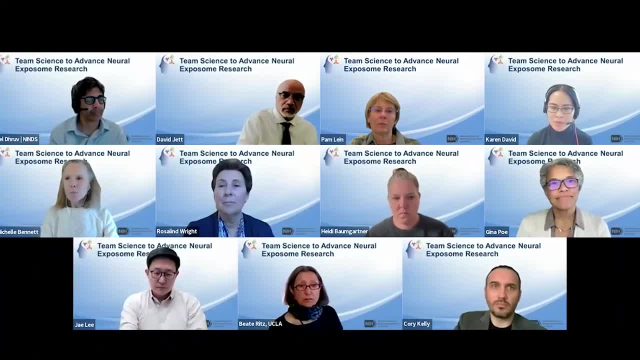 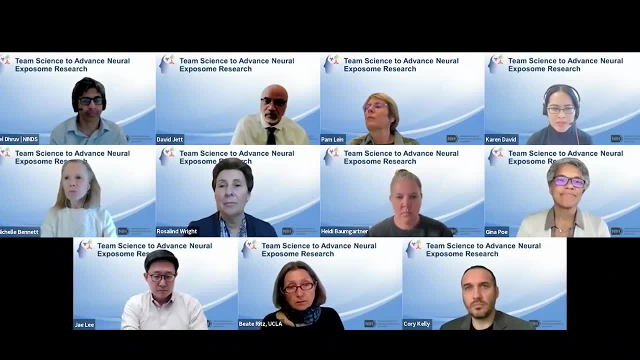 professionalability and the ability and expertise, and so corey was one of the SROs who worked with our team of SROs and it was it pretty much led to at least four, I think, I think, for reviewers, at least four reviewers. 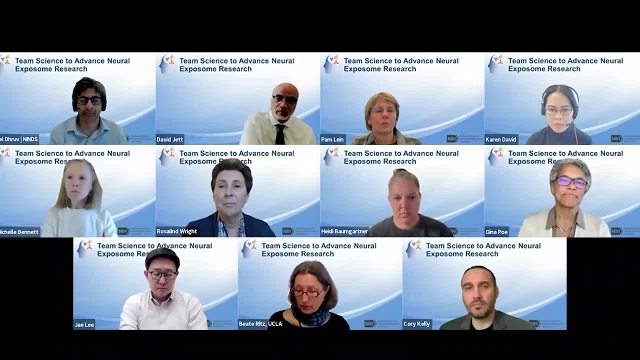 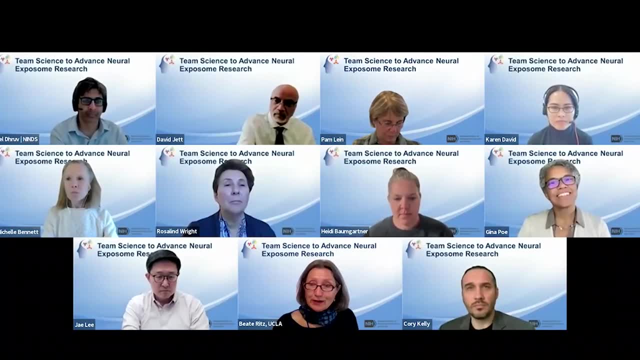 four reviewers per application to represent. make sure that we have the expertise representation. Thank you, Yeah, Beier Publicity Council. Nick, Yeah, I want to actually be hopeful and tell David, but yes, it seems like quite an effort. feedback because- and I think this question is partly about TEI listening to your case and you also close full circular text calculation. 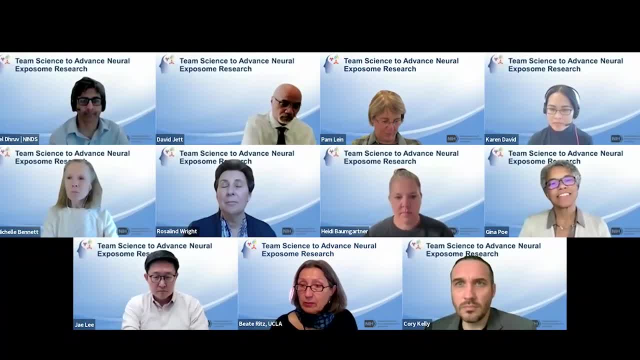 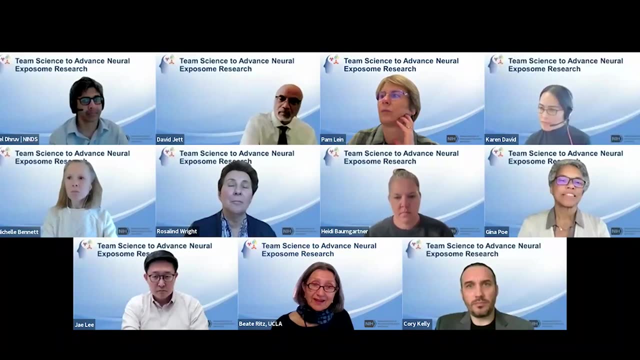 Thank you, cos to bring all these people to the table and to make it work. The good news is that on the environmental side, we have been trying to do this for the last decades already, So toxicologists and exposure scientists have actually talked to population scientists and MDs. 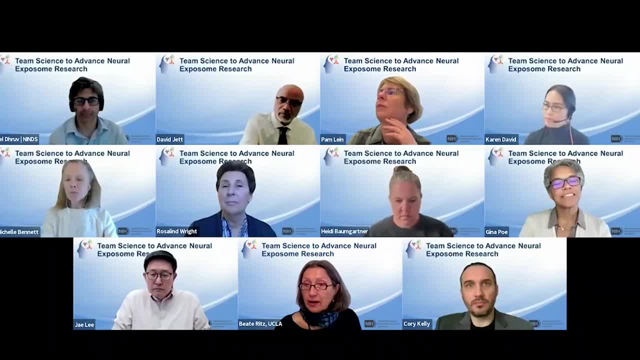 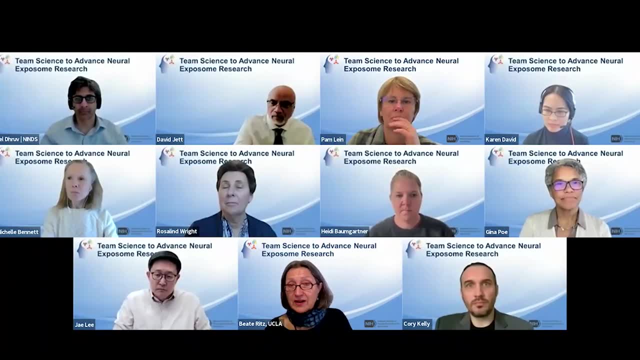 and there's a lot of collaboration already ongoing. I think it's less in the neuroscience community, or better between the environmental scientists and the neuroscientists, except for the few that actually in our community specialize on the brain. But I think that that gap can be bridged by requiring neuroscientists. 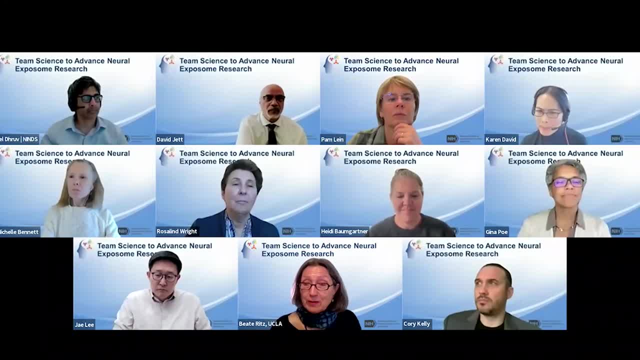 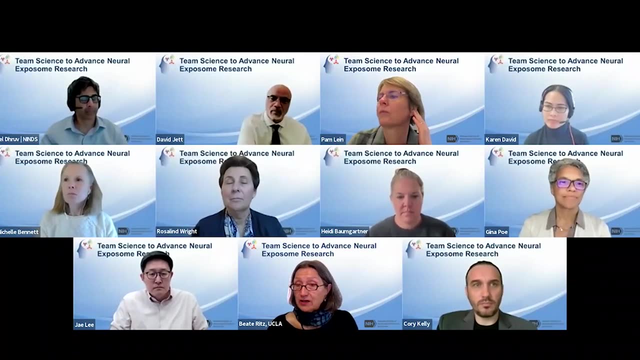 to actually work with people like us, or better, the people we trained, And they will learn from each other very quickly and it will become extremely exciting. If I hadn't had the experience of, you know, the Center Grants, I wouldn't now be funded by DOD in a project with IPSCs. 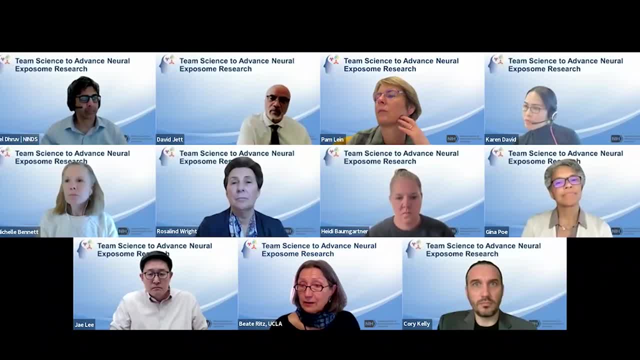 where we put the pesticides we are identifying in the fields that might be related to Parkinson's IPSCs, and do some really exciting experiments in the lab. Of course that's not me, That's the collaborators who had the insight to ask me. 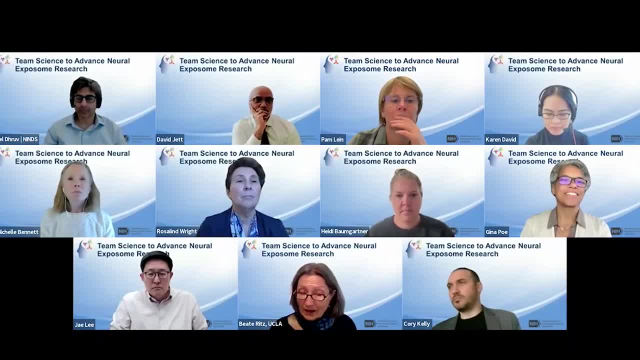 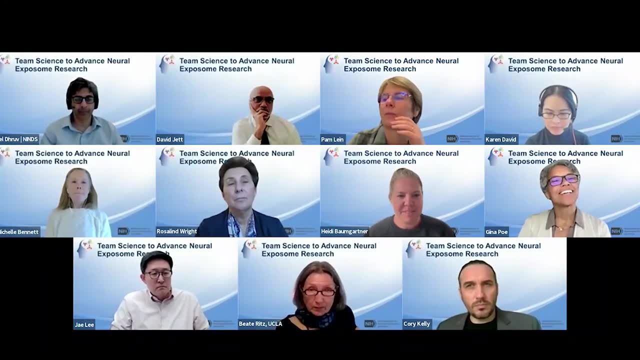 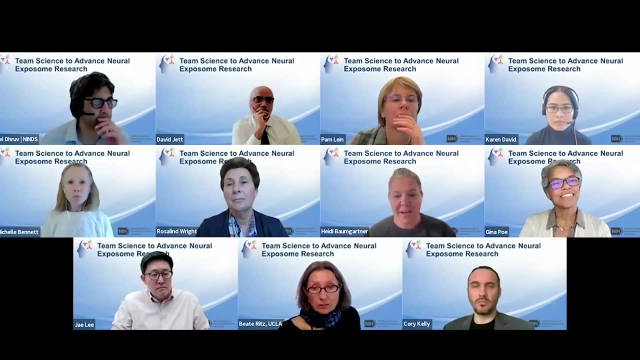 And I think this is possible. Thank you, That's absolutely right, Heidi. how do you? Yeah, I just wanted to jump on some of the things that have been said about the importance of funding. You know our group relies almost entirely on volunteer efforts. 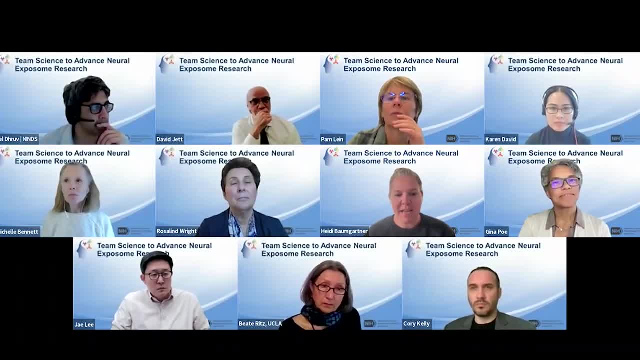 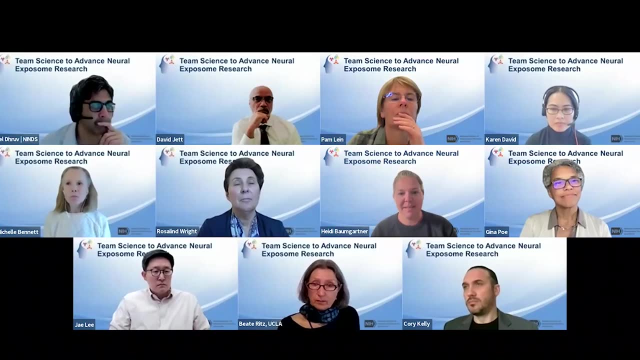 because it's been difficult for our group to get funding And part of that is because our projects develop like as they go. So we're not really well-suited for traditional funding mechanisms where you have a really well-defined problem and team. 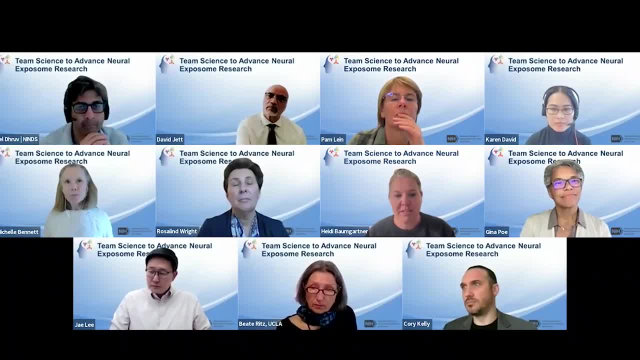 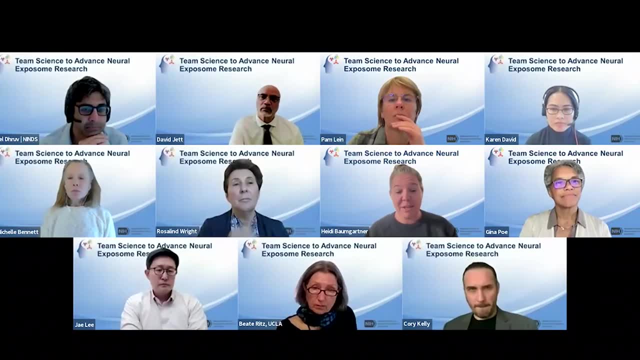 So we're not really well-suited for that kind of composition from the start. And funding is crucial also to the diversification effort. You know, by relying on volunteer efforts we're really limiting participation to people who have the luxury of time and other funding. 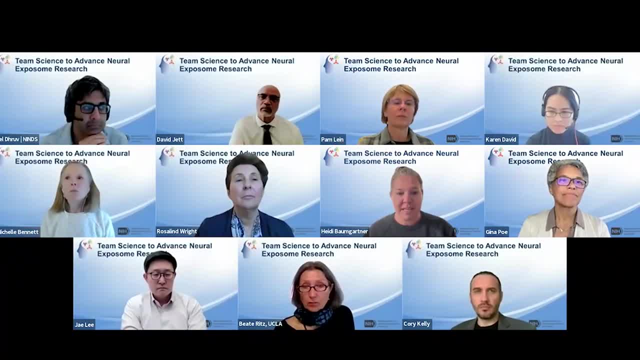 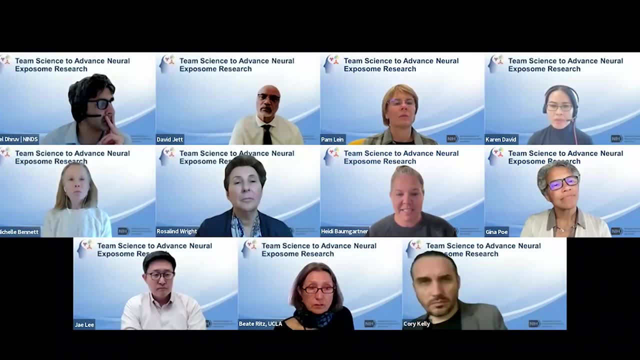 So I just- And then also I want to really jump on what Beate said earlier about using her voice and like her status as a reviewer, as a reviewer, recommender, to amplify the importance of contributions to team science. We're constantly trying to raise awareness of that. 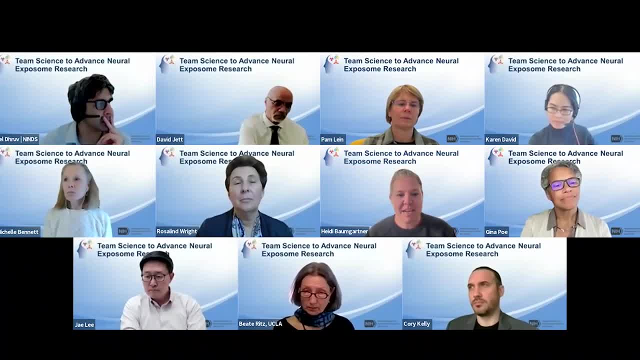 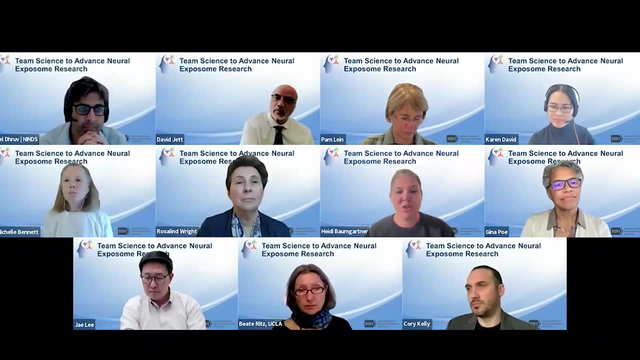 So I just want to put a plea out there for everybody who's sitting on, you know, review panels for funding applications or reviewing tenure applications, things like that- to use your clout as senior scientists to sort of change the incentive model, to help change the perception of these contributions. 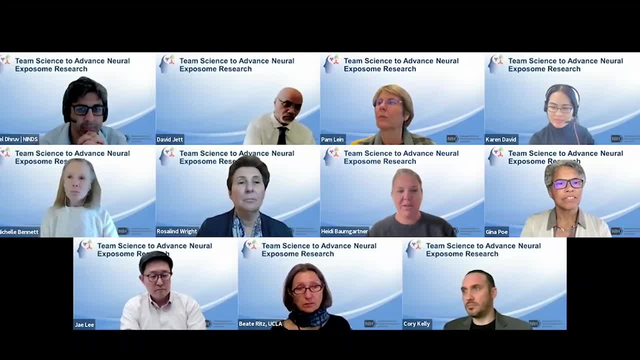 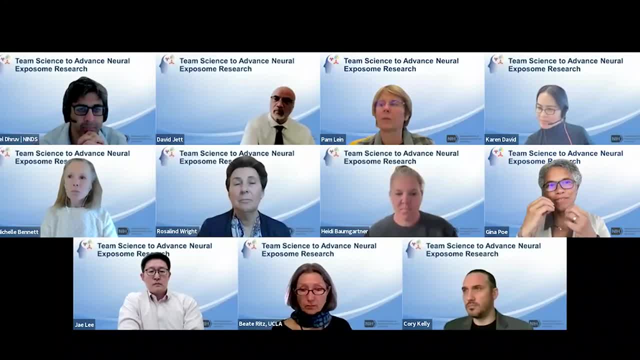 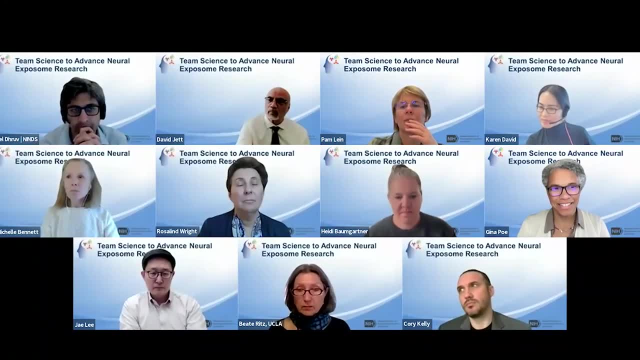 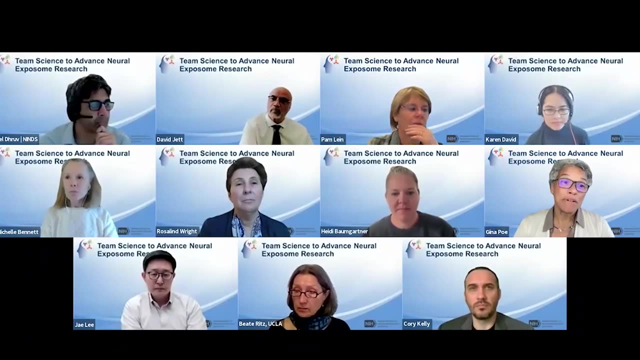 which was that a lot of these collaborations are organic, They develop quickly, They happen quickly And their funding mechanisms are things that you know happen slowly. you know, from the idea to getting the grant could be a minimum nine months, And so maybe do we need to change the way that we process these ideas. 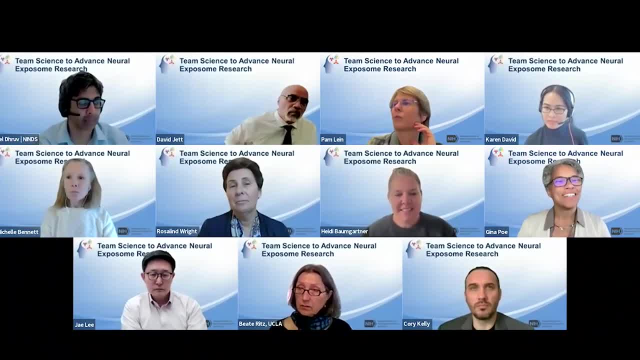 these ideas and pitch them and get them through council and all of that so that it speeds up the process. Because, yeah, you're right, it really does limit diversity if you're relying on people who are already well funded and already plugged in. 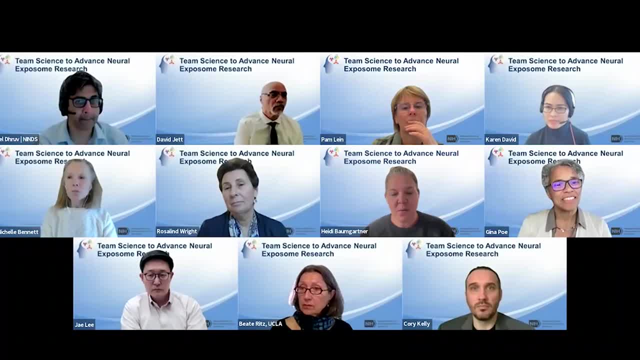 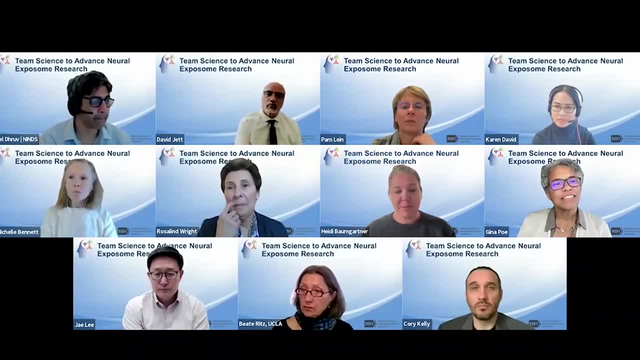 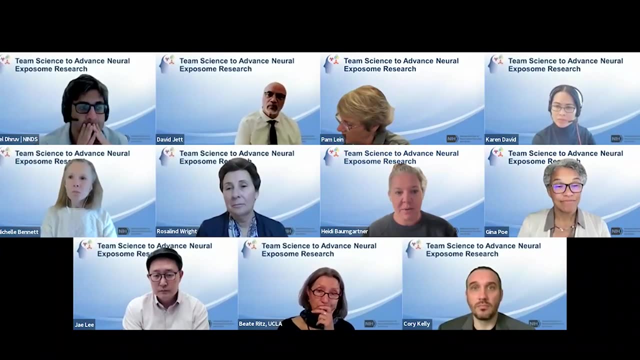 So yeah, Yeah. So one thing that we've pursued some opportunities but from our perspective, there just aren't enough out there is. what we really need from our perspective is funding for the infrastructure and for the central support that's not tied to a specific empirical project, because that's. 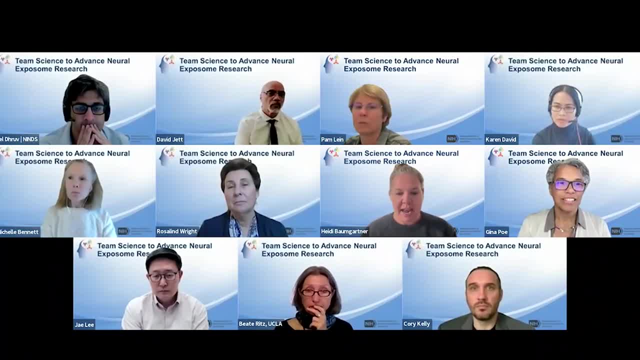 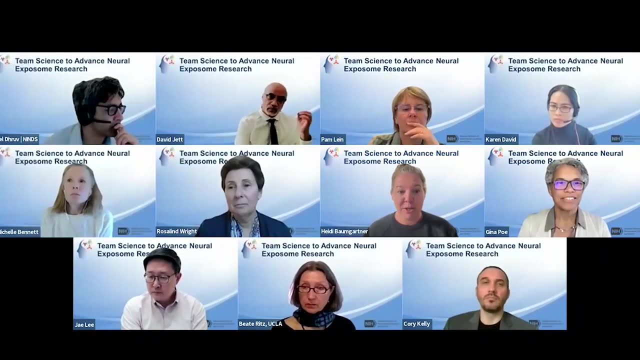 really what helps move these projects forward is to not have to have projects like redevelop that infrastructure and those support teams on a project by project basis, but to have that central infrastructure that can support multiple projects and learn from projects to apply to the next project. 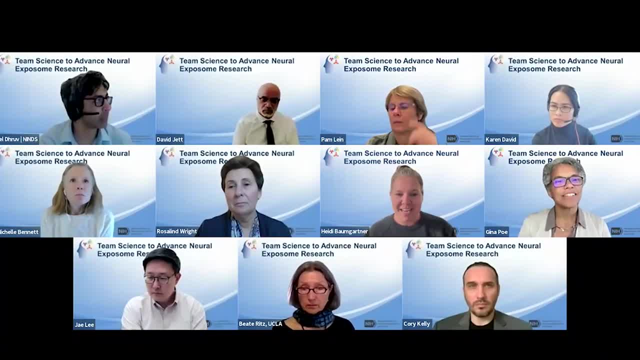 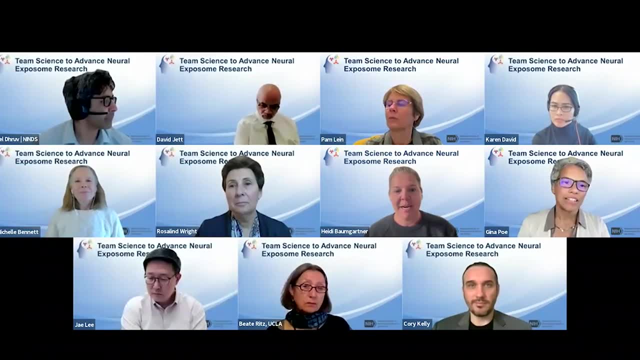 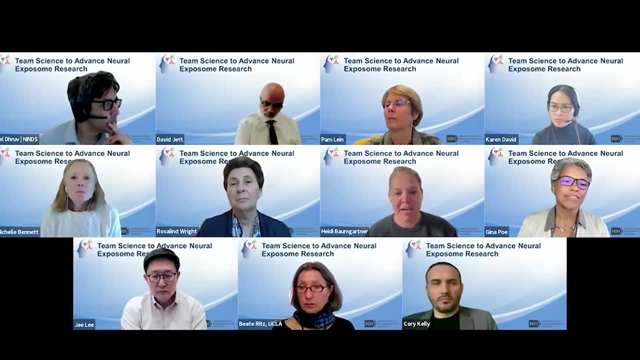 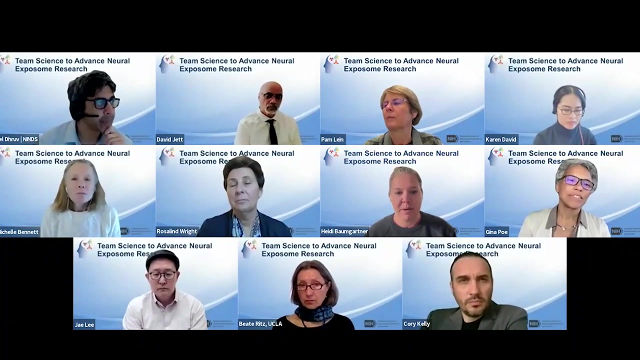 So my position Is funded sort of by institutional money and we're using things together, but it's a very unique situation that my position even exists And so, yeah, like having having funding out there to support infrastructure is crucial, I think, to help help these things be sustainable and build upon projects as they go forward. 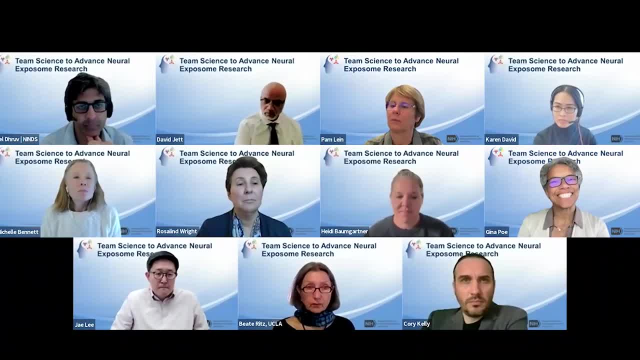 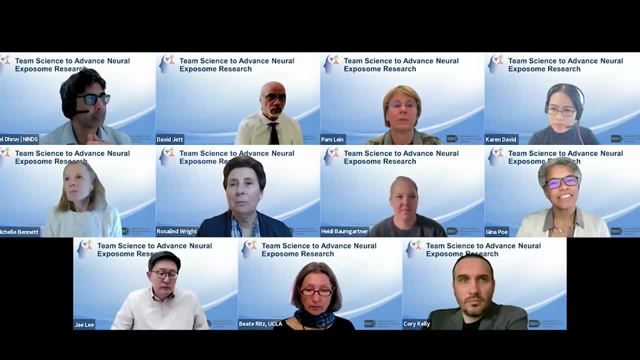 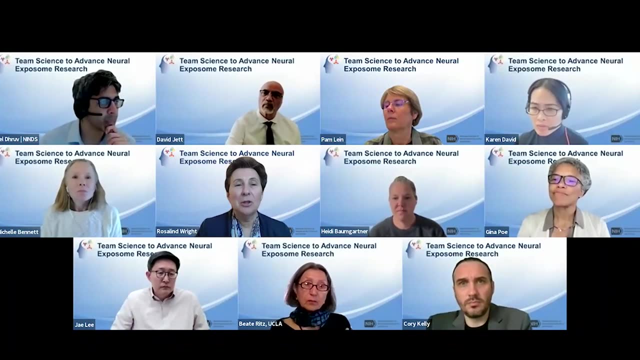 Great idea. Thank you, Rosalind. Yeah, I just wanted to recognize there's some comments in the chat. I know from Gary Miller and then Michelle Bennett that there are. there are examples of being promoted and institutions certainly recognizing team side. they are what my point was. they're not systemically there. 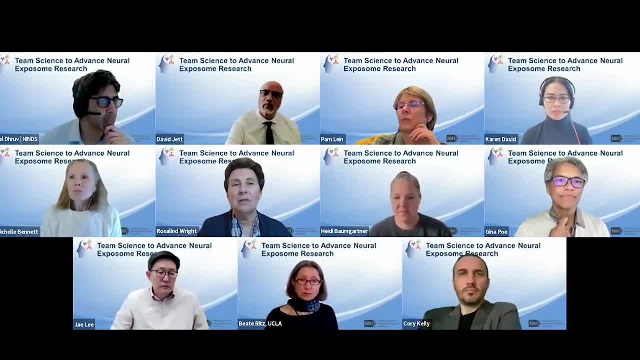 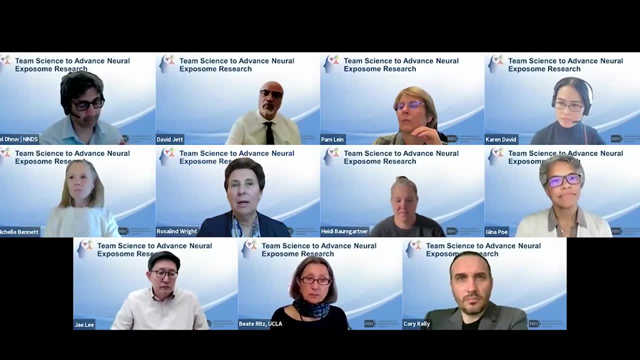 I'm part of the CTSA there, 60. some CTSA is across academic medical centers. I can tell you we spend a lot of time talking about how do we do this more systemically, how do we bake this in, because we do think it's critical. 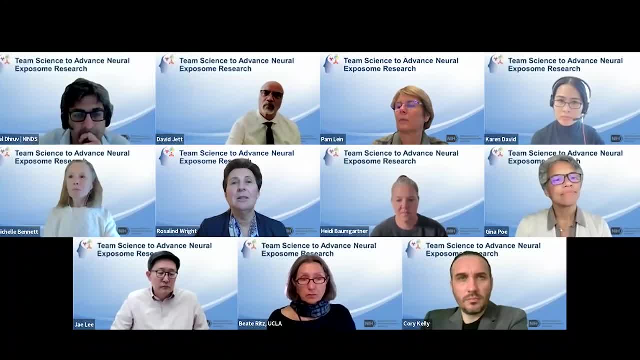 And we're talking about some ways to do it through your societies, to our, our positions, when we're doing ten, your letters, etc. but we have to be, I think, a little bit more purposeful in thinking about how to make that happen more fit, more quickly. that's what, what I'm. 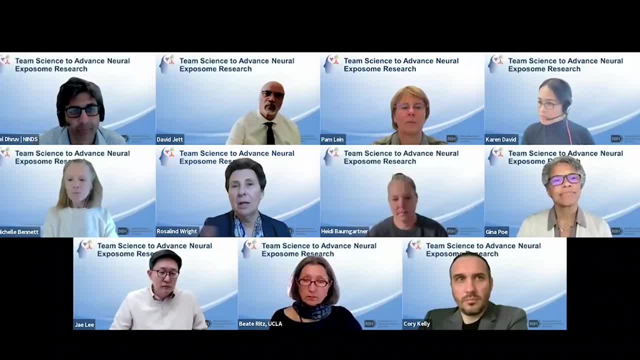 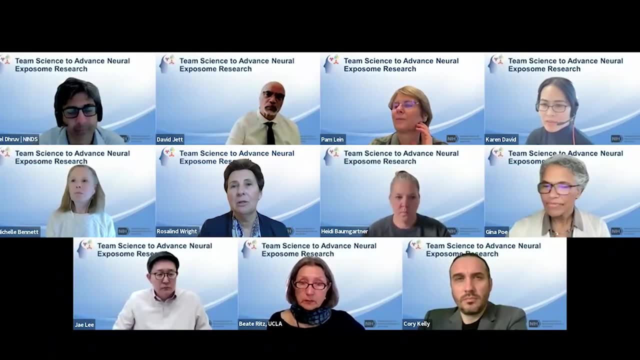 saying. I also want to put a plug in for the echo program- and David had mentioned in his talk that there you're already connected with the echo program- which is the influence, The environmental influences on child health outcomes. so we're starting early in pregnancy, childhood 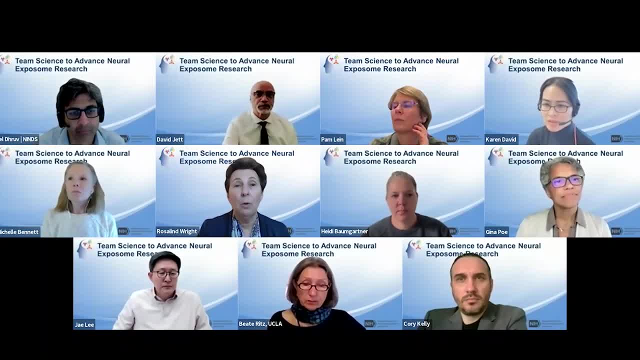 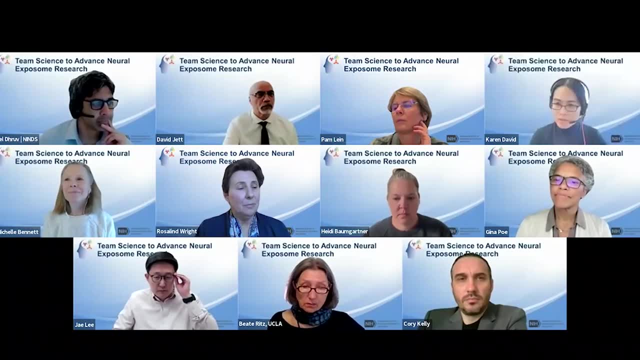 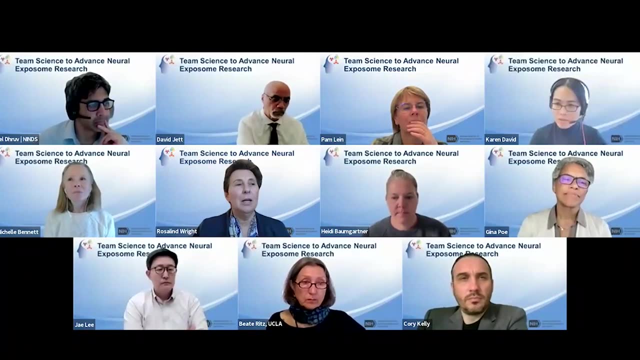 following up neural development is, in neural behaviors, one of the four key areas, the five key areas that, if you call, count positive health, which is key. um, we, you know, seven years ago, we came together, existing cohorts and then coming together and creating a harmonized protocol to 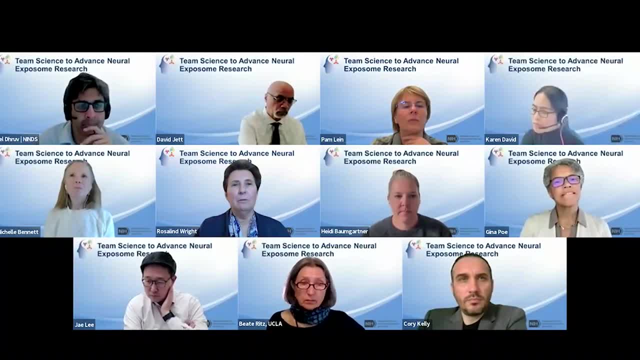 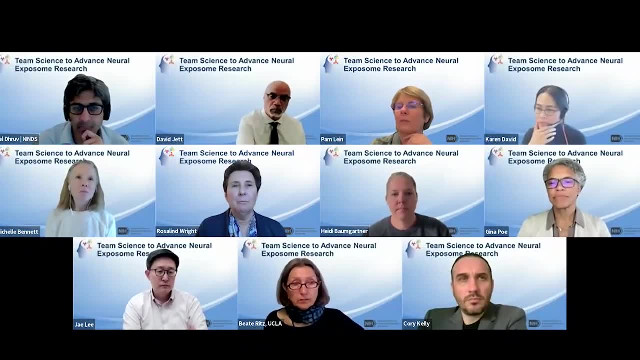 go forward with. and we were, we're, still are. we're very diverse. we're now in the second seven year period, and and and. in the beginning there were people who just i didn't want to get out of my comfort zone. i like the psychosocial. i'm going to stick to that. and and when, and we, we kind of. 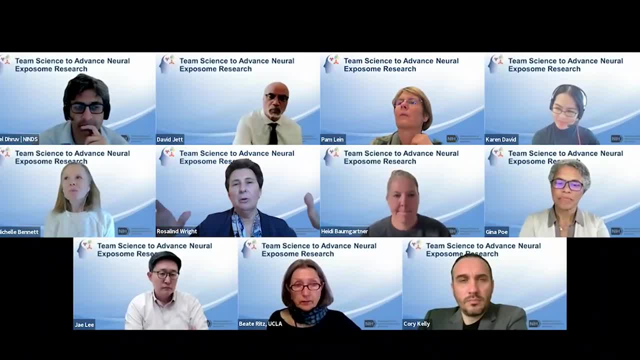 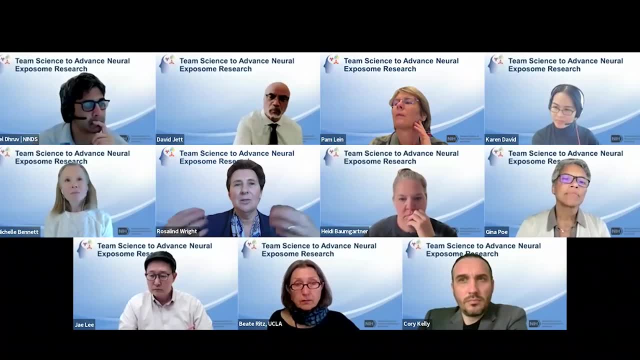 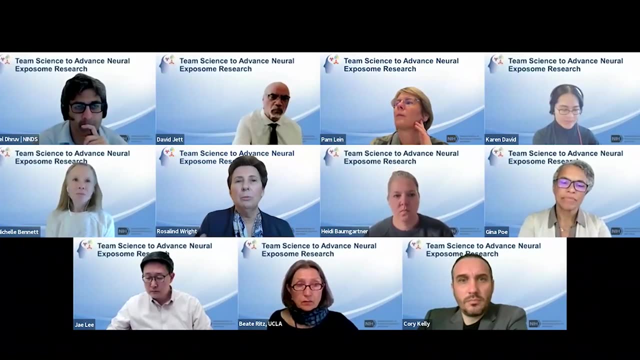 forced it in all of our face-to-face meetings, our ongoing steering committee meetings, the talks that we had, cross-fertilization of environmental scientists with social scientists looking at the same outcome area, that kind of thing, and gradually people started to feel a little bit more comfortable in understanding. 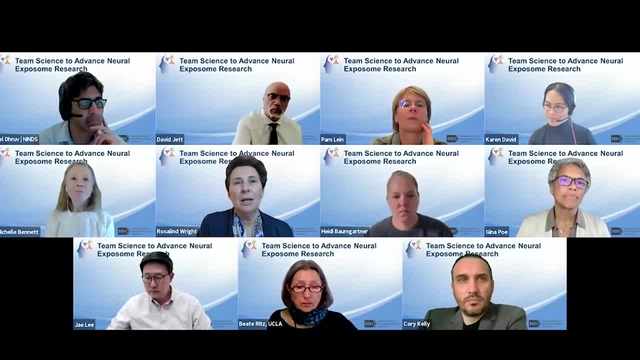 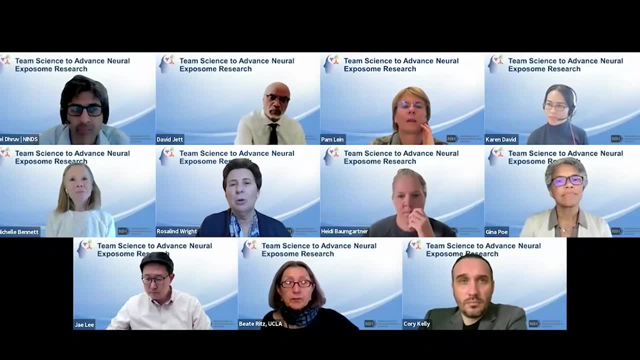 you know, we really do need to think about these two things together. you cannot think of one and in isolation of the other, geospatial, whatever- and again i would say, we don't have to do it all to make big progress. so so that's one way, david, you don't have to put everybody in the room together. 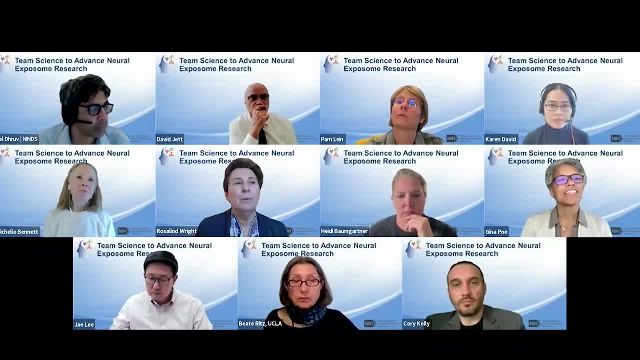 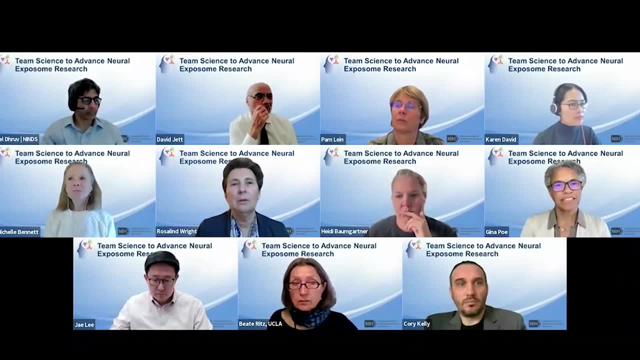 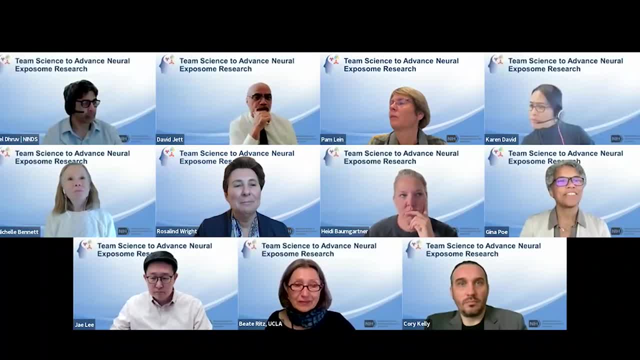 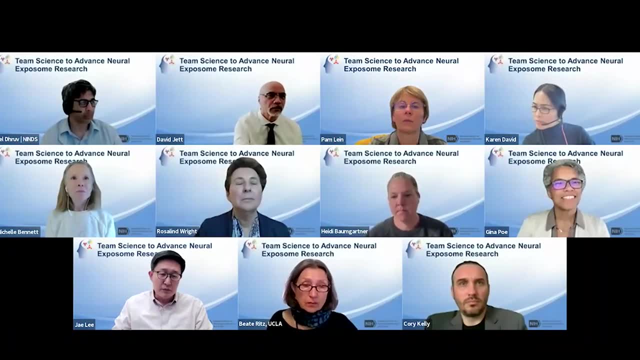 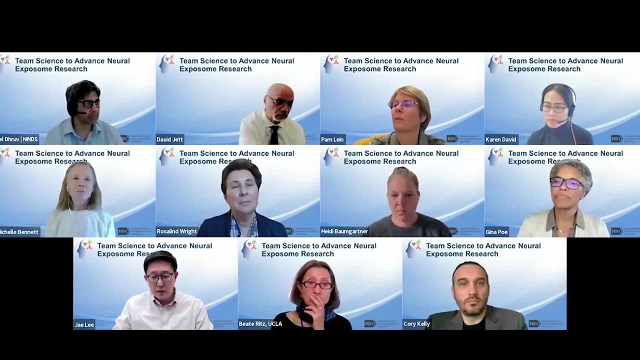 but we're still going to make big progress back and forth. thank you, yes, yeah, with the authorship and, i guess, um contribution issue, we also have a ctsa here and it's it's- uh, it's discussed heavily and it's really a catalyst for team science training, and so we 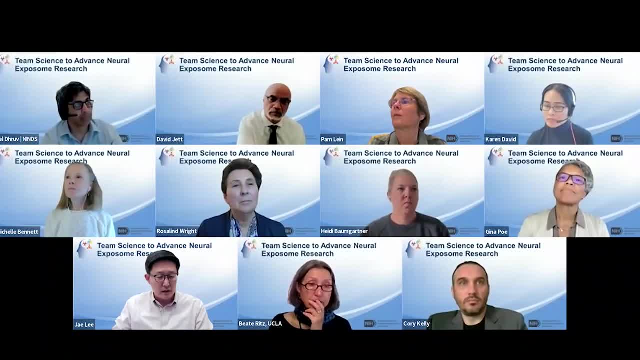 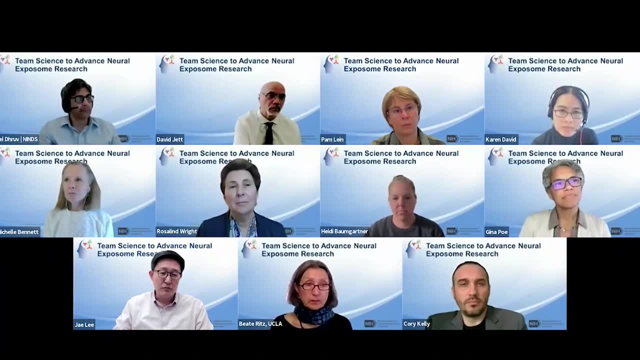 certainly appreciate that at the university of miami- um, you know, we- we have a faculty here talking and coming to me- there are a lot of important things we've done in our. that is, it can be defined classically as a team science player- contribute significantly, and then when it comes to promotion and tenure, you know it's overlooked and so 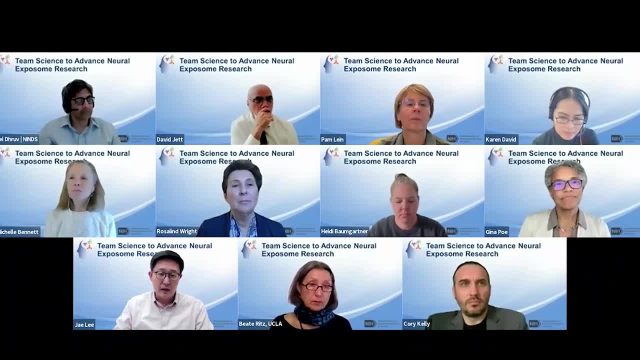 fortunately we have a department chair that recognizes that and really pushes for it. so I think there are mechanisms still in place. for example, if your chair is supportive and is willing to, you know, argue that in front of the promotion and tenure committee. you know those kind of things. 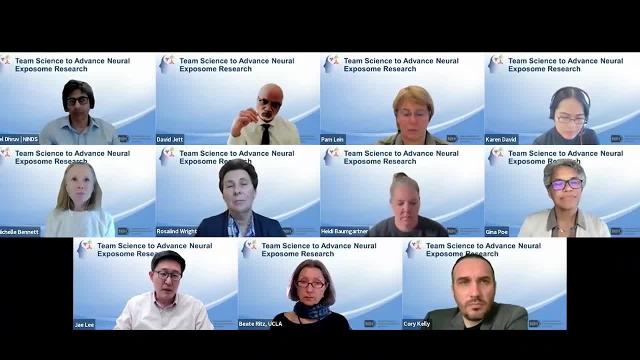 help. but yeah, there are. there are very few systematic process in place. and then I think the I think somebody brought up the contact PI issue at the NIH level and and so you know this is something that I had faced when we got the RM1 grant is that? 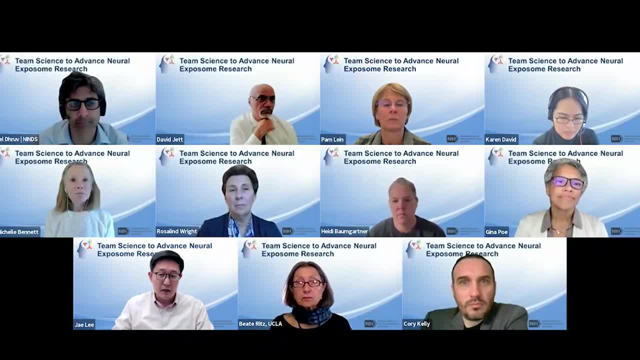 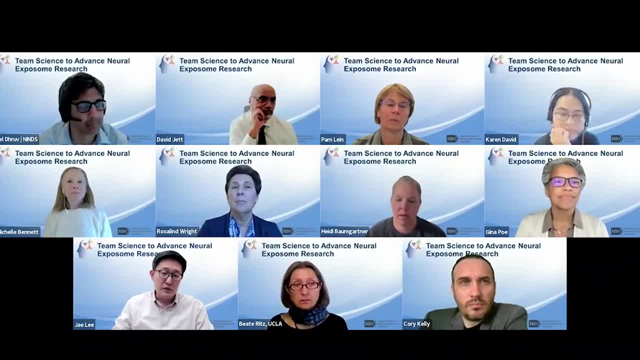 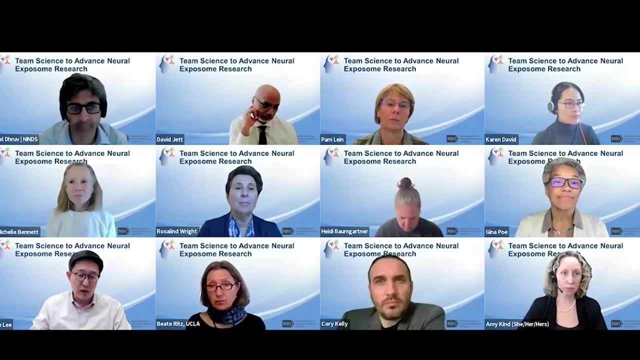 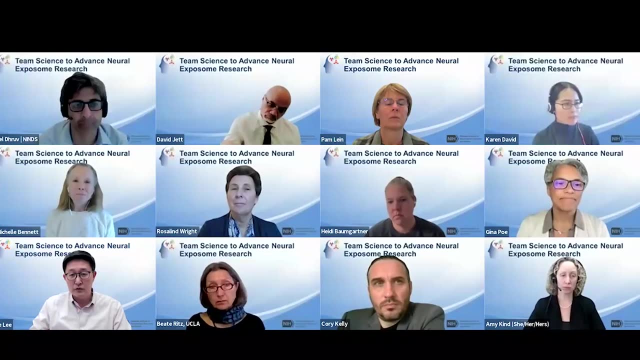 and they're certainly be searchable. but when it comes to things like blue ridge rankings, where they you know, I rank the departments according to NIH funding right. my other co-institutes, Rutgers and um Georgetown, are not listed as the recipients of that right, and and so from their chairs. 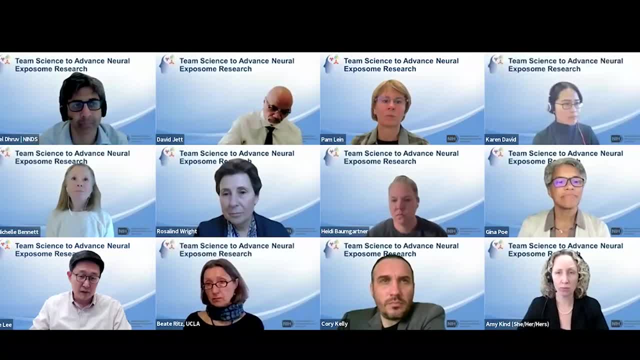 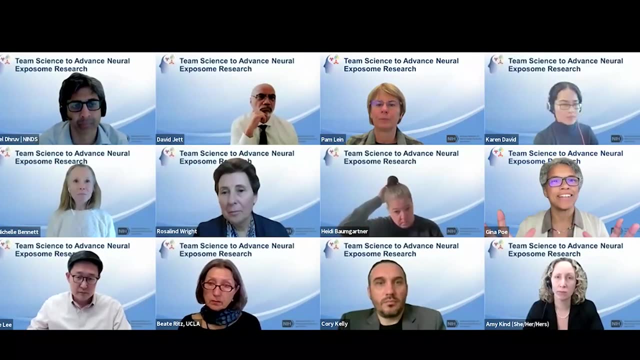 perspective that puts their, the MPIs, at a significant disadvantage. so I think those are, you know, some things that maybe the NIH could possibly work on. yeah, it seems very solvable. and also the authorship order is, you know, the first and last office. that's a very neuroscience discipline. 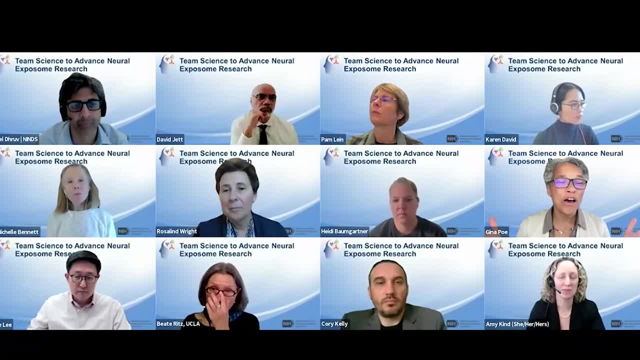 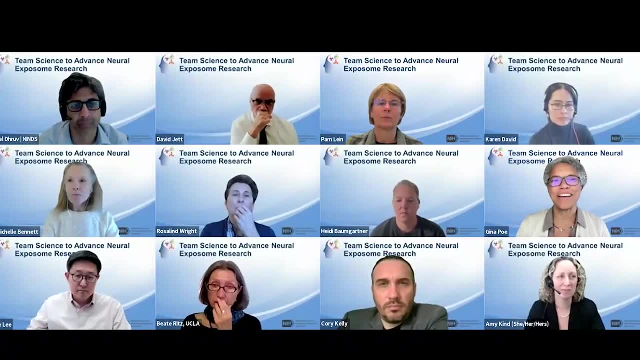 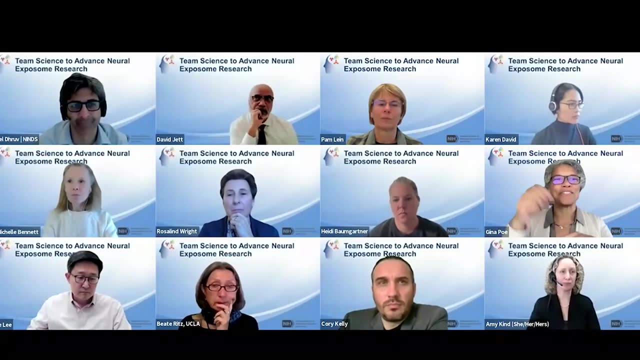 problem. there are other disciplines that have a hundred, hundred, hundred, hundred, hundred hundred authors on a paper and they just list them alphabetically, and so maybe there's a way in this electronic age that authorship doesn't have to be linear, but rather could be a cloud of authors. 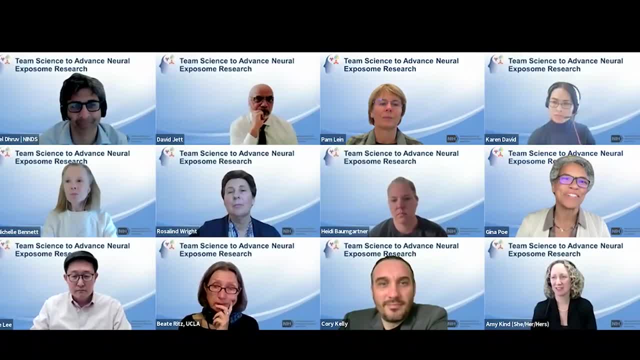 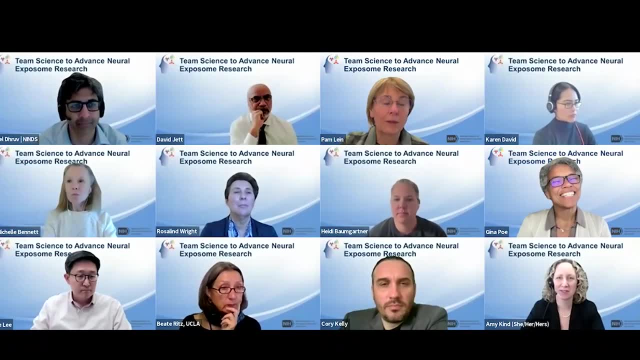 that you could just click on any one person and get what their contributions were, instead of there being a first and last authorship. you know, Pam, what were you thinking? yeah, thank you. um, so I want to ask a question, actually the NIMDS staff, which will be very good. 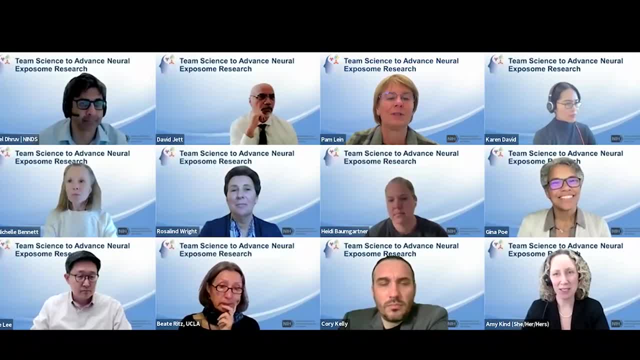 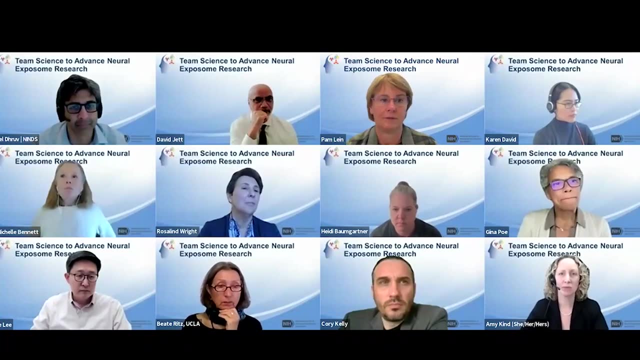 and very helpful for the working group to know your perspective on this, which is um. you know, I think one thing that all the subcommittees within the working group have been discussing is: uh, cross, um, or I should, trans Institute, trans funding agency initiatives, because of the fact that 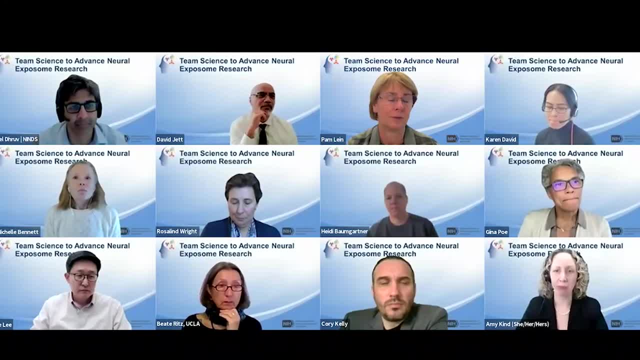 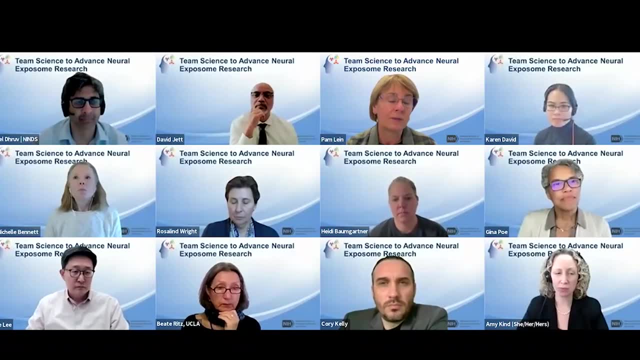 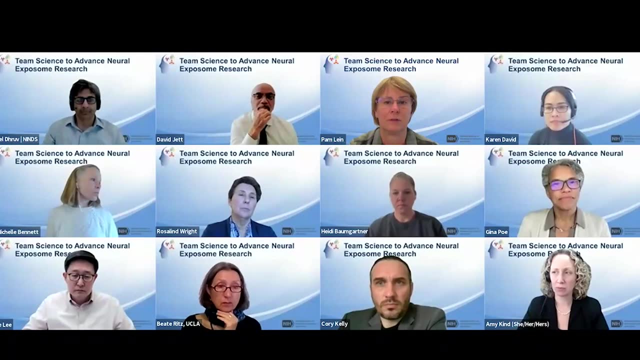 inter interdisciplinary science and neural expose on science. research is going to be very expensive and we understand there are limited funds that are available within any given Institute and that some of the expertise required for exposomic research resides already in other agencies, other other Institutes, thinking primarily, for example, of NSF. um, you know what? what is the reality? I mean is if 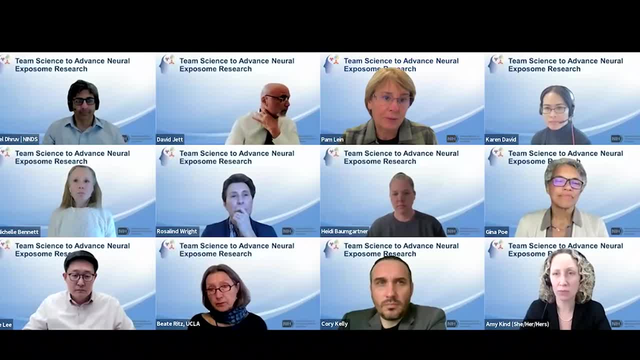 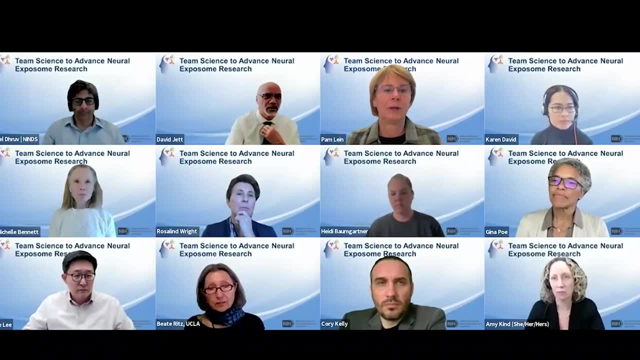 we propose this as a solution. is that something that's even feasible? um, are you know? are there examples of that happening? I know with across Institutes that happens, but it would be helpful to the committee to understand from you all you know, what are the resources available and what are. 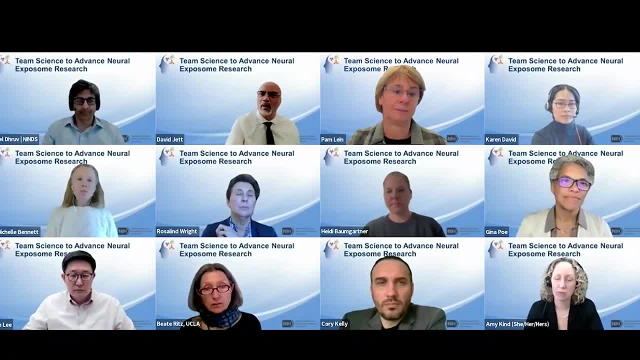 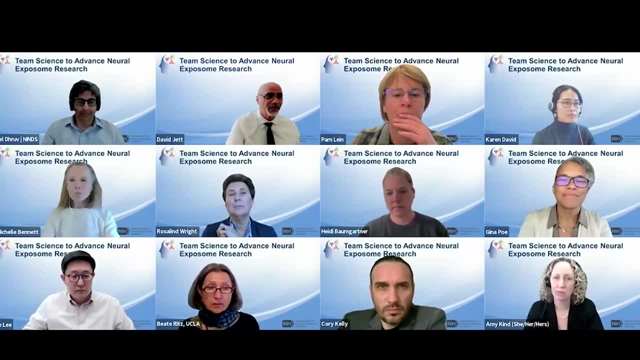 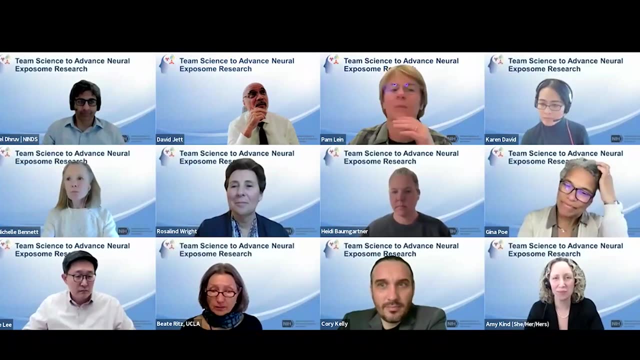 your limitations on really promoting this type of big team science. well, I mean, I, I just type: well, you can tell we've been working together for 30 years or whatever. because I just put that in the chat and I did, I decided not to put it in there. I think that there's one good thing about this whole extra song. 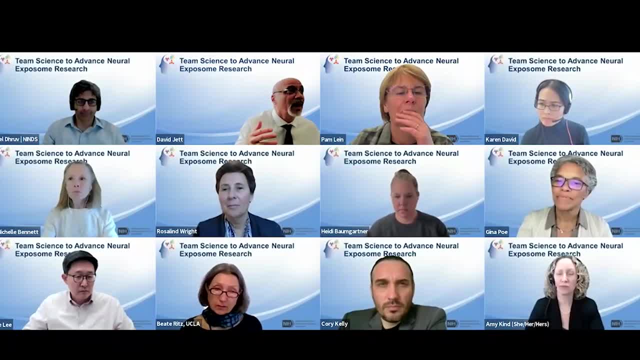 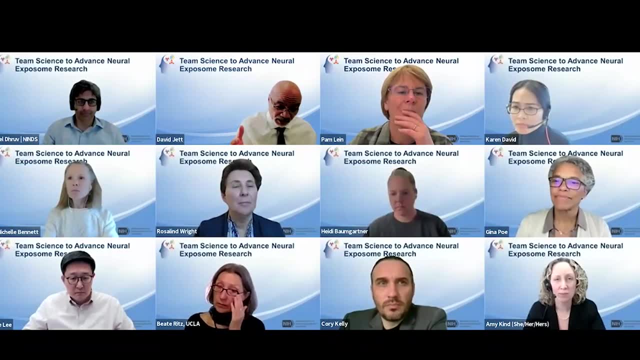 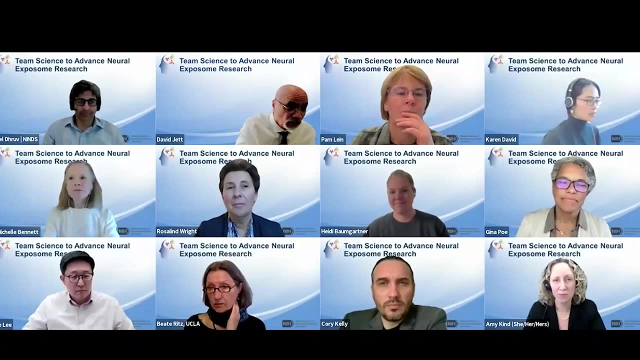 thing, um, how should I put this? I'll just say this: it's actually bringing the ics together. remember, I just talked to you about the thing where any social and chemical and sleep and climate, it's not gonna work without collaboration among the ics. no chance, no chance, and so, um, I have been 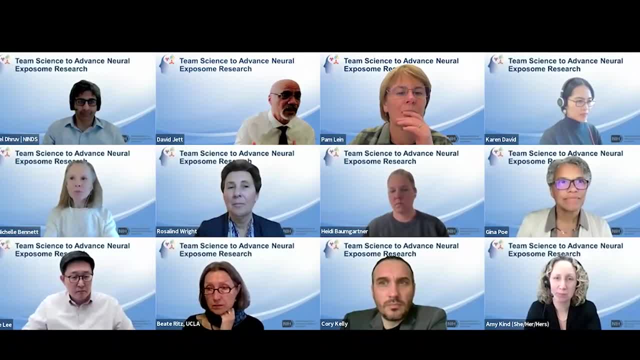 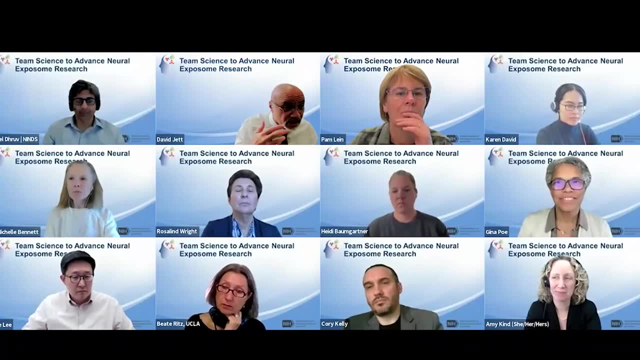 here forever, but I have never collaborated with more ics in the last two years than ever out of my two 20 some years here. so it's, it's, it's coming along, it's coming along. we have to understand that this is not about you know who has what and who doesn't have what and all those things and competition and everything. 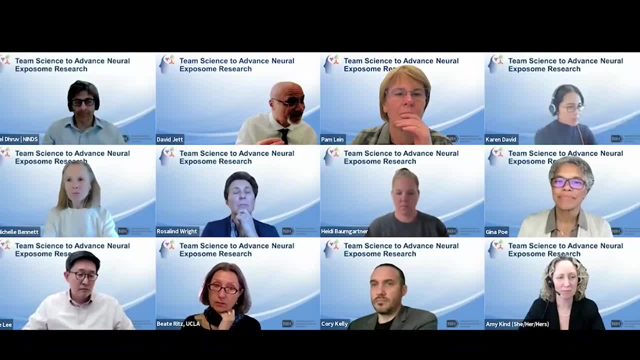 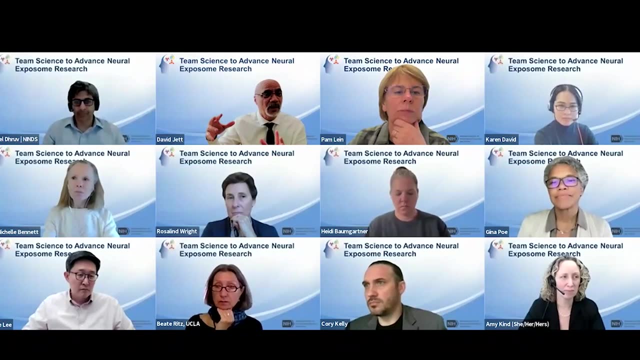 it's about, it's not going to happen if we don't do this, and everybody's starting to get to that. so I'm I'm actually pretty optimistic on this and I have been. I can list with you know, certainly in IEHS I mean we have, for instance, we have a um environmental, an NIH environmental, uh group. 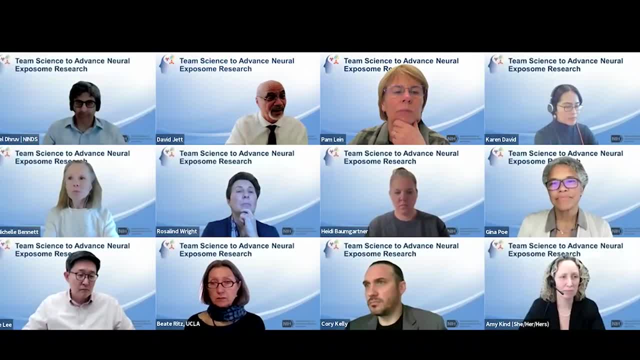 and the co-chairs are me and one from uh in IEHS, and so things like that are happening now and I'm optimistic that it's going to be even better, as we realize we have to do this, if we're going to do it, so and everybody's on board with extra song. 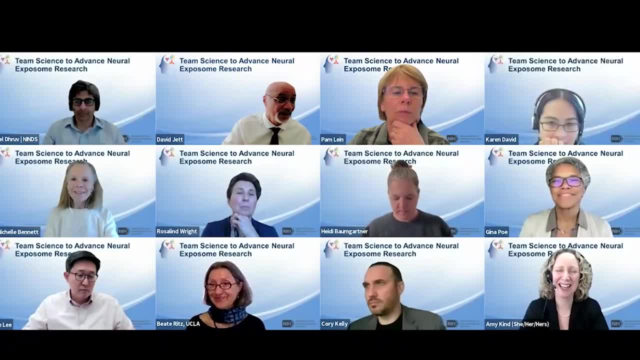 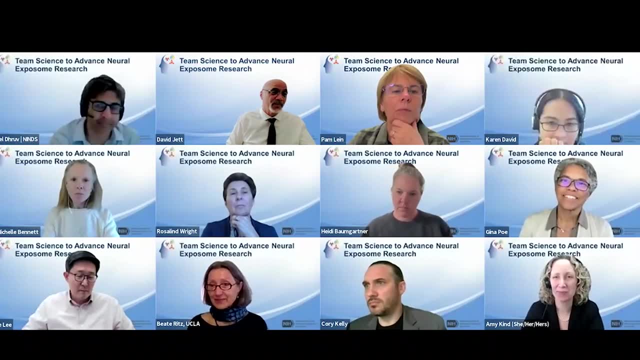 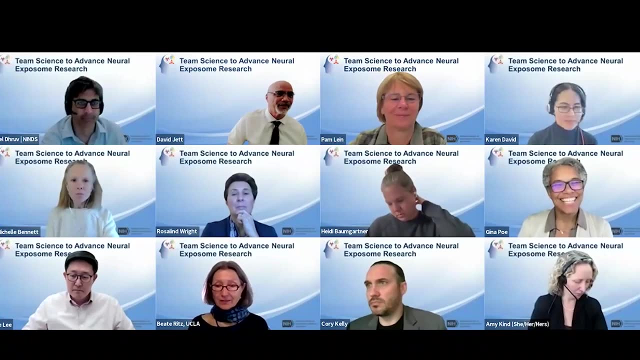 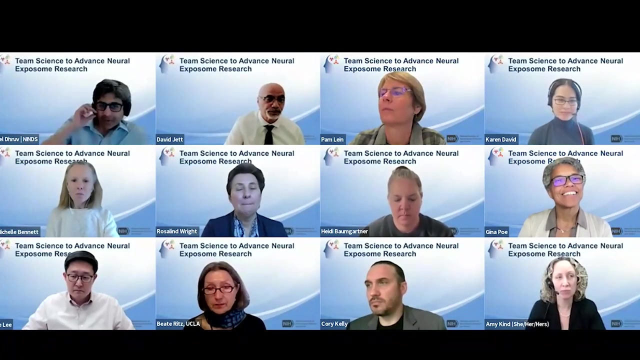 at first it was like: what is it exosome? now everybody knows what it is and they're, they're, they're getting, um, really excited about it. so I, but you've got, really you took it out of my head. yeah, Neil, thanks. uh, just while we're in between, uh, some of these questions, I just have a logistical thing. 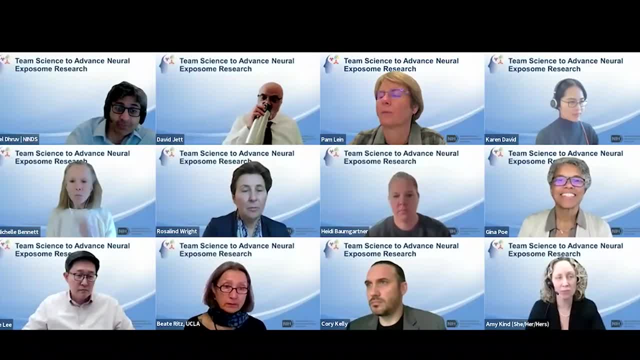 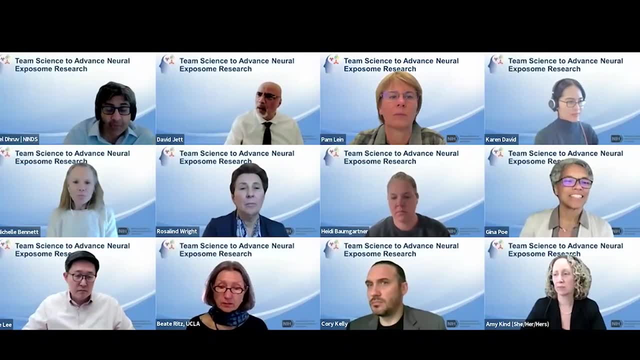 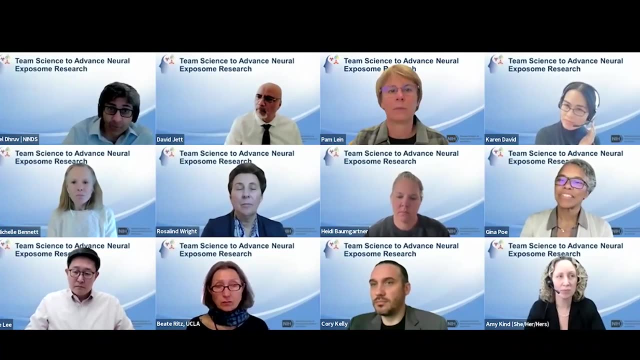 which is, I know, um, we're at the end of our scheduled time and I understand there may be some people that need to drop off. that's totally fine. I think we're going to keep this going for about another 15 minutes. if you uh have to go, that's fine and um, you know, once again, we're. 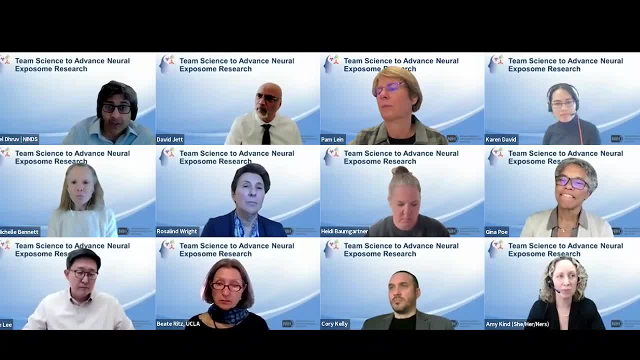 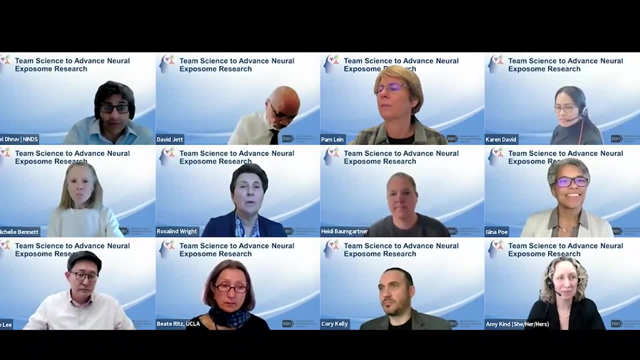 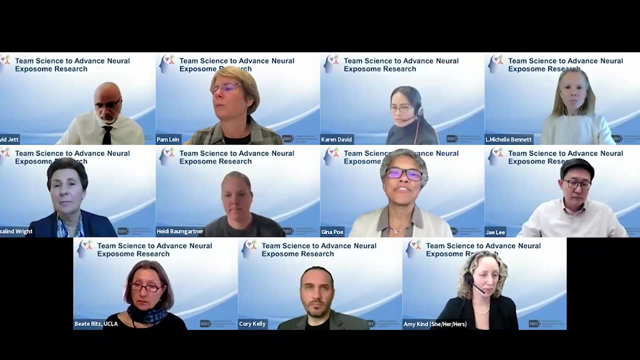 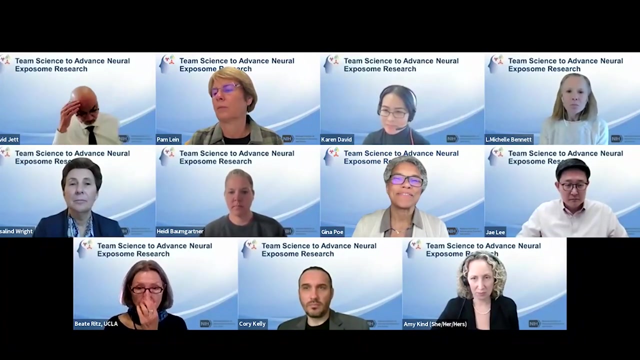 recording the uh, this workshop, and I'm going to share it with everyone that uh has been here, the panelists, the attendees, uh, everyone. so thank you all. thank you, Neil. yeah, has anyone not been able to um contribute to this? have things to say? how about Amy? how are you? what are you thinking? what's important in your mind? 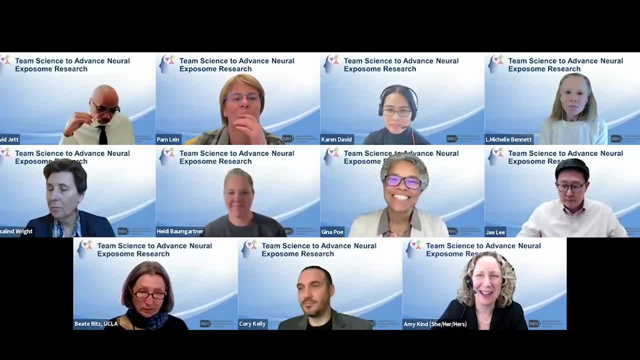 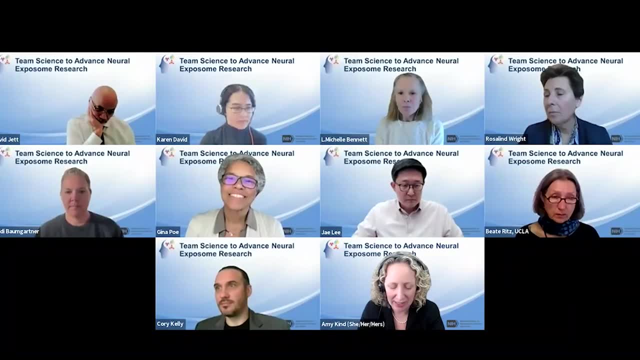 oh sure, thank you so much for for, uh, asking, I've been listening and just really these presentations over the course of today. This has been a wonderful, wonderful session. One of the things that I'm reflecting on in thinking of team science is, of course, 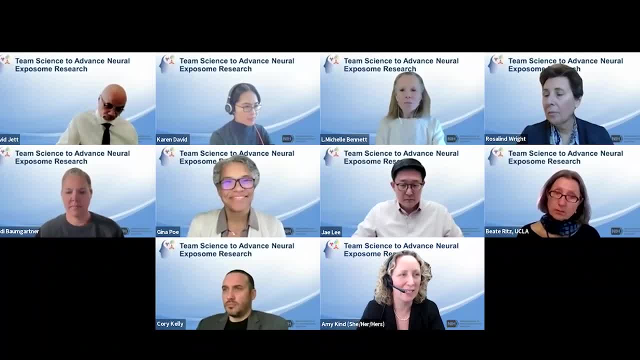 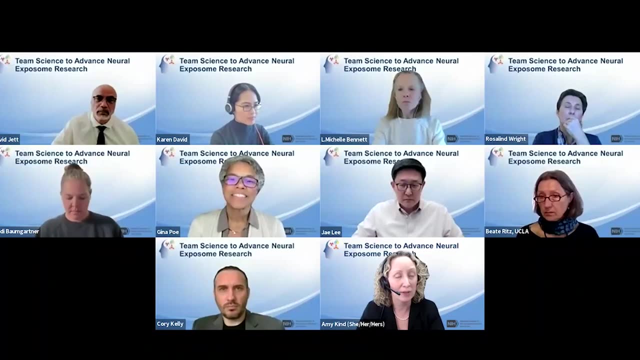 thinking beyond the academic bubble and thinking into the community, into different decision makers at all levels that potentially could hold both resources and access towards intervention, towards mitigation of some of the adverse exposures within the exposome. And I would be so interested to hear our panelists. 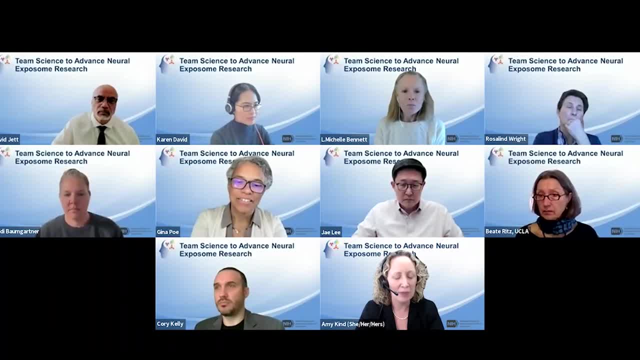 and the group consider that and consider thinking about partnerships beyond the traditional academic and research ones. So perhaps weighing in on that and weighing in on the different infrastructure and processes that would be required to facilitate that most successfully, That's a great question, Thanks. 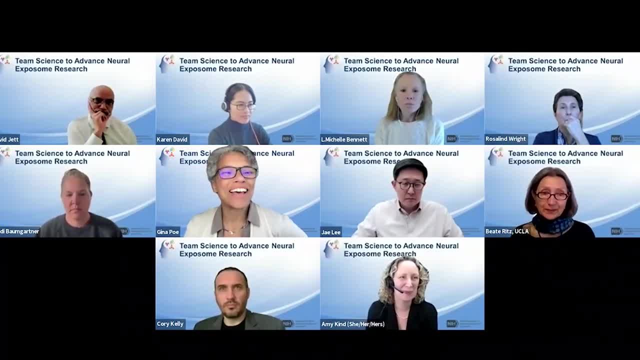 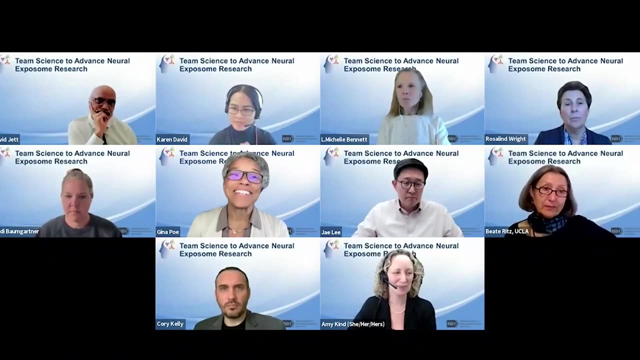 Who wants to tackle that one? Has anyone reached out outside of our traditional academic scientific enterprise to collaborate on a neuro-exposome or other project? How do you, for example, gathering community? Yeah, Piere, Yeah, I think, for environmental scientists? 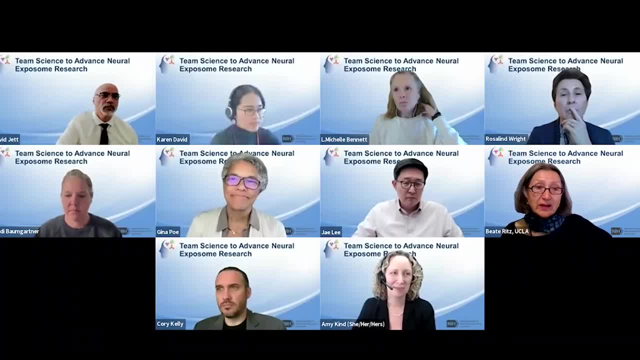 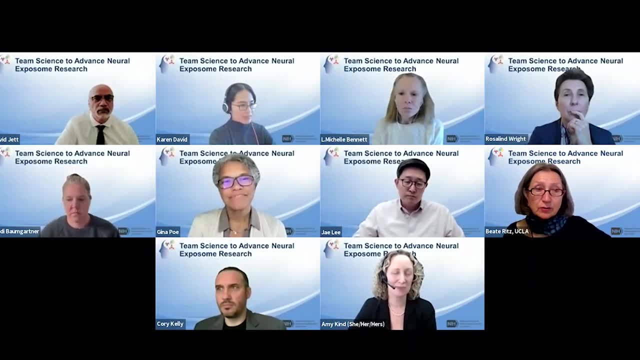 it's a natural. you know, we cannot study environmental causes if we don't go out in the community and we talk to people in the community and to leaders and we engage with different stakeholder groups, either patient groups or you know. 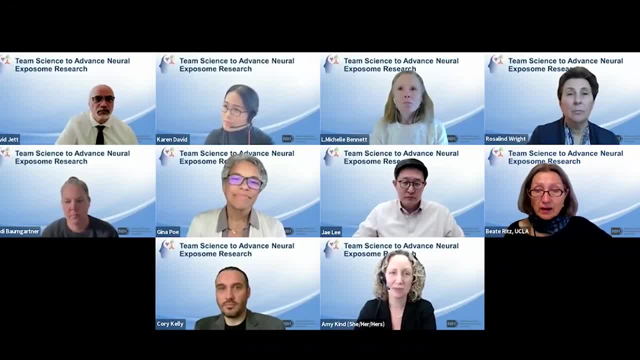 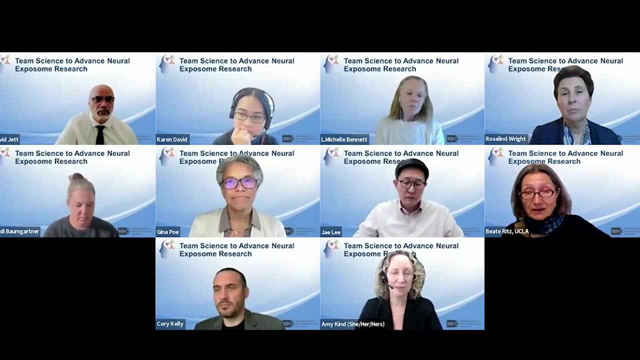 community activists, et cetera, et cetera, And I think the best model for this has been NIEHS. that actually has been funding within the center, grants a lot of these community outreach projects and actually made them mandatory. And because of that, 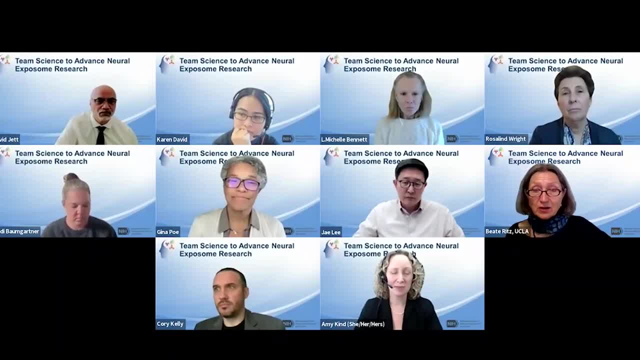 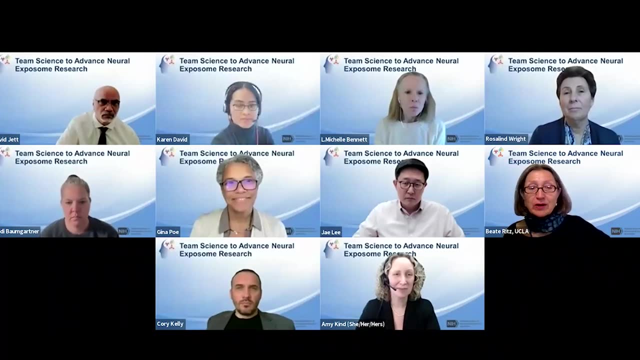 a lot has happened on the community side And there is a lot of collaboration, a lot of collaboration going on. When we talk about lab science, that might be a lot harder because you know it's a disciplinary issue. However, when it comes to sampling, 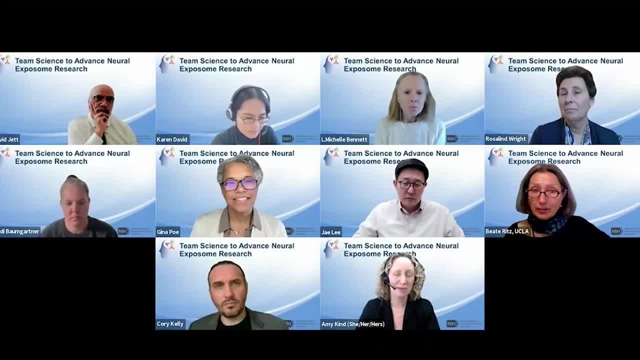 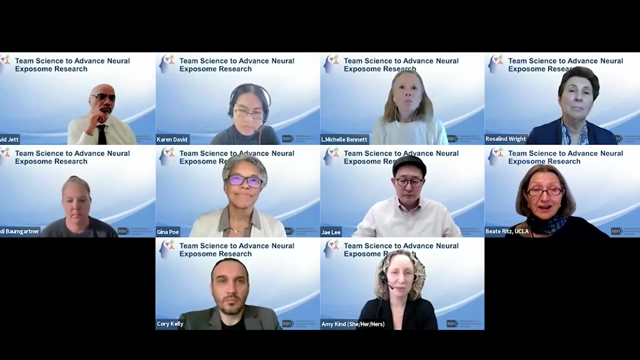 and when it comes to maybe engaging with partners in the community that disseminate information that you know, reach out to schools, reach out to certain groups and make the information that we generate in the lab then available to the community so that they can participate in that way. 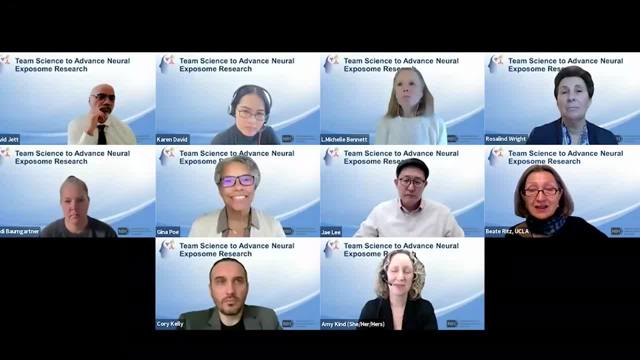 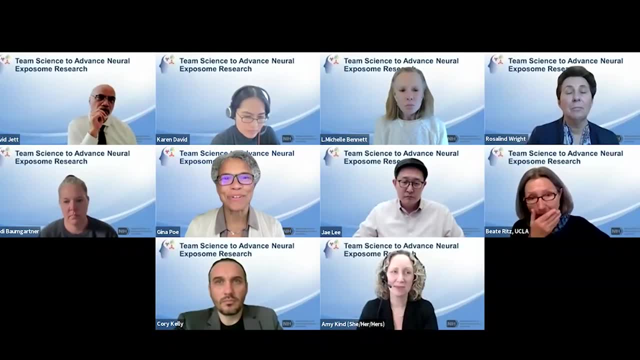 And there's an actual dialogue about it. I think that that makes a big difference. Yeah, I think your point about dialogue is important, because we have things we can learn. We're not- we tend to think of ourselves at the peak of the ivory tower. 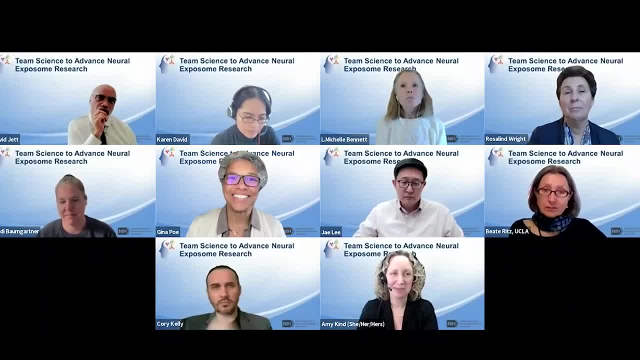 but in fact, you know, we're all community members too, And we learn from that. We learn from each other, So we need to listen just as much as we speak. I love that. Yeah, Rosalyn, Yeah, I would agree with everything that Beata said. 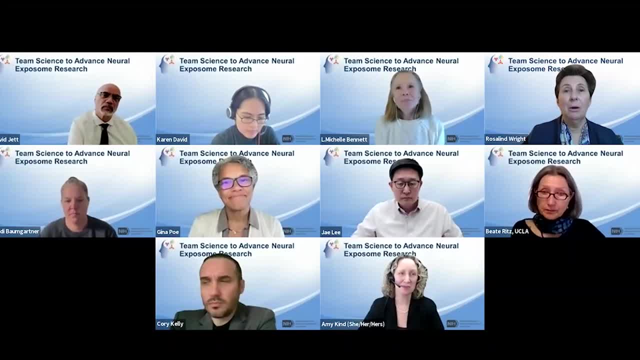 NIHS is a great example of that. Environmental health researchers have been doing this in a major way for quite some time, And you have to- I mean I can't- every time I've reached out to community in different ways. what my prior was of what might be the priorities. 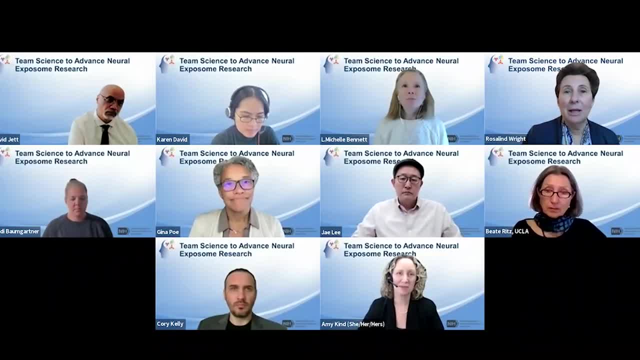 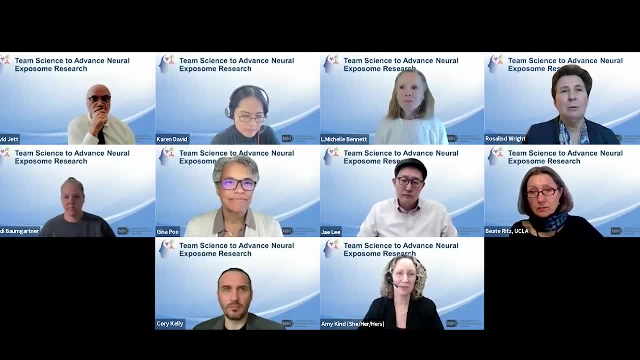 and the things that they're concerned about often turn out to not be the case and things that I might. you might think, oh, I'm going into community with lower resources, et cetera, on the macro level, And you go in and you just find amazing things. 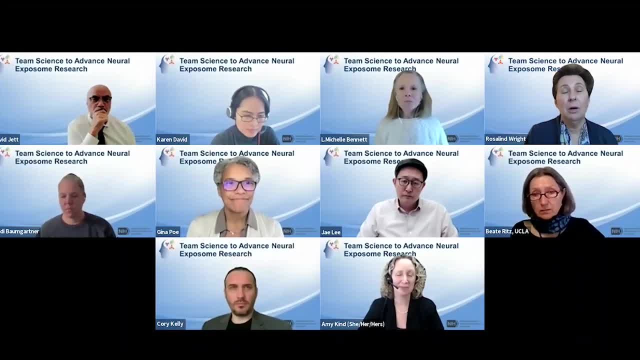 about resiliency factors And I would always, I would also say to folks: we're not just when we're looking at the exposome, we're not just looking at the risk factors, We're also looking for the resiliency factor. 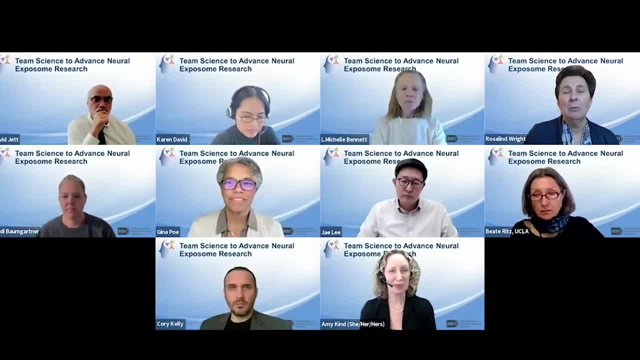 There's a balance all across the life course, right, And some of those might be nutrition. Some of those might be social connectedness, right, Some of those might be nutrition. Some of those might be social connectedness. Some of those might be social connectedness. what have you? 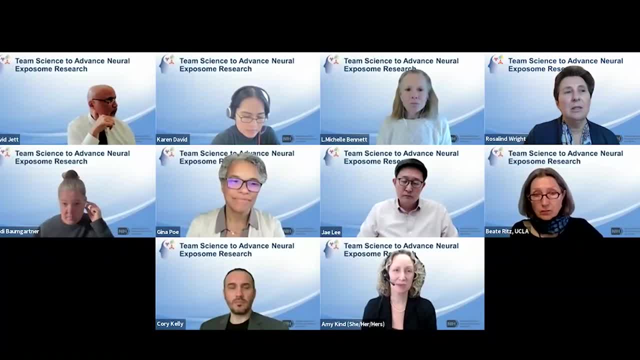 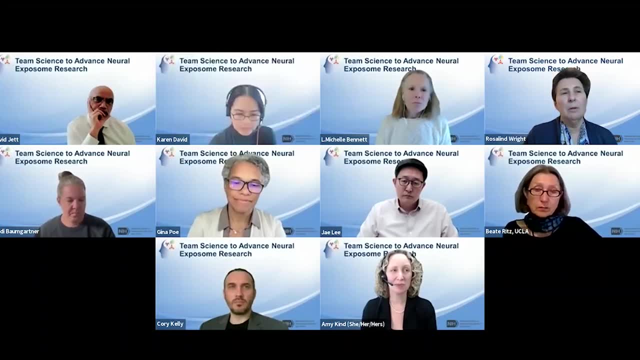 And again those are very broad. It's, and I think, climate science and climate change. And when you're coming from an academic medical center, academic medical centers are actually drilled in on climate change and how it's going to affect healthcare delivery and needs. 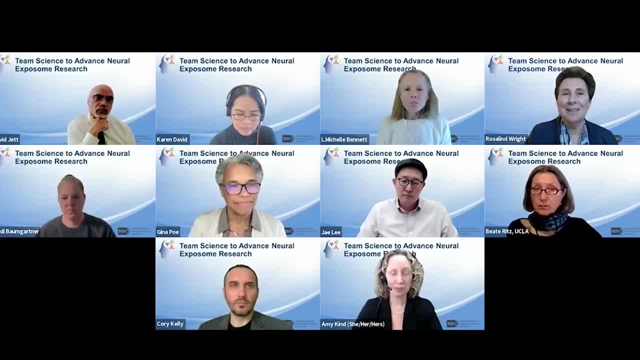 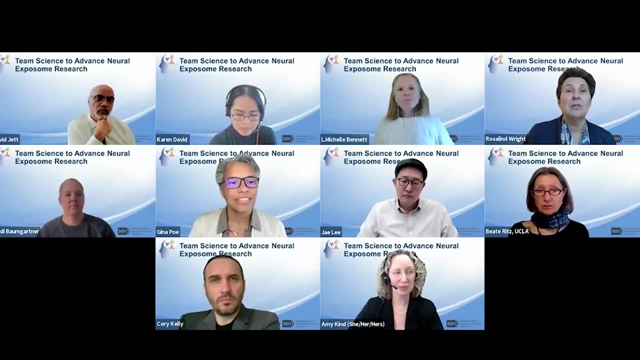 And it's the that's a lever we could pull, because we know climate is going to affect all these aspects of exposome that we're talking about, from the social eco-anxiety to, you know, to air pollution. differences, changes in, you know. 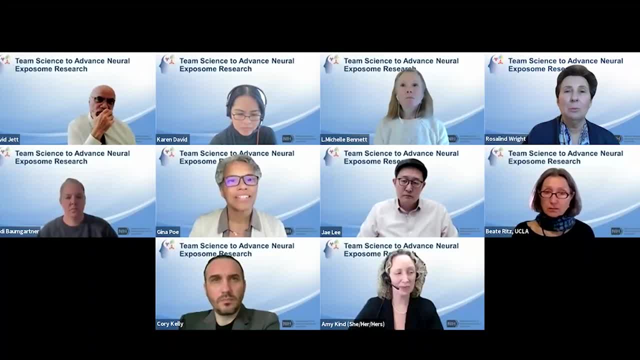 wildfire smokes. I mean New York city was the most polluted you know city on the planet. on June 8th this year I was sitting in my office, all of a sudden dark at 2 PM. We're seeing things. we're all experiencing it. 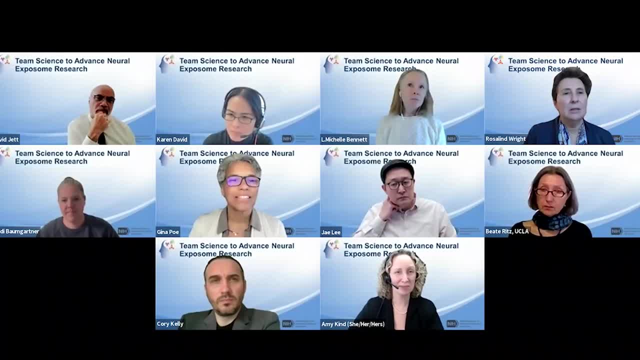 People are keyed in. I think it's a good thing to think about leveraging And for more funding for getting the ICs together around, and, whether you're focusing in on neurosciences or other things, I think that that's that's important. 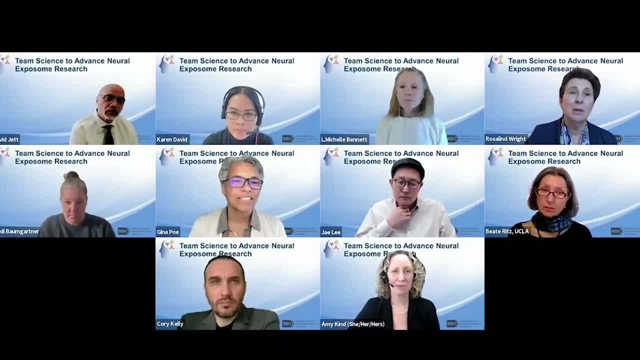 And it's important to know that all the academic medical centers know what's going to cost them and they're laser focused And so we're. you know you got to kind of pick up on those trends, I think, and take advantage for things you're trying to do. 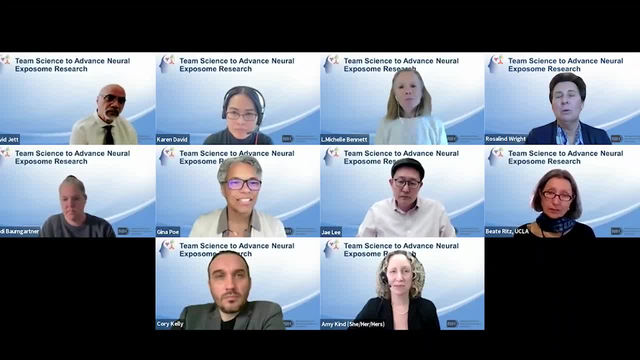 And and I and I, we're doing that in our communities. We're we're spending a lot of time in our communities now teaching them how to use GIS mapping to just on a level where they can actually start to see. oh my goodness. 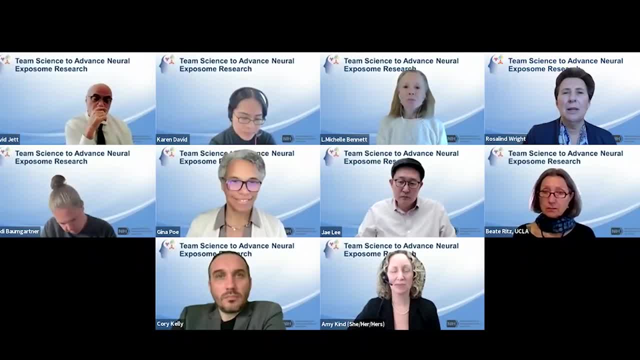 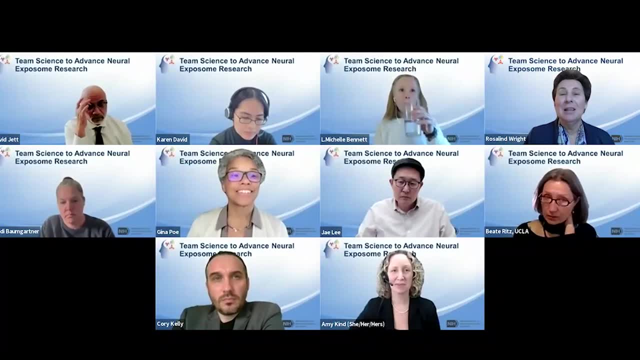 Yeah, this is what happens. and and crowdsourcing- Someone else brought that up in in one of their talks with you know I forget how many countries across you know that was amazing to me. tools like that- Yeah, I think it's. there's a lot. 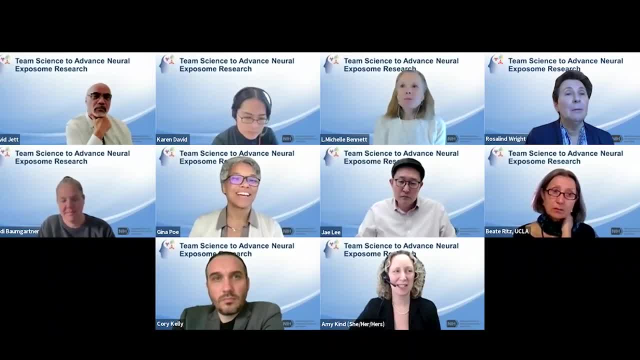 of exciting things going on in that area. Yeah, I totally agree, Amy. Yes, So I just love these responses that have been offered by Rosalyn and Vita and I I must. I just like to expand on it a bit. 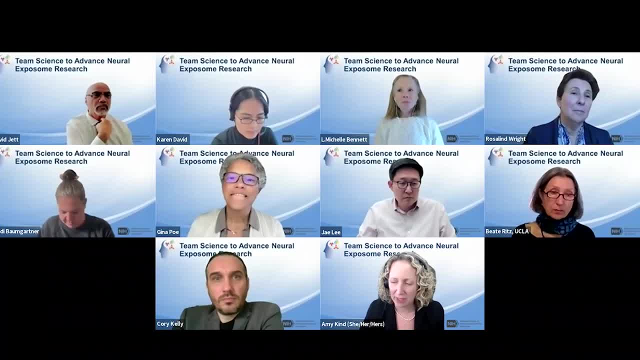 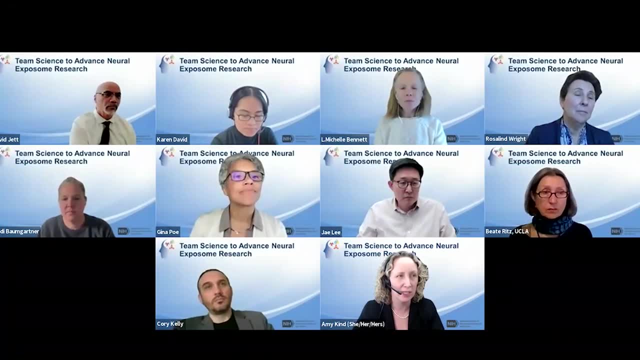 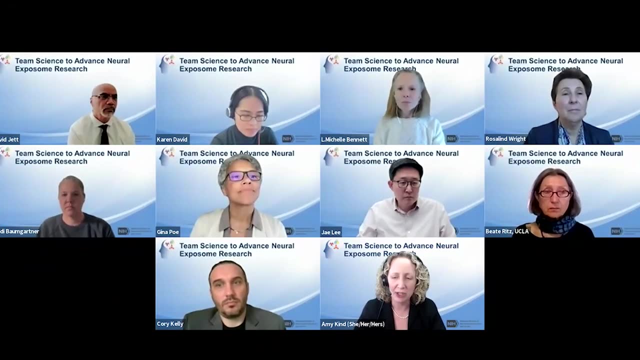 I was just actually at a community action panel last evening about lead and lead poisoning and children's lead concerns within a deeply disadvantaged inner city neighborhood context, And I've been involved with a number of these community initiatives And one of the things that I think is incredible. 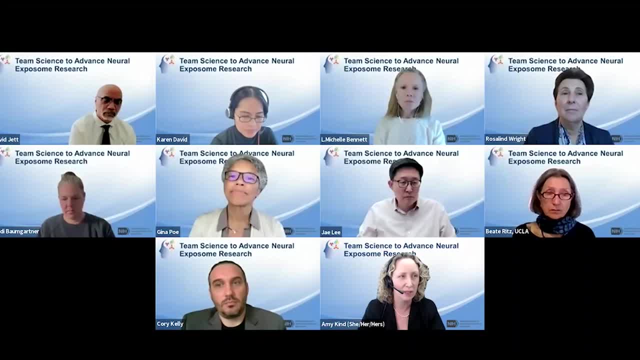 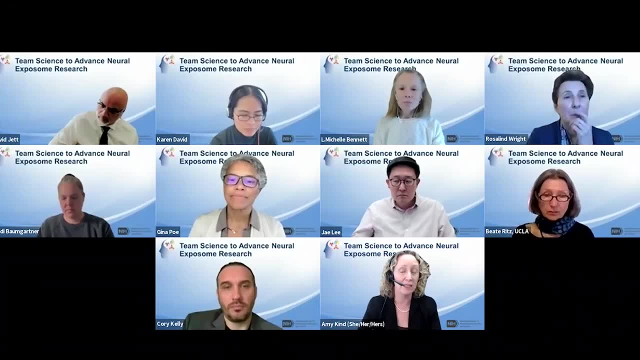 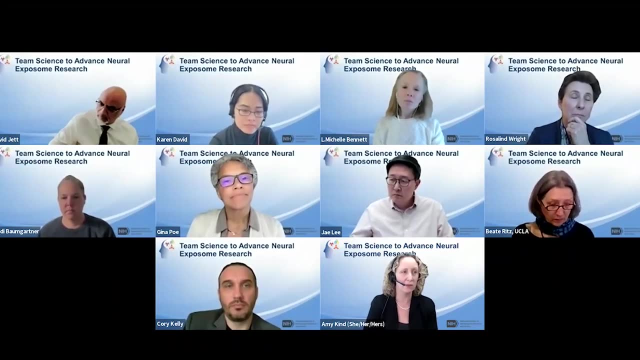 and incredibly important is to recognize the power of the community itself as an intervention towards the exposome and also the incredible motivation that I, at least, I have personally seen in my own experience that communities at the local level, county level, city level, will take this information and and move it. 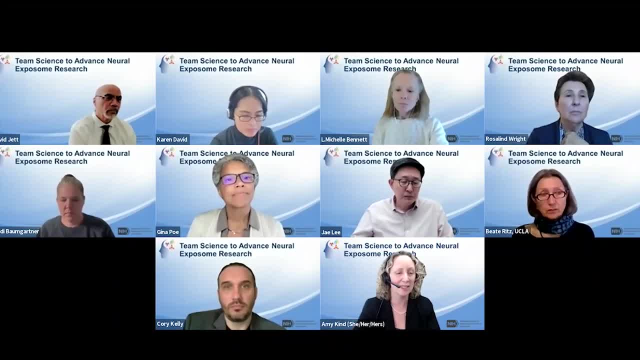 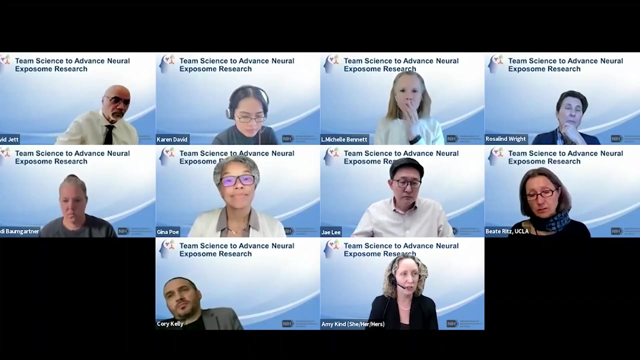 to action ability quite quickly, in a way that doesn't necessarily rely directly on NIH resources or NSF- the traditional research resources- but could potentially form the kernel of a really wonderful natural experiment And thinking about resilience and change in intervention from a policy or community action level. 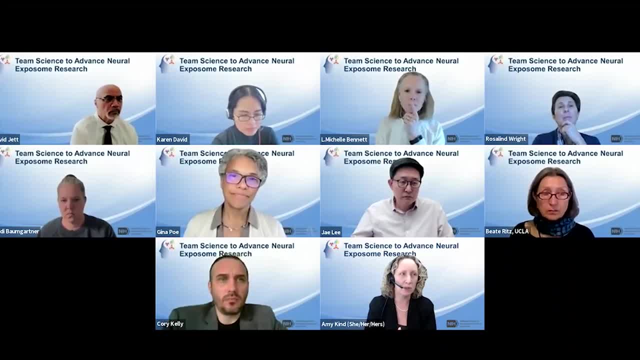 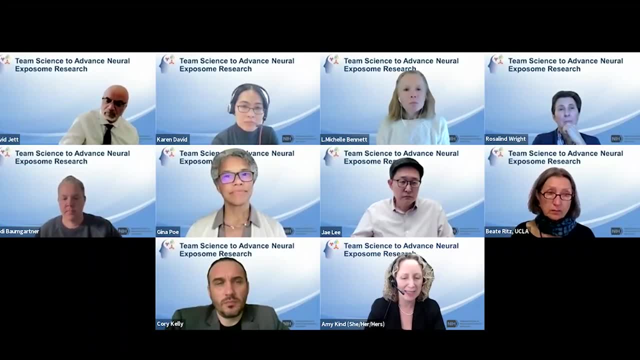 So just to put a plug in for that, for the importance of science that truly integrate some of these community levers in a way that potentially could rigorously assess the outcomes from an exposome level and follow those forward. I think there's some great examples that are going on now. 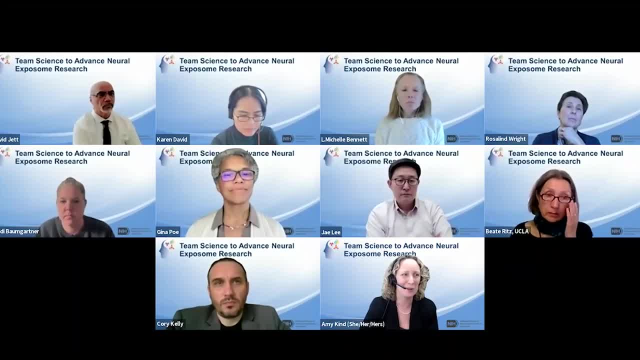 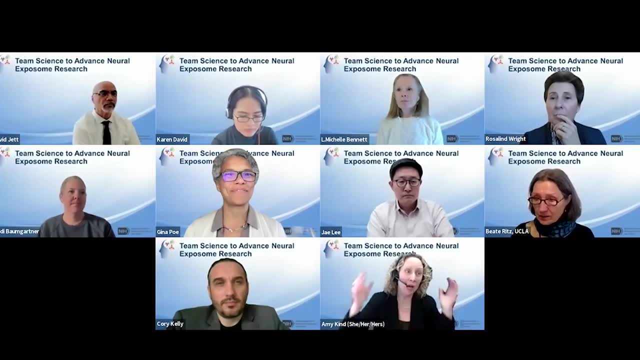 but of course the science would have to be nimble and quite pragmatic. So, exciting times though, Absolutely. Can you give us just one example? Can you think of one? Well, certainly, with the work that we do, we partner with communities all the time. 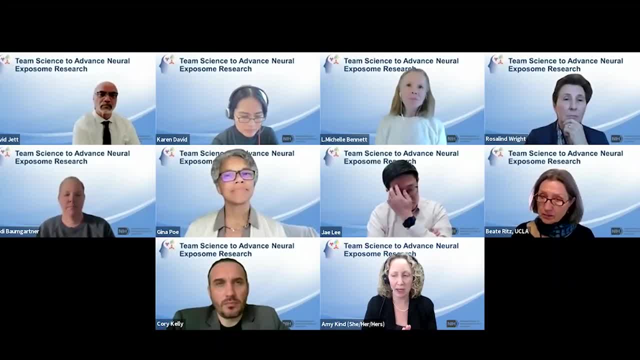 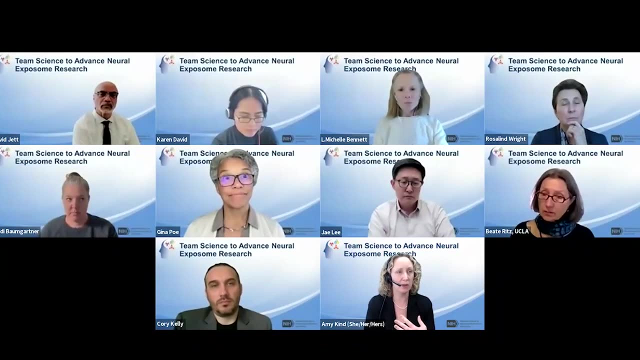 Let me just bring up the panel that I was involved in last evening. We were trying to bring together different groups around childhood lead poisoning in inner city Milwaukee And it has brought together the waterworks department about how things should be targeting and what types of algorithmic approaches. 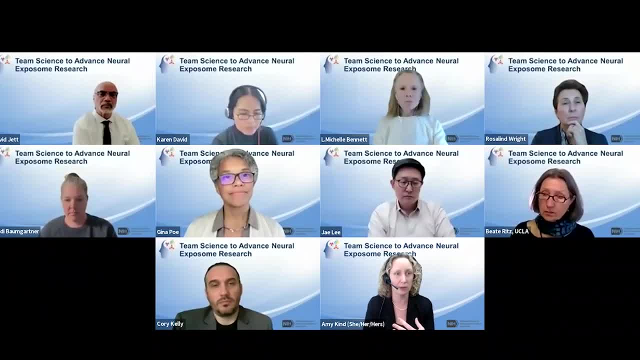 and data should be used to prioritize where those backhoes are sent and where the resources are sent Family members to understand that they need to advocate for themselves and their children at all levels. Different lawyers were there talking about how different types of policy changes need. 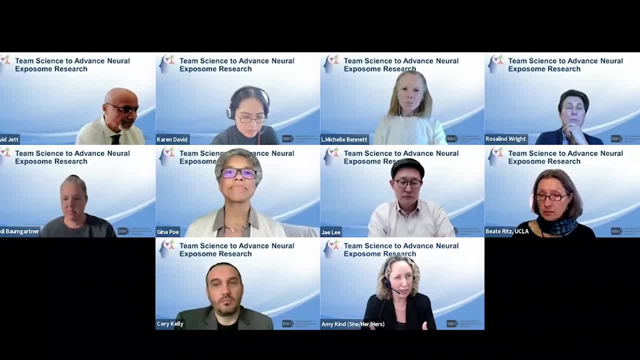 to go forward, and then city officials were there as well, And when I think about that kind of impetus that is going forward, the potential to follow that, to document and to study how effective or unaffected it is towards some of these locally targeted initiatives, 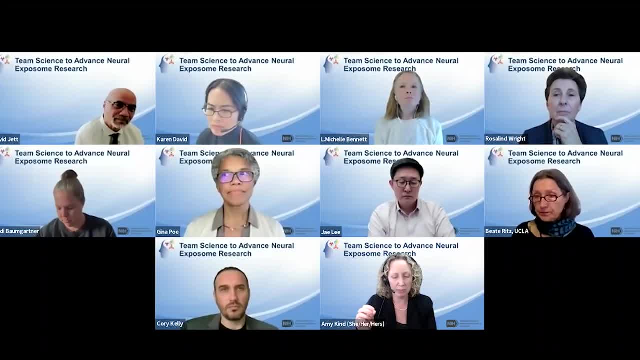 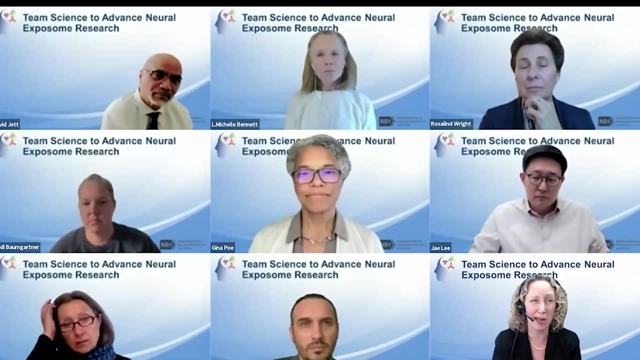 at least in the city of Milwaukee. their approach, instead of being reactive to lead level detection in children, is to try to take a proactive approach right now, but to target it on certain most disadvantaged zip codes- just a very small area, but it accounts for probably 70% of the lead poisonings. 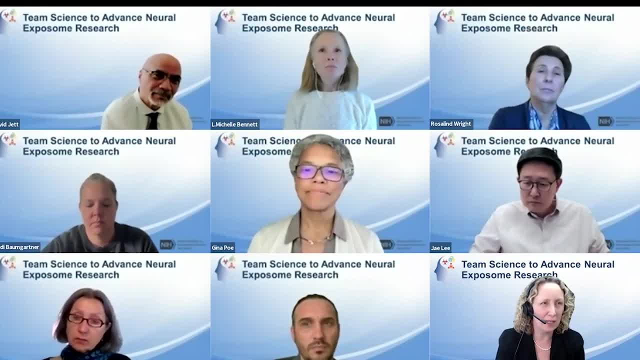 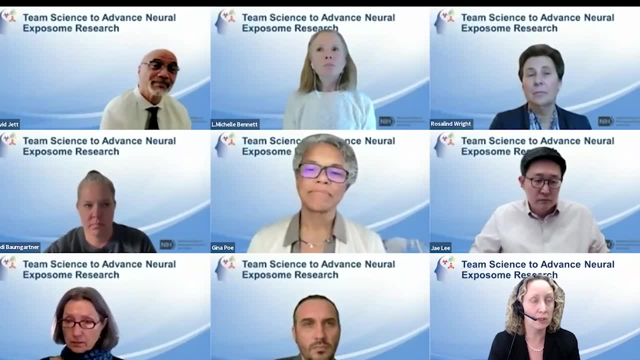 in that particular city. So it's a really kind of innovative approach from a policy level. And I'm seeing this in other cities across the country. We've all heard of Flint, of course, but these issues of this intersectionality of our inner city, crumbling infrastructure. 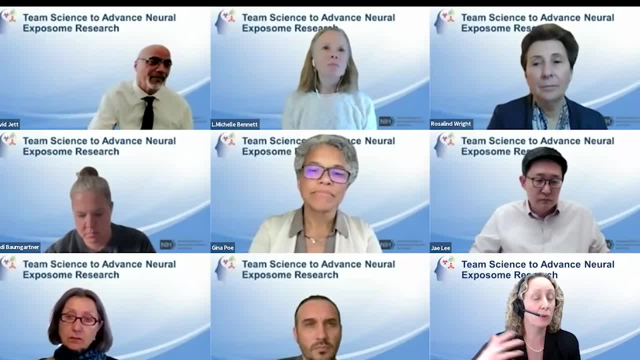 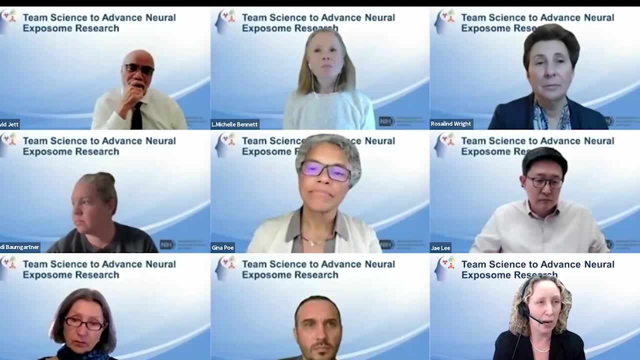 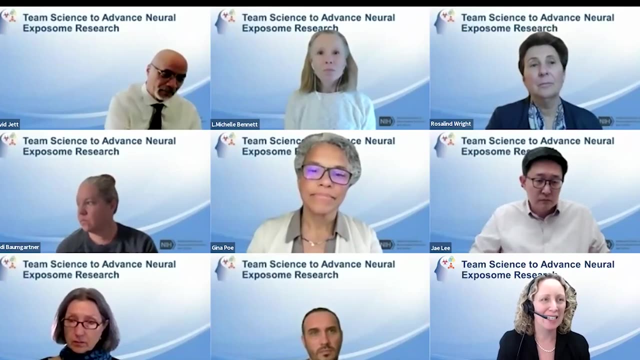 with adverse exposomal exposures is profound, And of course we could come up with examples in Native American communities, rural communities and others as well. But I do think that the power of the community to bring resources to the table is really profound, And it's been my experience. 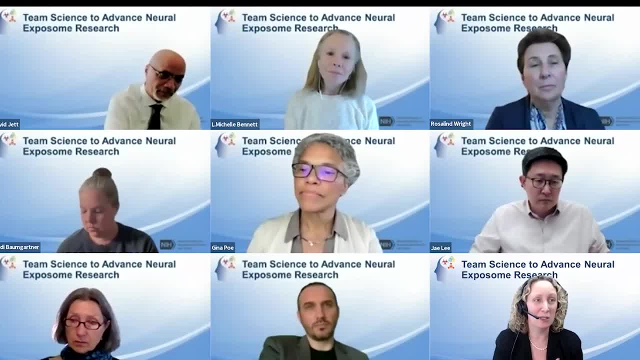 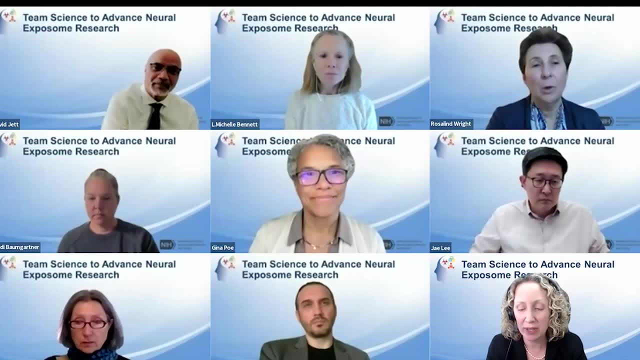 I get very, very excited around many of these issues because it touches them so deeply in the health of their children and themselves over their life course. So, yeah, I do think that it's a, it would be a wonderful area of study. but again, 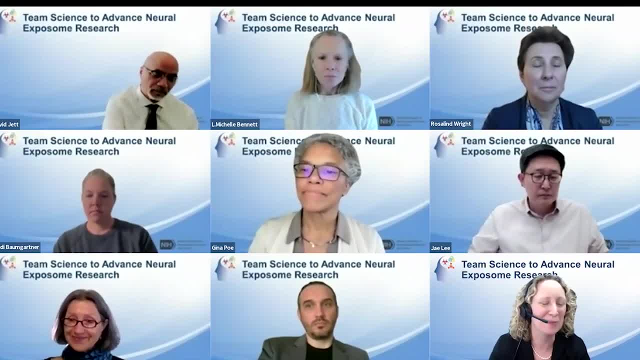 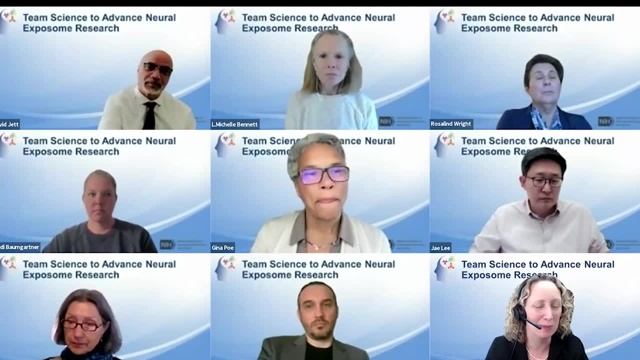 it would require multidisciplinarity. We'd have to think about nimbleness. We'd have to think about pragmatic issues that sometimes make research a little bit messy, but a whole lot of excitement and fun, of course. I love it. 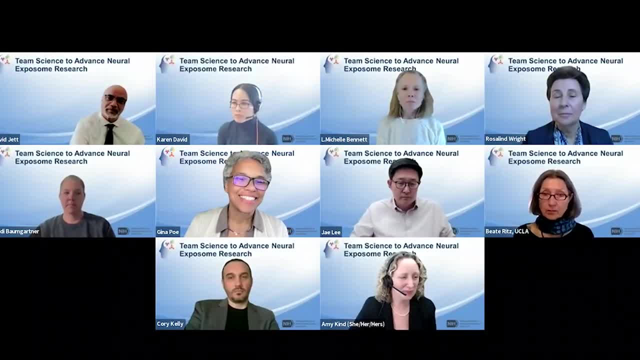 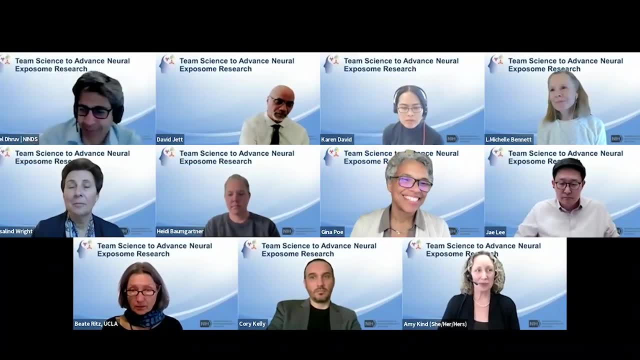 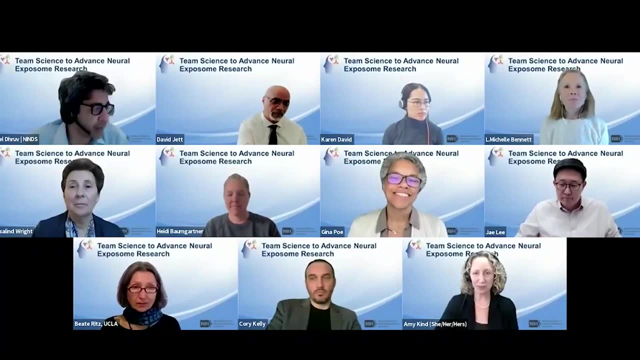 Neil, are we getting to be about the time where we need to wrap up? Yeah, I was just checking the clock, So we're now at time. I'd like to. I'd like to thank everyone for their participation and for coming to this workshop. 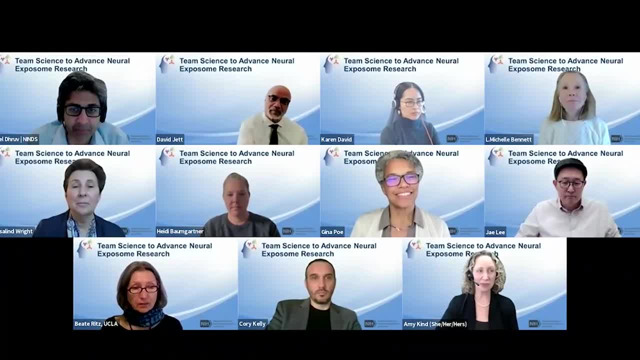 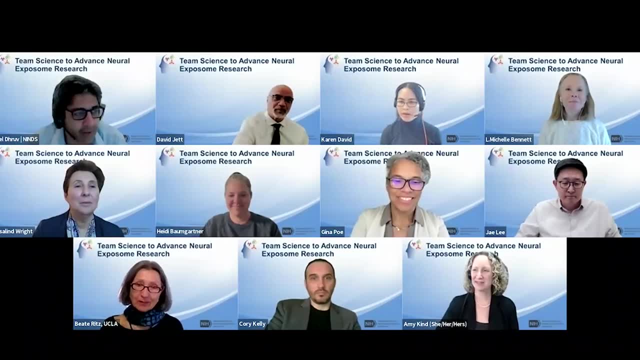 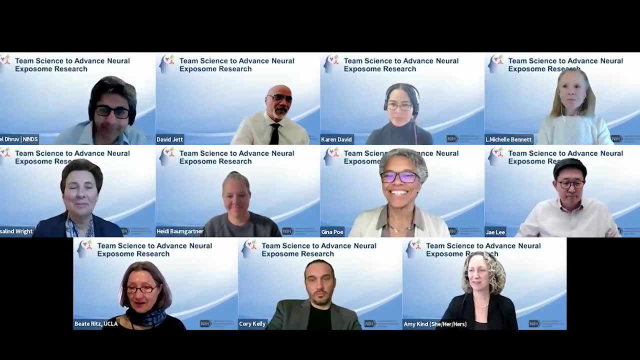 It was fascinating and I learned a lot. I hope that all of you did too. Thank you know. thank you to everyone. Thank you for working. What's that? Oh, Amazing, right? Yes, Thank you guys. This was absolutely fantastic. 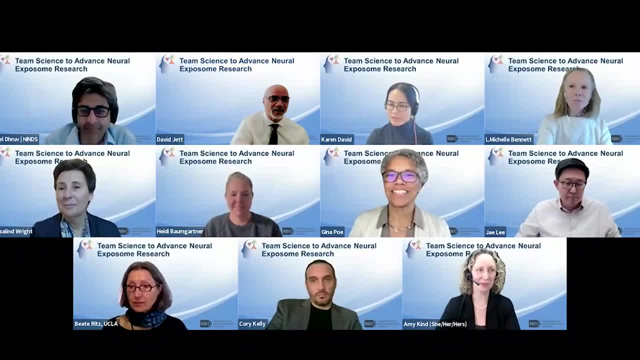 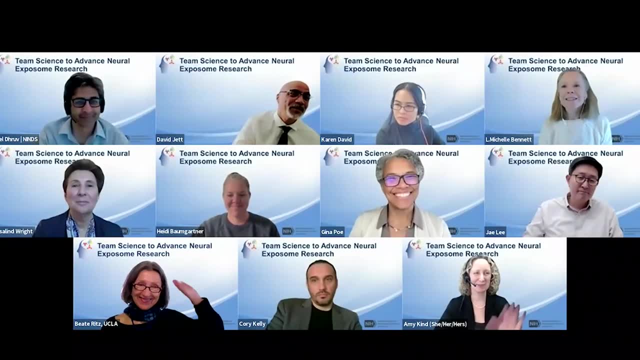 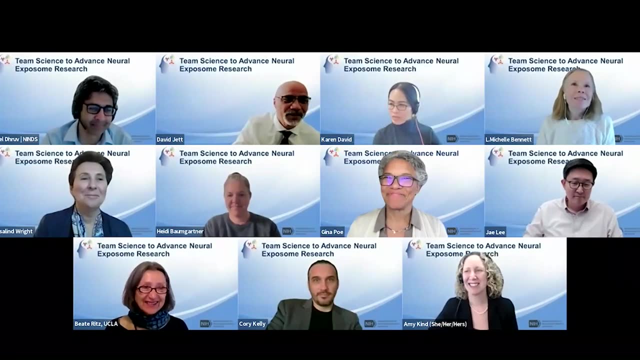 I can't tell you how helpful this is going to be for our office, and please come back. Thank you for having us. Thank you, Gina. Thank you, Thank you, Gina, for the real help with this. I have about five more questions. 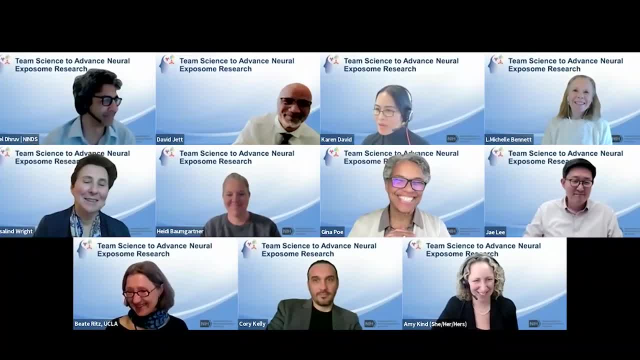 but I'm not going to do that. All right, Thanks everybody, Thanks all, Yeah, Terrific.